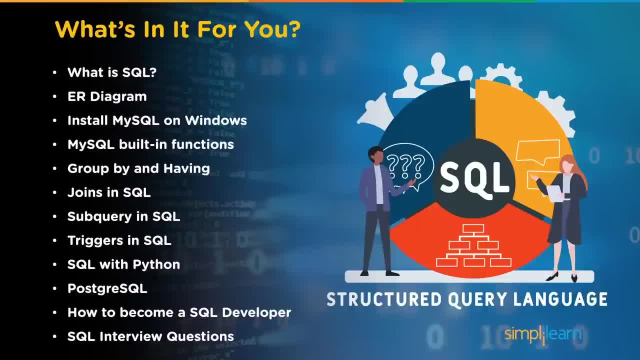 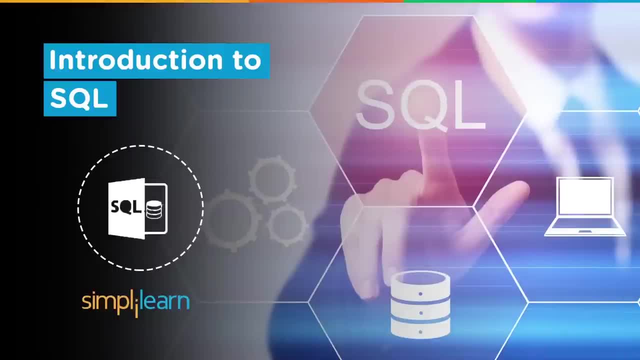 developer and see the top SQL interview questions that are frequently asked in the interviews. So let's get started with what is SQL? In this session we are going to learn about databases, how data is stored in relational databases, and we will also look at some of 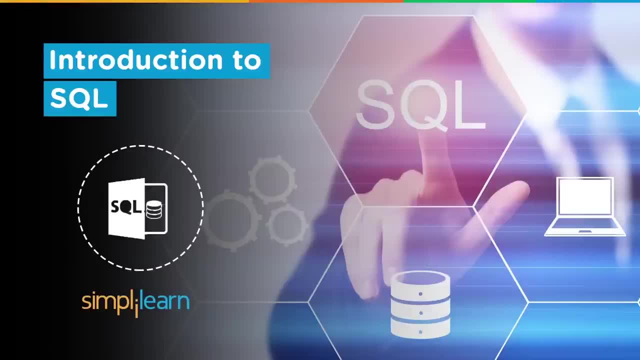 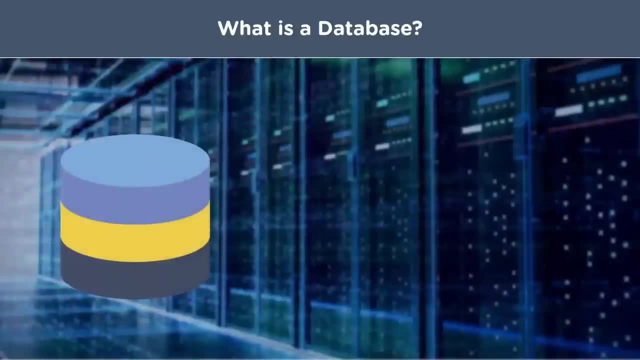 the popular databases. Finally, we will understand various SQL commands on MySQL Server. Now let's get started. 1. What is a database? 2. What is a database? According to Oracle, a database is an organized collection of structured information or data. 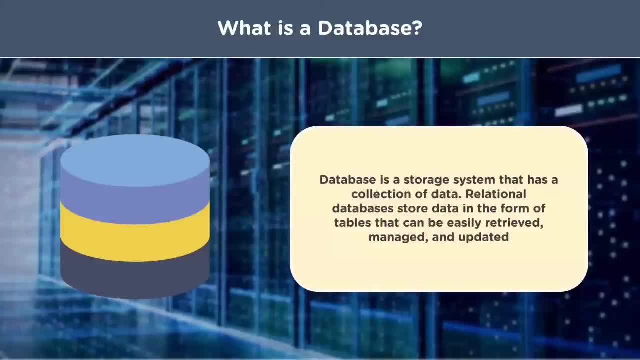 that is typically stored electronically in a computer system. A database is usually controlled by a database management system or DBMS, So it is a storage system that has a collection of data. Relational databases store data in the form of tables that can be easily retrieved, managed and updated. You can organize data. 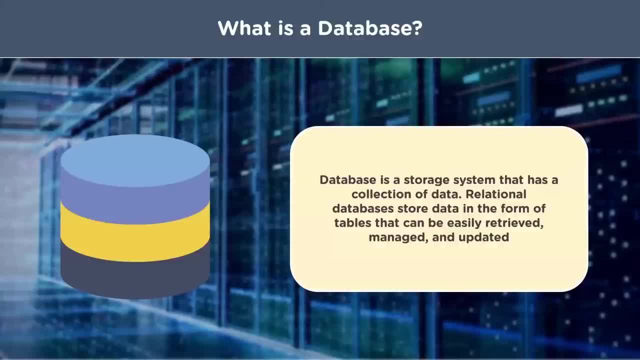 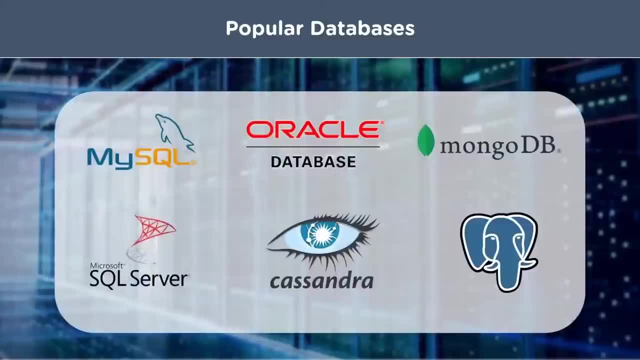 into tables, rows, columns and even fields 2. columns and index it to make it easier to find relevant information. now, talking about some of the popular databases, we have mysql database. we also have oracle database. then we have mongodb, which is a no sql database. next we have microsoft sql server. next we have apache cassandra, which is 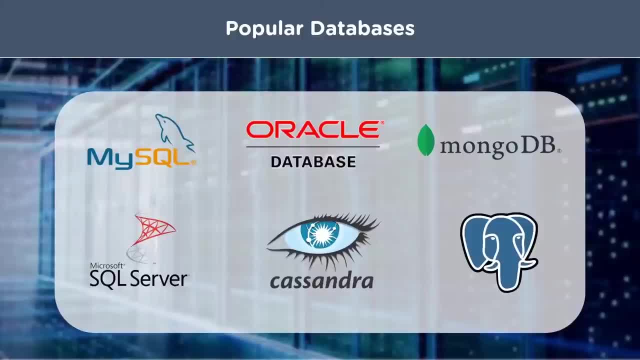 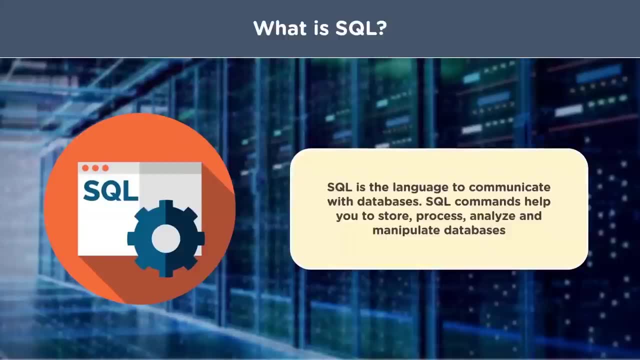 a free and open source. no sql database and finally we have postgres sql. now let's learn what is sql. so sql is a domain specific language to communicate with databases. sql was initially developed by ibm. most databases use structured query language, or sql, for writing and querying. 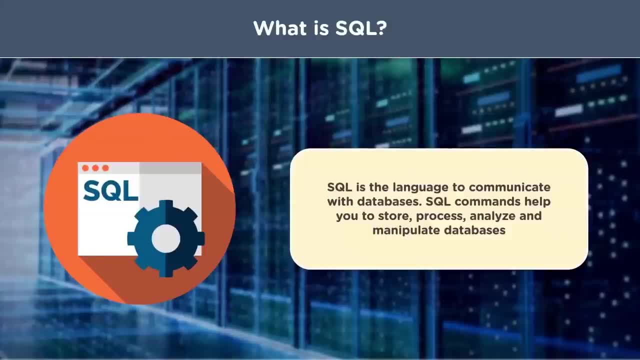 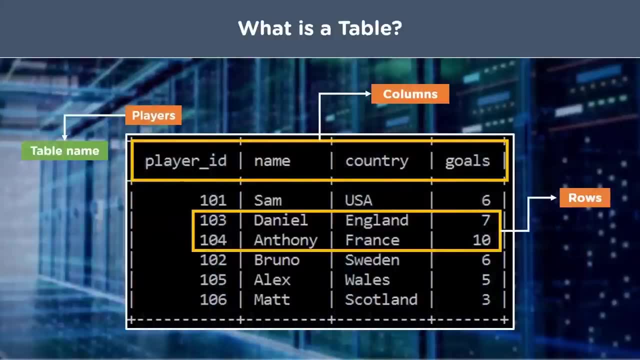 data sql commands help you to store, process, analyze and manipulate databases. with this, let's look at what a table is. so this is how a table in a database looks like. so here you can see the name of the table is players. on the top you can see the column names. so we have the player id, the player name, the country to. 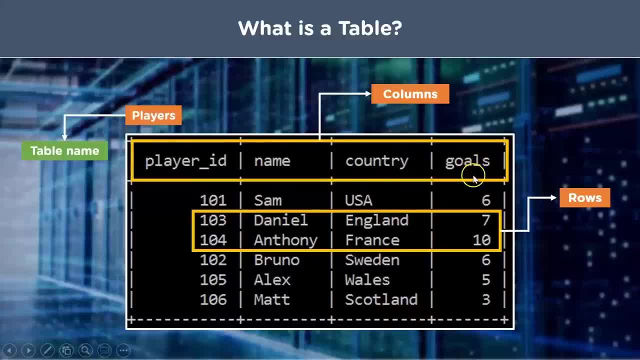 which the player belongs to, and we also have the goals scored by each of the players, so these are also known as fields in a database. here each row represents a record or a tuple. so you have the player id, which is 103 here. the name of the player is daniel, he is from england, and the number of 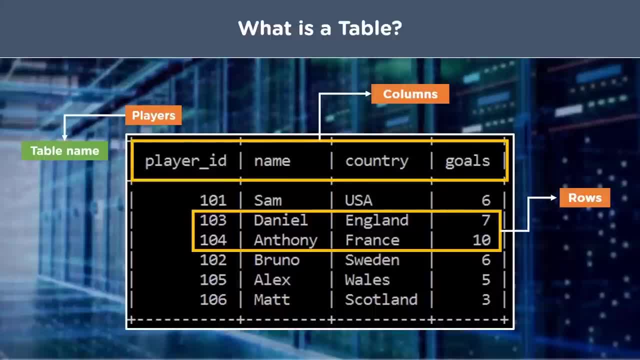 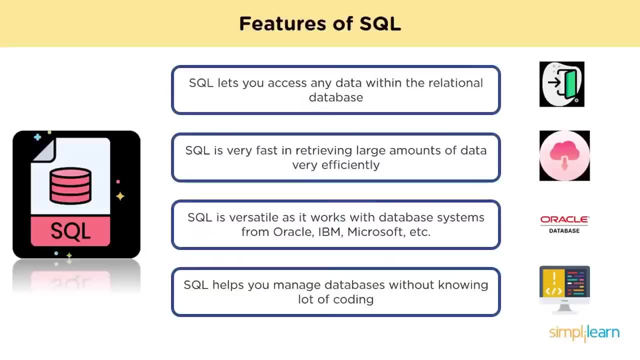 goals he has scored is seven, so you can use sql to find the number of goals he has scored in a database. so sql commands to query, update, insert records and do a lot of other tasks. now we'll see what the features of sql are. sql lets you access any information stored. 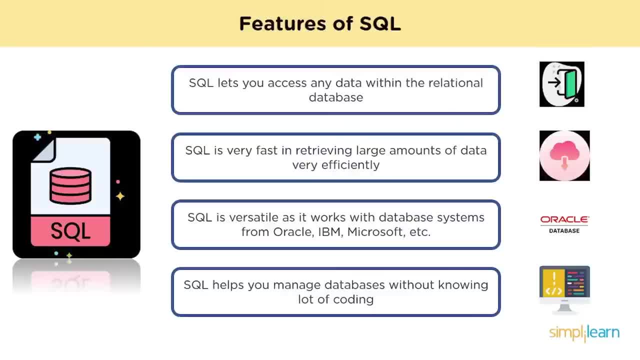 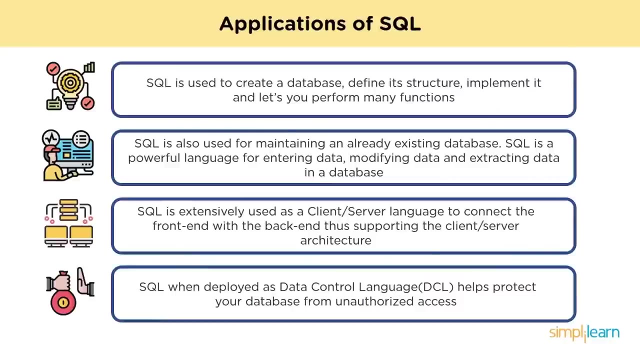 in a relational database. with sql queries, data is extracted from the database in a very efficient way. the structured query language is compatible with all database systems, from oracle, ibm to microsoft, and it doesn't require much coding to manage databases. now we will. applications of SQL. SQL is used to create a database, define its structure. 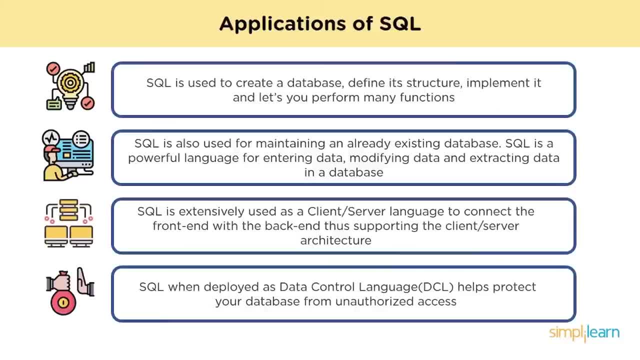 implement it and lets you perform many functions. SQL is also used for maintaining an already existing database. SQL is a powerful language for entering data, modifying data and extracting data in a database. SQL is extensively used as a client-server language to connect the front-end with the back-end. thus, 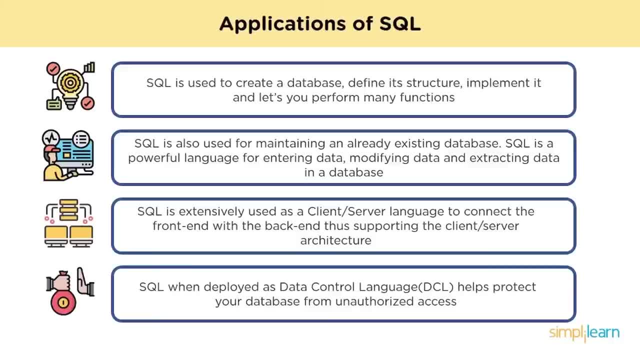 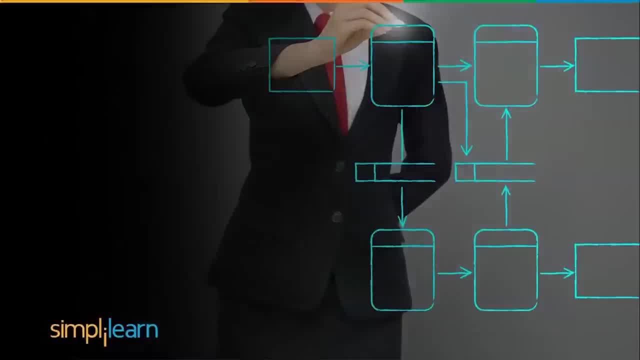 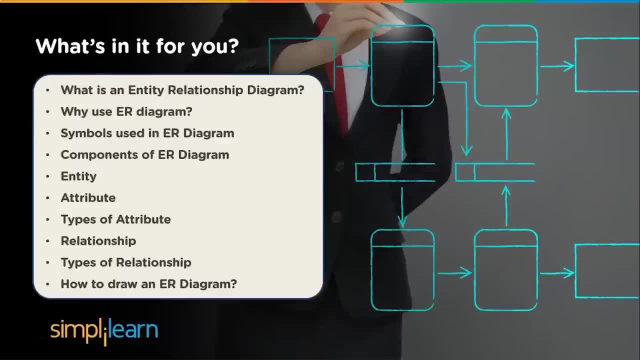 supporting the client-server architecture SQL. when deployed as data control language, DCL helps protect your database from unauthorized access. In this session we will learn about the Year Diagram, starting with what is an Year Diagram and why it's been so much used by the companies. Then we will learn about the 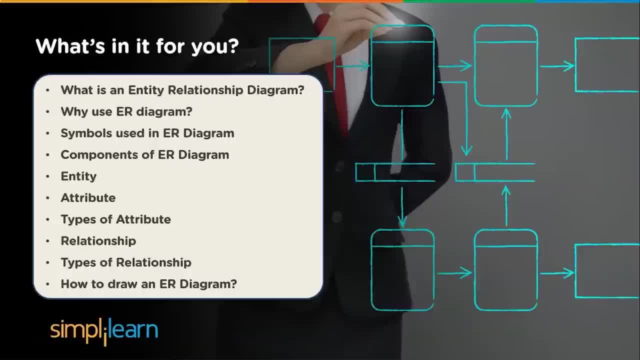 symbols used in the Year Diagram and get familiar with the components of it. So, hey everyone, I am Abhisar Aujar from Simply Learn, and welcome to this video about the Year Diagram. But before we begin, if you love watching tech videos, subscribe to our channel and 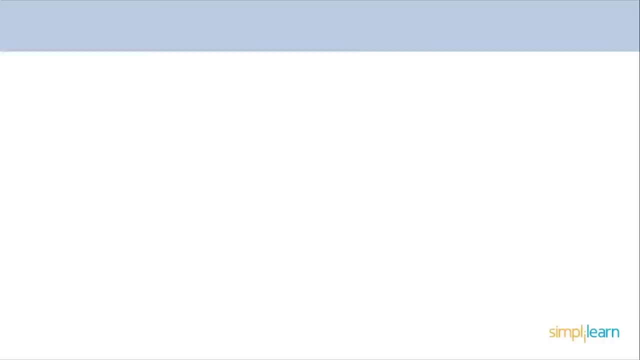 hit the bell icon to never miss an update. Let's start. Have you ever wondered how these big e-commerce companies manage their tons of data that keeps updating every second And these datasets keep on updating in their databases To perform operations on this data. 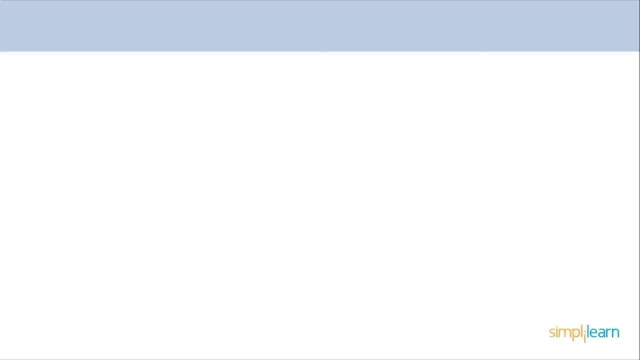 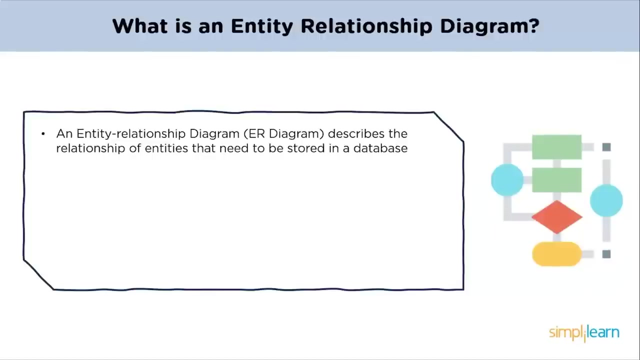 they should have a conceptual understanding of these databases And this is done by understanding Year Diagrams of the database. So let's understand what an Year Diagram is. An Entity Relationship Diagram describes the relationship of entities that needs to be stored in a database. Year Diagram is mainly a structural design for the database. It is 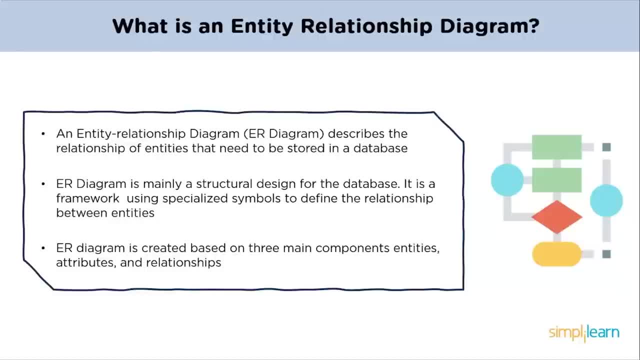 a framework made using specialized symbols to define the relationship between entities. Year Diagrams are created based on the three main components: entities, attributes and relationships. Let's understand the use of Year Diagrams. Let's learn the use of Year Diagrams with a help of a real-world example Here. 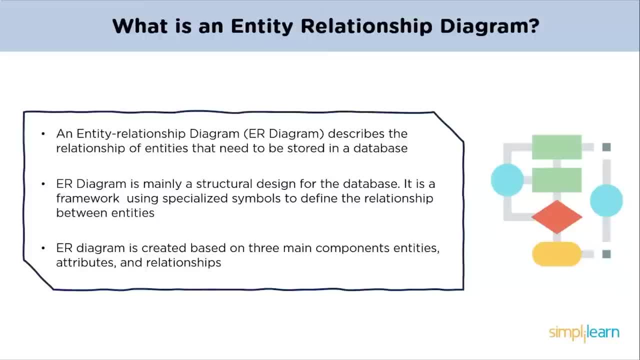 a school needs all its student records to be stored digitally, So they approach an IT company to do so. A person from the company will meet the school authorities, note all their requirements, describe them in the form of Year Diagram and get it cross checked. 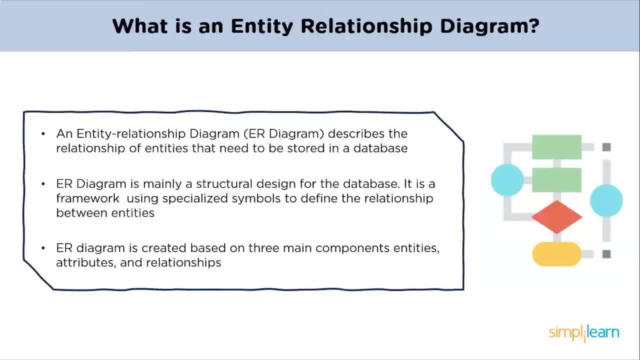 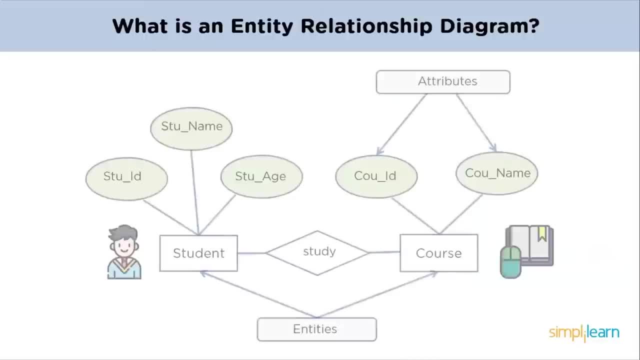 by the school authorities. As the school authorities approve the Year Diagram, the database engineers would carry further implementation. Let's have a view view of an year diagram. The following diagram showcases two entities, student and course, and their relationship. The relationship described between student and course is many to many as a course can. 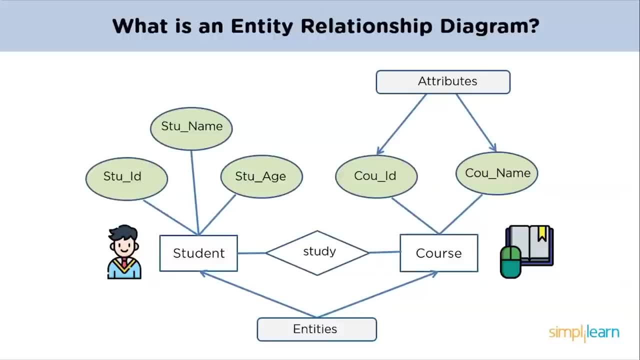 be opted by several students, and a student can opt for more than one course. Here, student is the entity and it possesses the attributes, ie student id, student name and student age, and the course entity has attributes such as course id and course name. 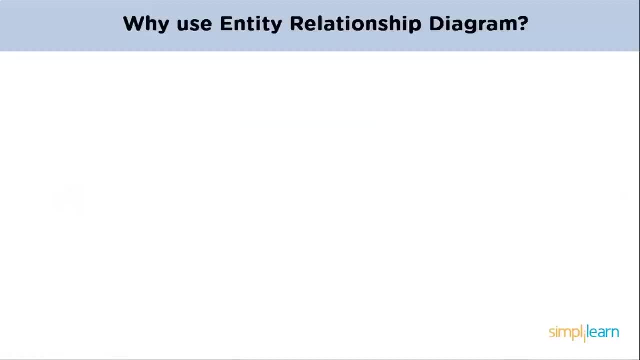 Now we have an understanding of year diagram. Let us see why it has been so popular. The logical structure of a database provided by year diagram communicates the landscape of business to different teams in the company, which is eventually needed to support the business. 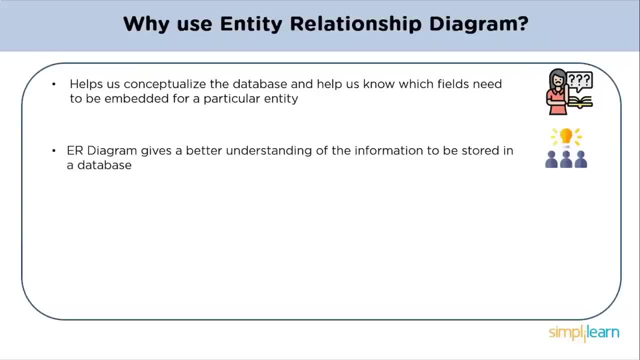 Year diagram is a GUI representation of the logical structure of a database which gives a better understanding of the business of the information to be stored in a database. Database designers can use ER diagrams as a blueprint, which reduces complexity and helps them save time to build databases quickly. 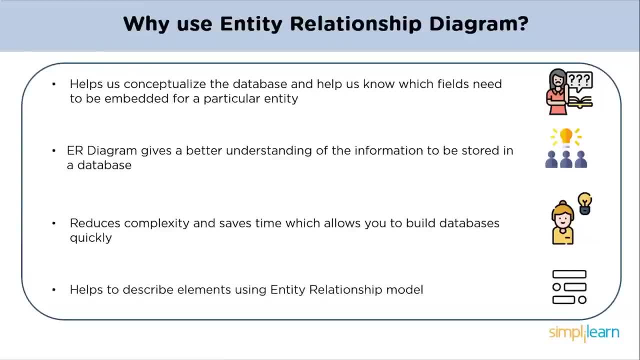 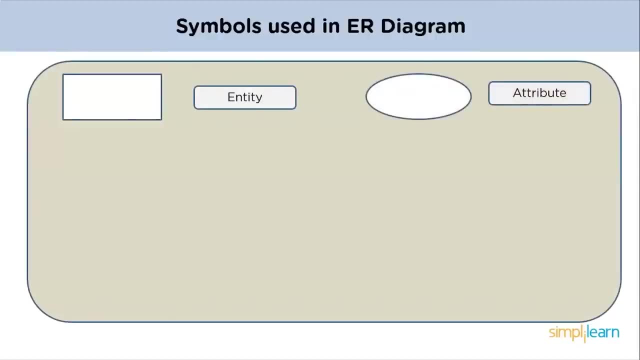 ER diagrams helps you identify the entities that exist in a system and the relationships between those entities. After knowing its uses, now we should get familiar with the symbols used in ER diagram. The rectangle symbol represents the entities. oval symbol represents attributes. a rectangle. 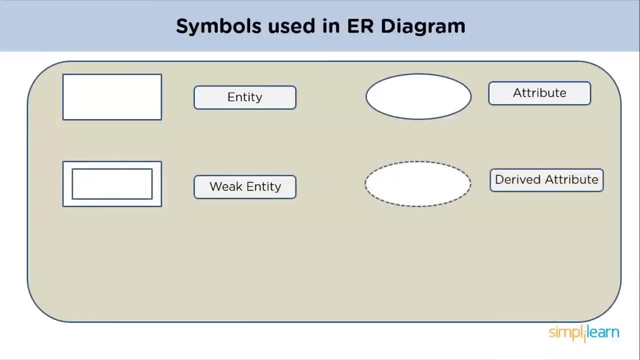 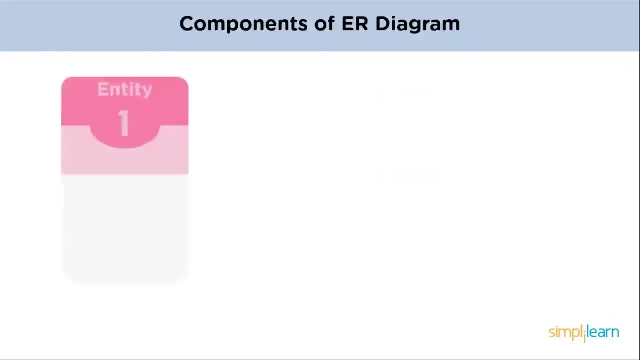 embedded in a rectangle represents a weak entity. a dashed oval represents a derived attribute. a diamond symbol represents a relationship among entities. double oval symbol represents multi-valued attributes. Now we should dive in and learn about the components of ER diagram. There are three main components of ER diagram: entity, attribute and relationship. 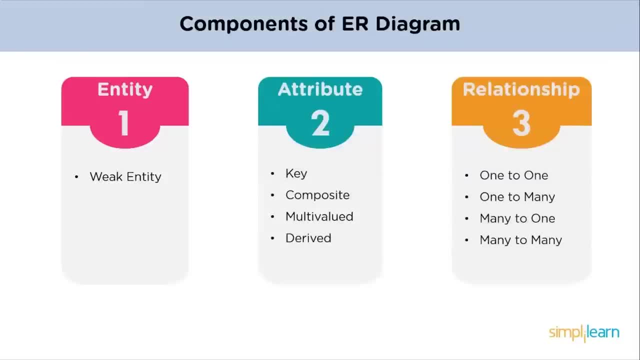 Entities have weak entity attributes are further classified into key attribute, composite attribute, multi-valued attribute and derived attribute. Relationships are also classified into one-to-one relationships, one-to-many relationships, many-to-one relationships and many-to-many relationships. Let's understand these components of ER diagram. 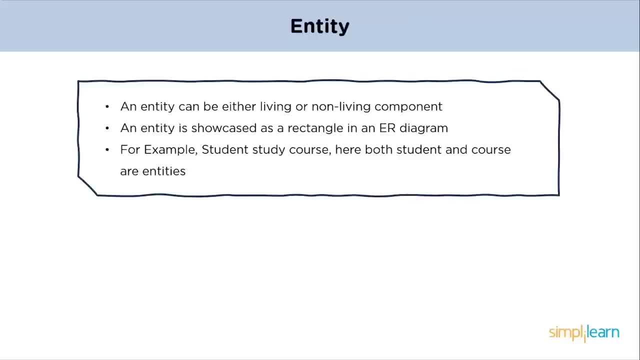 Starting with entities. an entity can be either a living or a non-living component. An entity is short for a living or a non-living component. An entity is another way of calling entity and should be Own or owned or owned. that has different αλλάist properties. 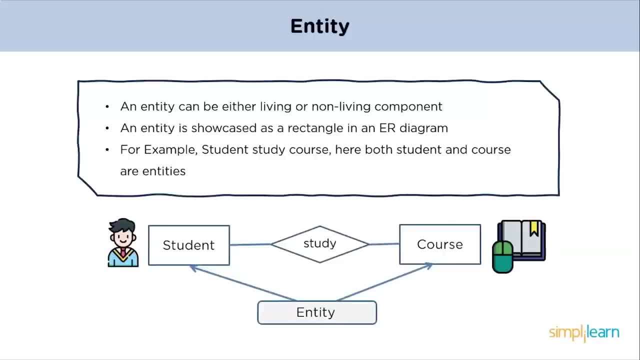 Let us explain our common khác to see how entities can be classified. they can be a site, as an entity, or或者 a location. we would give an example or an API, and will be called an entity, and we will call it an active till reform it. 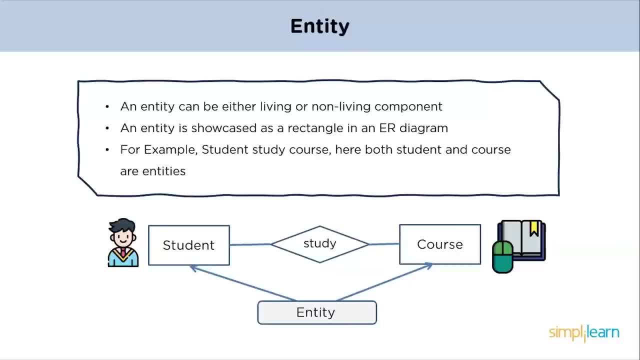 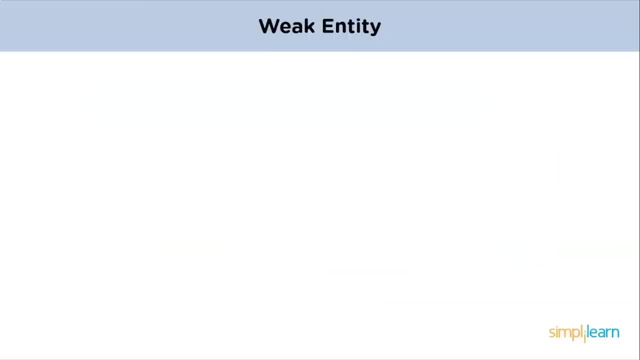 Entities can be called entities and also their identity does not log exactly to. we can call an entity Things which can be called as entities, can be called categories, they can be called一些 moving objects or they can be called other kinds of activity or, as breadth, opportunities, numeral. 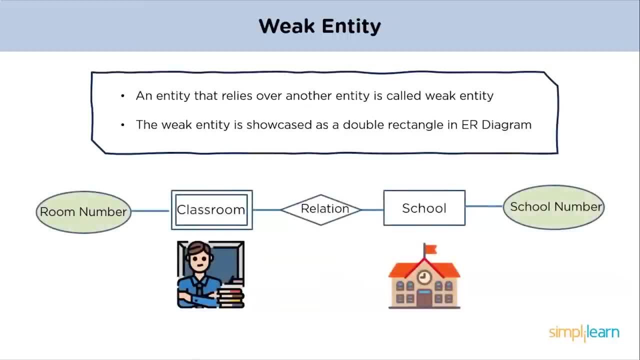 objects which can be called from within that physical forms of it, like space. space object Textiles can often be called entities, Greater cartoons and programs or objects that you can call interface initiatives and nations. Hello, the school is a strong entity because it has a primary key attribute: school number. 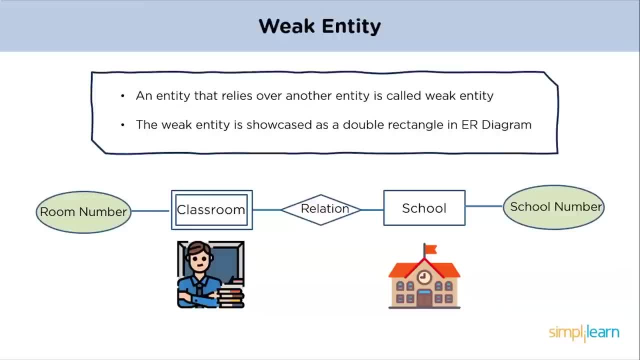 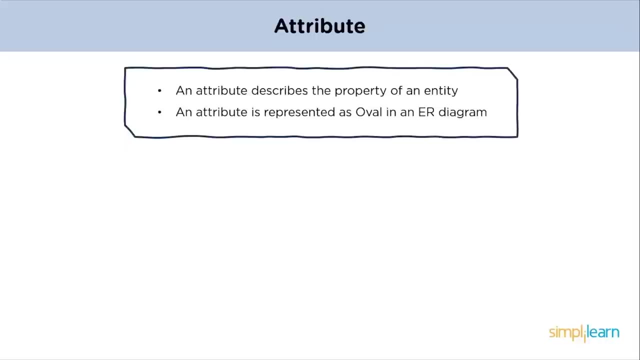 Unlike the school, the classroom is a weak entity because it does not have any primary key and the room number attribute here acts only as a discriminator and not a primary key. Now let us know about attributes. Attribute- An attribute, exhibits the properties of an entity. 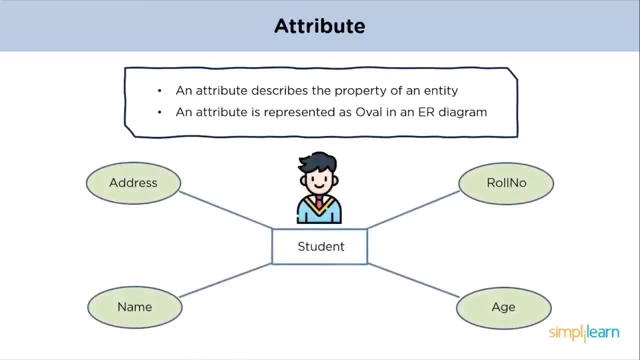 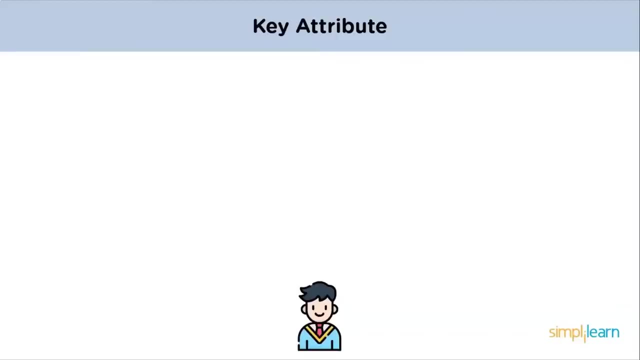 An attribute is illustrated with an oval shape in an ER diagram. In the example below, student is an entity and the properties of student, such as address, age, name and room number, are called its attributes. Let us see our first classification under attribute ie- key attribute. 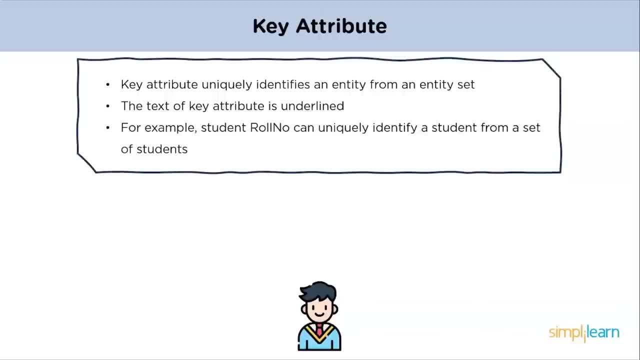 The key attribute uniquely identifies an entity from an entity set. The text of a key attribute is underlined In the example below. we have a student entity and it has attributes- name, address, room number and age- But here room number can uniquely identify a student from a set of students. 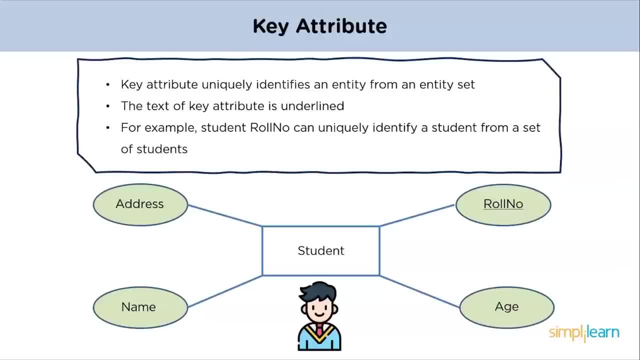 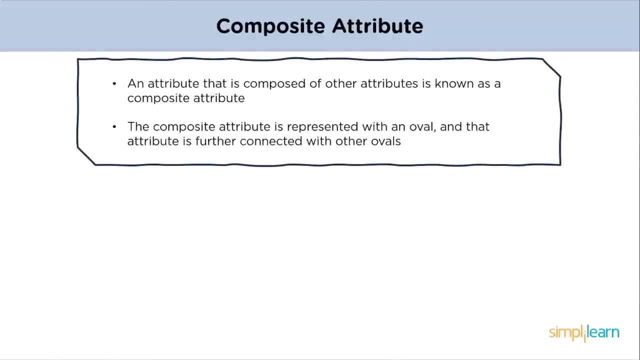 That's why it is termed as a key attribute. Now we will see composite attribute. An attribute that is composed of several other attributes is known as a composite attribute. An oval showcases the composite attribute and the composite attribute oval is further connected with other ovals. 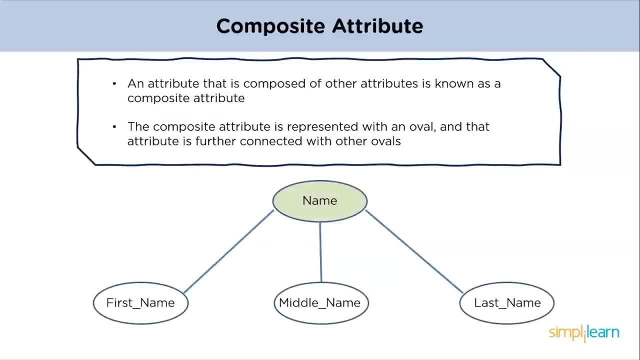 In the example below we can see an attribute Name which can have further subparts, such as first name, middle name and last name. These attributes with further classification is known as composite attribute. Now let's have a look at multi-valued attribute. 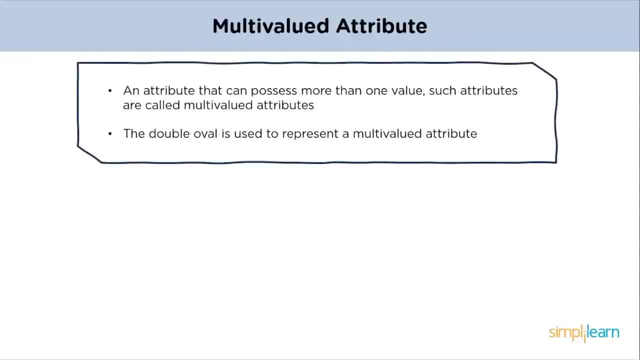 An attribute that can possess more than one value are called multi-valued attributes. These are represented as double oval shape In the example below. the student entity has attributes phone number, role, number, name and age. Out of these attributes, phone number can have more than one entry and the attribute 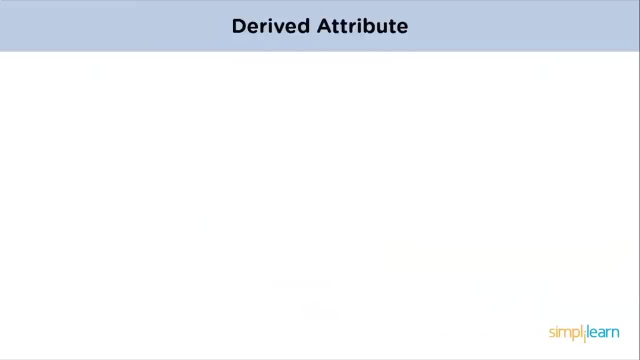 with more than one value is called multi-valued attribute. Let's see derived attribute. An attribute that can be derived from other attributes of the entity is known as a derived attribute. In the year diagram, the derived attribute is represented by dashed oval. 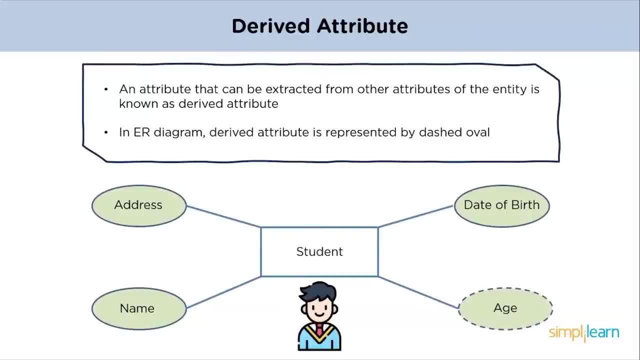 And in the example below, student entity has both date of birth and age as attributes. Here, student entity has both date of birth and age as attributes. Age is a derived attribute, as it can be derived by subtracting current date from the student date of birth. 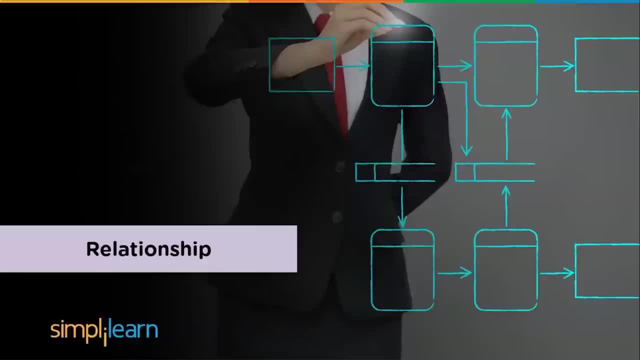 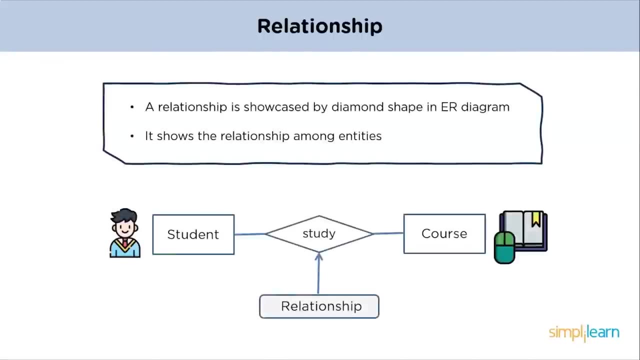 Now, after knowing attributes, let's understand relationship in year diagram. A relationship is showcased by the diamond shape in the year diagram. It depicts the relationship between two entities In the below example: student, study course. Here both student and course are entities and study is the relationship between them. 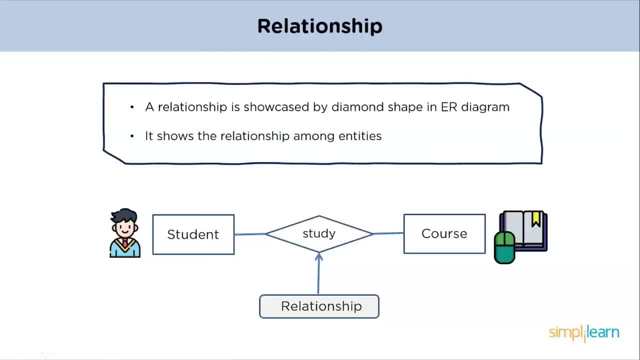 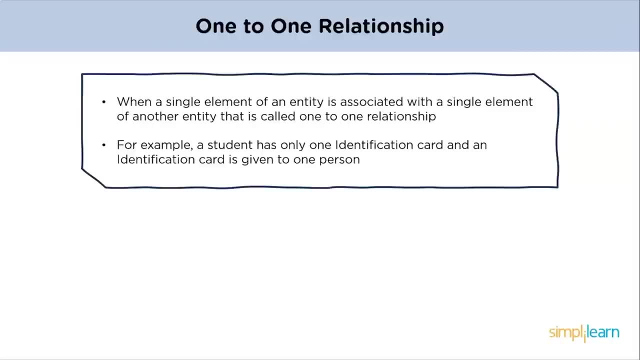 Now let's go further. Now let's go through the type of relationship. First is one-to-one relationship: When a single element of an entity is associated with a single element of another entity. This is called one-to-one relationship. In the example below, we have student and identification card as entities. 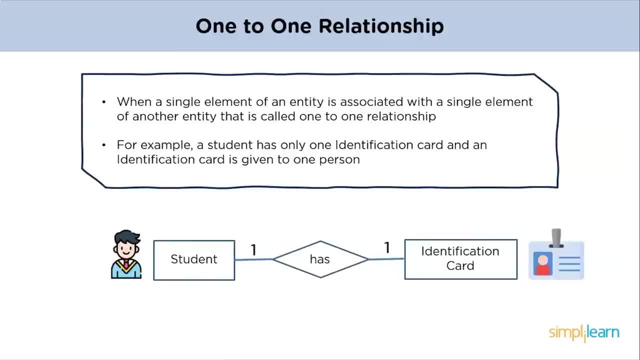 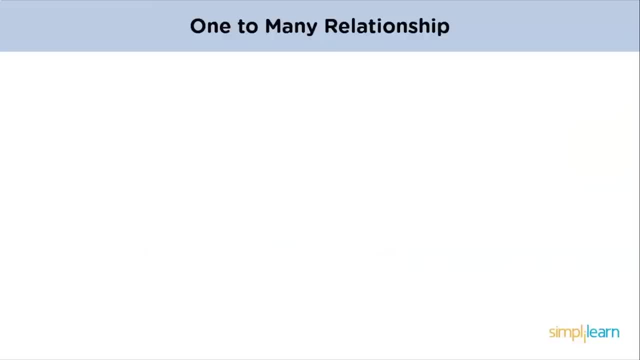 We can see, a student has only one identification card and an identification card is given to one student. It represents a one-to-one relationship. Let's see the second one: One-to-many relationship When a single element of an entity is associated with more than one element of another entity. 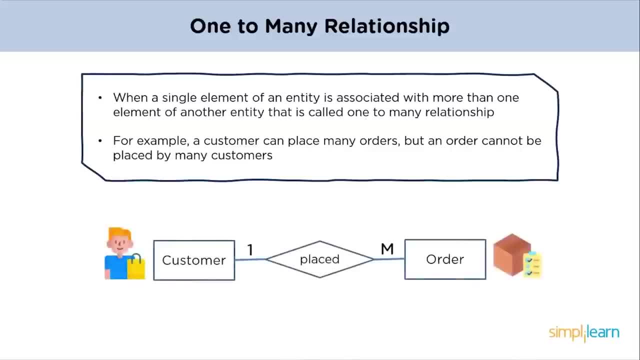 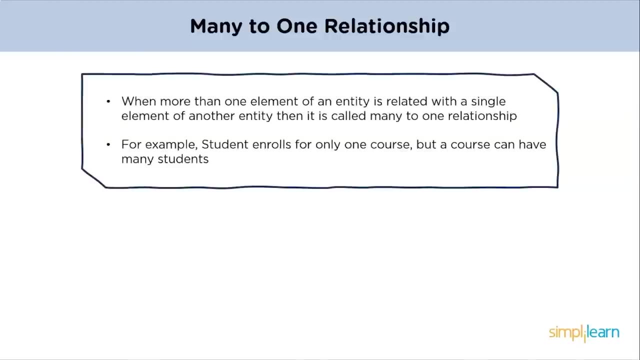 is called one-to-many relationship. In the below example, a customer can place many orders, But a particular order cannot be placed by many customers. Now we will have a look at many to-one relationship When more than one element of an entity is related to a single element of another entity. 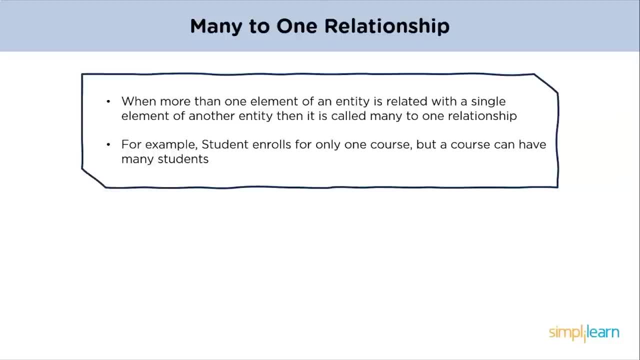 it is called many-to-many relationship. Next is a single-manied relationship- See example below- to one relationship. For example, students have to opt for a single course, but a course can be opted by number of students. Let's see many to many relationship When more than one element 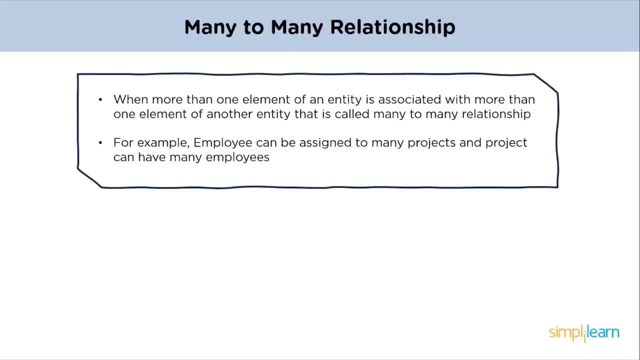 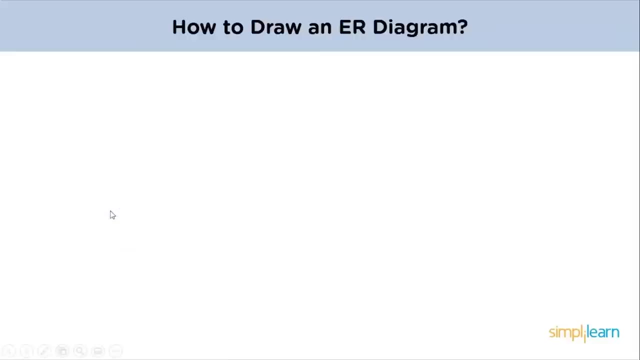 of an entity is associated with more than one element of another entity is called many to many relationship. For example, an employee can be assigned to many projects and many employees can be assigned to a particular project. Now, after having an understanding of VR diagram, 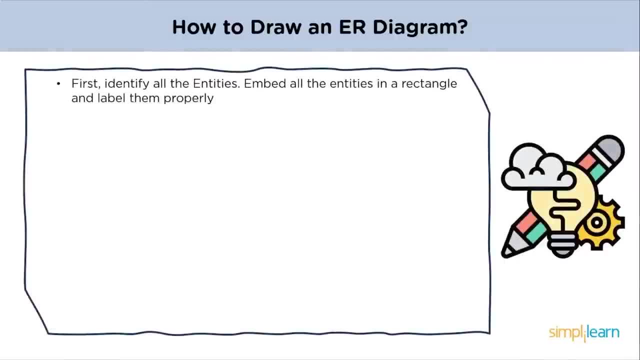 let us know the points to keep in mind while creating the VR diagram. First, identify all the entities in the system. Embed all the entities in a rectangular shape and label them appropriately. This could be a customer, a manager, an order, an invoice, a schedule, etc. Identify relationships. 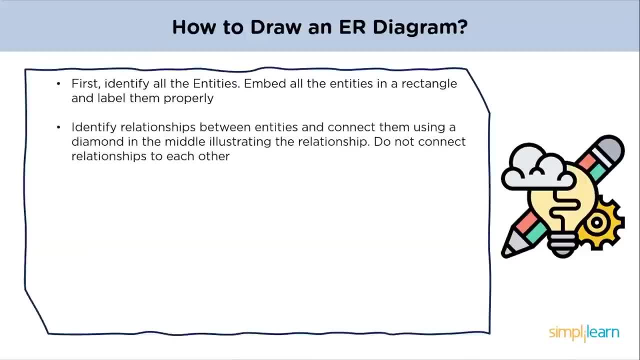 between entities and connect them using a diamond in the middle illustrating the relationship. Do not connect relationships. Connect attributes with entities and label them appropriately, and the attribute should be in oval shape. Assure that each entity only appears a single time and eradicate any redundant entities or relationships in the VR diagram. Make sure your VR diagram supports 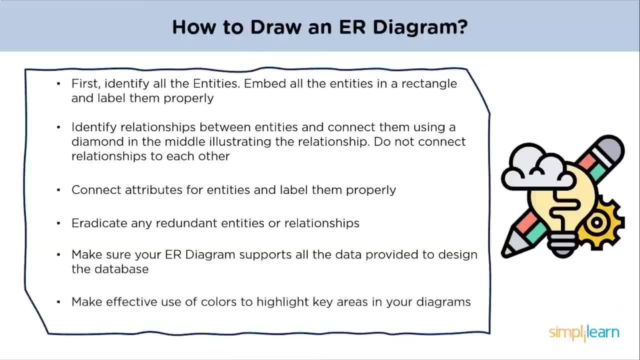 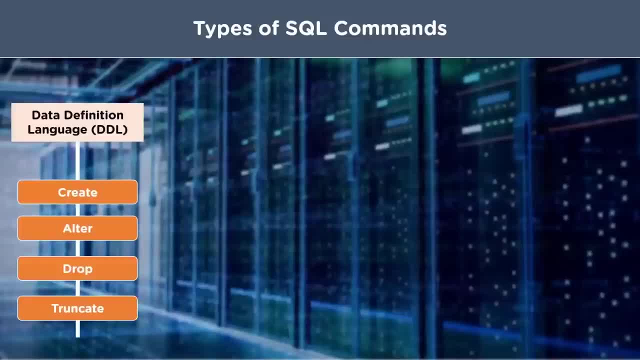 all the data provided to design the database. Make effective use of colors to highlight key areas in your diagrams. There are mainly four types of SQL commands. So first we have data definition language, Data definition language or DDL. So DDL commands change the structure of the table, like creating. 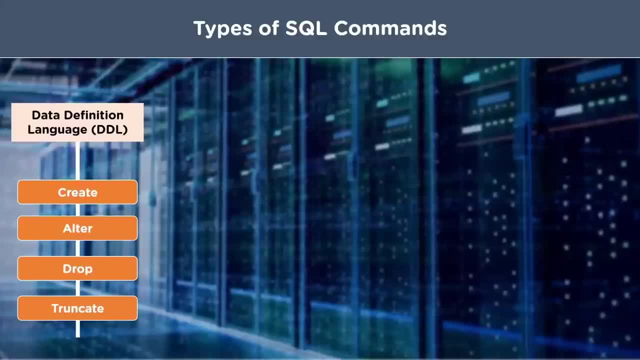 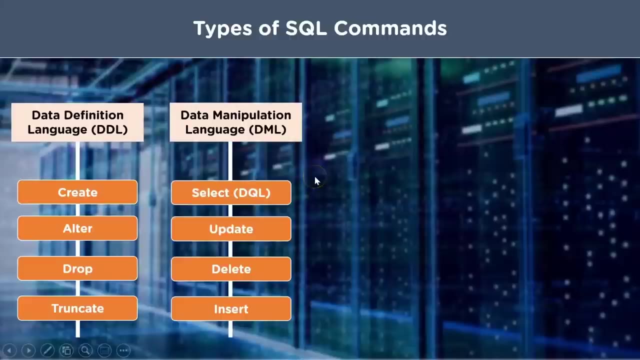 a table, deleting a table or altering a table. All the commands of DDL are auto committed, which means it permanently save all the changes in the database. We have create, alter, drop and truncate as DDL commands. Next we have data manipulation language or DML, So DML. 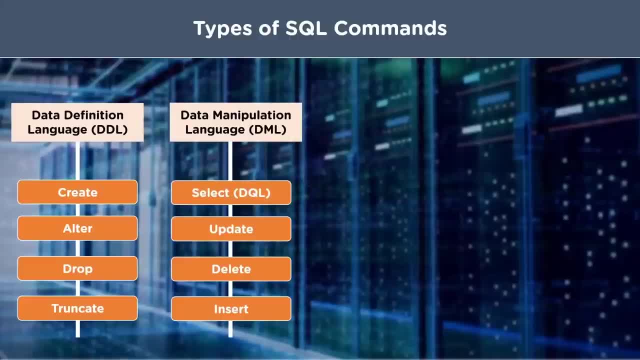 commands are used to modify a database. It is responsible for all forms of changes in the database. DML commands are not auto committed, which means it can't permanently save all the changes in the database. We have select, update, delete and insert as DML commands. Now select command. 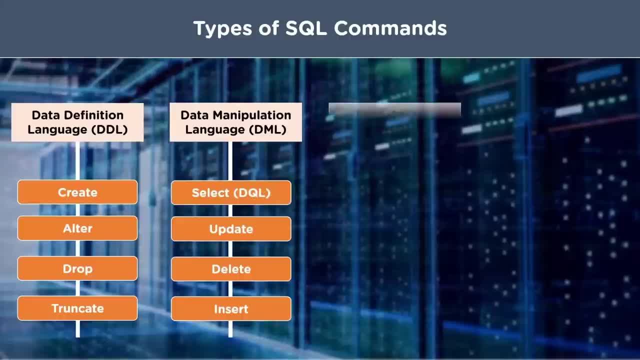 is also referred to as DQL or data query language. Third, we have data control language, or DCL, So DCL commands allow you to control access to data within the database. These DCL commands are normally used to create objects related to user access and also control the distribution. 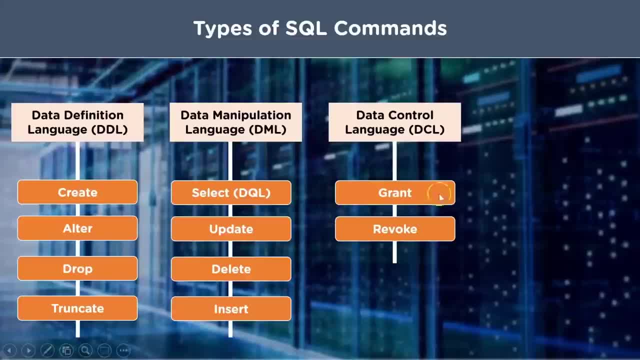 of privileges among users. So these commands are normally used to create objects related to user access and also control the distribution of privileges among users. So we have grant and revoke, which are the examples of data control language. Finally, we have something called as transaction control language or TCL, So TCL commands allow the user to manage. 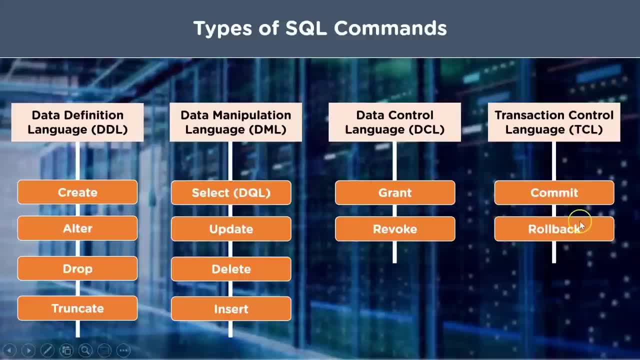 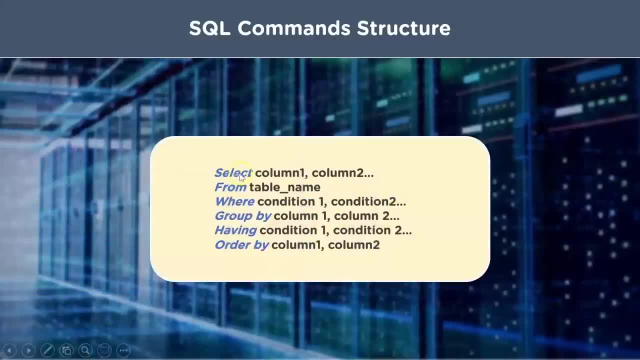 database transactions. Commit and rollback are example of TCL. Now let's see the basic SQL command structure. So first we have the select statement. So here you specify the various column names that you want to fetch from the table. We write the table name using the FROM statement. Next we have the WHERE clause to filter out. 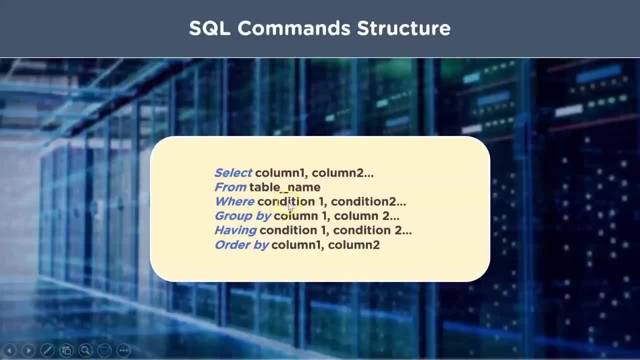 a table based on some conditions. So here you can see WHERE condition 1, CONDITION 2 & so on. Then we have the GROUP BY clause that takes various column names, So you can write GROUP by column 1, column 2 & so on. Next we have the HAVING clause is to filter. 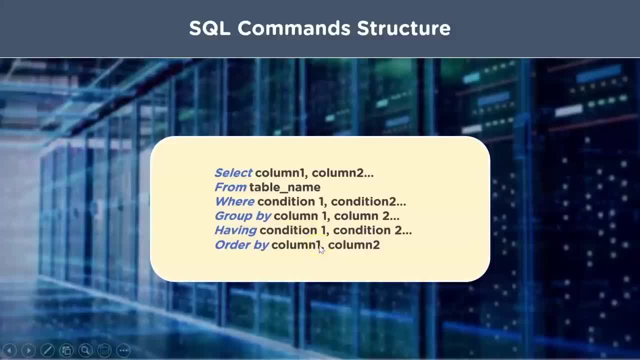 out tables based on groups. Finally, we have the ORDER BY clause to filter out the result in ascending or descending order. Now we have taken down ACUM gel easily from table using this不行 dessever method of first question. we have to yılif, according to the toujours of ES ultimate goal. we can undervalue 3's. 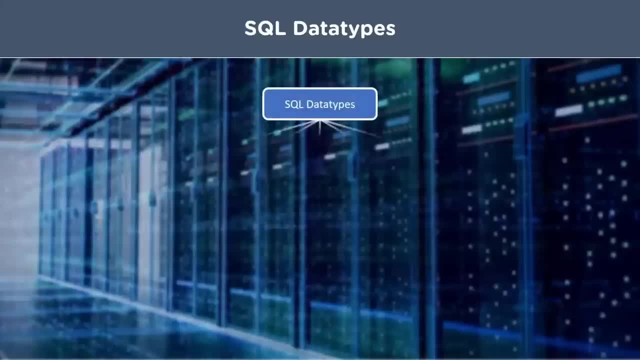 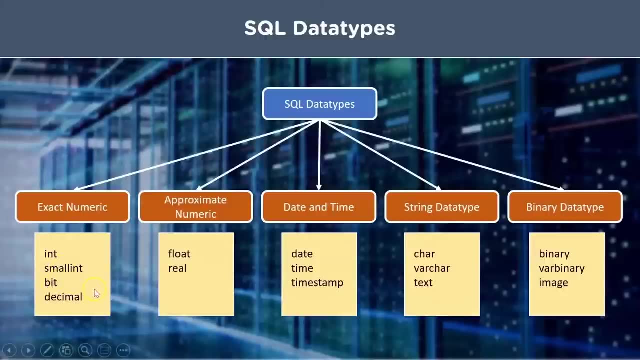 Now talking about the various data types in SQL. So we have Exact Numeric, which has Integer, Small Int, Bit and Decimal. Then we have Approximate Numeric, which are Float and Real. Then we have some Date and Time data types, such as Date, Time, Timestamp and others. 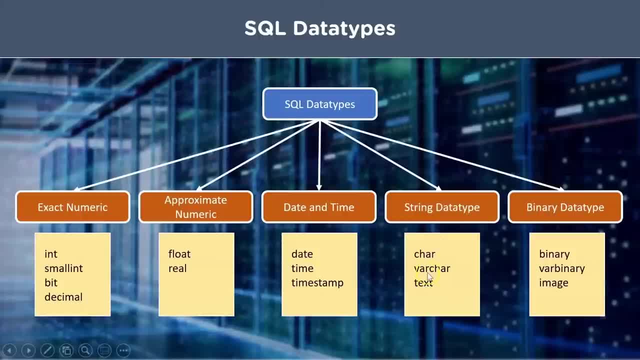 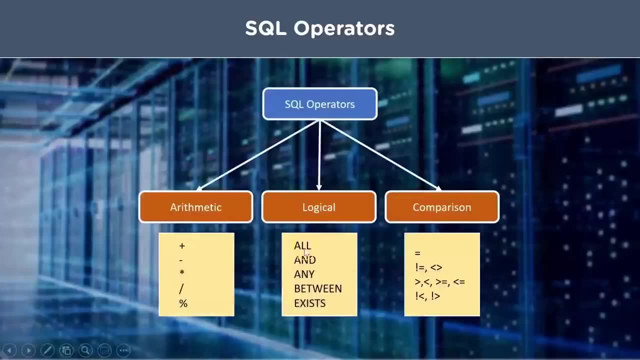 Then we have String data type, which includes Car- this is Work Car and Text. Finally, we have Binary data types, and Binary data types have Binary, Var, Binary and Image. Now let's see some of the various operators that are present in SQL. So first we have our basic arithmetic operators. 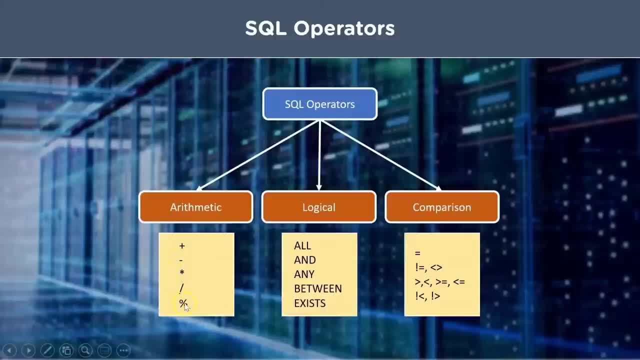 so you have Addition, Subtraction, Multiplication, Division and Modulus. Then we have some Logical operators like All And Any Or Between, Exists, and so on. Finally, we have some Comparison operators such as Equal to Not equal to. There is Greater than Less than Greater than Equal to. 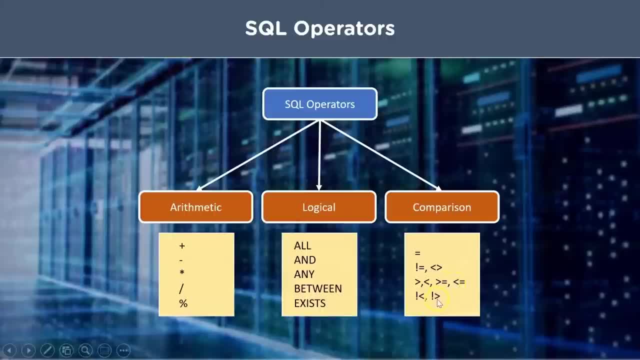 or Less than, equal to, Not less than or Not greater than. Now let me take you to my MySQL Workbench, where we will learn to write some of the important SQL commands, use different statements, functions, data types and operators that we just learned In this session. 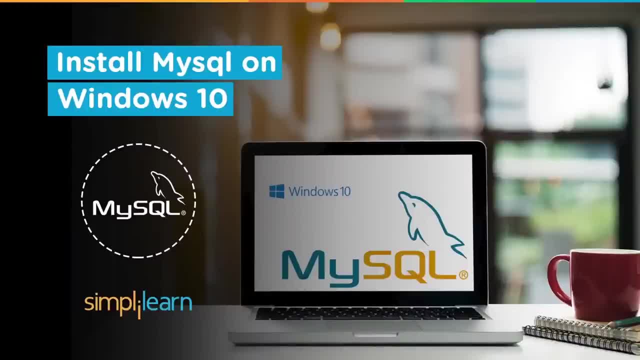 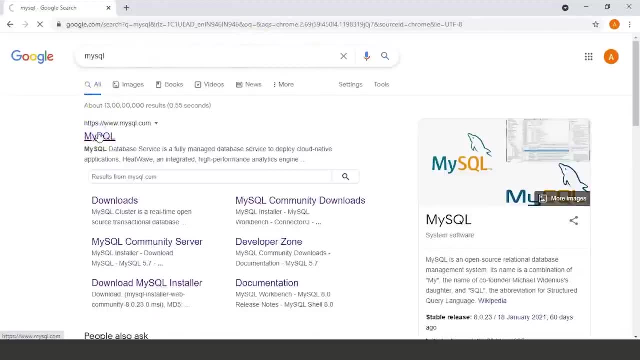 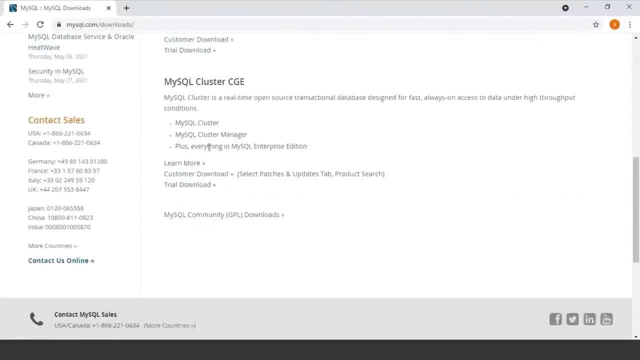 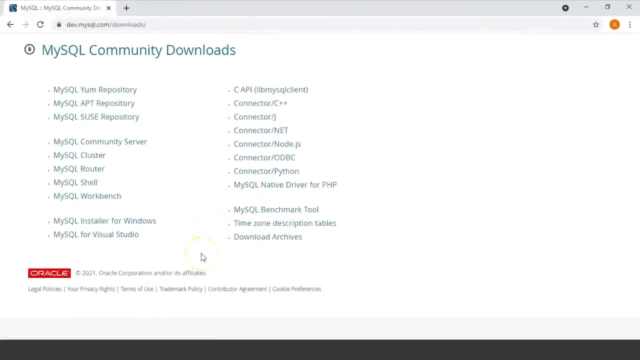 we will learn how to install MySQL Workbench and then we will run some commands. Firstly, we will visit the official Oracle website, that is mysqlcom, and now we will move to the Downloads page. Now scroll down and click on MySQL GPL Downloads. Now, under Community Downloads, click on MySQL Installer for Windows. 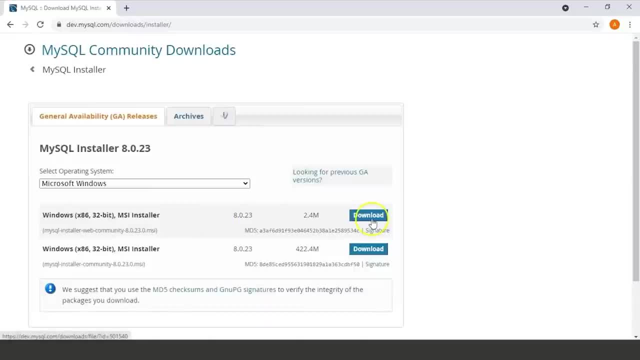 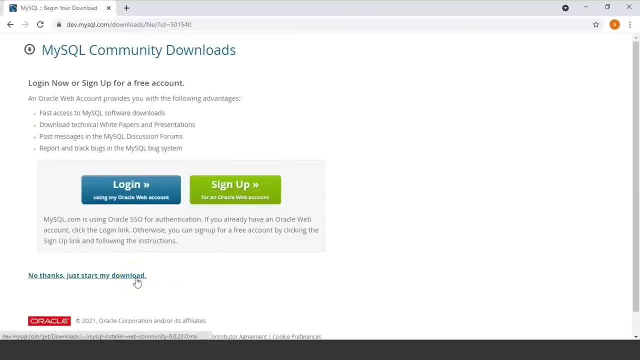 The current versions are available to download. I will choose this installer and click the Download button Now here. just click on No Thanks, Just start my download. Once the installer has downloaded, open it. You may be prompted for permission. click Yes. This opens the installer. You will be asked to choose the setup type. 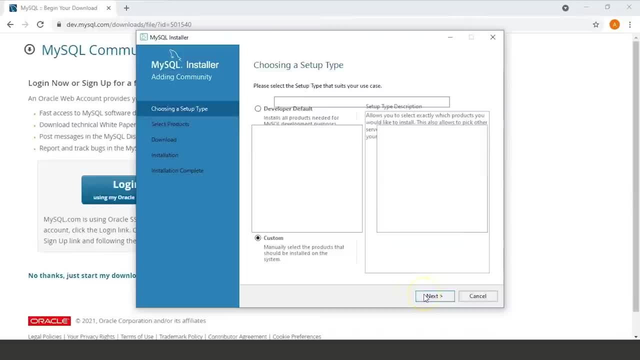 We will go with Custom. Click Next. Now you have to select the products you want to install. We will install only the MySQL Server, MySQL Shell and the MySQL Workbench. Expand MySQL servers by double clicking on it And choose the version you want to install And click on this arrow. 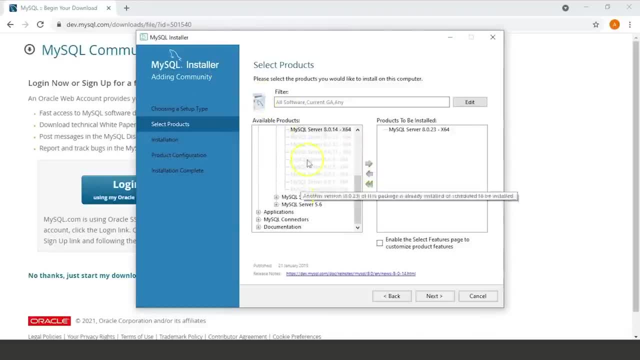 Now you have to do the same thing for applications. Expand Applications And choose the MySQL Workbench version you want to install And click on the arrow. We will do the same thing for MySQL Shell And choose the latest version, Click on the arrow. These are the products that have to be installed in a system. 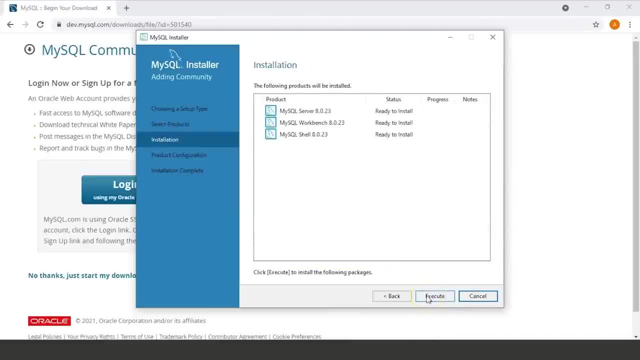 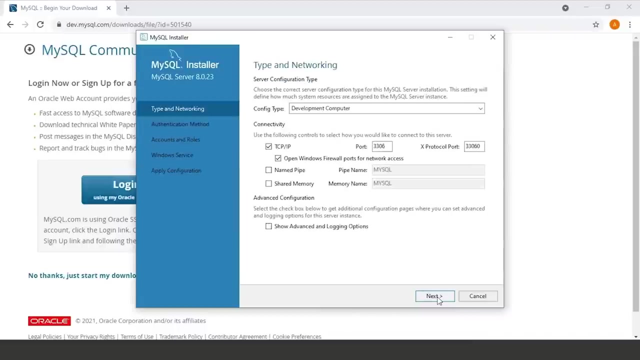 Now we will click Next Now click Execute to download and install the server. This may take a while depending on your internet speed. As the download is completed, click Next Now you will see the product configuration. Click Next Now we will configure our SQL Server Instance. Here we will go with the default settings. 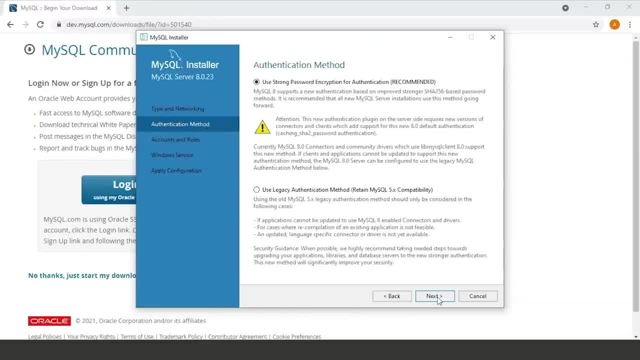 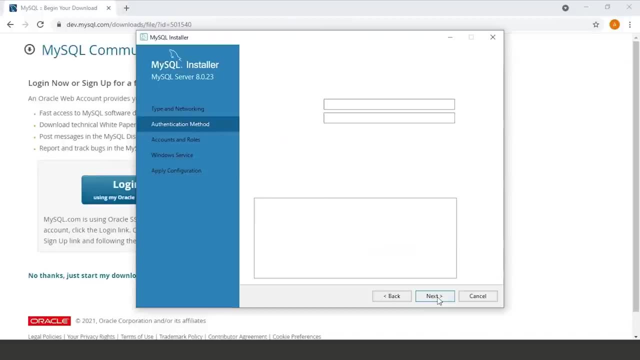 And click Next And under Authentication, select Use strong password encryption for authentication, which is recommended, And click on Next. Now, here, set the password for your root user. By the way, root is the default user. This user will have access to everything. Now I will set my password. 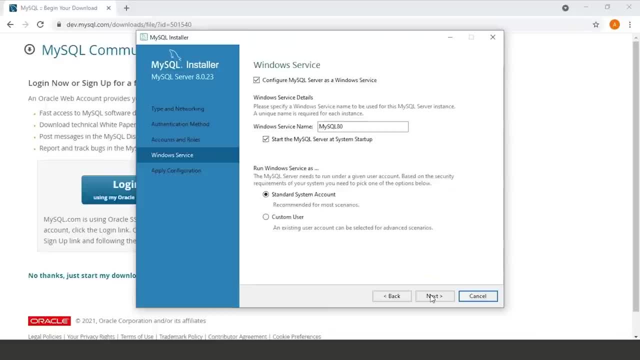 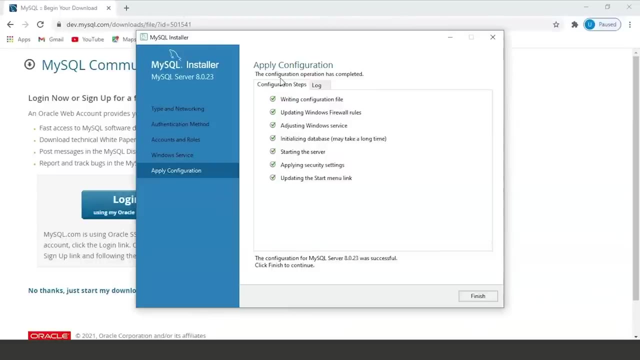 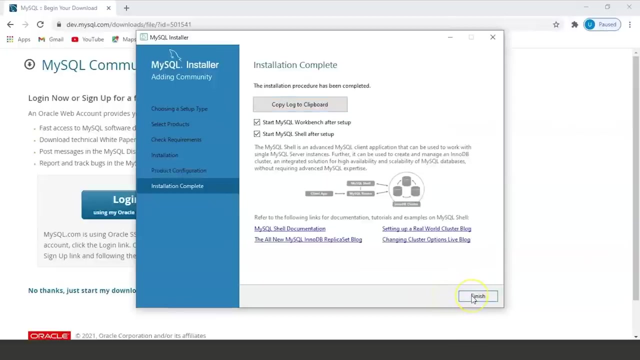 Now I will click on Next And here also we will keep the default settings And click on Next Now to apply configuration. we will execute the process Once all the configuration steps are complete. click Finish Now you will see the installation is complete. It will launch MySQL Workbench and MySQL Shell after clicking on Finish. 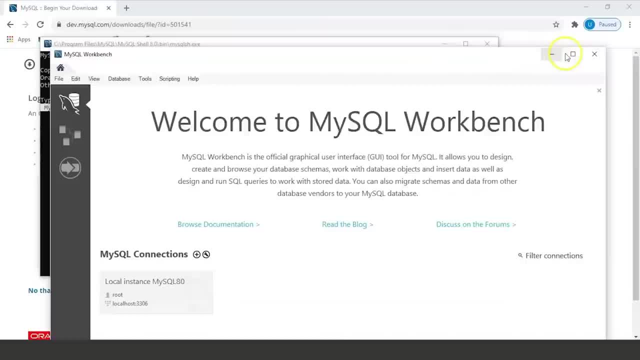 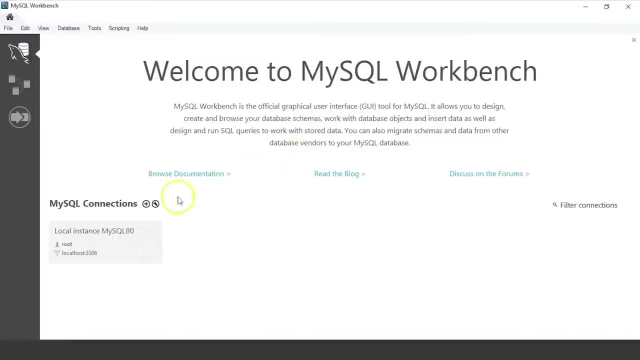 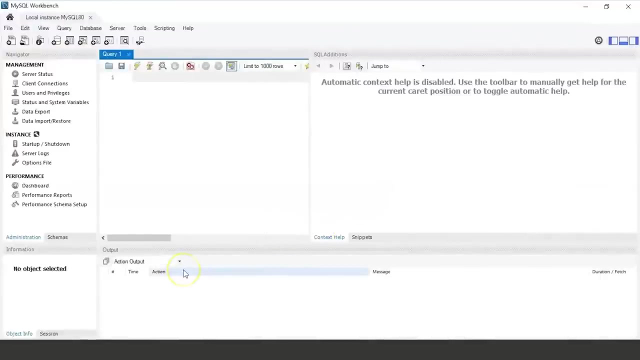 Now the Shell and Workbench has started. Now we will connect by clicking on the root user. It will ask for a password. Enter the Password And it will connect successfully. Click Connect, Click Connect. Now the workbench has started. now we will just connect the server. 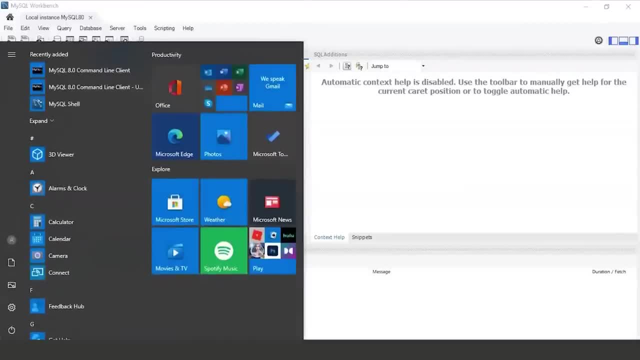 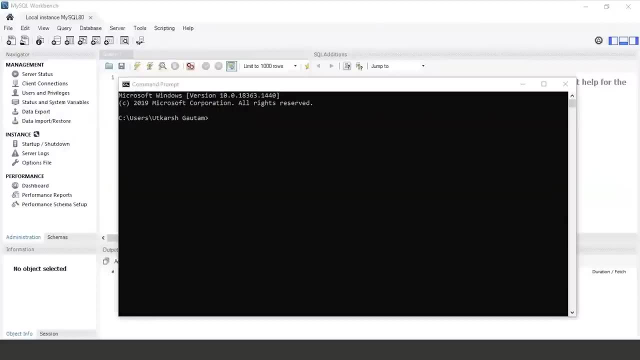 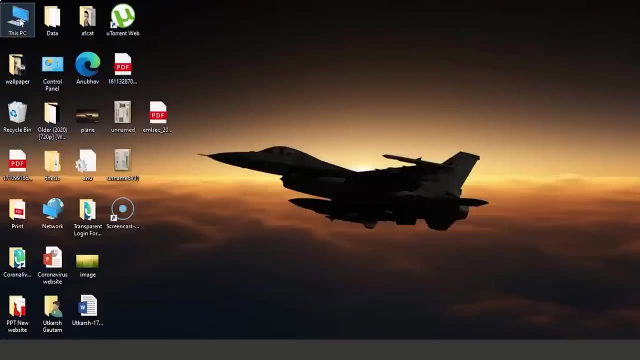 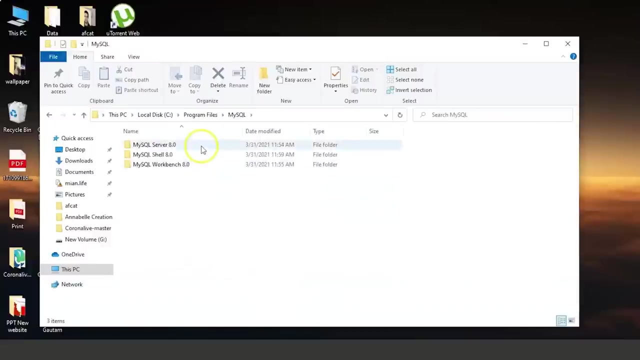 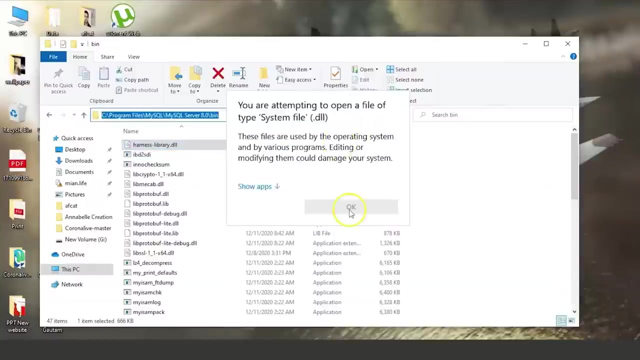 So first we will open command prompt, Now we will reach the path where mysql files are present. we will go into this pc local industry program files, mysql, mysql server 8.0, bin, and now we will copy this path. 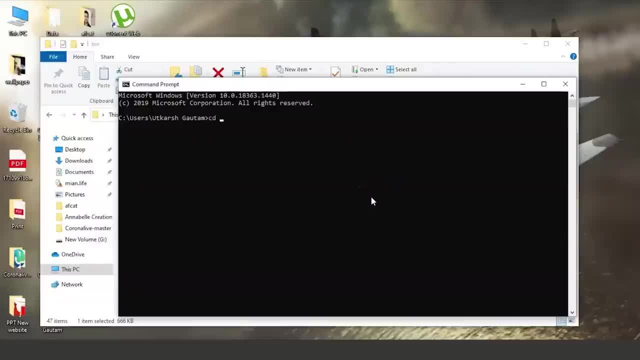 Now we will open the command prompt and write a command- cd space- and paste the link and press enter. Now we will write another command, Type: mysql minus u, space root minus p and press enter. Now it will ask for your password. Just enter the password and press enter. 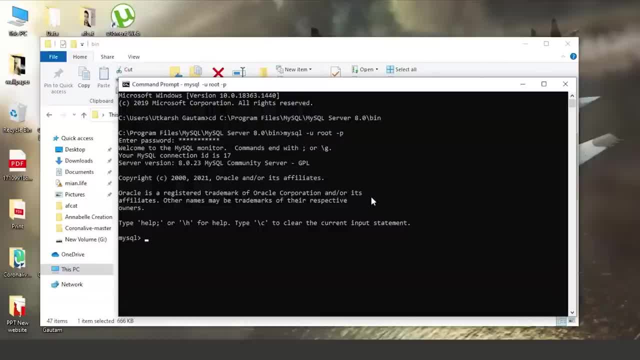 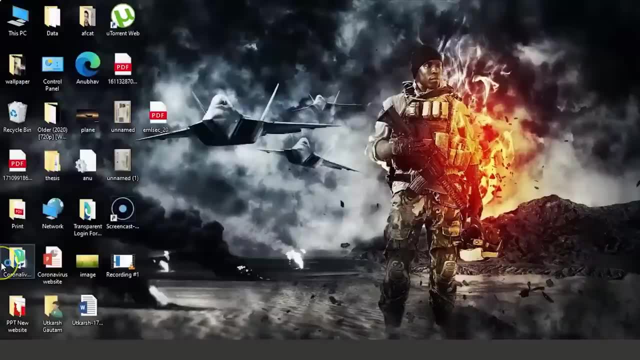 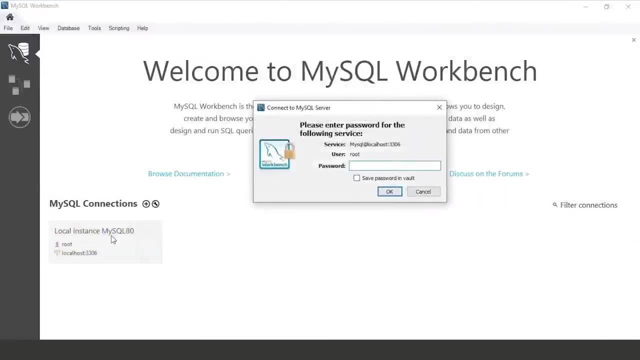 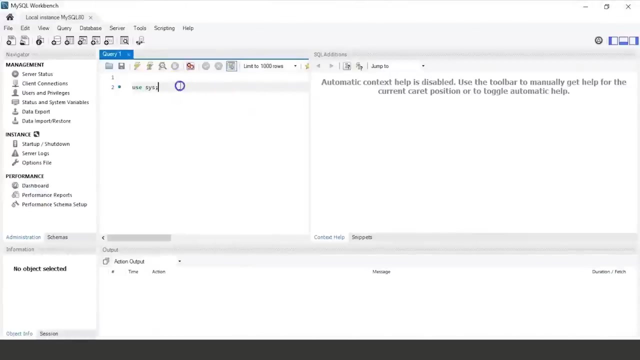 Now the server has started, and now we will see some commands in mysql workbench. First we will open mysql workbench. Ok, Now we will click on the local instance, mysql 80- and enter the password to connect to the local host. The mysql workbench has started. 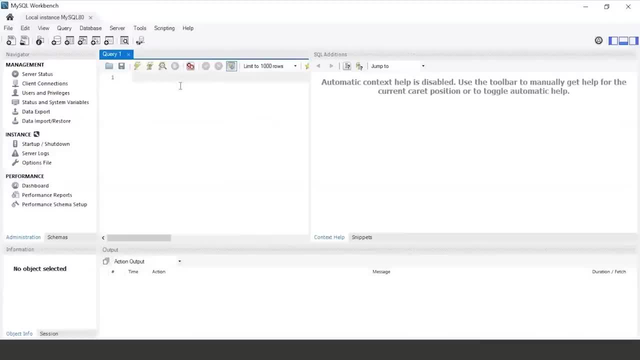 Now we will see some commands. The first command we will see is show databases. Ok, Show databases, semicolon. and now we will select the whole command and click on this execute button and here we will see the result in the result grid. These are the databases that are stored already in the database. 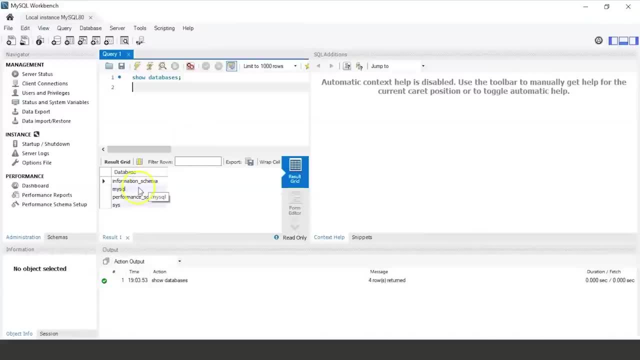 Now there are four databases, That is, information schema, mysql, mysql and mysql. Now we will see some commands: Information schema, mysql, performance schema and sys. Now we will select one of the databases. We will use mysql. Now we have selected the mysql database and now in this database we will see which tables. 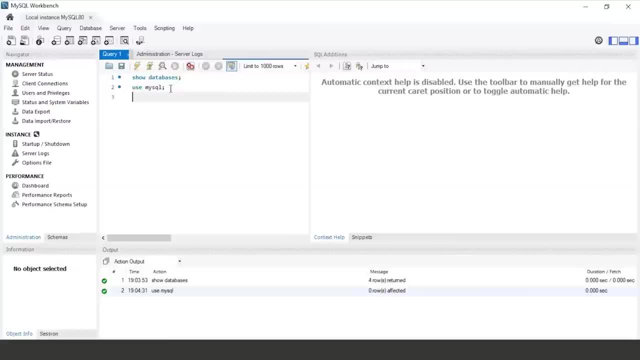 are stored in this mysql database. To see that we will run a command show tables, We will select the command and click on the execute button. These are the tables that are stored in this mysql database, That is, columns, underscore, private component db and much more. 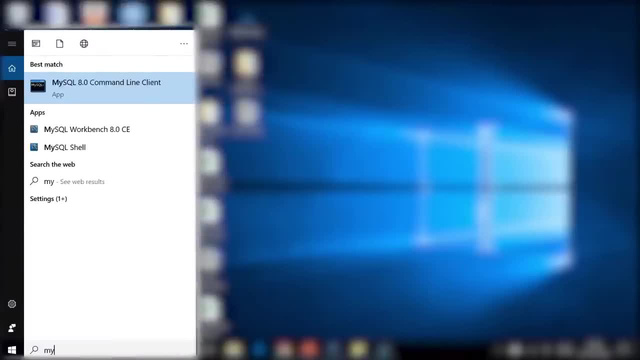 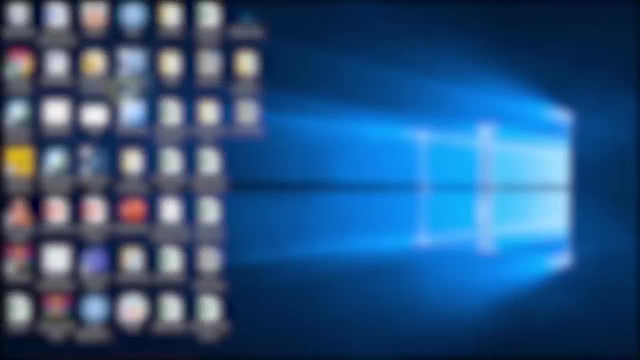 Now, let me now go ahead and open my mysql workbench. So in the search bar I will search for mysql workbench. You can see I am using the 8.0 version. I am going to open it. Let me open it. 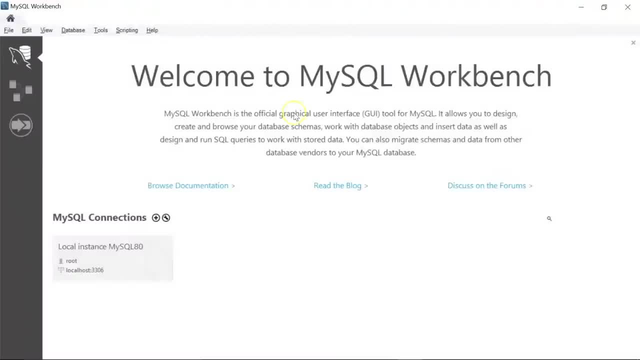 I will click on it and here it says: welcome to mysql workbench. and below, under connections, you can see I have already created a connection which says local instance. Then you have the root, the local host and the port number. Let me click on it. 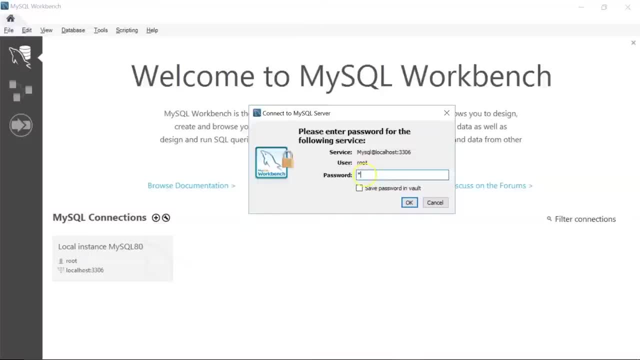 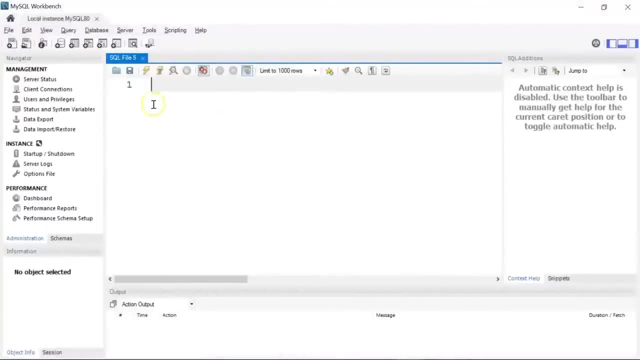 You can see the service. The username is root and I will enter my password and hit ok. Now this will open the sql editor. So this is how the mysql workbench looks like. Here we learn some of the basic sql commands. So first let me show you the databases that are already present. 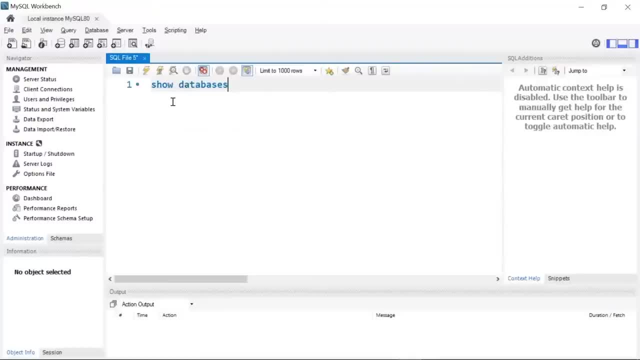 So the command is show databases. You can hit tab to auto-complete. I will use a semi-colon, I will select this and here on the top you can see the execute button. So if I run this below you can see the output. 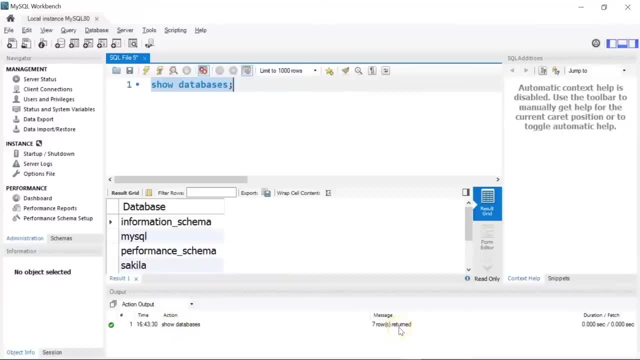 It says show databases. Seven rows are returned, Which means currently there are seven databases. You can see the names. All right. Now let's say I want to see the tables that are present inside this database called world. So I will use the command use world, which is the database name. 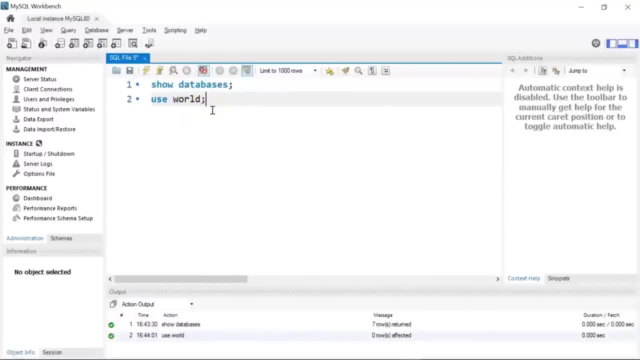 Now let me run it. So currently I am using the world database. So to display the tables that are present in the world database, I can use the show command and write show tables. give a semi-colon and I will hit control enter. this time to run it. 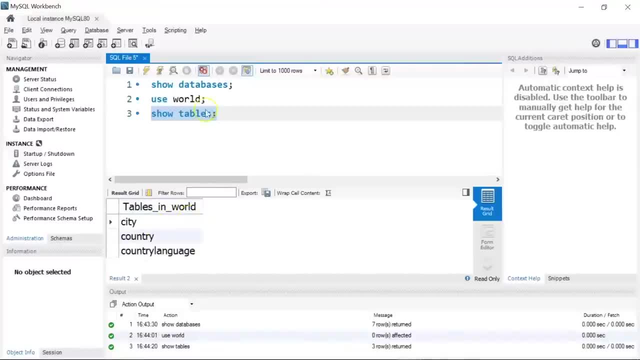 All right, So you can see the tables that are present inside this world database. So we have three tables in total: city, country and country language. Now, if you are to see the rows that are present in one of the tables, you can use the select. 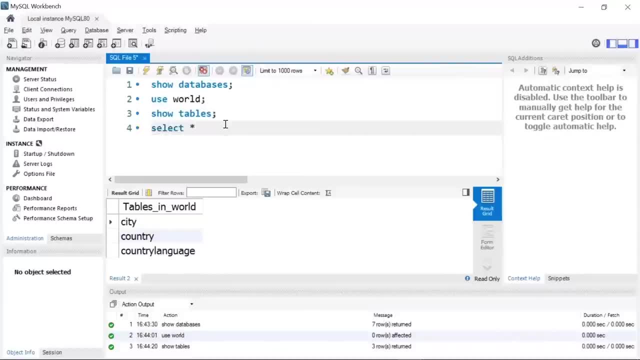 command. So I will write select star, Which basically means I want to display all the tables that are present in the world database. Now, if you are to see the rows that are present in one of the tables, you can use the select command. 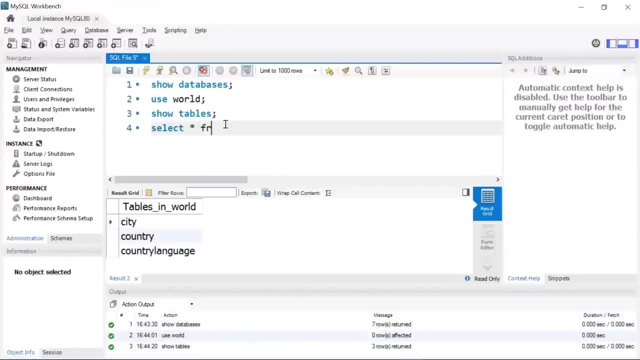 So I will write select star, Which basically means I want to display all the columns. So star here means to display all the columns. Then I will write my from the table name that is city. So this command is going to display me all the rows that are present inside the city. 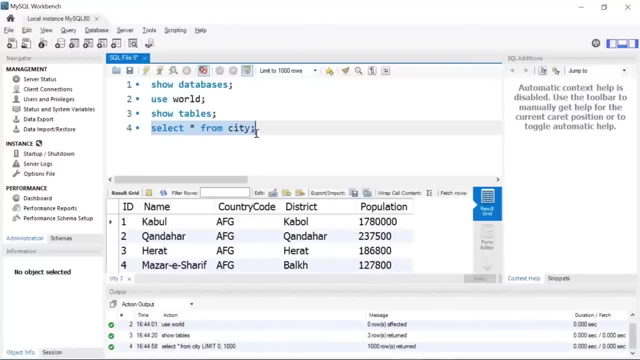 table. So if I hit control enter, All right, You can see the message here. It says thousand rows were returned, which means there were a total thousand records present inside the city table. So here you can see this. It's an ID column, a name column. this country code, district and population. 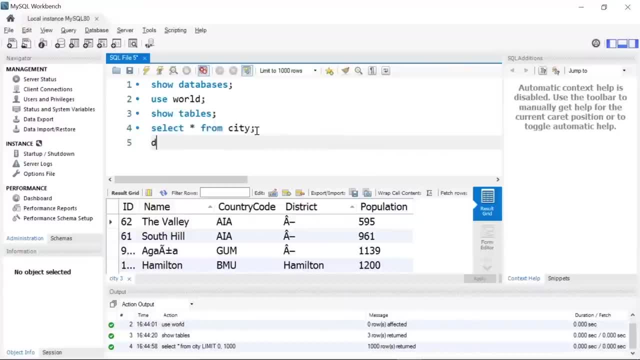 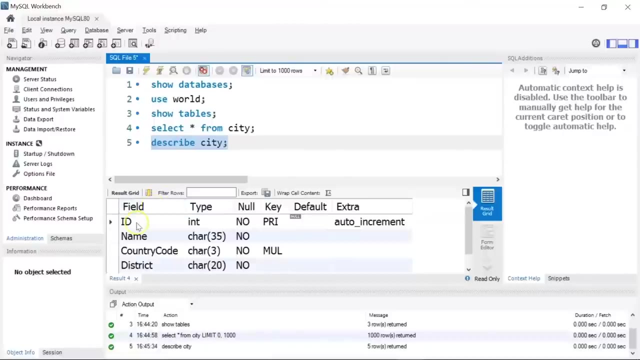 All right. Similarly, you can check the structure of the table by using the describe command. So I'll write describe And then I'll give the table name. that is city. Now let's just run it. There you go. The field shows the column names. 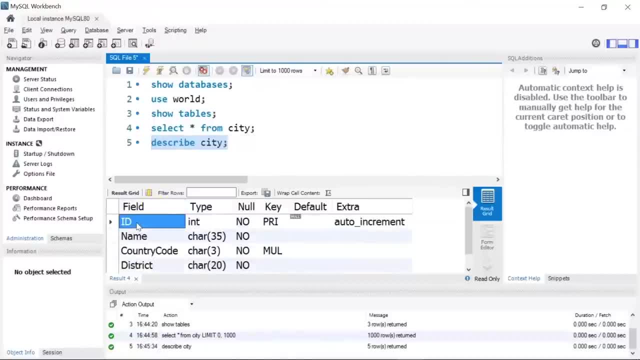 So we have ID name, country code, district population Type. here shows the data type of each of the columns. So district is character 20,, ID is an integer. population is also integer. null says yes or no, which means if no, then there are no null values. 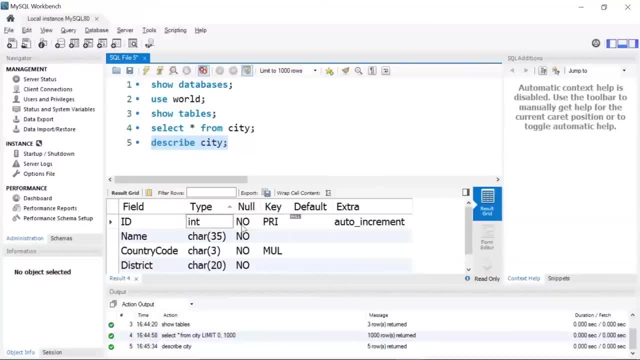 If it's yes, which means there are null values in your table. Key here represents whether you have any primary key or foreign key, And these are some extra information. Now let's learn how to create a table in MySQL, So I'll use the create table command for this. 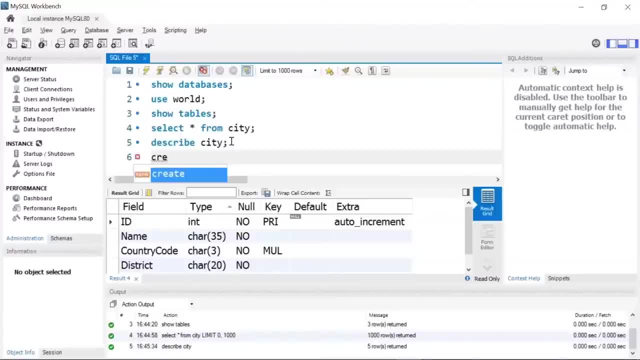 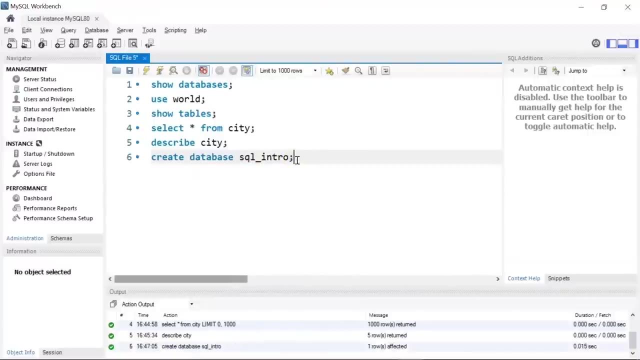 And before that: Okay, So I'll create a database and I'll name it as SQL intro. So the command is create database and I'll give my database name. that is SQL underscore intro. I'll give a semicolon and hit control enter. 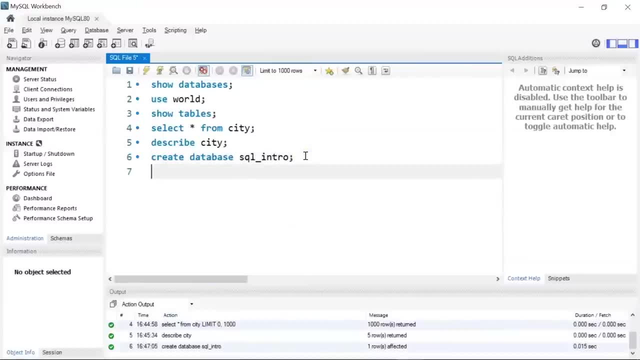 You can see I have created a new database. Now if I run this command, that is, show databases, you can see this newly created database. that is SQL intro. If I scroll down, there you go. You can see the name here: SQL intro. 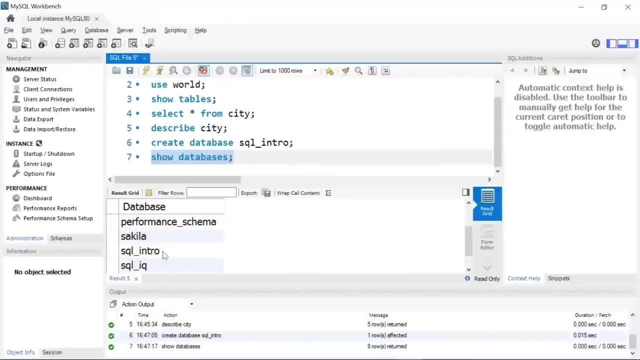 Okay, Now, within this database, we'll create a table called employee details. Now, this will have the details of some employees. So let me first show you how to create a table that will be present inside the SQL intro database. So I'll use the command create table and then I'll give my table name. that is going to be. 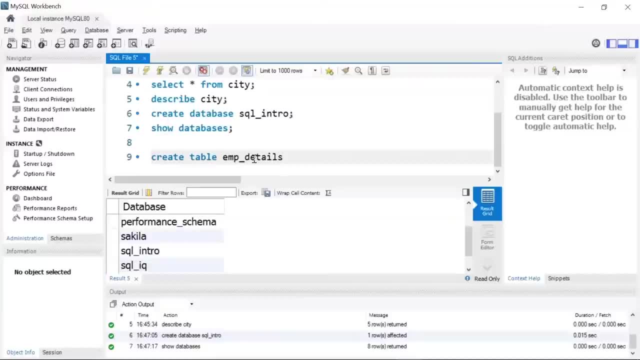 employee underscore- intro. Okay, So I'm going to create a table called employee details. Next, the syntax is to give the column names. So my first column would be the name column, which is basically the employee name, followed by the data type for this column, since name is a text column. 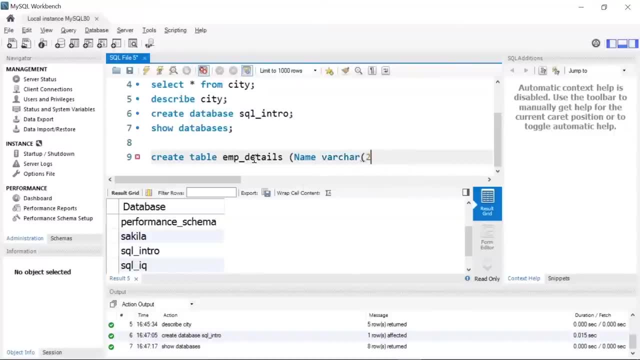 So I'll use varchar and I'll give a value of 25.. So it can hold only 25 characters, Okay Next. Okay Next. we have the age of the employee. Now, age is always an integer, so I'll give int. 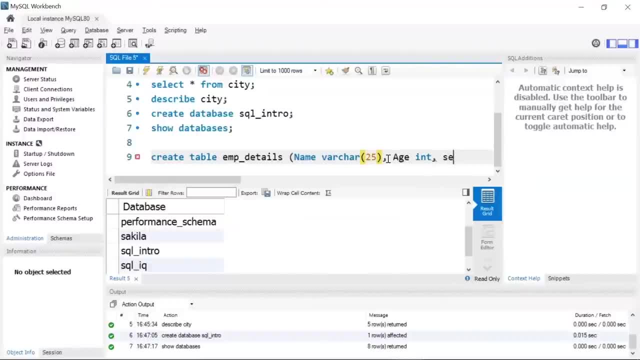 Okay, then we can have the gender of the employee. So gender can be represented as f or m: f for female and m for male. So I'm using the car data type or character data type, and I'll give the value as one. 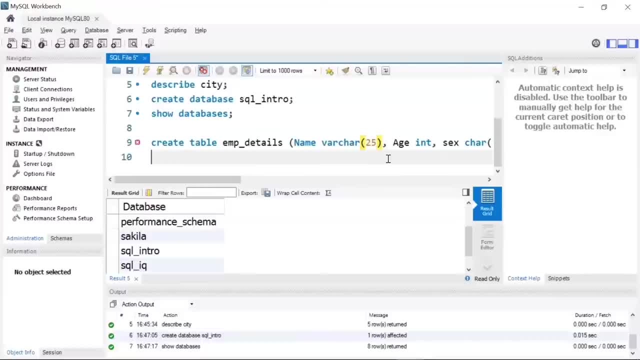 Then let's have the date of join, or DOJ. Okay, and this is going to be of data type date, all right. next, we'll have the city name, that is, the city to which the employee belongs to. so, again, this is going to be worker 15. finally, we'll have 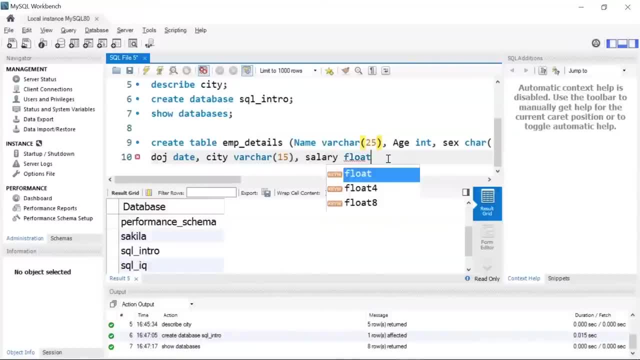 a salary column and salary. we'll keep it as float, since salary can be in decimal numbers as well. now i'll give a semicolon, all right, so let me just quickly run through it. so first i wrote my create command, then the table, which is also a keyword, followed by the table name, which 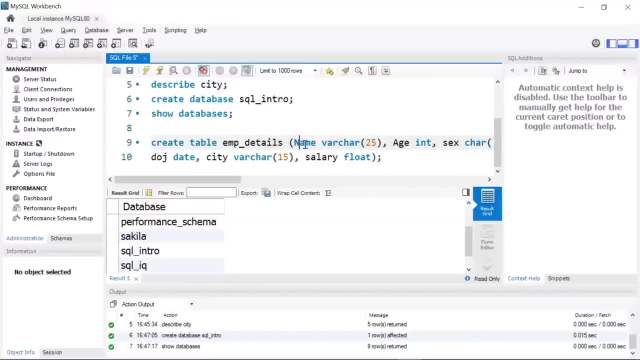 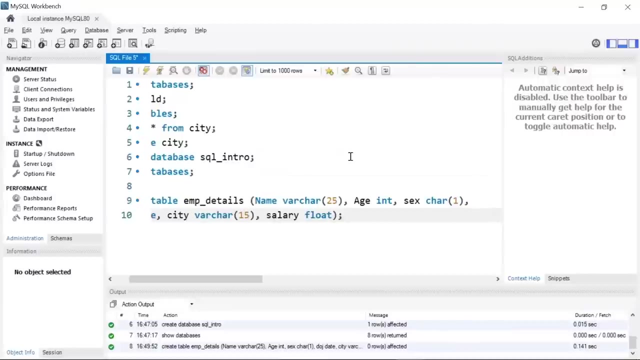 is employee details here, and then we give the column names, such as name, age, this gender, date of join city and salary. for each of the columns we also give the data type. all right, so let me just run it okay. so here you can see we have successfully created. 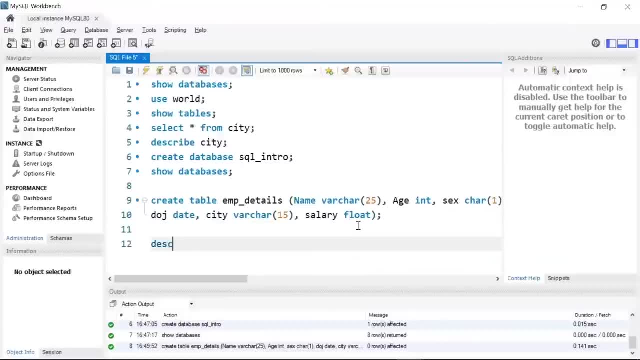 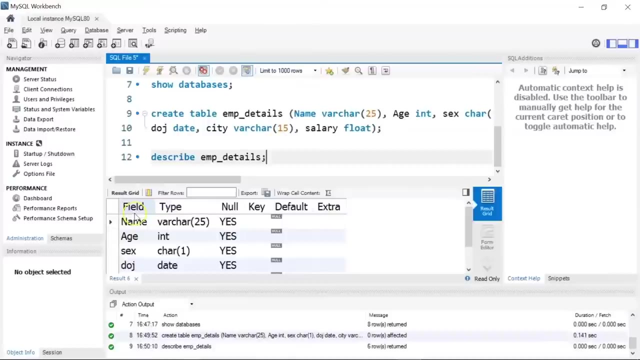 our first table. now you can use the describe command to see the structure of the table. i'll write describe: emp underscore details. if i run this there you go. so under field you can see the column names. then you have the data types. null represents if the table can accept null values or not, and these are basically empty and we haven't set any. 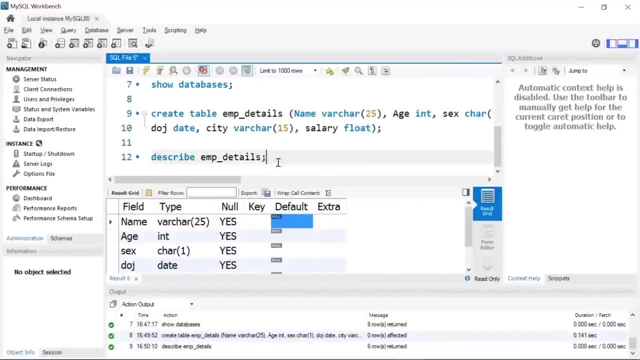 default constraint. all right, moving ahead, now let's learn to add data to our table using the insert command. so on a notepad i have already written my insert statement, so let me just copy it and then i'll explain it one by one. all right, so if you see this, so we have used 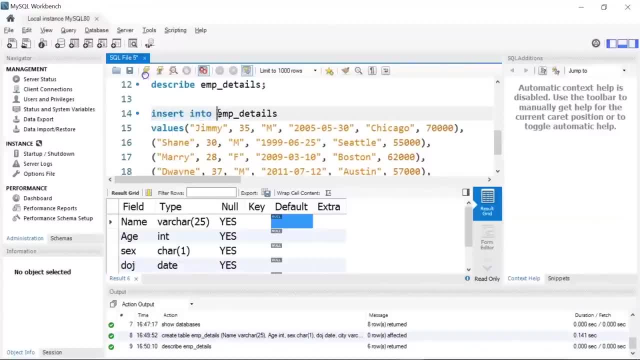 an insert into statement or a command, followed by the table name, that is, emp details. then this is the syntax using values i have passed in all the records. so first we have jimmy, which is the name of the employee, then we have 35, which basically represents the age, then m means the gender or the. 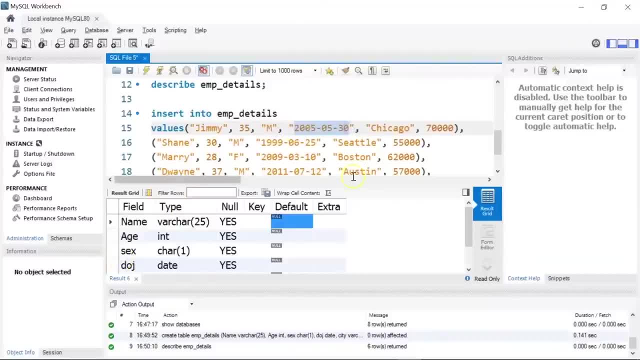 sex. then we have the date of join. next we have the city to which the employee belongs to and the salary of the employee. so this particular information represents one record, or a tuple. similarly, the next employee we have is shane. you can see the age. another information, then we have 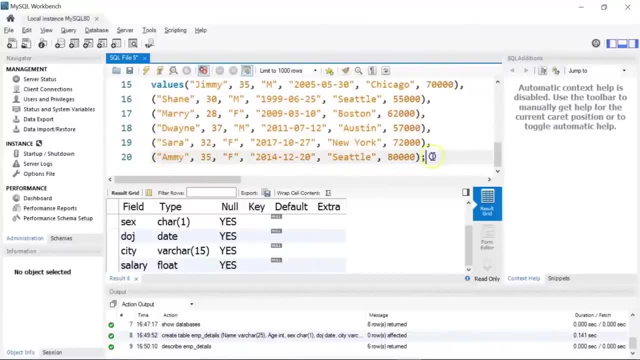 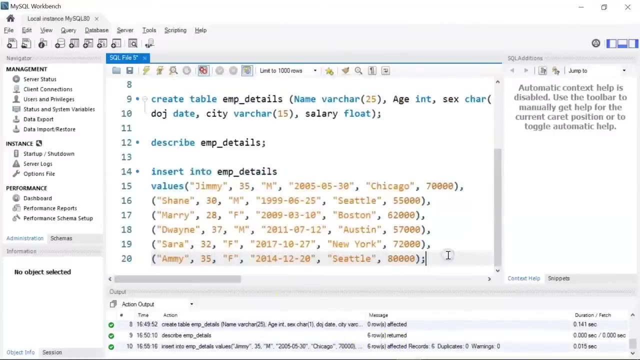 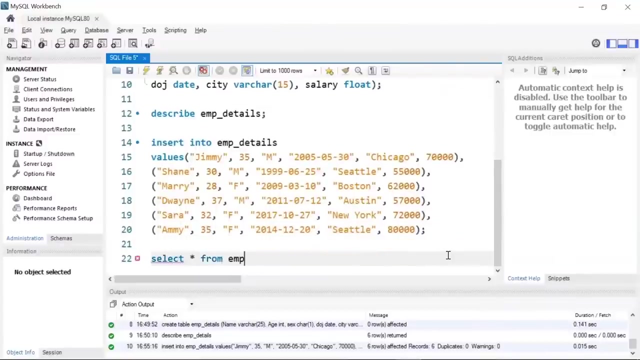 mary, this dwayne, sarah and amy. all right, so let me go ahead and run this. so this will help you insert the values in the table that you have created. you can see we have successfully inserted six records. now to display the records, let me use the select statement. so i'm using select star from. 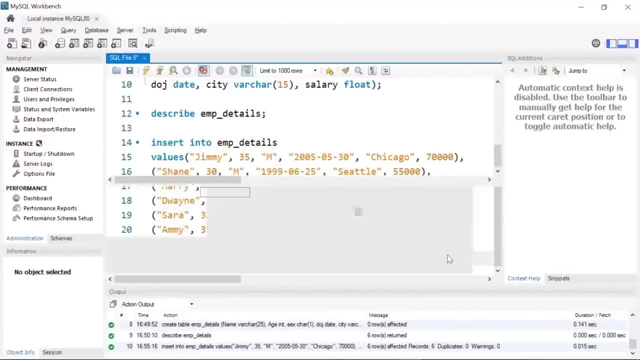 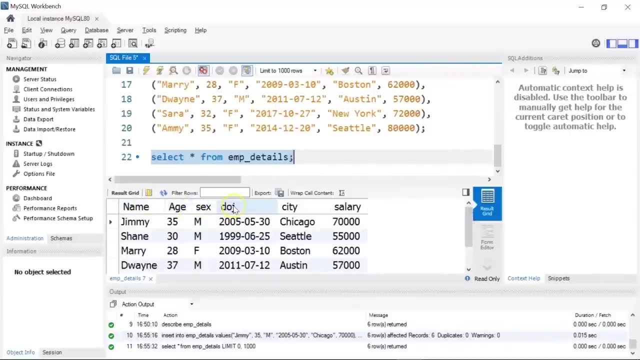 emp underscore details. if i run this, you can see my table here and the values it has. so we have the name column, the age column, the state of join city, salary, and these are the values that you can see here. moving ahead now, let's say you want to see the unique city. 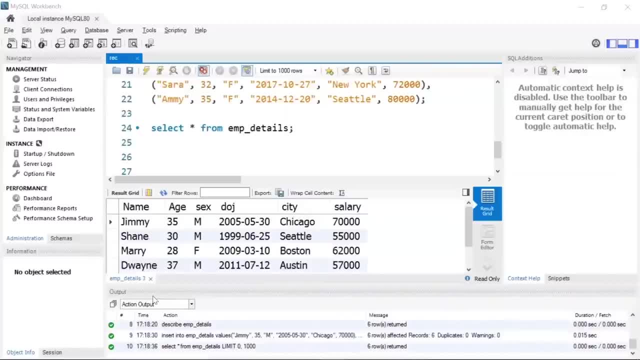 present in the table. so in this case you can use the distinct keyword along with the column name in the select statement. so let me show you how you can print the distinct city names that are present in our table. now, if you notice this table clearly, we have Chicago, Seattle, Boston, Austin, this New York and this Seattle. 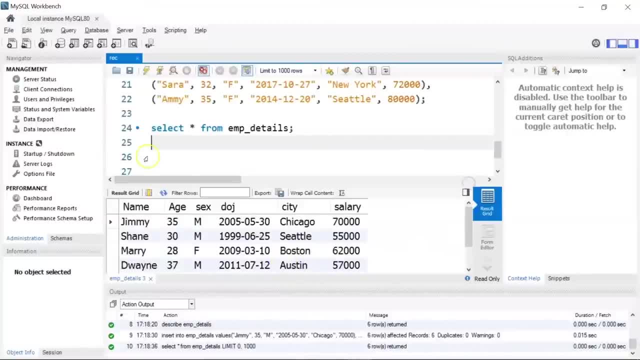 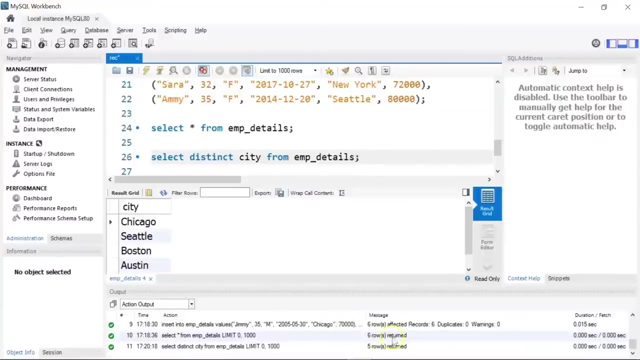 repeated again. so I only want to print the unique values. so for that I can write my select statement as select distinct. then I will give my column name, which is city, from my table name, that is EMP details. if I run this, you can see my query has returned five rows and these are the values. so we have Chicago, Seattle. 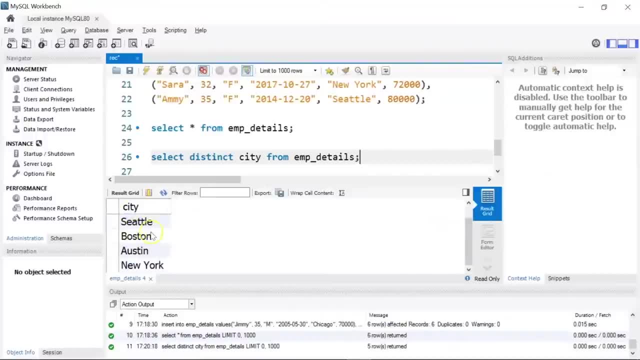 which was repeated twice, it's just been shown once. then we have Boston, Austin and New York. now let's see how you can use the EMP details to print the distinct city names. so let me show you how you can print the distinct city names. so we have Chicago. Seattle, which was repeated twice, is just been shown once. then we have Boston, Austin and New York. now let's see how you can use the. 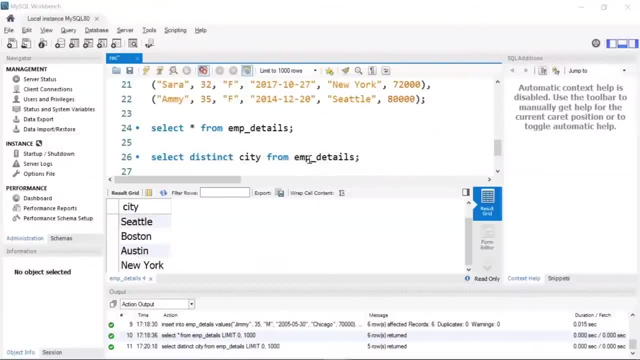 inbuilt aggregate functions in SQL. so suppose you want to count the number of employees in the table, so in that case you can use the count function in the select statement. so let me show you how to do that. so I'll write select, I'll use my function name, that is, count. now, since I want to know the total number of. 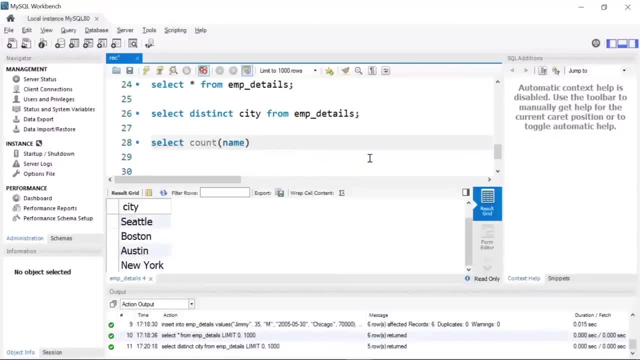 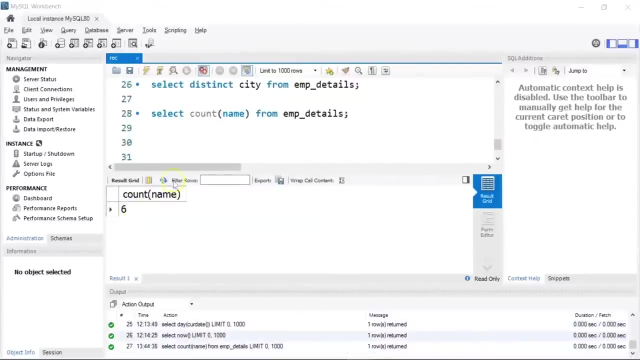 employees. I'm going to use their name inside the brackets from employee underscore details. now, if I run this, this will return the total number of employees that are present in the table. so we have six employees in total. now. if you see here in the result it says count name. now this column is: 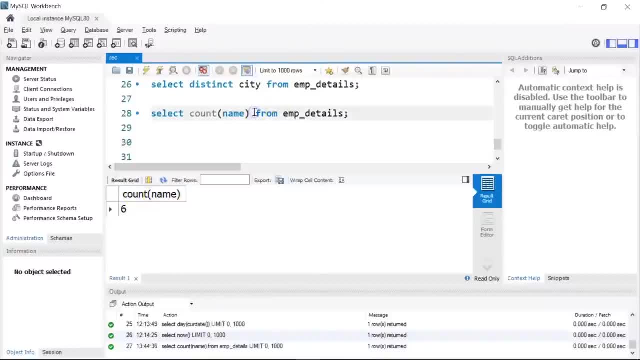 actually not readable at all. so what SQL provides is something called as an alias name, so you can give an alias to the resultant output. so here I can write select count of name and use an alias, as as I can give an alias as count, underscore name and run this. 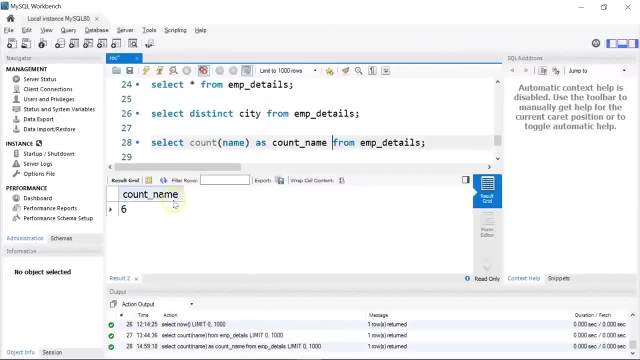 statement again. there you go. you can see here in the resultant output we have the column name as count name, which was our alias name. now, suppose you want to get the total sum of salaries. you can use another aggregate function called sum. so I'll write my select statement. 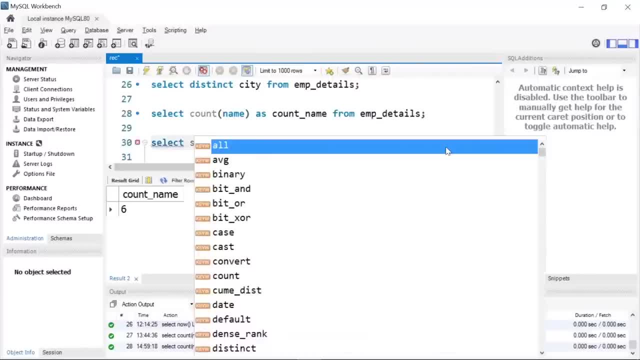 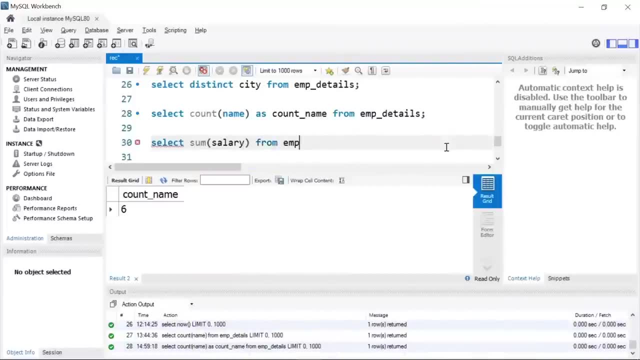 and this time instead of count I'm going to write sum. and since I want to find the sum of salaries inside the bracket, I will give my salary column from table name, that is, employee details. if I run, this will result the total sum of salaries. so 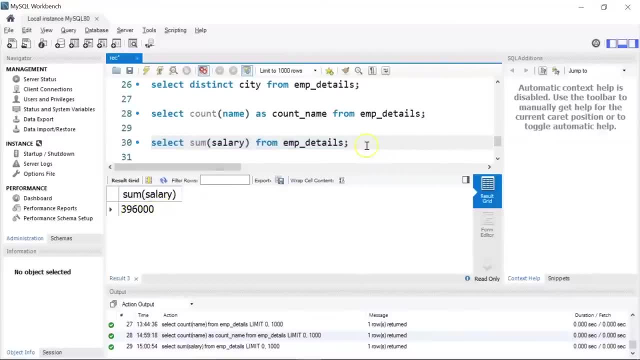 basically, it adds up all the salaries that were present in the salary column. now you want to find the average salary, so instead of sum, you can function, which is AVG. so this will give you the average salary from the column salary, so you can see it here. this is average salary. now, if you want, you can. 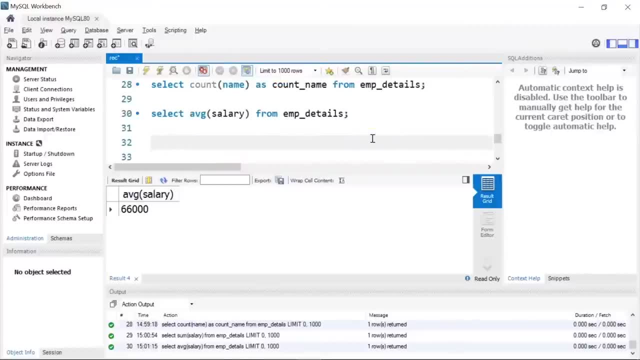 give an alias name to this as well. now you can select specific columns from the table by using the column names in the select statement. so initially we were selecting all the columns. for example, like you saw here, the star represents that we want to see all the columns from the employee details table now. 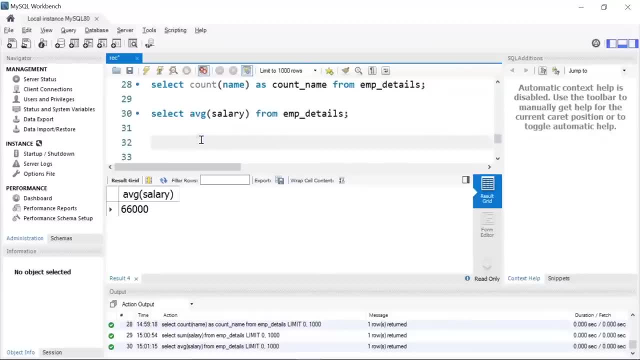 suppose you want to see only specific columns, you can mention those column names in the select statement. so let's say I want to select just the name, age and the city column from my table, that is, employee details. so this will result in displaying only the name agent, city column from the table, if I run it. 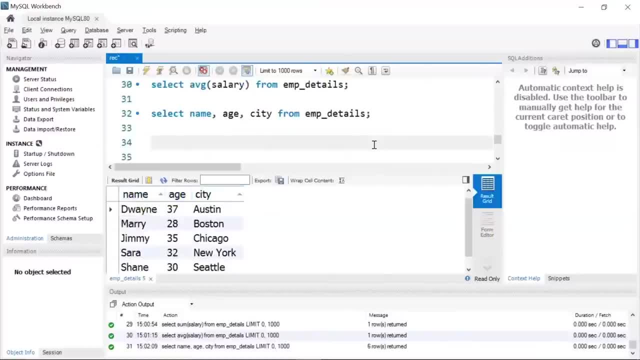 there you go. it has given only three columns to me. now. SQL has a where clause to filter rows based on a particular condition. so if you want to filter your table based on of specific conditions, you can use where clause. now, where clause comes after you give your table name. so suppose you want to find the 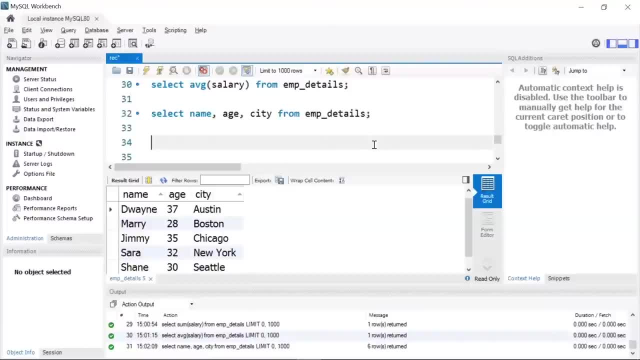 employees with age greater than 30. in this case you can use a where clause. so let me show you how to do it. I'll write select star from my table name, that is, employee details, and after this I'll use my where clause so I'll write where: age greater than 30. if I run this, it will give me 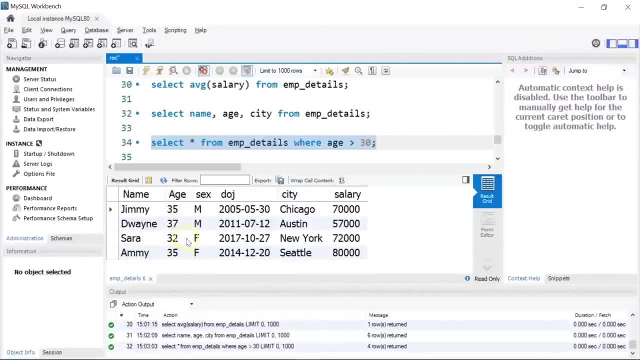 the output where the age is only greater than 30. so it excluded everything that is less than 30. so we have four employees whose age is greater than 30 here. now suppose you want to find only female employees from the table? you can also use a where clause here, so I'll write. 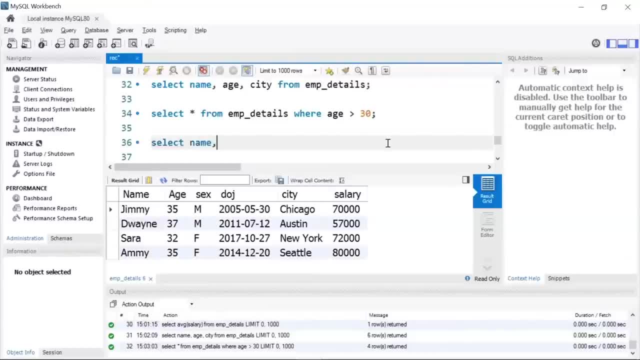 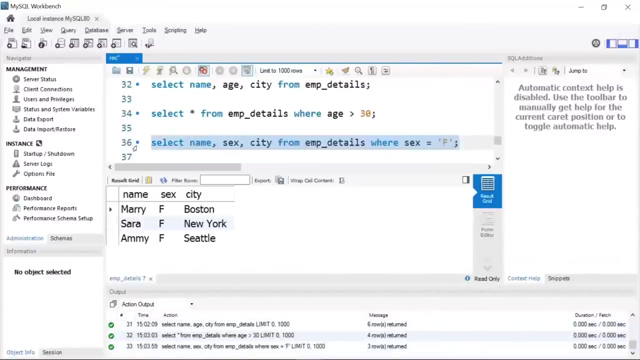 select. let's say I want only the name, the gender which is sex here, comma city- from my table, that is employee details, where I'll give my column name that is sex is equal to. since I want only the female employees, I'll give F and run this statement. okay, you can see here our employee table has. 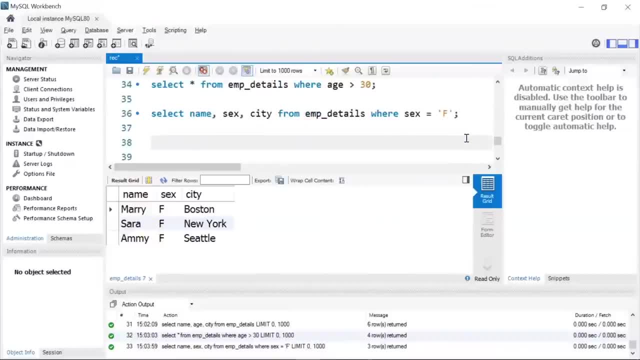 three female employees. now suppose you want to find the details of the employees who belong to Chicago or Austin. in this case you can use the or operator. now the or operator in SQL displays a record if any of the condition separated by or is true. so let me show you what I mean. 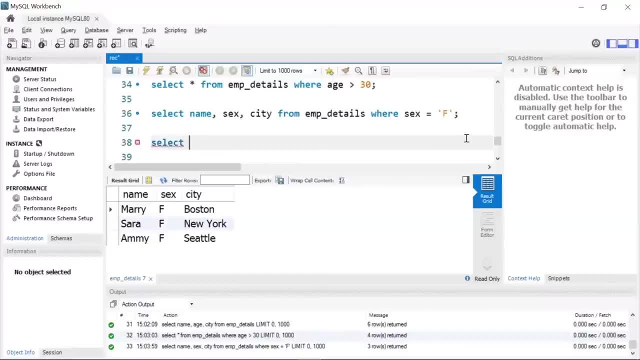 so, since I want the employees who are from Chicago in Austin, I can use an or operator. so I'll write select star from EMP details, which is my table name, then I'll give my where clause, where city equal to. I'll give my city name as Chicago and then I am going to use the OR operator or city. 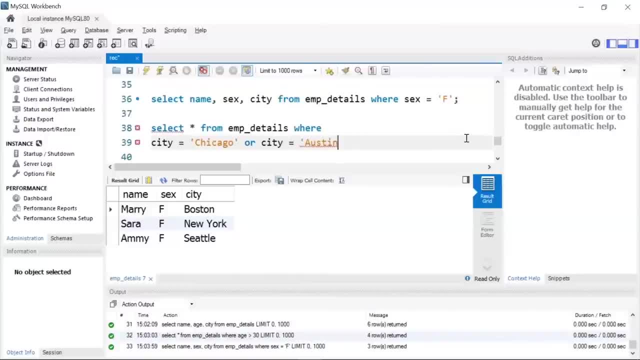 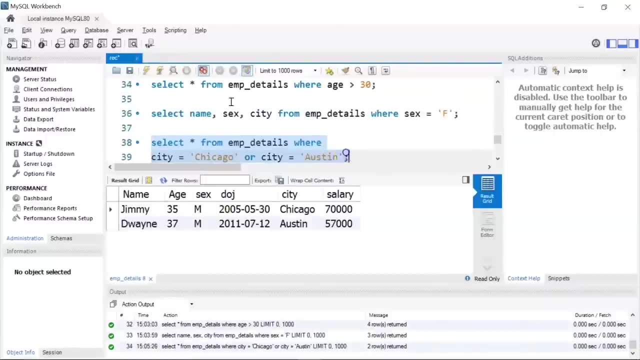 equal to. i'll write austin, i'll give a semicolon and let me run it. there you go. so in the output you can see all the employees who belong to the city chicago and austin. now there is another way to write the same sql query so you can use an in operator to specify. 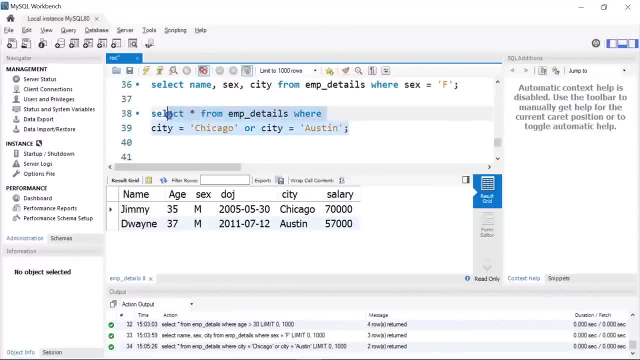 multiple conditions. so let me just copy this and instead of using the or operator, this time i'm going to use the in operator, so i'll delete this. after the where clause i'm going to write where, city and use the in operator. inside bracket i'll give my city names as: 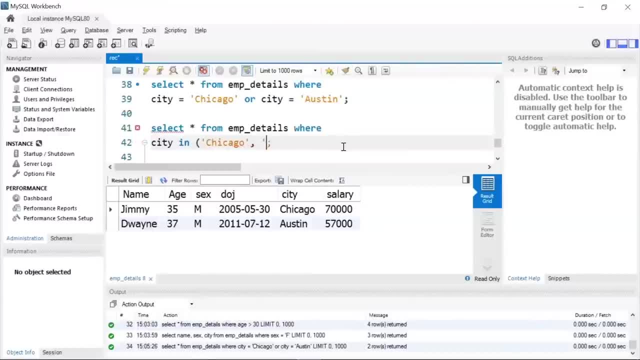 chicago and i want austin. so i'll give a comma and write my next city name that is austin. so this query is exactly the same that we wrote earlier. let me run this. you will get the same output. there you go. so we have jimmy and dwayne, who are from. 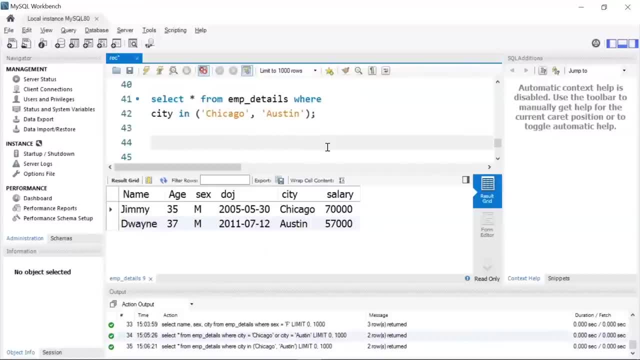 chicago and austin respectively. now sql provides the between operator that selects values within a given range. the values can be numbers, text or dates. now suppose you want to find the employees whose date of join was between 1st of jan 2000 and 31st of december 2010? so let me show you how to do it. 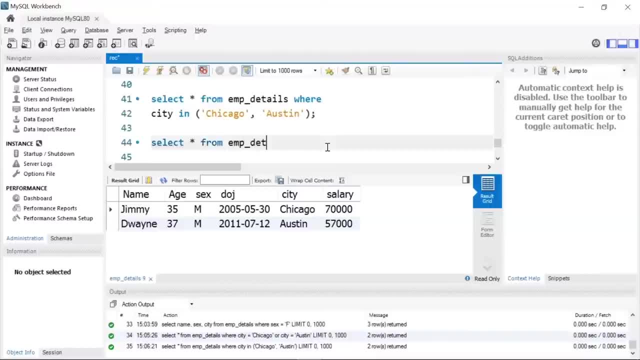 i'll write select star from emp details where my date of join, that is, doj, between. i'll give my two date values, that is, first of jan 2000, and i'll give my second value, the date value that is December 31st of december 2010. so every employee who has joined between 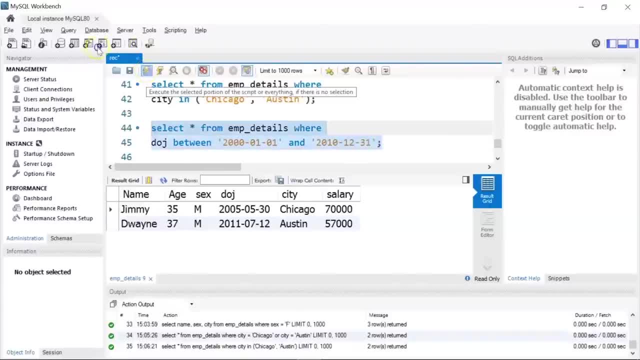 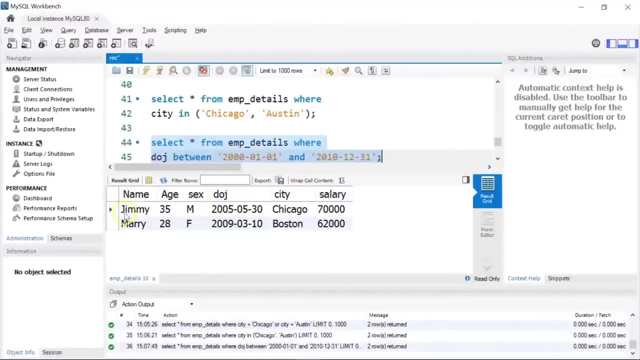 these two dates will be displayed in the output. if i run it. we have two employees who had joined between 2000 and 2010, so we have jimmy and mary here who had joined in 2005 and 2009 respectively. all right now, in where clause you can use the and. 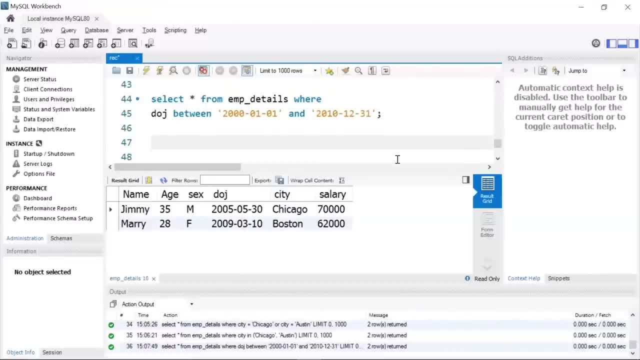 operator to specify multiple conditions. now the and operator displays a record if all the conditions separated by and are true. so let me show you an example. i'll write select star from employee details table where i want the age to be greater than 30 and i want sex to be male. 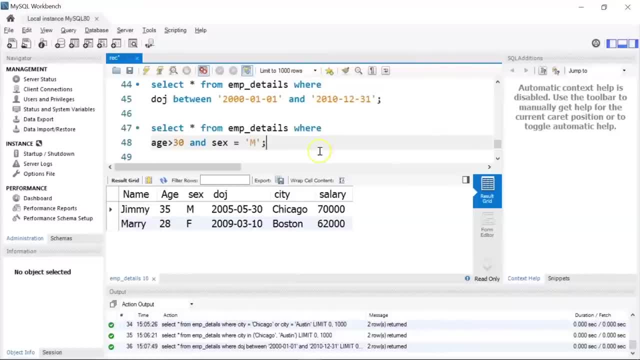 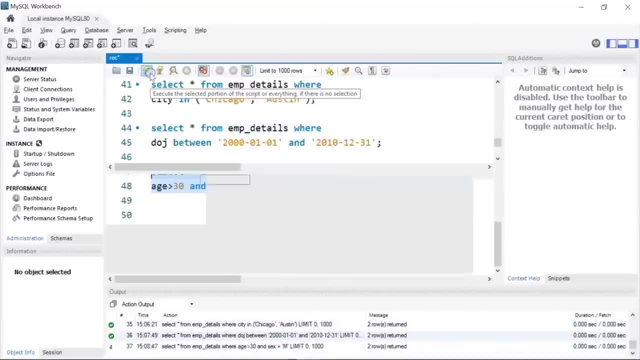 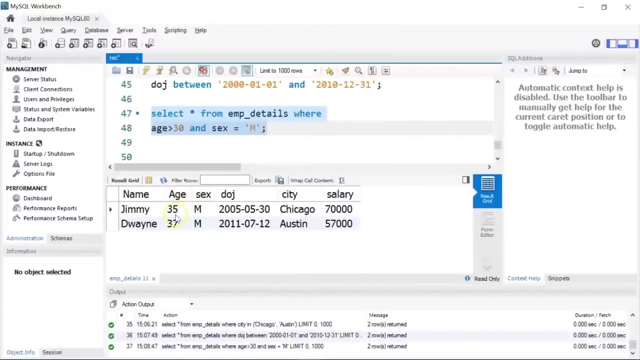 all right. so here you can see. i have specified two conditions. so if both the conditions are true, only then it will result in an output. if i run it, you can see there are two employees who are male and their age is greater than 30. now let's talk about the group by statement in sql. 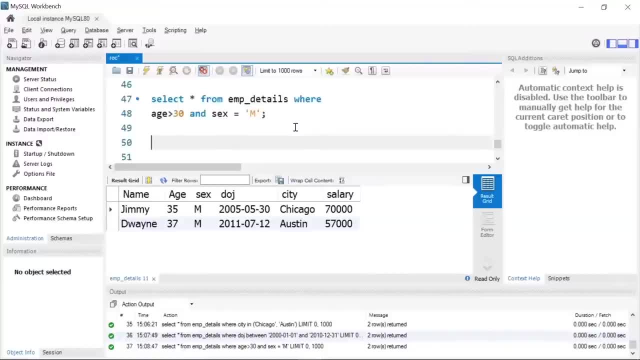 so the group by statement groups rows that have the same values into summary rows like, for example, you want to find the average salary rate of the employee and you want to find the average salary of customers in each department. now, the group by statement is often used with aggregate functions. 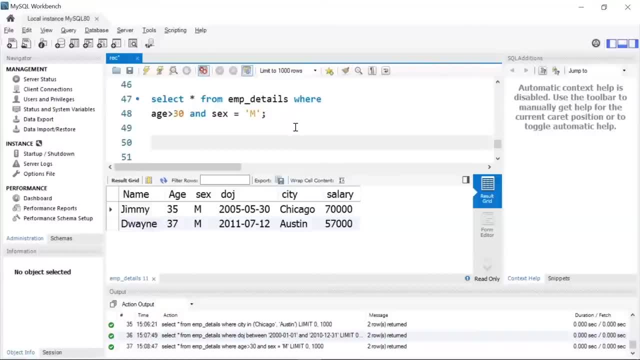 such as count, sum and average, to group the result set into one or more columns. let's say we want to find the total salary of employees based on the gender. so in this case you can use the group by clause. so i'll write select, let's say sex comma. i want to find the total sum of salary. 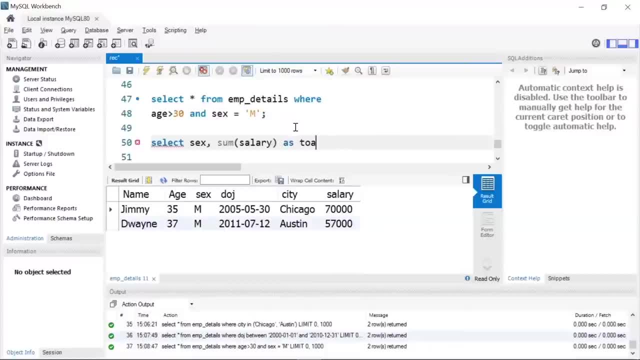 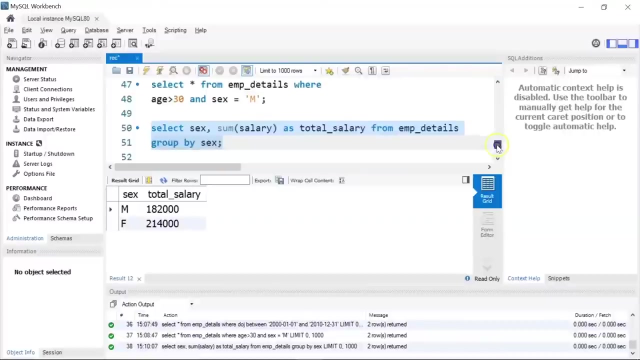 as i'll give an alias name, let's say total salary from my table name, that is, employee details. next, i am going to group it by sex. okay, let me run it. there you go. so we have two genders, male and female, and here you can see the 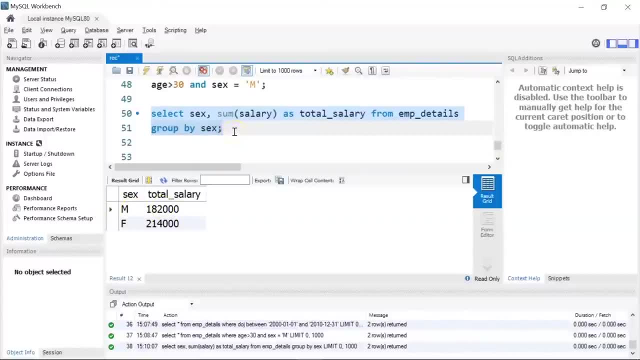 total salary. so what this means is that if i group it by sex comma, i want to find the total salary. as sql statement did was first it grouped all the employees based on the gender and then it found the total salary. now sql provides the order by keyword to sort the result set in ascending or descending. 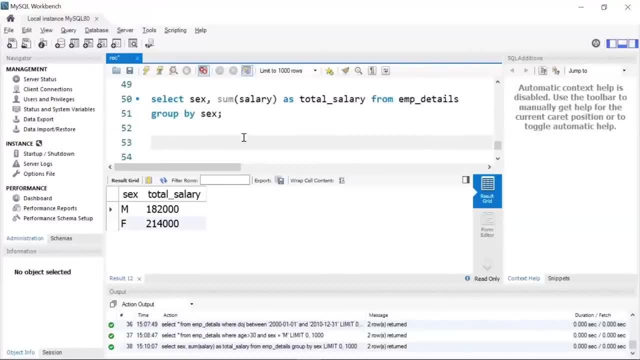 order. now the order by keyword sorts the records in ascending order by default. to sort the records in descending order you can use the desc keyword. so let's say i want to sort my employee details table in terms of salary. so i'll write select star from emp, underscore details and i'll use my order by clause on the salary column. 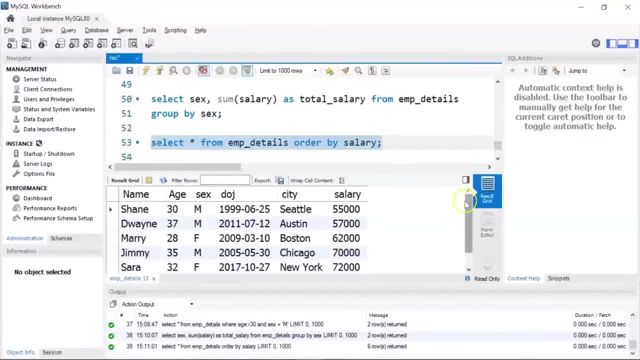 so this will sort all the records in ascending order of the salary, which is by default. you can see the salary column is sorted in ascending order. now suppose you want to sort the salary column and display it in descending order. you can use this keyword, that is desc. 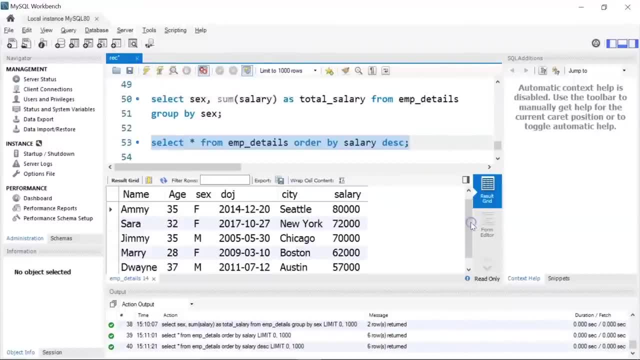 let me run it. you can see the output now. this time the salary is sorted in descending order and you have the other values as well. now let me show you some basic operations that you can do using the select statement. so suppose i write select and do an addition operation. let's say 10 plus 20, and i'll 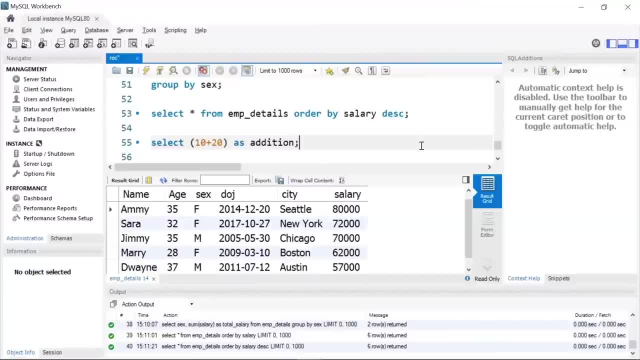 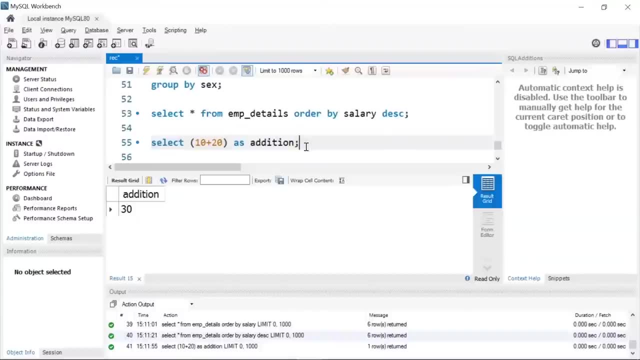 give an alias name as addition. if i run this, it will give me the sum of 10 plus 20 plus 20 plus 20, 10 and 20, that is 30.. similarly, you can use the subtraction operator and you can change the alias name as, let's say, subtract. let's run it, you get minus 10.. 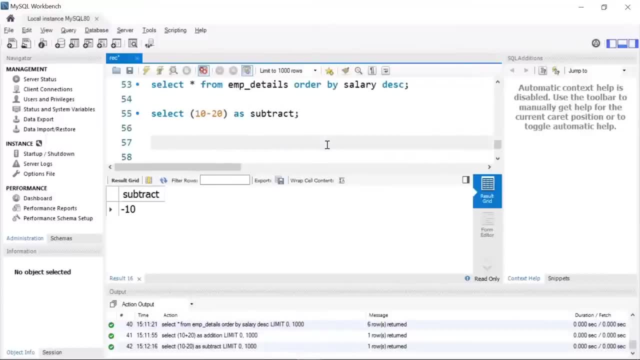 now there are some basic inbuilt functions. there are a lot of inbuilt functions in sql, but here i'll show you a few. suppose you want to find the length of a text or a string? you can use the length function. so i'll write select and then use the length function. i'll hit tab to auto. 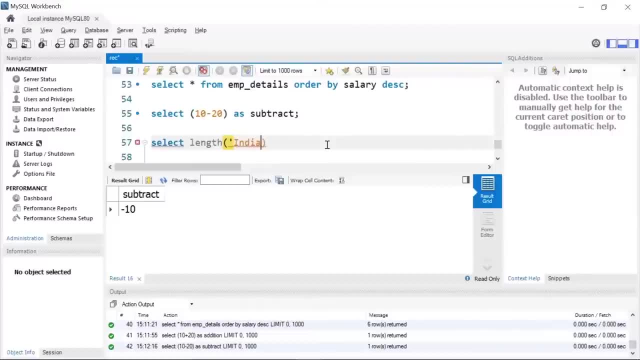 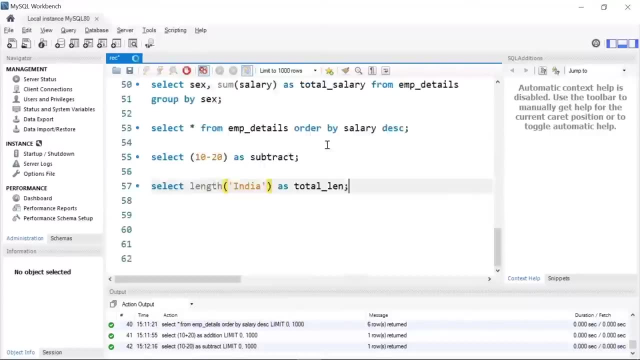 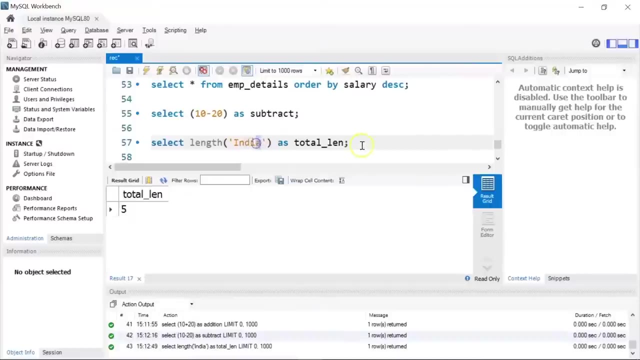 complete. let's say i want to find the length of country india and i'll give an alias as total length. if i run it, you see here it returns five, because there are five letters in india. there's another function called repeat, so let me show you how repeat works. so i'll write. 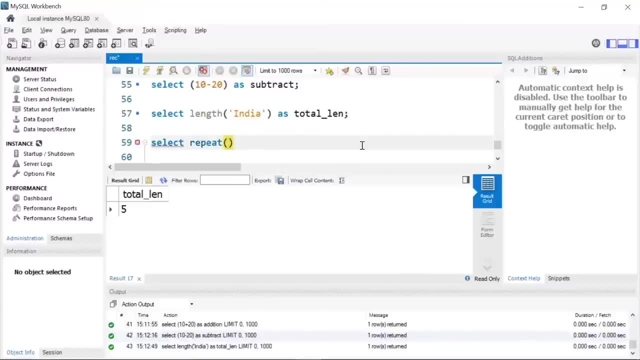 select repeat. let's say i want to repeat the symbol that is at the rate. i'll put it in single quotes because it is a text character and i want to repeat this character for 10 times. close the bracket and let's run it. you can see here in the output it has printed at the rate. 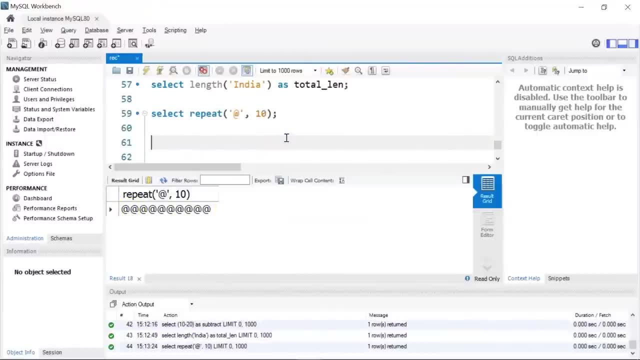 10 times. you can count it all right now. let's say you want to convert a text or a string to uppercase or lowercase. you can do that as well, so i'll write, select and use the function called upper. let's say i want to convert my string, that is, india, to uppercase. i'm not giving in any. 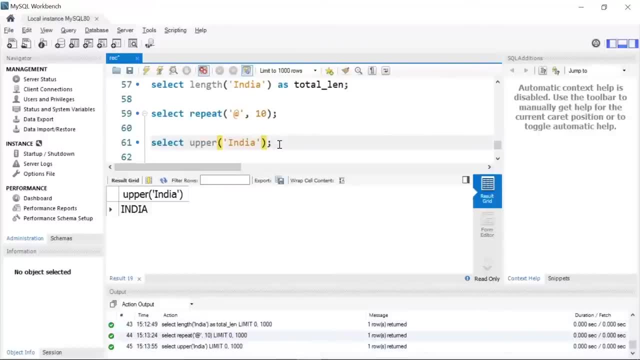 alias name. if i run this, see, my input was capital i and everything else was in small letter. in the output you can see it has converted my input to all caps. similarly, you can change this. let's say you want to print something in lowercase, you can use the. 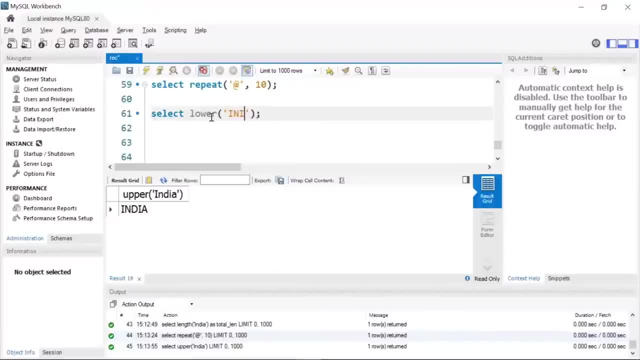 lower function. let's say this time everything is in uppercase. if I run it, it converts India to lowercase. now let's explore a few date and time functions. let's say you want to find the current date. there's a function called cur, which stands for current, and this is the function I'm 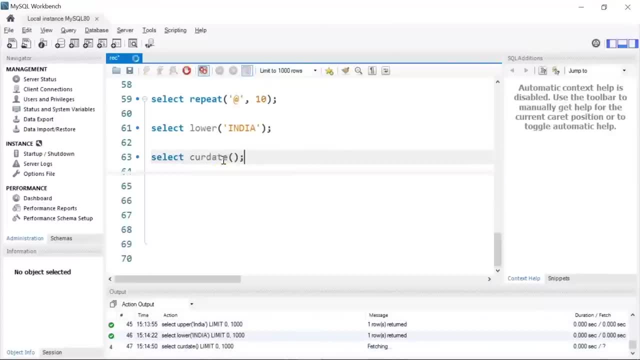 talking about which is current date. if I run this, you will get the current date, that is, 28th of Jan 2021, and let's say you want to extract the day from a date value so you can use the day function. let's say, I'll use day and I want to find the day from my current date. 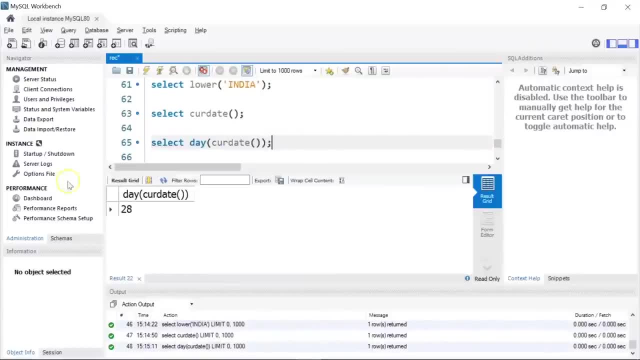 you can use the day function. let's say, I'll use day and I want to find the day from my current date. if I run this, you get 28, which is today's day now. similarly, you can also display the current date and time, so for that you can use a function that is called now, so this will return the current date. 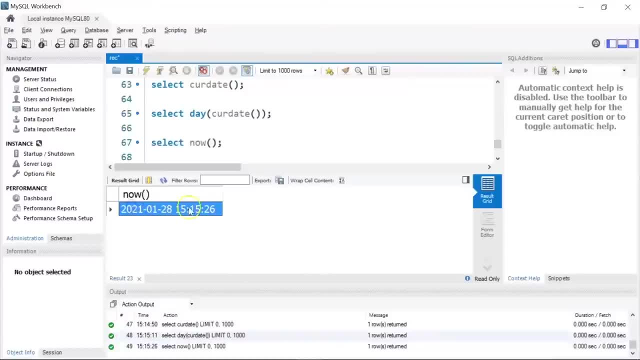 and time. you can see this is the date value, and then we have the current time. all right, and this brings us to the end of our demo session. so let me just scroll through whatever we have used. so let's see what we have used. so let's see what we have used. so let's see what we have used. 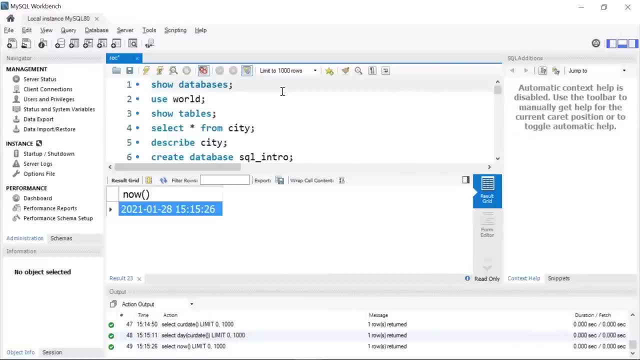 learned. so first I showed you how you can see the databases present in MySQL. then we used one of the databases and checked the tables in it. then we created another database called SQL intro. for our demo purpose we used that database and then we created this table called employee details, with 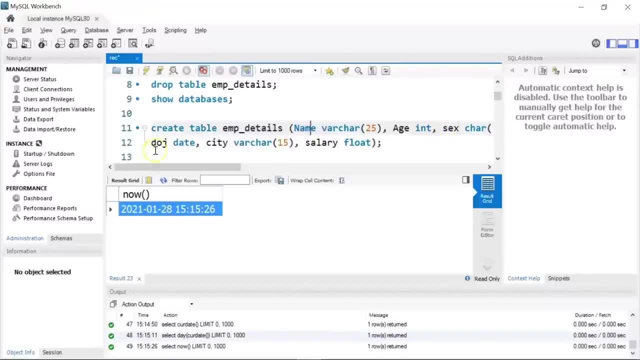 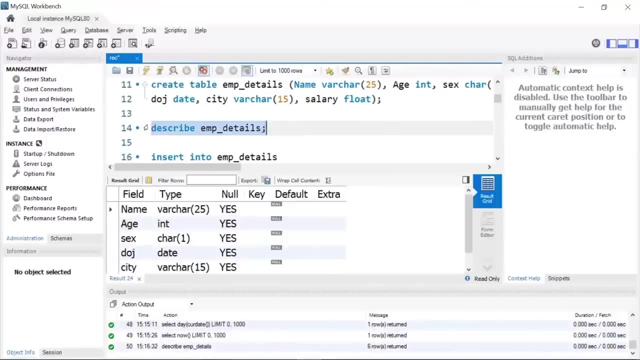 column names like name, integer, the sex, date of join, city and salary. I showed you the structure of the database and then we created another database called employee details, with column database. let me run this again so you get an idea. you can see, this was the structure of our table. 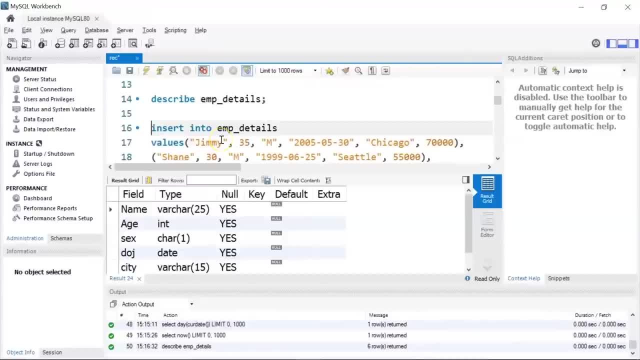 then we went ahead and inserted a few records. so we inserted records for six employees. so you have the employee name, the each, the gender, the date of China, the city to which the employer belongs to and the salary of the employee. then we saw how you can use the select statement and display all. 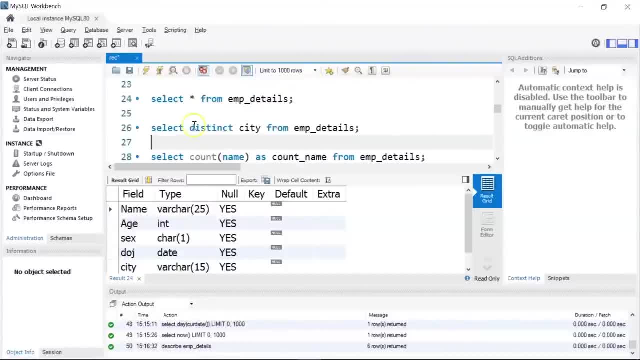 the columns present in the table. we learned how you can display your copyTransfer using SQL arrow, the unique city names. we learnt how to use different aggregate functions like count, average and sum. then we learnt how you could display specific columns from the table. we learnt how to use where clause, then we used an or operator. we 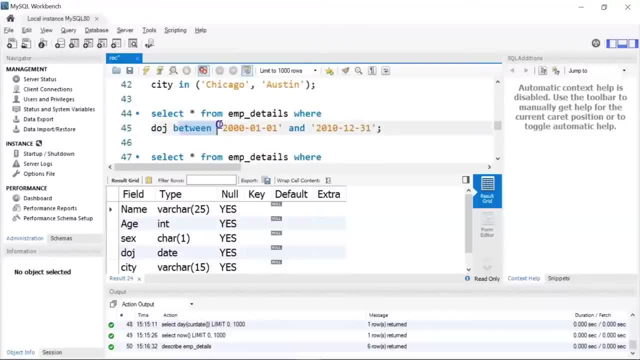 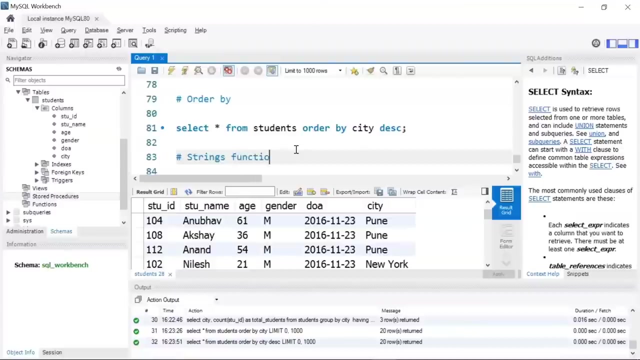 learnt about in operator the between operator. then we used an and operator to select multiple conditions. finally, we learnt about group by order, by, and some basic SQL operations. now it's time to explore some string functions in mysql. so I have given a comment. string functions first. let's say you want to 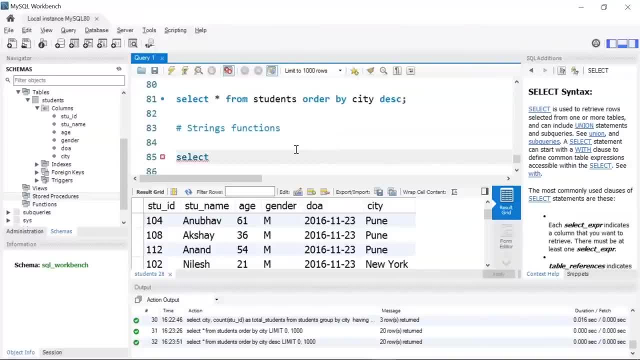 convert a certain string into uppercase so I can write select. the function I use is upper and within this function you can pass in the string. let's say, I'll write India. if you want, you can give an alias name as, let's say, uppercase. I'll give a semicolon and let's run it. there you go. so my input. 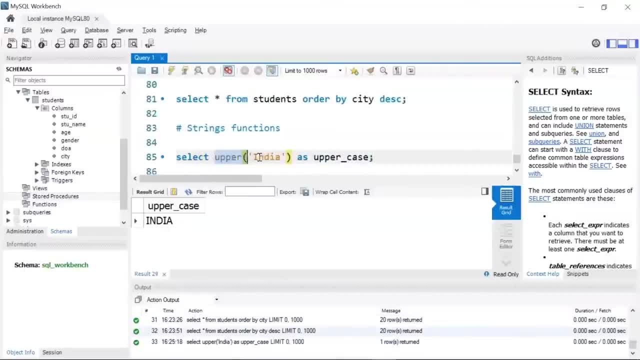 was in sentence case and, using the upper function, we have converted everything into uppercase. similarly, let me just call, copy this and I'll show you. if you want to convert a string into a lowercase, you can use the lower function. I'll run this. you can see the result. everything is in. 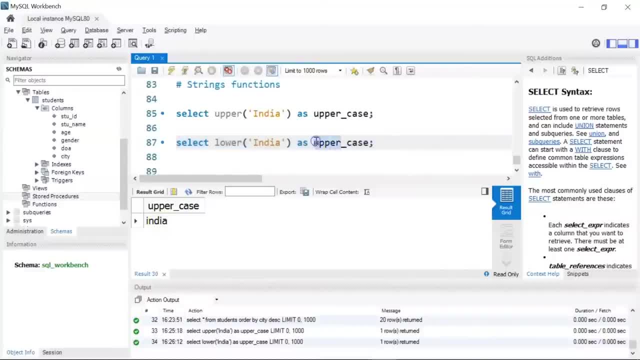 lowercase. now, of course, I need to change the alias name to lowercase now, instead of using lower as the function. there is another function that mysql provides, which is called the lcase. I'll just edit this and write lcase and let's say I'll write india in. 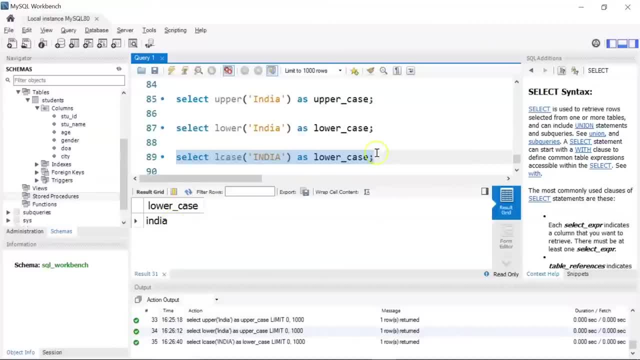 uppercase. let's run it. it returns me the same result. cool. now moving on, let's say you want to find the length of a string. you can use the character length function. I'll write select, use the function character length, and I'm again going to pass it back. so I'm going to pass based on my name as well. so I give it an servir. I'm going toChange the stranger length and passing it into theや. 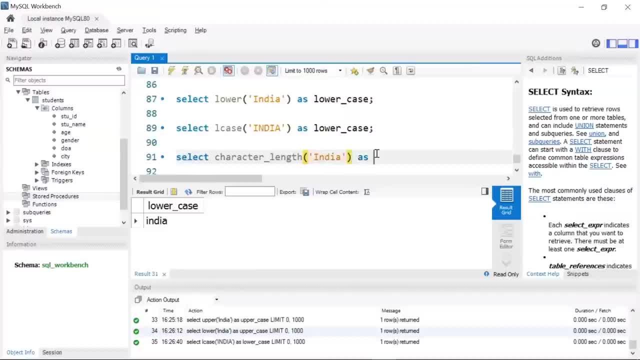 my string as india as, let's say, total length. let's run it this time. i'm going to hit control enter to run my sql command. there you go. it has given us the right result, which is five, because india has five characters in it. now these functions you can also apply. 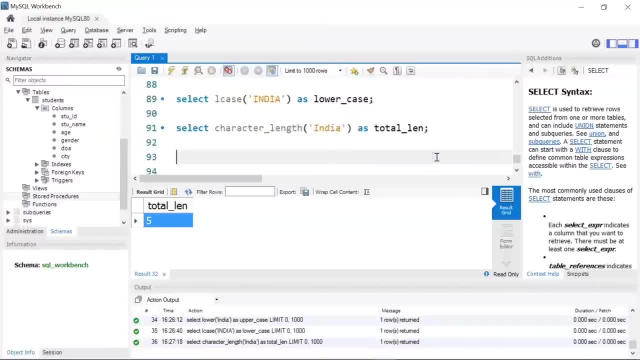 on a table. now let me show you how to do it. let's say we already have the students table and you want to find the length of each of the student names. so here you can pass stu underscore name and you can give the same alias name. let's say total length. 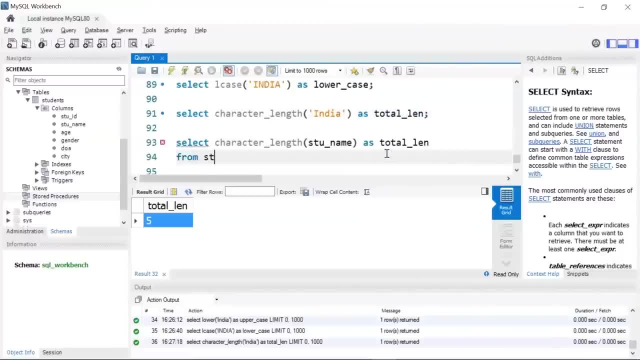 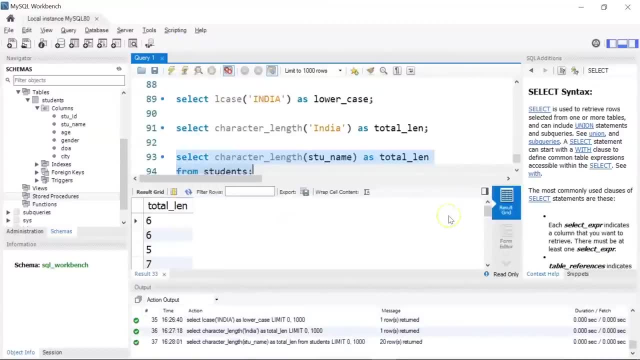 and then you can write from table name that is students. if i run this, you can see the output. it has given me total 20 rows of information. this is not readable actually. let me also display these student names so that we can compare their length. all right, i'll run this again. 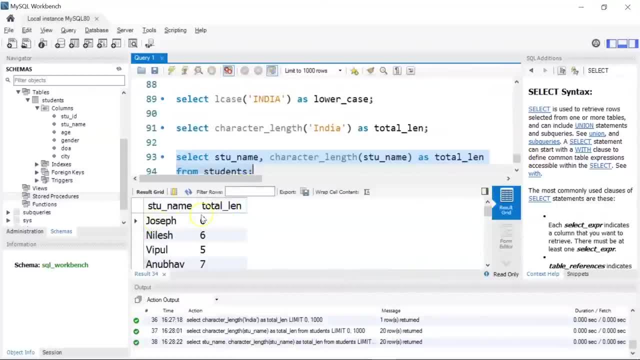 and now you can see the result. so joseph has six characters, niles has six, vipul has five, anubhav has seven. similarly, if you see, akshay has six, tanishka has seven, raghav has six, cummins has seven, rabada has six. 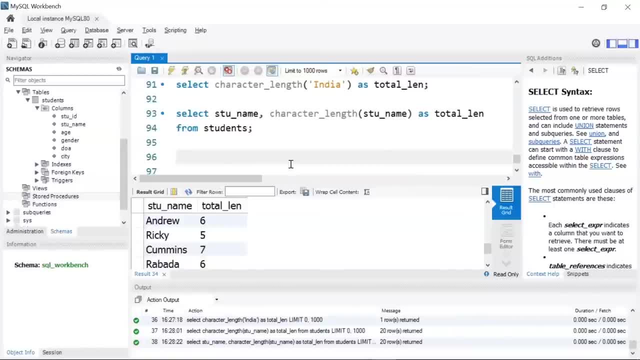 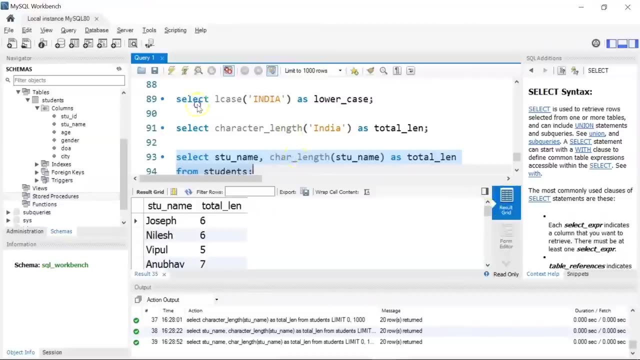 so on and so forth. now, instead of using this character length, you can also use the function char length. it will work the same way. let's see the result. there you go. it has given us the same result. you can either use character length or char length, or you can also use the function char length. 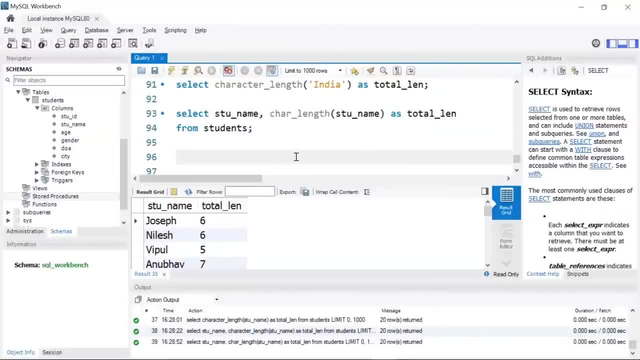 so let's say i have a very interesting function called concat. so the concat function adds two or more expressions together. let's say i'll write select, we'll use the function concatenate. the function is actually concat and i'm going to pass in my string values. let's say india. 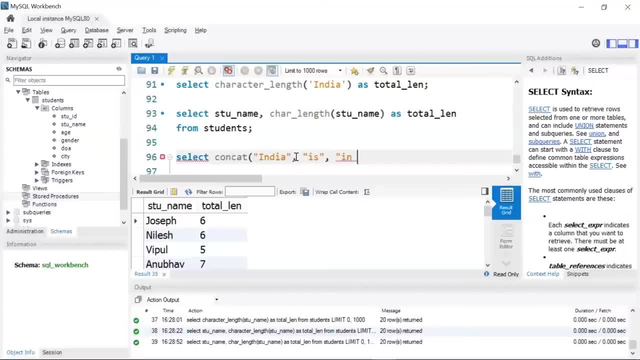 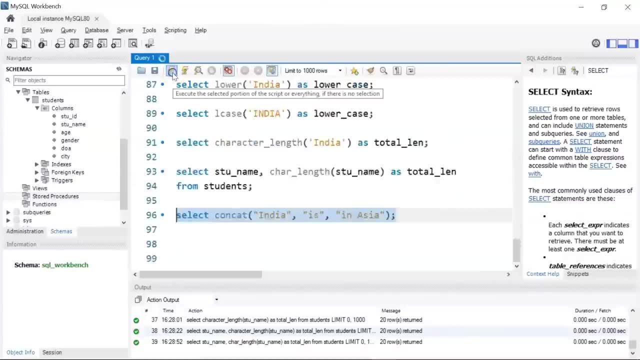 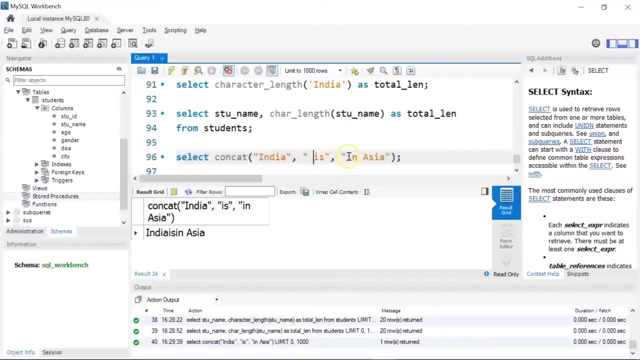 is in asia. let's run this and see our result. you can see here it has concatenated everything. let us make it more readable. i'll give a space in between so that you can read it clearly. now this is much more readable. india is in asia and, if you want, you can give an alias. 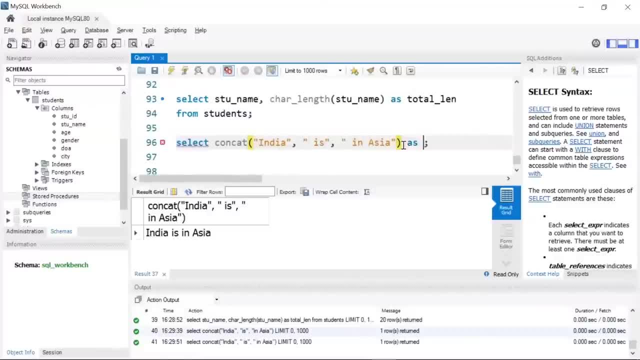 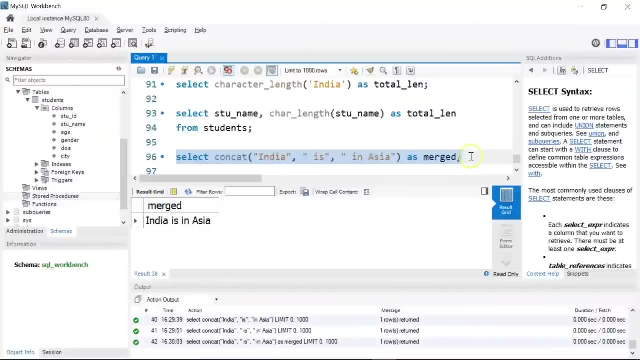 name as well as, let's say, merged, so let's say merge. there you go. now. the same concat operation you can also perform on a table. i'm going to use the same students table. let's say i want to return the student id followed by the student name, and then i am going to merge. 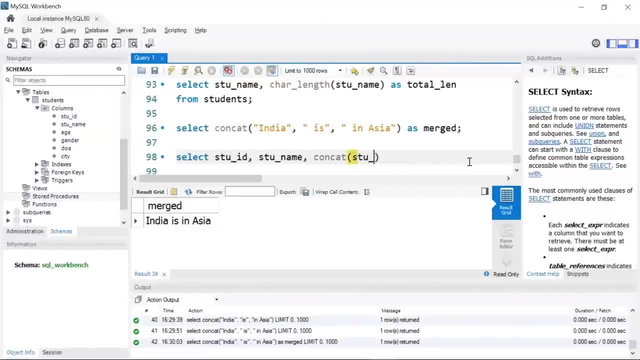 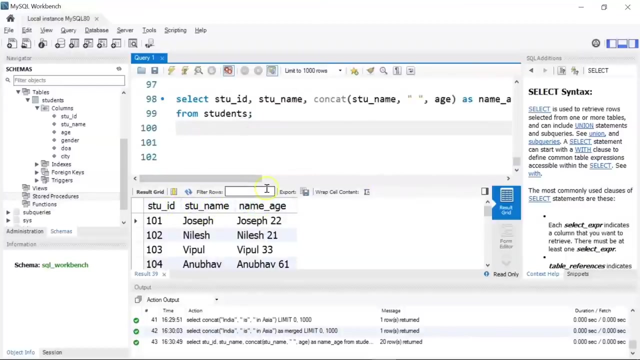 the student name, followed by a space, followed by the age of the student, and i can give an alias as, let's say, name underscore age. from my table, that is, students. let's see how this works. okay, you see, here the result is very clear. we have the student id, the student name and the concatenated column that we 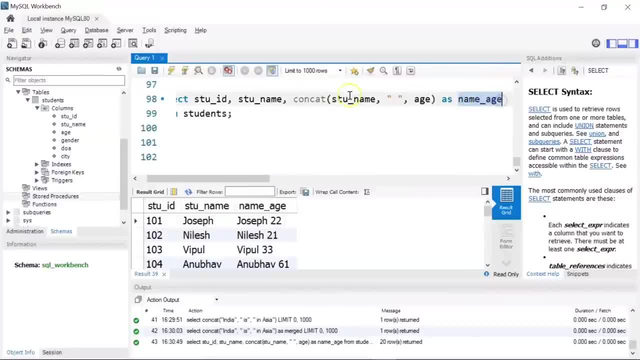 created in the table, which was name underscore age, where we have the student name with a space followed by the age of the student. if i scroll down, you can see the rest of the results. cool, now, moving ahead, let's see how the reverse function works in mysql. 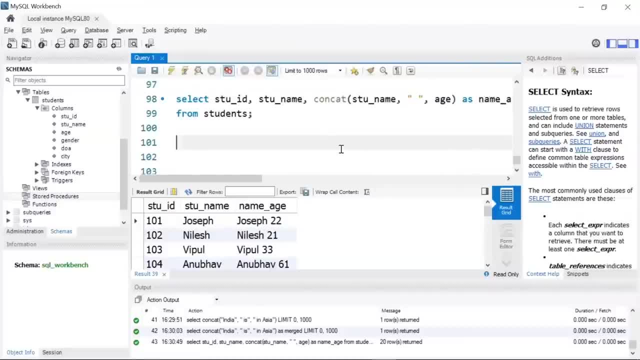 so the mysql reverse function returns a string with the characters printed in reverse order. so suppose i write select reverse, i'll use the same string again. let's say i have india. let's run it. you will see all the characters printed in reverse order. again you can perform. 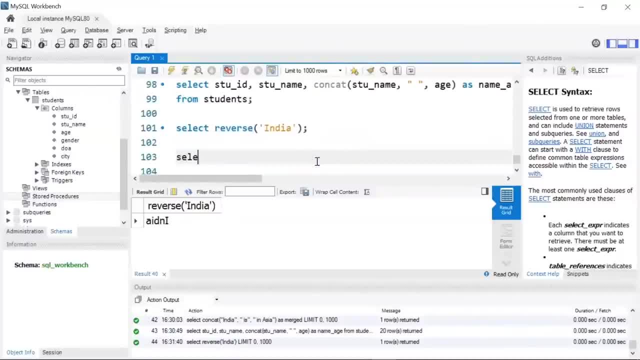 the same operation on a table as well. let's say i'll write select reverse and i'll pass in the column as student name from my table. that is students. let's run it. it gives you 20 students and all the names have been printed in reverse order. okay. 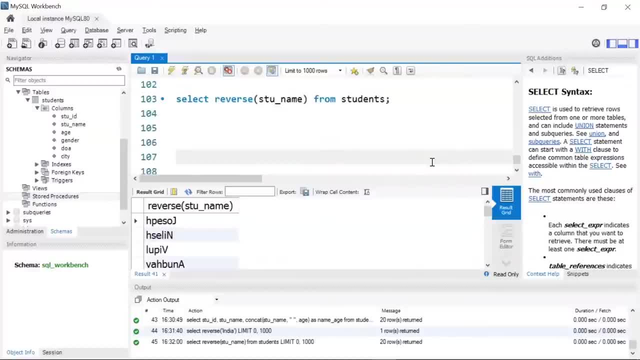 now let's see what the replace function does. so the replace function replaces all occurrences of a substring within a string, within a new substring. so let me show you what i mean. i'll write select, replace. i'll pass in my input string which is, let's say, orange is a vegetable. 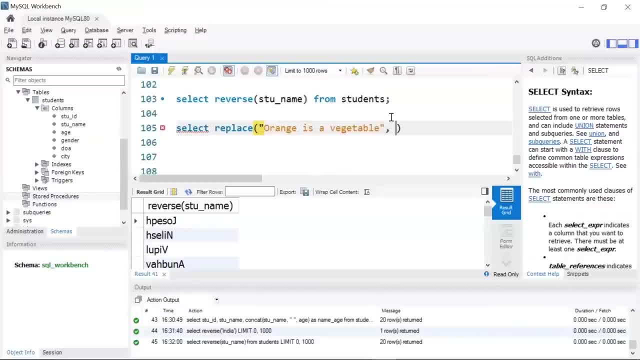 which is ideally incorrect. i am purposely writing this so that i can replace the word vegetable with fruit. okay, so what this replace function does is it will place the does is it is going to find where my word vegetable is within the string, my input string, and it is going to replace my word vegetable with fruit. let's run. 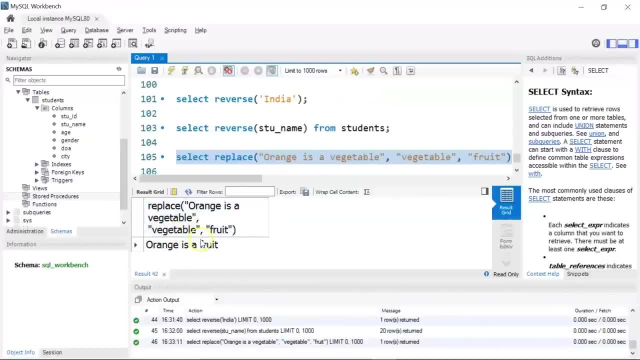 it and see the output. there you go. now. this is correct. which is orange is a fruit. all right, now MySQL also provides some trim functions. you can use the left trim, right trim and just the trim function. so let me show you how this left trim works. left trim or L trim removes the leading space characters. 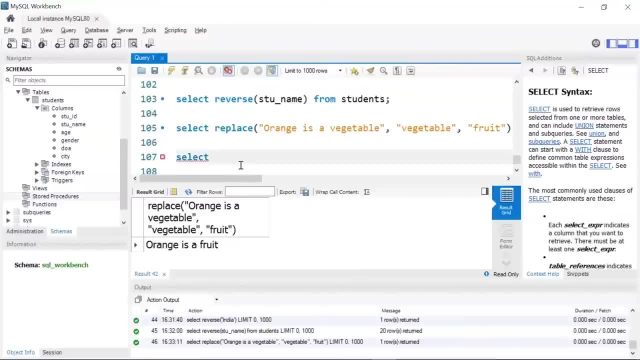 from a string passed as an argument. so say, I write select, I'll use the left trim function, which is L trim, and then I am going to purposely give a few spaces in the beginning of the string. I will give a word, let's say India, and then I: 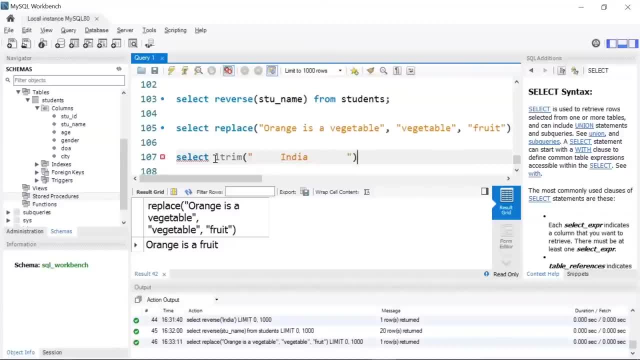 will give some space after the word India and see how the L trim works. if I run this, it gives me India, which is fair enough. but before that, let's first find the length of my string. so I'll use my length function here and within this function I am going to find the length. 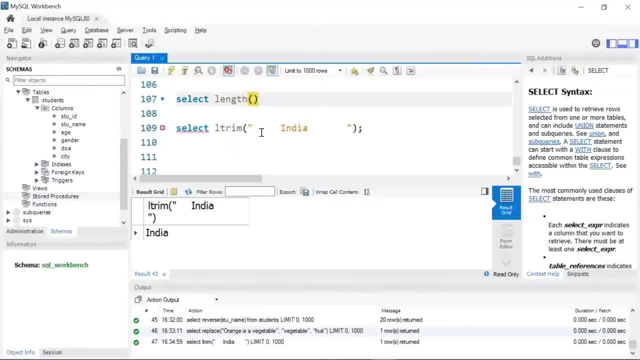 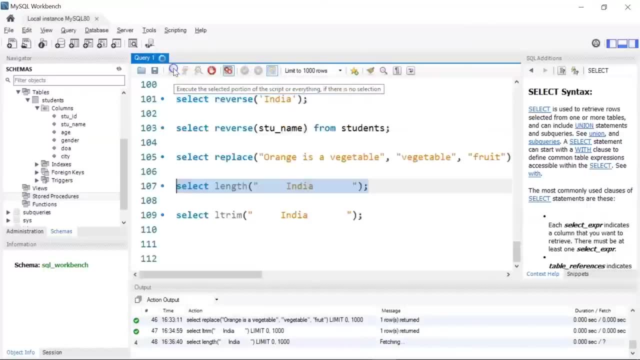 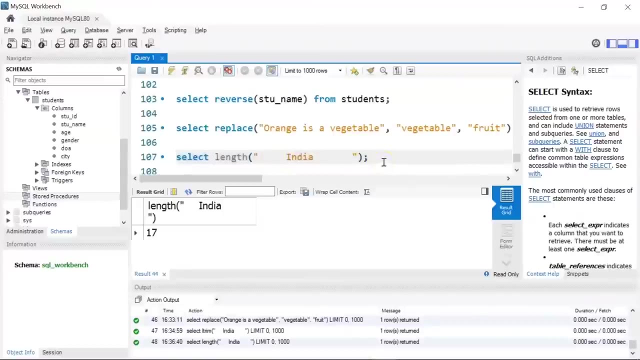 of my string which has India, along with some leading and trailing spaces. I'll paste this here. give a semicolon and I'll run it. okay, so the entire string is 17 characters long, or the length of the string is 17.. now, say I use L trim on my same string, what it returns me is India. 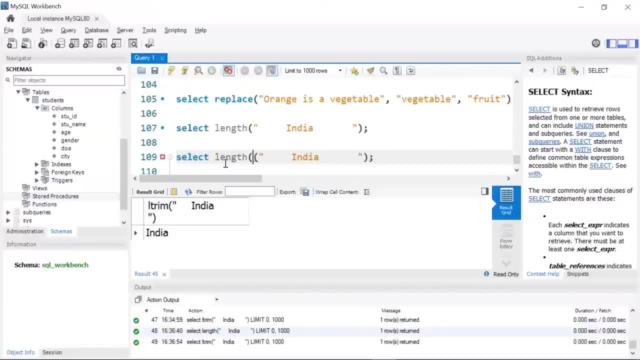 and if I run length over it you can see the difference. as in: you can see how many spaces were deleted from the left of the string. you can see here now it says 17 and I'm going to use L trim. let's see the difference. it gives me 12, the reason. 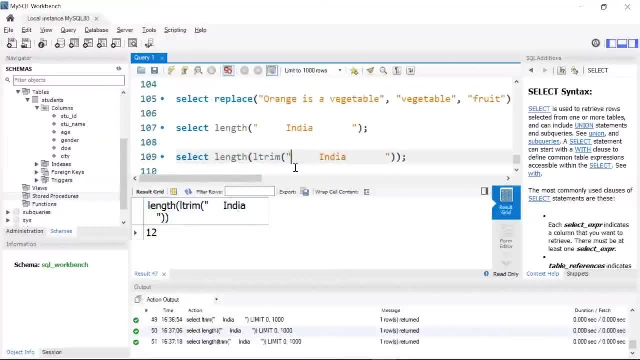 being it has deleted five spaces from the left. you can count it 1, 2, 3, 4 & 5, so 17 minus 5 is 12, which is correct. similarly, you can use the R trim function, which removes the trailing spaces from a string. trailing spaces are these spaces. when you use left trim, it deletes the. 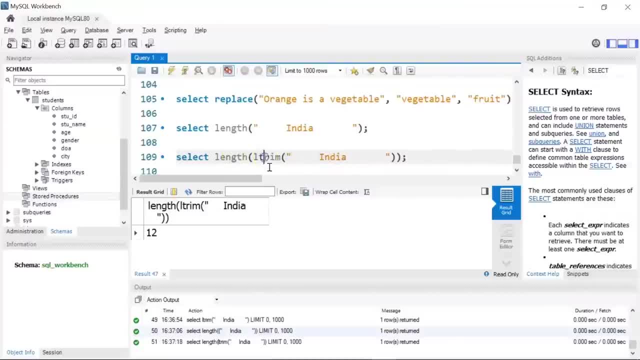 leading spaces, which is this. now let me just replace L trim with R trim, which stands for right trim, and see the result. so the length is 10 now, the reason being: it has deleted seven spaces from the right of the string, if you can count it one. 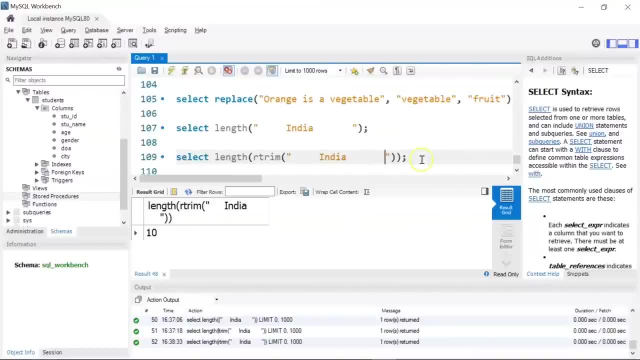 three, four, five, six and seven. cool, you can also use the trim function, which will delete both the leading and the trailing spaces. so here, if I just write trim and I'll run it, it gives me five, because India is total five characters long and it has deleted all the leading and the trailing spaces. all right, 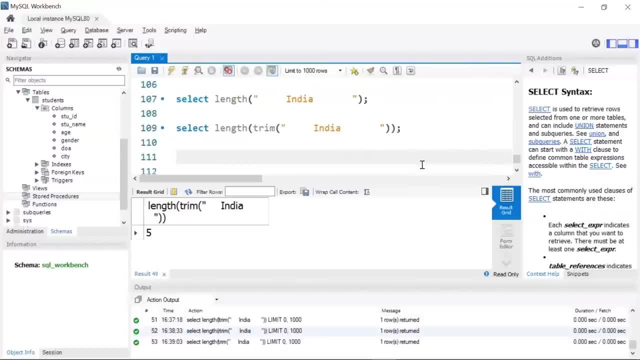 there's also a function called position. in mysql. the position function returns the position of the first occurrence of a substring in a string. so if the substring is not found with the original string, the function will return zero. so let's say I'll write select position I. 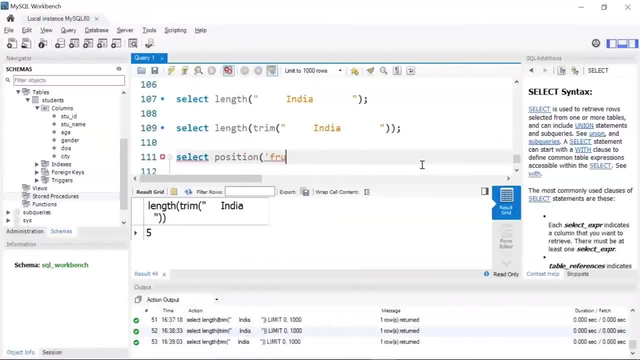 want to find where fruit is in my string, that is, orange is a fruit. I'll give an alias as name. the some error here. it should be within double quotes. now let's run it and see the result. okay, it says at the 13th place or at the 13th position. 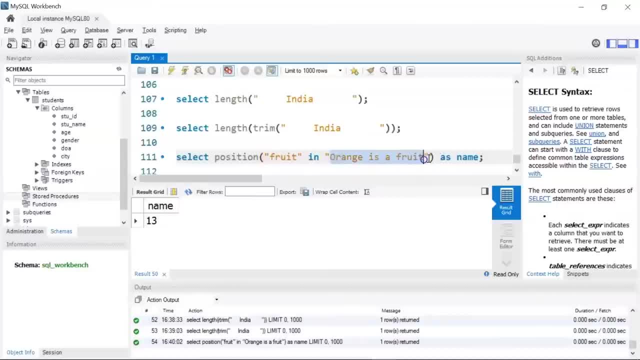 we have the word fruit in our string, which is oranges of fruit. now the final function we are going to see is called ASCII. so the ASCII function returns the ASCII value for a specific character. let's say I write select ASCII of the letter small a. if I run this, it will give me the ASCII value, which is 97. let's 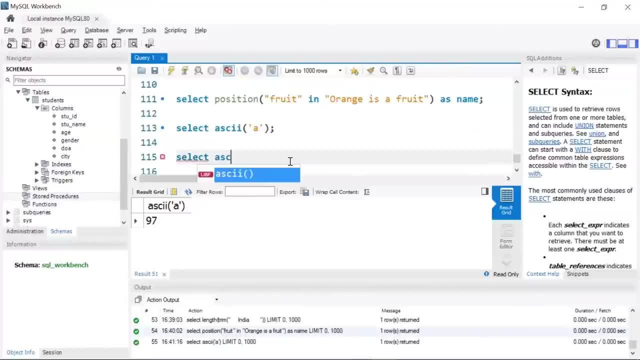 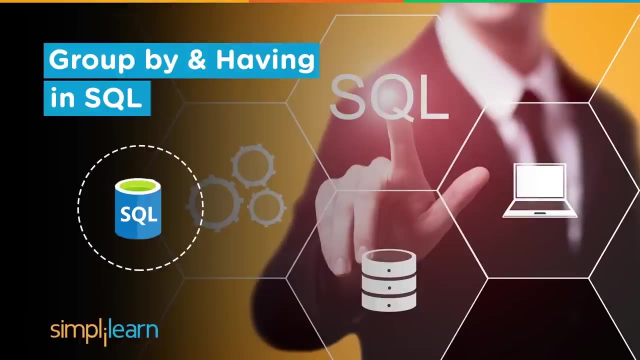 say you want to find the ASCII value of 4, let's see the result: it gives me 52. alright, in this session we are going to learn two important SQL statements or clauses that are widely used, that is, group by and having. first we'll understand the basics of group by and having and then jump into my sequel. 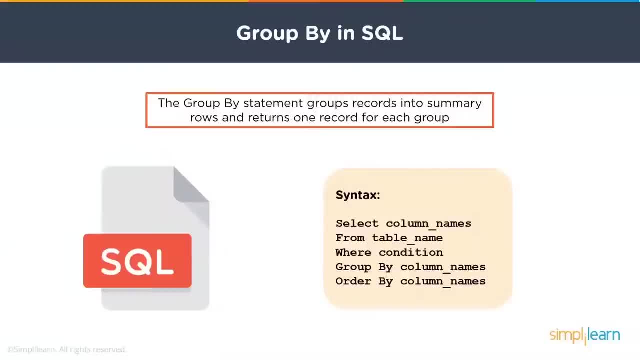 workbench to implement these statements. so let's begin first. what is group by in SQL? so the group by statement or clause groups records into summary rows and returns one record for each group. it groups the rows with the same group by item expressions and computes aggregate functions for the resulting group a. 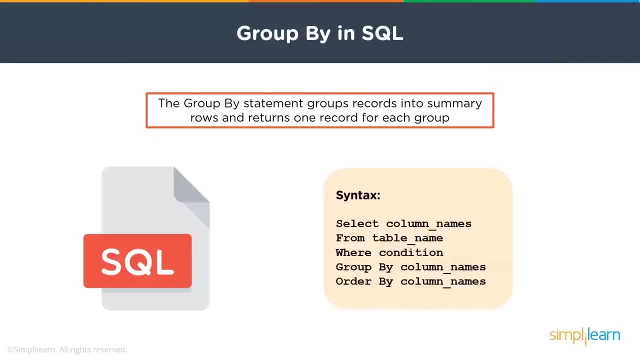 group by clause is a part of select expression. in each group, no two rows have the same value for the grouping column or columns. now below you can see the syntax of group by statement and clause by. so first we have the select statement and then followed by the column names that we want to. 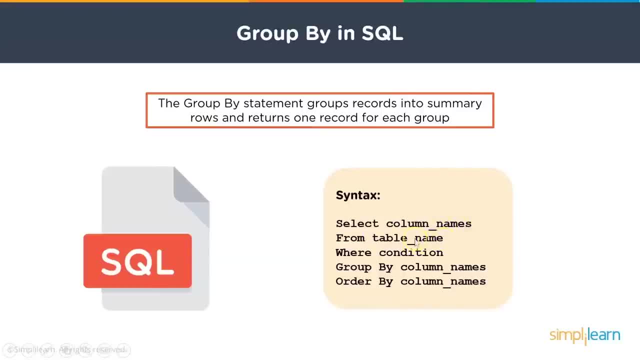 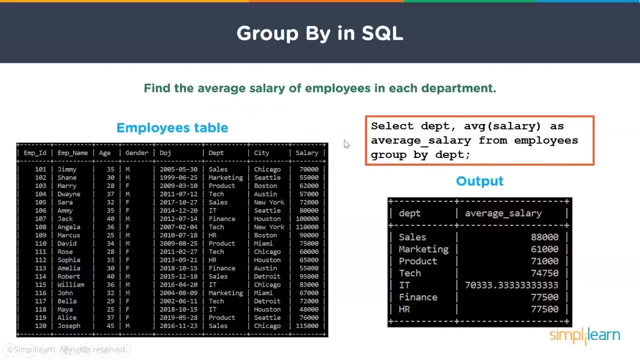 select from. we have the table name, followed by the where condition, and next we have the group by clause and here we include the column names. finally, we have the order by and the column names. now here is an example of the group by clause. so we want to find the average salary of employees. 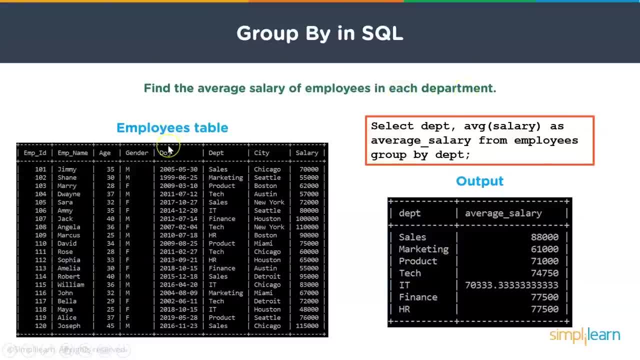 for each department. so here you can see. we have the employees table. it has the employee id, the employee name, the age of the employee, we have the gender, the date on which the employer joined the company. then we have the department to which each of these employees belong to. we have the city to. 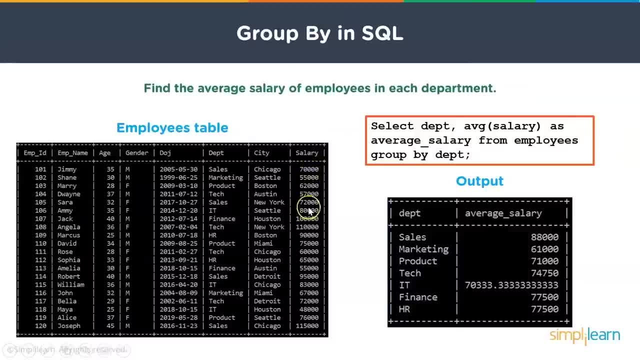 which the employees belong to, and then we have the salary in dollars. so actually we'll be using this employees table on mysql workbench as well. so if you were to find the average salary of employees in each department, so this is how your sql query with group by clause would look like. so we have. 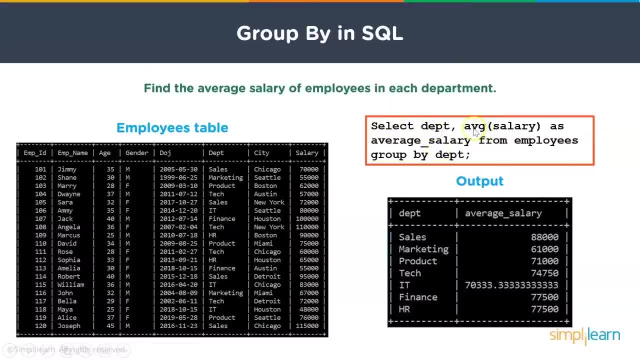 selected department and then we are using an aggregate function that is avg, which is average, and we have chosen the salary column and here we have given an alias name which is average, underscore salary which appears in the output you can see here from employees, and we have grouped it. 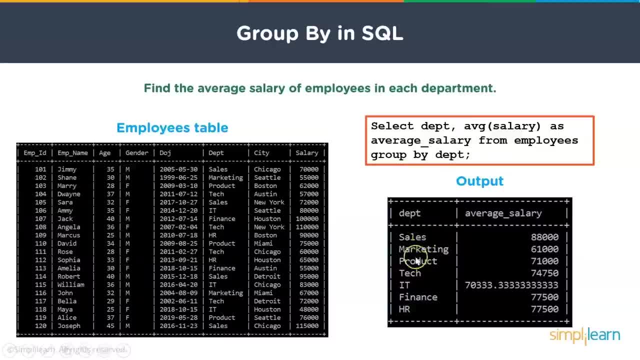 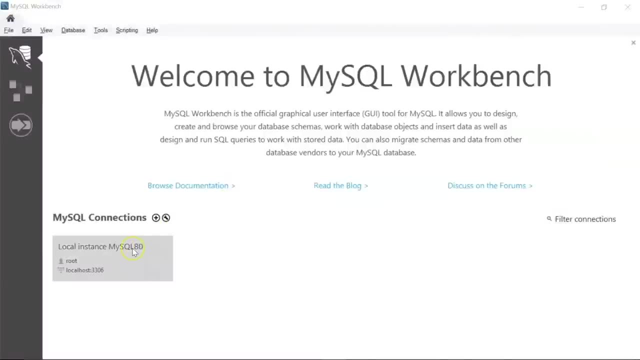 by department. so here in the output you can see we have the department names and the average salary of the employees in each department. now let me take you to my mysql workbench, where we will implement group by and solve specific problems. okay, so i am on my mysql workbench, so let me 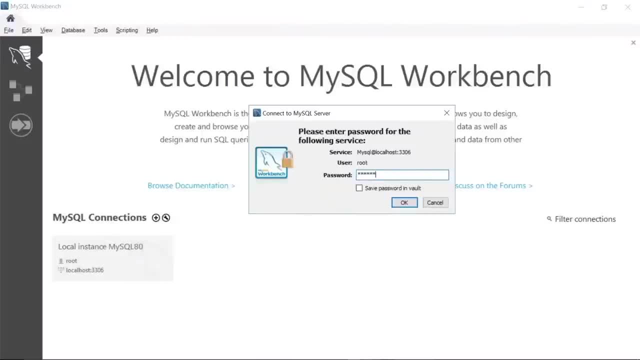 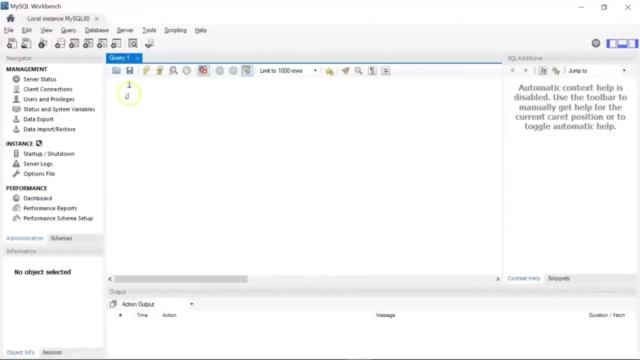 make my connection. first i'll enter the password so this will open my sql editor. so first of all let me check the databases that i have. so i'll use my query, that is, show databases. let's run it. okay, you can see we have a list of databases here. 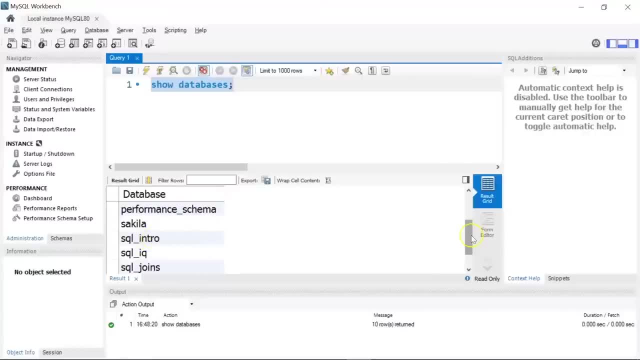 i'm going to use my sql underscore intro database so i'll write use sql underscore intro. so this will take us inside this database. i'll run it all right now. you can check the tables that are present in sql underscore intro database. if i write show tables, you can see the list of tables that are already present in this database. 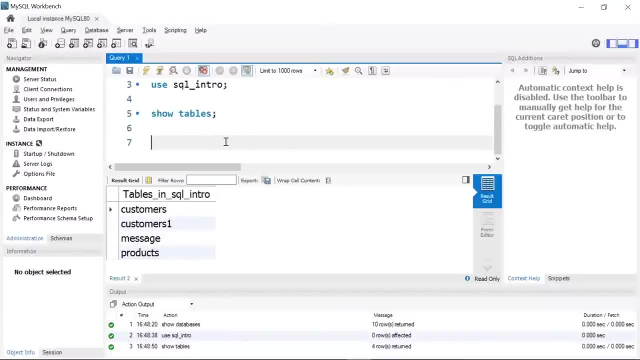 to do our demo and understand group by as well as having let me first create an employee table. so i'll write create table- employees. next i'll give my column name as employee underscore id, which is the id for each employee. i'll give my data type as 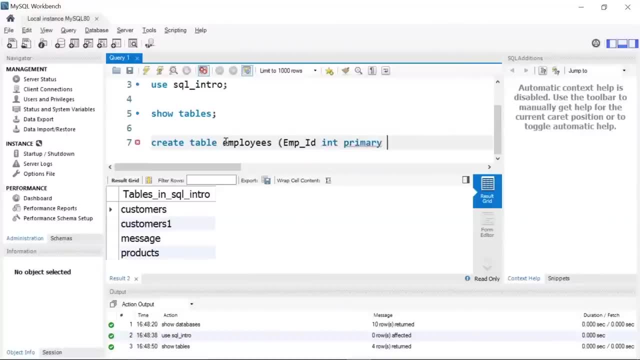 integer and i'll assign employee id as my primary key. next, i'll give employee underscore name and my data type would be var car i'll give the size as 25. my third column would be the age column. age would obviously be an integer. then i have 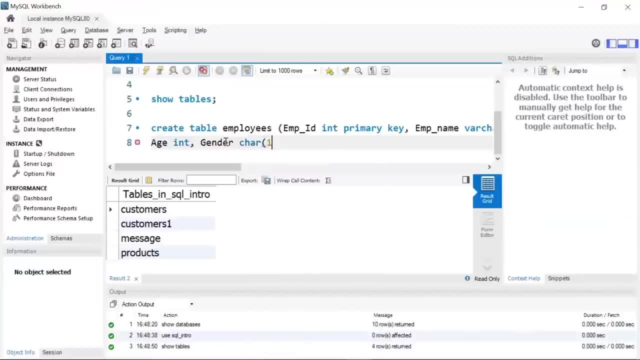 my gender column. i'll use character data type and assign a value of one or size of one. next we have the date of join and the data type will be date. we have the department column as well. this is going to be of varkar and 20 will be the size. 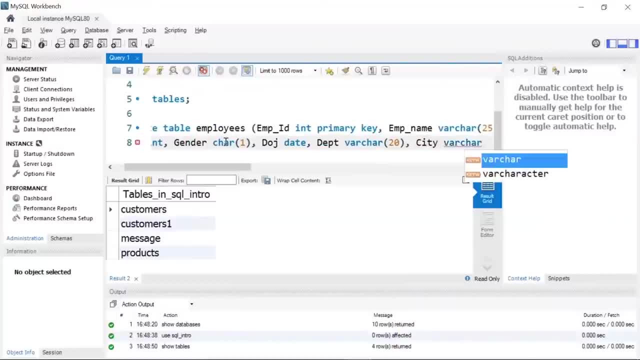 next, we have the city column, which is actually the city to which the employee belongs to, and finally, we have the salary column, which will have the salary for all the employees. okay, now let me select and run this. you can see, here we have successfully created our table. 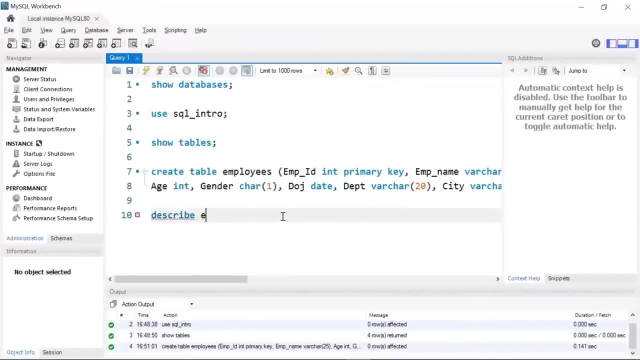 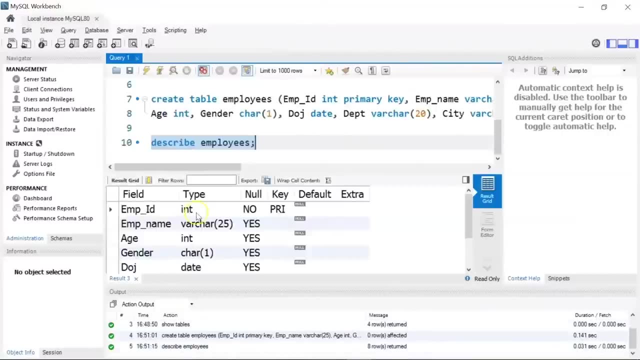 now to check if our table was created or not, you can use the describe command. i'll write: describe employees. you can see the structure of the table so far. all right. now it's time for us to insert a few records into this employees table, so i'll write. 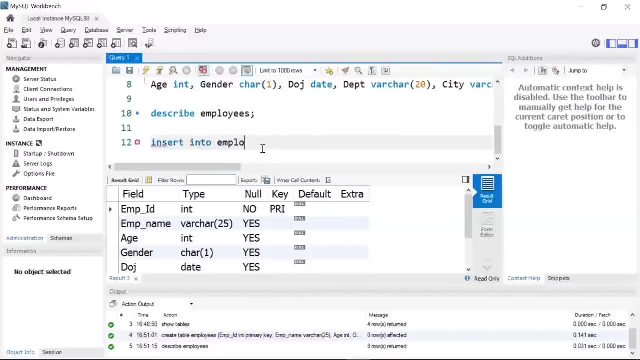 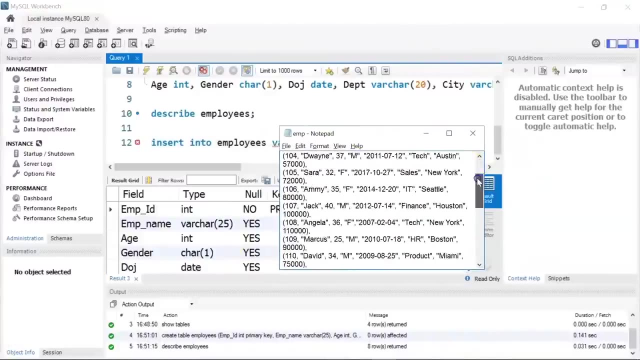 insert into employees and i'll copy paste the records which have already written on a notepad. so let me show you. so this is my emp notepad and you can see i have already put the information for all the employees. so let me just copy this and we'll paste it here. 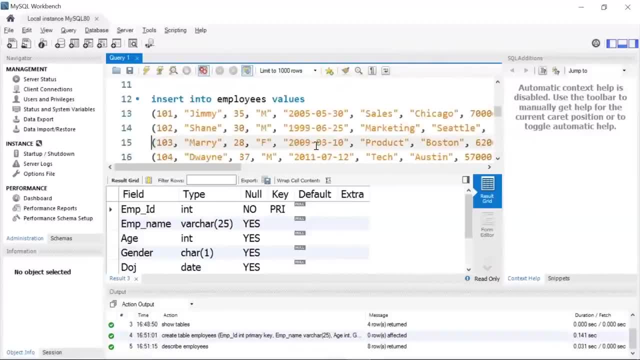 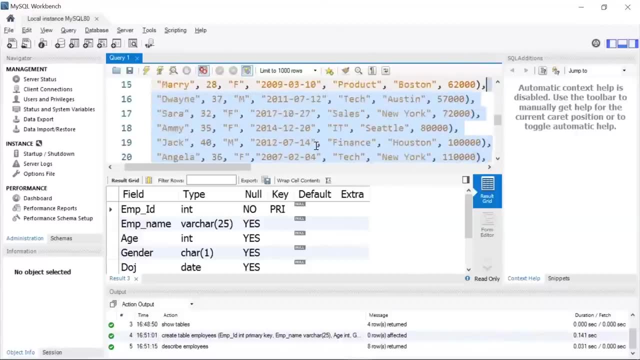 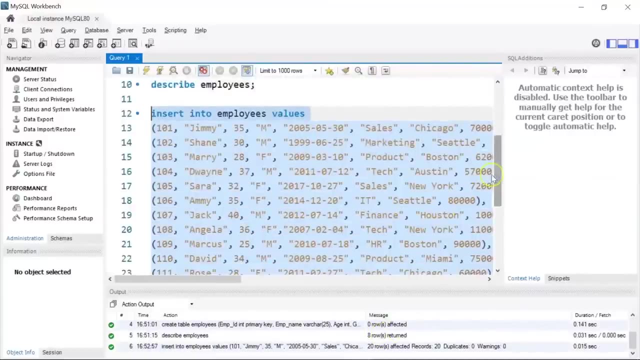 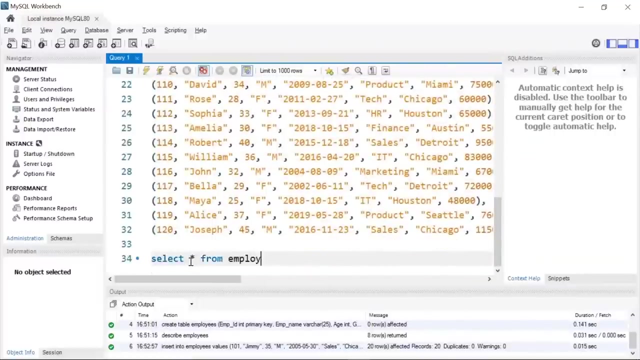 all right, let me go to the top and verify if all the records are fine. all right, so let's run our insert query. okay, so you can see here we have inserted 20 rows of information and now let's check the table information or the records that are present in our employees table. 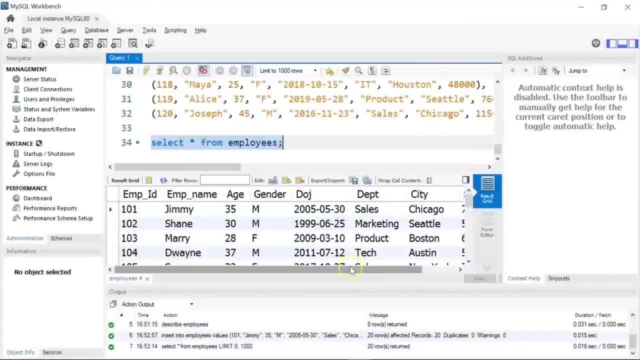 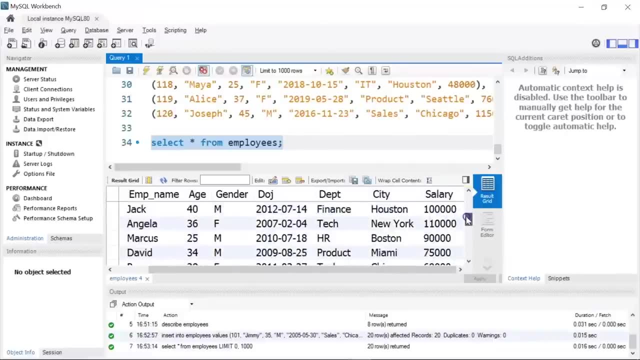 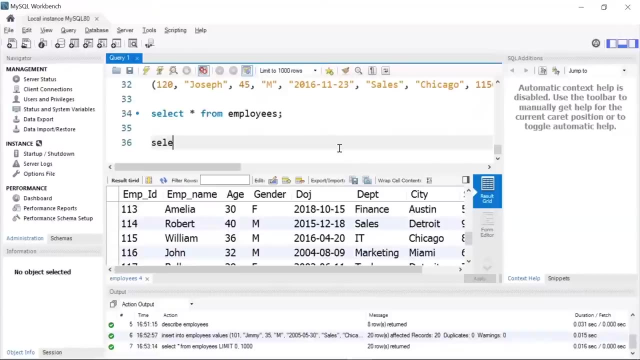 i'll write select star from employees. if i run it you can see here. i have my employee id, the employee name, age, gender, we have the city salary and in total we have an employeerat here. so let's have inserted 20 records. now let me run a few sql commands to check how the structure of our table 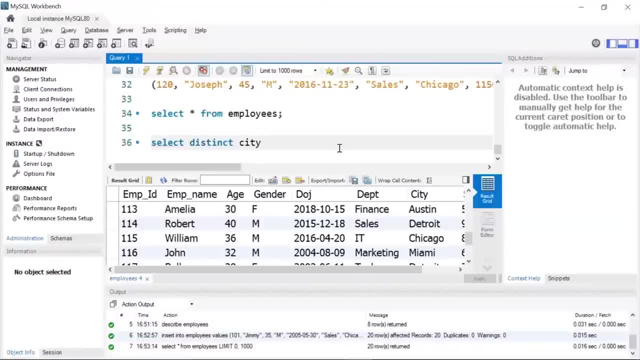 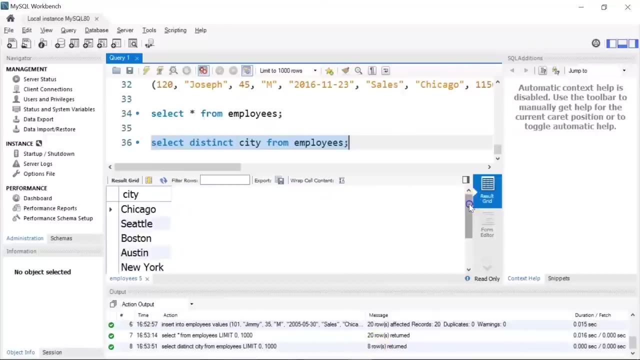 is, let's say, i want to see the distinct cities that are present in our table, so i'll write select distinct city from employees. if i run this, you see here there are total eight different cities present in our employees table. so we have chicago, the chattel, boston, we have new york. 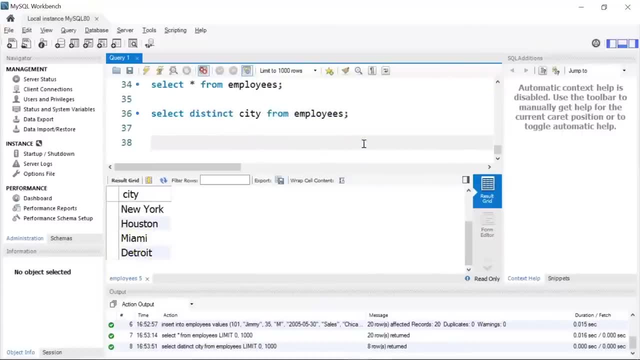 miami and detroit as well. now, let's say you want to know the total number of departments that are present so you can use distinct department. if i run this all right, you can see we have seven rows returned and here are the department names. so we have. 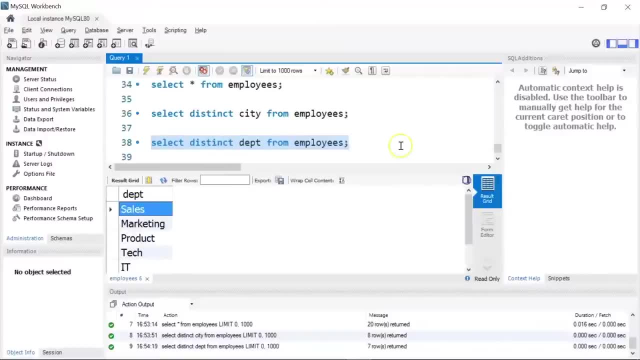 sales, marketing, product tech, it, finance and hr. all right now let me show you another sql command. now this is to use an aggregate function. so i want to find the average age of all the employees from the table, so i can write select avg, which is the aggregate function for average. inside that, i have passed my 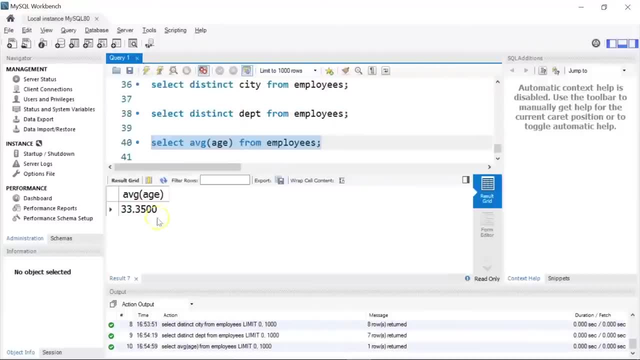 age column from employees, if i run this. so the average age of all the employees in our table is 33.35. now say you want to find the average age of employees in each department. so for this you need to use the group by clause. i'll give a comment here. i want to find the average age in each department. 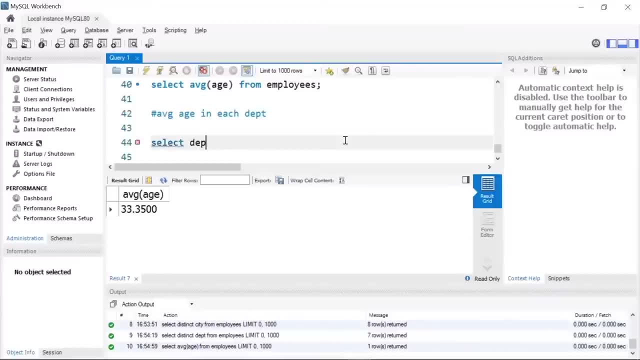 so I'll write select department comma. I'll write average of age from employees group by department. now if I run this you can see here we have our seven departments on the left and on the right you can see the average age of employees in each of these departments. now you can see here in the output it says AVG of. 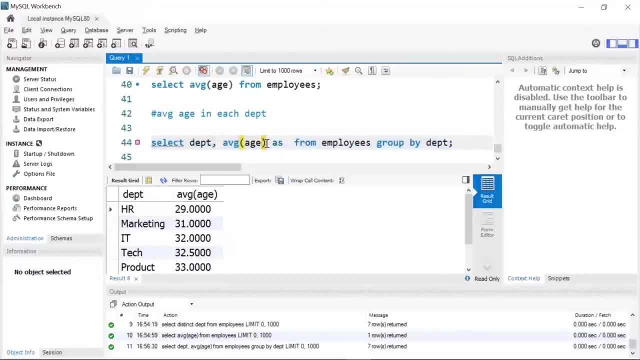 age, which is not readable, so I can give an alias name as average age. all right, I can bring this down and if you want, you can round the values also so you can round the decimal place. so I'll use a round function before the average function and the round function. 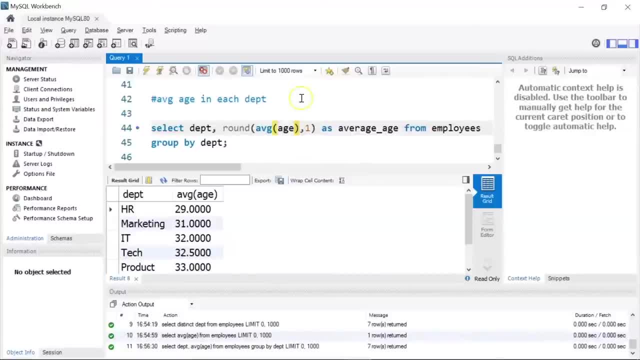 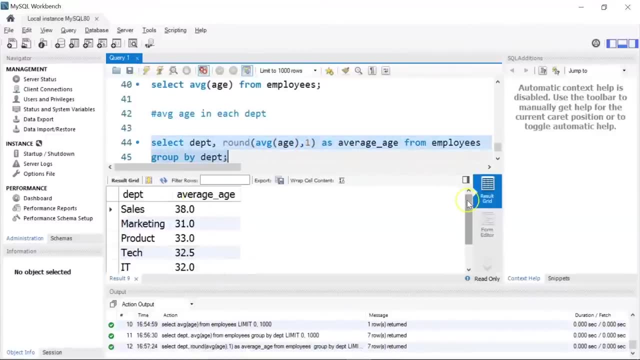 takes two parameters. one is the variable and the decimal place you want to round it to. so if I run this, there you go. you can see. here we have the average age of all the employees in each of these departments. all right, now, suppose you want to find the total salary of all the employees for each department, so you can. 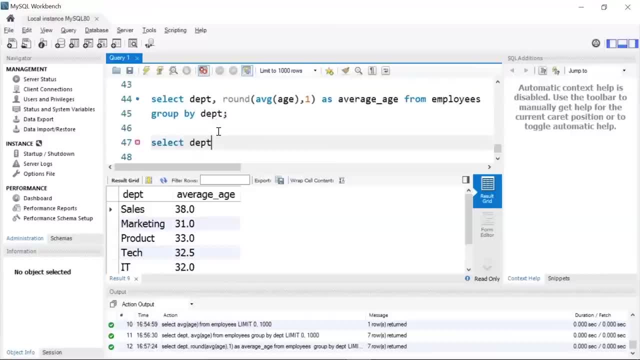 write select department comma. now I want the total salary, so I'll use the sum function and I'll pass my column as salary from employees group by department. let's run this query. you can see here in the output we have the different departments and on the right you can see: 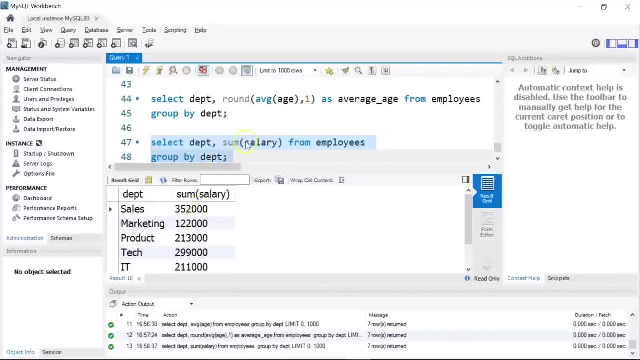 the total salary of all the employees in each of these departments. now, here also, you can give an alias name as total underscore salary. let's run it again and you can see the output here: all right now, moving ahead. you can also use the output here: all right now, moving ahead, you can also. 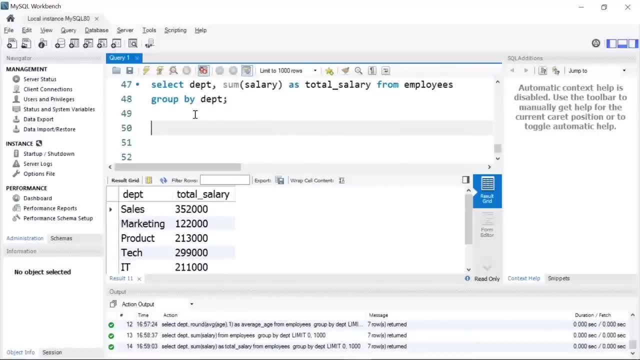 use the order by clause along with the group by clause. let's see, you want to find the total number of employees in each city and group it in the order of employee ID. so to do this I can use my select query. I'll write select count of. 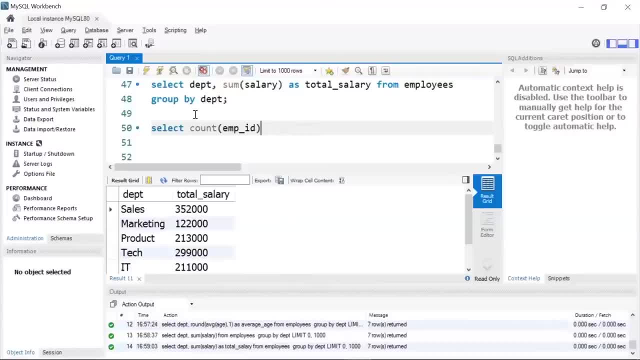 let's say employee ID, and I want to know the city as well, from employees group by city. and next you can use the order by clause. I'll write order by count of employee ID and I'll write DESC, which stands for descending. if I run this query, you can see here on the left you have the count. 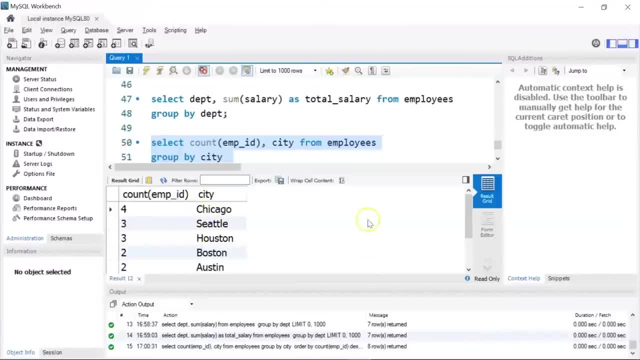 of employees and on the right you can see the city names. so in Chicago we had the highest number of employees working, that was four. then we had Seattle, Houston, Boston, Austin and the remaining also had two employees. so in this case we have ordered our result based on the count of employee ID, in descending order. 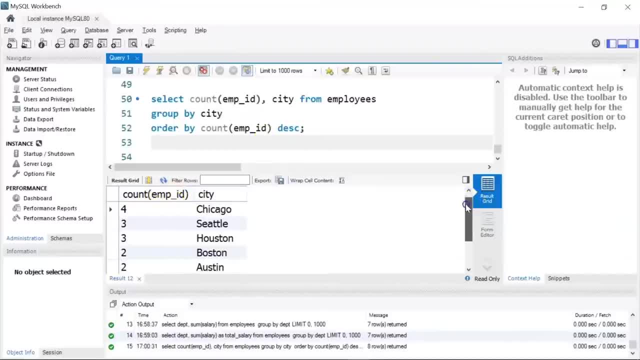 so we have the highest number appearing at the top and then followed by the lowest. okay, now let's explore another example. suppose we want to find the number of employees that joined the company each year. we can use the year function on the date of joining column. then we can count the employee IDs and 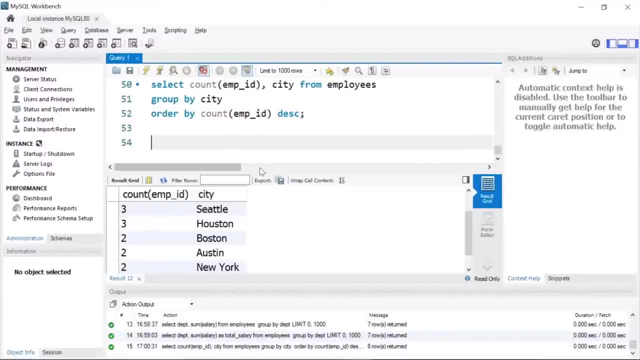 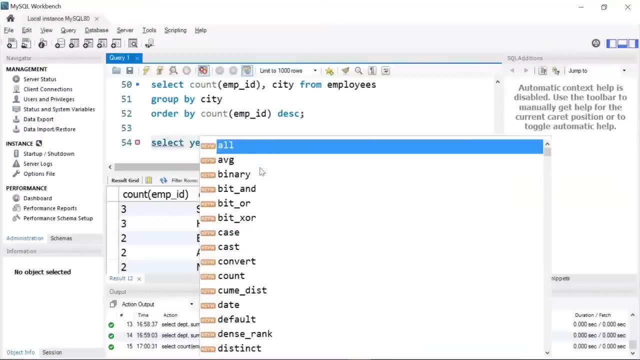 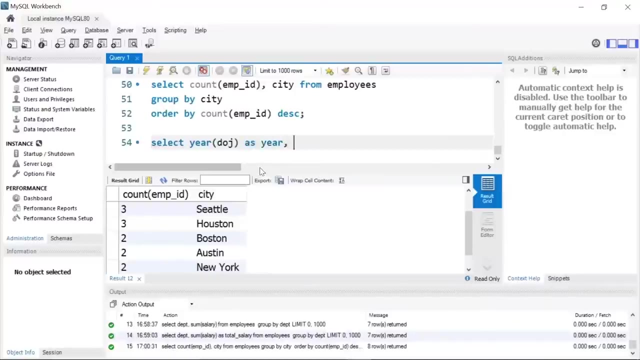 group the result by each year. so let me show you how to do it. so I'll write select. I'm going to extract year from the date of join column. I'll give an alias as year. next I'll count the employee ID from my table name, that is employees, and I am going to group it by. 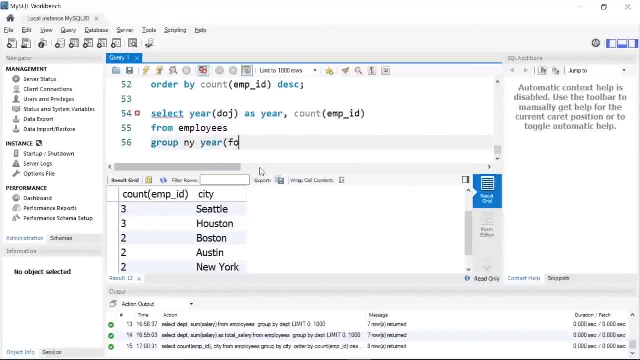 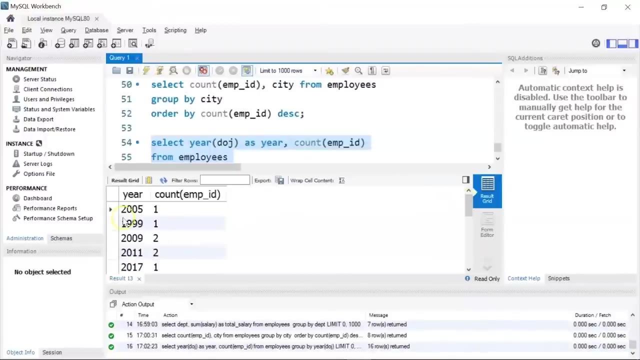 year, date of join. here is a semicolon. alright, so let's run this grid. you see, here in the result we have the year that we have extracted from the date of join column and on the right you can see the total number of employees that joined the company each year. so we have in 2005. 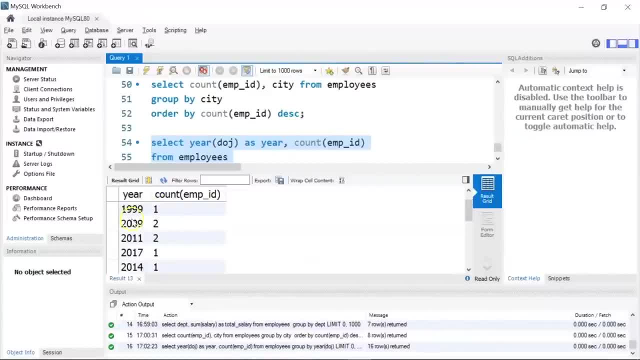 two hours gone away, one employee. similarly we have in 2009. there were two employees. if i scroll down, you have information of other years as well. if you want, you can order this as well based on year or count. okay, now you can also use the group by. 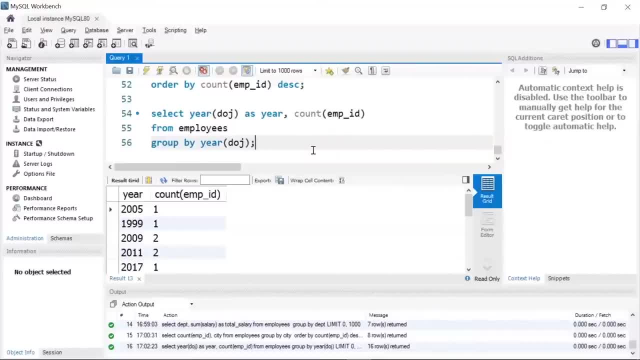 to join two or more tables together. so to show you this operation, let me first create a sales table. so I'll write create table sales and the sales table will have columns such as the product ID, which is going to be of integer type. then we have the. 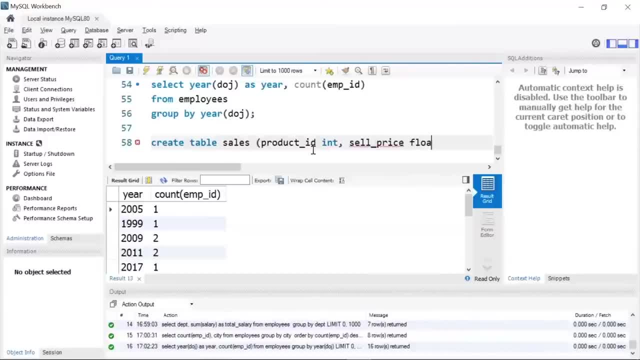 selling price of the product. now this will be a, a float value. then we have the quantity sold for each of the products, so I'll write quantity. quantity will be of integer type. next we have the state in which the item was sold and state. I'll put it as: 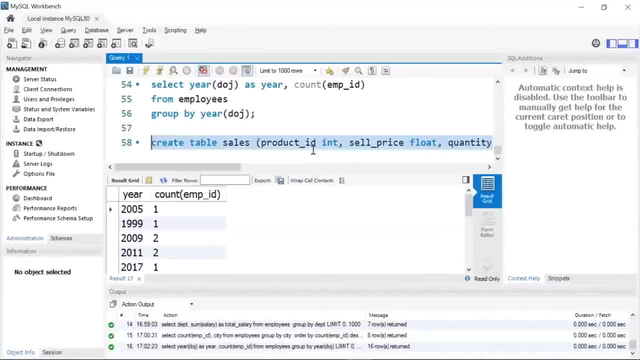 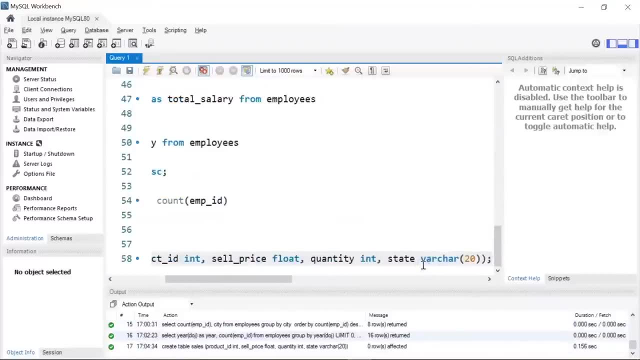 worker and give the size as 20. let's run this so that we'll create our sales table. alright, so we have successfully created our sales table. next, we need to insert a few values to our sales table. so I've already written this table as a sales table and I've already written this table as a sales table. 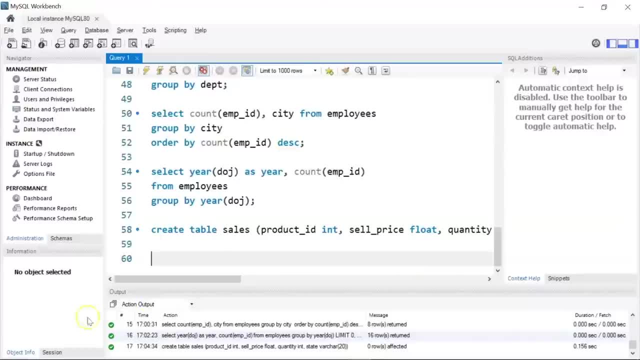 so I've already written this table as a sales table. so I've already written this table as a sales table. so the goal here is that we have to product to is 10 and 1, and then we have to query it and then we have to. 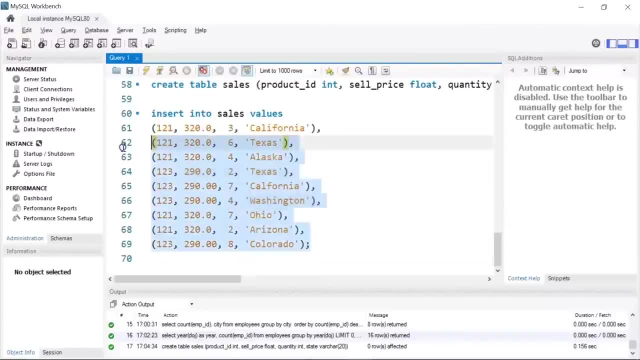 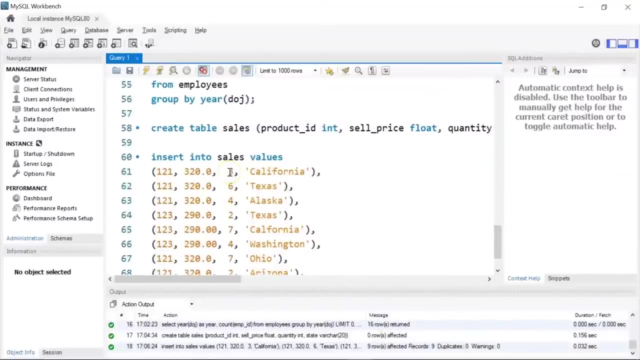 type ans, t and then we write our standard inside the rules and then we've got all our queries and then we've got all the things that we've writen over this table. so let me just run it through what we have inserted. so the first column is the. 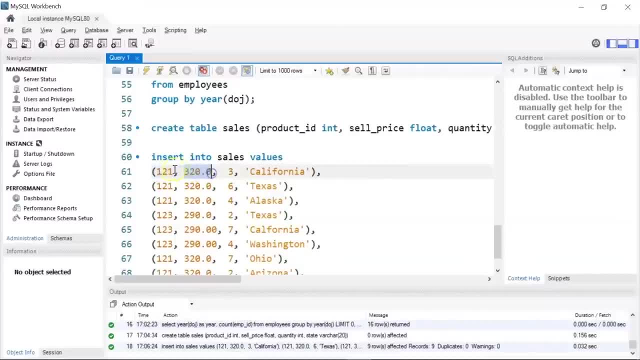 product ID column. then we have the selling price at which this product was sold. then we have the quantity that was sold and in which state it was sold. so we have California, Texas, Alaska. then we have another product ID which is 1, 2, 3, and these are the states in which the products were sold. so let me just 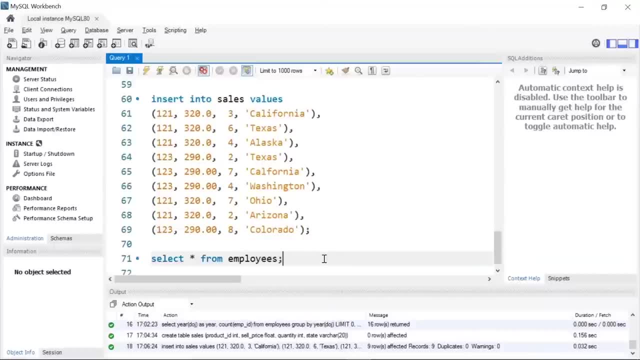 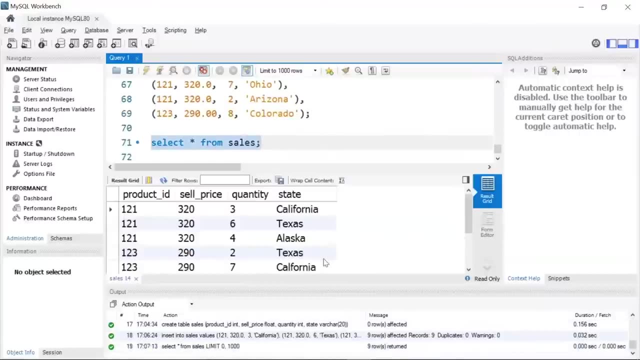 confirm with the select statement. I'll write select star from sales run this. you can see we have successfully created our table. okay, now suppose you want to find the revenue for both the product IDs one to one, and let's say one to three, since we have just two product ids here. 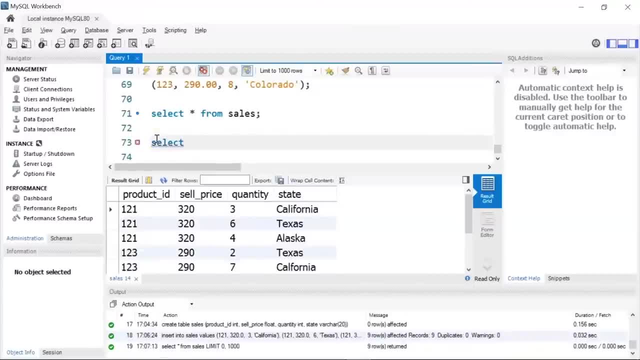 so for that you can use the select query. so i'll write select product id. next i want to calculate the revenue. so revenue is nothing but selling price multiplied by the quantity. so i'll use the sum function to find the total revenue and inside the sum function i'll use 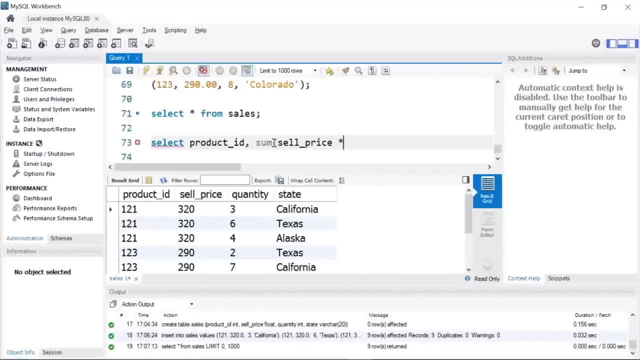 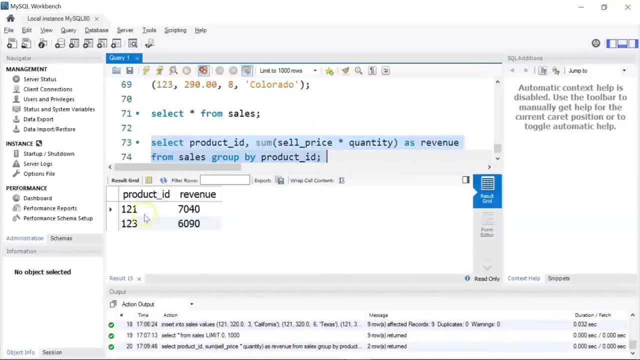 my selling price column multiplied by my quantity column. i'll give this an alias name as revenue from my table name, that is sales. finally, i'll group it by product id. let's run it there you go. so here you can see, we have the two product ids: one, two one and one two three. 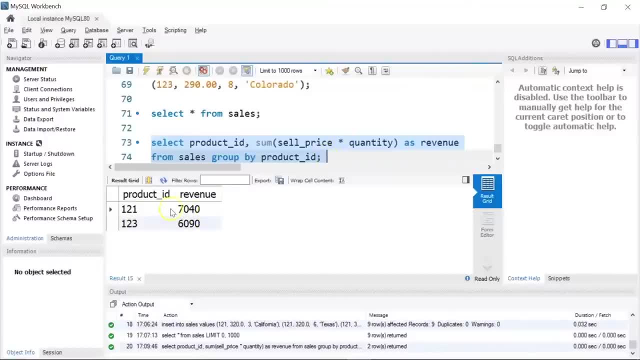 and here you can see the revenue that was generated from these two products. all right, now let's say we have to find the total profit that was made from both the products- one two one and one two three. so for that i'll create another table. now. this table will have the cost price of both the products, so let me create the. 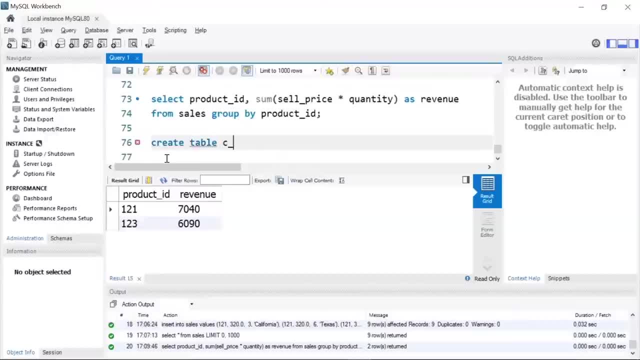 table. first i'll write create table. let's say the table name is c- product, which stands for the cost price of the products. i'll give my first column as product id- this will be an integer- and i'll have my second column as cost price. cost price will have floating type values. 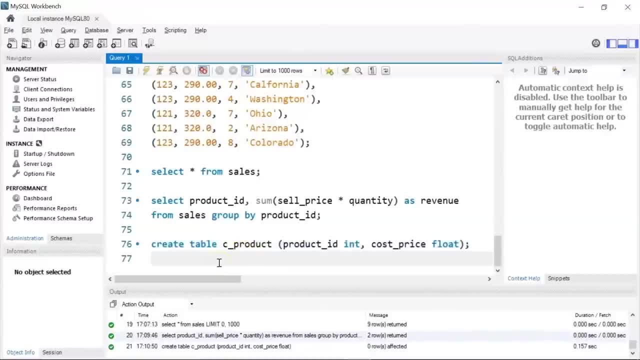 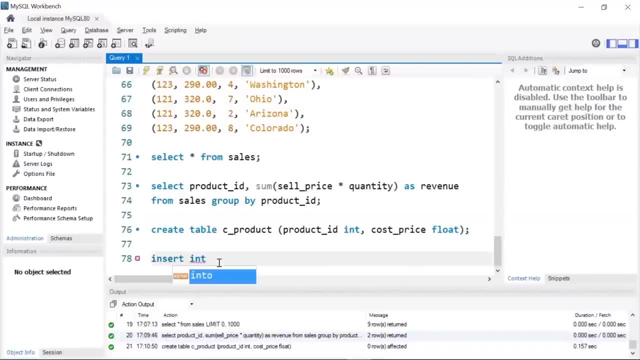 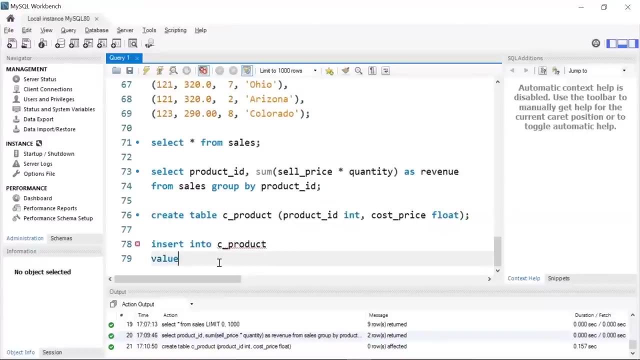 let's run this. so we have successfully created our product cost table. now let me insert a few values into the c product table. so i'll write: insert into c underscore product. i'll give my values for one to one. let's say the cost price was 270 dollars for each. 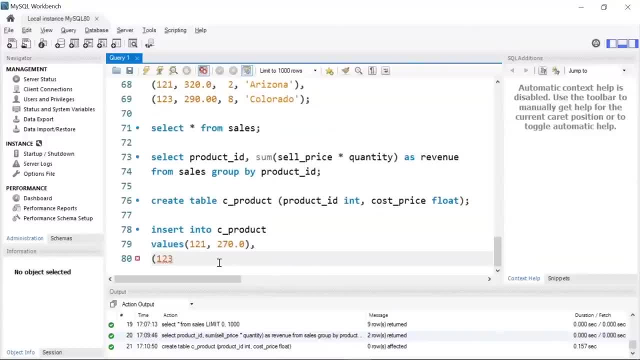 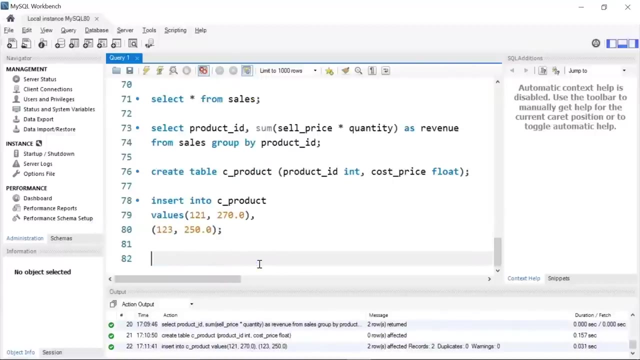 and next we have my product as one, two, three, and let's say the cost price for product one, two, three was 250 dollars. let's insert these two values, okay. next we'll join our sales table and the product cost table. so this will give us the profit that was generated for each of the products. so i'll write select. 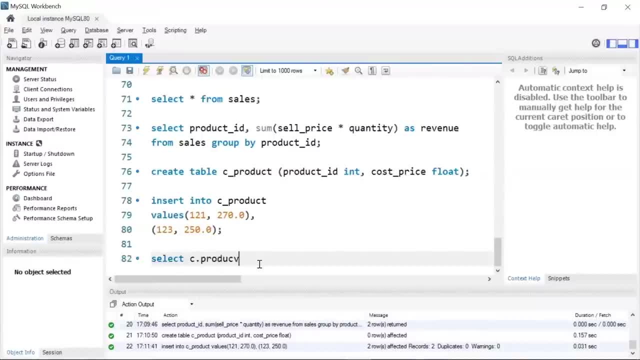 c dot product underscore id comma. i'll write sum s dot. sell underscore price. now here c and s are alias names. so if i subtract my cost price from the selling price, that will return the profit that was generated. i'll multiply this with s dot quantity. close the bracket. i'll give an alias name as profit from sales, as s. so here s stands. 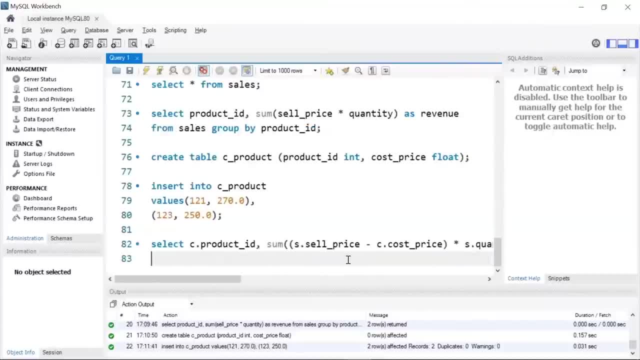 for the sales table. i'm going to use inner join c underscore price of the selling price. so i will write: enter join miti dot salary in a p88 and start the sale table. okayale, the company sale is done and the topic of today is outstanding tips and tricks. in sales tab. Serving value of sales is a very helpful piece to be men's learning technology. there are several strategies for decision making. you might be interested in sharing your tables with your friends, not just on the subject, but I think you are very interested in learningIVE knowledge. 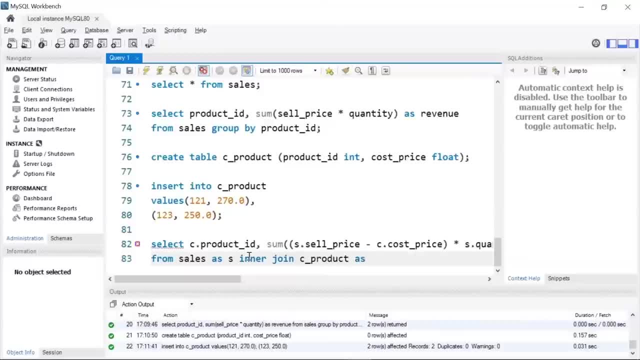 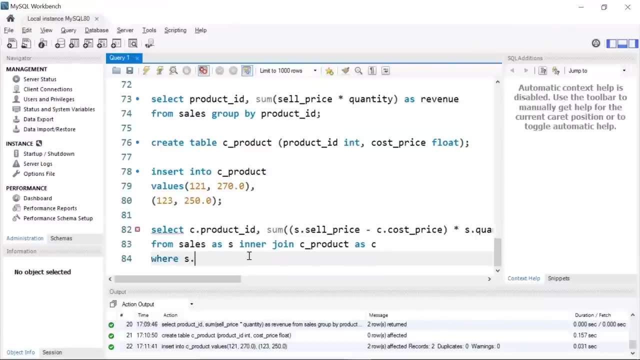 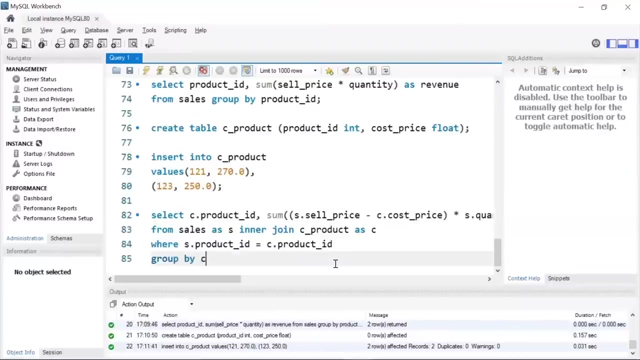 product table, as the alias name should be C, where S dot product underscore ID is equal to C dot product underscore ID. we are using product underscore ID because this column is the common column to both the tables and finally, I am going to group it by C dot product underscore ID. alright, so let me tell you. 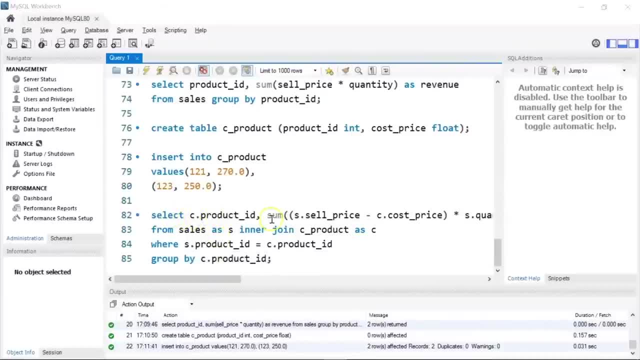 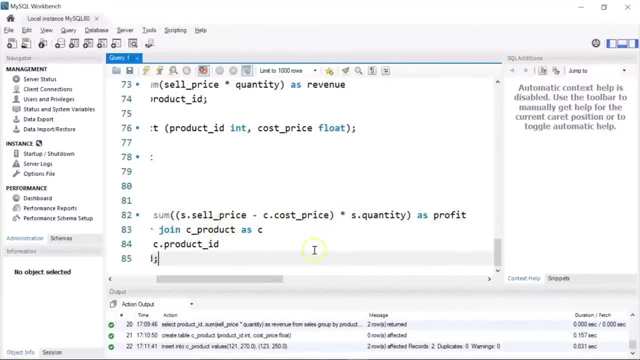 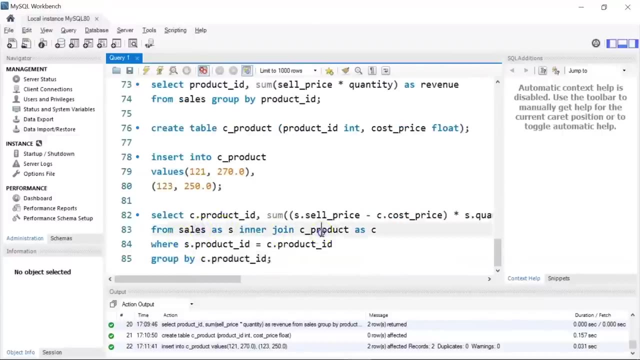 what I have done here. so I am selecting the product ID. next, I am calculating the profit by subtracting the cost price from the selling price and I have multiplied the quantity column. I am using an inner join to connect my sales and the product cost table and I am joining on the column that is product ID, and I have 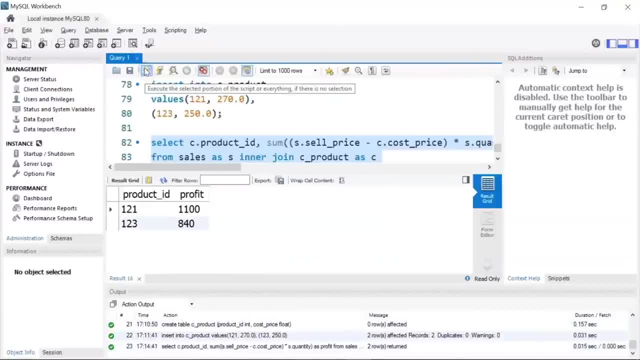 grouped it by C dot product ID. let's run this. there you go. so here you can see: for product ID one to one, we made a profit of eleven hundred dollars, and for product ID one to three, we made a profit of eight hundred and forty dollars. so 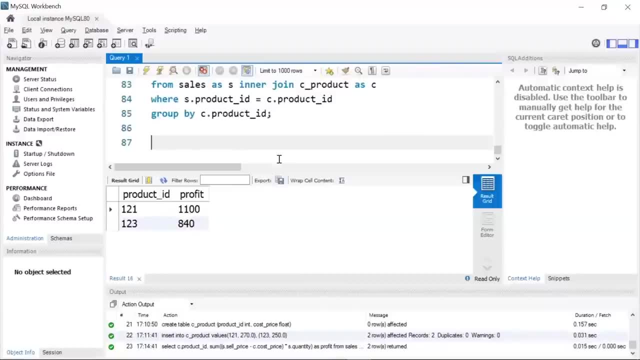 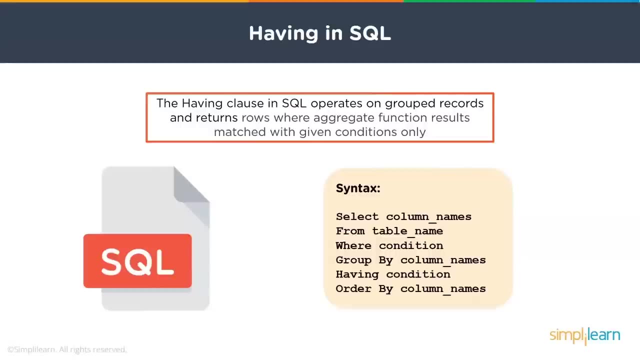 now that we have learnt group by in detail, let's learn about the having clause in SQL. the having clause in SQL operates on grouped records and returns. rows were aggregate function results matched with given conditions only. so now having and wear clause are kind of similar, but wear clause can't be used. 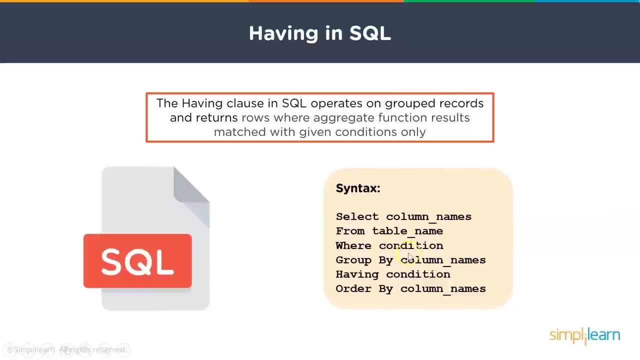 with an aggregate function. so here you can see the syntax of having clause. you have the select statement followed by the column names from the table name, then we have the wear conditions, next we have the group by. finally we have having and at last we have order by column names. so you can see, here we have a question at hand. 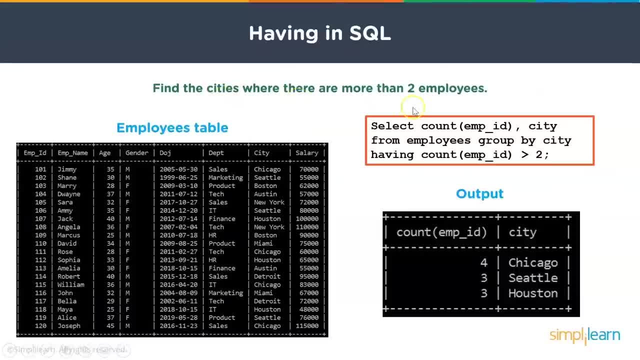 we want to find the cities where there are more than two employees. so you can see the employee table that we had used in our group by clause as well. so if you were to find the cities where there are more than two employees, so this is how your sql query should look like. so we have 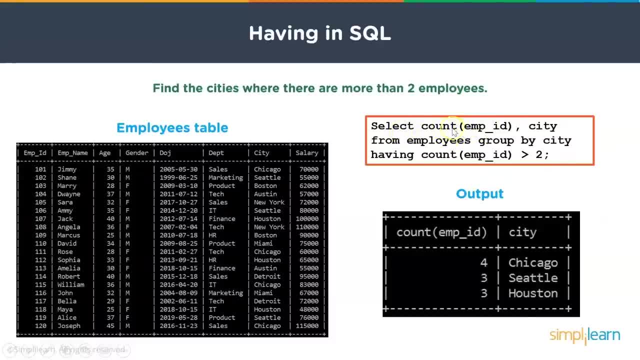 selected the employee id and we are finding out the count using the count function. next, we have selected the city column from employees, we have grouped it by city and then we have used our having clause. so we have given our condition: having count of employee id should be greater than two. so if you see the output, we have the different city names and these were the. 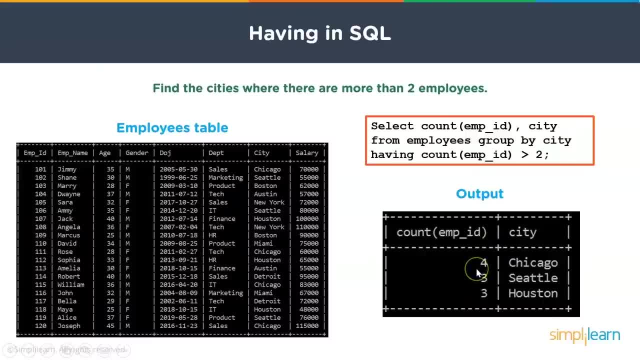 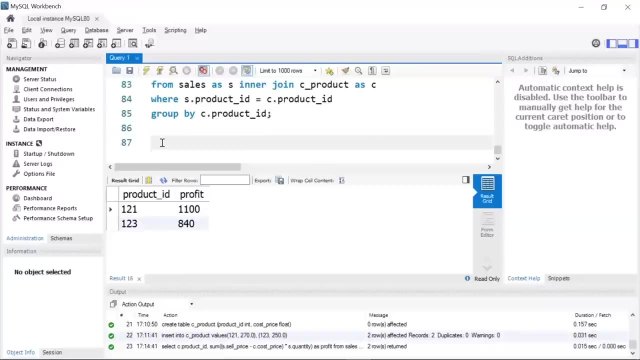 cities where the count of employees was greater than two. all right, so let's go to our mysql workbench and implement how having works. so suppose you want to find those departments where the average salary is greater than seventy five thousand dollars? you can use the having clause for this. so let me first run my 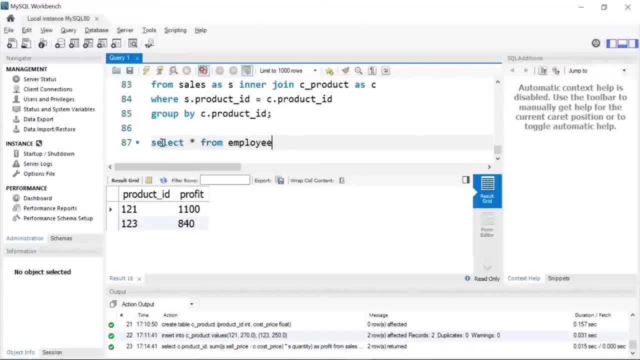 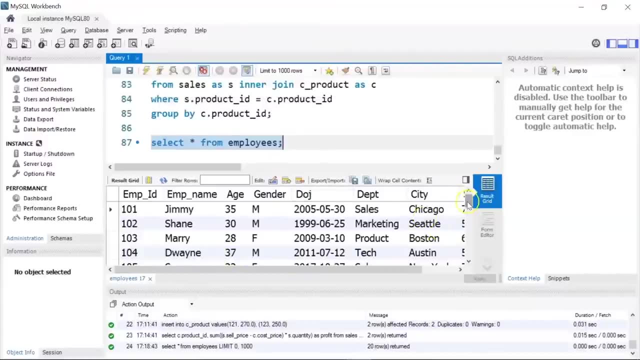 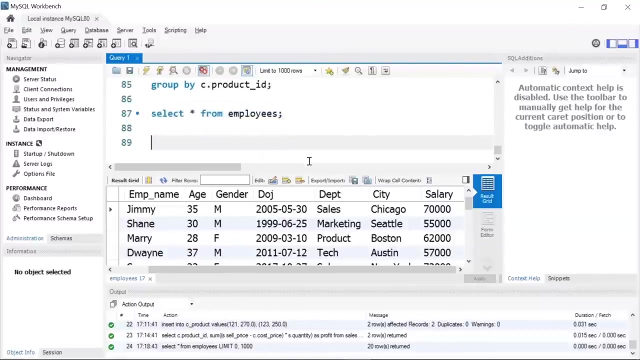 table, which is employees. if i run this, you can see we had inserted 20 rows of information and the last column we had was salary. so the question we have is: we want to find those departments where the average salary is greater than seventy five thousand dollars. so let me show you how to do it, so I'll write: select department. 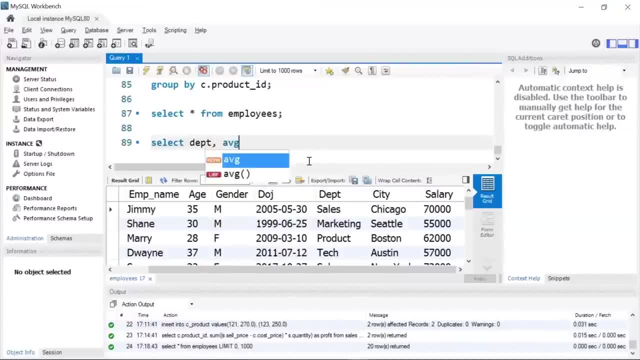 comma. I'll use the aggregate function, that is, average salary. I'll give an alias name as AVG underscore salary from employees. next, we'll use the group by clause and I want to group it by each department and then I'm going to write my having clause. so in having clause I'll use my condition, that is, having average of salary. 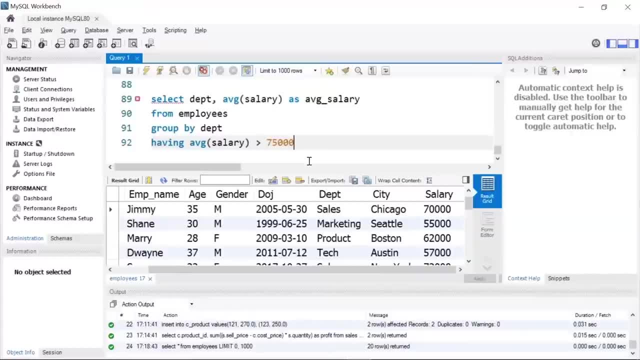 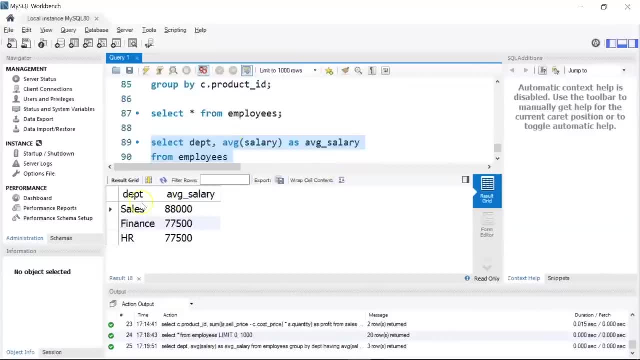 greater than seventy five thousand dollars. let's run it and see the output. so let's run it and see the output. there you go. so here you can see. there were total three departments in the company, that is, sales, finance and HR, where the average salary is greater than seventy five thousand dollars. okay, next let's see. you want. 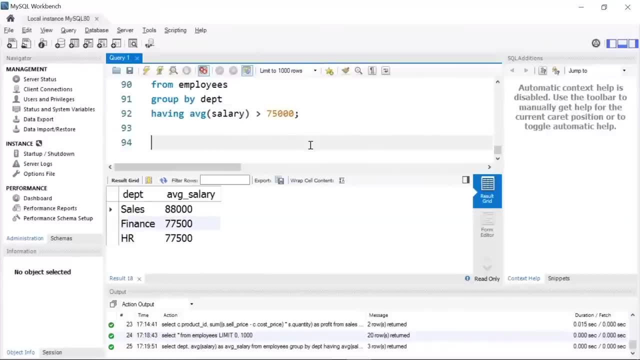 to find the cities where the total salary is greater than two hundred thousand dollars. so this will again be a simple SQL query. so I'll write select city comma and I'll I want to find the total salary, so I will use the sum function and I will pass my column as salary, as I will give a alias name as total from employees group by city, and then I am going to use my having clause. 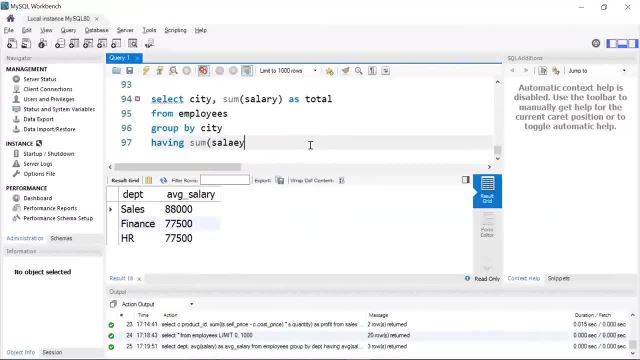 I will pass in my condition as having sum of salary greater than $200,000.. All right, So let's run this query. There you go. So the different cities are Chicago, Seattle and Houston, where the total salary was greater than $200,000. 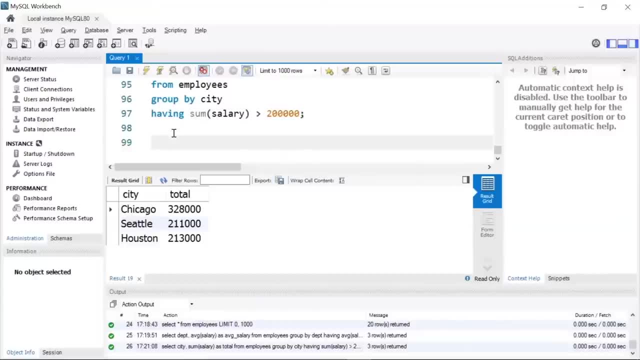 Now suppose you want to find the departments that have more than two employees. So let's see how to do it. I will write select department comma. This time, since I want to find the number of employees, I am going to use the count function. I will write count star as employee underscore count or EMP underscore count, which is my alias name from employees. 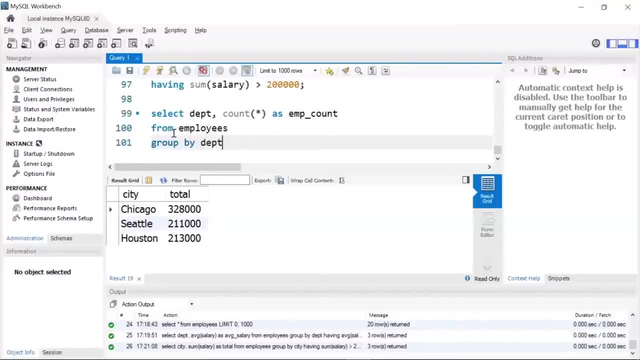 Next I will group it by department: Having- I will give my condition count star- greater than two. Let's run this Okay. So you have departments such as sales, product tech and IT where there are more than two employees. Okay, Now you can also use a where clause along with the having clause in an SQL statement. 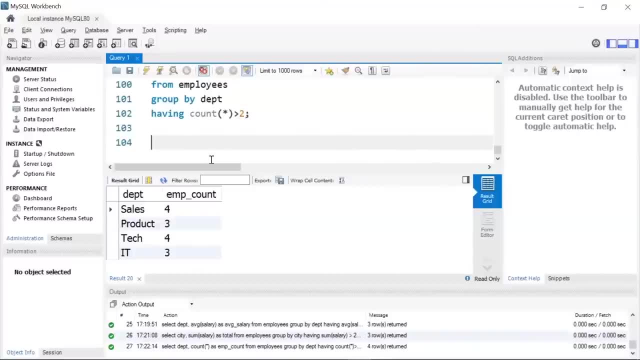 So let's see how to do it. So suppose I want to find the cities that have more than two employees, than two employees, apart from Houston, so I can write my query as select city comma count star as EMP count from employees where I'll give my condition: city not equal to. 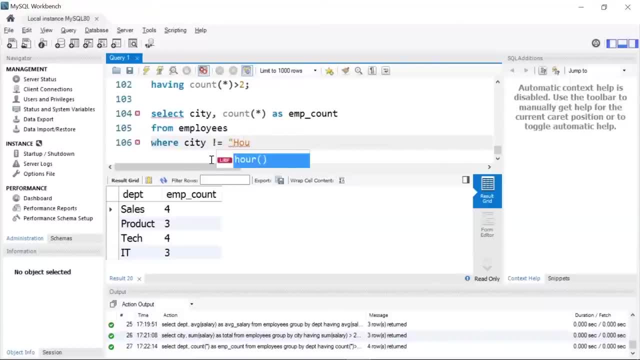 Houston. I will put it in double quotes, since I don't want to see the information regarding Houston. you I'll group it by city having count of employees greater than two. if I run this query, you see we have information for Chicago and Seattle only and we have 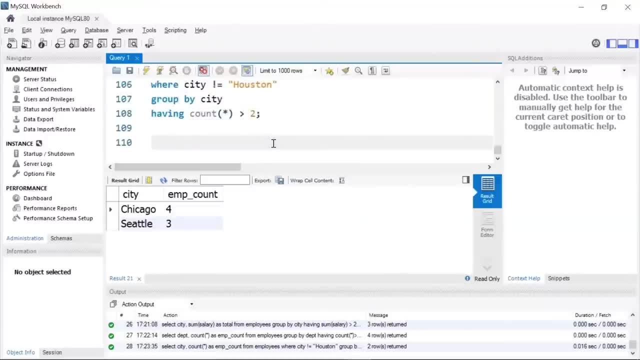 excluded the information for Houston. now you may also use aggregate functions in the having clause. that does not appear in the select clause. so if I want to find the total number of employees for each department that have an average salary greater than $75,000, I can write it. 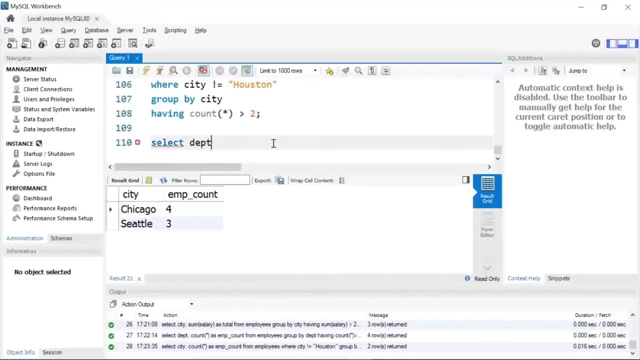 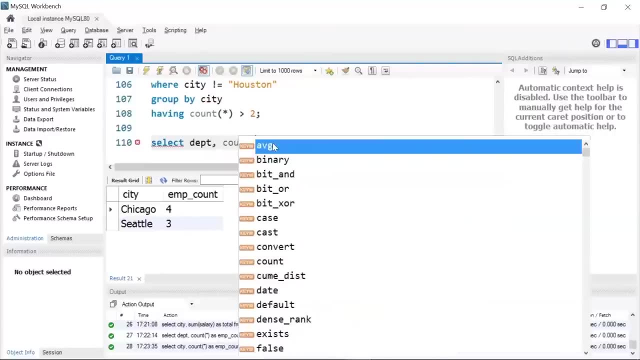 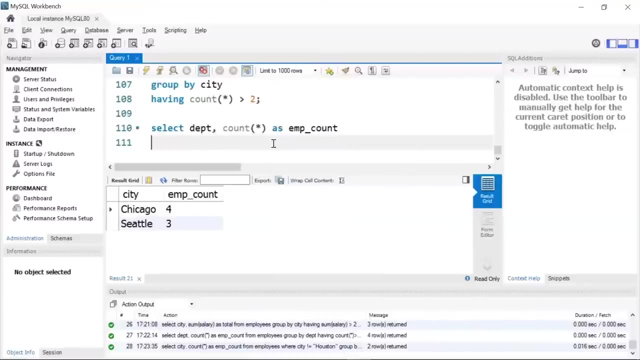 something like this: to select department comma count star as EMP count from employees, employees group by department, and in the having clause I am going to provide the column name. that is not present in the select expression, so I'll write: having average salary greater than 75,000. this is another way to use the having clause. 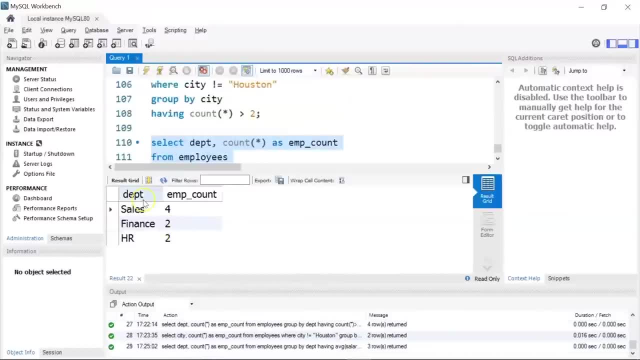 let's run this all right. you can see we have department sales, finance and HR, and you can see the employee count where the average salary was greater than 75,000. okay, so let me run you from the beginning what we did in our demo. so first we created a table called employee, then we inserted 20 records to this. 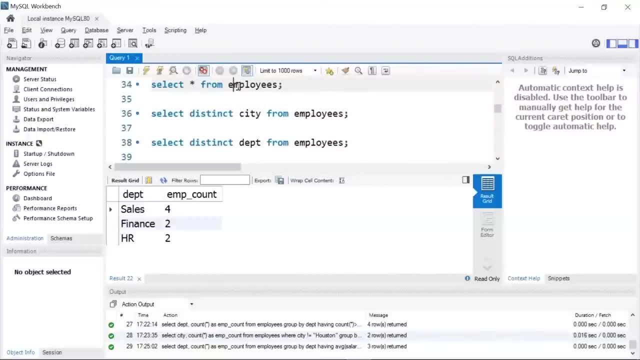 table. next we explode a few SQL commands like distinct, then we used average and finally we started with our group by clause, followed by looking at how group by can be used along with another table and we joined two tables, that was sales and product cost table, to find the average salary greater than 75,000 and 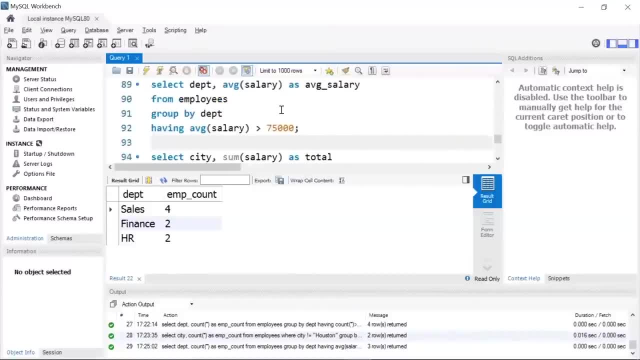 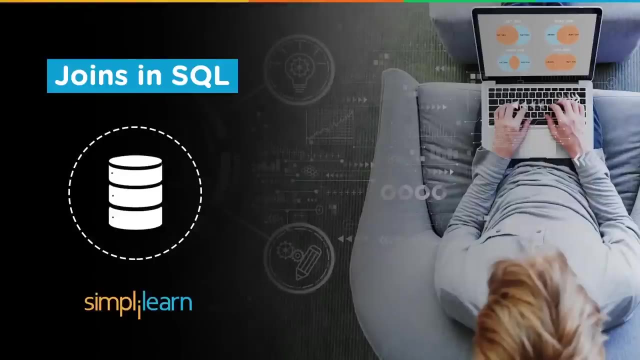 find out the profit. then you learned how to use the having clause. so we explored several different questions and learned how to use having an SQL. in this session, we will learn about joints in SQL. joints are really important when you have to deal with data that is present on multiple tables. I'll help you. 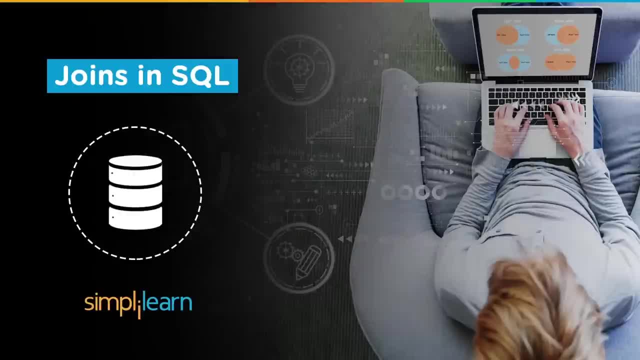 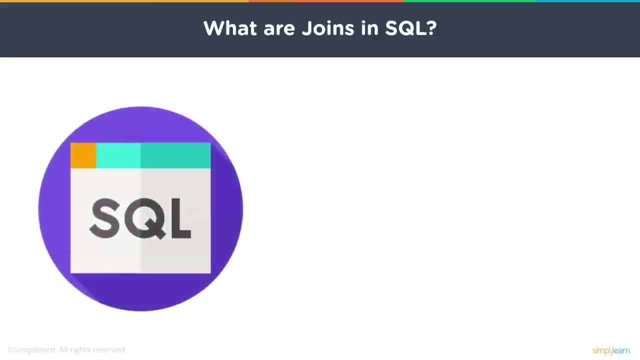 understand the basics of joints and make you learn the different types of joints with hands-on demonstrations on my SQL workbench. so let's get started with what are joints in SQL? SQL joint statement or command is often used to fetch data present in multiple tables. SQL joints are used to combine rows of. 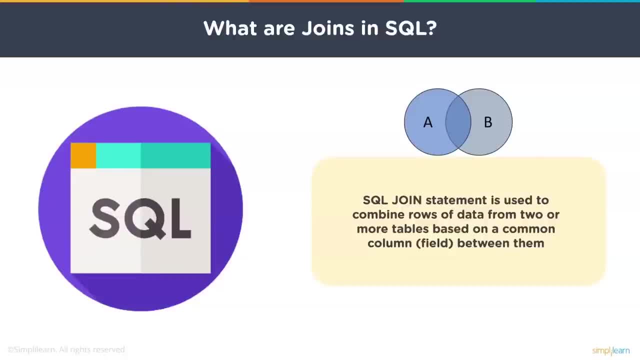 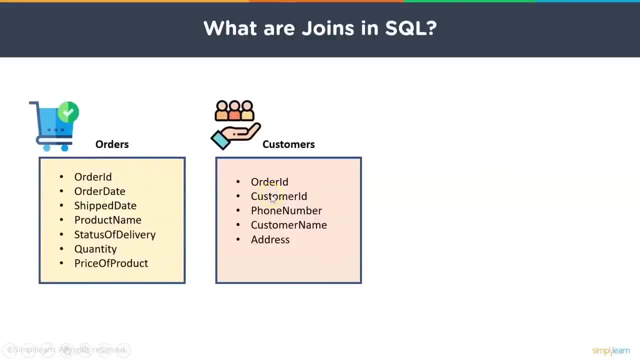 data from two or more tables based on a common field or column between them. now consider this example where we have two tables, an orders table and a customers table. now the order table has information about the order ID, which is unique. here we have the order date, that is with. 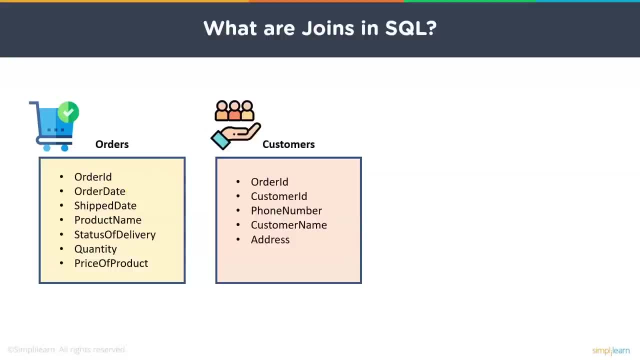 the order and the shift Automatic, that is, with yet another table over the Stelle in this table when the order was placed. then we have the shift date. this has information about the date on which the order was shipped. then we have the product name, which basically is the names of different products. we have the 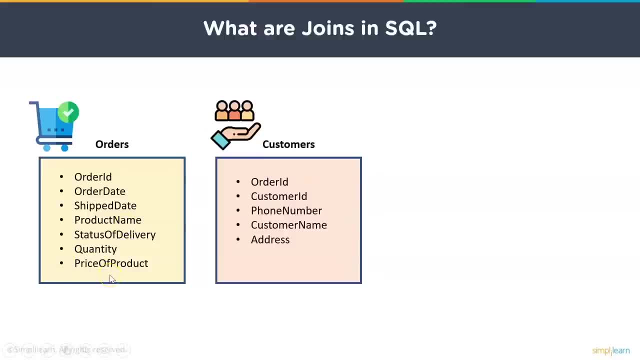 status of delivery, whether the product was delivered or not, or whether it was cancelled. then we have the quantity, which means the number of products that were ordered, and finally, we have the price of each product. similarly, we have has information about the order id, which is the foreign key here. then we have the customer id. 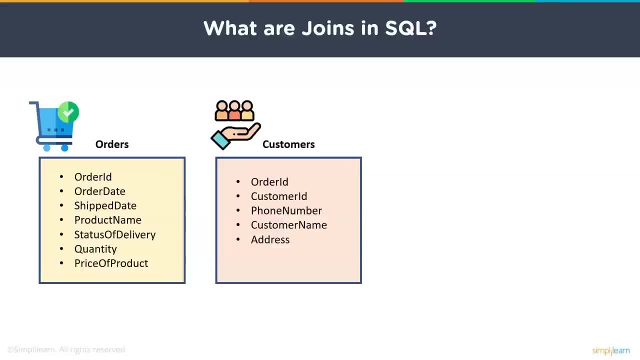 which is the primary key for this table. we also have the phone number, customer name and address of the customers. now suppose you want to find the phone numbers of customers who have ordered a laptop now to solve this problem, we need to join both the tables, the reason being the phone numbers. 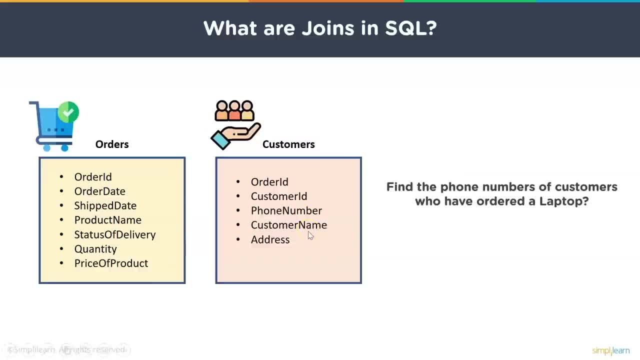 are present in the customers table, as you can see here, and laptop, which is the product name, is present in the orders table, which you can see it here. so, using a joint statement, you can find the phone numbers of customers who have ordered a laptop. now let's see another problem where you need to find the customer names who have ordered. 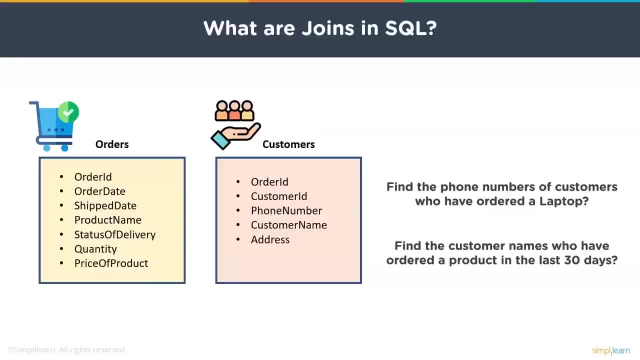 a product in the last 30 days. in this case, we want the customer name present in the customers table and the last 30 days order information, which you can get from the order date column that is present in the orders table. okay, now let's discuss the different. 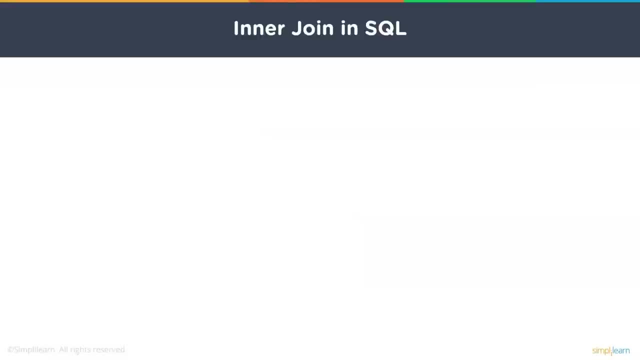 types of joins, one by one. so first we have an inner join, so the sql inner join statement returns all the rows from multiple tables, as long as the conditions are met. from the diagram above you can see that there are two tables: a and b. a is the left table and b is the right table, the orange. 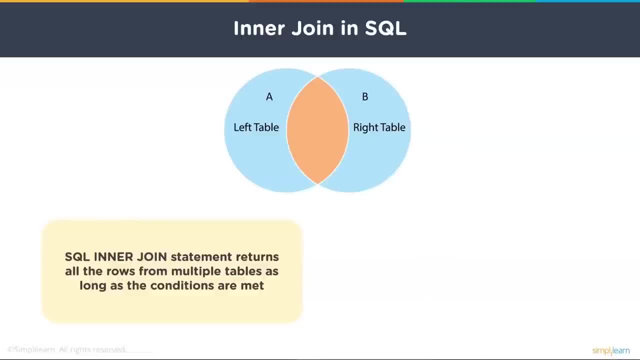 portion represents the output of an inner join, which means an inner join returns the common records from both the tables. now you can see the syntax here. so we have the select command and then we give the list of columns from table a, which you can see. here is the left table. 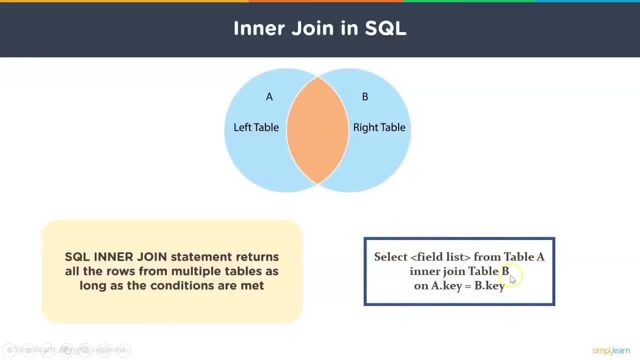 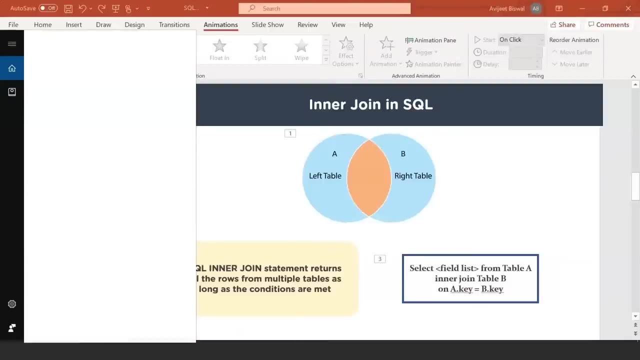 followed by the inner join keyword and then the name of the table, that is b, on a common key column from both the tables a and b. now let me take you to the mysql workbench and show you how inner join works in reality. so here i'll type mysql: 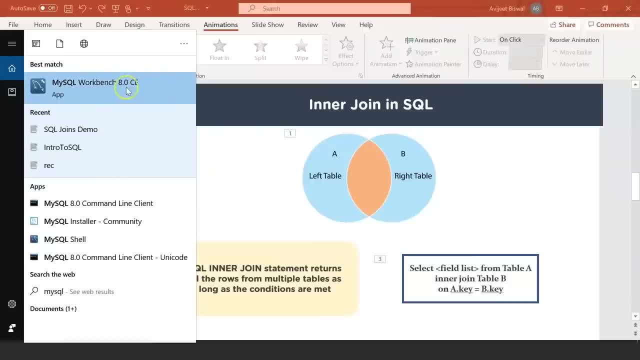 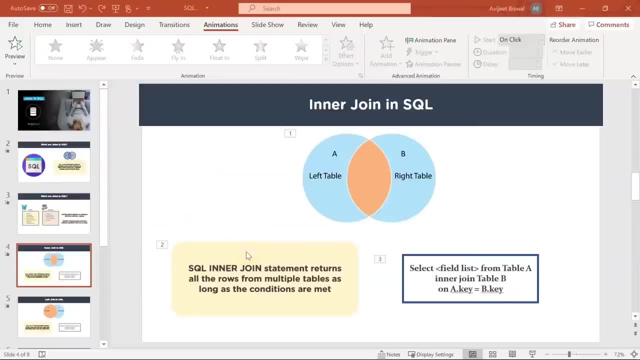 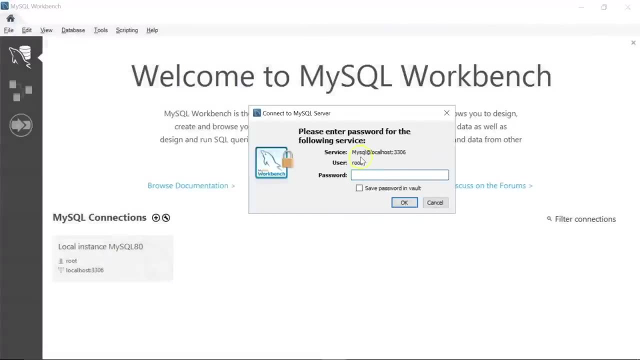 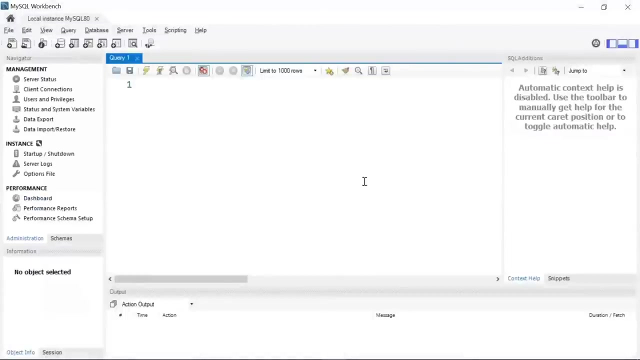 you can see, i have got mysql workbench 8.0 version installed. i'll click on it. it will take some time to open. okay, i'll click on this local instance and here i'll give my password. okay, so this is how an sql editor on mysql workbench looks like. 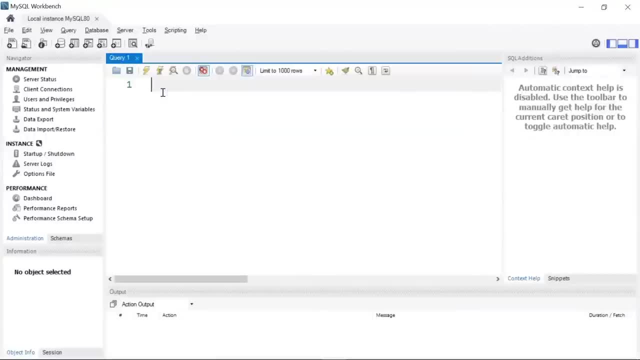 so first of all, let me go ahead and create a new database. so i'll write: create database. this is going to be my command, followed by the name of the database that is going to be sql underscore joins. if i give a semicolon and hit control, enter, this will create a new database. you. 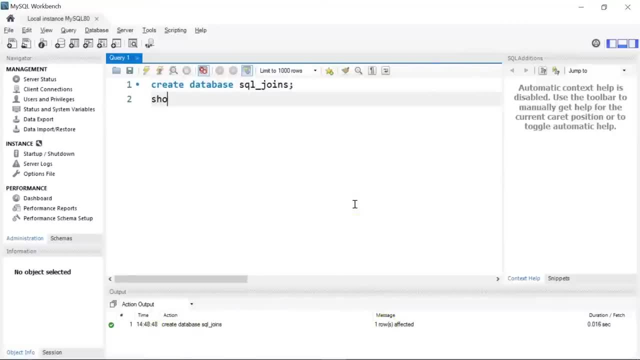 can see here one row affected. now you can check whether the database was created or not using show databases command. if i run it here, you can see i have sql joins database created. now i'll use this database, so i'll write: use sql underscore joins. okay, now to understand inner join. consider that: 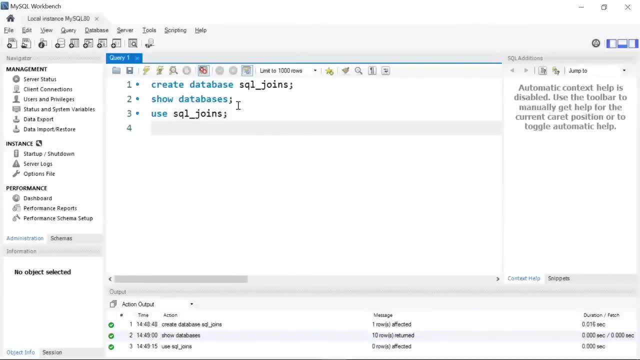 there is a college and in every college you have different teams for different sports, such as cricket, football, basketball and others. so let's create two tables: cricket and football. so i'll write create table and my table name is going to be cricket. next i'm going to create two columns. 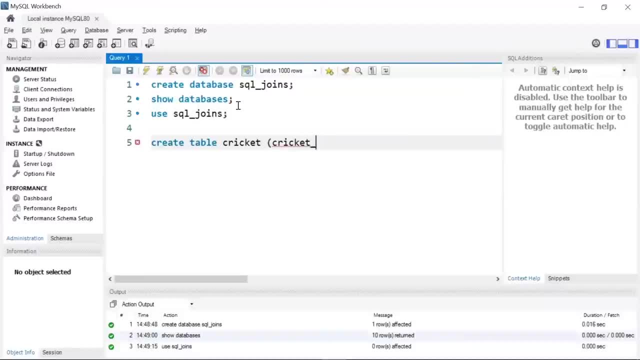 in this table the first column is going to be cricket id. then i am going to give the data type as int and use the auto increment operator. i'm using auto increment because my cricket id is going to be my primary key. then i am going to give: 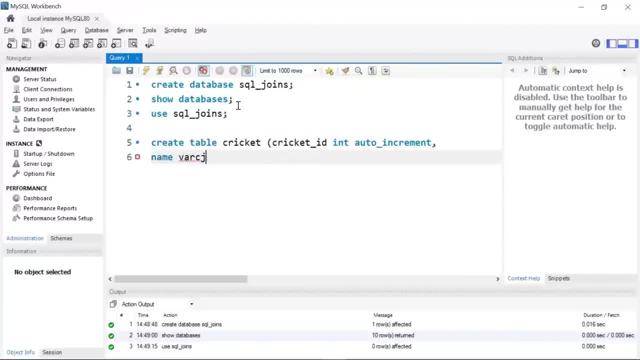 the name of the students who are part of the cricket team and for this i will use varchar data type and give the length as 30.. i'll give another comma and i will. i'll assign my cricket id as primary key. within brackets i'll give cricket. 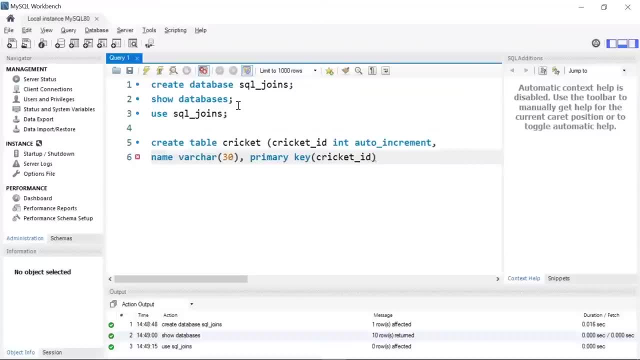 underscore: id. cricket id is nothing but a unique identifier for each of the players. like you have roll numbers in college, okay, let me just run it all right. so we have successfully created our cricket table. similarly, let me just copy this and i'll paste it here. i'll create another table called 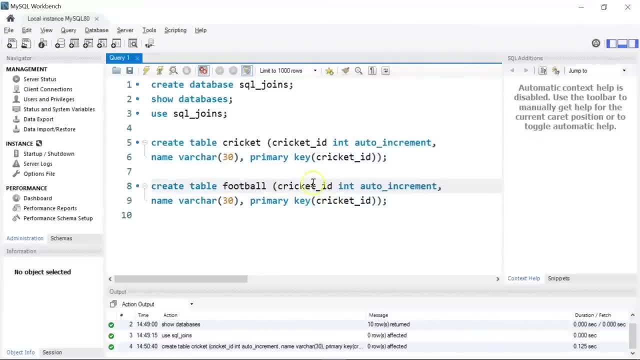 football. this will have the information of all the students who are part of the football team and instead of cricket, i am going to give this as football id, all right, and the name column will have the names of the students. i'll change my primary key to football. 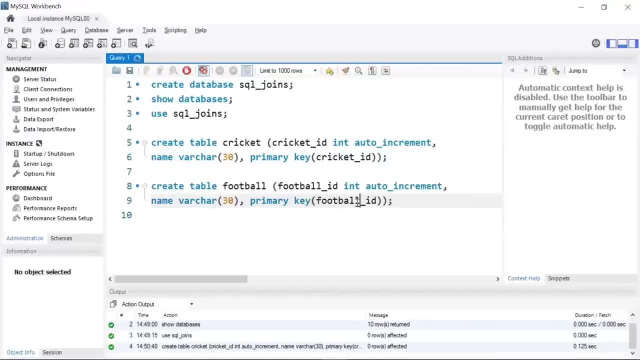 id. all right, let me run this okay. so now we have also created our football table. the next step is to insert a few player names into both the tables, so i'll write my insert into command. first, let's load some data to our cricket table. so i'll write cricket and i'll give my name column. 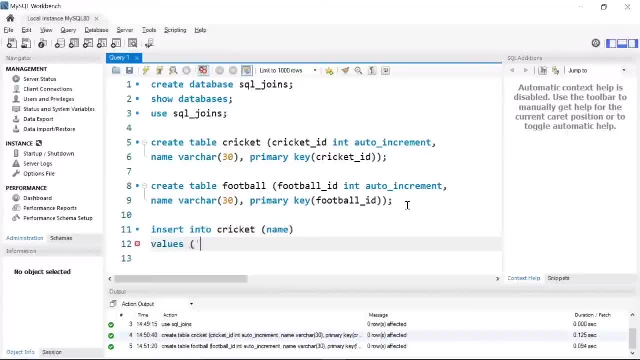 followed by values, and here i'll give some names, such as, let's say, stuart. you give another comma. the next player i'll choose is, let's say, michael. similarly, i'll add a few more. let's say, we have johnson. the fourth player i'll take is, let's say, hayden. 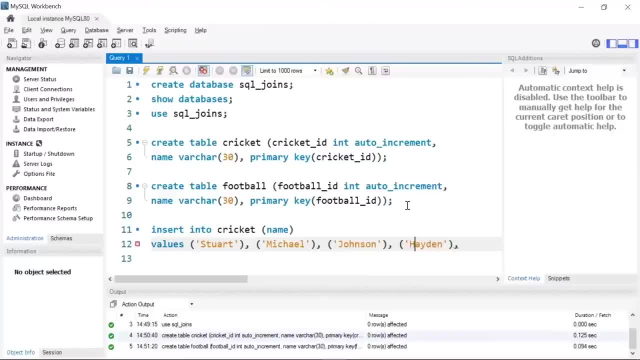 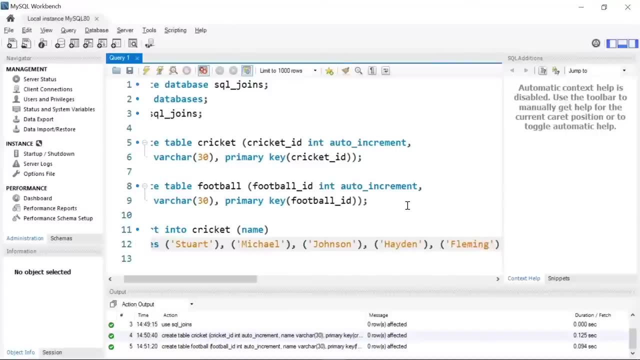 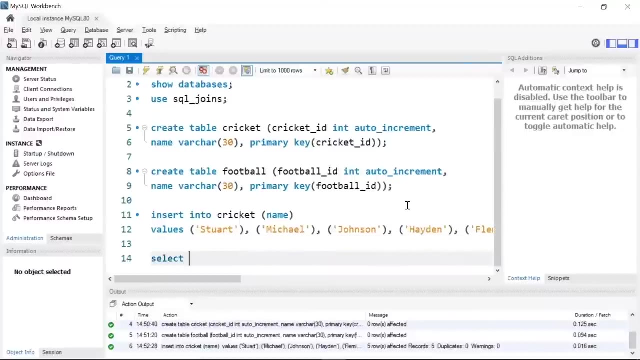 and finally we have, let's say, fleming arnold. ok, now i'll give a semicolon and run this. okay, so let me just check if all the values were inserted properly. for this, i'll use select star from table. that is cricket. if i run it, you can. 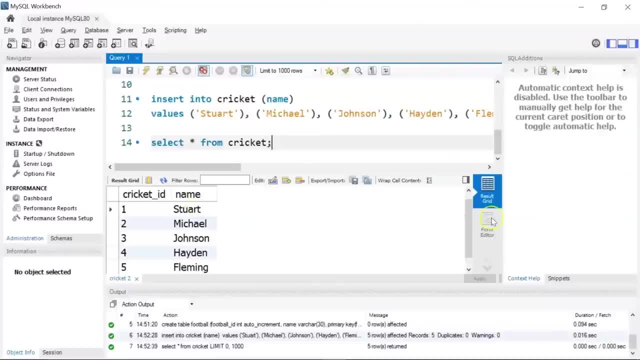 see, i have created a table and have successfully inserted five rows of information. now, similarly, insert a few student names for our football table. so I'll change this to football and obviously there would be students will be part of both cricket and football team. so I'll keep a few repeated names, let's say Stuart Johnson. 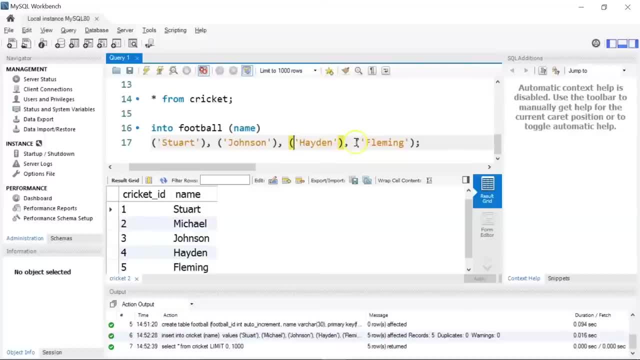 and let's say Hayden, are part of both cricket and football team, then we have, let's say, Langer, and let's say we have another player in the football team, that is Aston. I'll just run it okay. you can see. there are no errors. so we have successfully. 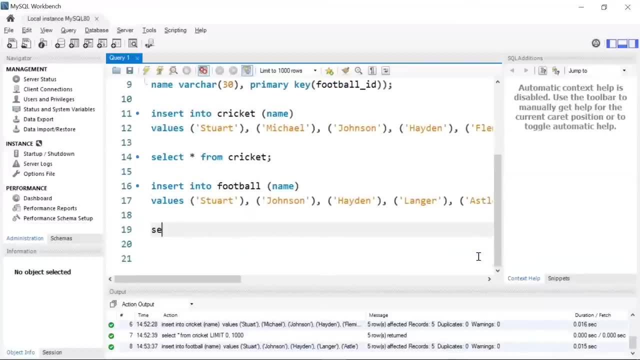 inserted values to our football team as well. let me just recheck it. I'll like to say that we have successfully inserted values to our football team as well. let me just recheck it. I'll write: select star from football. all right, so we have five players in the. 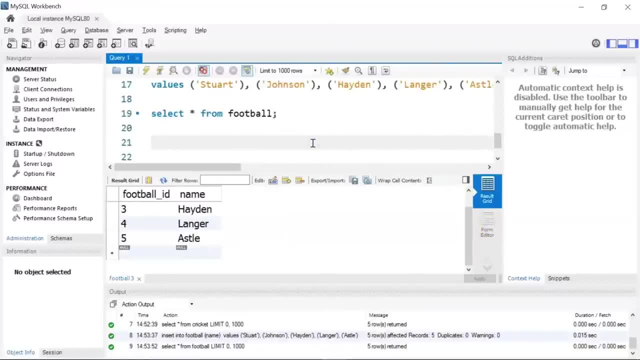 football team as well. okay, now the question is: suppose you want to find the students that are part of both the cricket and football team. in this case, you can use an inner join, so let me show you how to do it. so I'll write: select star from cricket. as I am using an 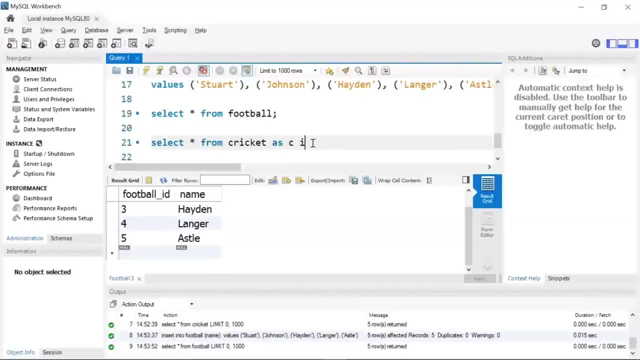 alias name as C, which stands for cricket. then I am going to write inner join. my next table is going to be football as F, which is an alias name for the football table. then I am going to use the on command or operator and then I'll give. 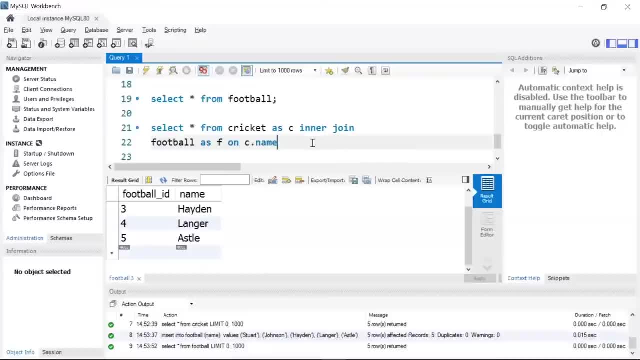 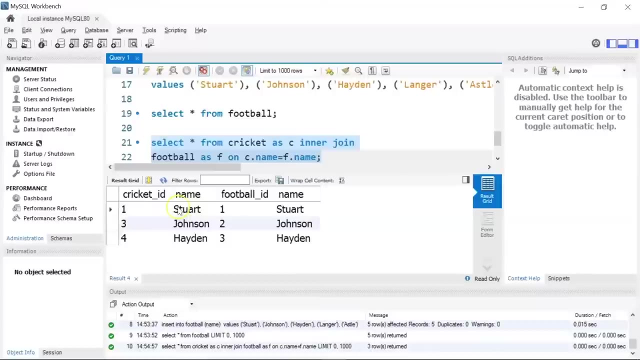 the common key that is name here. so C dot name is equal to F dot name and so, based on this name column from both the table, my inner join operation will be performed. so let's just run it. there you go. so Stuart Johnson and Hayden are the. 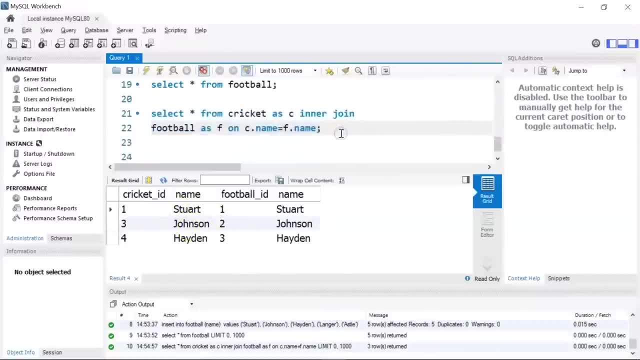 only three students who are part of both the teams. all right, now you can also individually select each of the columns from both the tables. so let's say I write: select C- dot- cricket- underscore ID comma C- dot name. comma F- dot- football underscore ID comma F- dot name from. I'll write. 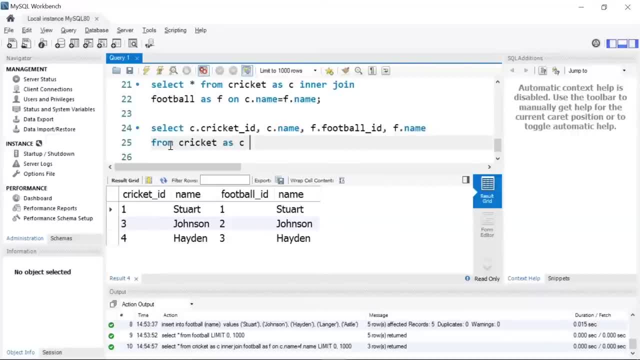 cricket as C inner join, football as F on C dot name is equal to F dot name. now if I run this, you see we get the same output here as well. all right, now let's explore another example to learn more about inner joins. so we have a database. 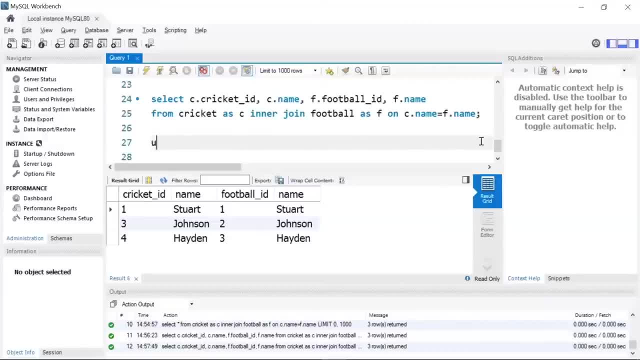 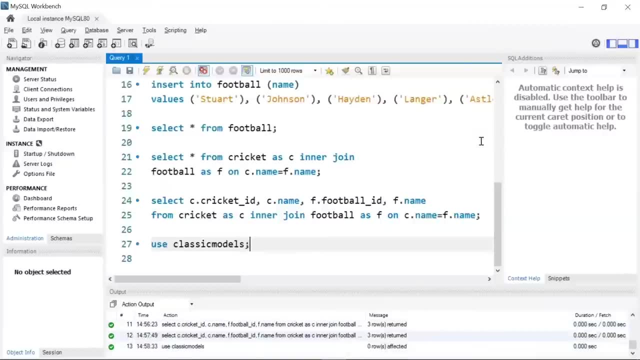 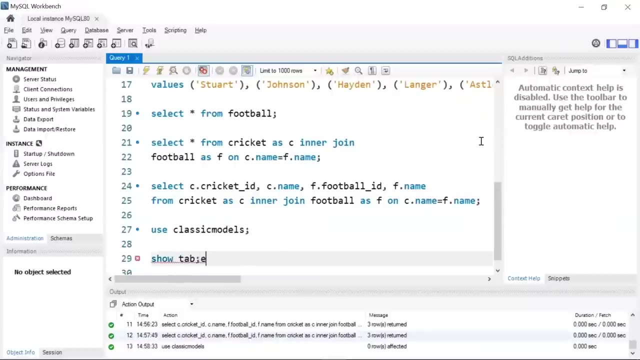 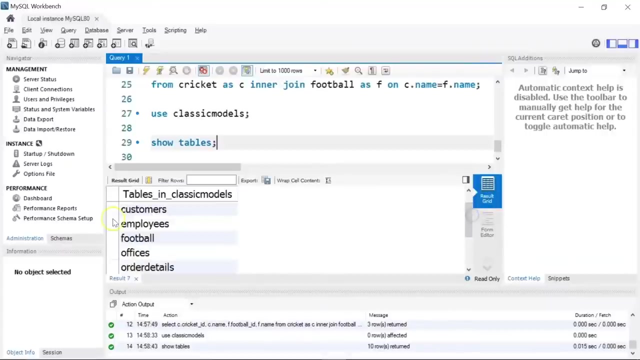 called classic models. let me first use classic models. I'll run this. okay. now let me just show the different tables that are part of classic tables. all right, so here you can see. there are tables like customers, there's employees office, there's office details, orders, payments, products and product. 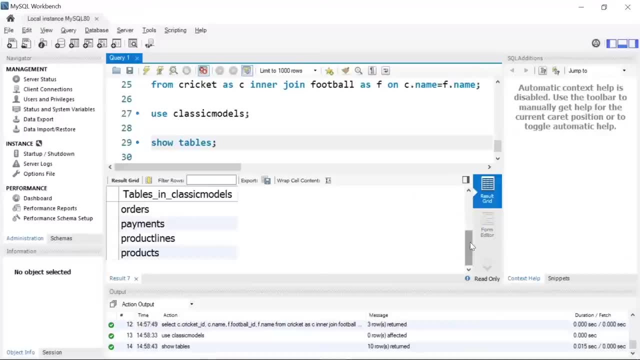 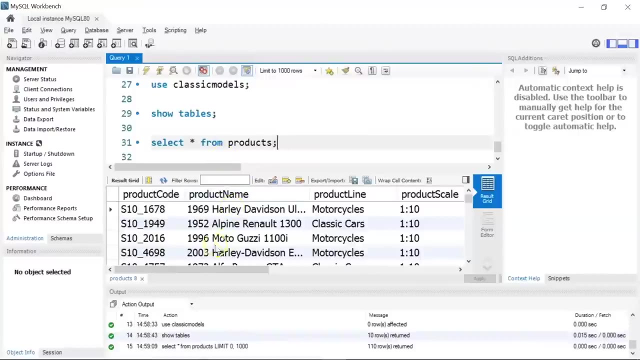 lines as well. all right, so let me use my select statement to show what are the columns present in the products table. okay, so this product table has information about different product names. you have the product code now. this product code is unique. here. we also have the product. 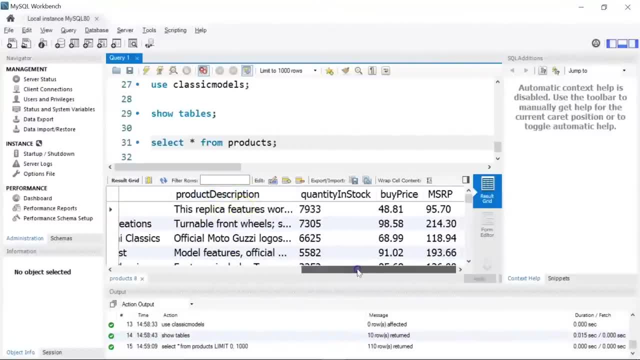 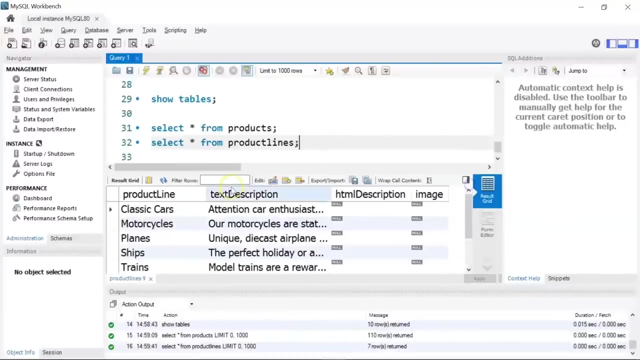 vendor, a little description about the product. then we have the quantity in stock, buying price and MSRP. let's see what we have in product lines now. if i run it, you see here we have the product line, which is the primary key for this table. then we have the textual description for each of the products. 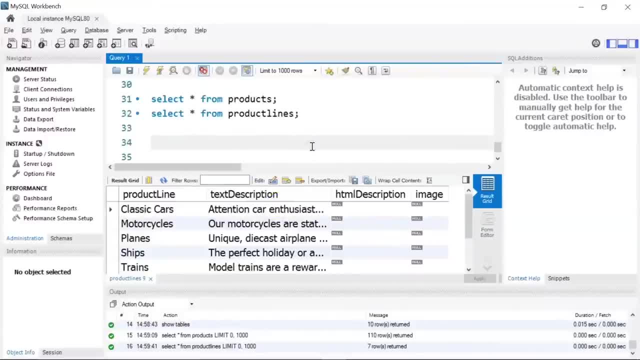 this is basically some sort of an advertisement. all right, now suppose you want to find the product code, the product name and the text description for each of the products. you can join the products and product lines table. so let me show you how to do it. i'll write my情況. 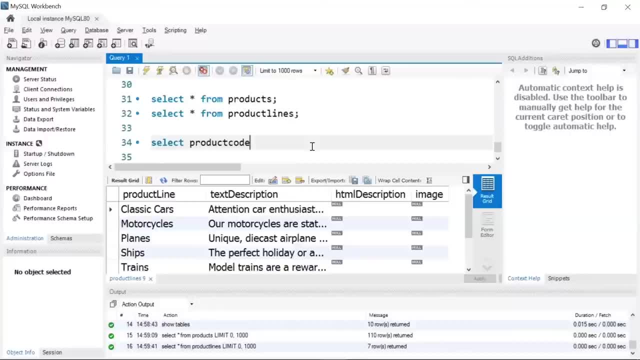 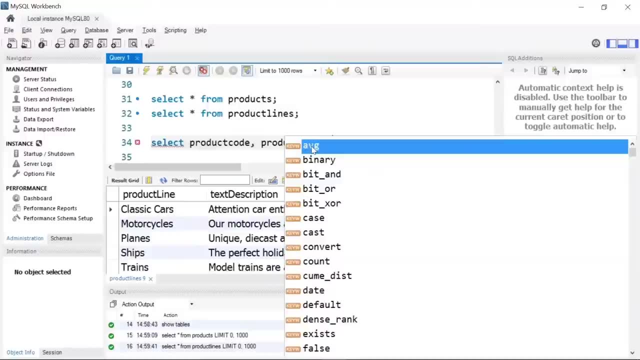 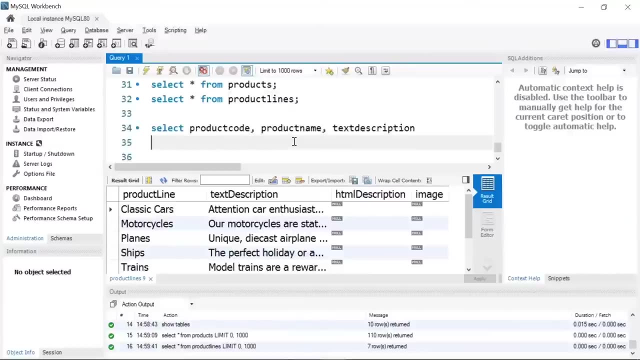 select statement and choose my columns as product code. then we have product name and let's say I want the text description so I'll write this column name. okay, then I'll use from my first table that is products inner join product lines I can use using the common key column, that is product line close. 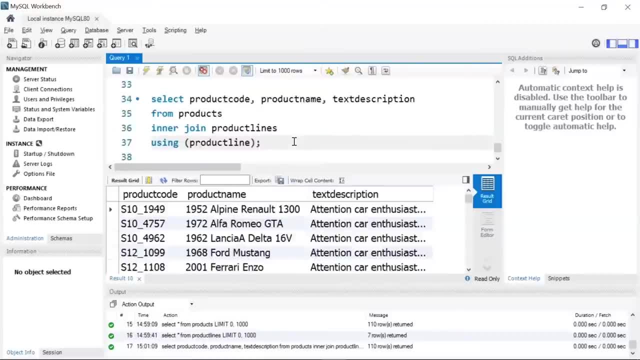 the bracket. I'll give a semicolon and if I run it, there you go so you can see the different product codes. then we have the different product names. you can see the different product codes, then we have the different product names and the textual description for each of the products. so this we did by joining. 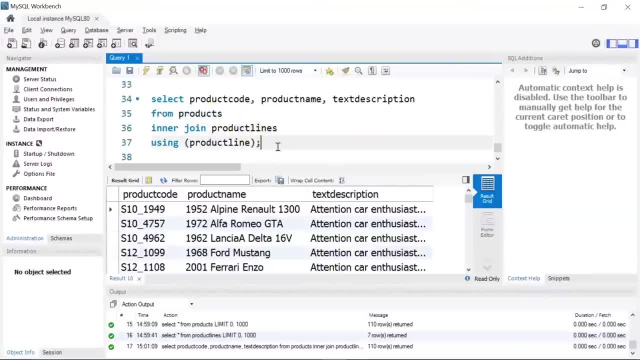 the products table and the product lines table. alright, now suppose you want to find the revenue generated from each product order and the status of the product. to do this task we need to join three tables, that is, orders, order details and products. so first let me show you what are the 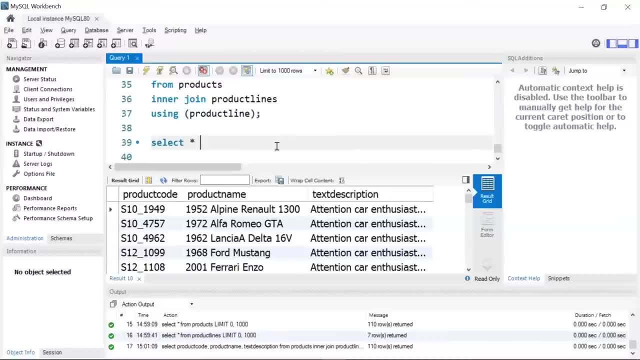 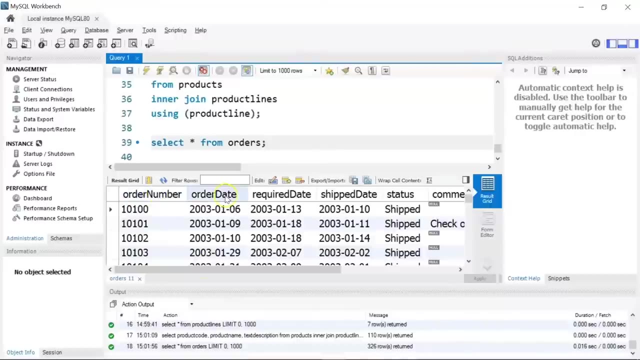 columns we have in these three tables. have obviously seen for the products table. now let me show you for orders and order details table. so i'll write select star from orders, fire on it you can see it has information about the order number, the date on which the order was placed. we also have the shipment date. we 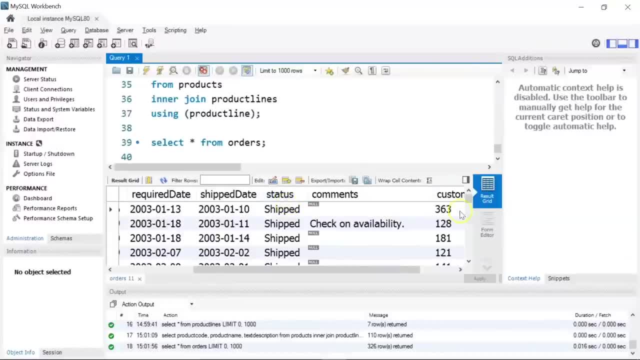 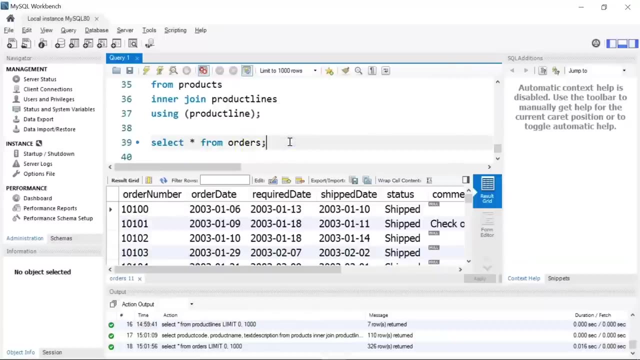 also have the status column, which has information regarding whether the order was shipped or cancelled. then we have some comments column. we also have the customer number who ordered this particular product. similarly, let's check what we have under order details. so i'll write select star from order details. if i run it, you can see it has the order number, the. 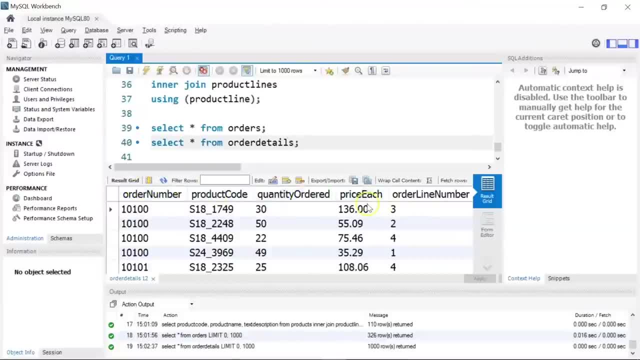 product code, quantity of each product. we have the price of each product, then we have the order line number. okay, so using the product orders and order details, let's perform an inner join. so i'll write: select o dot order number comma o dot status comma. i need the. 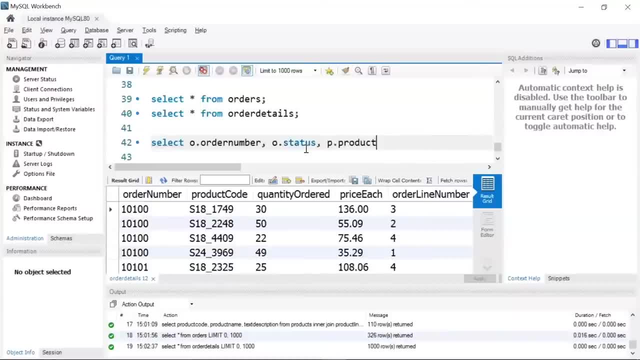 product name which i'll take from the products table. so i'll write p dot product name. now here o p are all alias name for the tables, orders products, and i'll use od for order details comma. since we want to find the revenue, we actually need to find the product of quantity. 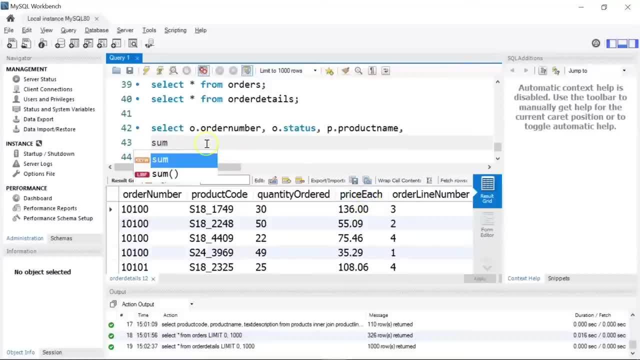 ordered into price of each product. so i'll use a sum function and inside the sum function i'll give quantity ordered multiplied by the price of each item. i'll use an alias as revenue, then i'll use my from clause from orders as o inner join order details, as i'll use an alias name as od on. 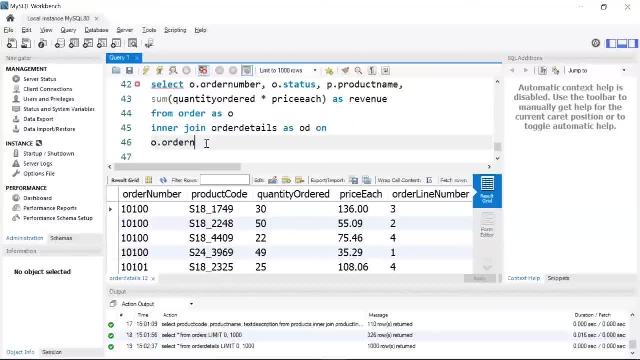 i'll write o dot order number is equal to od dot order number. i'll use another inner join and this time we'll join the products table. so i'll write inner join products as p on p dot product code is equal to od dot product code. and finally, i'll use the group by clause and group it by order number. 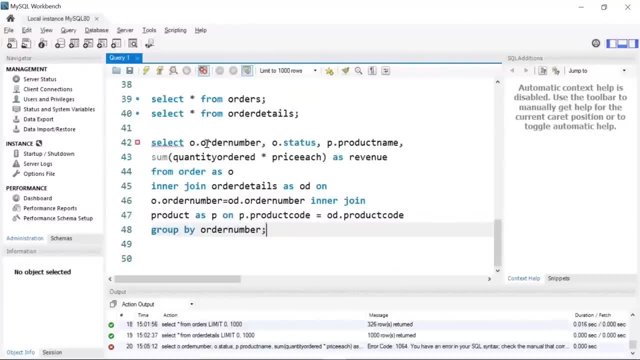 all right, let me run this. okay, there's some mistake here. we need to debug this. it says you have an error in your sql syntax. check the manual, all right. okay, i think the name of the tables is actually orders and not order. all right, now let's run it. 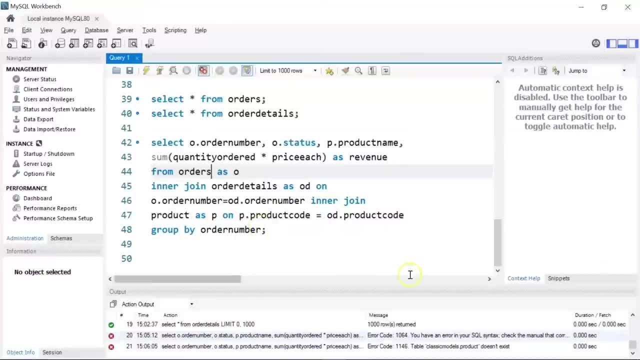 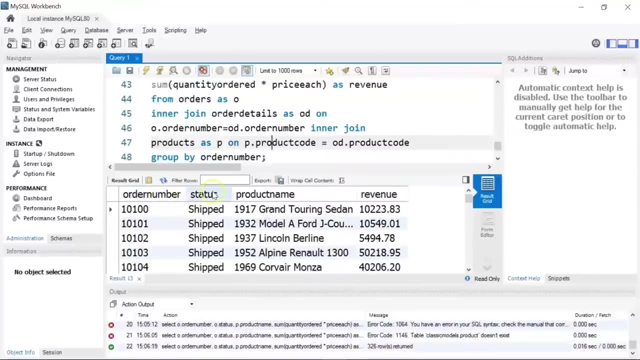 okay, there's still some error. it says classic models dot product doesn't exist. so again, the product name is- i mean, the table name is products and not product. so let's run it again. all right, there you go. so we have the order number, the status, the product name and the revenue. 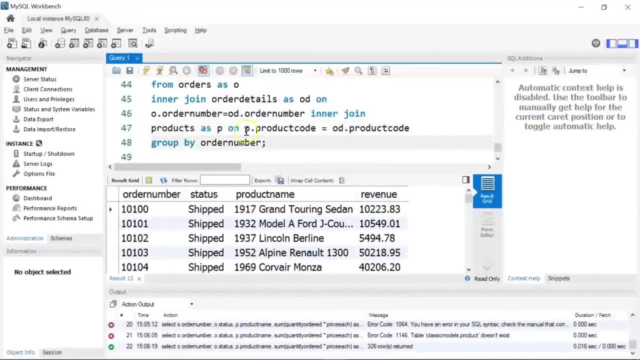 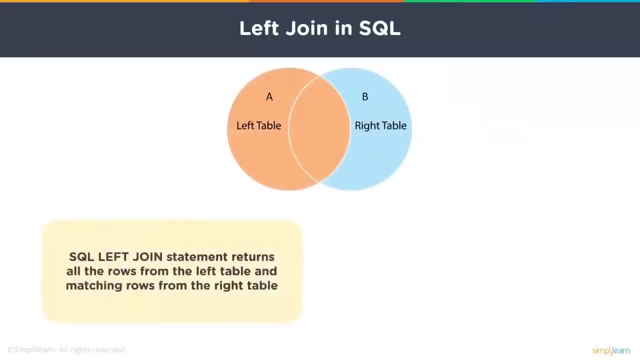 this. we got it using inner join from three different tables. now talking about left joins, the sql left join statement returns all the rows from the left table and the matching rows from the right table. so if you see this diagram, you can see we have all the rows from the left table. 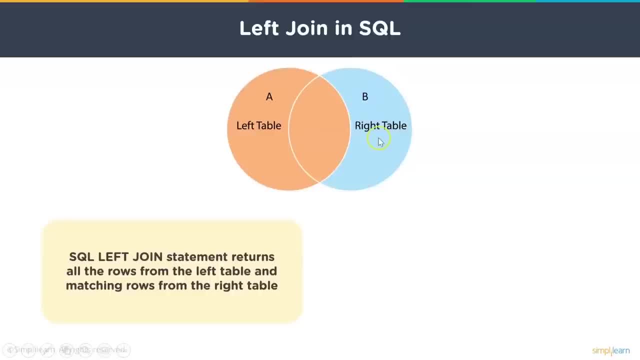 that is a, and only the matching rows from the right table, that is b. so you can see this overlapped region and the syntax for sql left join is something like this: so you have the select statement and then you give the list of columns from table a, which. 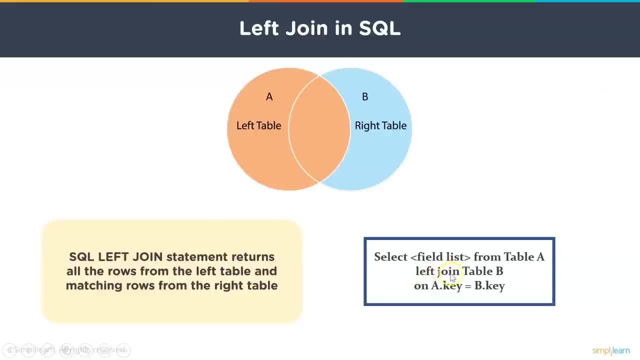 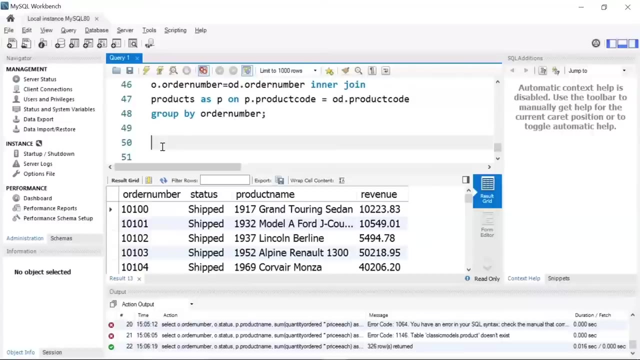 is your left table, then you use the left join keyword, followed by the next table, that is table b on the common key column. so you write: a dot key is equal to b dot key. okay, now in our classic models database we have two tables: customers and orders. so if you want to find, 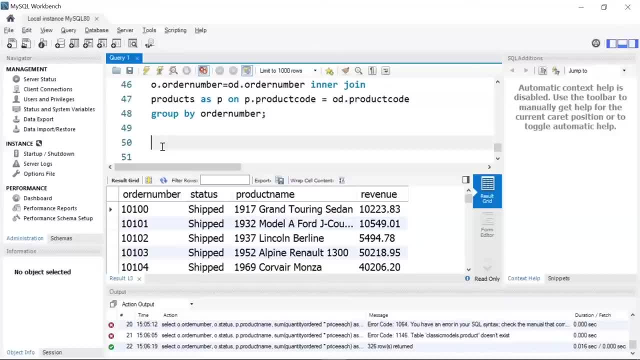 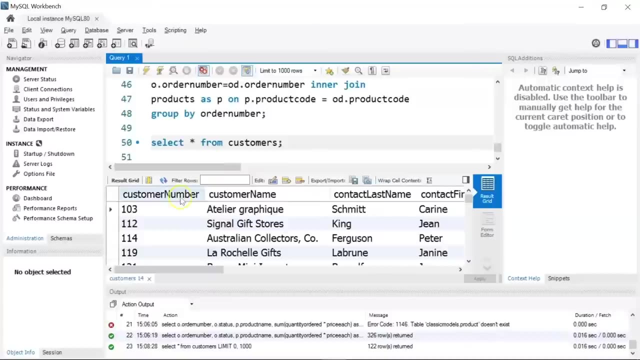 the customer name and their order id. you can use these two tables, so first let me show you the columns that are present in customers and orders. i think orders we have already seen. let me first show you what's there in the customers table. okay, so you can see, we have the customer number. 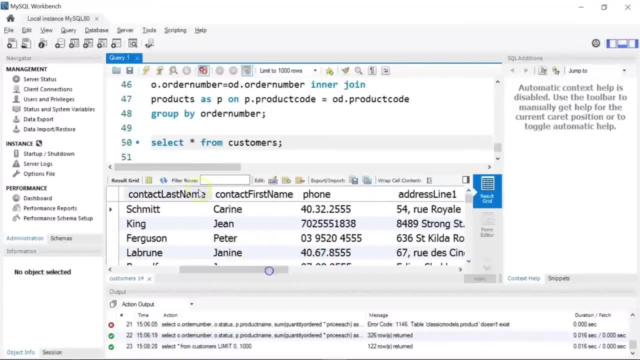 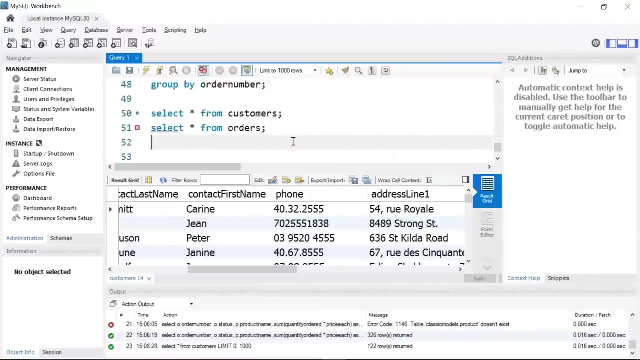 the name of the customer, then we have the contact last name, the contact first name. we have the phone number, then there's an address column. there are two address columns actually. we have the city name, the state and we have other information as well. and similarly we have our orders table. so i'll write select, start from orders, so i'll write select. 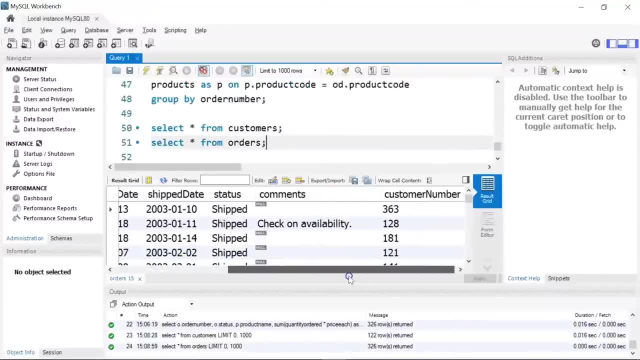 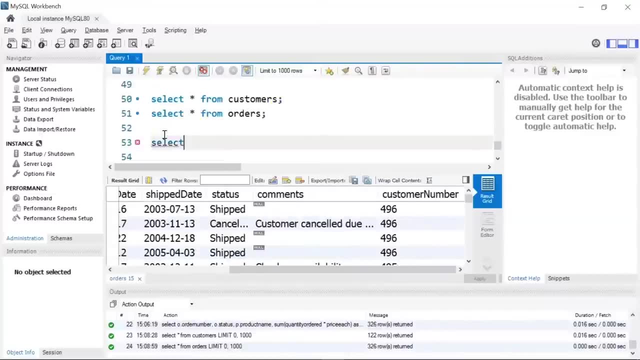 star from orders, where on this you can see: these are the information available in the orders table. okay, so let's perform a left join where we want to find the customer name and their order ids. so i'll write select c dot customer name, or let's say: first we'll choose the customer number. 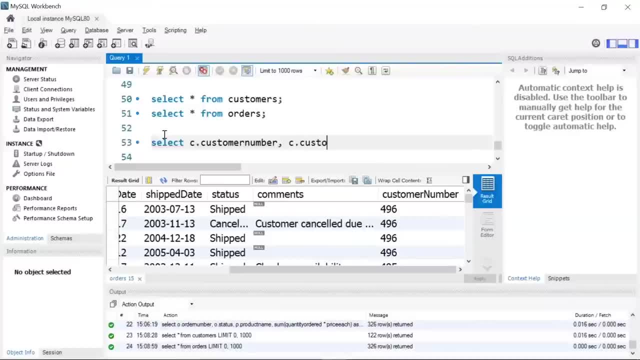 comma. then i want the customer name, so i'll write c dot customer name. then we have the order number column which is present in the orders table, and let's say i also want to see the status. then i'll give my left table, that is customers, as c left join. 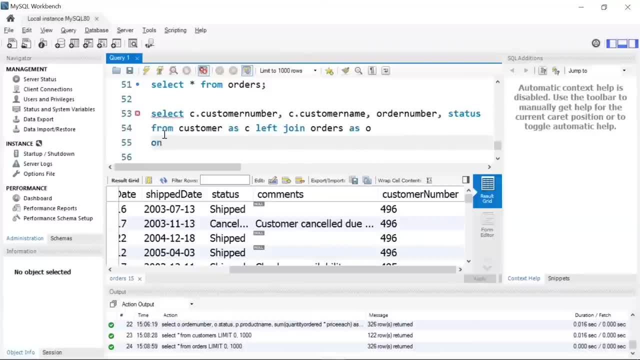 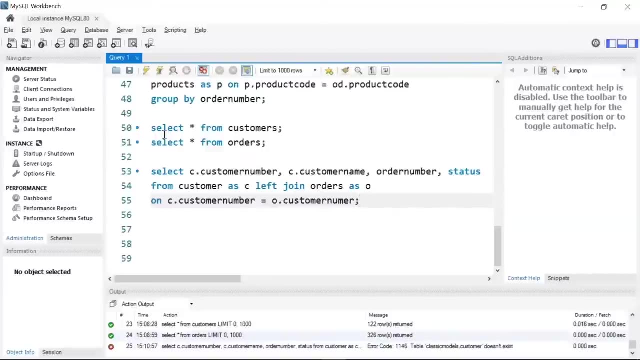 orders as o on c dot customer number equal to o dot customer number. let's run it okay again. there is some problem. all right, so the table name is customers. let's run it. so there's another mistake here. this is customer number, so b is missing. cool, let me run it all right. so here you can see we have the information regarding. 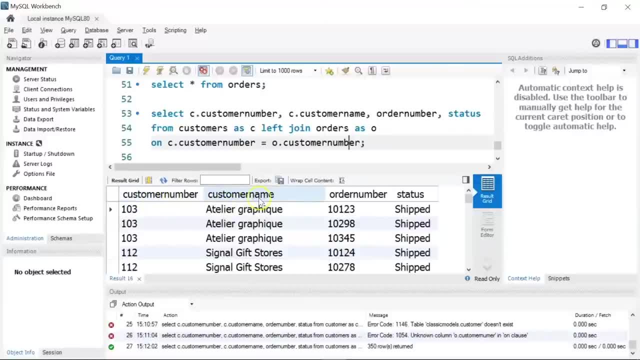 the customer number, then the respective customer names. we have the order number and the user name, the status of the shipment. so if I scroll down, you'll notice one thing: there are a few rows you can see which have null values. this means for customer number 125 and for this particular customer name, there were no orders and 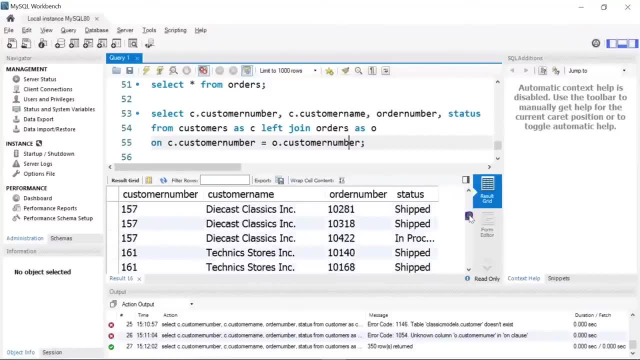 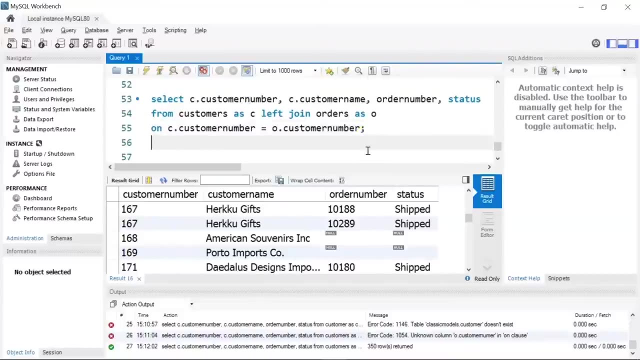 similarly, if I scroll down, you will find a few more null values. you can see here: there are two null values here for customer number 168 and 169. there were no orders available all right now. to check those customers who haven't placed any orders, you can use the null operator. so what I'll do is here, I'll just 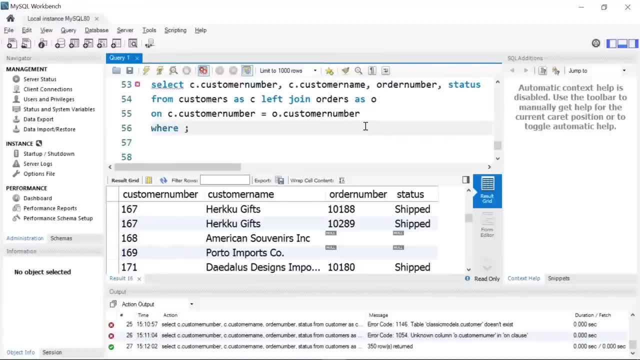 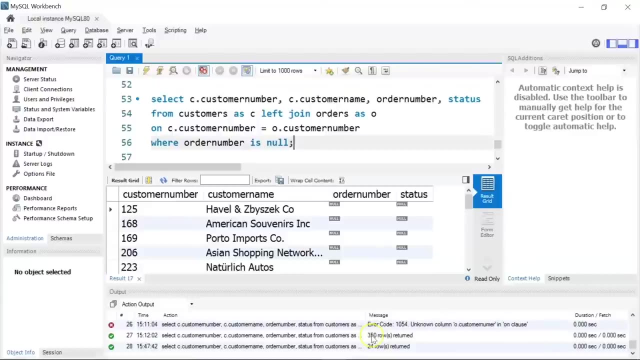 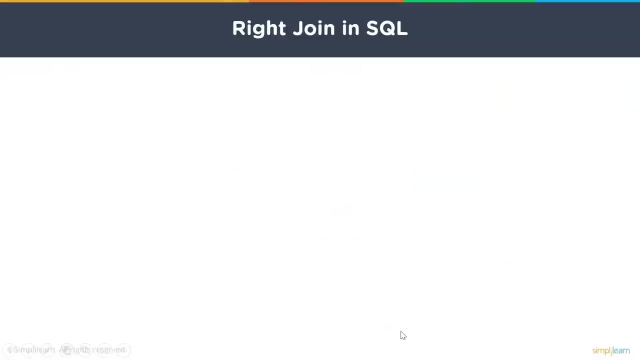 continue with this, I'll use a where clause and write where order number is null. now let me run this. okay, so here you can see there are 24 customers from the table that don't have any orders in their names. okay, now talking about right joins. so SQL right join statement returns all the rows from: 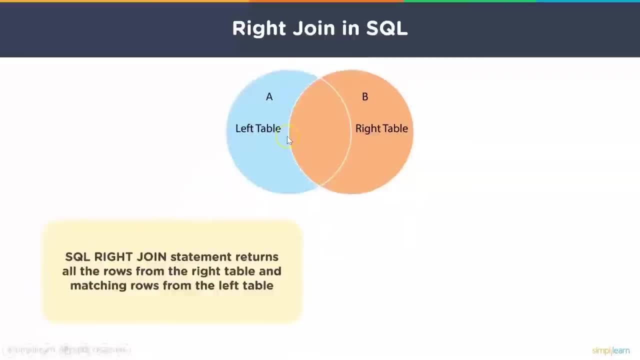 the right table and only matching rows from the left table. so here you can see, we have our left table as a and the right table as B, so the right join will return all the rows from the right table and only the matching rows from the left table. 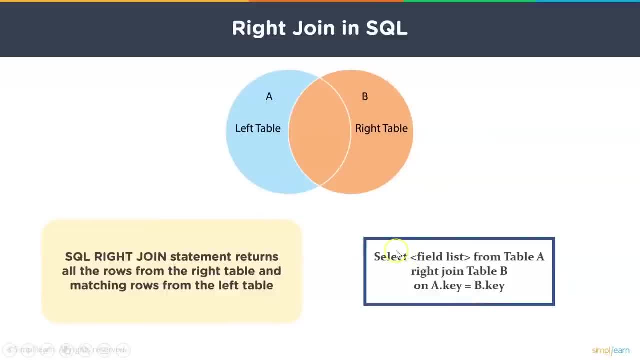 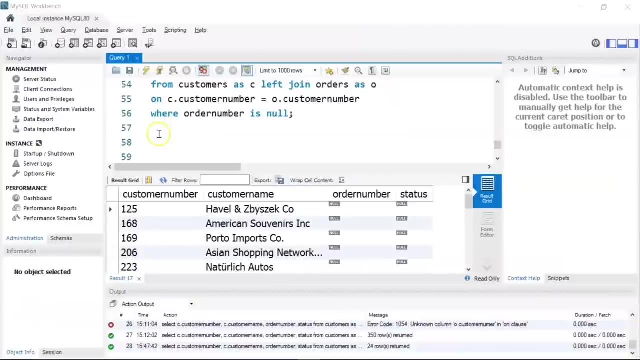 now talking about the syntax. so here you can see, we have the select statement. followed by the select statement, you will have the list of columns that you want to choose from. table a, right join. table B, on the common key column from both the tables. all right, now to show how right join works, I'll be using two. 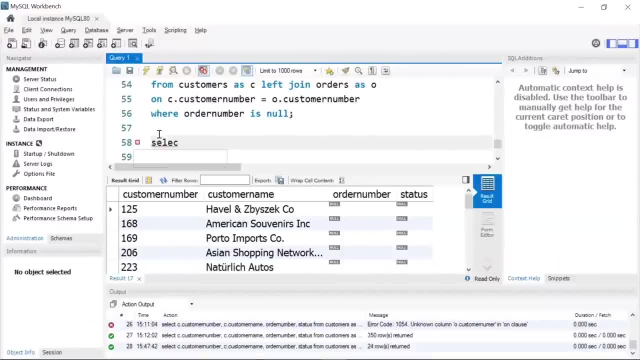 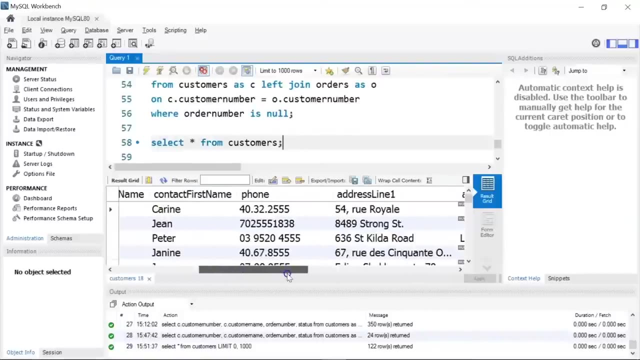 tables, that is, customers and employees. so let's see the rows of data that are present in the customer table first. so I'll write select star from customers. let's run it so. here you have the customer number, the customer name, then we have the phone number, the address of the customers you also have 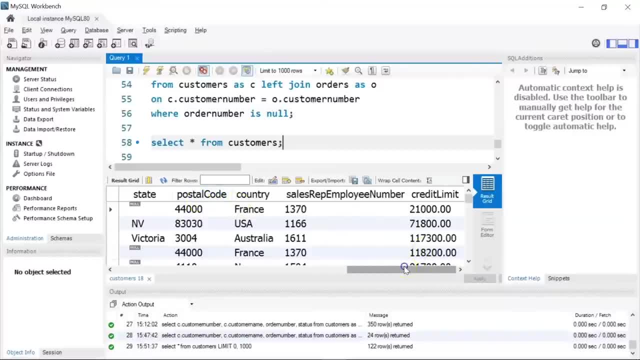 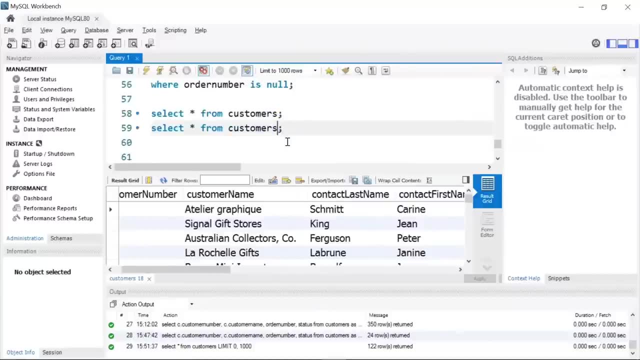 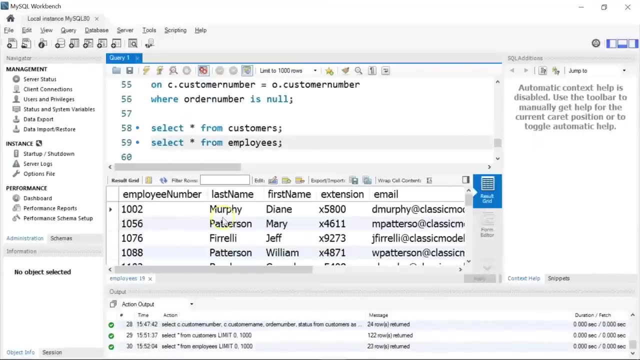 the country to which the customer belongs to, the postal code and the credit limit as well. similarly, let's see for the employees table: here I'll change customers to employees. let's run it okay. so we have the employee number, the last name, the first name, you have the. 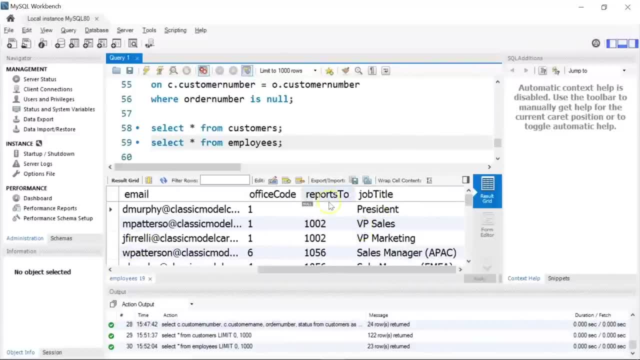 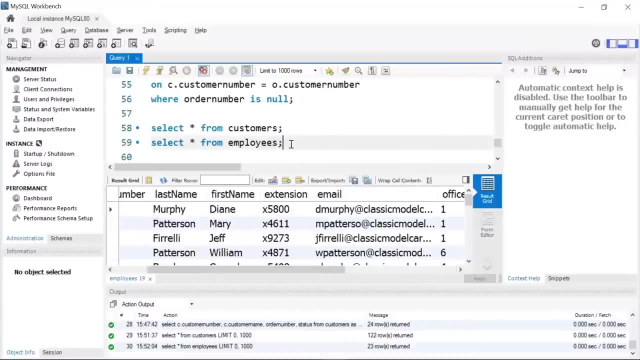 extension, the email ID, the job title and also reports to. here means the manager. okay, so based on these two tables, we'll find the customer name, the phone number of the customer and the email address of the employee and join both the tables, that is, customers and employees. so let me show you the command, so I'll write. 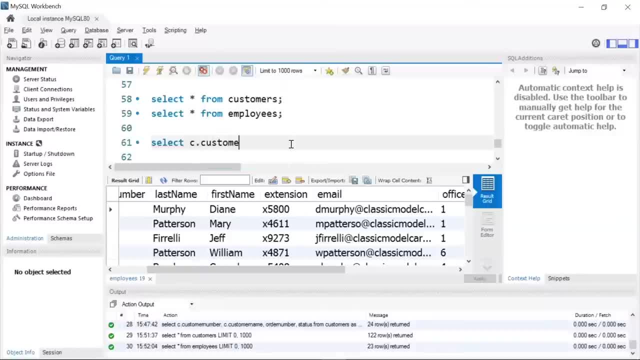 select c dot customer name commas, then we have c dot phone. I'll give a space here. next I want the employee number from the employee table, so I'll write E dot employee number comma. E dot. email from customers as see right. join sheer website's business and here we found this command. all the time we do not have to Ghost hochooo, this is just to get. 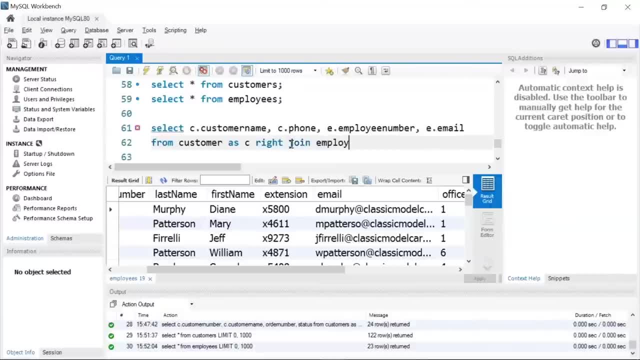 employees as E on E dot. my common key column is employee number here, so I'll write E dot. employee number is equal to C dot. we have sales representatives employee number and I'm also going to order it by the employee number column. okay, so you can see. I have my customer name selected from the customers table. 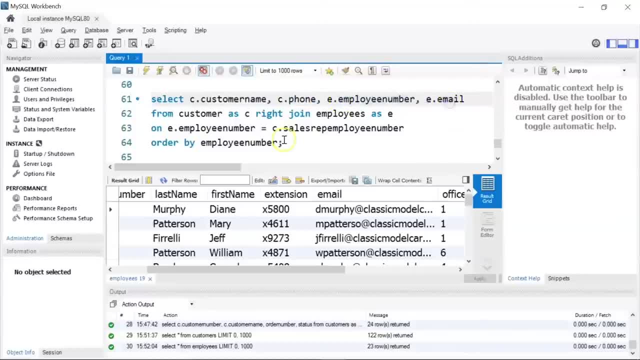 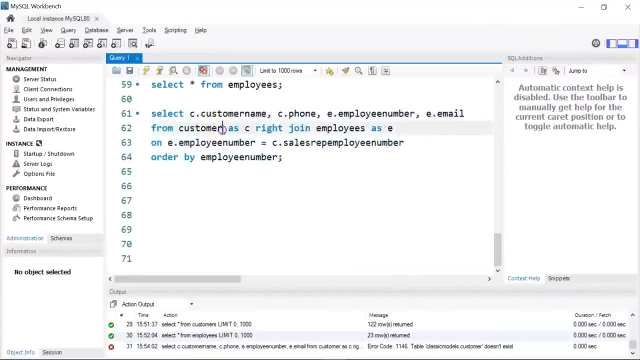 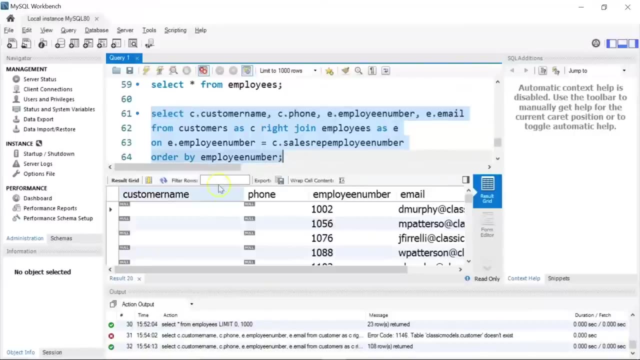 the phone number of the customer, then we have the employee number and the email address. so let me run it. okay, there's some problem? all right, so the table name is customer number and then we have the customer number and then we have the customers. actually, let's run it once again. there you go, so you can see here. 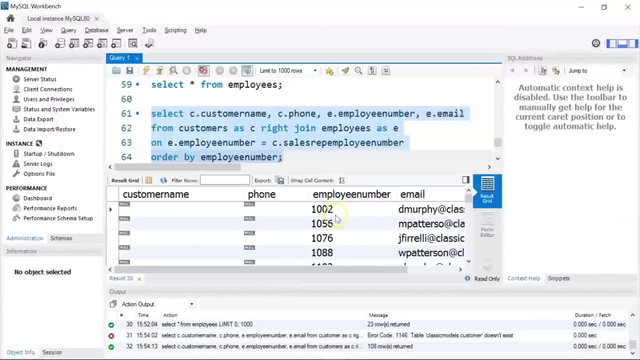 we have all the values selected from our right table, which is the employees table. you can see rights on employees, which means your employees table is to the right, and then we have the customer name and phone numbers of the customers from the customer table, which is actually your left table. so you have a few. 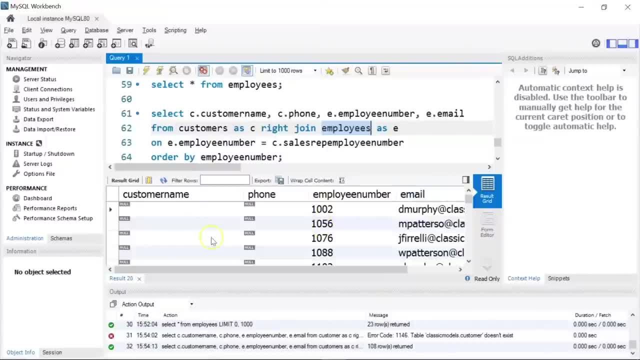 employee numbers such as 1002. there's 1056 which don't have any customer name or phone numbers. okay, so there's another popular join which is very widely used in sql, known as self joins. so self joins are used to join a table to itself. so in our database we have a table called employees. 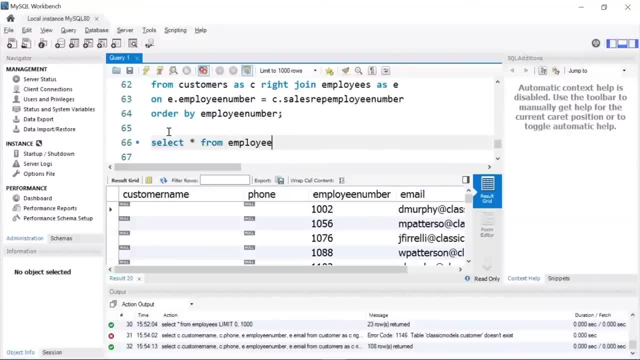 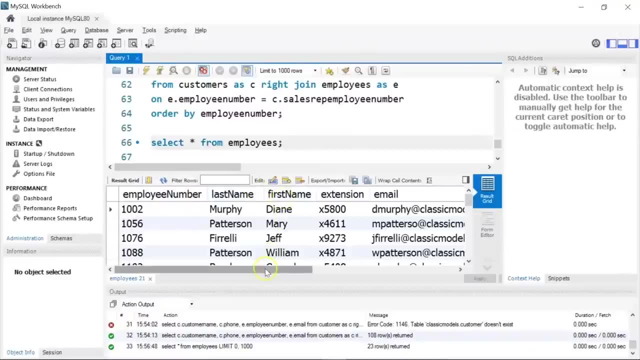 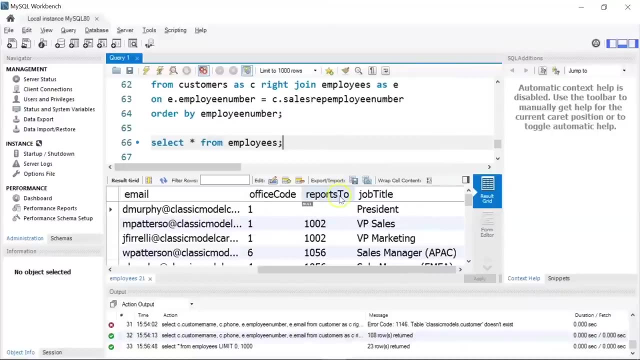 let me show you the table first. all right, so here you can see, we have the employee number, the last name, the first name of the employee, we have the email id and here, if you see, we have a column called reports 2. now this you can think of as the manager column. so the way to read is: 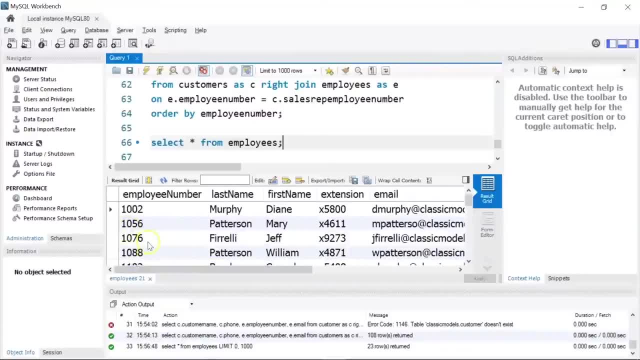 for example, for employee number 1056, the manager is 1002. so if you check the following WHISPLEW associate number 1056, you will see a manager is 1002. so if you check the following WHISPLEW associate number 1056, you will see a manager is 1002. so if you 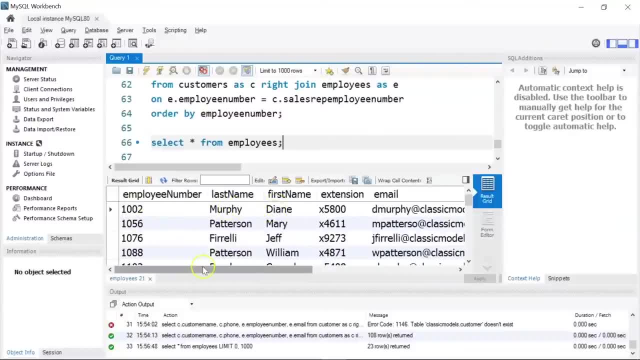 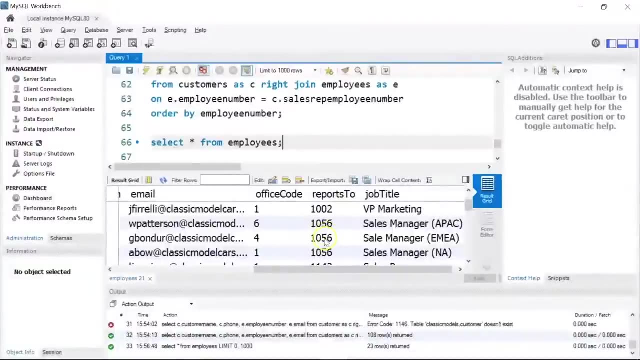 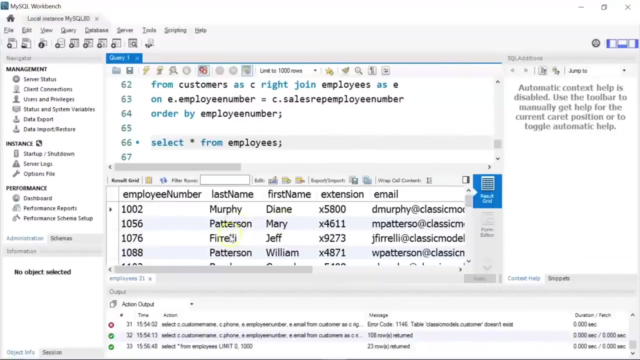 for 1002, we have dane murphy. then if i scroll down, let's say for employee number 1102, yeah, for employee number 1102 the manager is 1056. so here you can see who is. at 1056 you have mary patterson. similarly, if i scroll down, let's say for employee number 1188, we have 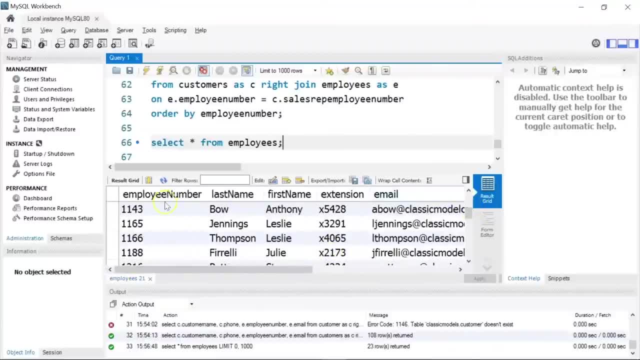 the manager as 1143. now, if i check the table, at 1143 we have anthony bow. so so the employee julie farelli reports to anthony bow. all right now. suppose you want to know who is the reporting manager for each employee. so for that you can use a self join. so let me show you how. 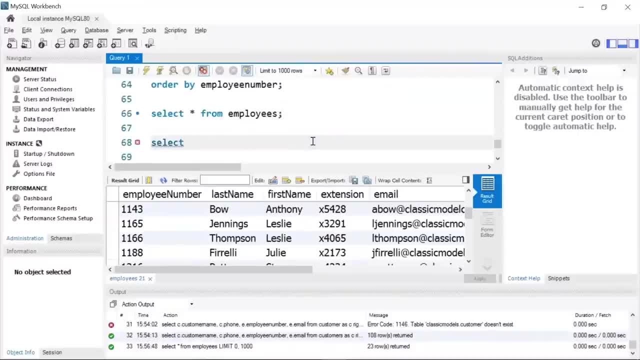 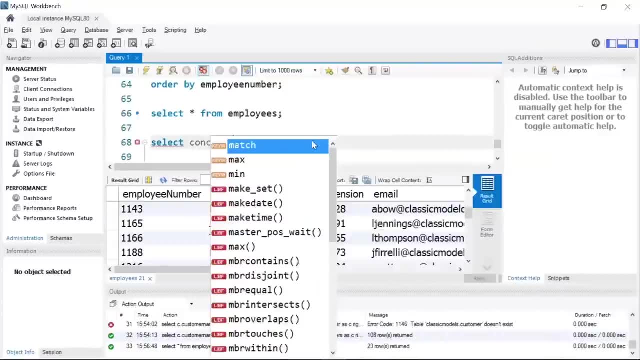 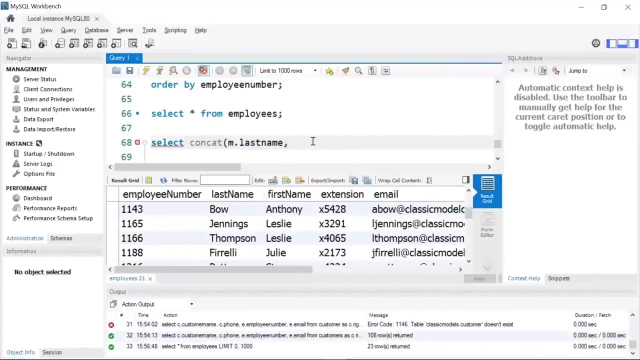 to join this employees table. I'll write select and then I am going to use a function called concat within brackets. I'll start with my alias name, that is, M dot, then I'll write last name. I'm going to concat last name, followed by a comma. then I'll have my first name. I'll close this bracket and then I'm going to give. 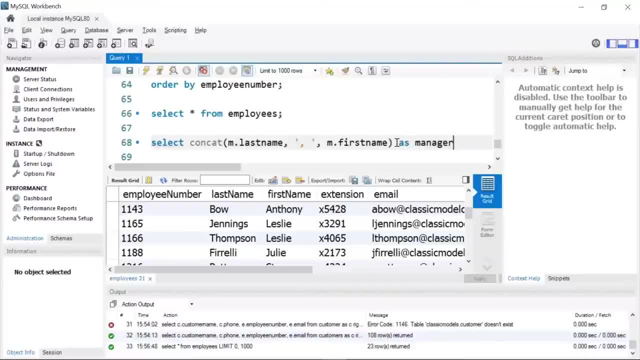 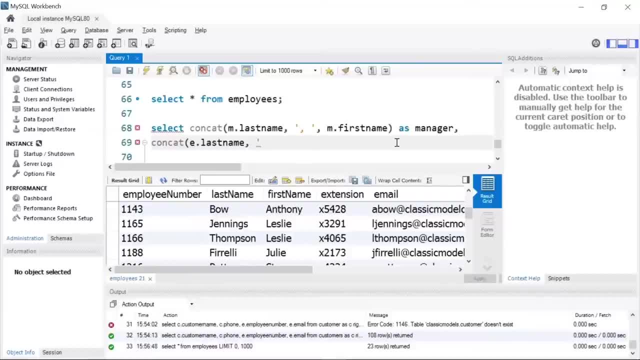 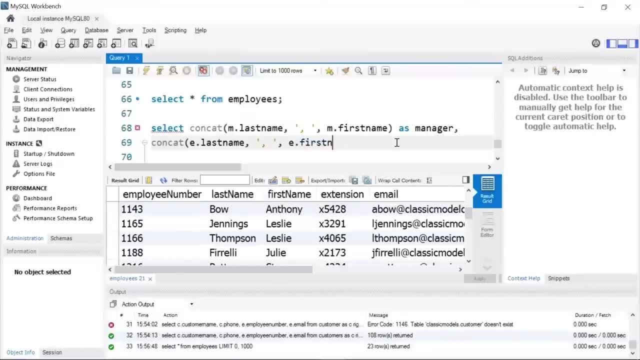 quotes. I'll give my comma and then I'll write E dot first name. I close this. write E dot first name. I close this. write E dot first name. I close this bracket. I'll give an alias as let's say bracket. I'll give an alias as let's say: 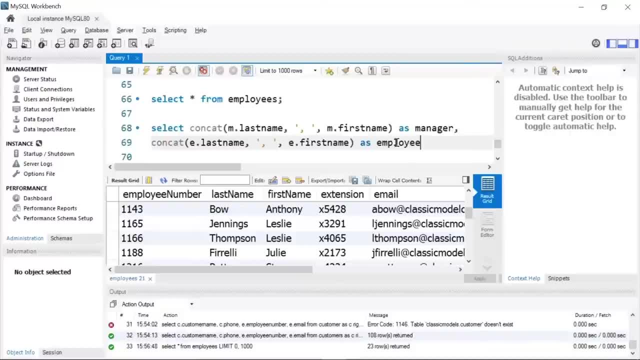 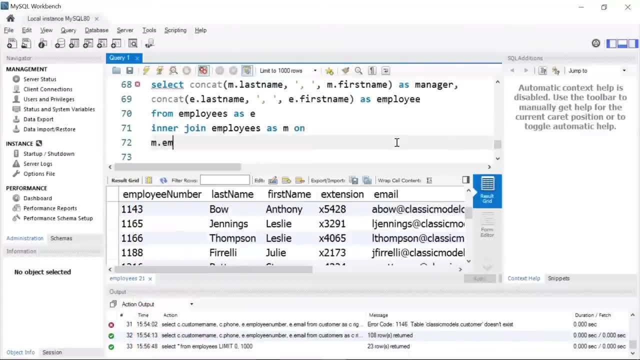 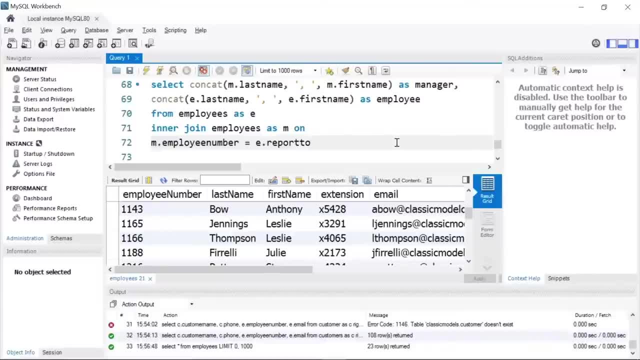 dot. I'll use my common key column as dot. I'll use my common key column as employee number. so I'll write M dot employee number. so I'll write M dot employee number. so I'll write M dot. employee number is equal to E dot. here I'm. 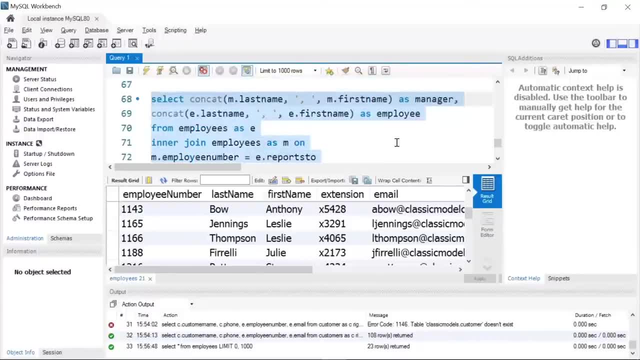 employee number is equal to E dot. here I'm. employee number is equal to E dot. here I'm going to use the reports to column and going to use the reports to column, and going to use the reports to column, and okay, now let's run this. there you go, so. 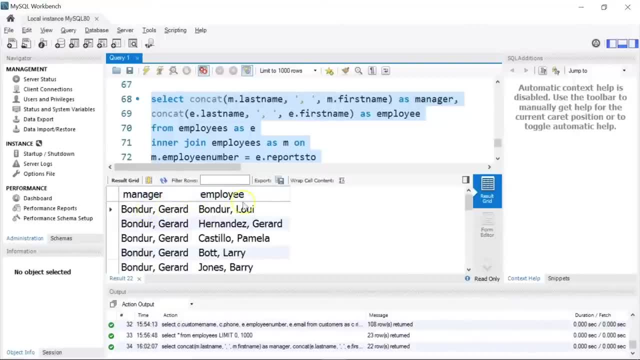 okay, now, let's run this, there you go. so okay, now, let's run this, there you go. so you have your two columns as manager and you have your two columns as manager and you have your two columns as manager and employee. so for employee Louie bonder, 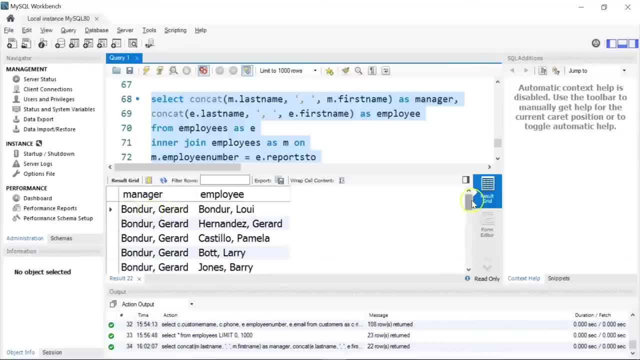 employee: so for employee Louie bonder. employee: so for employee Louie bonder. the manager is Zerat bonder. similarly, if the manager is Zerat bonder. similarly, if the manager is Zerat bonder. similarly, if I scroll down, you have there are. 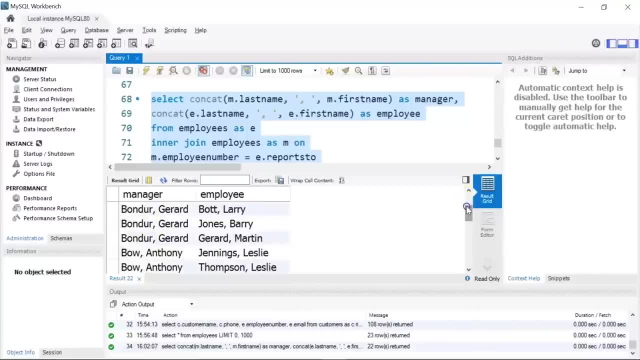 I scroll down, you have, there are. I scroll down, you have, there are multiple employees reporting to this, multiple employees reporting to this, multiple employees reporting to this particular manager. similarly, we have our particular manager. similarly, we have our particular manager. similarly, we have our manager as Anthony bow and we have. 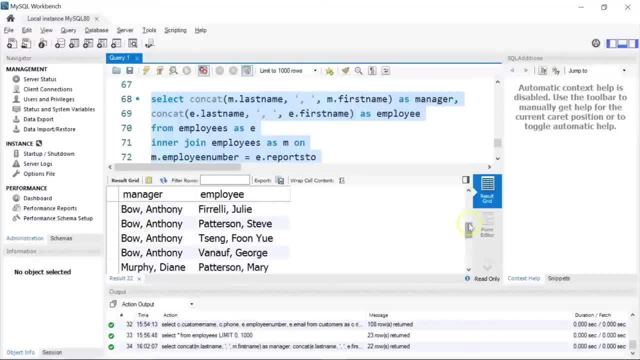 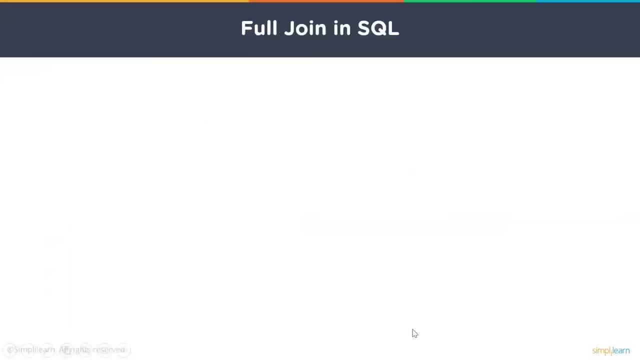 different employees who are reporting to different employees, who are reporting to different employees, who are reporting to this particular manager, and so on. this particular manager, and so on. this particular manager, and so on. all right now, moving ahead. all right now, moving ahead. all right now, moving ahead. now let's see what a full join is. so 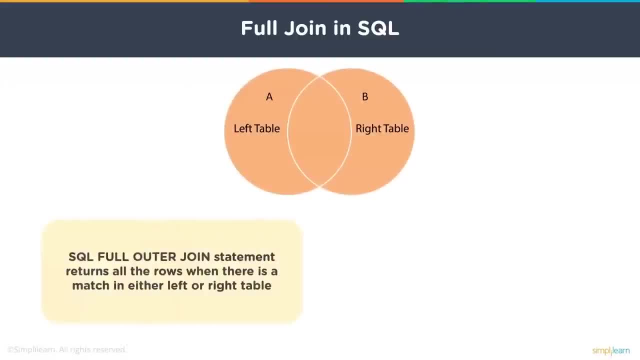 now let's see what a full join is. so now let's see what a full join is. so SQL full outer join statement returns. SQL full outer join statement returns. SQL full outer join statement returns all the rows when there is a match in: all the rows when there is a match in. 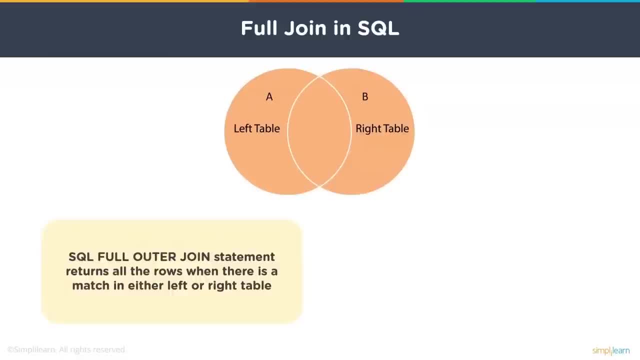 all the rows when there is a match in either left or right table. now you must either left or right table now. you must either left or right table now. you must remember that my sequel workbench does remember that my sequel workbench does remember that my sequel workbench does not support full outer join by default. 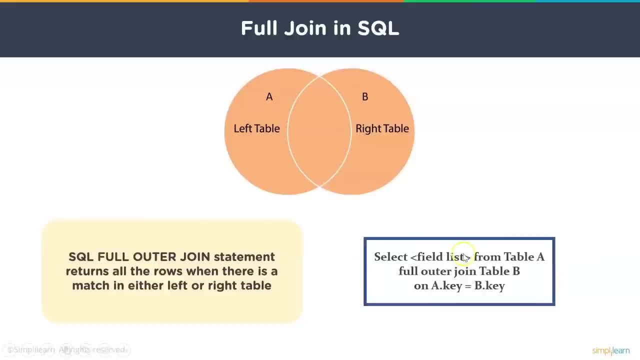 not support full outer join by default. not support full outer join by default, but there's a way to do it so by default. but there's a way to do it so by default. but there's a way to do it so by default. this is how the syntax of full outer 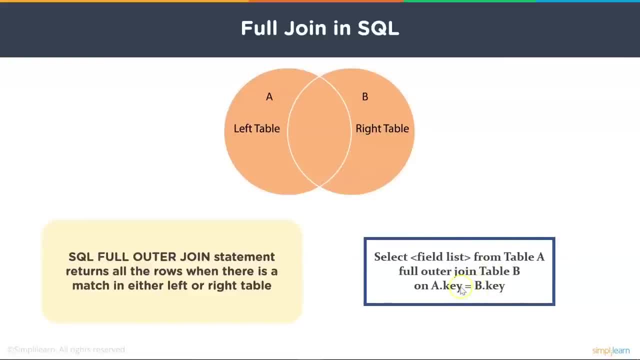 this is how the syntax of full outer. this is how the syntax of full outer join looks like now this statement will join. looks like now this statement will join. looks like now this statement will work on other SQL databases. like work on other SQL databases. like work on other SQL databases like Microsoft SQL server. but it won't work. 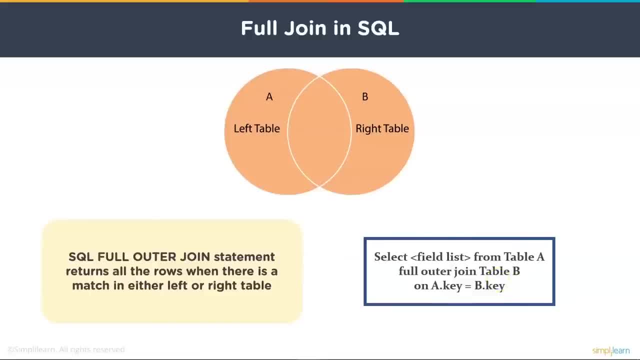 Microsoft SQL server, but it won't work. Microsoft SQL server, but it won't work. on my sequel workbench I'll show you the on my sequel workbench. I'll show you the. on my sequel workbench. I'll show you the right way of using full outer. join on my. 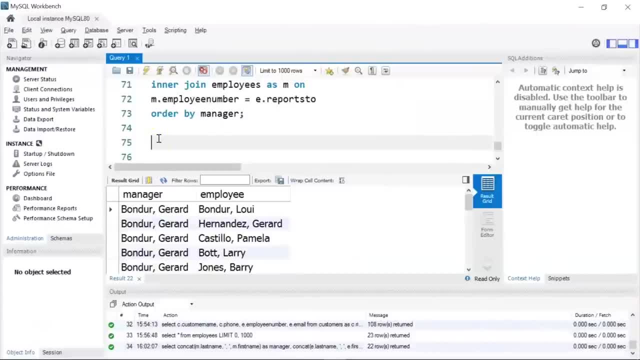 right way of using full outer join on my right way of using full outer join on my sequel workbench. so to so full outer sequel workbench. so to so full outer sequel workbench. so to so full outer join. I am going to first use a left join. 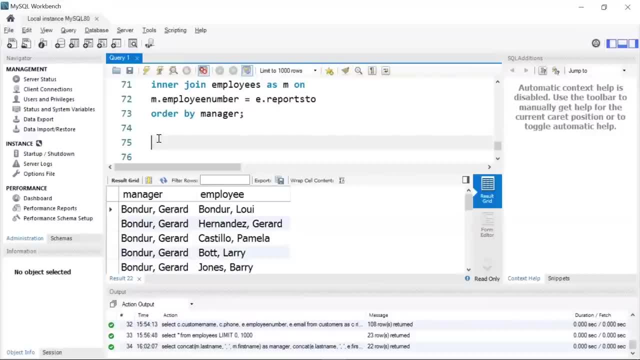 join. I am going to first use a left join join. I am going to first use a left join, and then we'll also use a right join, and then we'll also use a right join, and then we'll also use a right join, and finally we'll use a union operator. so 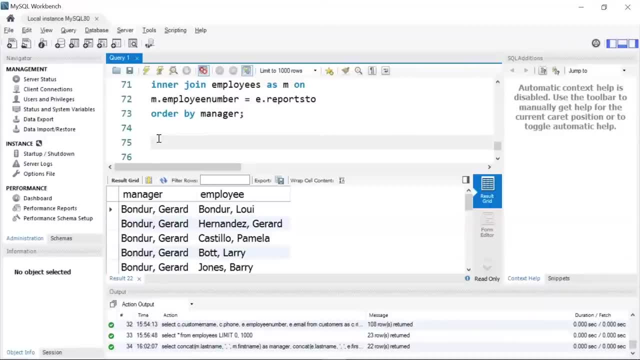 and finally, we'll use a union operator. so and finally, we'll use a union operator. so the union operator is used to combine. the union operator is used to combine. the union operator is used to combine: the result set of two or more select. the result set of two or more select. 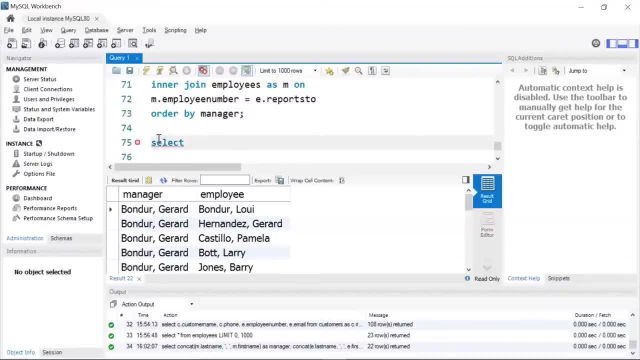 the result set of two or more select statements. so first of all, let me write statements. so first of all let me write statements. so first of all let me write C dot customer name. so for this example, C dot customer name. so for this example, C dot customer name. so for this example, I'm using the customer table and the 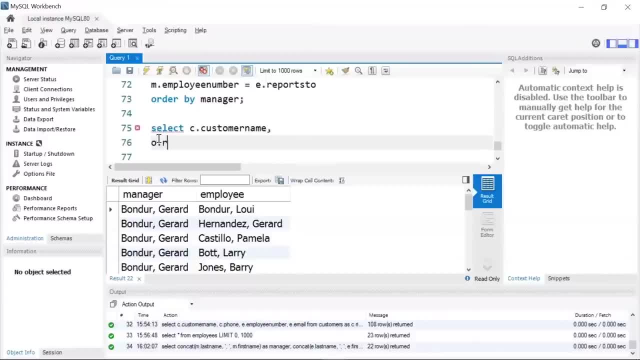 I'm using the customer table and the. I'm using the customer table and the order table: comma o dot order number. so order table: comma o dot order number. so order table: comma o dot order number. so I just want to know the customer name. I just want to know the customer name. 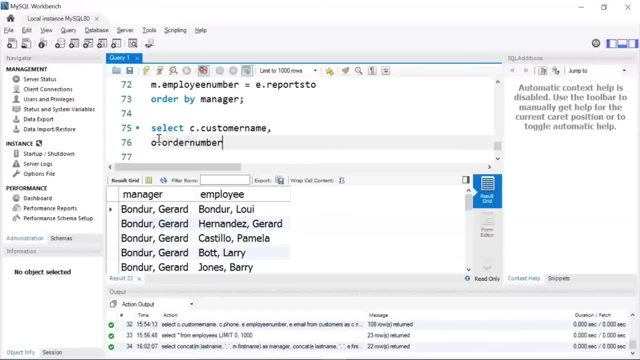 I just want to know the customer name and the order number related to the and the order number related to the and the order number related to the customer from. I have customers as C customer from. I have customers as C customer from. I have customers as C left. join. I'll write orders as O on C. 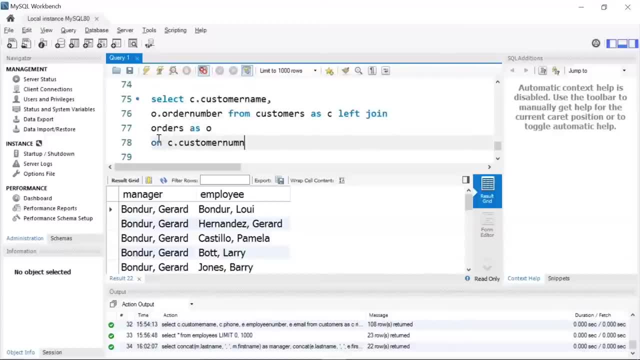 left join. I'll write orders as O on C. left join. I'll write orders as O on C. dot customer number is equal to o dot. dot customer number is equal to o dot. dot customer number is equal to o dot customer number. let me just copy this: 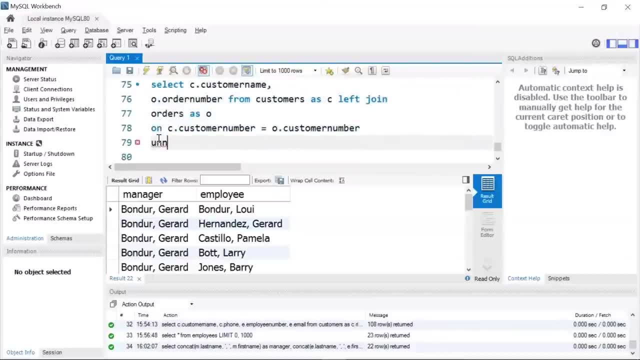 customer number. let me just copy this customer number. let me just copy this. and after this I am going to use my, and after this I am going to use my, and after this I am going to use my. union operator, so union operator is used. union operator, so union operator is used. 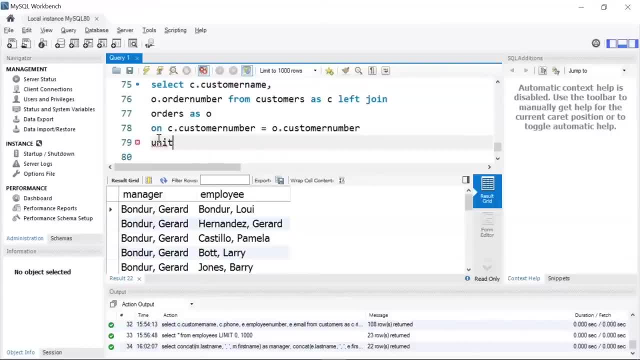 union operator, so union operator is used to, to to merge results from two or more tables, so merge results from two or more tables. so merge results from two or more tables. so basically, this performs a vertical join. basically this performs a vertical join. basically this performs a vertical join. and next I am going to use my right. 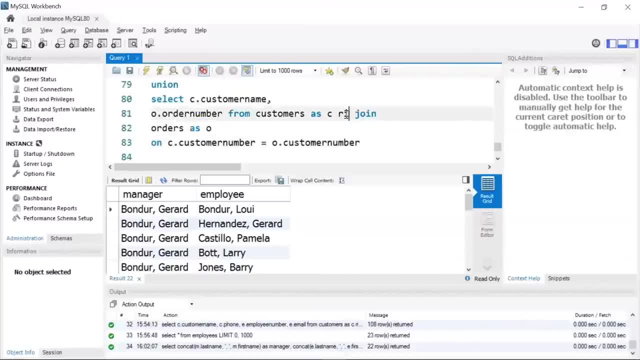 and next I am going to use my right, and next I am going to use my right join operation. so here instead of left join operation. so here instead of left join operation. so here instead of left join, I will write right join. I will write right join. I will write right. this tall looks fine, let me just run it. 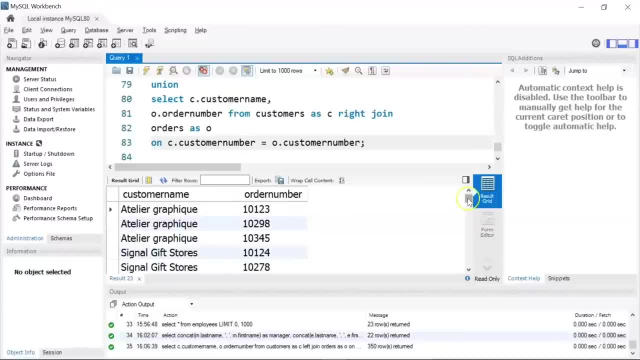 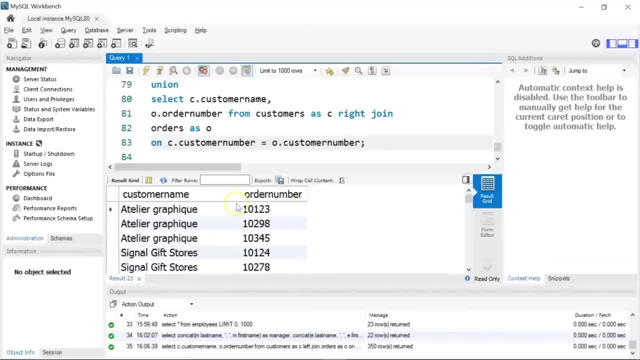 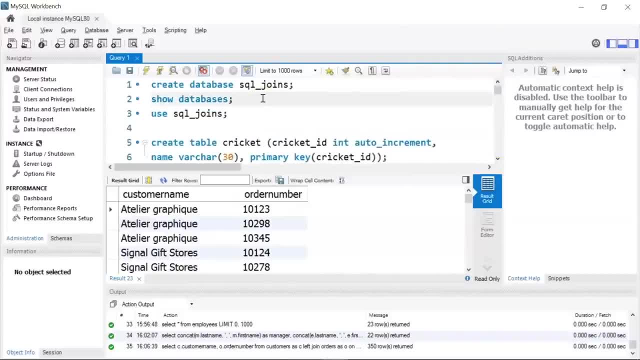 that each customer had placed alright. so that each customer had placed alright. so that brings us to the end of our demo. that brings us to the end of our demo. that brings us to the end of our demo session. so let me just run through session. so let me just run through. 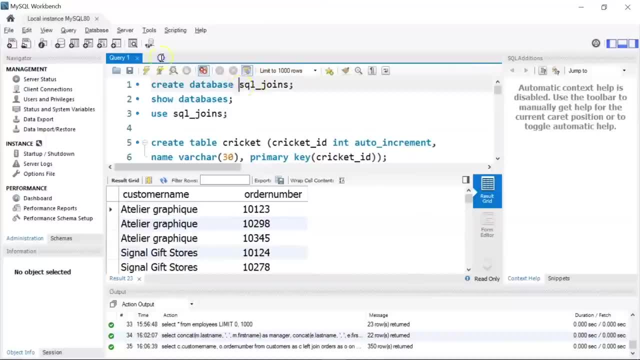 session. so let me just run through whatever we did in this session. so first, whatever we did in this session. so first, whatever we did in this session. so first we created a database called SQL joins. we created a database called SQL joins. we created a database called SQL joins. then we created two tables like cricket. 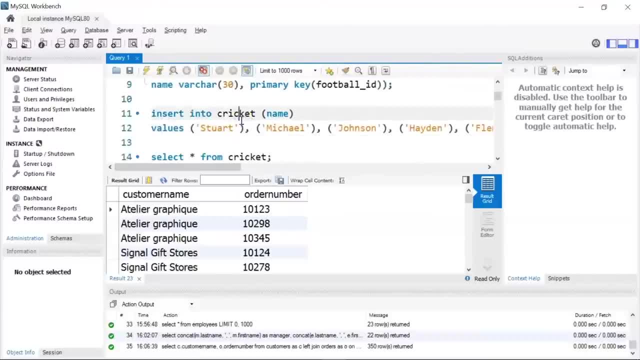 then we created two tables like cricket. then we created two tables like cricket and football, then we had inserted a few. and football, then we had inserted a few, and football, then we had inserted a few rows to each of these tables. then we rows to each of these tables, then we 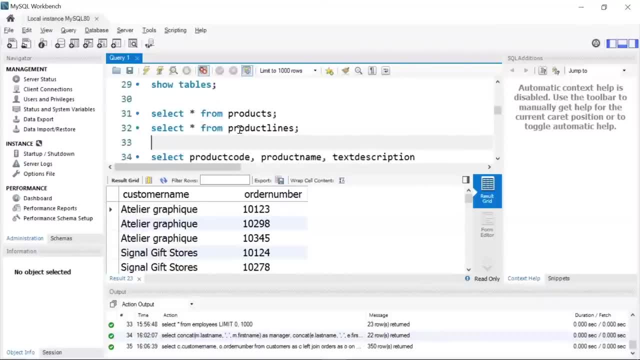 rows to each of these tables. then we used this table to learn about inner, used this table to learn about inner. used this table to learn about inner join. next, we used a database called join. next, we used a database called join. next, we used a database called classic models. it had multiple tables, so 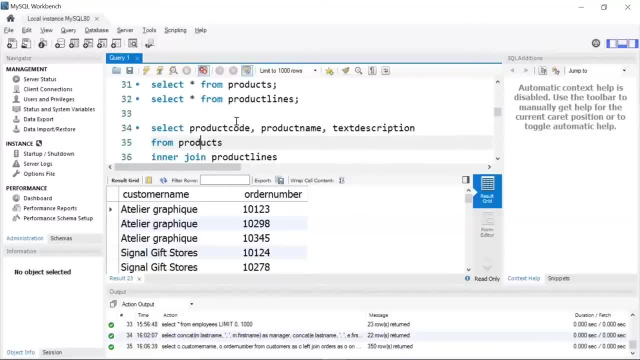 classic models: it had multiple tables. so, classic models: it had multiple tables. so we explored all of these tables. like we explored all of these tables. like we explored all of these tables like products: there was product lines, orders. products: there was product lines, orders products. there was product lines, orders customers and employees, and learnt how. 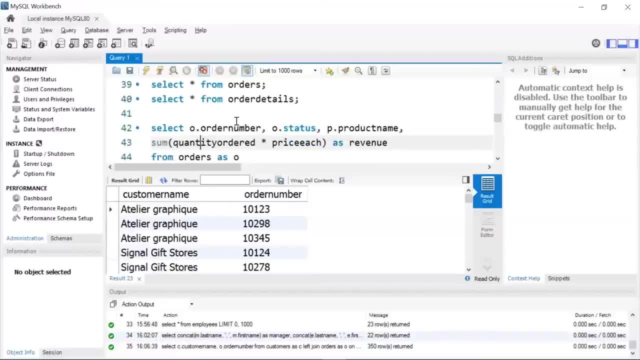 customers and employees and learnt how customers and employees and learnt how to use inner join, left join, self join to use inner join, left join, self join. to use inner join, left join, right join as well as full outer join in this video- right join as well as full outer join in this video. 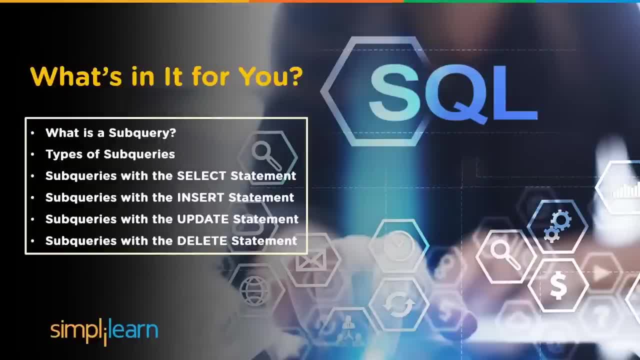 right join as well as full outer join. in this video, we will learn what is a sub. we will learn what is a sub. we will learn what is a sub query and look at the different types of sub query. and look at the different types of sub query and look at the different types of sub queries. then we learn sub queries. 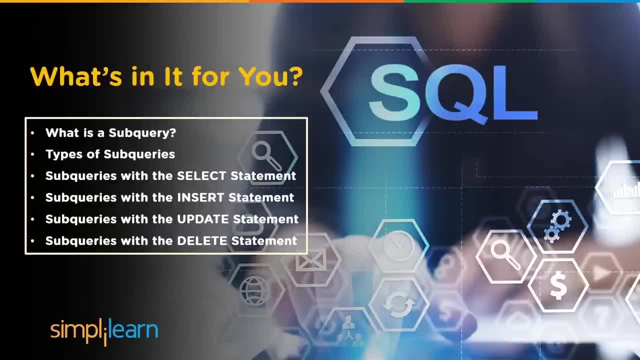 queries, then we learn sub queries. queries, then we learn sub queries, with select statement followed by sub, with select statement, followed by sub, with select statement, followed by sub queries with insert statement. moving queries with insert statement. moving queries with insert statement. moving further, we will learn sub queries with 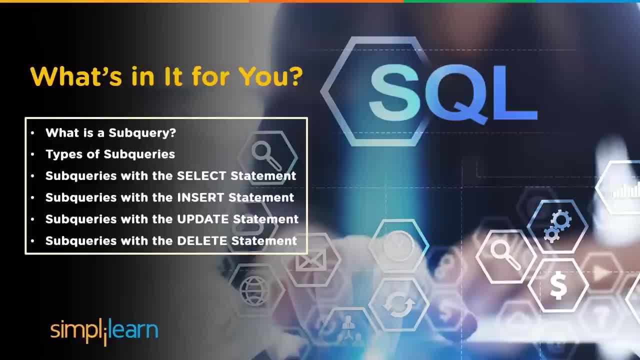 further we will learn sub queries with further we will learn sub queries with the update statement and finally we look the update statement and finally we look the update statement and finally we look at sub queries with delete statement, all at sub queries with delete statement, all at sub queries with delete statement. all this we will be doing on our mysql. 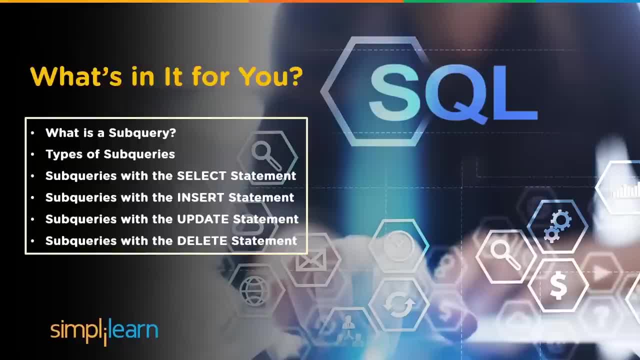 this we will be doing on our mysql, this we will be doing on our mysql workbench, workbench, workbench. so, before i begin, make sure to subscribe. so, before i begin, make sure to subscribe. so, before i begin, make sure to subscribe to the simply learn channel and hit the. 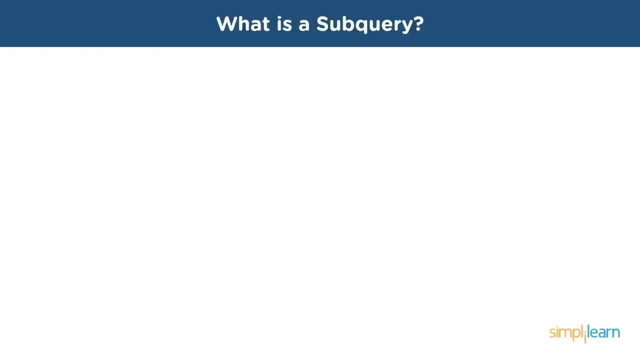 to the simply learn channel and hit the. to the simply learn channel and hit the bell icon to never miss an update. bell icon to never miss an update. bell icon to never miss an update. so let's start with what is a sub query. so let's start with what is a sub query. 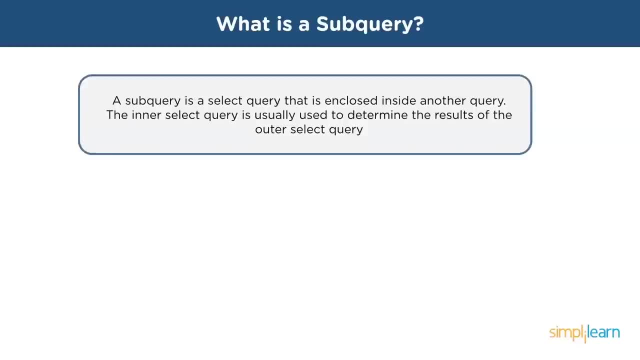 so let's start with what is a sub query? so a sub query is a select query, that is so. a sub query is a select query, that is so. a sub query is a select query that is enclosed inside another query. enclosed inside another query, enclosed inside another query. so if i show you, this is how. 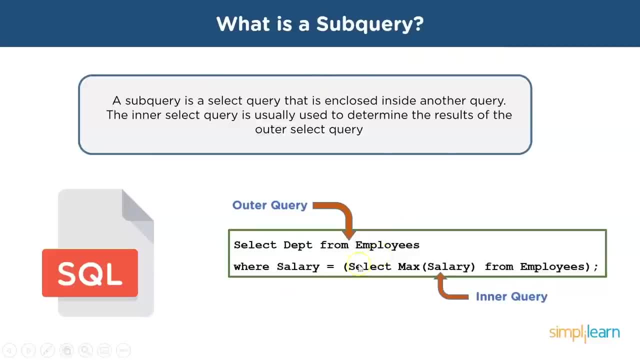 so if i show you this is how, so if i show you this is how the basic structure of a sub query looks, the basic structure of a sub query looks. the basic structure of a sub query looks like like like so here, whatever is present inside the. so here, whatever is present inside the. 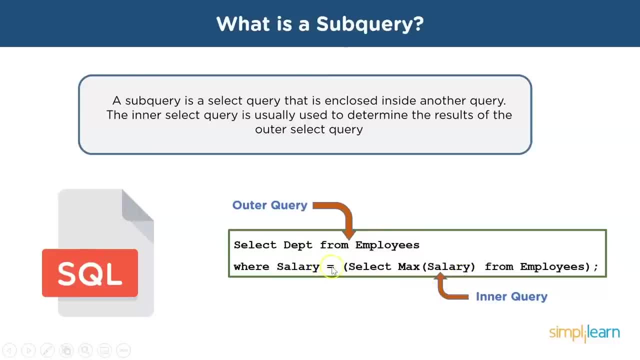 so here whatever is present inside the brackets is called as the inner query, brackets is called as the inner query, brackets is called as the inner query, and whatever is present outside is called, and whatever is present outside is called, and whatever is present outside is called the outer query. 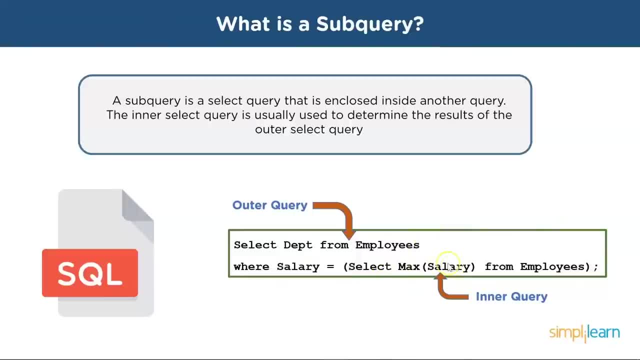 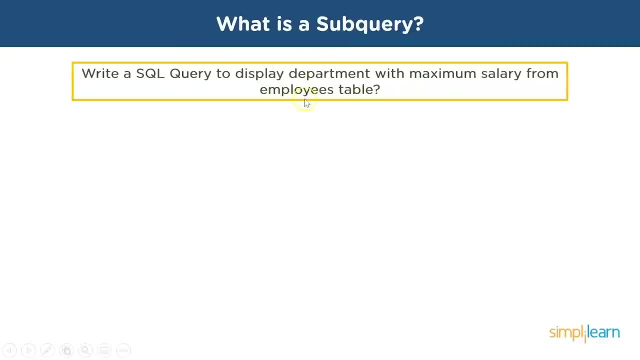 the outer query, the outer query. so first the inner query gets executed, so first the inner query gets executed. so first the inner query gets executed and the result is returned to the outer, and the result is returned to the outer and the result is returned to the outer. question at hand, which is to write a: 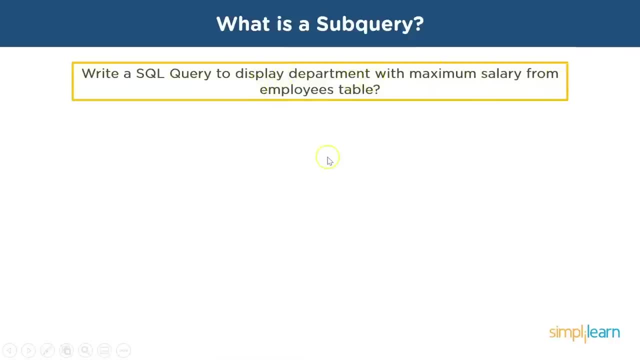 question at hand, which is to write a question at hand, which is to write a sql query to display department with sql query to display department with sql query to display department with maximum salary from employees table. maximum salary from employees table. maximum salary from employees table. so this is how our employees table looks. 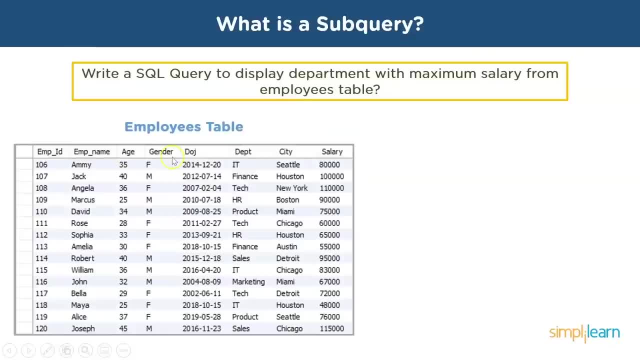 so this is how our employees table looks. so this is how our employees table looks like. it has the employee id: the like. it has the employee id: the like. it has the employee id, the employee name, age, gender. we have the employee name, age, gender. we have the. 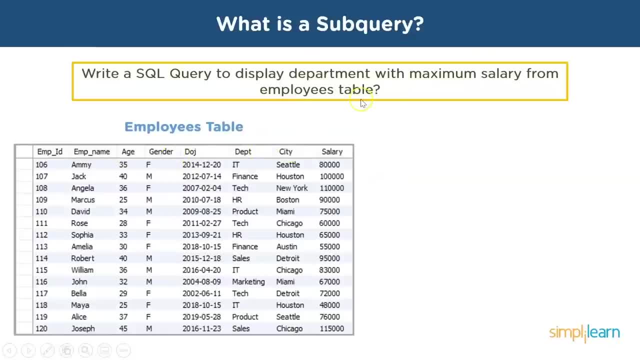 employee name, age, gender. we have the date of join department, city and salary: date of join department, city and salary. date of join department: city and salary. now to solve this query. now to solve this query. now to solve this query. my sub query would look like this: my sub query would look like this: 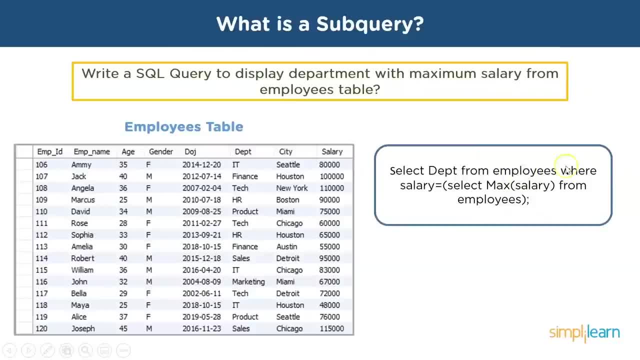 my sub query would look like this: so i'll first select the department from. so i'll first select the department from. so i'll first select the department from my table, that is employees. my table that is employees. my table that is employees, where i'll use the condition salary. 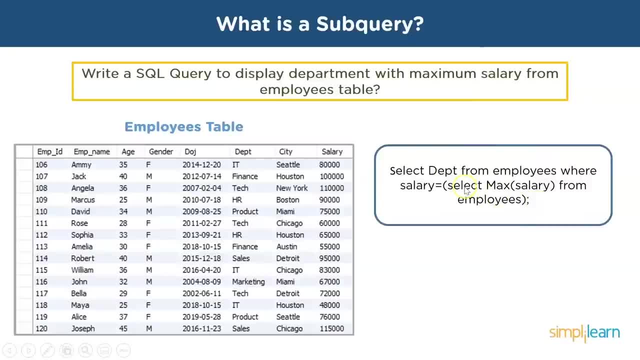 where i'll use the condition salary, where i'll use the condition salary equal to, equal to, equal to, and then i'll pass in my inner query, and then i'll pass in my inner query, and then i'll pass in my inner query which is select? which is select. 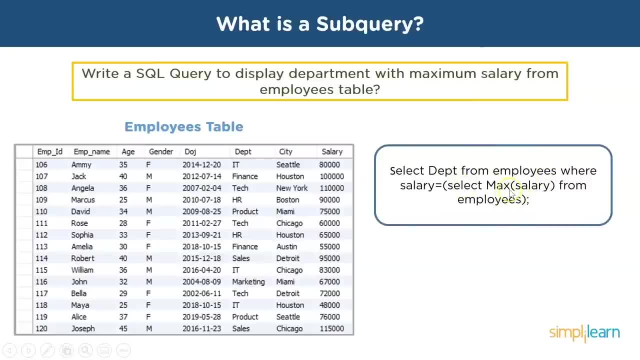 which is select max of salary from employees. so what this max of salary from employees? so what this max of salary from employees? so what this does is it will first return the maximum. does is it will first return the maximum. does is it will first return the maximum salary of the employees in the table. 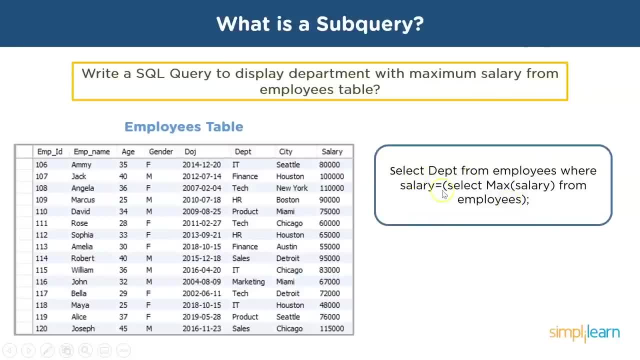 salary of the employees in the table. salary of the employees in the table, then our outer query will get executed. then our outer query will get executed. then our outer query will get executed based on the salary returned from the. based on the salary returned from the. based on the salary returned from the inner query. 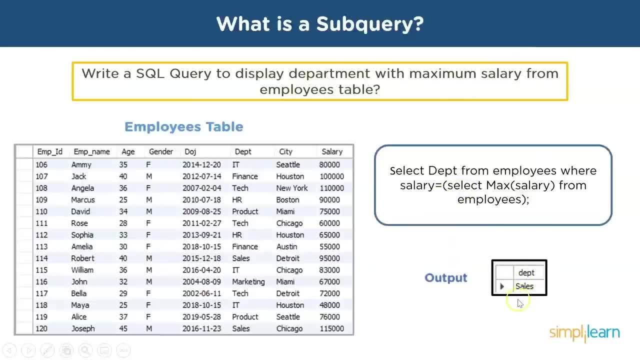 inner query. inner query. so here the output is department sales. so here the output is department sales. so here the output is department sales. has the. has the. has the maximum salary, so one of the employees. maximum salary, so one of the employees. maximum salary, so one of the employees from the sales department earns the. 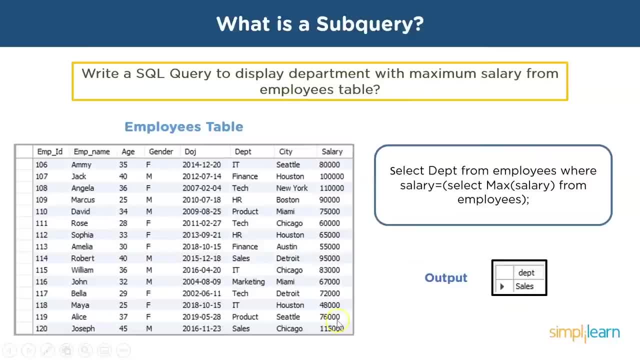 from the sales department earns the from the sales department earns the highest or the maximum salary highest or the maximum salary highest or the maximum salary. if you see in our table the, if you see in our table the, if you see in our table, the employee is joseph, who earns 115 000. 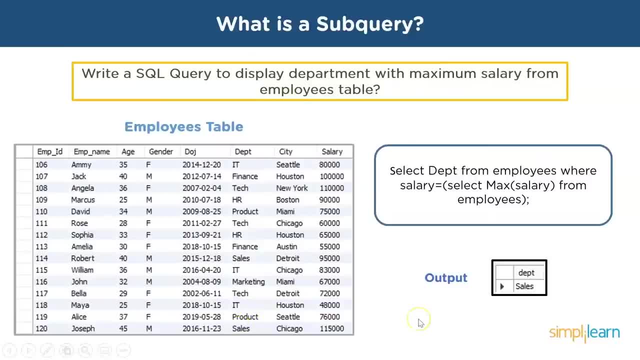 employee is joseph, who earns 115 000. employee is joseph, who earns 115 000. all right, and joseph is from the sales. all right, and joseph is from the sales. all right, and joseph is from the sales department, department department. now let's see how this query works. so now let's see how this query works. so now let's see how this query works. so here we have another question, which is here. we have another question, which is here. we have another question, which is to find the name of the employee with. to find the name of the employee with. 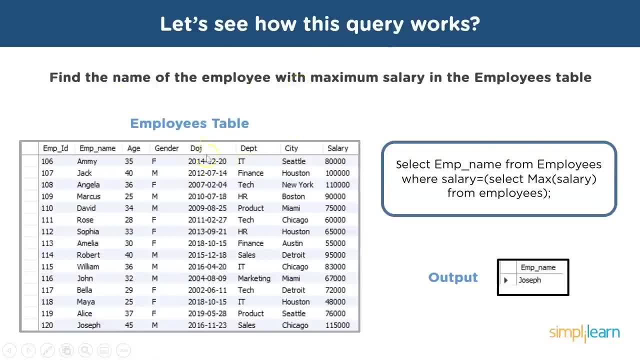 to find the name of the employee with maximum salary in the employees table. maximum salary in the employees table. maximum salary in the employees table. so this is our previous employees table. so this is our previous employees table. so this is our previous employees table that we saw. that we saw. 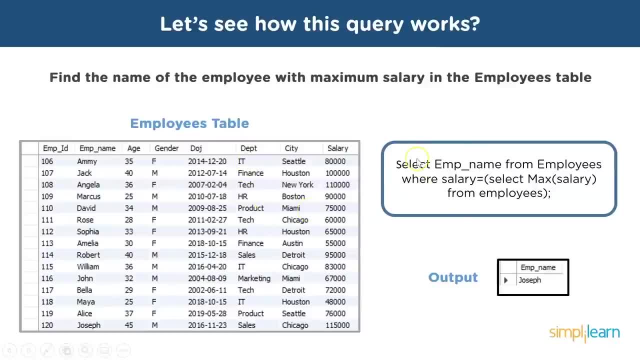 that we saw, and to find the employee who has the, and. to find the employee who has the. and. to find the employee who has the maximum salary. my sub query would look: maximum salary. my sub query would look: maximum salary. my sub query would look something like this: 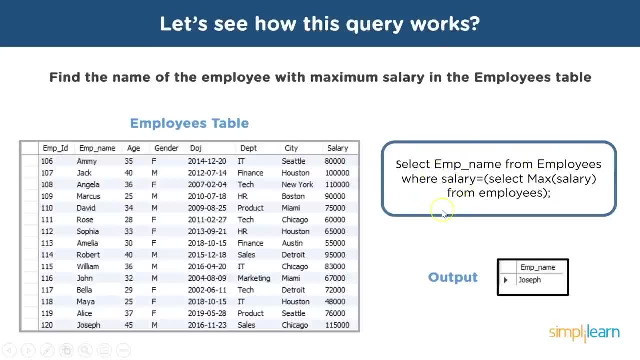 something like this, something like this: so i'm selecting the employee name from. so i'm selecting the employee name from. so i'm selecting the employee name from my table that is employees. my table that is employees. my table that is employees. where i'm using the condition salary. 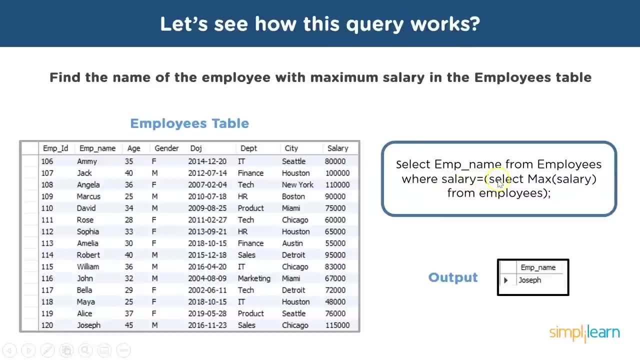 where i'm using the condition salary, where i'm using the condition salary equal to, equal to, equal to, and then i'm passing in my sub query, or, and then i'm passing in my sub query, or, and then i'm passing in my sub query or the inner query. 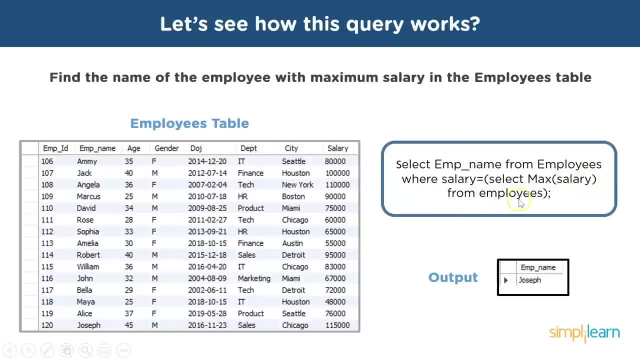 the inner query, the inner query. so first i'm selecting the maximum, so first i'm selecting the maximum, so first i'm selecting the maximum salary. this will return salary. this will return salary. this will return a particular value that is the highest, a particular value that is the highest. 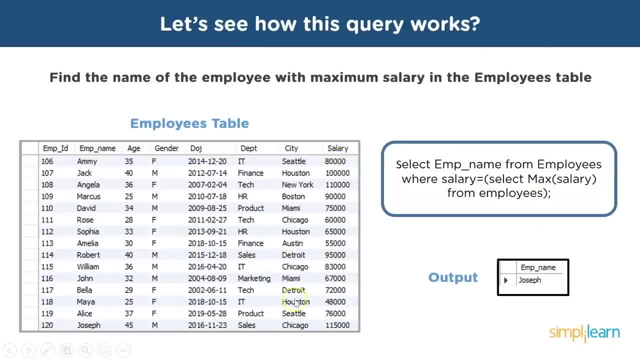 a particular value, that is, the highest salary from the table. salary from the table, salary from the table. and if you see our table, the highest and if you see our table, the highest and if you see our table, the highest salary is 115 000. salary is 115 000. 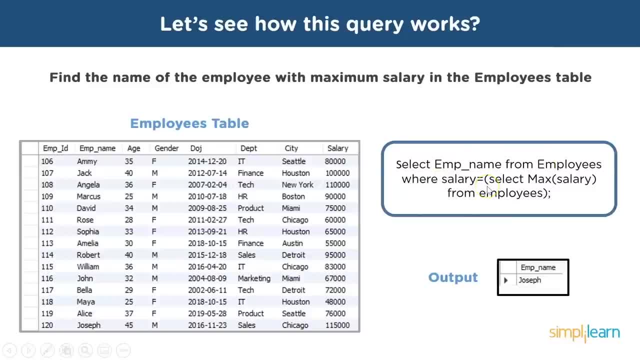 salary is 115 000, so our query becomes select employee name. so our query becomes select employee name. so our query becomes select employee name: from employees where salary equal to 115. from employees where salary equal to 115. from employees where salary equal to 115 000, so the employee name is: 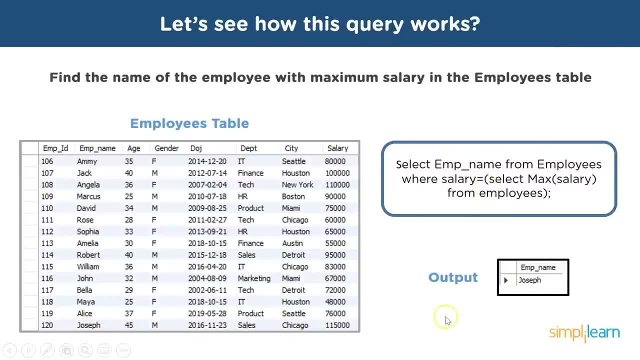 000, so the employee name is 000. so the employee name is joseph here and that's the output. joseph here and that's the output. joseph here and that's the output now. if you want to break it down now, if you want to break it down, 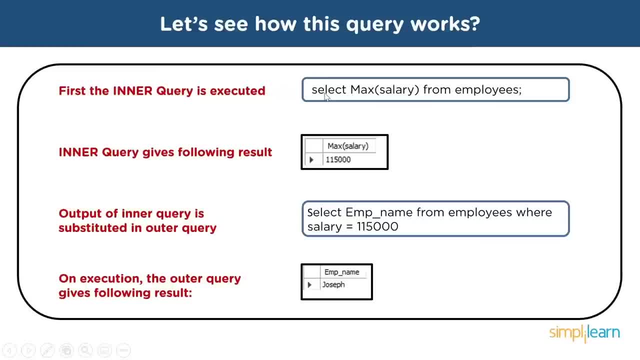 now, if you want to break it down here, you can see first the inner query. here you can see first the inner query. here you can see first the inner query: gets executed, gets executed, gets executed. so our sql query will first execute the. so our sql query will first execute the. 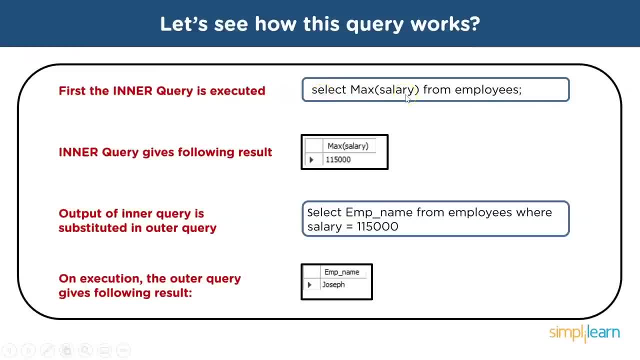 so our sql query will first execute the inner query that is present inside inner query that is present inside inner query that is present inside brackets. select maximum salary from brackets. select maximum salary from brackets. select maximum salary from employees. the result is 115 000 employees. the result is 115 000. 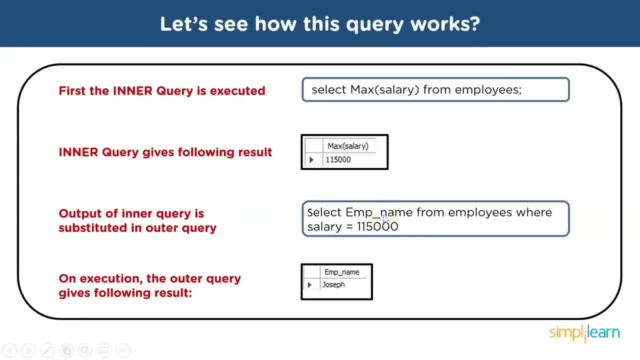 employees. the result is 115 000- and then, based on the return result, our. and then, based on the return result, our. and then, based on the return result, our. outer query gets executed. outer query gets executed. outer query gets executed, so the query becomes select employee name. 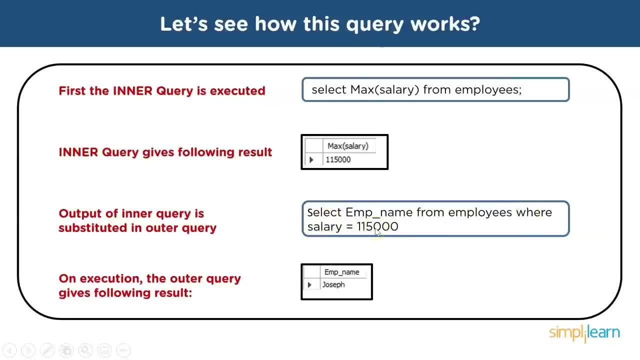 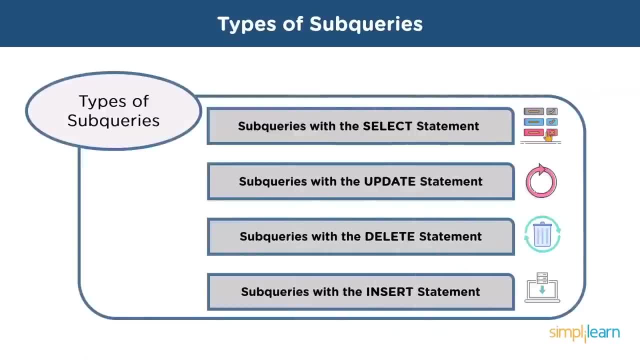 so the query becomes select employee name. so the query becomes select employee name: from employees. where from employees? where from employees, where? so you can write sub queries using. so you can write sub queries using. so you can write sub queries using: select statement- update statement. select statement- update statement. 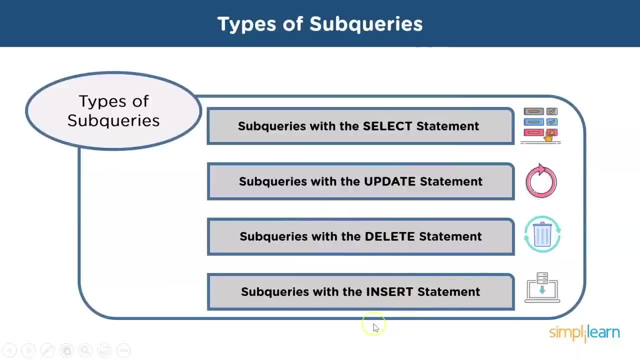 select statement, update statement, delete and insert statement. we'll delete and insert statement. we'll delete and insert statement. we'll explore each of this with the help of explore each of this, with the help of explore each of this with the help of example, on my mysql workbench. 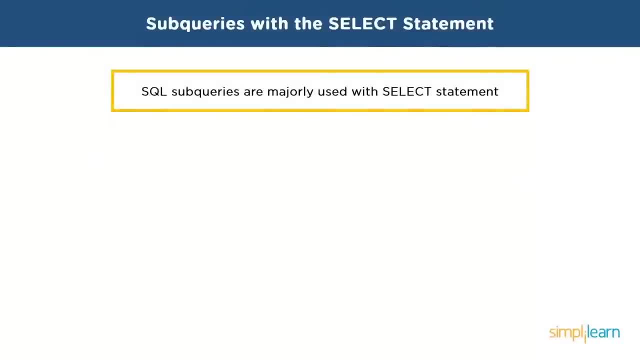 example on my mysql workbench. example on my mysql workbench. so let's learn sub queries with the. so let's learn sub queries with the. so let's learn sub queries with the select statement, select statement, select statement. so sub queries are majorly used with the. 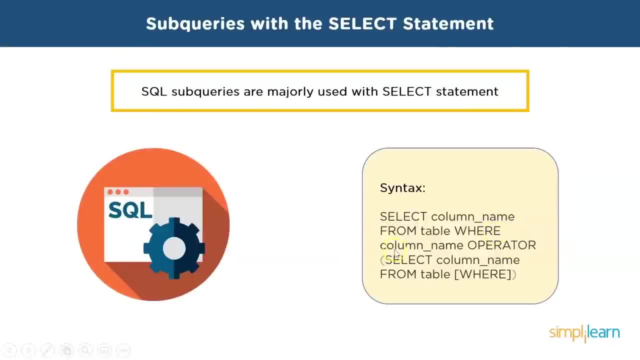 so sub queries are majorly used with the, so sub queries are majorly used with the select statement. and this is how the select statement and this is how the select statement and this is how the syntax looks like you select the column. syntax looks like you select the column. 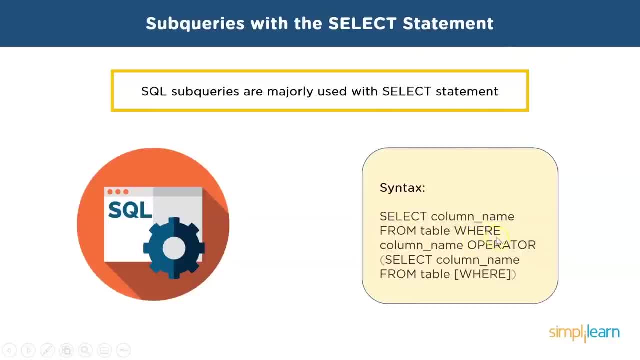 syntax looks like you select the column name from the table name, then you have name from the table name, then you have name from the table name, then you have the, the, the, where condition, followed by the columns. where condition followed by the columns. where condition, followed by the columns that you want to pass the operator. and. 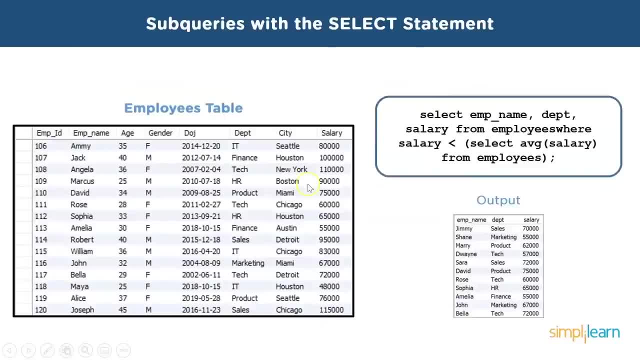 that you want to pass the operator and that you want to pass the operator and inside that, inside that, inside that, you have this sub query. so here is an: you have this sub query. so here is an: you have this sub query. so here is an example that we will perform on our 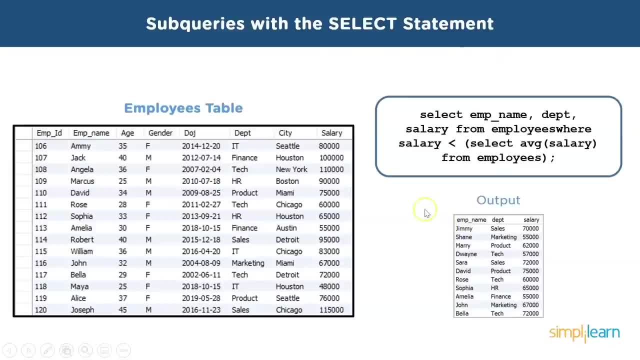 example that we will perform on our example, that we will perform on our mysql workbench. so in this example we mysql workbench. so in this example we mysql workbench. so in this example we want to select all the employees who want to select all the employees who 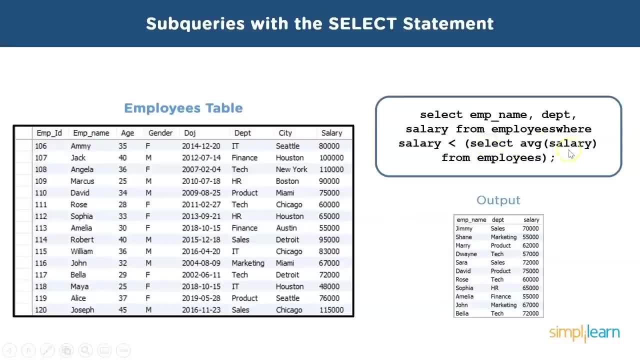 want to select all the employees who have have have a salary less than average salary for a salary, less than average salary for a salary, less than average salary for all the employees, all the employees. this is the output, so let's do this on. this is the output, so let's do this on. 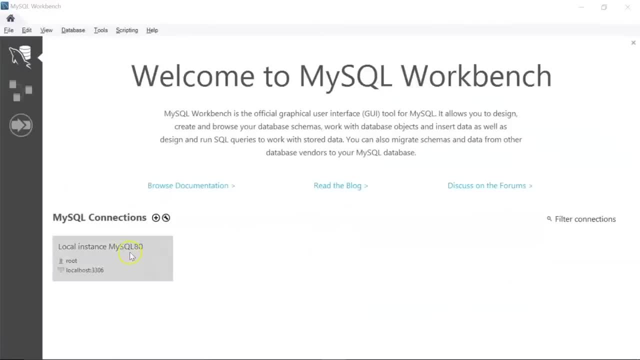 this is the output, so let's do this on my mysql workbench, my mysql workbench, my mysql workbench. all right, so let me log into my local. all right, so let me log into my local. all right, so let me log into my local instance instance. 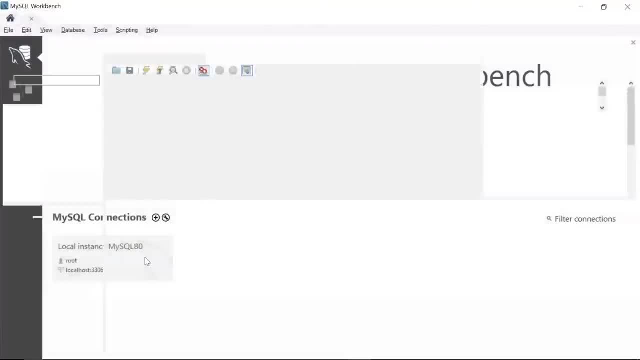 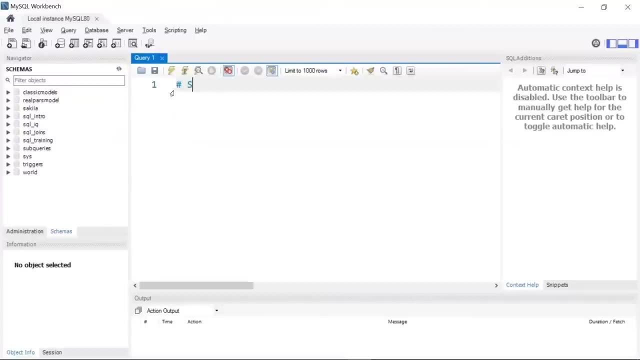 instance, i'll give my password. okay, so you can see i'm on my mysql. okay, so you can see i'm on my mysql. okay, so you can see i'm on my mysql: workbench, workbench, workbench. so let's start by. so let's start by. 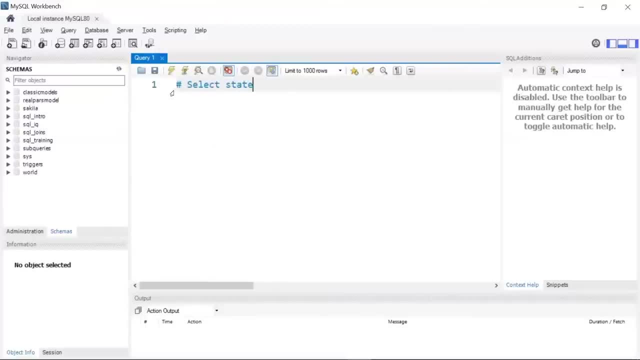 so let's start by writing our subquery using the. writing our subquery using the. writing our subquery using the select statement: select statement, select statement. okay, so for this demo session, we'll be okay. so for this demo session, we'll be okay. so for this demo session, we'll be using a database, that is, sub queries. you. 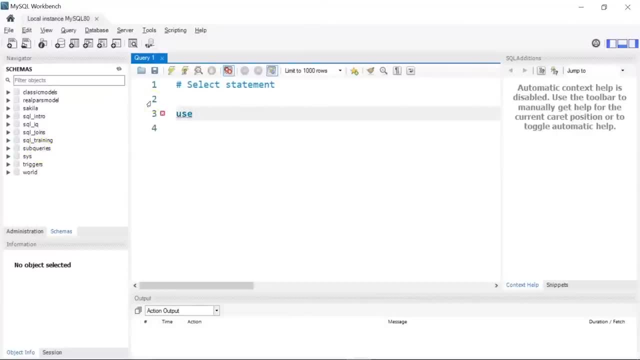 using a database that is sub queries. you using a database that is sub queries. you can see it here. i have a database called: can see it here. i have a database called: can see it here. i have a database called sub queries, sub queries, sub queries. so i'll. 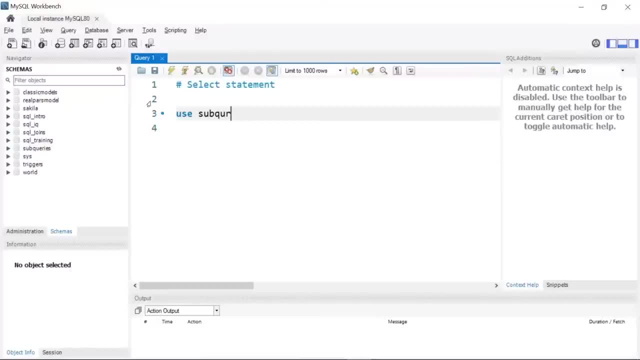 so i'll. so i'll use this, use this, use this sub queries database, sub queries database, and we'll create a few tables as well. okay, if i run it. okay, if i run it. okay, if i run it. now we are inside the sub queries database. now we are inside the sub queries database. 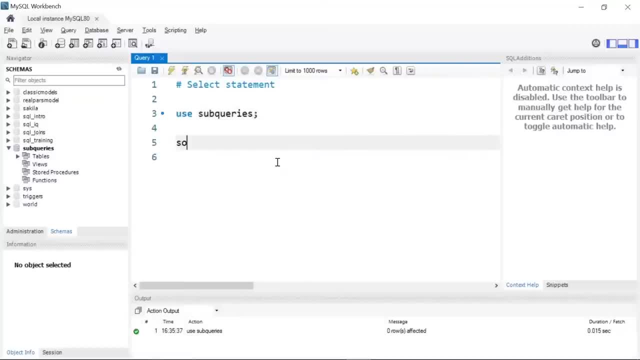 now we are inside the sub queries database, so let me just show you the tables that are. let me just show you the tables that are. let me just show you the tables that are present inside this database. i'll write: present inside this database. i'll write: present inside this database. i'll write: show tables. 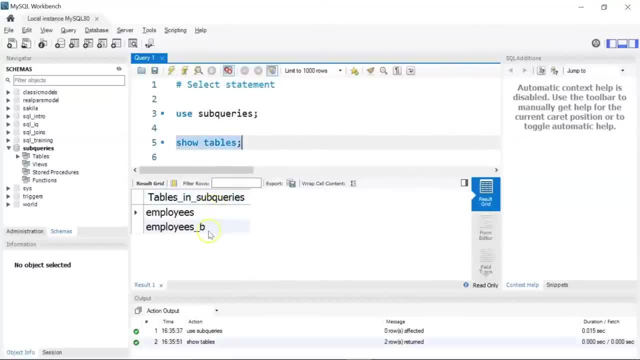 if i run it, if i run it, if i run it, okay, there are two tables employees and okay, there are two tables employees and okay, there are two tables employees and employees underscore b. employees underscore b. employees underscore b. we'll use this table throughout our demo. we'll use this table throughout our demo. 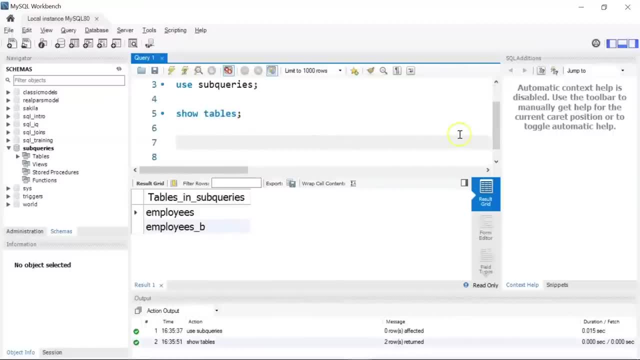 we'll use this table throughout our demo session. session session. all right, all right. all right, now for our select sub query. we want to now for our select sub query. we want to now for our select sub query. we want to fetch the employee name, the department. fetch the employee name, the department. 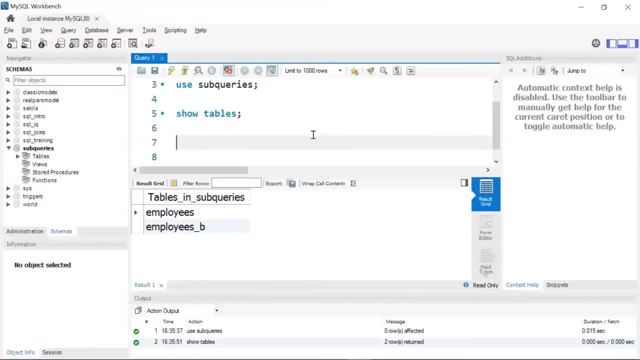 fetch the employee name, the department and the salary and the salary, and the salary whose salary is less than the average, whose salary is less than the average, whose salary is less than the average salary, salary, salary. so we will be using the employees table. so we will be using the employees table. 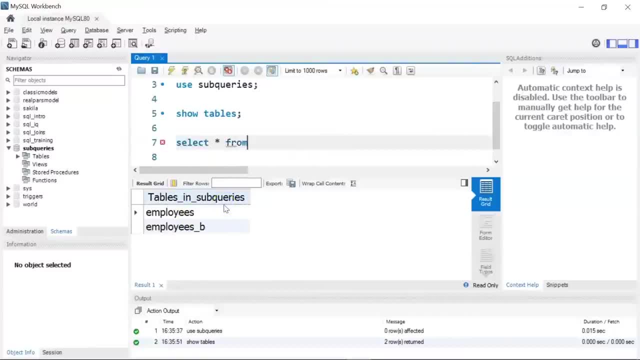 so we will be using the employees table. so let me first show you. so let me first show you, so let me first show you the records and the columns we have in the records and the columns we have in the records and the columns we have in the employees table. 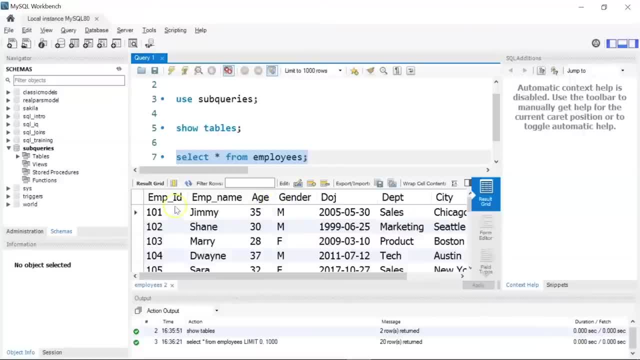 so i'll write select star from. so i'll write select star from. so i'll write select star from employees and run it okay. you can see employees and run it okay. you can see employees and run it okay. you can see, here we have 20 rows of information. 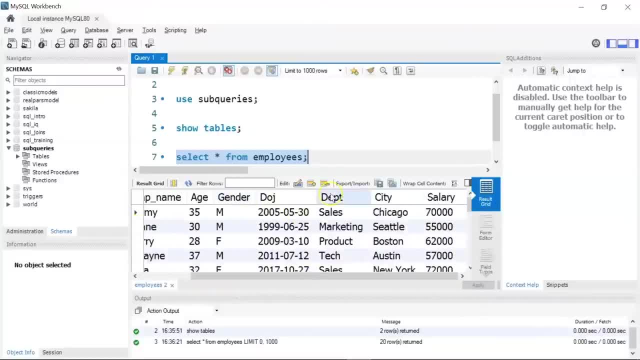 here we have 20 rows of information. here we have 20 rows of information. we have the employee name, the employee id. we have the employee name, the employee id. we have the employee name, the employee id. age, gender- date of join department. age, gender, date of join department. 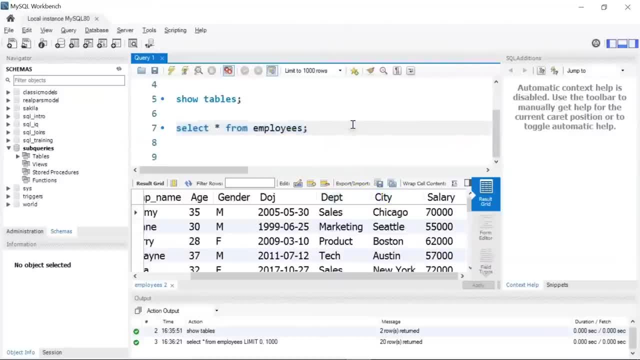 age, gender, date of join department, city and salary. so this is the same city and salary. so this is the same city and salary. so this is the same table that we saw in our slides table that we saw in our slides table that we saw in our slides. okay, 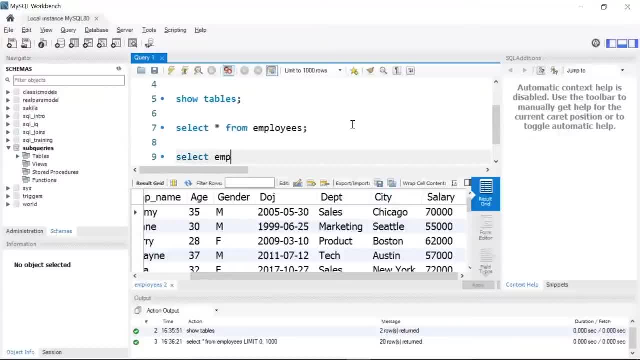 okay, okay, now for our sub query. i'll write select. now for our sub query. i'll write select. now for our sub query, i'll write select. i want to choose the employee name. i want to choose the employee name. i want to choose the employee name, the department and the salary. 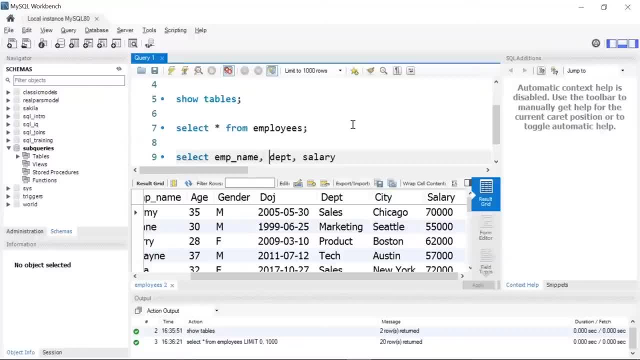 the department and the salary. the department and the salary. there should be a comma here instead of. there should be a comma here instead of. there should be a comma here instead of a period: a period, a period next. i'll give my table name. that is. next. i'll give my table name, that is. 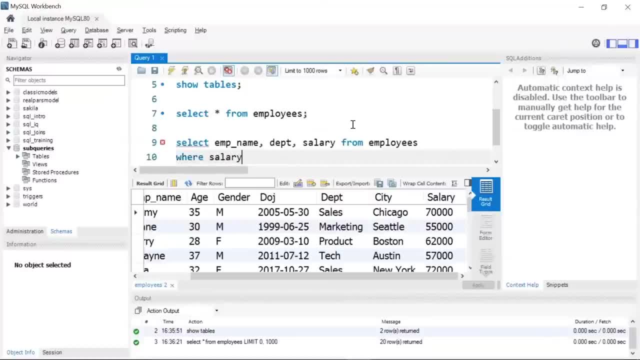 next i'll give my table name, that is, employees where employees where employees where my salary is less than and after this, my salary is less than. and after this, my salary is less than. and after this, i'll start my inner query or the sub. i'll start my inner query or the sub. 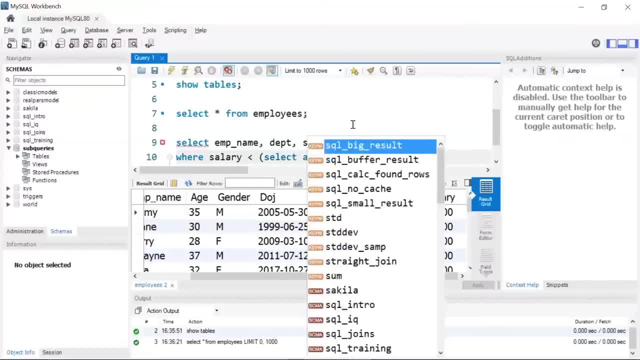 i'll start my inner query or the sub query. i'll write select query. i'll write select query. i'll write select average salary. so i'm using the avg average salary. so i'm using the avg average salary. so i'm using the avg function to find the average salary of. 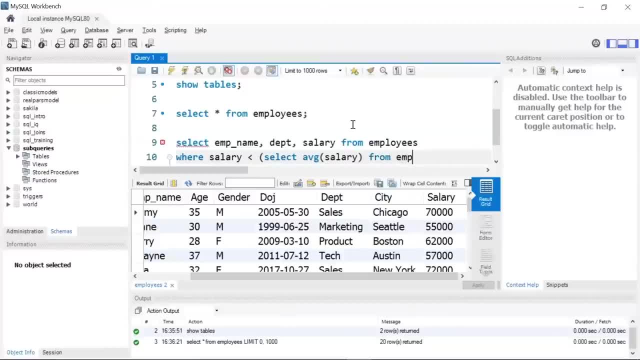 function to find the average salary of function. to find the average salary of all the all, the all the employees from my table. that is employees from my table. that is employees from my table. that is employees. if i give a semicolon, if i give a semicolon. 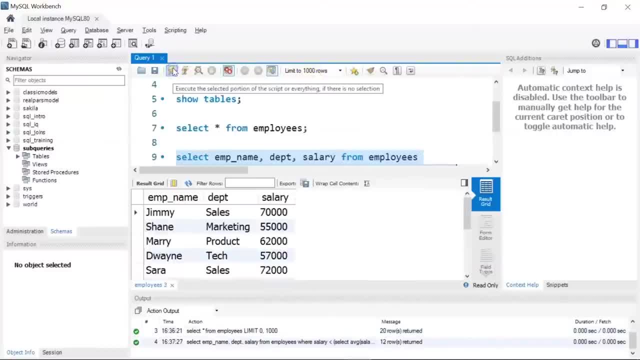 if i give a semicolon and run this and run this and run this, you'll see the output. you'll see the output. you'll see the output. so we have total 12 employees in the. so we have total 12 employees in the. so we have total 12 employees in the table whose salary is less than the. 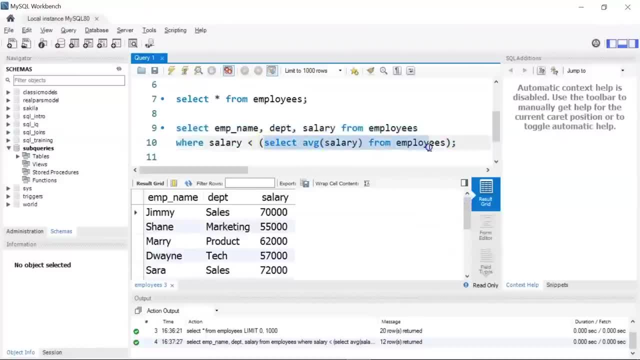 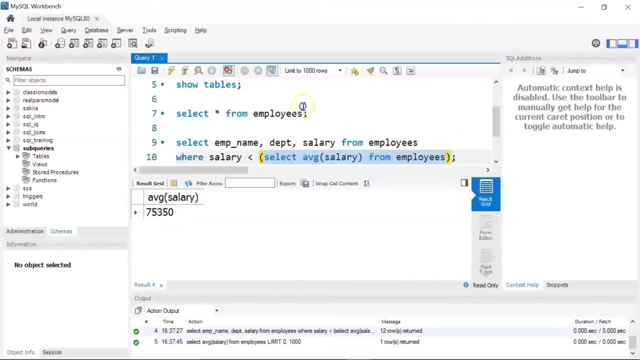 table whose salary is less than the table whose salary is less than the average salary: average salary, average salary. now, if you want, you can check the now. if you want, you can check the now. if you want, you can check the average salary, average salary. average salary: three hundred and fifty dollars. 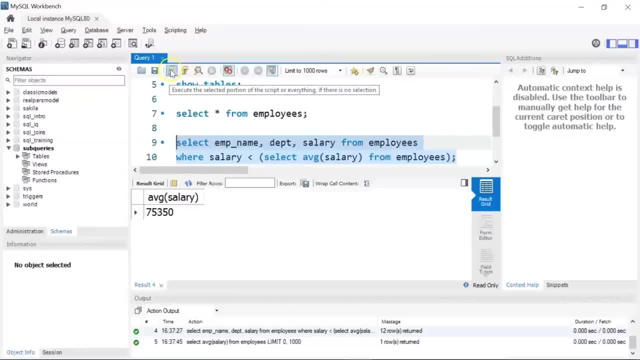 three hundred and fifty dollars. three hundred and fifty dollars. now the employees who have a salary less. now the employees who have a salary less. now the employees who have a salary less than the average salary, than the average salary, than the average salary. so these are the people. 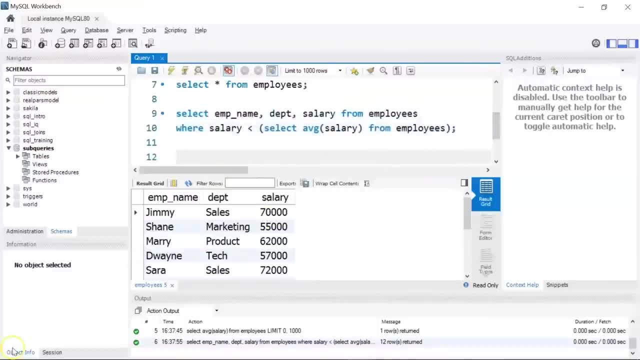 all, right now moving back to our slides. all right now moving back to our slides. all right now moving back to our slides. okay, okay, okay. now let's see how you can use sub queries. now let's see how you can use sub queries. now let's see how you can use sub queries with the insert statement. 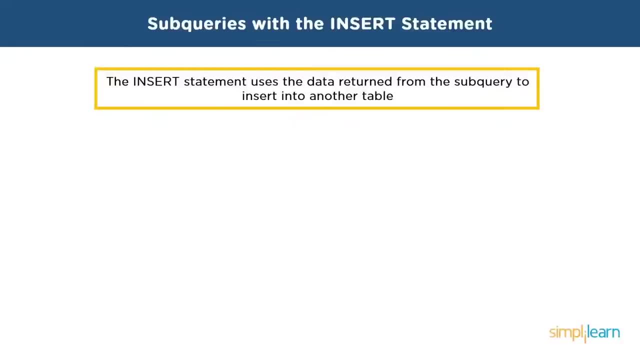 with the insert statement. with the insert statement. now the insert statement uses the data. now the insert statement uses the data. now the insert statement uses the data written from the sub query to insert. written from the sub query to insert. written from the sub query to insert into another table. 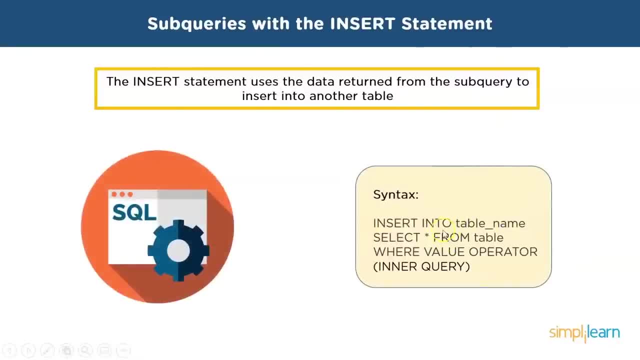 into another table, into another table. so this is how the syntax looks like. so, so this is how the syntax looks like. so so this is how the syntax looks like. so you write insert into table name, you write insert into table name, you write insert into table name, followed by select individual column. so 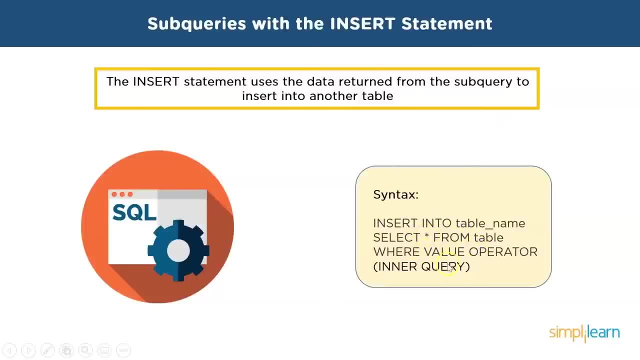 followed by select individual column. so followed by select individual column. so start from start, from start from the table use the where clause, and then the table use the where clause, and then the table use the where clause, and then you give the operator, followed by the. you give the operator, followed by the. 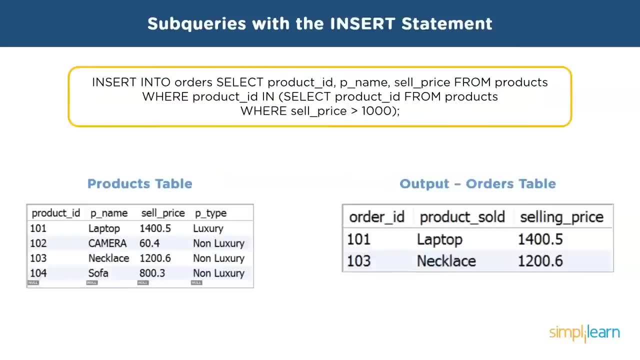 you give the operator, followed by the inner query or the sub query, inner query or the sub query, inner query or the sub query. so here we will explore a table called so here we will explore a table called so here we will explore a table called products table. 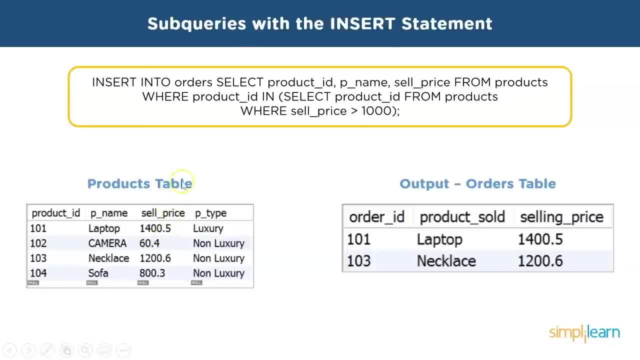 products table. products table. we are going to fetch few records from. we are going to fetch few records from. we are going to fetch few records from. the products table based on a condition. the products table based on a condition. the products table based on a condition, that is: 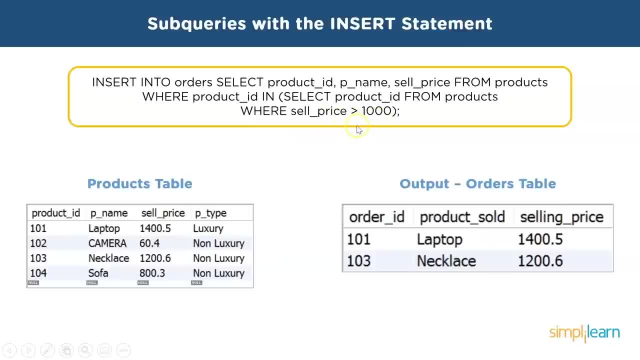 that is, that is the selling price of the product. should the selling price of the product, should the selling price of the product should be greater than be greater, than be greater than hundred dollars. so only those records hundred dollars, so only those records hundred dollars. so only those records will fetch and put it in our orders. 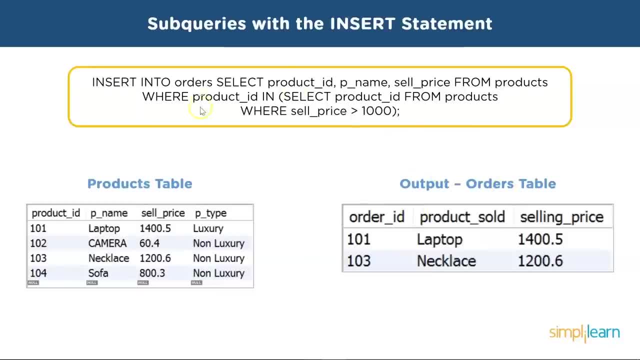 will fetch and put it in our orders. will fetch and put it in our orders. table, table, table. all right, so we are going to write this. all right, so we are going to write this. all right, so we are going to write this query on my, my sql workbench. so let's. 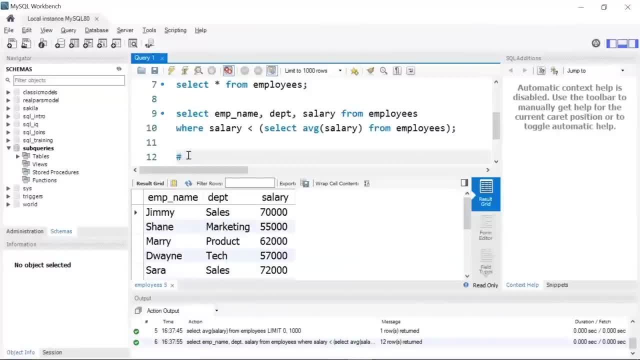 query on my, my sql workbench. so let's query on my- my sql workbench. so let's do it, do it, do it. i'll give my comment, as i'll give my comment, as i'll give my comment as: update sub query. update sub query. update sub query. all right, 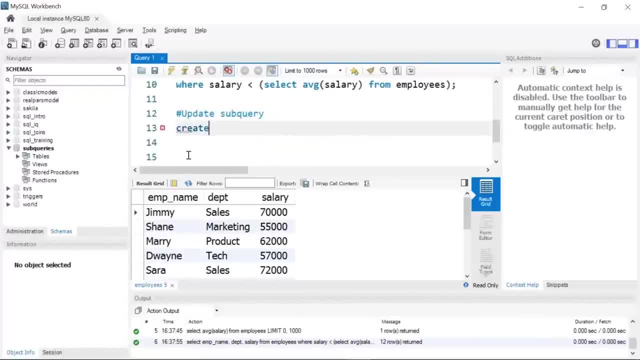 all right, all right. so first of all, let's create our table. so, first of all, let's create our table. so, first of all, let's create our table. that is, that is, that is, products. so i'll write: create table products. so i'll write: create table. 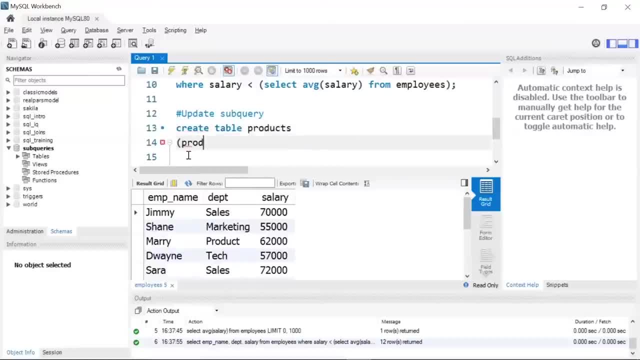 products. so i'll write: create table products- products- products. then we'll give our column names: the. then we'll give our column names: the. then we'll give our column names. the first column would be the product id of first column would be the product id of first column would be the product id of type. 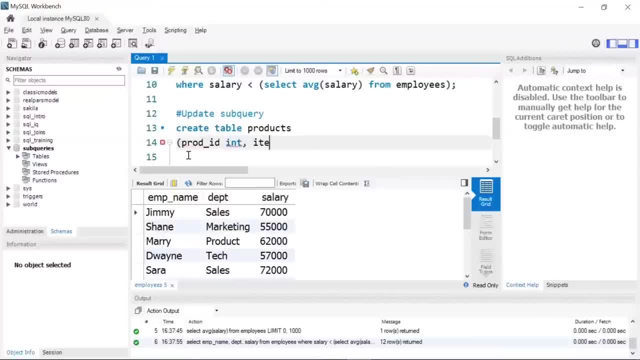 type: type integer. then we have the column as integer, then we have the column as integer, then we have the column as item, or the item or the item or the product which is of type. product which is of type product which is of type varchar 30. varchar 30. 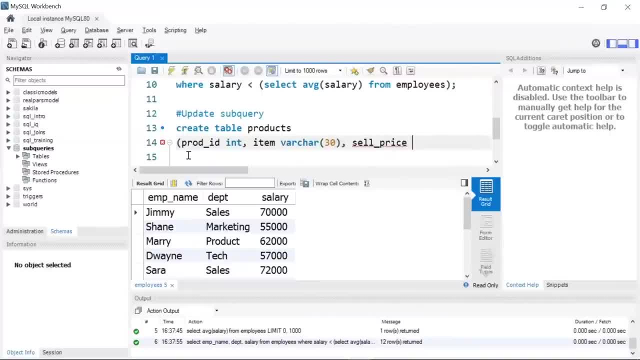 varchar 30. next we have the next, we have the next, we have the selling price of that product. the selling price of that product, the selling price of that product, the selling price will be of type float, selling price will be of type float, selling price will be of type float. and finally, we have another. 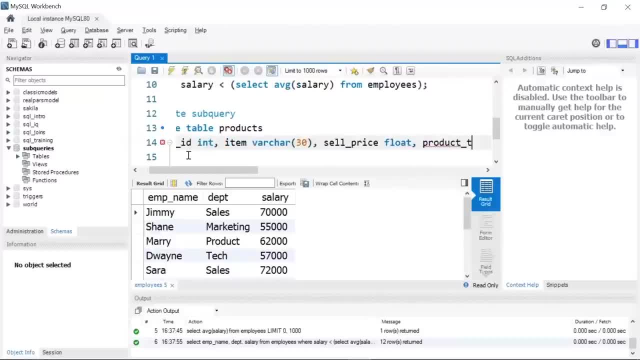 and finally we have another, and finally we have another column, which is called the product type. and again product type is of, and again product type is of, and again product type is of. the data type: varchar. i'll give the size. the data type: varchar. i'll give the size. 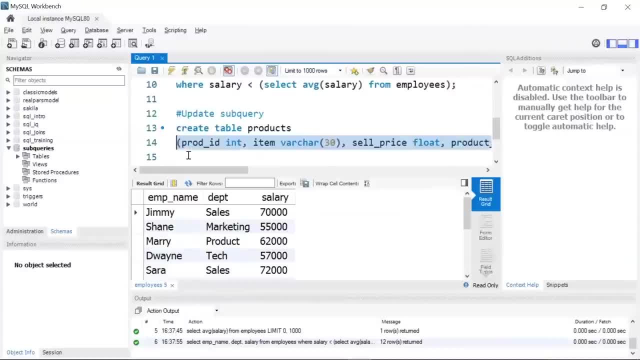 the data type varchar. i'll give the size as 30, as 30, as 30. close the bracket and give a semicolon. close the bracket and give a semicolon. close the bracket and give a semicolon. now, let's just now. let's just now, let's just run it. 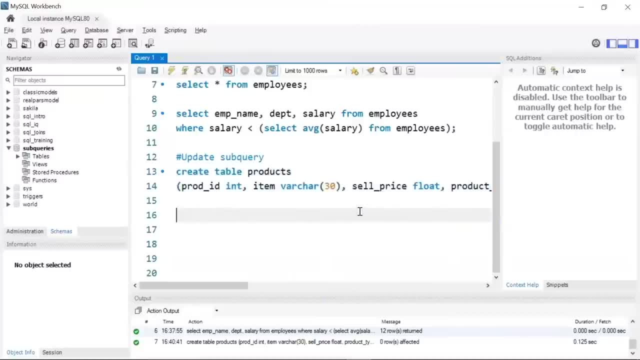 run it. run it okay. so we have successfully created our okay. so we have successfully created our okay. so we have successfully created our products: table products- table products- table. now. let's insert a few records to our now. let's insert a few records to our now. let's insert a few records to our products: table. 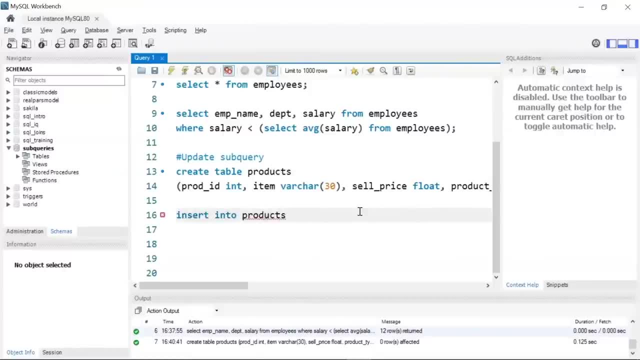 products table: products table. so i'll write insert into. so i'll write insert into. so i'll write insert into products: products, products, followed by values. i'll give, i'll give. i'll give four records. the first product id is 101. four records: the first product id is 101. 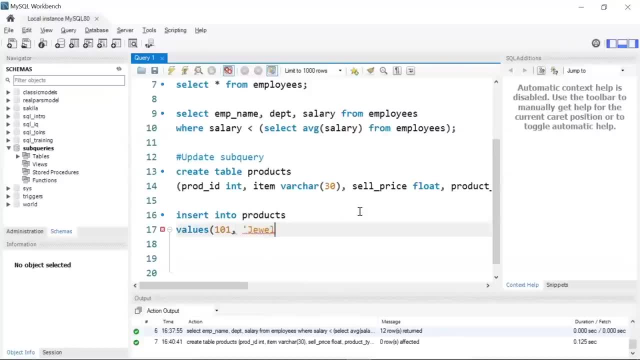 four records. the first product id is 101. the product is: the product is. the product is, let's say jewelry, let's say jewelry, let's say jewelry, then the selling price is, let's say $800, and the product type is: it's a luxury product. next, let's insert one more product detail. the product ID is 102, the product: 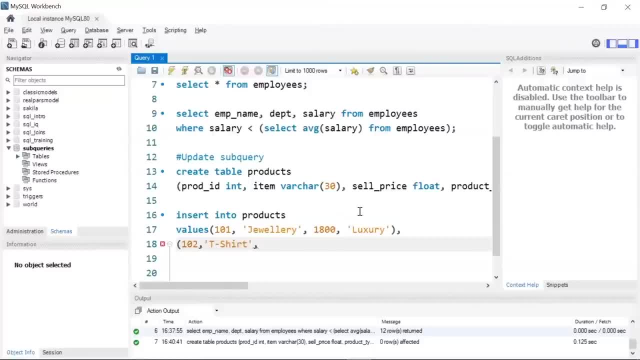 is, let's say, t-shirt, the price is, let's say, $100 and the product type is non-luxury. next, I'll just copy this to reduce our task. we'll edit this. the third products ID is 103. the product is laptop and let's say the price is $1,300 and it's a luxury product. I'll paste: 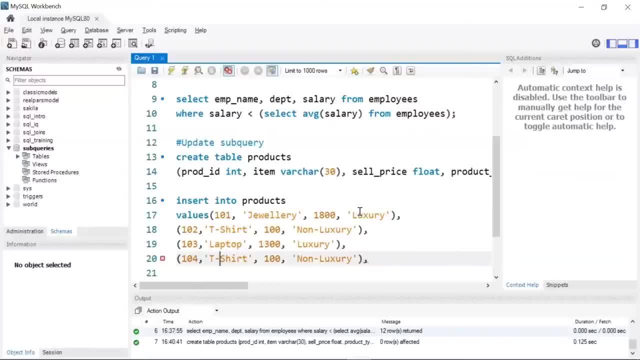 again and finally, I'll enter my fourth product which is, let's say, table, and the price is $400 and it's a non-luxury product. I'll give a semicolon and we'll insert these four records to our products table. you can see we have inserted. 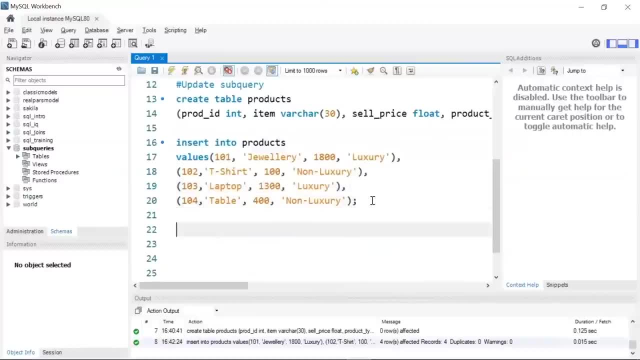 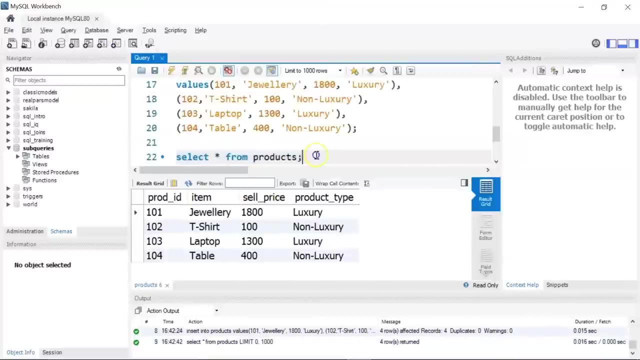 four records. let's just print it now so I'll write select star from products. if I run it you can see we have our four products ready. now we need to create another table where we are going to put some records from our products table, so that new table is going to. 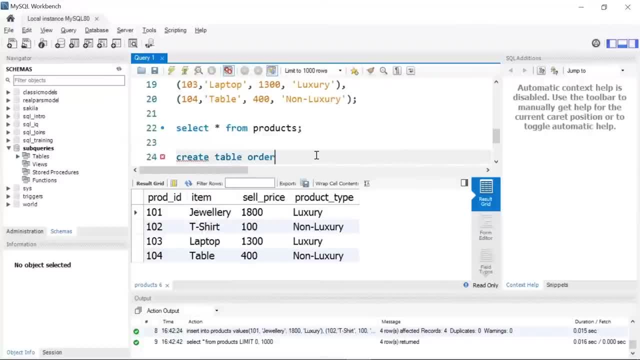 be the orders table, so I'll write create table orders. now it will have three columns: the order ID. order ID will be of type integer. then we have product underscore sold. this will be of type varying character, of size 30 and finally we have the selling price. 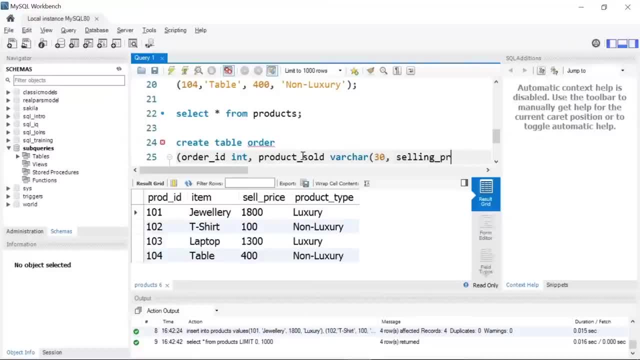 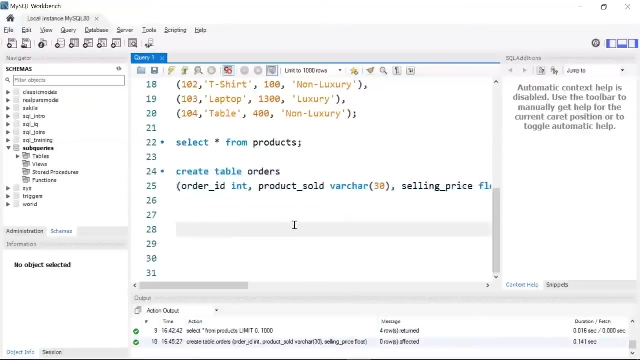 column. this will be of type float. let's create our orders table. the table name should be orders and there is some mistake here. okay, should close the brackets. okay, let me run it. so we have our orders table ready. now let's write our insert sub query. so I am going to insert into my table. that is orders, and 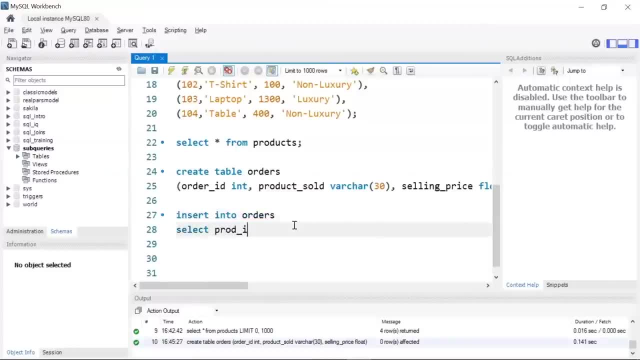 I'll select the product ID comma, the item and the selling price or the sell price from my table, that is, products. where I'll write product ID in, I'll write my inner query: select prod ID or the product ID from products. next I will give a where clause where the selling price is greater than $1,000. 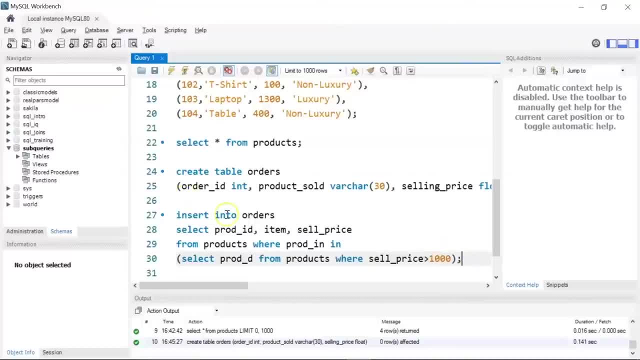 so let me tell you what I am going to do here. I am going to insert into my orders table the product ID, the item name and the selling price from my products table where the product ID has this condition. so let me first run this condition for you, which is: select prod ID from: 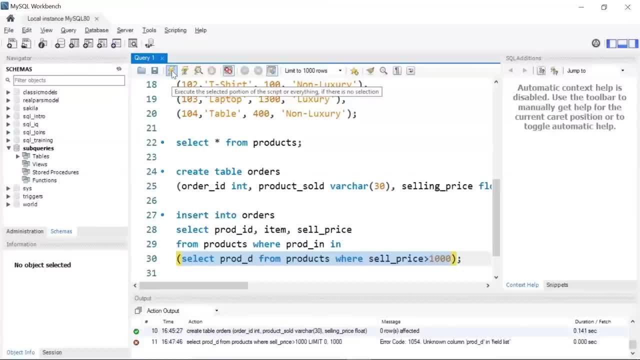 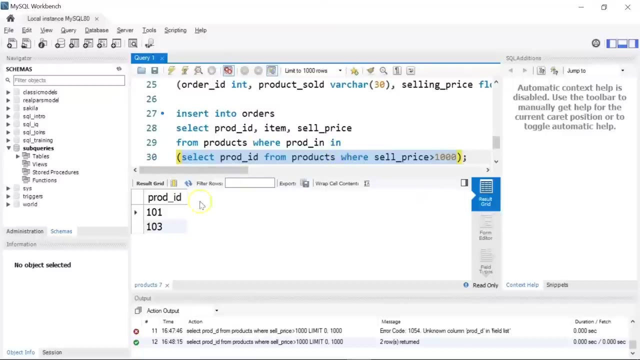 products where the selling price is greater than 1000. if i run this, okay, there is some issue here. the column name is actually prod id. now let's run it again so that we can see the product ids of the products which have a selling price greater than 1000. so it is 101 and 103. now let's run the entire. 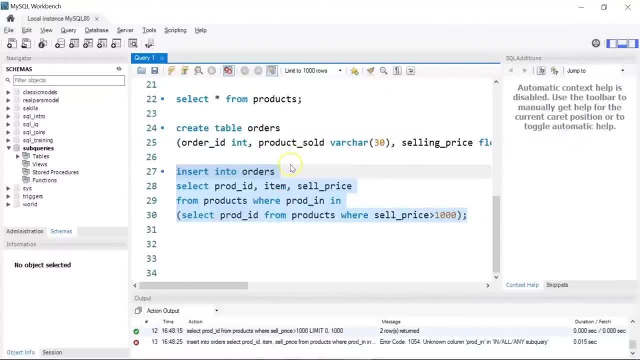 query. there is another mistake here. let's debug the mistake now. this should be product id instead of product underscore in. let's insert again. all right, so we have successfully inserted two records to our table, that is orders. now let's see the orders table. i'll write select star from orders. 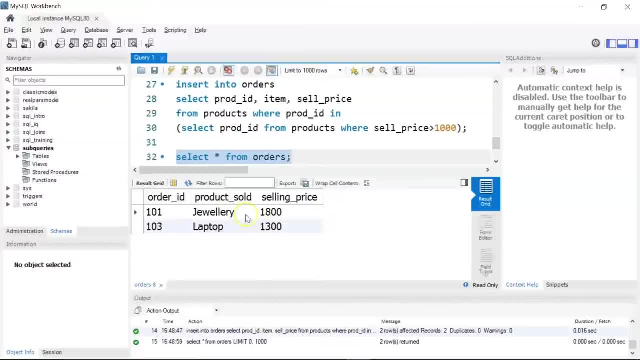 if i run it, there you go. so there were two products from our product table that were jewelry and laptop, which have a selling price greater than one thousand dollars. so the selling price for jewelry was eighteen hundred dollars and for laptop it was thirteen hundred dollars. so this is how you can use a sub query using the insert statement. all right, now going. 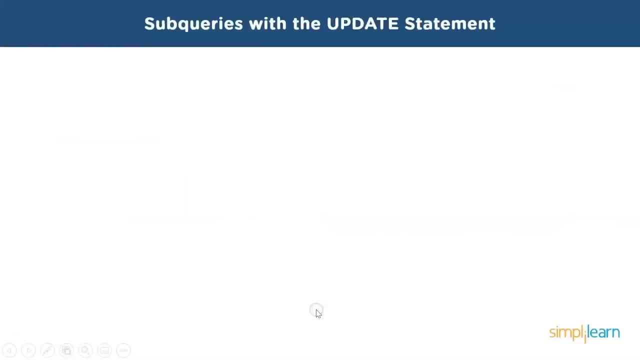 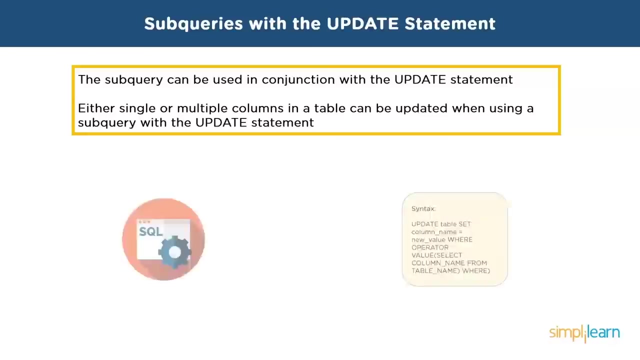 back to our slides again. all right, now let's see how you can use sub queries with the update statement. now the sub queries can be used in conjunction with the update statement, so either single or multiple columns in a table can be updated when using a sub query with the update. 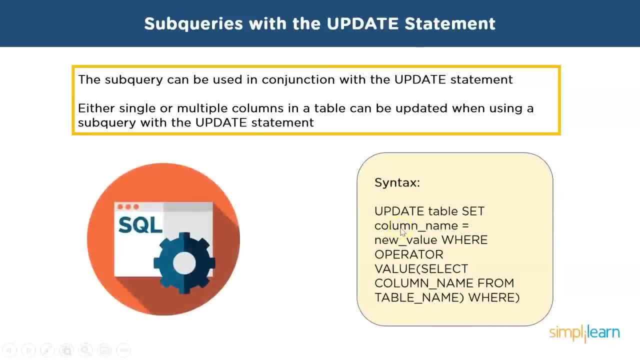 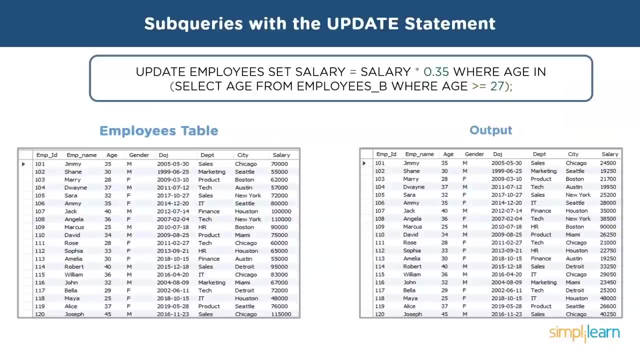 statement. so this is how the basic syntax of an update sub query looks like. so you write update table, followed by the table name, you set the column name, you give the where operator and then you write your inner sub query. so we are going to see an example. 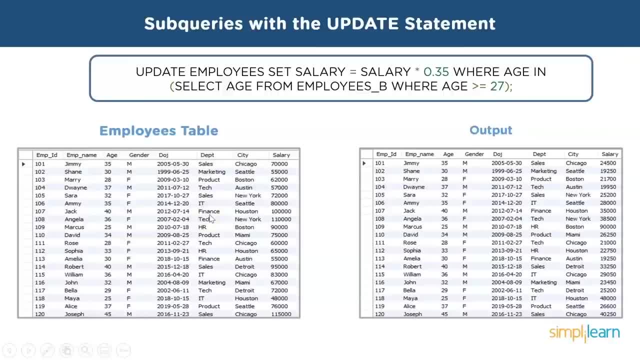 where we will use this employees table. and using this employees table, we will update the records of the salaries of the employees by multiplying it with a factor of 0.35, only for those employees which have age greater than 27. so we are going to use a new table called 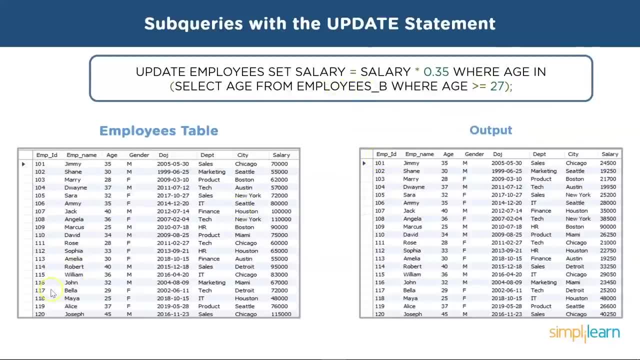 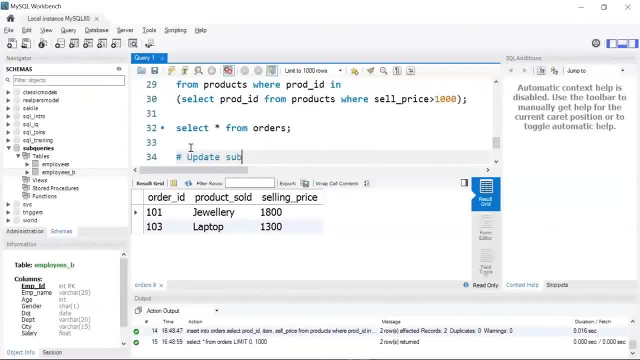 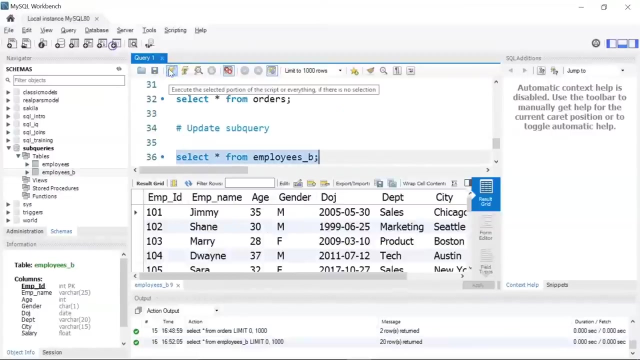 employees underscore b for this as well. so let's see how to do it. so i'll give my comment as update sub query. before we see the sub query, let's see what we have in the table: employees underscore b. this is basically a replica of the employees table. there you go. it has the 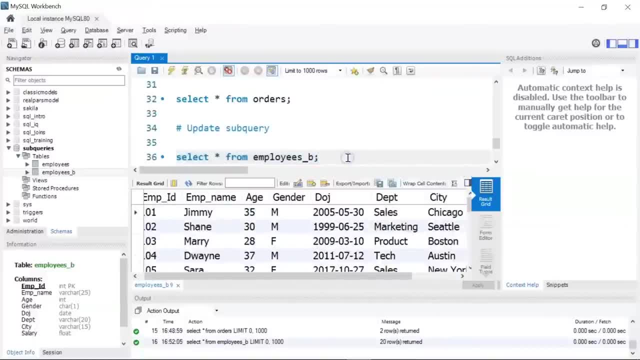 same records that our employees table has. we are going to use both the employees table and the employees underscore b table to update our records. so i'll write: update employees. set salary equal to. let me bring this to the next line. i'll write: set salary equal to salary multiplied by 0.35, where: 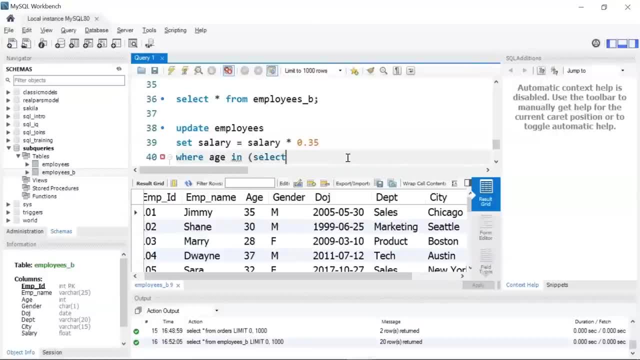 age in. then i'll write select age from my other table, that is, employees, underscore b, where age is greater than equal to, let's say, 27. all right, so let me run through this query and tell you what we are going to do. so i'm going to update the records of the employees table. 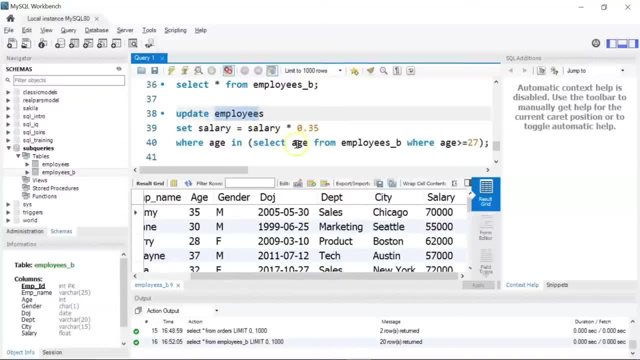 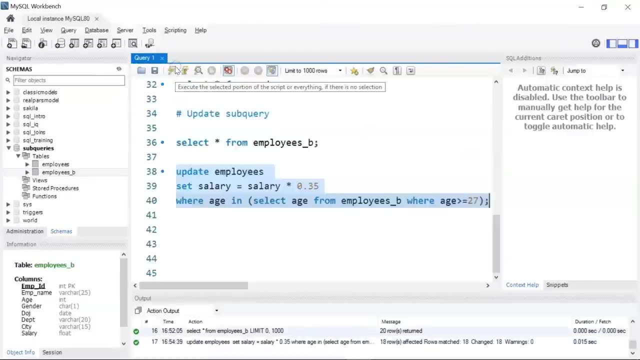 specifically for the salary column. so i'm checking: if the age is greater than 27, then we'll multiply the salaries of the employees with a factor of 0.35 in the employees table. let me just run this, then we'll see our output. okay, so it says 18 rows affected, which means there are total 18 employees in the table. 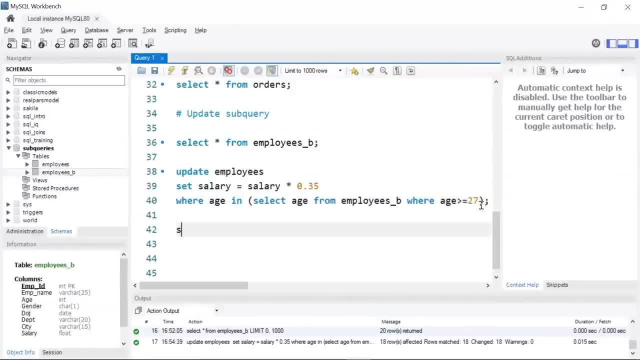 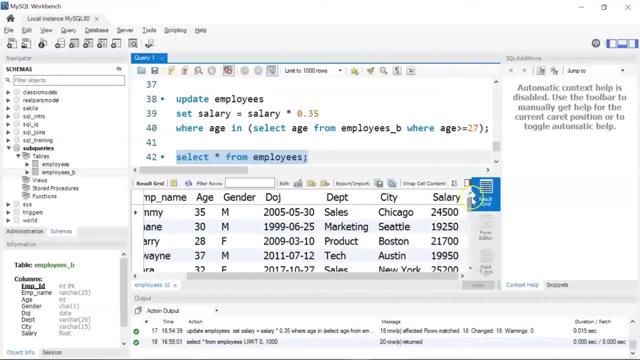 out of the 20 employees whose age is greater than 27.. now, if you see i'll write select star from employees, you can see the difference in the salaries. if i scroll to the right, you can see these are the updated salaries. okay, so if you check for employees who have an age less than or equal to 27- for example marcus, whose age is 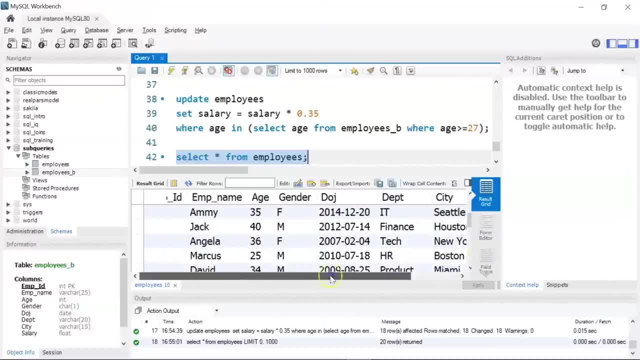 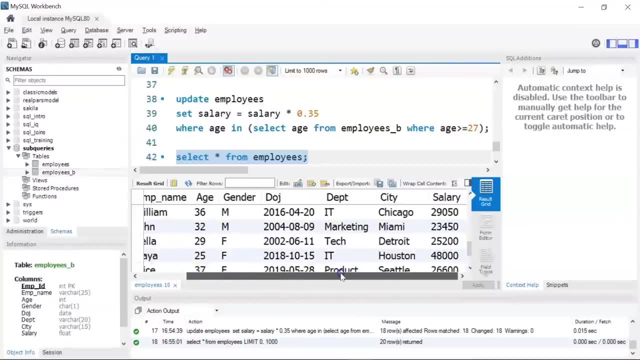 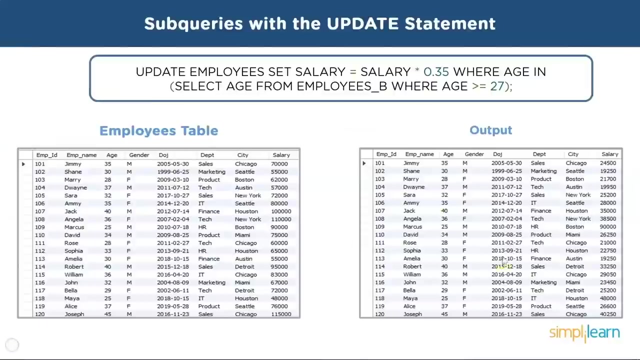 25. his salary is the same. we haven't updated his salary, then, if you see, if you have, okay, there is one more employee, maya. we haven't updated the salary of maya because the age is less than 27. all right, now let's go back to our slides again. as you can see, we got the same output on our mysql workbench. 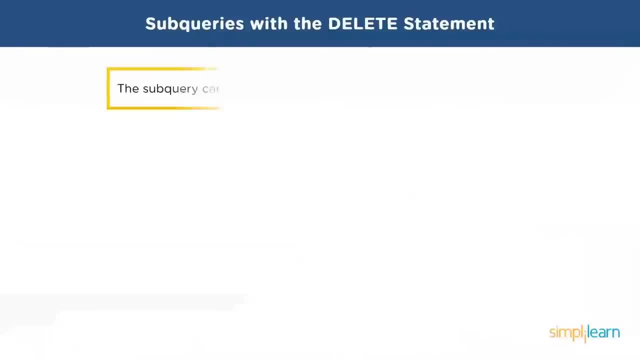 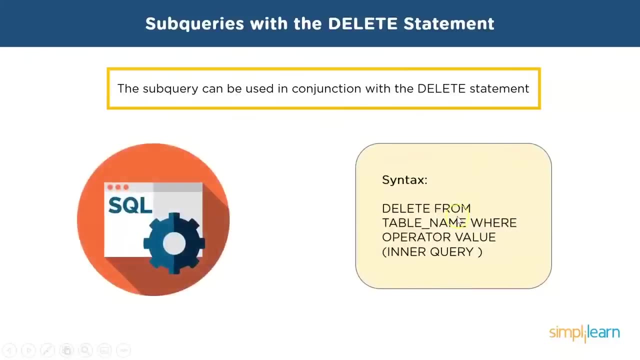 now let's explore how you can write sub queries for that delete statement. now sub queries can again be used in conjunction with the delete statement. so this is how the basic syntax of a delete query using sub query would look like. you write delete from the table name where clause the operator value, followed by the inner query within. 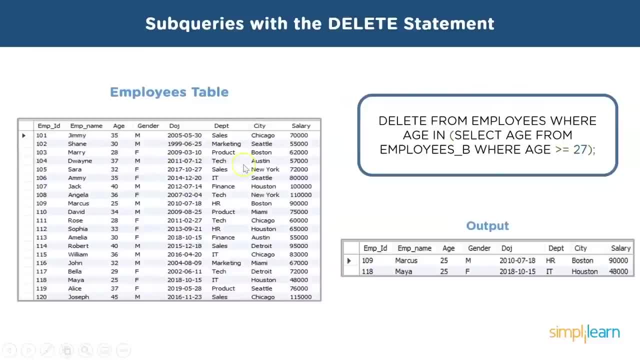 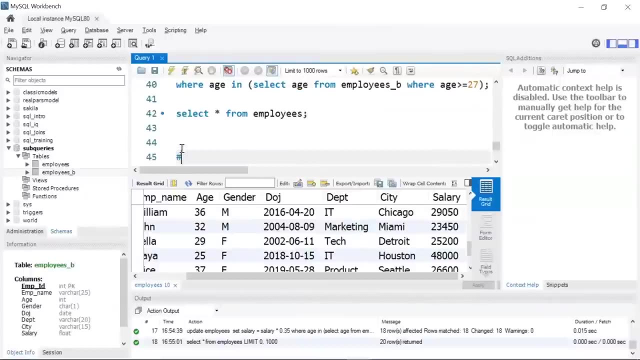 brackets. so here we are going to use the employees table and what we are going to do is we'll delete the employees whose age is greater than equal to 27. so let's see how you can do it. all right, so i'll give my comment as delete subquery. 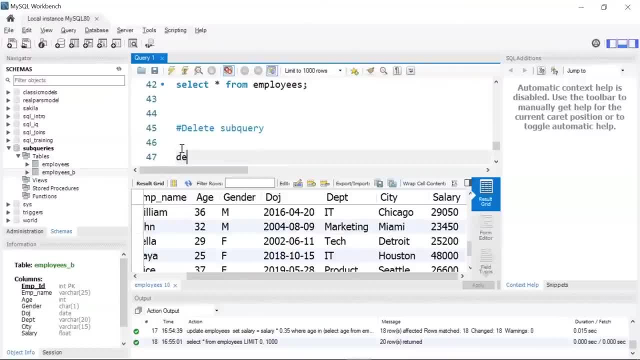 so we'll follow the syntax that we saw. i'll write delete from my table name. that is employees. i'll write where age in and then i'll start my inner query or the subquery. i'll write select age from employees underscore b where, and then i'll write delete from my table name. that is employees. 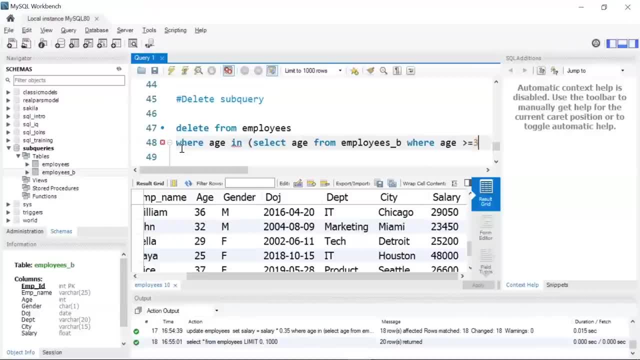 age is, let's say, greater than equal to 32, or let's say the age is less than equal to 32. close the bracket and i'll give my semicolon. let me first run the inner query for you so that you get an idea of the employees who are less than 32 years of age. so there are nine employees. 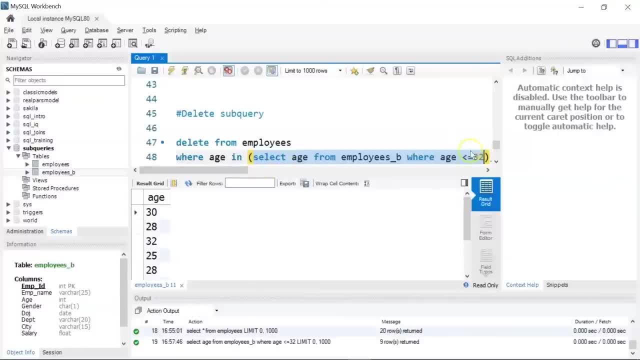 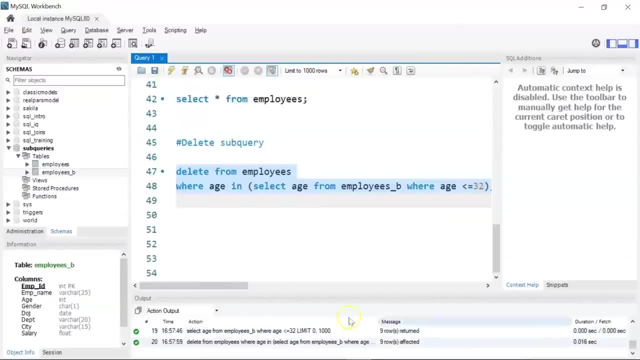 in the table who have an age less than equal to 32. so we are going to delete the records. so we are going to delete the records and we are going to delete the records. if i run this, okay, it says nine records deleted. now let's print or display what we have in the employees table. 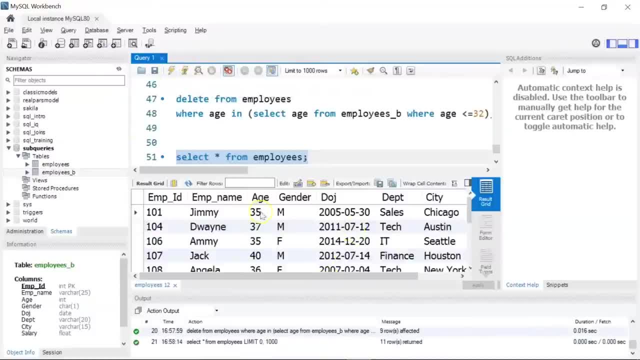 if i run this, there you go. so if you see the age table, we have total 11 employees now and all their ages are greater than 32 because we have deleted the records. so we are going to delete the records, all those employees who had an age less than equal to 32. okay, so let me show you from the beginning. 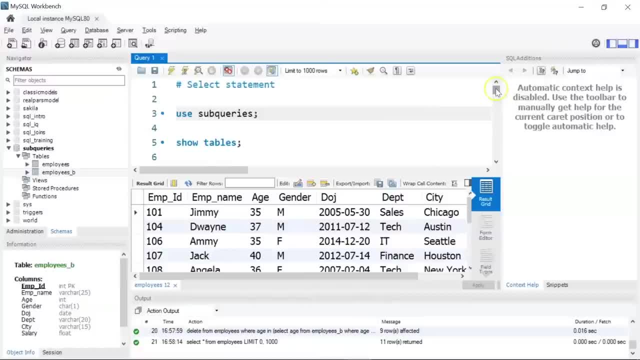 what we did. so first we used our sub queries database, then we used our employees table. so we started by looking at how you can use the sub query with a select statement. this should be insert instead of update. so we learned how to write an insert sub query. we used two tables: products and our orders table. 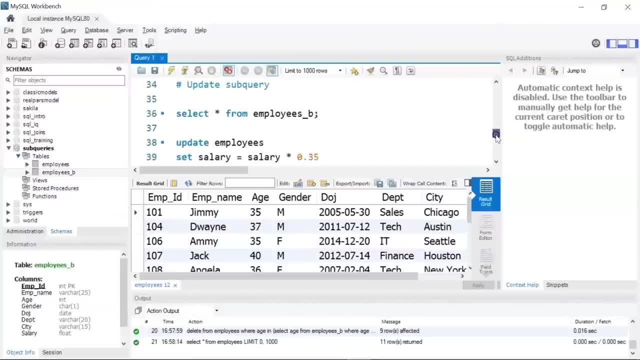 moving ahead, we saw how to write sub queries using the update command, so we updated the salaries of the employee by a factor of 0.35 for those who had an age greater than equal to 27. and finally, we saw how to use the sub query using the delete statement, so we deleted all those records for the employees whose age was less. 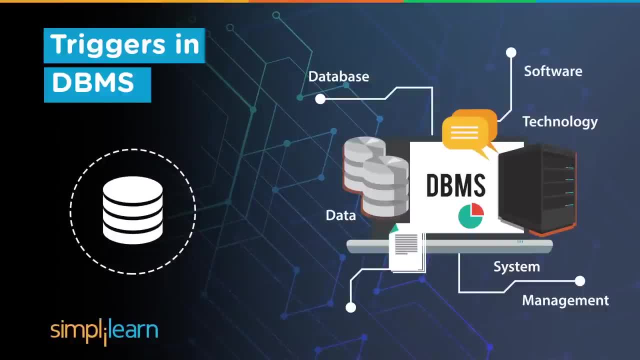 then equal to 32.. In this video, we will discuss an advanced SQL concept called triggers. We will learn what triggers are and how they can be used to solve problems. We'll look at how trigger queries are written on MySQL Workbench. So let's get started First. 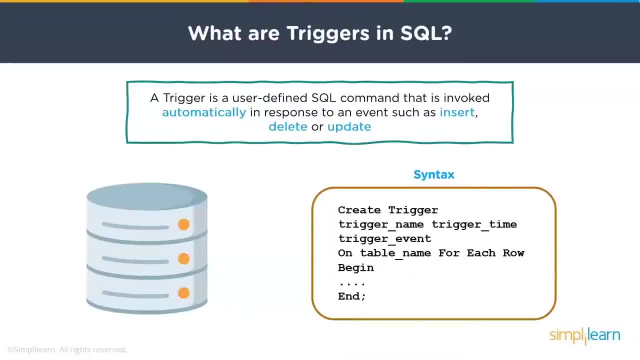 what are triggers in SQL. So a trigger is a user-defined SQL command that is invoked automatically when an event occurs. An event can be related to inserting, updating or deleting records in a table. In MySQL, triggers can be executed automatically by the oracle server. 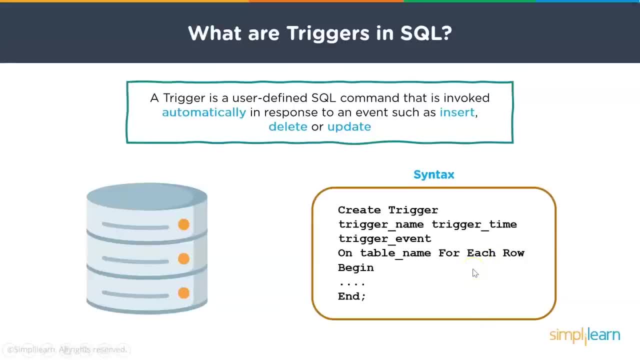 Below is how the syntax of writing a trigger is. So you write create trigger, followed by the trigger name. Now the trigger name should be a valid SQL name. Then we have the trigger time, the trigger event and then on the name of the table. Then we write for each row: begin. 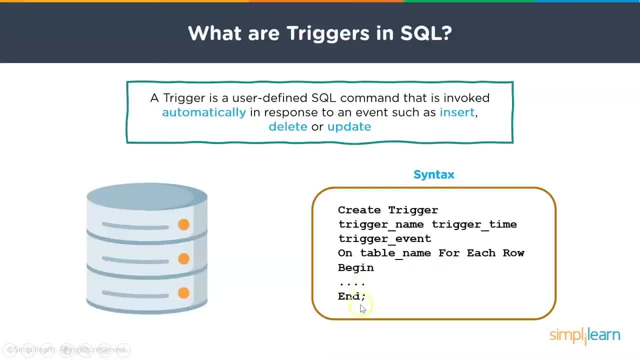 followed by the name of the table. Then we write, for each row, begin, followed by the name of the table, The list of SQL statements and finally we write end. Now, in the syntax, the trigger time represents either before or after an event, and a trigger event can be an insert, update or delete operation. 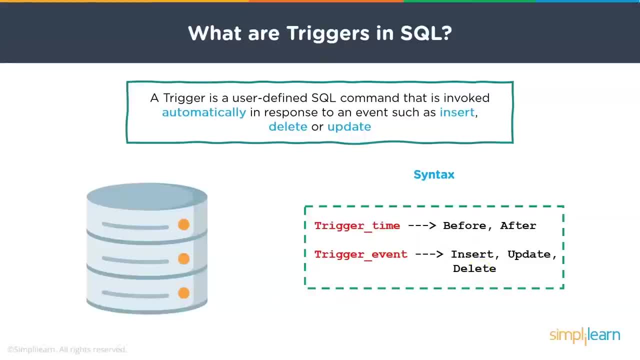 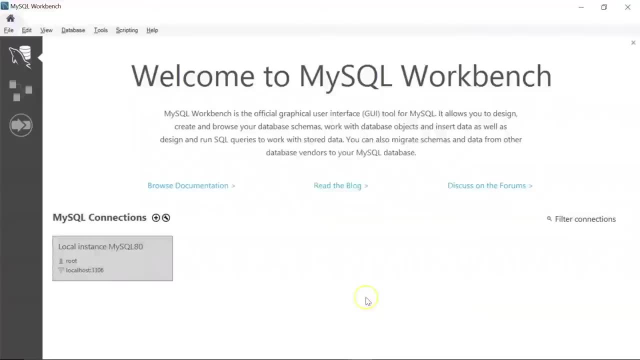 Now let me take you to MySQL Workbench, where we will learn how to create triggers and explore more on how it works. So I am on MySQL Workbench, So first let me go ahead and create my connection. I'll give my password. All right, now. this will take you to my SQL editor. Okay, so first and foremost, let me create a new. 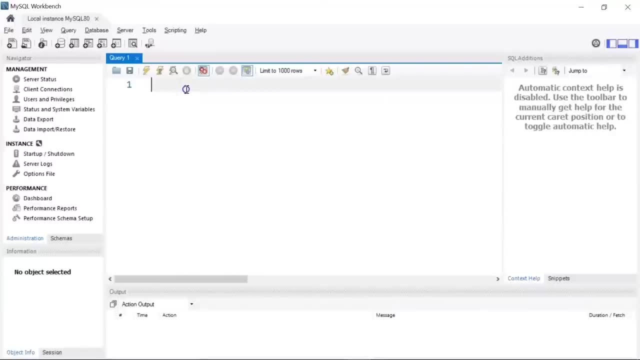 database called triggers, So I'll write my SQL command as: create database triggers. Let me run this Okay, so you can see here one row affected. I have created a new database. Let me run this Okay, so you can see here one row affected. I have created a new database. 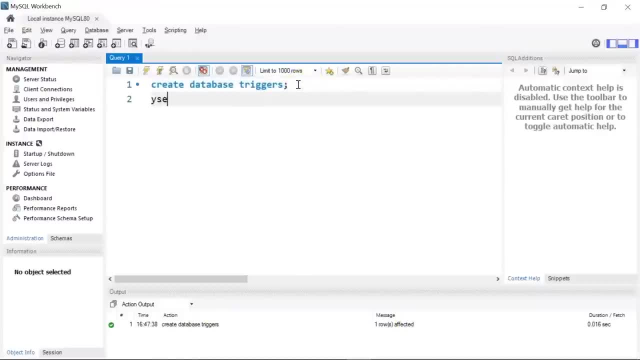 Let me run this. Okay, so you can see here one row affected. I have created a new database That is triggers. Next I'm going to move inside this database, So I'll write the command: use triggers. Let's run this Okay. now, inside this triggers database, we'll be creating our different. 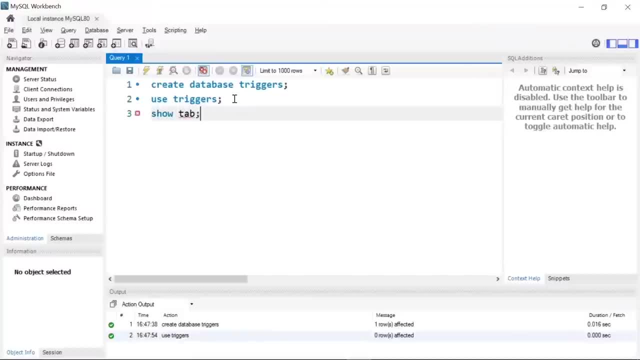 tables. So let's check. if we have any tables, I'll use the command show tables. Now you see there are no tables in this database. All right, first let's see how before insert trigger works. So for before insert trigger, we'll create a table called customers. 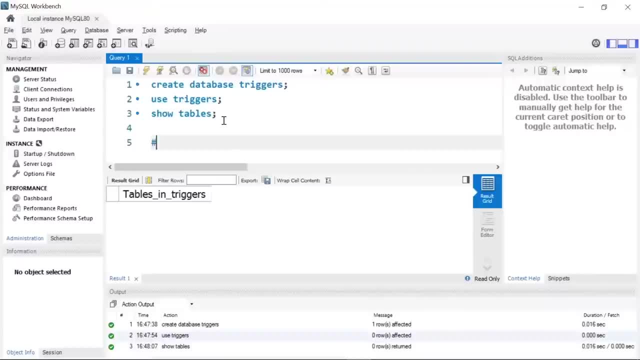 and verify the age of each customer. So I'll give a comment before insert trigger. So let me go ahead and create my customers table. I'll write create table- customers and I'll give my column names as cust underscore id, which is customer id. This is going to be an 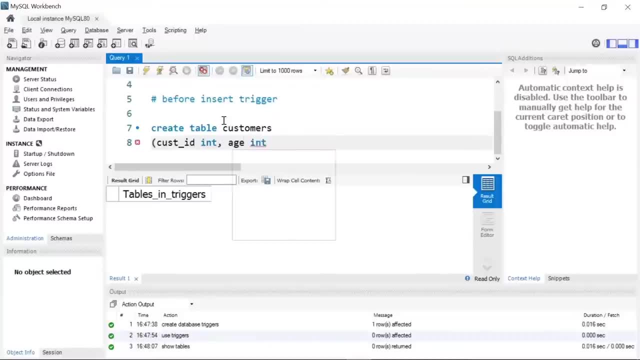 integer. Then we have the age of the customer. This is again an integer and we'll have the name of the customer. The name of the customer will be a worker type. I'll give the size as 30.. All right, let's create this table. 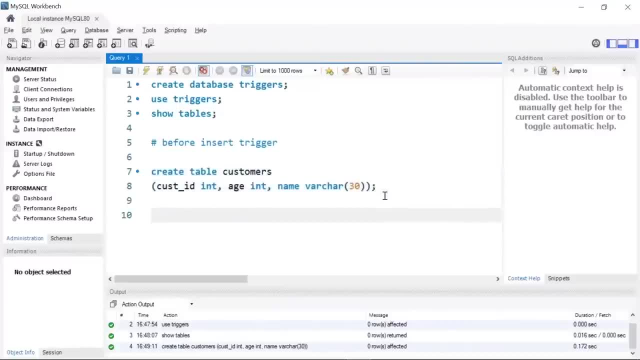 Okay, so we have successfully created our customers table. Now, moving ahead, I'm going to write my before insert trigger command. So we'll start with a delimiter. So a delimiter is a marker for the end of each command. Next I'll write my create trigger. 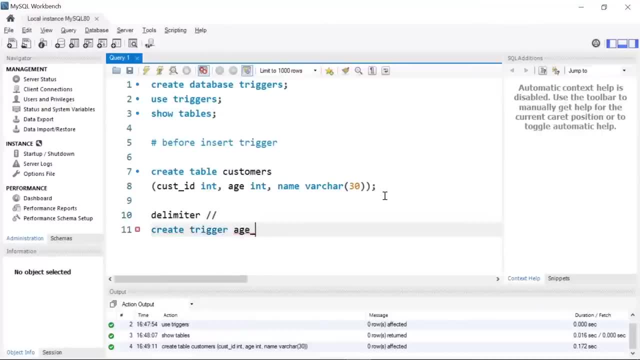 followed by the trigger name. I'll give a valid trigger name, such as age. underscore: verify. I'll write before trigger. it should be before insert on my table name would be customers. then I'll write for each row. if new dot age is less than zero, then set new dot age equal to zero, which means, while inserting your values, 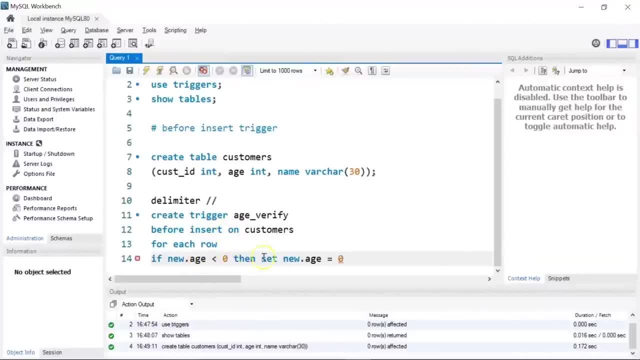 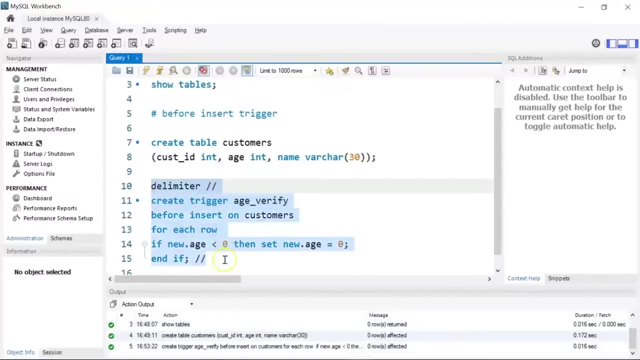 to the age column, in case the age value is negative, will convert the age to zero. I'll give a semicolon and then I'll write end if I'll give another semicolon and I'll close the delimiter. now let me run this. okay, so we have created our trigger. 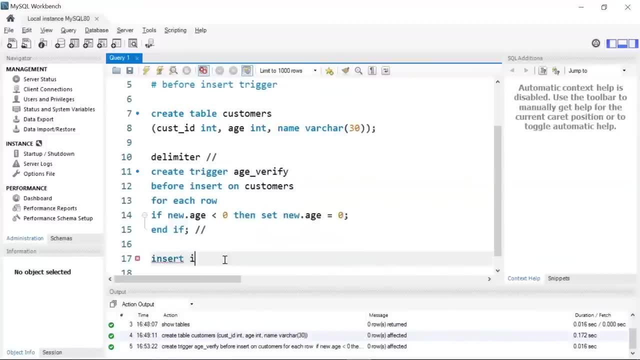 now let's insert a few values onto customers. so I'll write: insert into customers values 101, which is the customer ID. I'll give the age as 27 and let's say the name of the customer is James. let's insert another record, give the value as 102, and this time I'm purposely giving 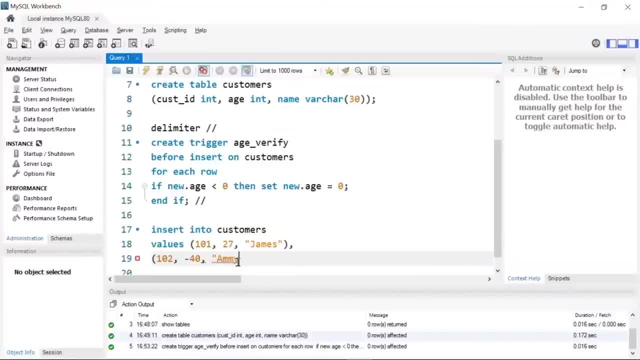 the age as minus 40, which is less than 0, so that you can see the output clearly. I've given the customer name. name is Ami. let's insert two more records. the customer ID with 103 has an age of 32 and let's say the name is Ben. I'll give another comma and finally we'll 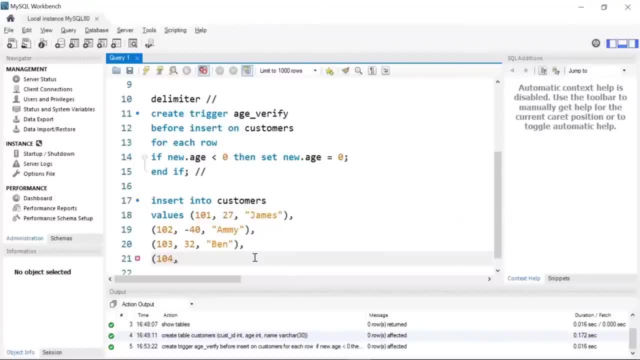 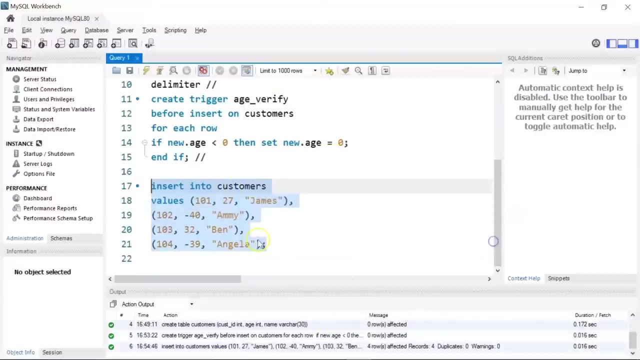 insert our fourth customer record. the customer ID is 104, the age I'm giving as minus 39, which is less than 0 again, and let's say the customer name is Angela. all, right now let me run this. okay, so we have successfully inserted four rows of information to our customers table. 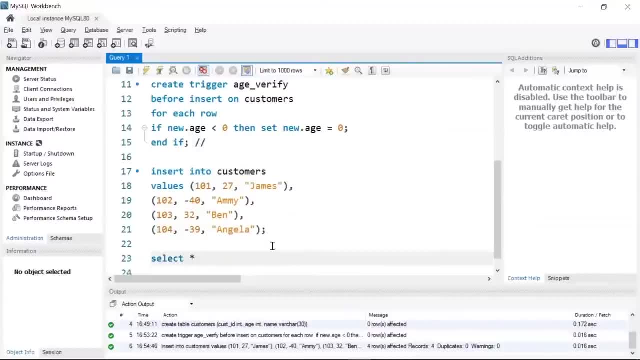 now let's see the difference, since we had created a age verified trigger which would change the values of the age column in case the age value is less than zero. so now that we have inserted four records to a customer. so let's see what we have in the customers table. now let me run it. there you go. so if you see this, 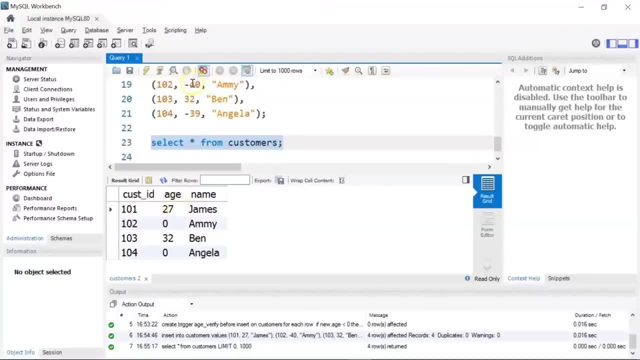 for those customers where the age was less than zero, such as 102 and 103. you can see here our trigger has automatically converted those values to zero. if you can see the trigger we had created, we had set our new age to zero if the age was less than zero and this is the output we get. so here we looked at how a before. 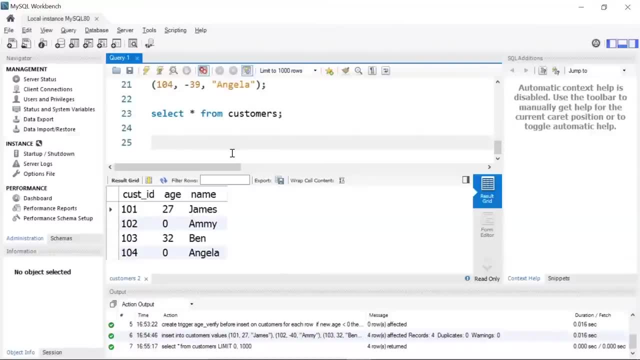 insert trigger works. alright, now moving ahead, let's understand how and after insert trigger works. so I'll give a comment here as after insert trigger you Now. in this example we'll create two tables: customers and message. Now the trigger will be fired if the birthday column has a null value in the customers table. 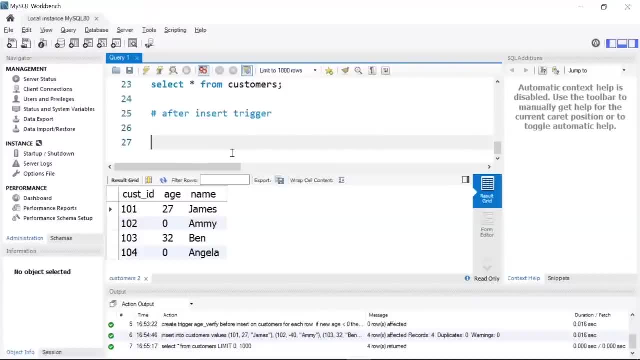 You will get a message to update your date of birth. Okay, so first let me create my customers table. Now, since we already have one customers table, I'll name it as customers1.. And let me give the column names. So the first column would be the ID column. 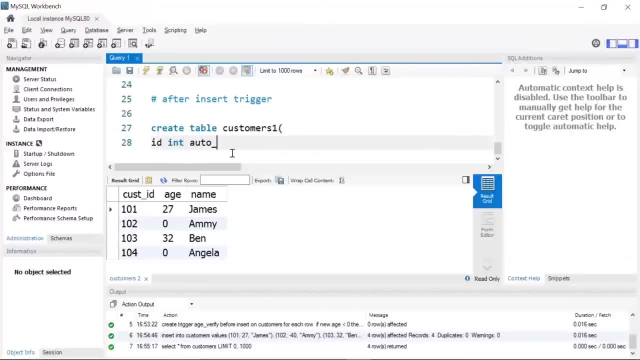 This is going to be an integer and I'll use the auto increment parameter, And this will be my primary key as well. Next, we'll have the name of the customer. This is going to be of type worker And I'll use not null constraint. 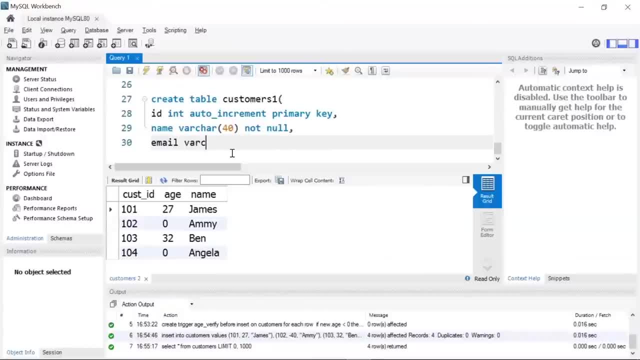 Next we'll have the Email ID of the customer. This is again going to be of worker type And the column we are interested in is the birthday column, So I'll write birth date. This is going to be of type date. 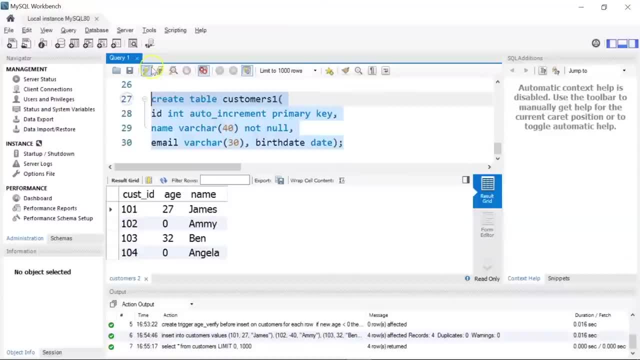 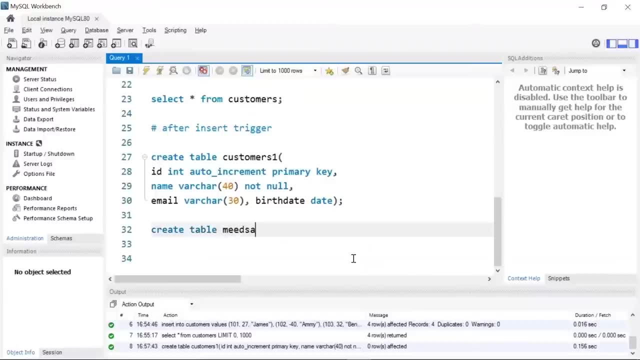 Okay, So let's create our table. All right, Now we'll create our second table, Which is going to be message. Let's create the columns. This will have ID int and I'll use the auto increment operator. 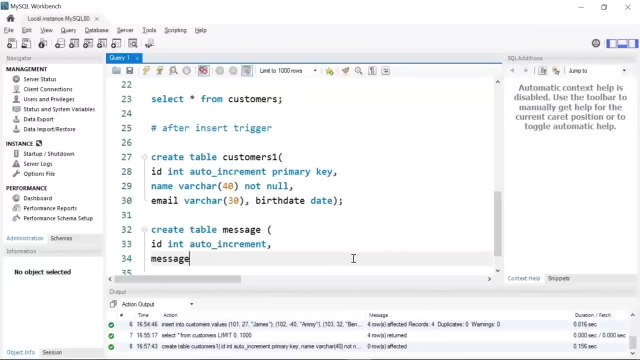 Next we'll have the message ID. This is going to be of integer type. We'll have a column called message. This will be of worker type, Let's say 300 characters And not null, And I'm going to set my primary keys. 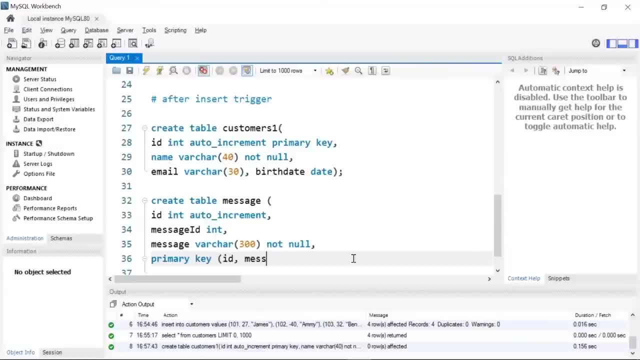 As ID and message ID. Let's create our second table then. So we have some error here. Let's debug the error. Okay, So I forgot to close the bracket here. All right, Now let me run this table. 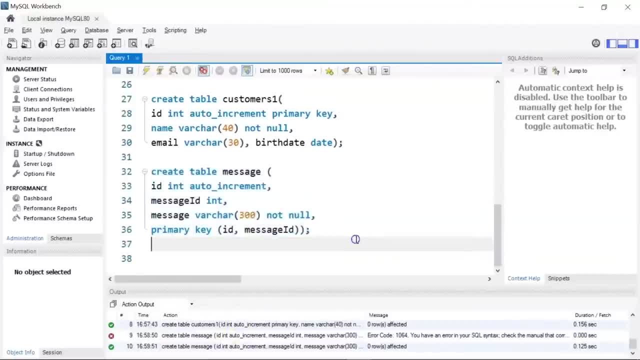 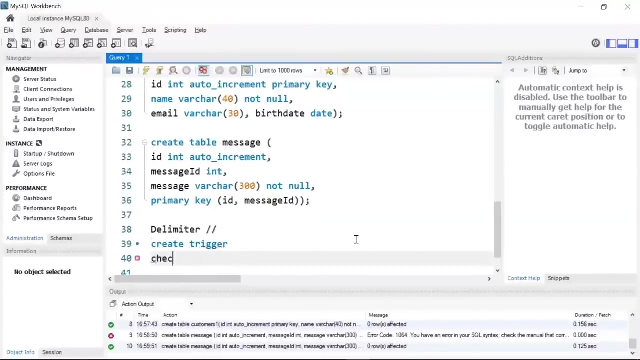 All right, So we have created our message table as well. Next I'll write my after insert trigger command, So I'll write delimiter. Next I'll use create trigger command, So I'll write create. My trigger name would be check underscore null. underscore date of birth. 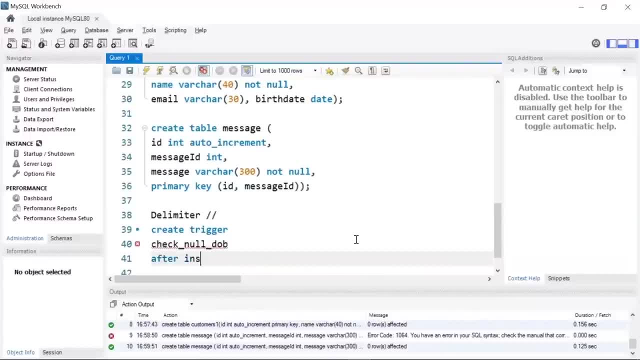 After insert on customers, one for each row, begin And then, if New Birth date Is null, Then we are going to insert into our message table. Give the columns as message ID and message And as a message values newid comma. I'm going to use the concat function where I'll give my message. 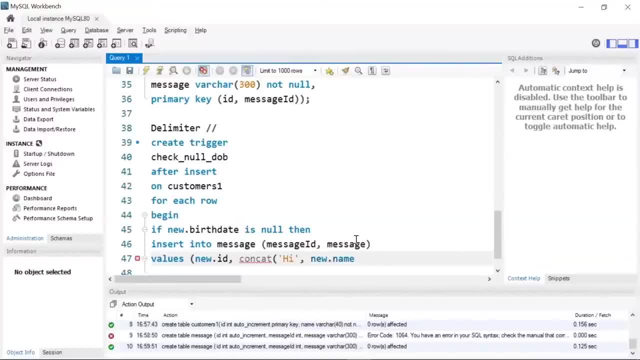 let's say hi, followed by the name, followed by, let's say: please update your date of birth. Okay, now I'll write end if I'll close the delimiter. Okay, so let me go to the top and recheck. 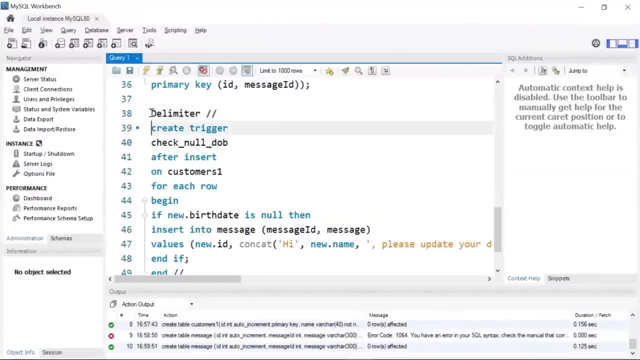 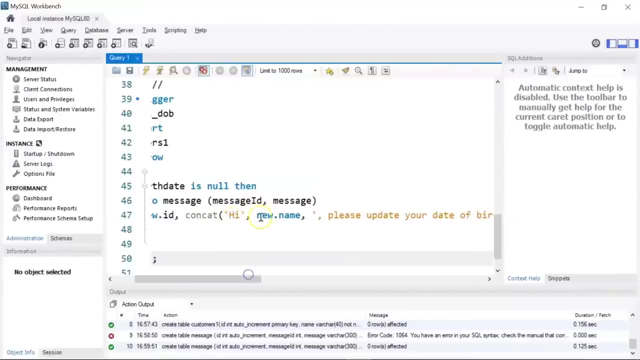 if we have created our trigger correctly. So I have my trigger name after insert on customers, one for each row begin: If our new birthday has a null value, then we'll pass in a message saying hi, the name of the customer. then the message would be: please update your date of birth. 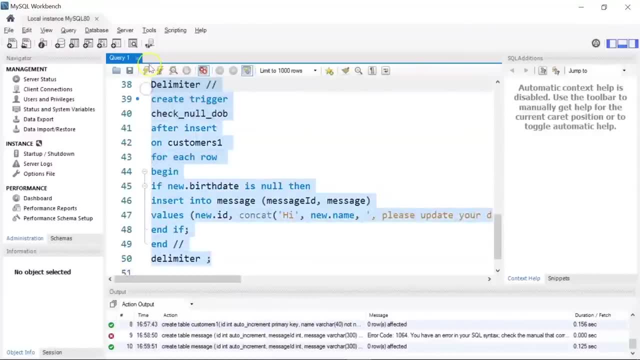 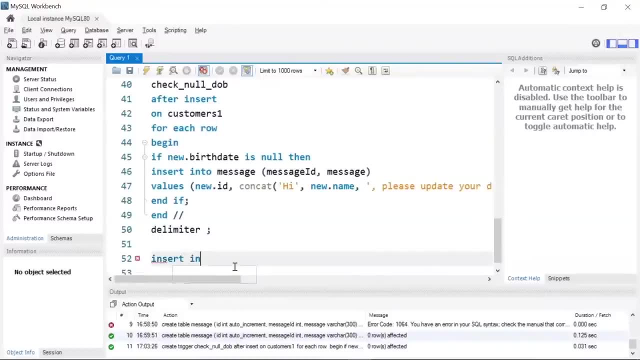 Alright, so let's run the trigger. Okay, now the next step is to insert a few records to customer table. So my name of the table is customers one. Okay, I'll give the column names as name, email, birth. okay, we'll pass in a few values. so our first customer's name, let's say, is: 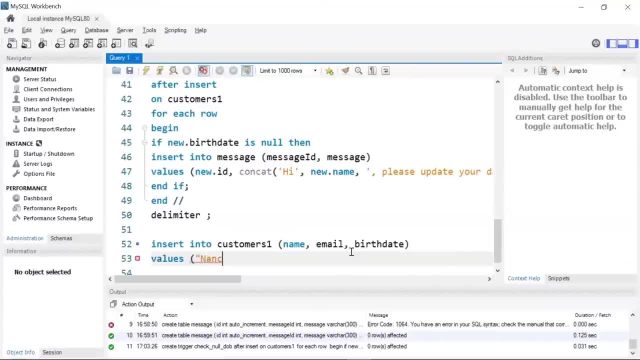 Nancy- comma. I'll give my email ID, let's say Nancy, at the rate ABC comm. now, let's say I'm purposely passing the date of birth as null, I'll give a comma. my next customer, let's say the name of the customer is Ronald, and then I'll give the email ID, such as Ronald, at the rate XYZ comm. and. 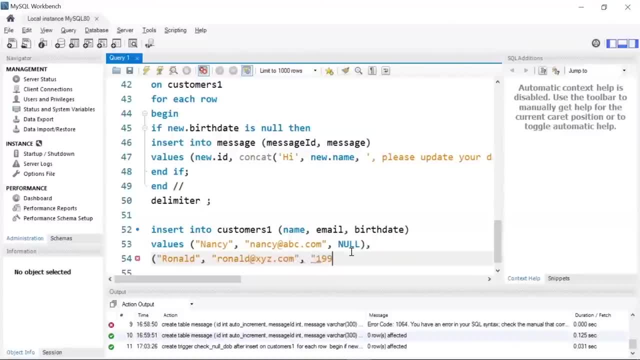 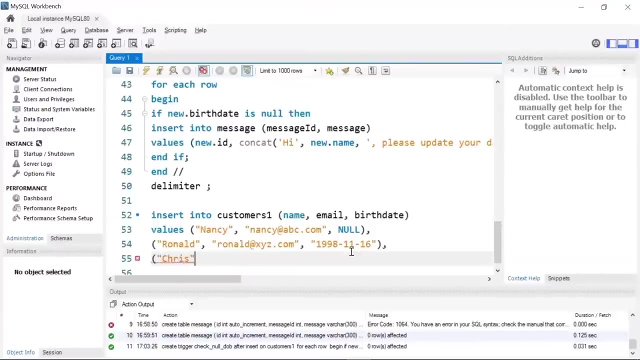 this time I'm going to pass in the date of birth, let's say 1998, November, and let's say 16th. okay, now we'll add another customer, let's say Krish, at the rate, XYZ comm. we'll give the email ID of Chris. so Krish at the rate. 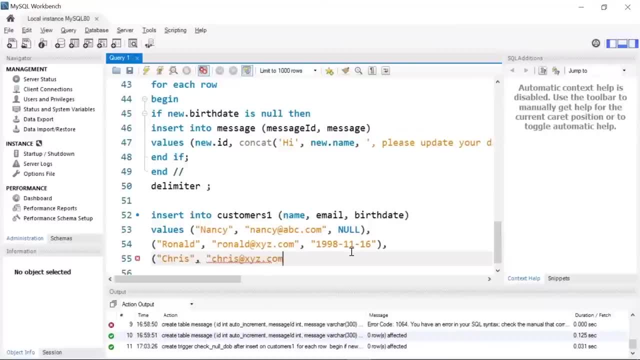 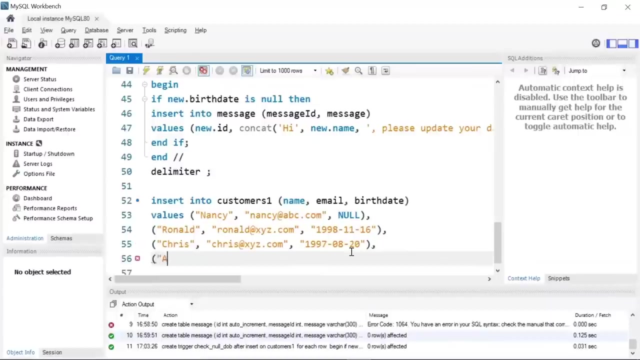 XYZ comm. and let's say we'll keep the date of birth as 1997 zero eight twenty. and finally we'll add one more request. we'll give the date of birth as 1997 zero eight twenty. and finally we'll add one more request for another customer, let's say Alice. I'll give the email ID as Alice at the. 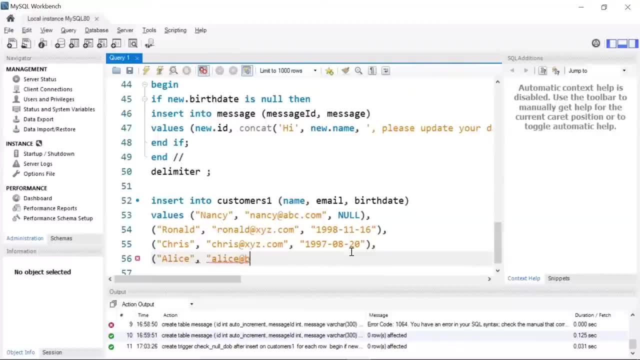 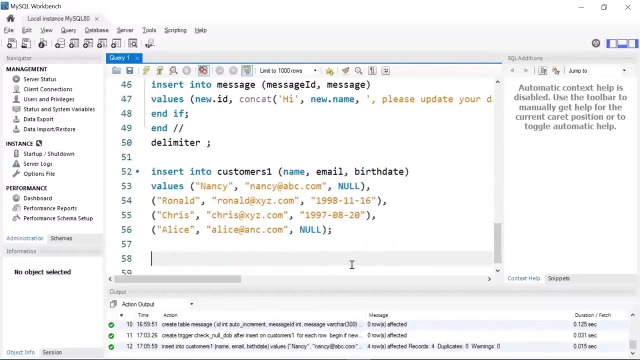 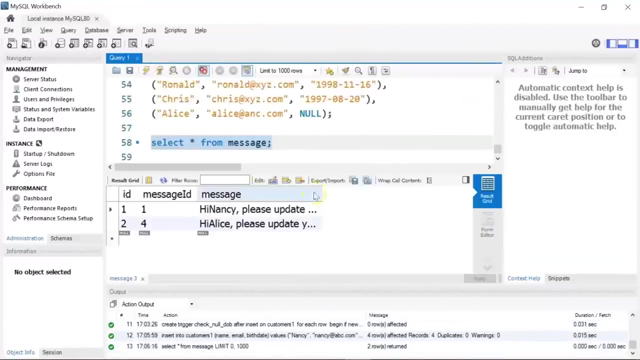 rate ABC comm, and this time I'll purposely pass the date of birth as null. all right, so let's run the insert query. okay, now let me display the message table for you so that you can see the output and how our after insert trigger works. there you go. 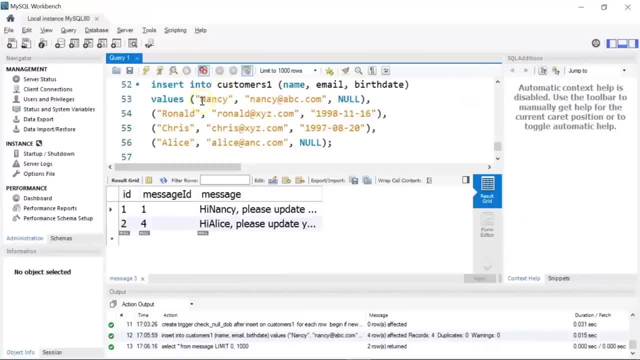 so, if you see this, we had inserted four rows of information, out of which the first customer ID and the fourth ID had null date of birth. so for those two values you have the messages: hi Nancy, please update your date of birth. and then you have hi Alice, please update your date of birth. now you 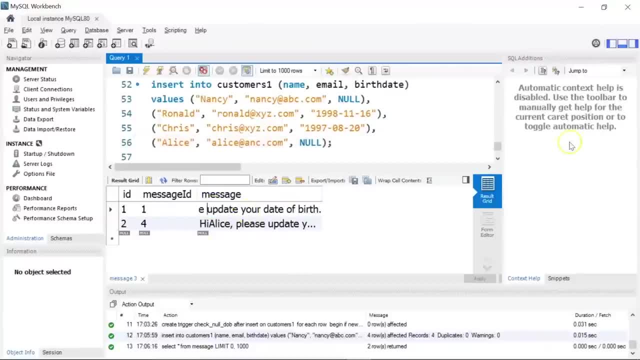 can give a space between hi and the name of the customer. all right, now, moving ahead, let's understand how before update trigger works. so I'll give a comment here, as before update. okay, now to show you how before update works. first we'll create a table called 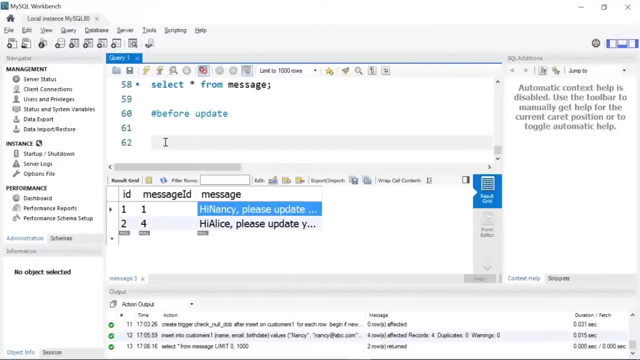 employees. all right, so let me create my table, that is, create table employees. I'll give my column as employee ID. this is going to be an integer type and it will be my primary key. next we'll have the employee name. this will be of varchar type and let's say the. 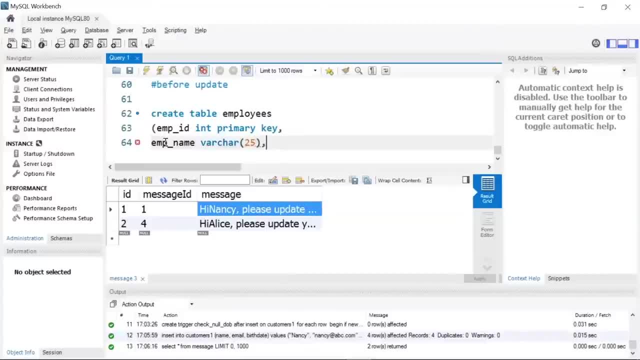 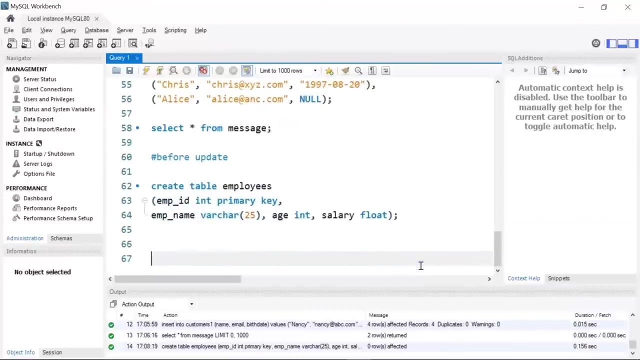 size would be 25 comma. then we'll have the age of the employee. age will be of integer type and finally we'll have the salary of the employee. salary will be of type float. let's create the figure. we have somewhere close to 20 and we'll give it 0.012, Dr. 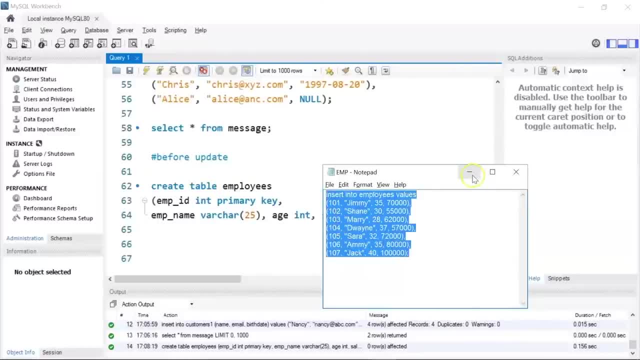 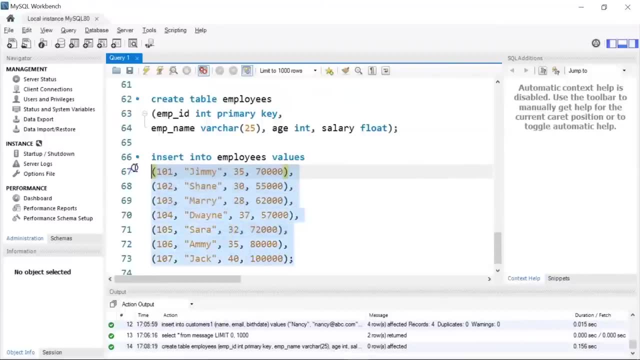 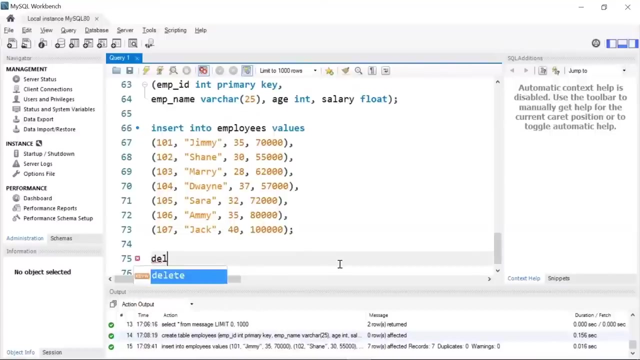 Ro an average right, so we should be able to do this. so the first thing we're going to do is ensure sandy cds table right. you create the table and then you're going to give the variable an ieurs table. next we'll write our before update trigger command. so, first and foremost, I'll write my 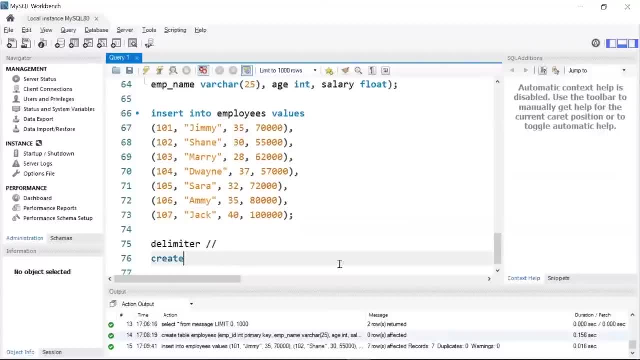 delimiter, followed by the create trigger command. I'll give my trigger name as update underscore trigger. let's bring this to the top. okay, I'll use before update. on my table, that is, employees. for each row, I'll write begin. my condition would be: if new dot salary is equal to, let's say, $10,000, I'll write then set new dot salary equal to. 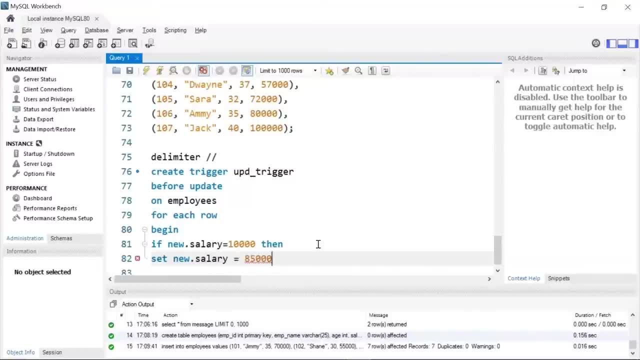 $85,000. I'll give a semicolon. then I'll use. else, if new dot salary is less than $10,000, then I'll set new dot salary to, let's say, $72,000. I'll give a semicolon. I'll end the if statement. I'll close the delimiter by giving a semicolon. 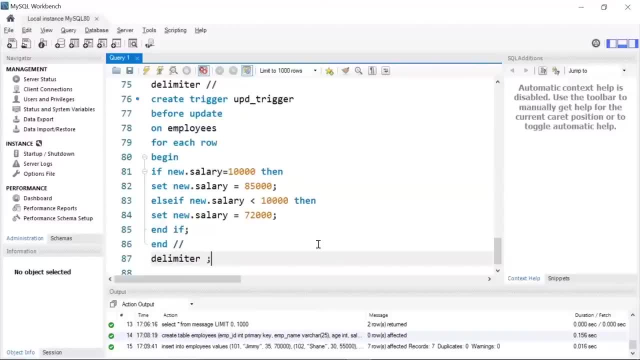 okay. so if you see the employees table, we have the salary values here now in case, while updating the table. if the salary is equal to $10,000, we'll set the new salary to $85,000. else, if the salary is less than $10,000, we'll set the salary column values to $72,000. 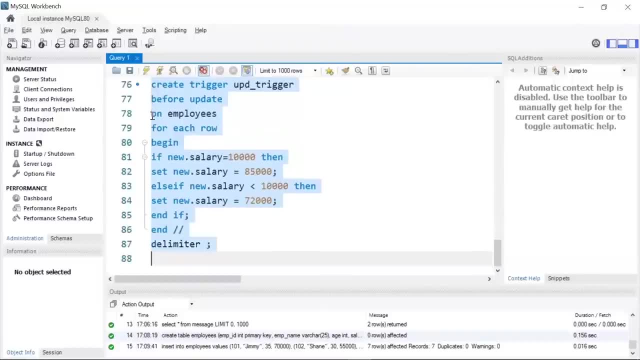 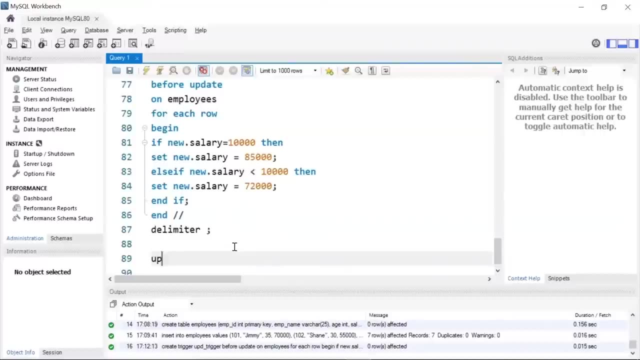 so let's go ahead and run this trigger query. all right, now let me use my update command, so I'll write update employees. I'll write: set salary is equal to, let's say, $8,000. now, if you see our trigger query, we are setting the salary to $8,000, which is clearly less than $85,000. so let's go ahead. 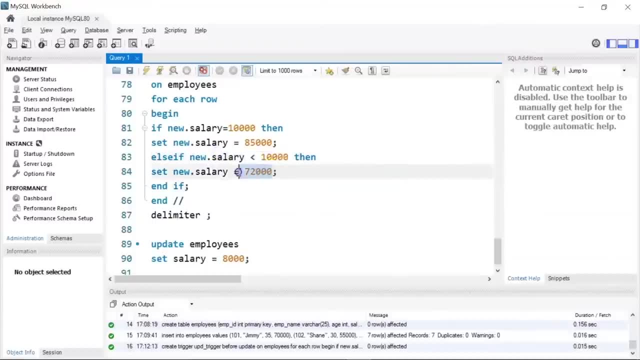 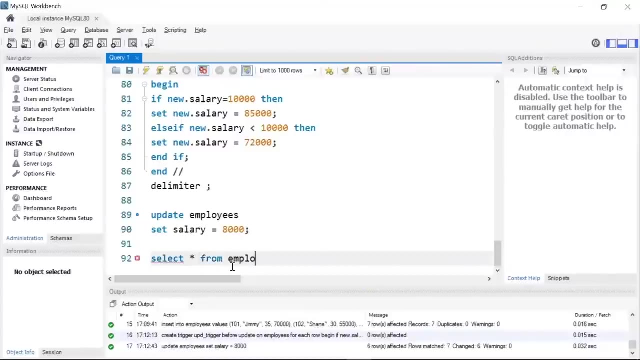 running this and this appears like we have an increase actually than $10,000, so our new salary would be $72,070- huge. so let me run this. okay, so you can see here six rows affected, so I'll right now select star from employees. let's run. 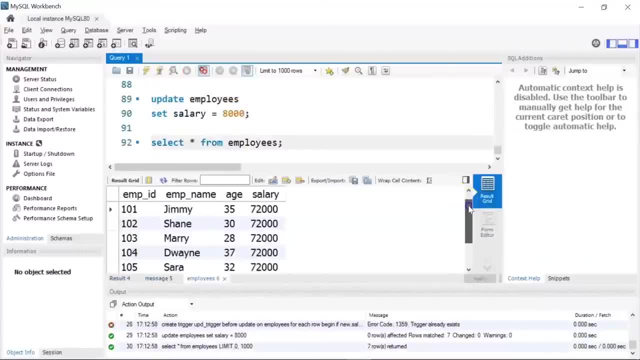 this. okay, if you see this, we have converted our salary column to $72,070 thousand dollars. since we updated the salary to eight thousand dollars and, according to our trigger query, if it's less than ten thousand dollars, the salary should be seven to two thousand dollars, which you can see here. 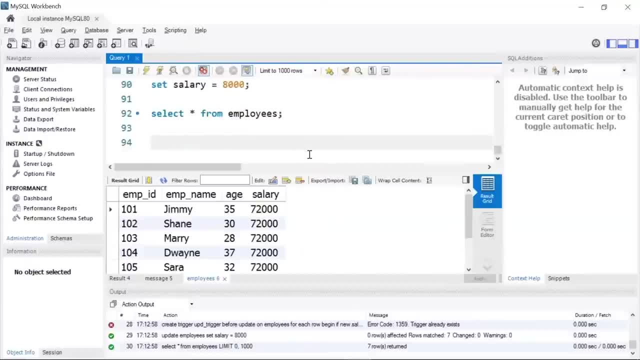 all right now moving to our final demo. this time we are going to explore how before delete trigger command works. so in this example we'll create a table called salary, will store the deleted record in a new table using the before delete trigger. so first I'll give my comment, as before trigger comments are: 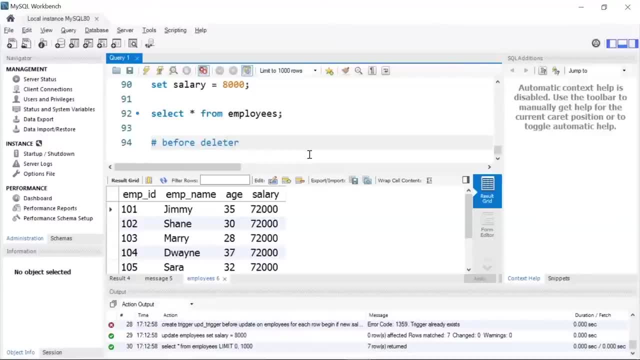 always useful, since they make your query more readable. so let me now create my salary table. so I'll write: create table salary. I'll give my you column names as e ID, which is employee ID, and I'll set it as primary key comma. I'll give another column, let's say valid, from, which means the date from which the 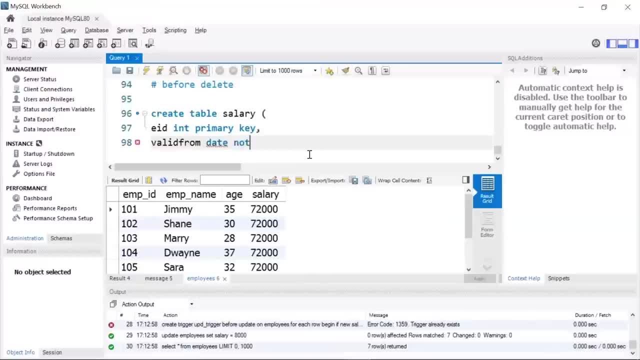 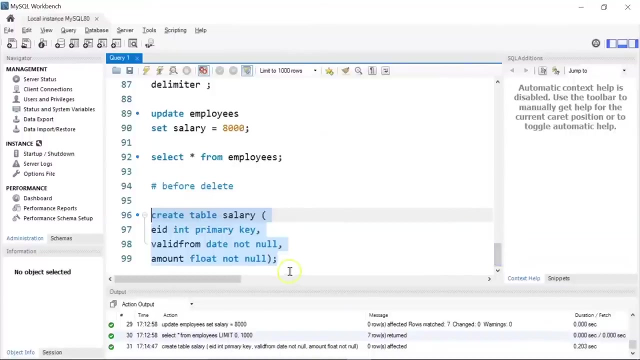 salary was effective is going to be of type date and not null, and then I'll have the amount. amount will be of type float and again, not null constraint. let me run the create table command. okay, so we have created our salary table. now the next thing is to insert a few values, so I'll 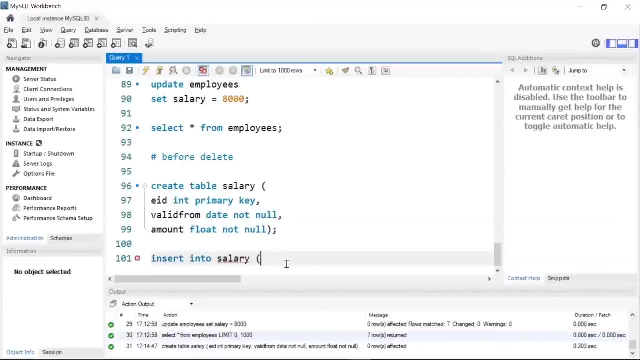 write insert into salary. I'll give my column names as e ID, comma valid from comma amount. I'll write values. my first employee ID would be 101, followed by a date, let's say 2005, May and 01, which is first of May 2005, let's say the amount is fifty five thousand. 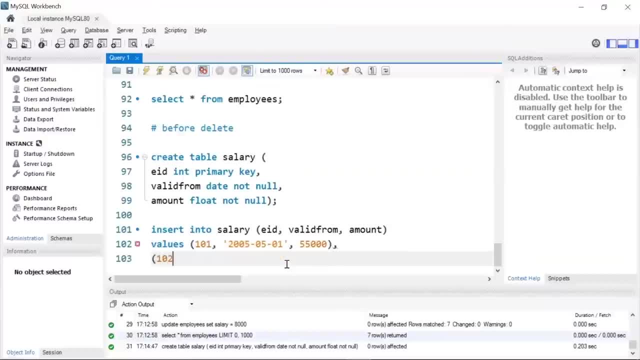 dollars. I'll give another row of information. this time the employee ID is hundred and two and I'll give a valid from date, let's say value of today, a valid from date, let's say the amount is sixty eight thousand. I'll give another employee ID, let's say one zero three, 2006. 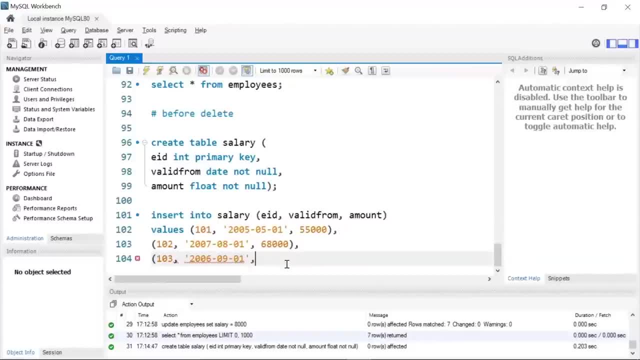 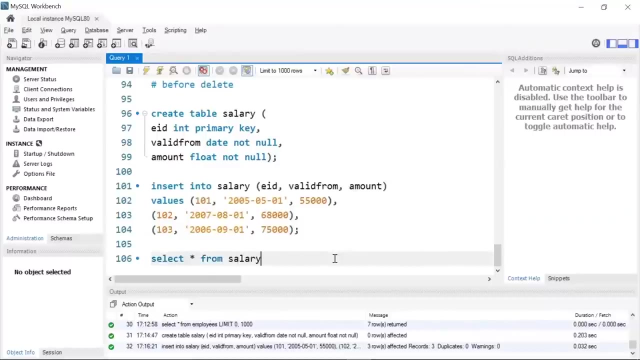 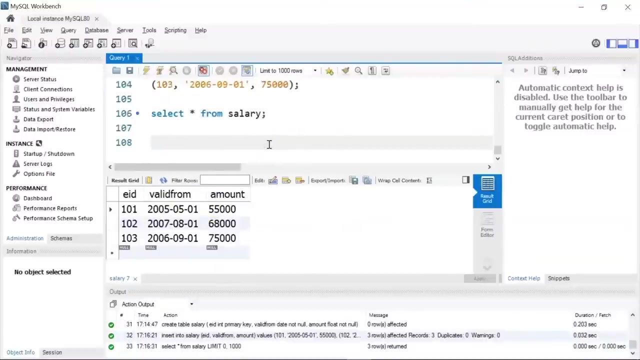 estrus: zero nine, zero one, zero five, excellent, and let's say the amount is $75,000. okay, let's run this. all right, you can verify also, so I'll write: select star from salary. you can see here we have inserted three rows of information, all right. the next step is to create another table. 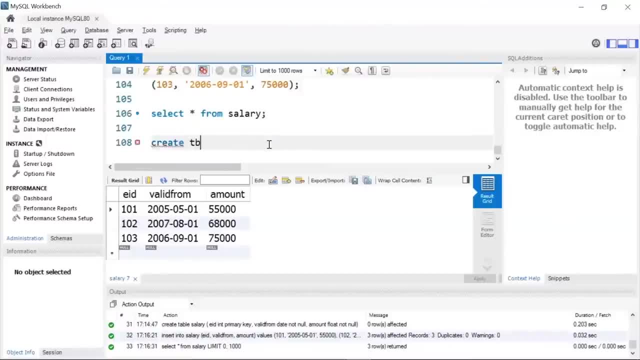 that will store the deleted rows. so I'll write create table. let's say the name of the table is create, or let's say salary delete. I'll write salary del. now this will have the ID. the type would be integer and primary key. I'll also use 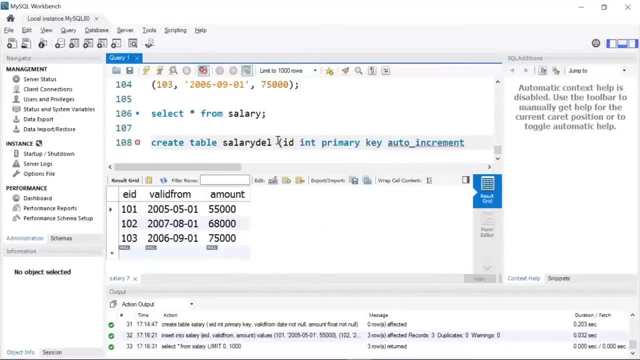 the auto increment operator. next we have the EID, which is of type integer. I'll write valid from date and not null. then I have the amount column, which is of type float and not null. my final column would be deleted at. the datatype will be timestamp. I'll use the 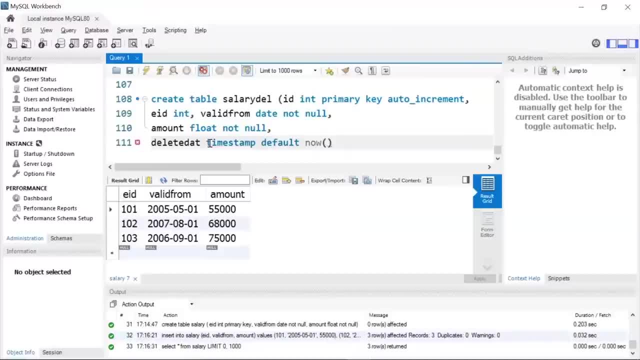 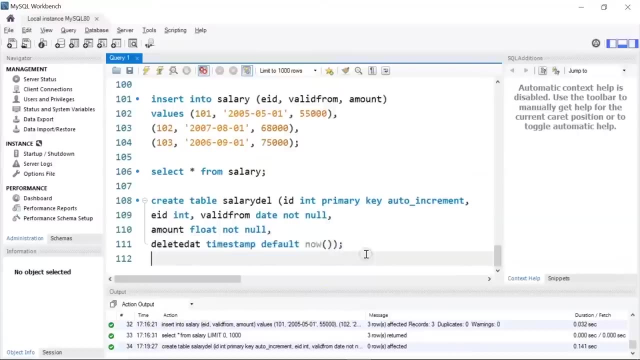 default constraint as now, so this will return the time and the date at which the record was deleted. all right, let me create this table, okay? finally, the third thing that I need to do is I need to create the timeline for the table, and I'll create a timeline for the table, okay, so let's proceed with the timeline. 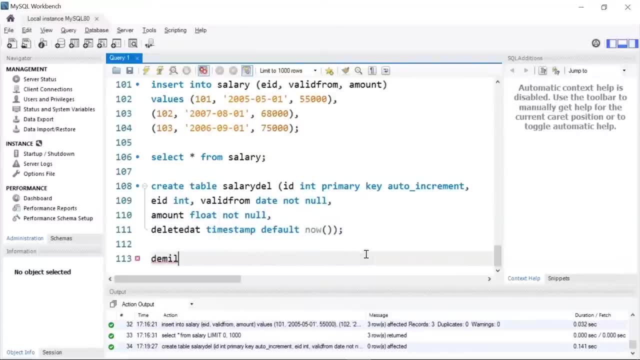 table itself. let's do that. so this is the first one. okay, let's do this. so let's let me write my before delete trigger command. so i'll first declare my delimiter. let's say: this time i'm using the dollar symbol. i'll write create trigger. 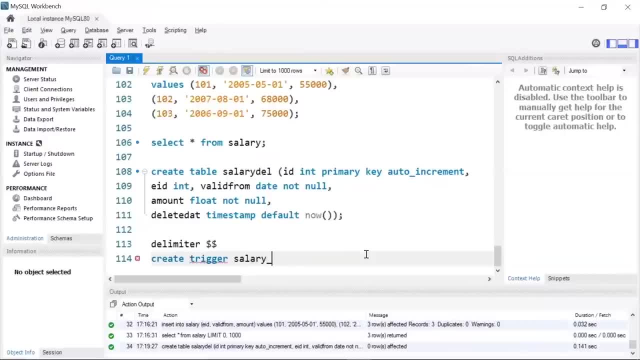 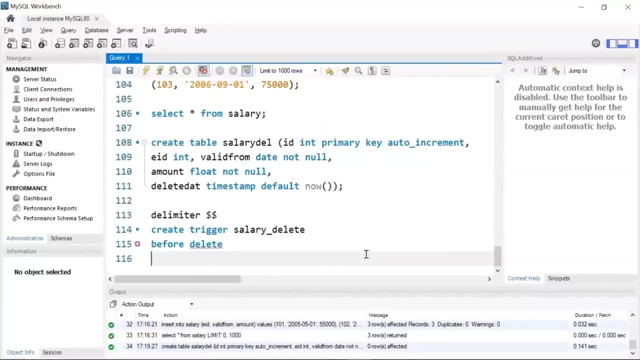 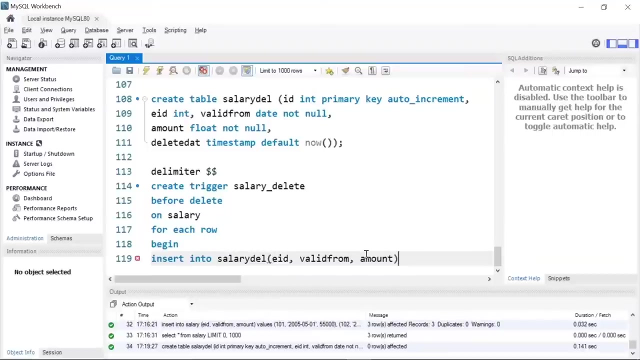 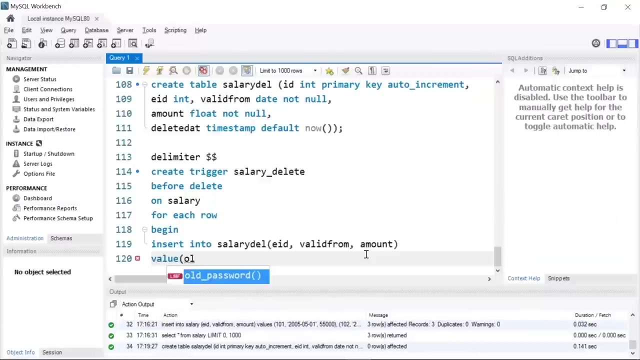 my trigger name would be salary underscore: delete. before before delete. on my table that is salary. for each row i'll write begin next. let's insert into salary delete. i'll give my columns as employee id: valid from and amount. now we'll insert a few values. i'll write values: old dot, eid. comma. old dot. valid from comma- old dot. 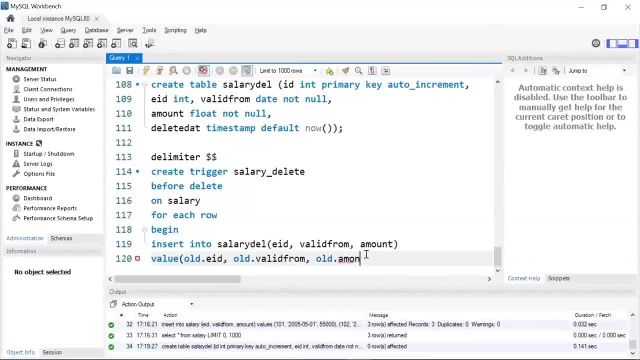 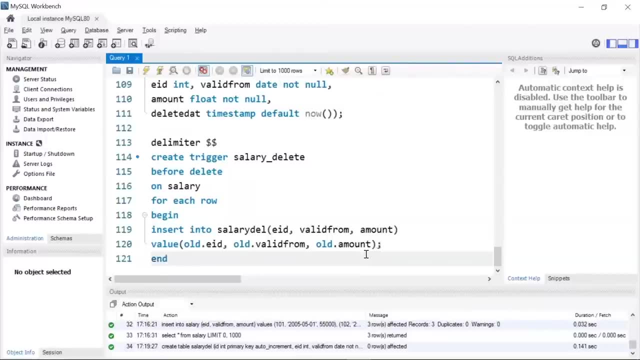 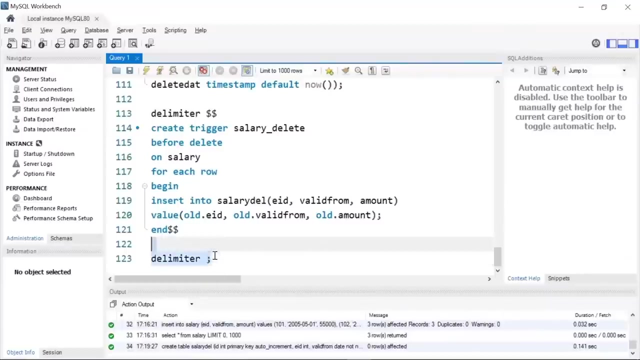 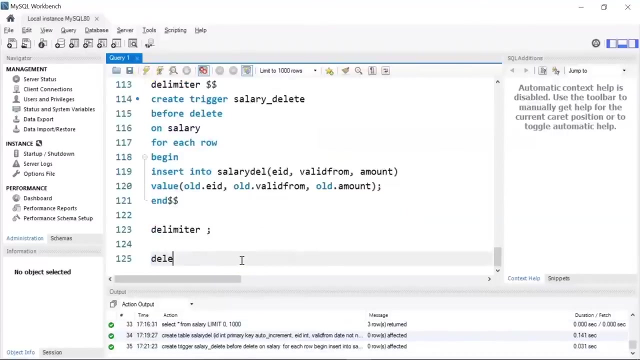 amount. i'm going to close with the delimiters, all right, so let's run our before delete trigger. all right, now let me go ahead and delete one of the records from the salary table. so i'll write: delete from salary where employee id is, let's say, student, say 103. let me run this query. 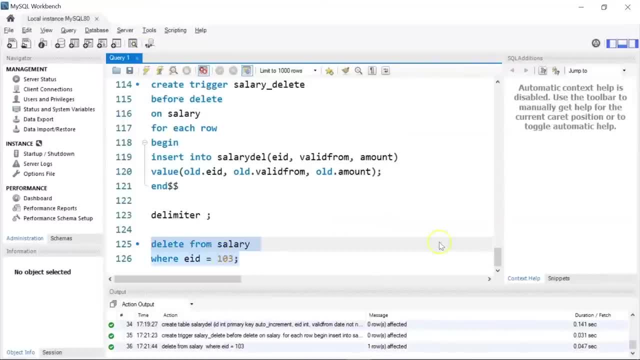 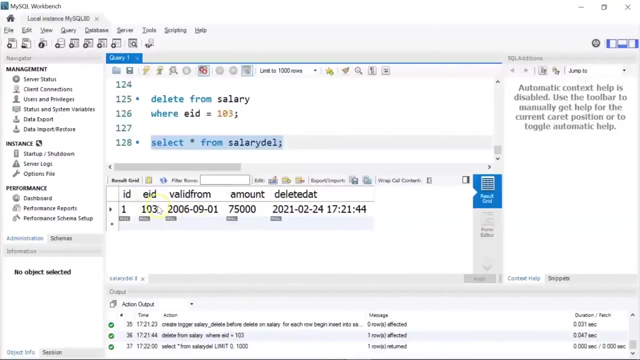 okay, so you have successfully deleted one of the records in the table. now, if you see our other table, that is, salary delete, you will find this information present in the salary delete column. so we had deleted one row of information, that is for employee id 103, which you can find it here now, the final. 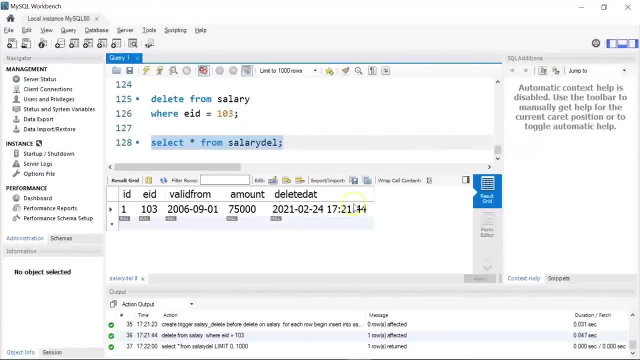 column that is delete at shows the time at which the information was deleted or the row was deleted. all right, so let me go to the top and just give you a recap of what we did in this demo. so first we created our database called triggers. then we started with before insert trigger, where 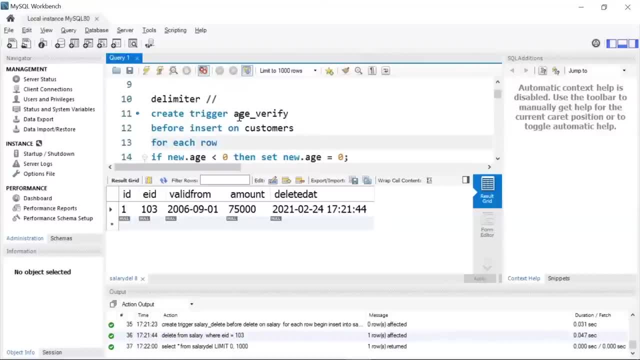 we inserted customer table and then we verified the age of the customers so we saw if the age was less than zero, then we set the age to zero. we inserted a few records to the customers table and purposely we inserted some negative age records and then we converted this age records. 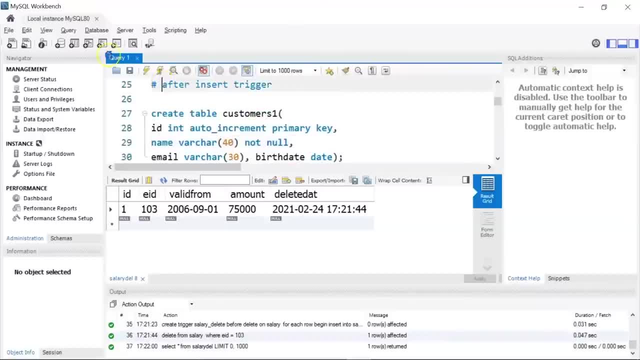 to zero. then we learned how an after insert trigger works. so we created two tables, customers one, and message. so wherever the customer's date of birth was missing, we passed in a message saying: hi, the name of the customer, please update your date of birth. all right now, moving ahead, we saw 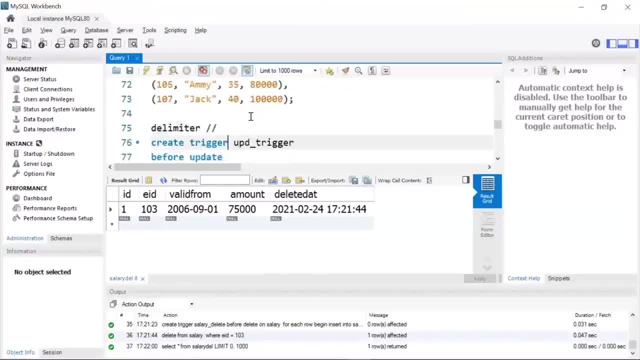 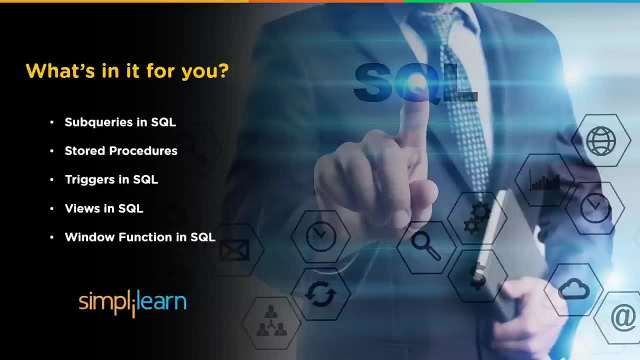 how before update trigger works. and finally, we learned about before delete trigger. so in this video we will learn sub queries in sql. we'll also have a look at stored procedures and learn about triggers in sql. we'll cover views in sql and look at some of the important windows functions in sql. now to learn all of these, we'll be using the mysql workbench. 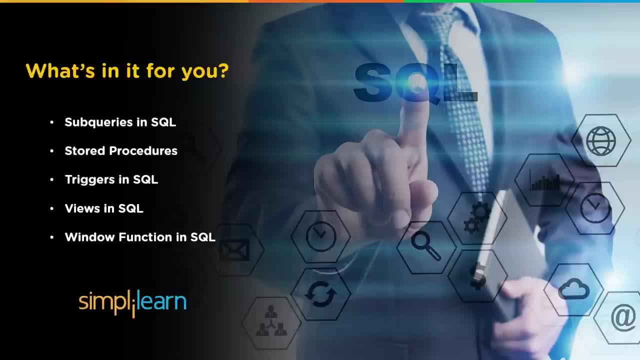 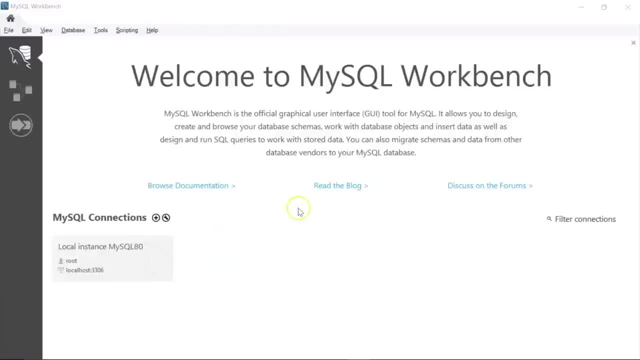 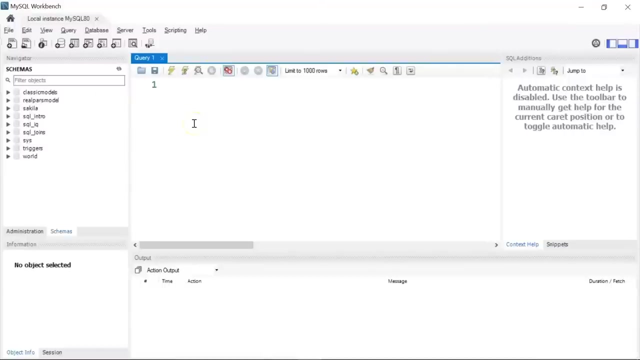 on windows. so let's get started with sub queries in sql. so let me head over to my mysql workbench. so currently i am on my mysql workbench. let me connect to the local instance. so i'll give my password. i'll click on ok, all right. so this is my mysql workbench query editor. so first we are going to 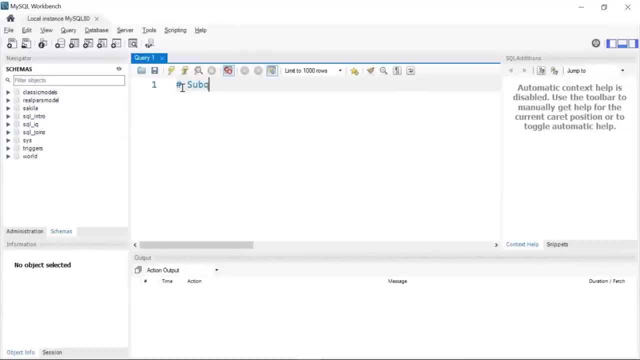 learn sub queries. let me give a comment and write sub queries, all right. so first of all, let's understand what a subquery is. so a subquery is a query within another sql query that is embedded within the where clause from clause or having clause. so we'll 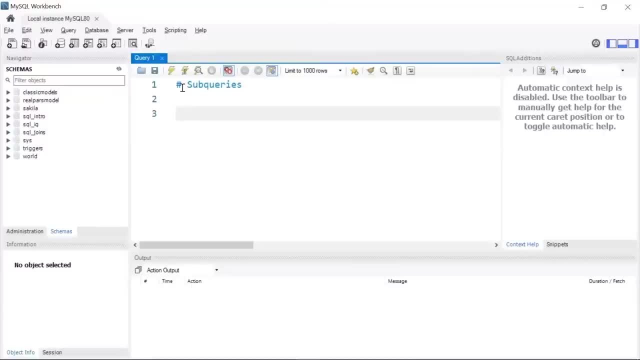 explore a few scenarios where we can use sub queries. so for that i'll be using my database, that is sql underscore intro. so i'll write my command: use sql underscore intro. now this database has a lot of tables. i'll be using the employees table that is present inside sql underscore intro. 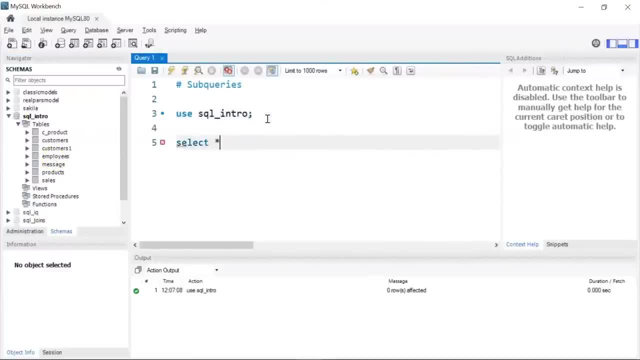 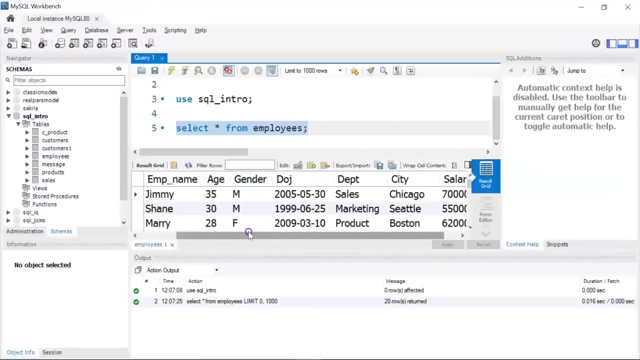 an employees table, so let me first show you the contents within this table. i'll write select star from employees. let me execute it. okay, you can see here we have the employee id, employee name, age, gender, there's date of join, department, city and salary and we have information for 20 employees. 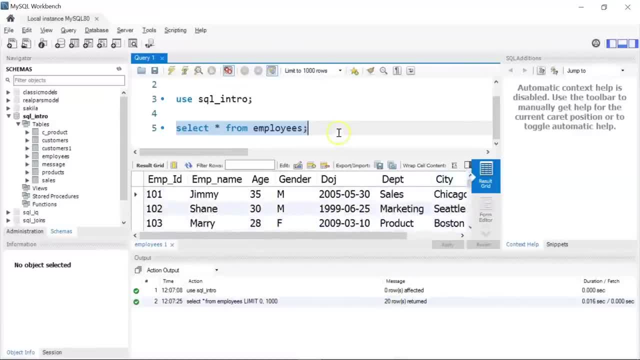 if i scroll down, you can see there are 20 employees present in our table. so let's see. you want to find the employees whose salary is greater than the average salary. in such a scenario, you can use a subquery. so let me show you how to write a subquery. i'll write the select statement. 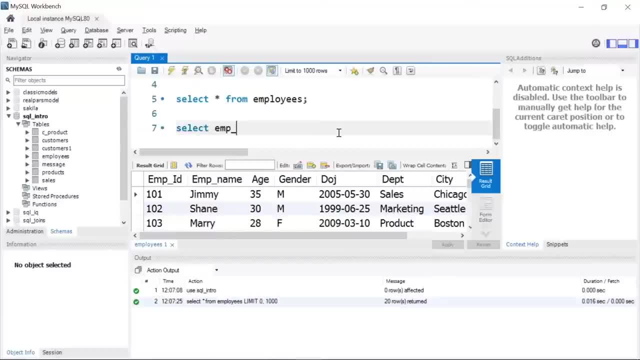 in the select statement i'll pass my column names that i want to display. so the column names i want are the employee name, then i want the department of the employee and the salary of the employee from my team, that is, employees. next i'll use a where condition where my salary should be greater than the average. 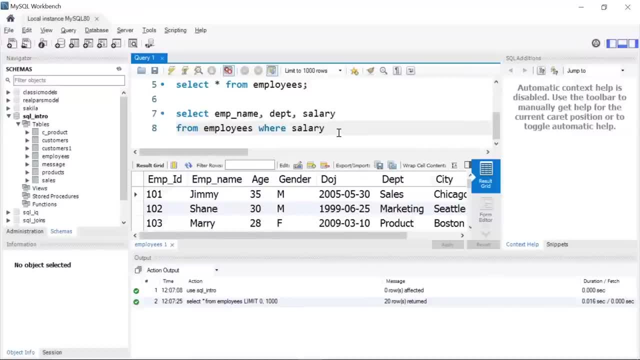 salary of all the employees. so i'll write salary greater than after this, i am going to write my subquery, so i'll give select average of salary from my table name, that is, employees, and i'll close the bracket and give a semicolon. so what it does is: first it is going to find the average salary of all the employees. that 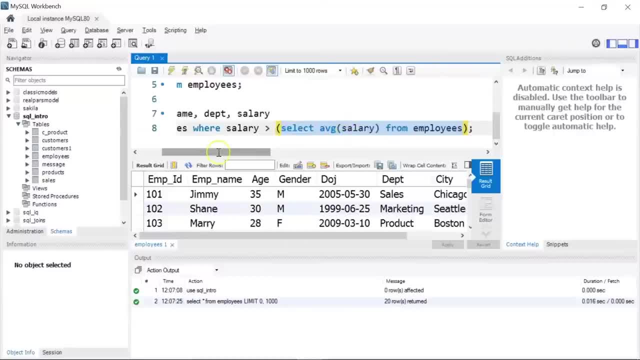 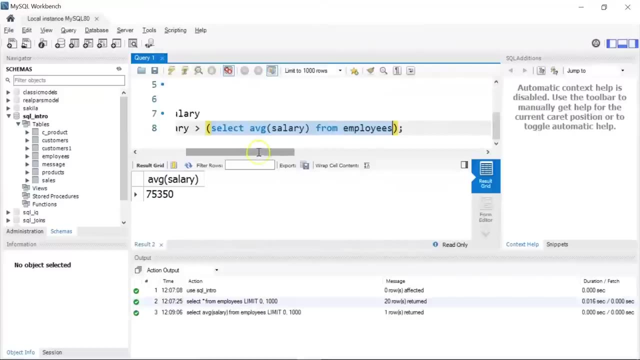 are present in our table once we get the average salary number. we'll use this where condition, where salary is greater than the average salary number. so the inside subquery. let me run it first. if i run this, this gives you the average salary of all the employees, which is: 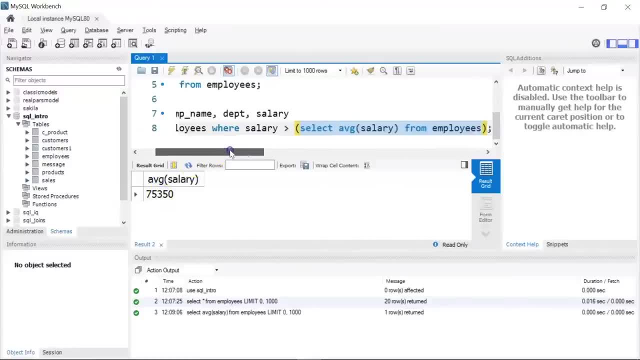 75 350 dollars. now i want to display all the employees who have salary greater than 75 350 dollars, so let's run our subquery. there you go. so there are eight employees in our table who have a salary greater than the average salary of all the employees. all right. next let's see another example. 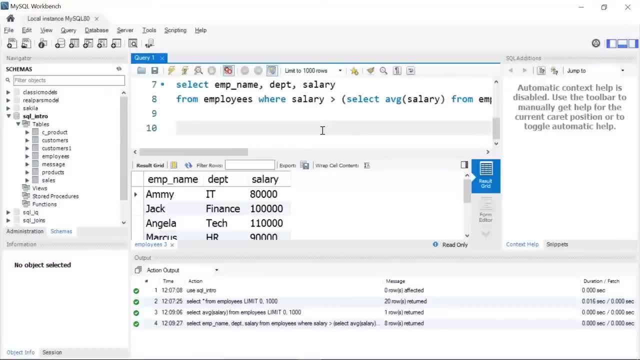 suppose this time you want to have a salary greater than the average salary of all the employees. so if you are Dave, you want to find the employees whose salary is greater than jail's salary. so we have one employee whose name is John. let me run the table once again. 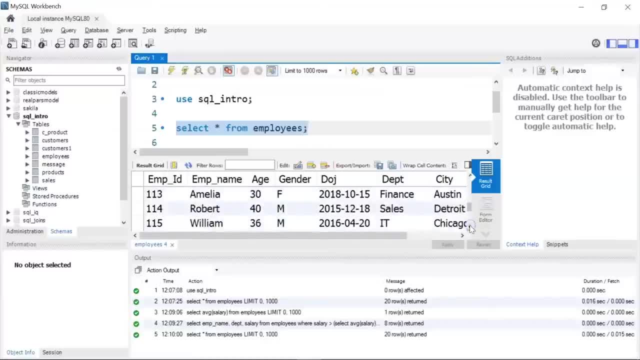 okay, if i scroll down, you see we have an employee as John. you see this: our employee id 116 is John and his salary is 67 000 dollars. all the employees whose salary is greater than John's salary, so basically, all the employees who are earning more than $65,000. I want to print them. so 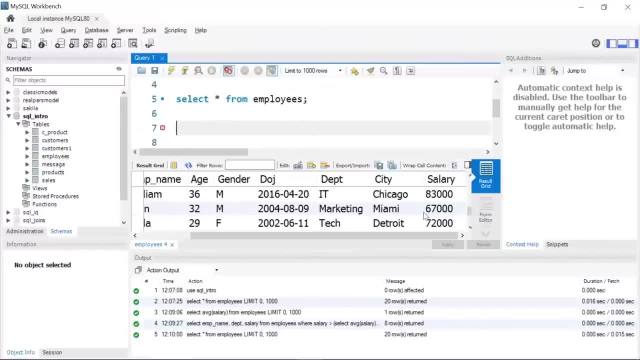 let's see how to do it. I'll write select. I want the employee name comma, the gender of the employee. I also want the department and salary from my table name, that is, employees. I'll write where salary is greater than. I'll start my opening bracket. inside the bracket I'm going to give my inner query, that is: 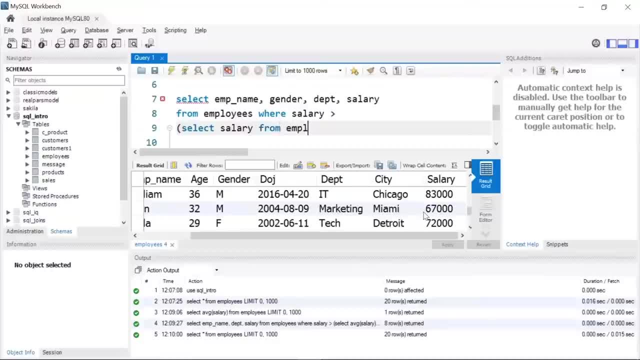 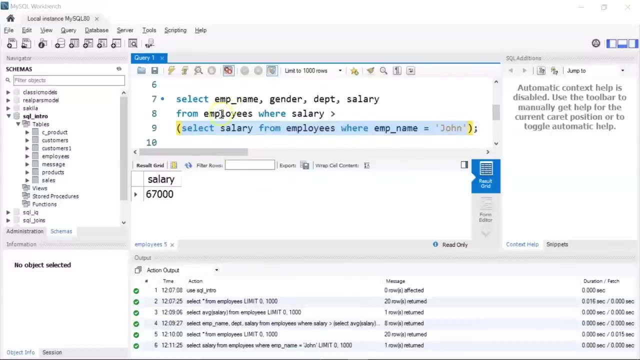 select salary from employees where the employee name is John. so, within single quotations, I'll give John as my employee. I'll end with a semicolon, so let me first run my inner query. so this will give us the salary that John has, which is $67,000. now I want the employees who 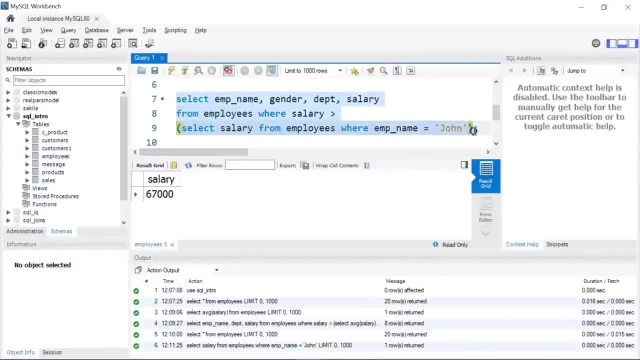 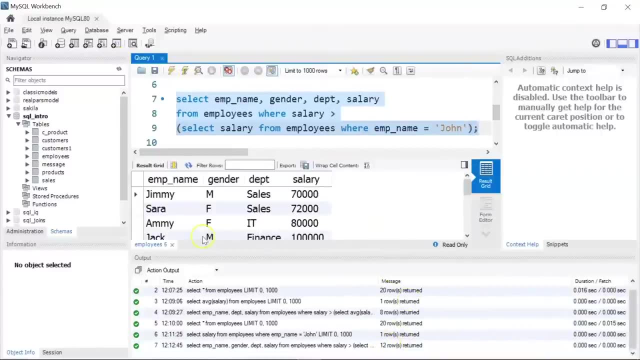 are earning more than $67,000, so let's run our sub query. okay, so you can see 12 rows returned, which means there are 12 employees in our table who are earning more than $67,000. you see here, all these employees have a salary greater. 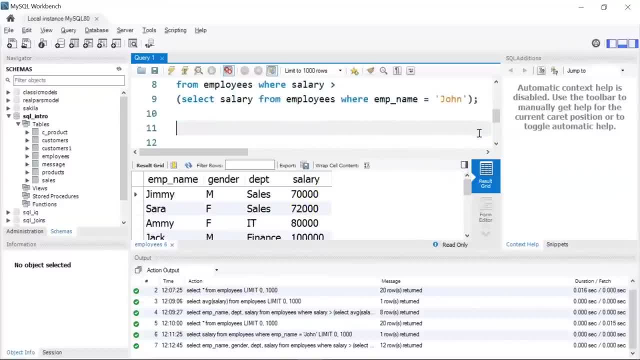 than $67,000. okay, now you can also use sub queries with two different tables. so suppose you want to display some information that are present in two different tables. you can use sub queries to do that. so for this example, we'll use a database that is called classic models. so we'll use a database that is called 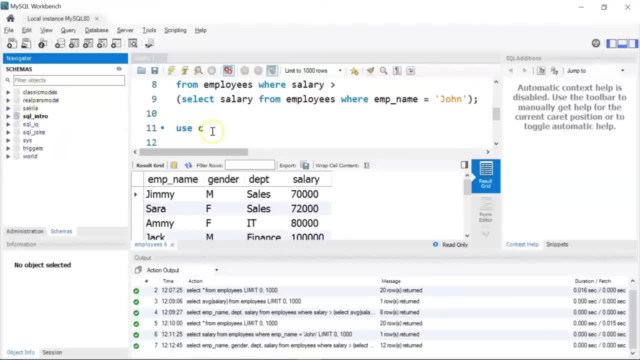 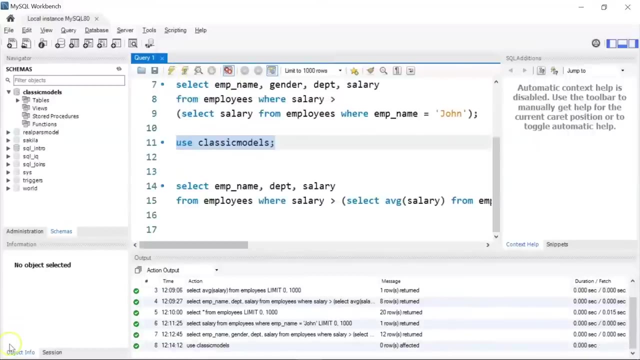 classic models. you can see the first database. so let me use this database called classic models. I'll write: use classic models now. this database was actually downloaded from the internet. there's a very nice website. I'll just show you the website name. so this is the website. that is my sequel tutorial dot. 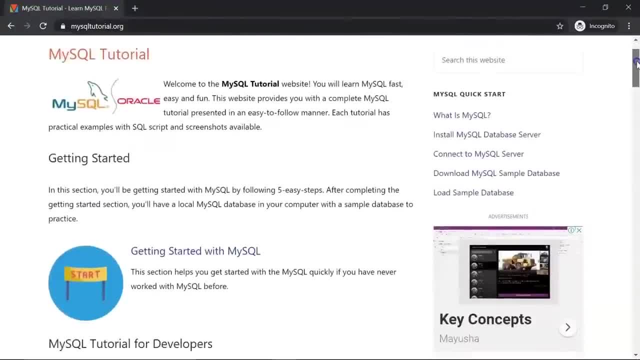 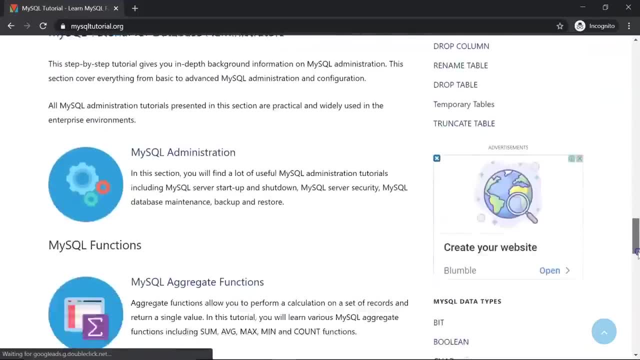 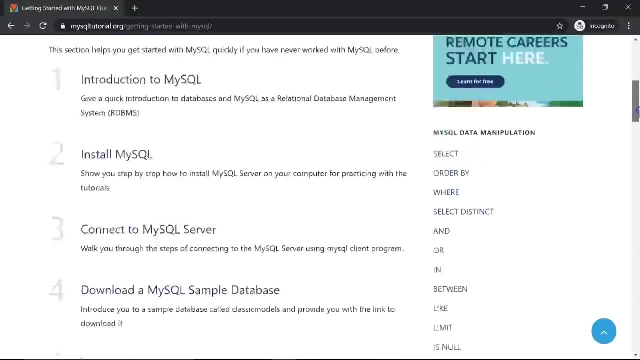 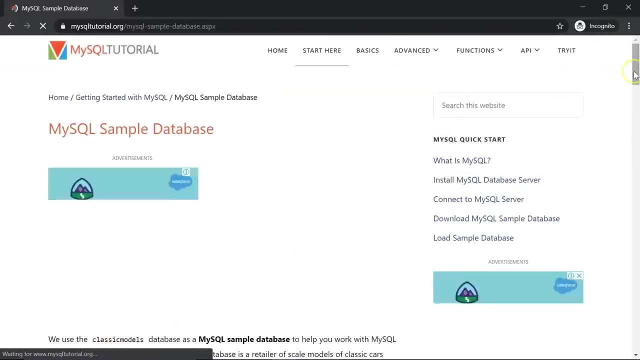 o-r-g. you can see here they have very nice articles, blogs from very many people, and then the second one is classic models. so this is very nice topic where you can learn mysql in detail. so we have downloaded the database that is classic models from this website. you see here they have a mysql sample database if you click on. 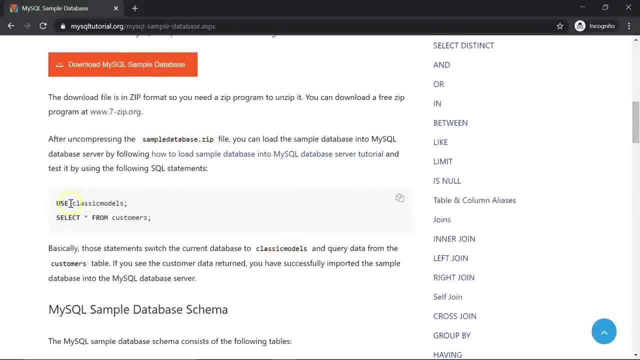 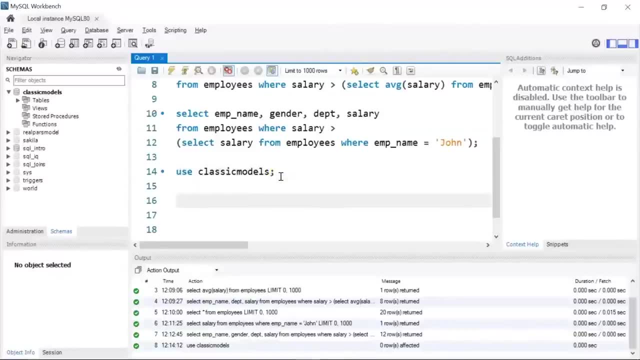 this it will take you to the link where you can download the database. so they have this download link which says download mysql sample database and the database throughout our demo session. if I expand the tables section, you can see there are a lot of tables that are present inside this classic models. 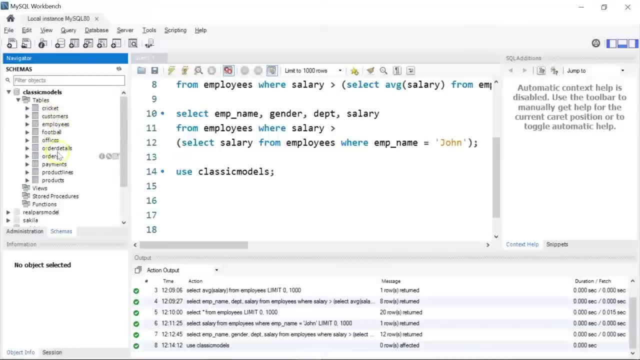 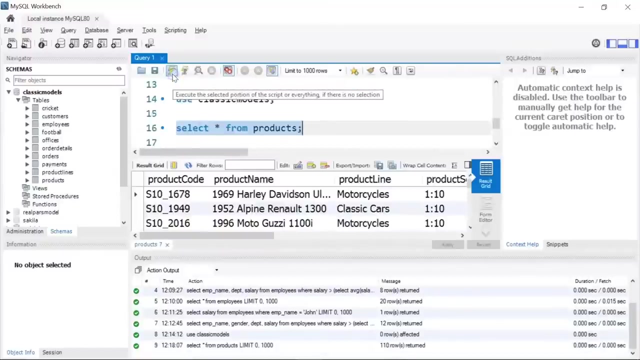 database. we have cricket customers as employees. office is orders, order lines and many more. so for our sub query we'll be using two tables, that is, order details and products table first. let me show you the content that is present inside the products table first. if I run this, you see here it says 110 rows. 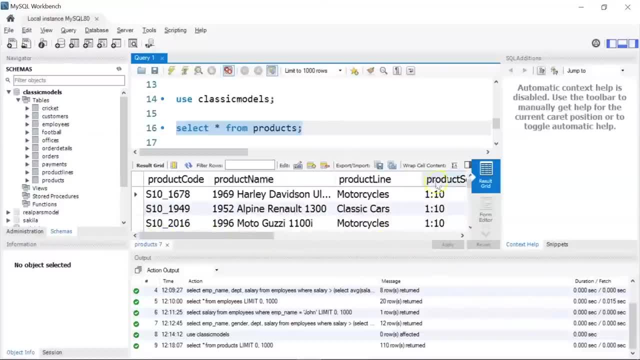 return, which means there are 110 different products that are present in our table, which has the product code, the product name, product line. we have the product vendor description: quantity in stock, by price, MSRP. the other table we are going to use is order details, which has the details of all the orders. let me show you the records: order. 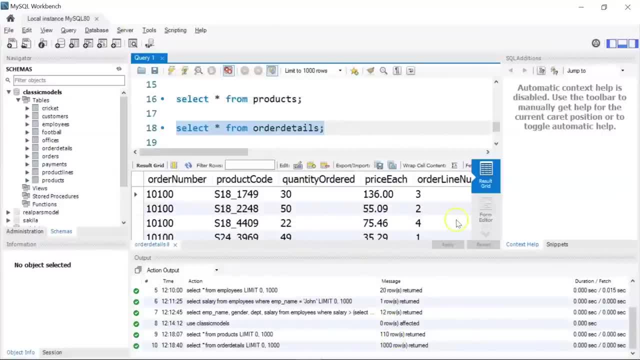 details tables has. okay, so there are thousand records present in this table. you have the order number, the product code, quantity, ordered price of each item. you have the order line number as well. okay, now we want to know the product code, the product name and the MSRP of the products. whose products? 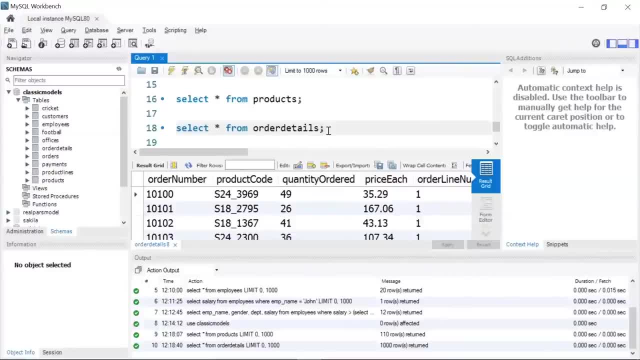 price of each product is less than $100. for this scenario, we are going to use two different tables and we are going to write a sub query. okay, so if you see, here in the order details table, we have a column called price each. I want to display the product code, the product name and the MSRP of the products which 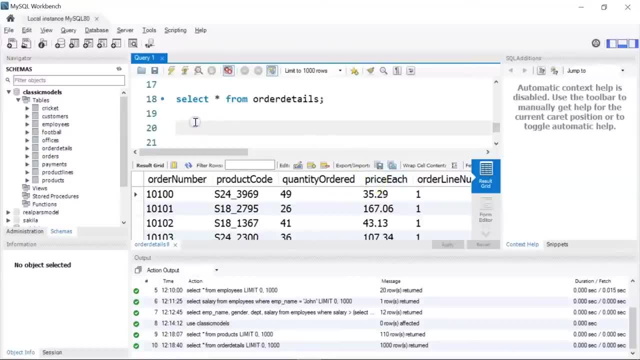 have a price of each product less than $100. so the way I am going to do is I will write select product code, comma, product name. now one thing to remember: that this product name is actually present inside our products table and product code is present in both the tables, that is, products and order. 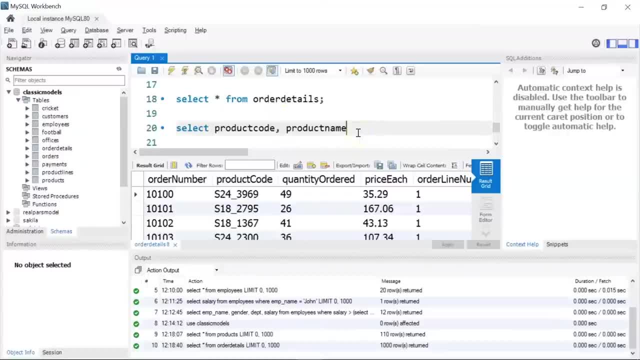 details here you can see. this is the product code, column comma MSRP, which is present inside the products table. again from my table, that is products and order details, where I'll write product code. I'm going to use the in operator. next I'll write my inner query, that is, select product code from my table order. 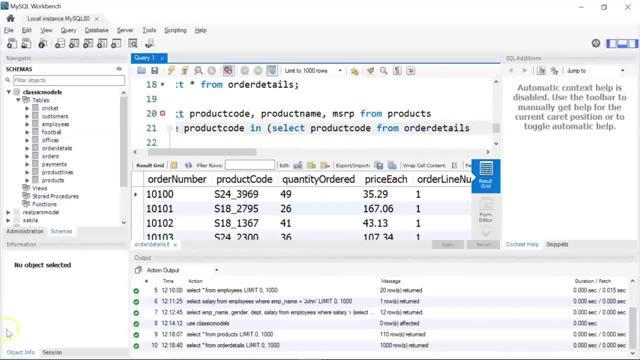 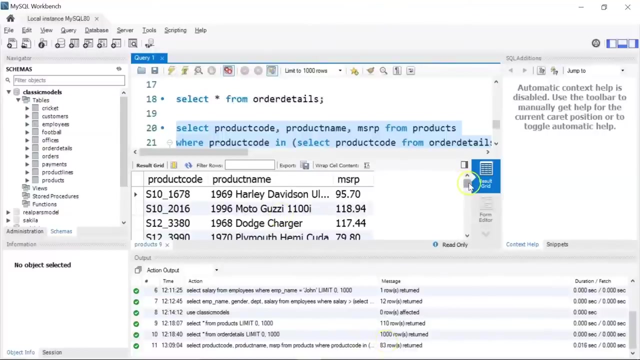 details where my price of each product is is less than $100. let me run this, okay, so you can see. there are total 83 products in our table which have a price less than $100. you can see the price here. okay, now we learn another advanced. 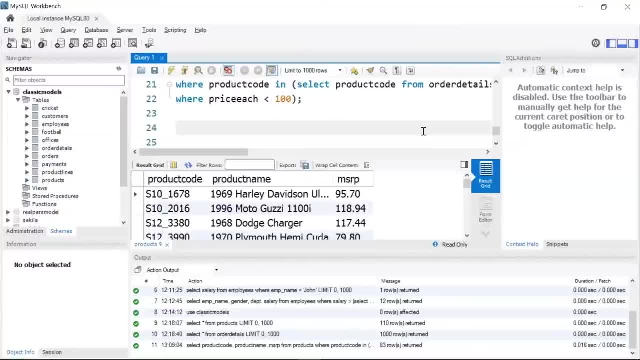 concept in SQL which is known as stored procedures. I'll just give a comment saying stored procedure. okay, so first let's understand what is a stored procedure. a stored procedure is an SQL code that you can save so that the code can be reused over and over again. so if you 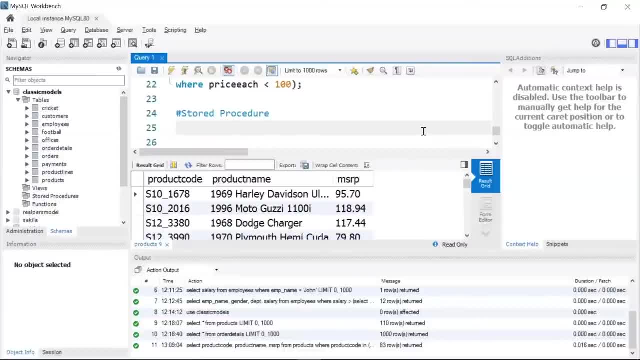 want to write a query over and over again, save it as a stored procedure and then call it to execute it. so in this example, I want to create a stored procedure that will return the list of players who have scored more than six goals in a tournament. so I have a database. 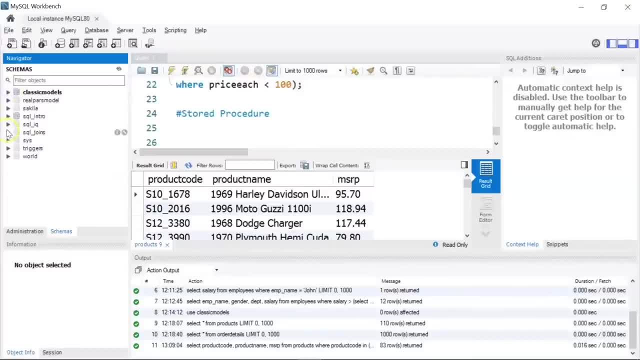 called SQL underscore IQ. these are a few databases that have already created. this database has a table called players. if I expand the tables option, you see we have a table called players and you can see the columns: player ID, the name of the player, the country to which the player belongs to. 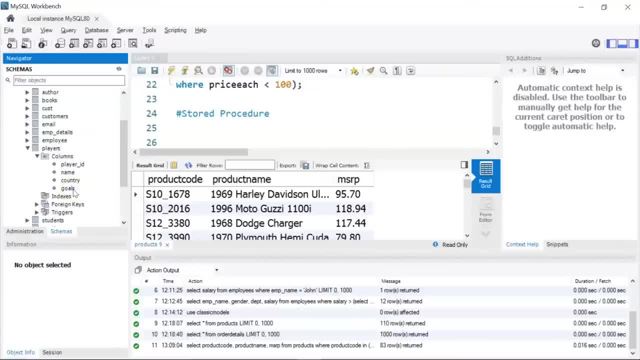 and the number of goals each player has scored in a particular tournament. so I'll write a stored procedure that will return the list of top players who have scored more than six goals in a tournament. so first of all, let me begin by using my SQL underscore. IQ database will run it. so now we are. 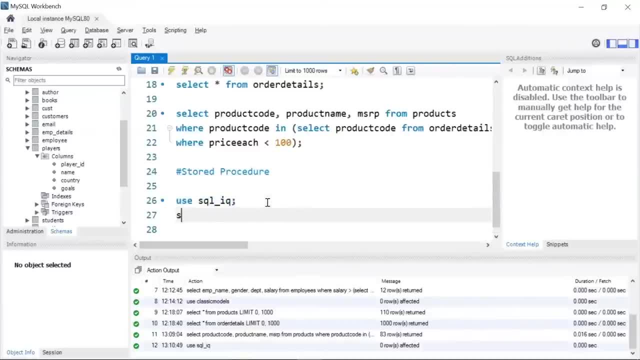 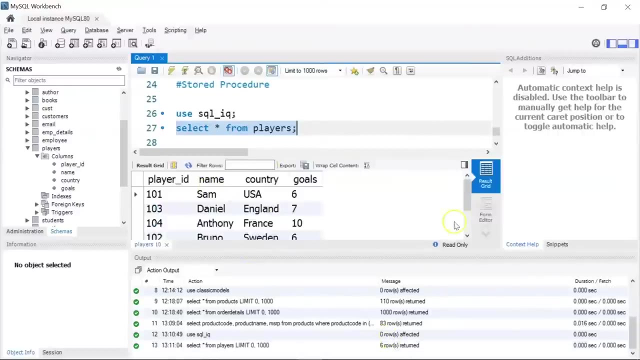 inside the SQL underscore IQ database. let me select star from players to show the values that we have in the players table. you can see there are six players in our table. we have the player ID, the names of the players, the country to which these players belong to and the 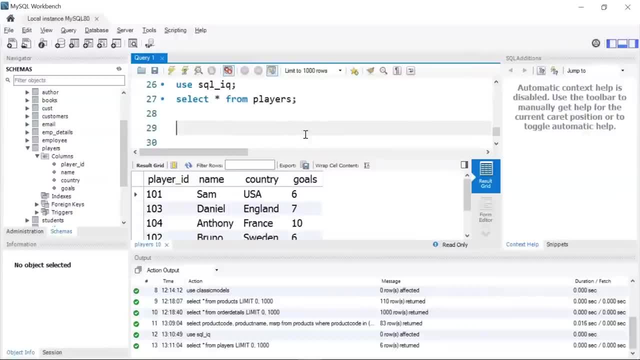 goals they have scored. so I'll write a stored procedure. so the stored procedure syntax is something like this: it should start with a delimiter. okay, in the delimiter I'll write && next I'll write create procedure, followed by the procedure name. let's say, I want to name my procedure as top. 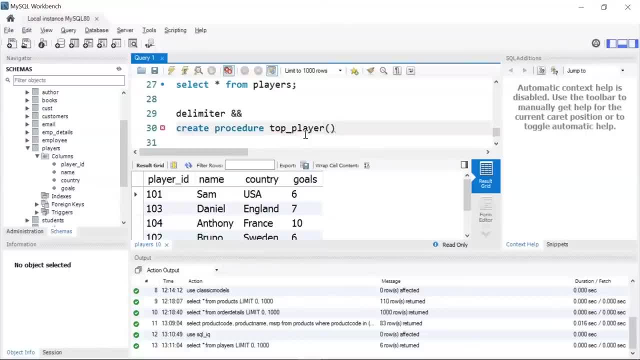 underscore players. next statement is begin. after begin, I'll write my select statement. I want to select the name of the player, the country and the goals each player has scored. from my table, that is players where I'll write goals- is greater than six, we'll give a semicolon. then I'll end my procedure with a delimiter. that was 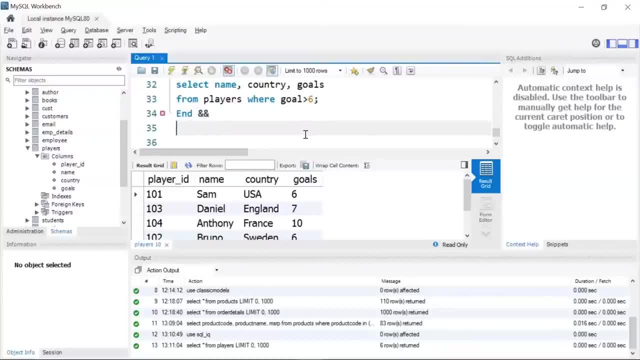 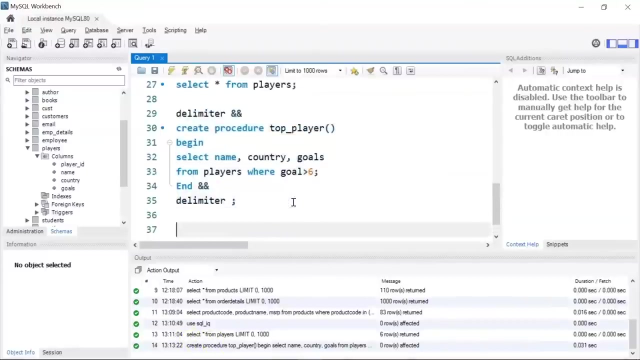 double ampersand. next I'll write delimiter and give a semicolon. now the semicolon suggests this is a default delimiter and there should be a space. okay, now let's run our stored procedure. there you go. so you have successfully created our stored procedure. now the way to run a stored. 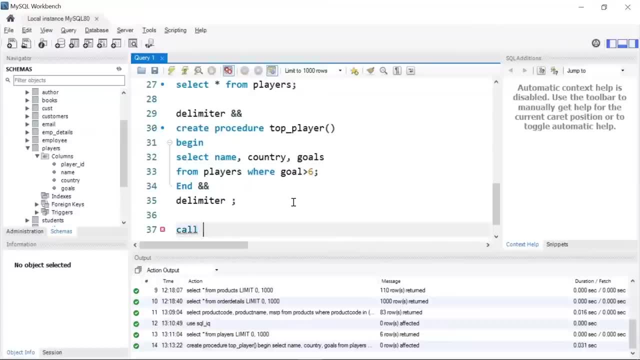 procedure is. you need to use the call method and give the procedure name, that is, top underscore players, in our case, with brackets and a semicolon. let's execute it okay. there is some problem here, so we made a mistake while creating a procedure. the name of the column is: 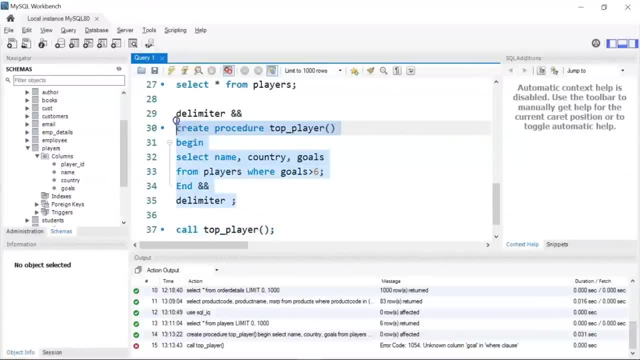 goals and not goal. let me create that procedure again. okay, it says the procedure top underscore player already exists. let's just edit the procedure: name instead of top player, we'll write it as top players and similarly we'll edit here as well. now let's create it again. okay, now to call my procedure. i'll write: call. 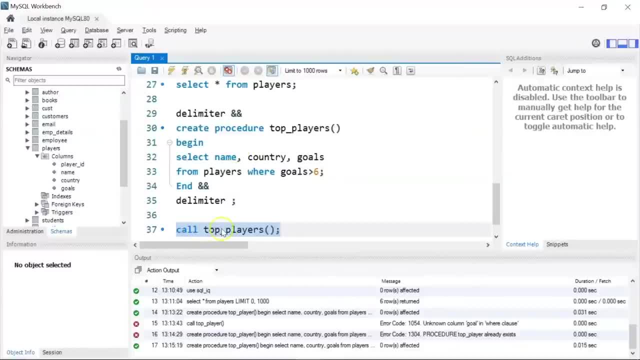 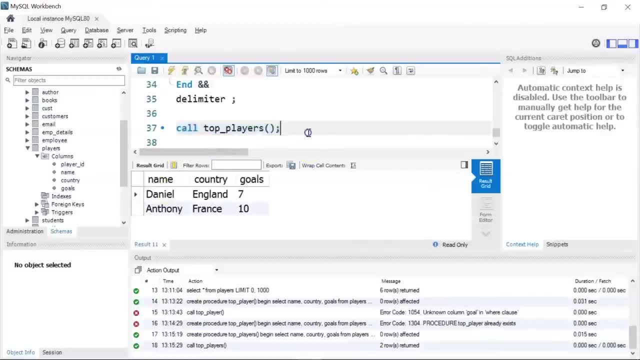 space followed by the procedure name, which is top underscore players. if i run this, you can see we have two players in our table who have scored more than six goals, so we consider them as the top players in a particular tournament. all right, now there are other methods that you can use while 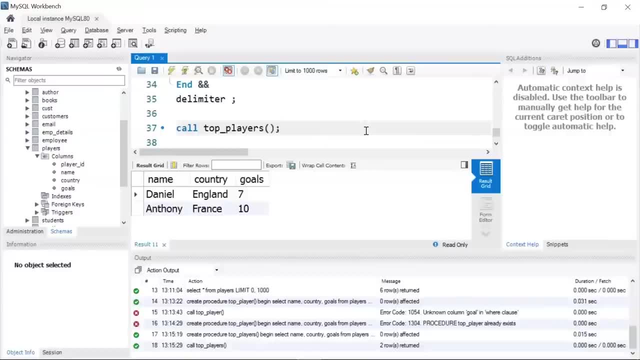 creating a stored procedure. one of the methods is by using an in parameter. so when you define an in parameter inside a stored procedure, the calling program has to pass an argument to the stored procedure. so i'll give a comment: stored procedure using in parameter. all right, so for this example, i'll create a procedure that will fetch or display. 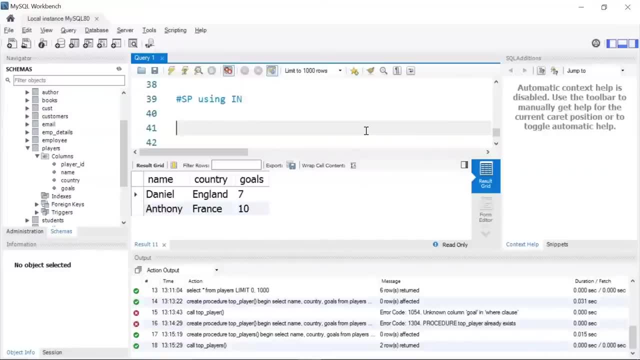 the top records of employees based on their salaries. so we have a table in our sql underscore iq database which is called employee details. i'm going to use this table. you can see. we have the name of the employee, the age, sex, then we have the date of join city and salary. 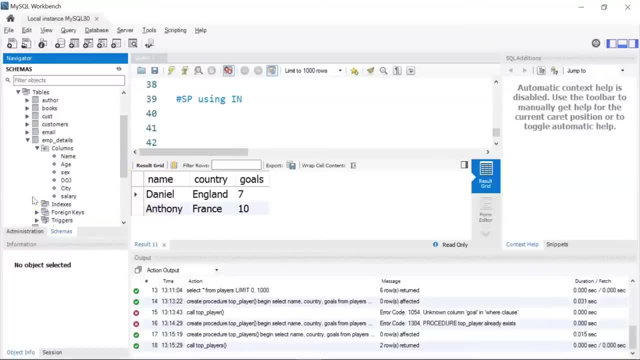 using this table, i'll create a procedure that will fetch or display the top records of employees based on their salaries, and we'll use the in parameter. so let me show you how to do it. i'll write delimiter- this time i'm going to use forward slash. i'll write create procedure. 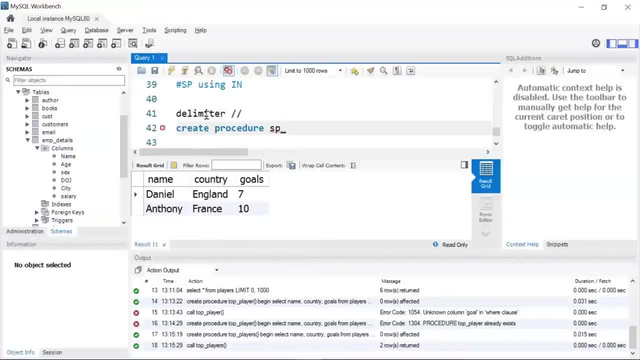 followed by the procedure name, let's say sp for stored procedure. sort by salary is the name of my employee and inside this procedure i'll give my parameter in. i'll create a variable, var, and assign a data type, integer. then i'll write begin, followed by my select statement where. 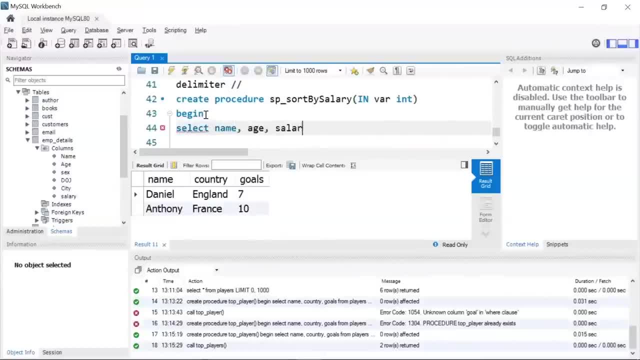 i'll select the name age salary from my table name, that is, emp details or employee details. i'm going to order this by salary descending and I want to display limited number of records, so I'm using this limit keyword and my variable var, which I created here. I'll end my select statement. 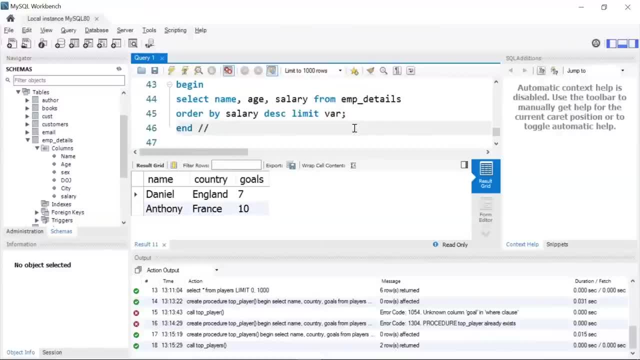 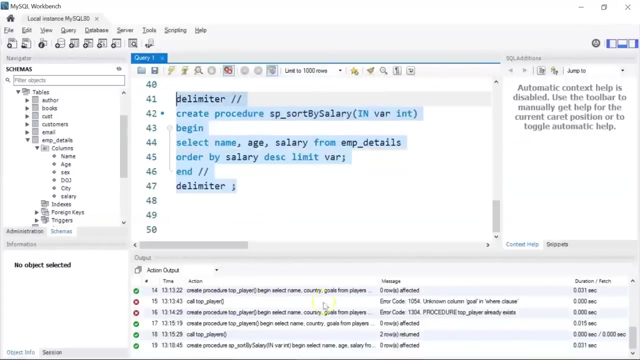 I'll end my stored procedure with forward slash and I'll go back to my default delimiter. that is semicolon. alright, so let me run this. there should be a space here, alright, so let's run this. okay, you can see we have successfully created our second stored procedure, which 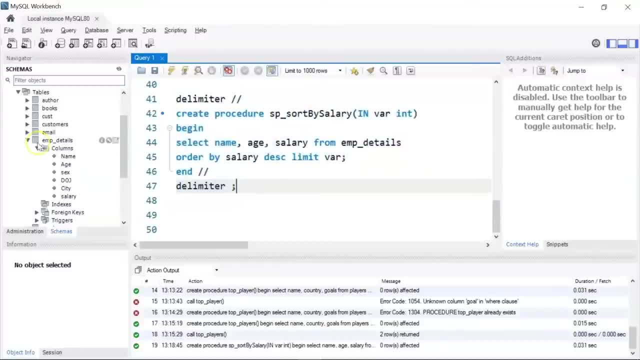 is sp underscore, so let's run this. okay, you can see we have successfully created our second stored procedure, which is sp underscore- sort by salary. now you can also check whether the stored procedure was created or not. here you have an option to see the stored procedures. let me just refresh this and you can see we have three stored procedures that we have created so far. one is sp underscore- sort by salary. the other two were top underscore player and top underscore players. okay, now let's call our stored procedure. 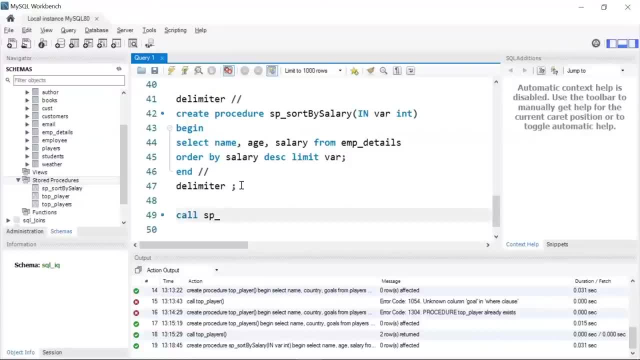 I'll write call space followed by the stored procedure name, which is sp. underscore. sort by salary and inside this I'll give my parameter, which was actually var, and this var we have used in limit. let's say I want to display only the top three records of the employees. 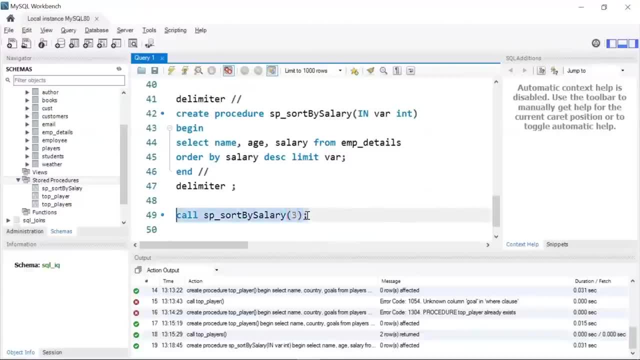 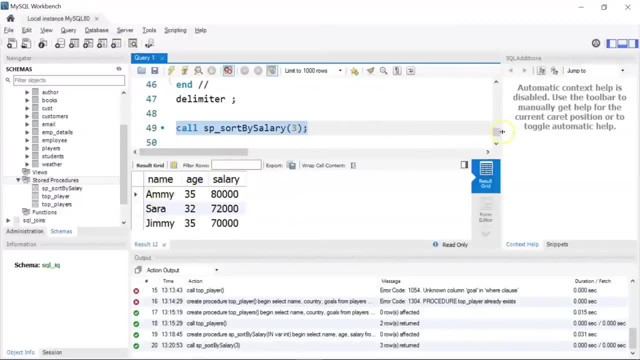 who have the top three highest salaries. okay, so let me run it. there you go so Amy, Sarah and Jimmy, but the top three employees who have the highest salary. so you saw how you could use the in parameter in a stored procedure. we created a variable and that variable we 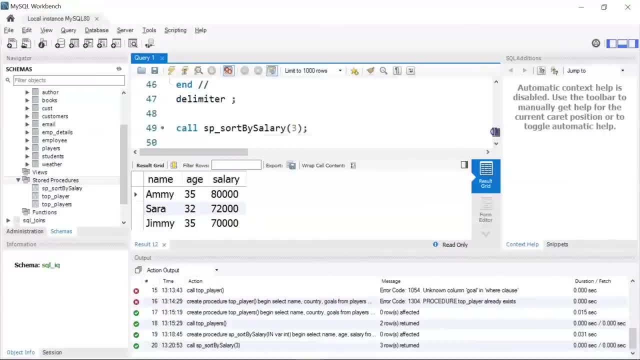 used in our select statement and we called our stored procedure and passed in that variable. okay, now, instead of a select statement inside a stored procedure, you can also use other statements. let's say update. so I'll create a stored procedure to update the salary of a particular employee. so in 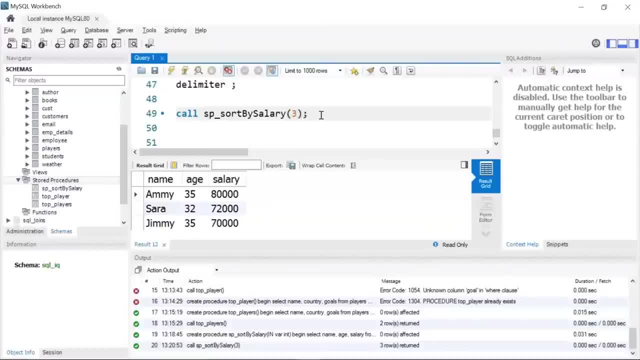 this procedure. instead of select statement, we'll use the update command. in this example, we'll use the in operator twice. so let me show you how to do it. I'll write my delimiter first, which is going to be forward slash, then I'll write create procedure, my name of. 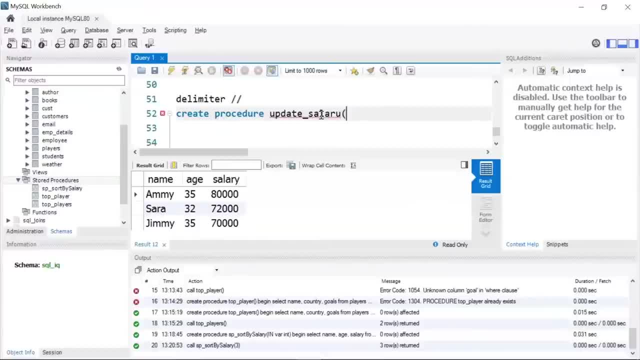 the procedure is going to be update salary and inside the update salary name I'll write in and then temp underscore name, which will be a temporary name variable, and the type I'll assign is varkar 20. I'll again use my in parameter. I'll write in next my 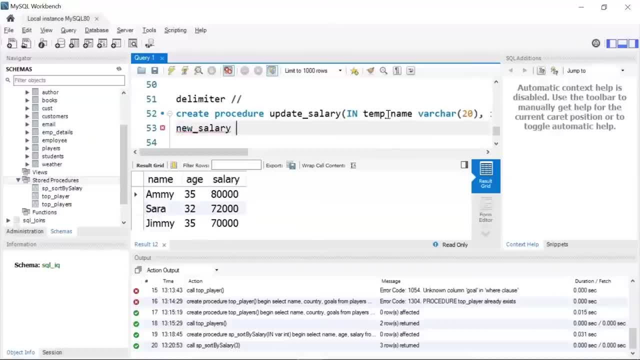 other variable would be new underscore salary and the data type would be float. I'll write begin and write my update command or update statement. I'll write update table name. that is employed details. set salary equal to new undaque oh salaried pya name is equal to my. 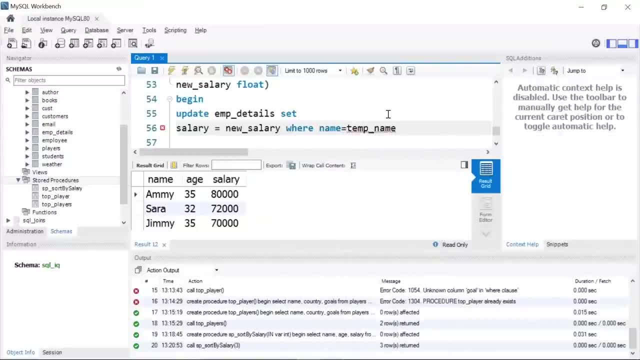 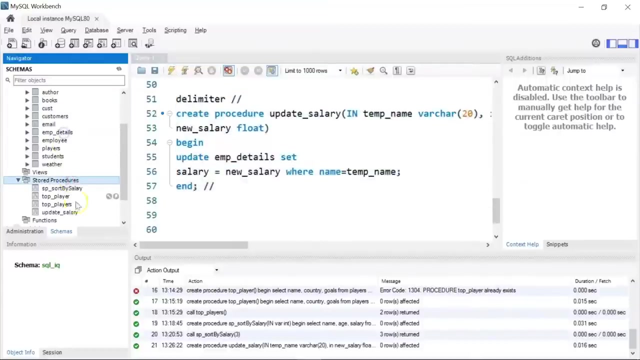 temporary variable, that is temp underscore name. so this is my temporary update command and I'll end the delimiter. alright, so let's run this. okay, we have successfully created our stored procedure. if I refresh this, you can see I have my stored procedure: update underscore salary. okay, now let's say: 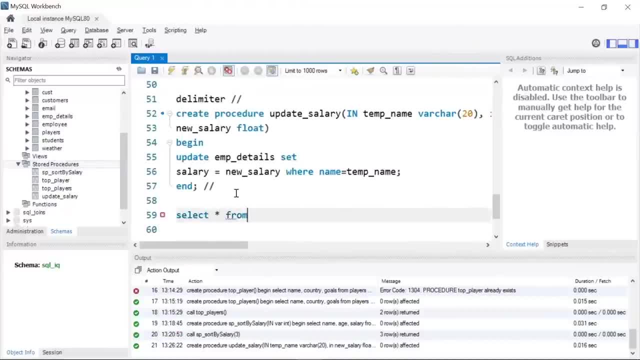 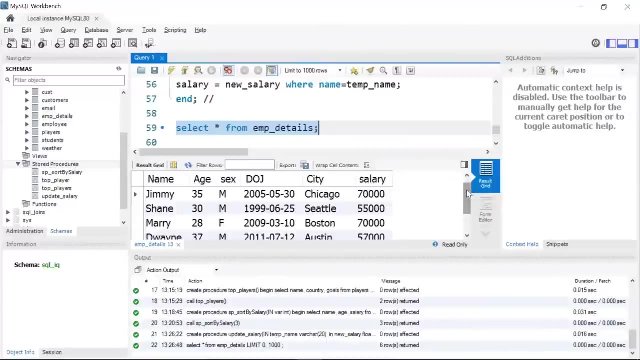 first of all I'll display my records that are present inside employee underscore details table. okay, so we have six rows of information. let's say you want to update the salary of employee Jimmy, or let's say Mary, from 70,000 to let's say 72,000, or let's say 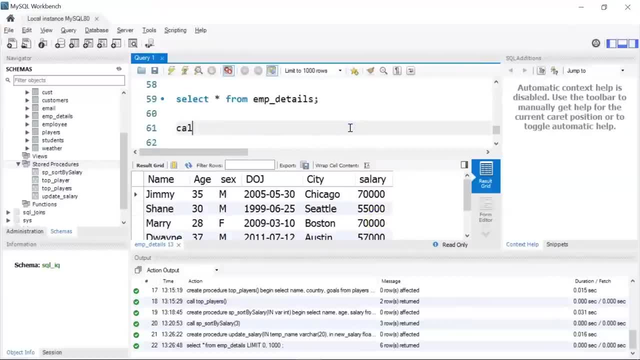 80,000, or let's say 70,000, or let's say 80,000, or let's say 80,000, or let's say 80,000. so I'll call my stored procedure, that is, update underscore salary, and this time I'm going to pass in two parameters. the first parameter will be: 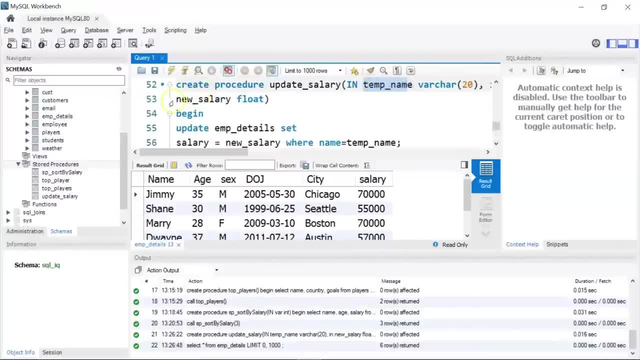 the employee name and next, with a comma, I'll give my new salary that I want to. so my employee name, let's say, is Mary, and the salary I want is to be updated is, let's say, $80,000. I give a semicolon and I'll run it. you can see it says one row affected. now let's check our table once again. 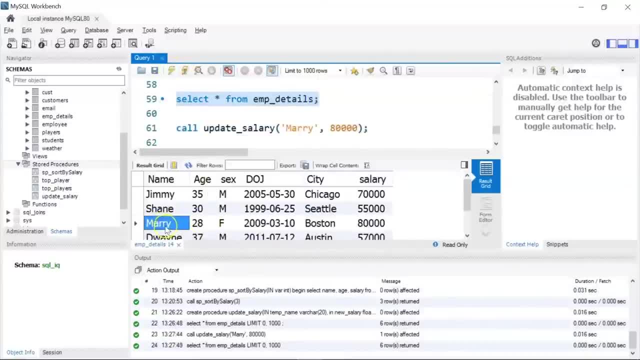 there you go, if you see this record for Mary, we have successfully updated the salary to 80,000 moving ahead. we learn to create a stored procedure using the Out parameter, so i will give a nu 같아요 out parameter, so i'll give a new salary to eighty thousand dollars for moving ahead. we learn to create a store procedure using the out parameter, so I'll give an nuance up value to a very high. 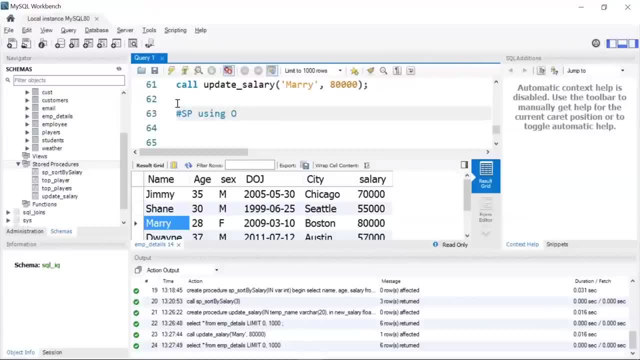 comment. stored procedure using out parameter. okay, so suppose we want to get the count of total female employees. we will create total employees as an output parameter and the data type would be an integer. the count of the female employees is assigned to the output variable, which is total underscore EMPs. 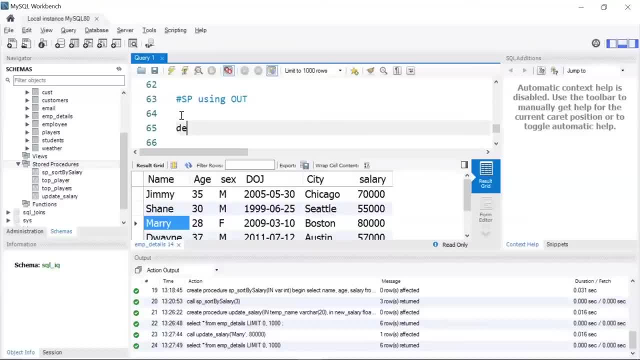 using the into keyword. let me show you how to write a stored procedure using the out parameter. so first I'll declare my delimiter to forward slash. I'll write create procedure followed by the procedure name. it is going to be SP, underscore, count, employees and inside this I am going to give my 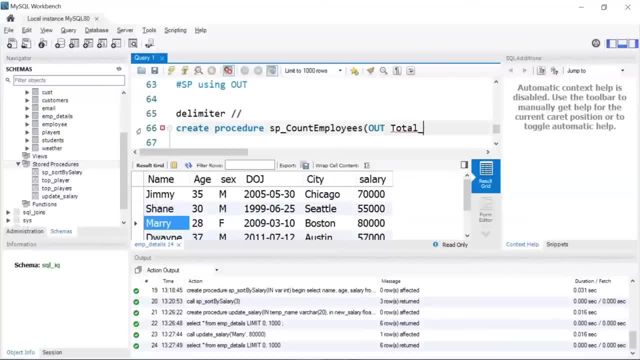 procedure name. it is going to be SP, underscore count employees. and inside this I am going to give my out parameter and the variable name, that is total, underscore EMPs, which is total employees, and the data type will be integer. next I am going to write begin, followed by my select statement, that is select. I want the count of total. 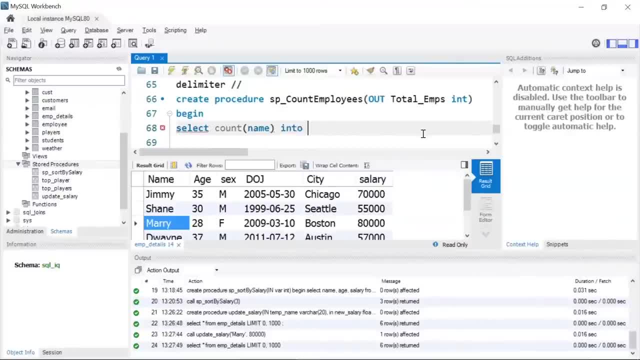 employees and the output. I am going to put into my new variable, that is total underscore, EMPs from my table. that is EMP underscore, again, followed by the detailchart details where sex is equal to F, which means female, I'll give a semi colon, next I'll end it with the delimiter and I'm going to change the delimiter. 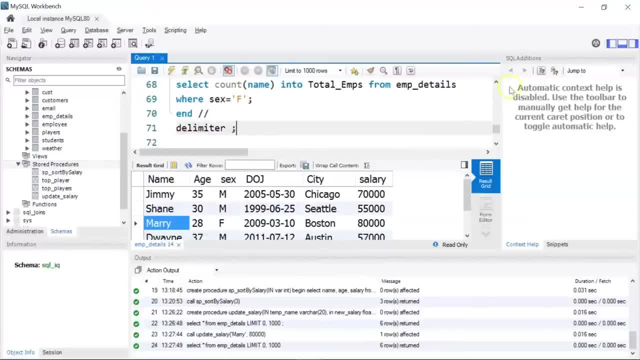 to a default delimiter, that is and다 surat tan Schools, and below I will put a second letter F. I am going to change the delimiter to a default delimiter, that is: 점 is colon. so let me tell you what i am doing here. i am creating a new stored procedure. 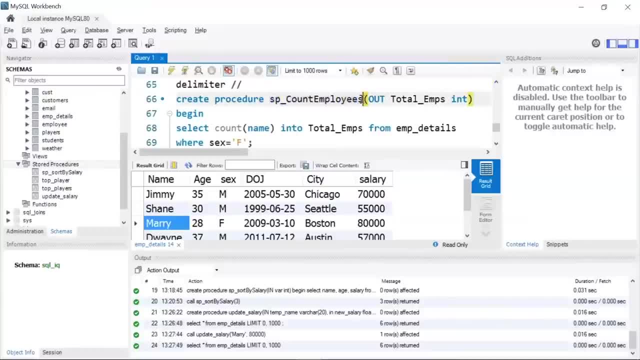 that is, sp underscore count employees. using this stored procedure i am going to count the total number of female employees that are present in our table emp underscore details. so i have used my out parameter and i am creating a new variable called total underscore emps. the data type is integer. here in the select statement i am counting the names of the employees. 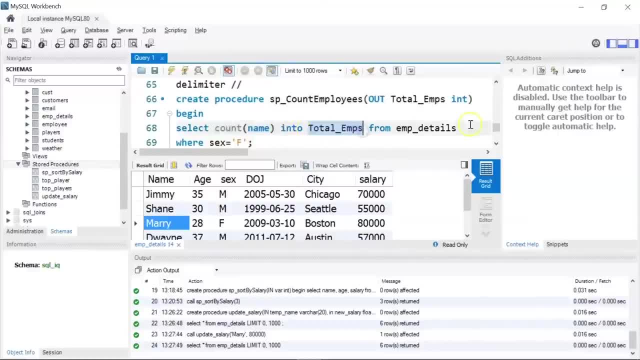 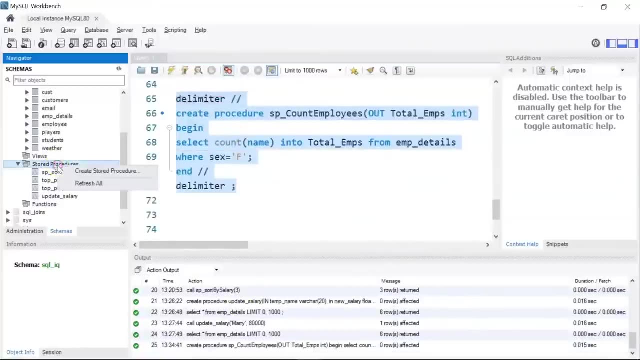 and the result. i am storing it in total underscore emps. i have used my where condition where the gender or the sex is female, so let's run this, okay. so we have created our stored procedure. let's refresh this. okay, you can see we have our new stored procedure: sp underscore count employees. now to call it. i'll write call. 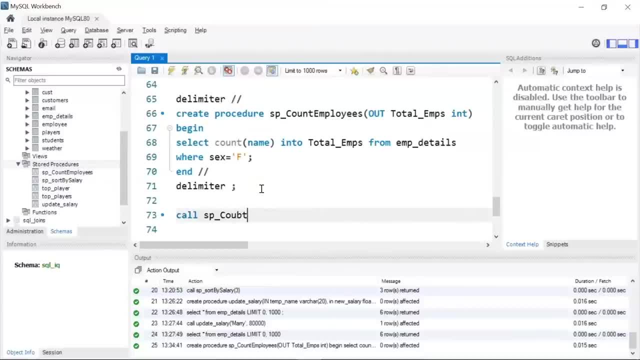 the name of the procedure, that is, count underscore sp. underscore count employees within brackets. i'll pass in the parameter as at the rate f underscore emp. i'll give a semicolon, then i'll write: select at the rate f underscore emp as female employees. okay, so as is an alias name, let's run this one by one. first i'll call my procedure and. 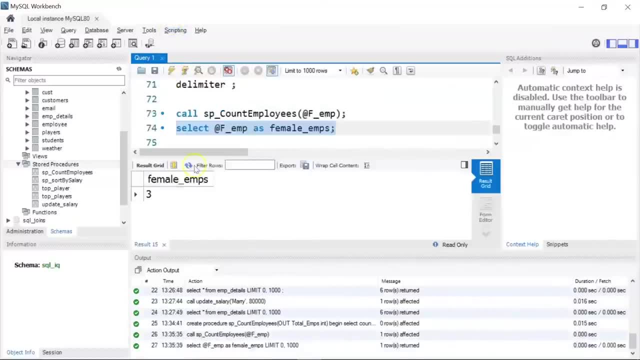 then we'll display the total number of female employees. you can see in our table we have three female employees, all right. now, with this understanding, let's move on to our next topic in this tutorial on advanced sql. now we are going to learn about triggers in sql. 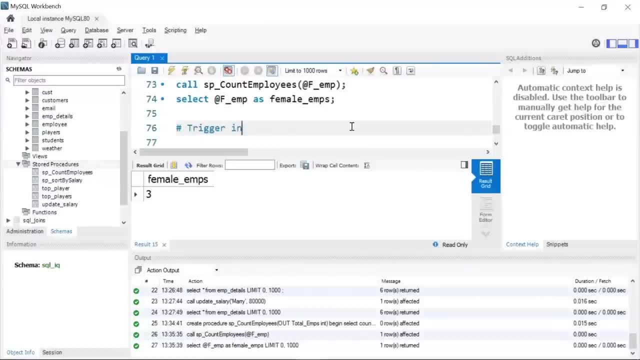 so i'll give a comment here. triggers in sql. so first let's understand what is a trigger. so a trigger is a special type of stored procedure that runs automatically when an event occurs in the database server. there are mainly three types of triggers in sql. we have the data manipulation trigger. 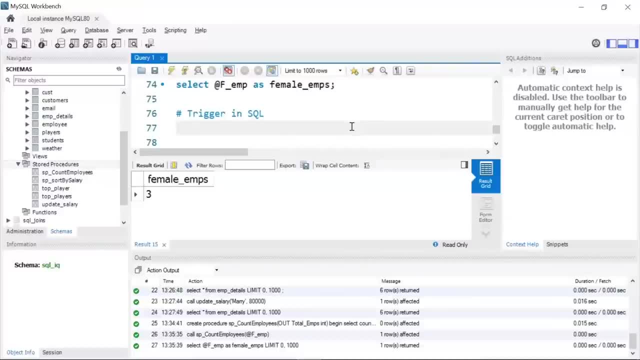 we have the data definition trigger and login triggers. in this example, we learn how to use a before insert trigger. so we will create a simple students table that will have the students role number, the age, the name and the students marks. so, before inserting the records to our table, 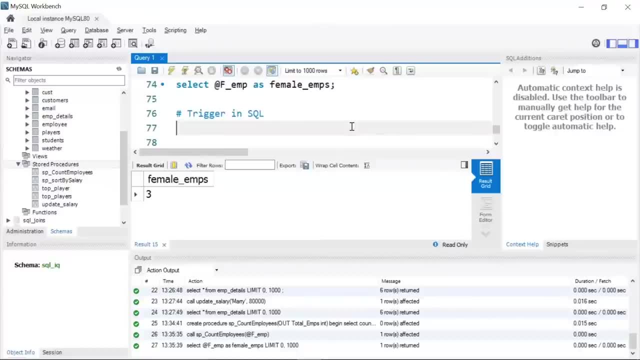 we'll check if the marks are less than zero. so, in case the marks are less than zero, our trigger will automatically set the marks to a random value. let's say 50. so let's go ahead and create our table. that is, students. all right, so i'll write. 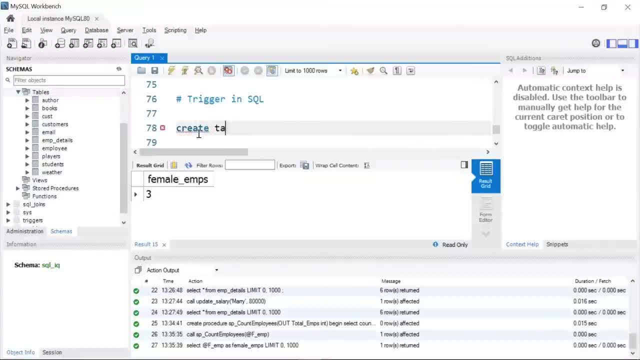 create table: student. now this table will have the student role number. the data type is integer. it will have the age of the students. again, the data type is integer. we have the names of the students, so the third column would be name. audience size. i'm giving it as 30. finally, we have the marks as floating type, so let's create. 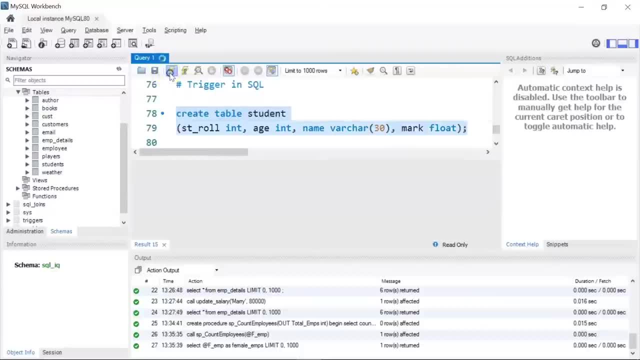 this table, which is student. so we have created our table. now i'll write my trigger command. so trigger command will start with delimiter, like how our usual stored procedures have. you can get this table here in ourıls 환경. next, this time I will write create trigger. then you need to give the name of the trigger. 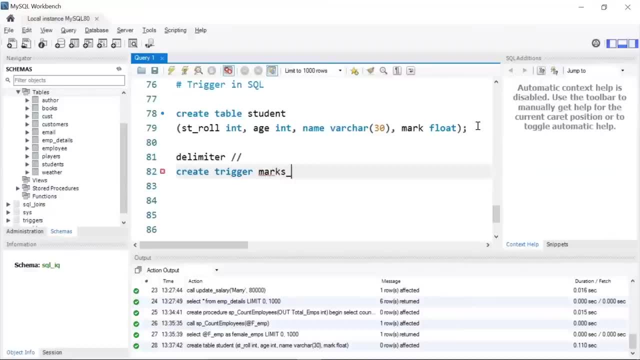 that is mark underscore. let's say verify. I am going to use a before insert trigger so I will write before insert on my table name. that is student. next I will write for each row. if new dot marks is less than 0, then will set new dot marks equal to 50. so this is the 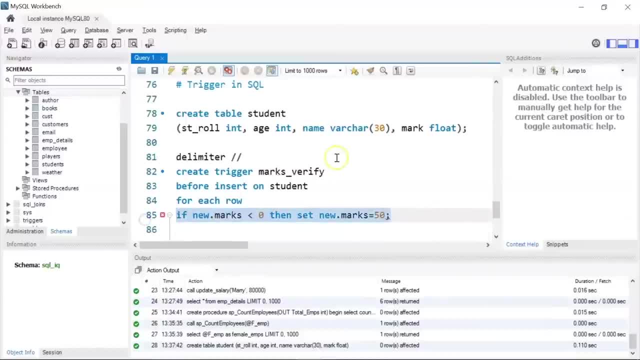 my condition first we will check before inserting. if any student has marks less than 0, will assign a value 50 to that student, because usually the marks are not less than 0 in any exam. I will write end if semicolon and I will close the delimiter. so this is my trigger command. 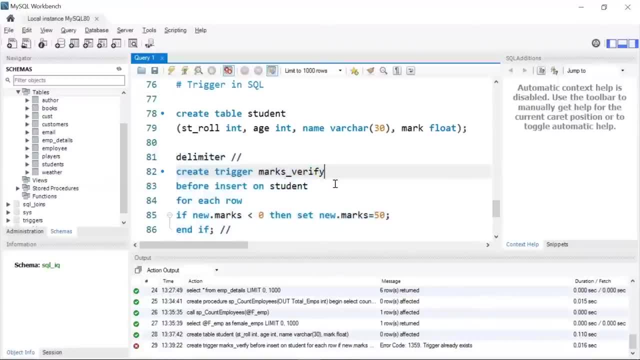 next. in this case we need to update the trigger name. let's say, I will write marks underscore- verify underscore- student for st. let's run it again. ok, there is an error here because in our table the column name is mark and not marks, so here we need to change it as mark. 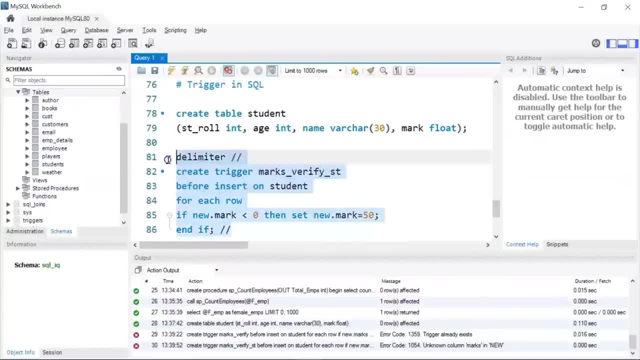 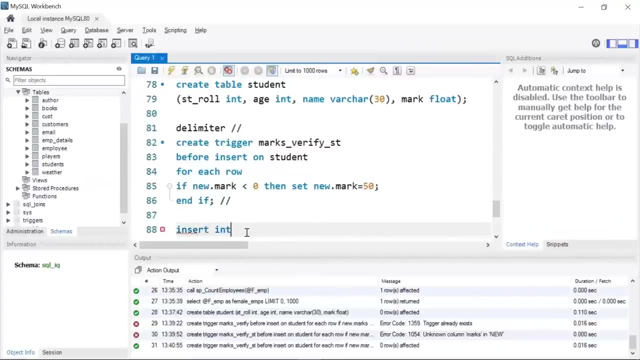 instead of marks already. let's run it. ok, so we have created are trigger. now let me insert few records to the student table. so I'm write: insert into student. I will write values. I will give the values as 501, which is the student roll number, the age passed only. it will give the 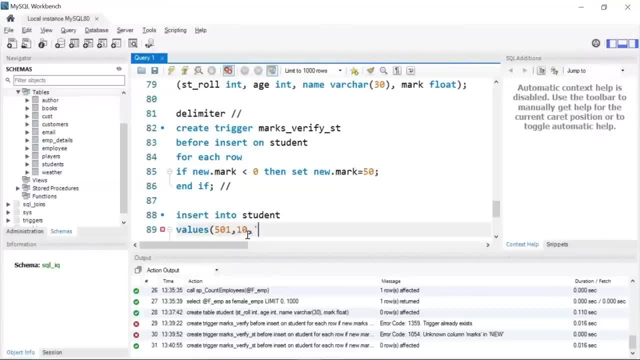 values as 58ato. maximum weight, let's say 10, the name is- it's a Ruth, and the marks is, let's say 75.0. give a comma. we'll insert our second student record. student roll number is 502, age is 12, the name is, let's say Mike, and this time I'm purposely giving a value of. 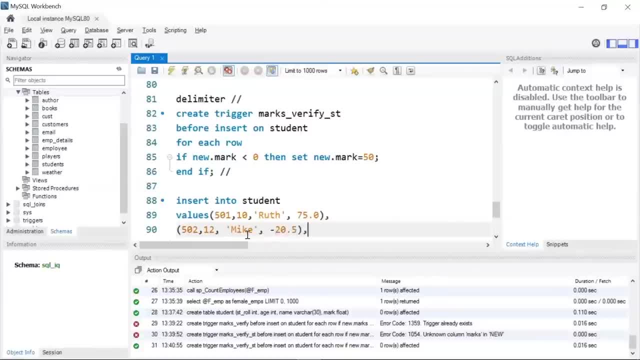 minus 20.5 give another comma. we'll insert the third record for student roll number 503. age is 13, the name is Dave and let's say the marks obtained by Dave is 90. now we'll insert our final record for student number 504. the age is: 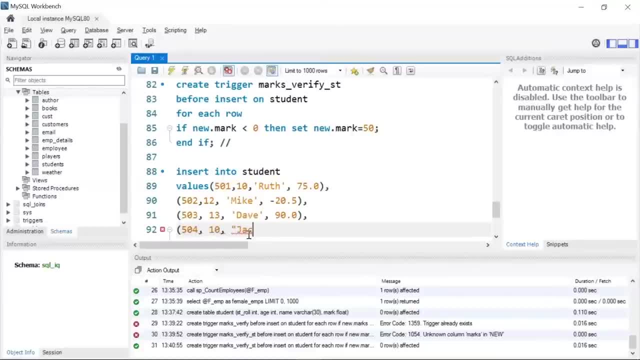 10 name, I'll enter as Jacobs, and this time again I'm purposely giving the marks in negative. 12 point, let's say 5, close the bracket and give a semicolon and I'll run my insert statement. okay, so we have inserted four rows of information to our student table. 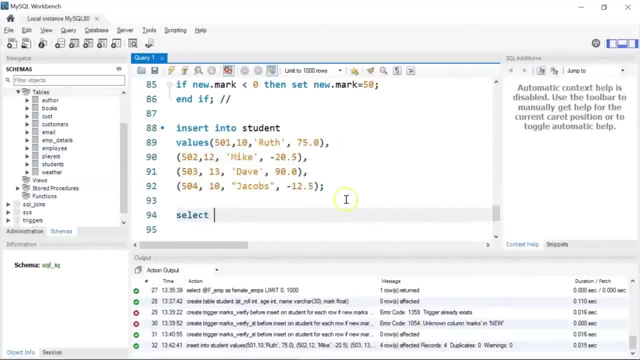 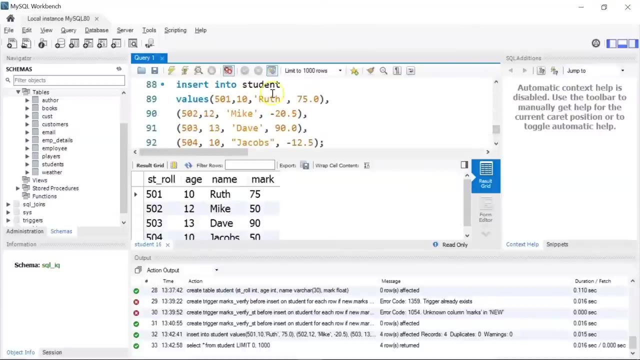 now let me run the select query. I'll write select star from student. if I run this, you see the difference. there you go. so originally we had inserted: for 502 the marks was minus 20.5 and for 504, for Jacobs, the marks was minus 12.5. our trigger: automatically. 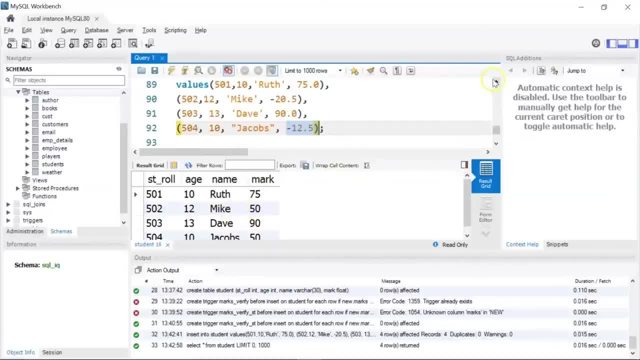 converted the negative marks to 50 because when we created our trigger, we had set our marks to 50 in case the marks were less than 0. so this is how a trigger works. now you can also drop a trigger or delete a trigger. you can just. 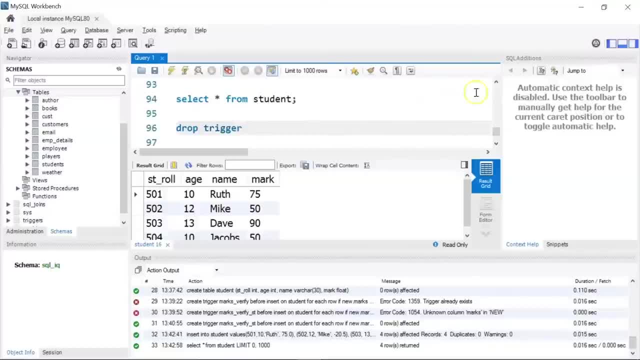 write drop trigger followed by the trigger name. in this case, our trigger name is marks, underscore break pi, underscore st. I'll just paste this here and if you run this, it will automatically delete your trigger. you give this as a comment. okay, now moving on. now we are going to learn. 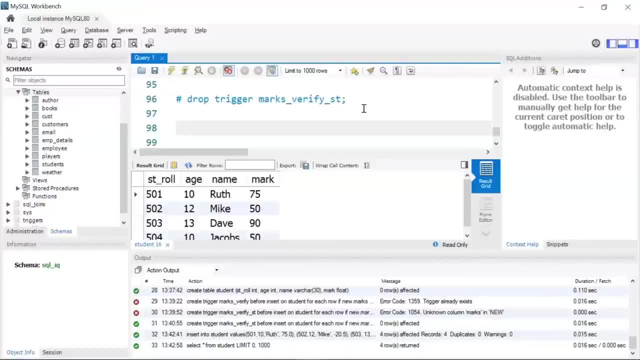 about another crucial concept in SQL which is very widely used. this is known as views. so views are actually virtual tables that do not store any data of their own, but display data stored in other tables. views are created by joining one or more tables. I'll give a comment as views in SQL. okay, now to 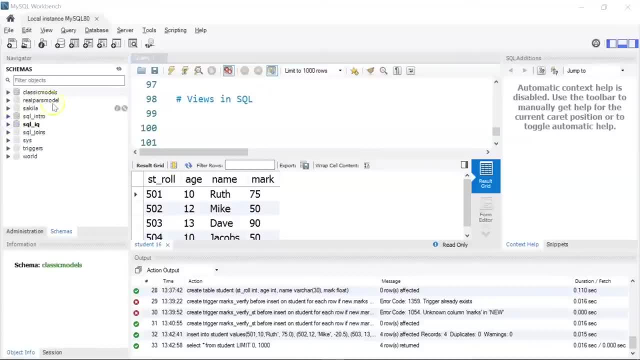 learn views. I am going to use my table, which is present inside classic models database. now, this database, as I mentioned, we had downloaded. we had downloaded it from the internet. so first of all let me write. you use classic models, so I'll switch my database first. all, right, now we are. 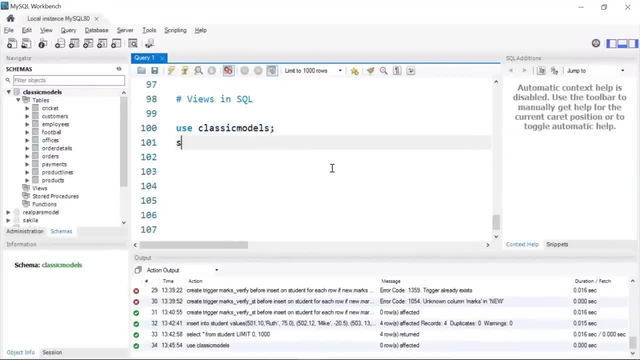 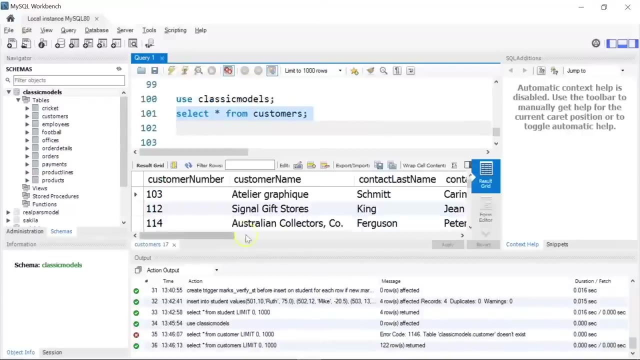 inside classic models. so here let me show you one of the tables which is called customers. so I'll write select star from customers. okay, I missed s here, let's run it again. so this is my customer table, which is present inside classic models database. it has the contact last name, the contact first name, the customer name, customer number. 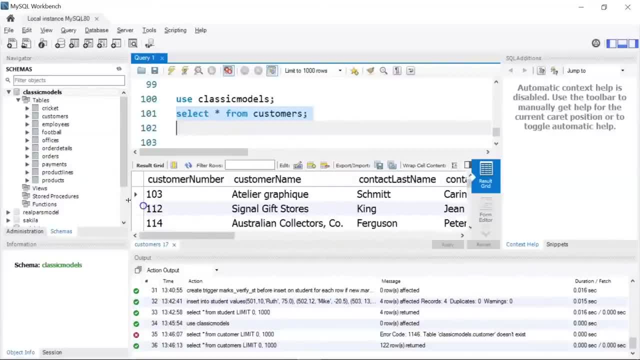 we have the address, state, country and other information. now I'll write a basic view command using this customer table. the way to write is: I'll write create view followed by the view name, which is undercode details. then you write as select as a name. then you write as select a name. 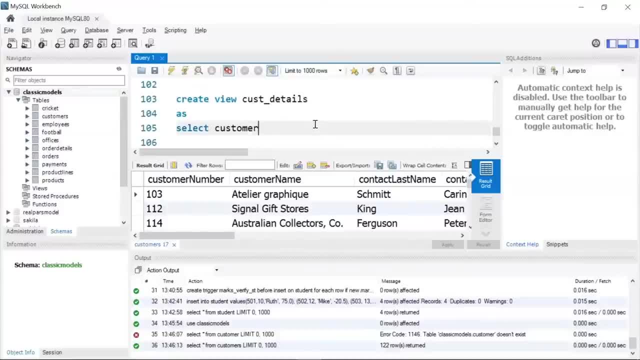 then you write as a name. am going to select a few column names from my original customer table, which is this one. so I need the customer name. let's say I need the phone number and the city. so you have this information here. you have the phone number and the. 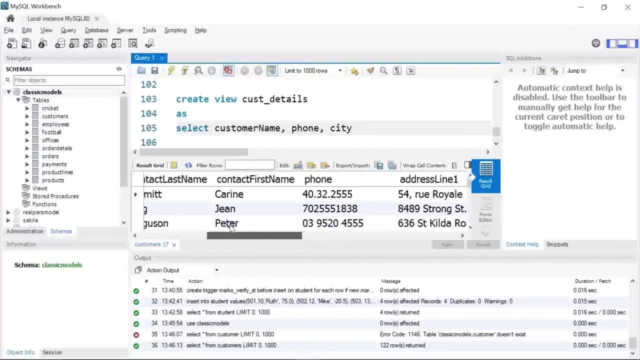 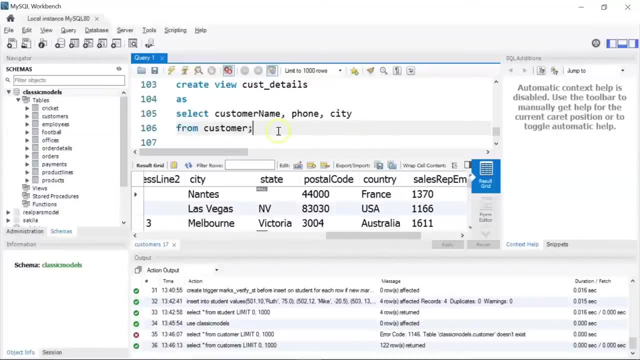 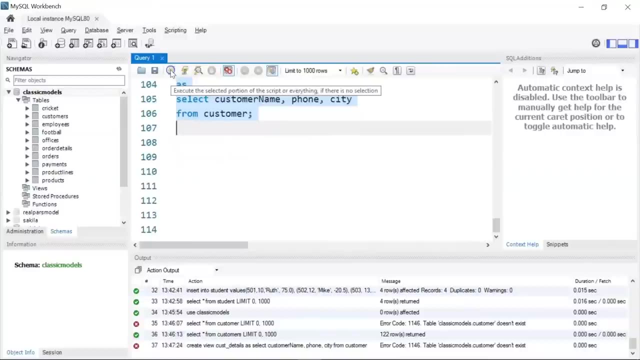 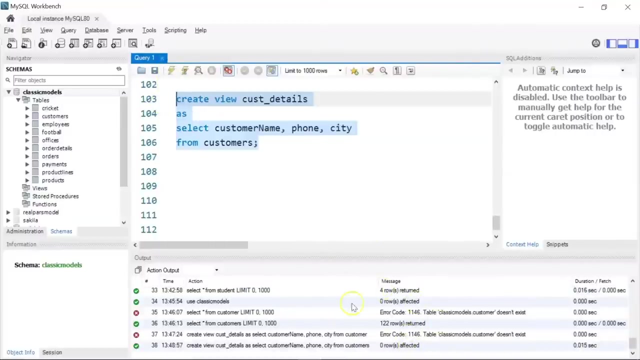 city. all right, I'll write from my table that is customers. if I run this, my view- that is, cust details- will be created. let's run it. there's some error here because the name of the table is customers and not customer. I'll give an S and I'll run it again. all right, so you can see we have created our view and to 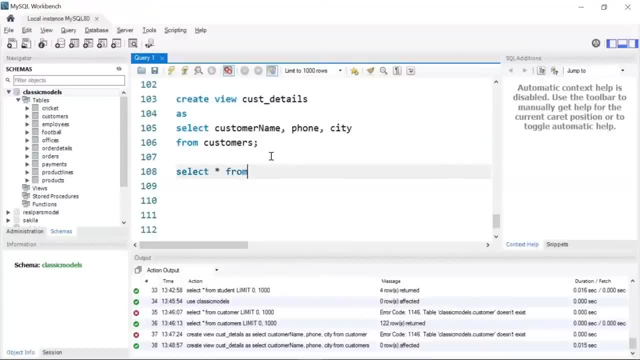 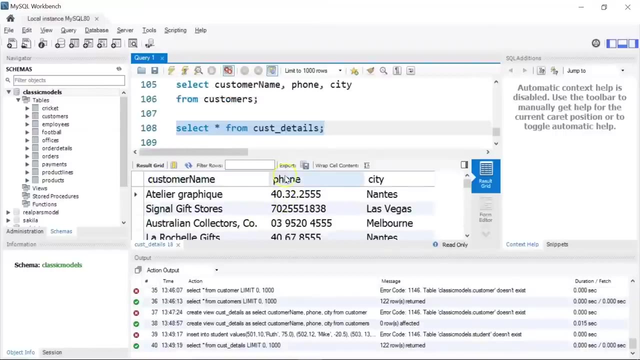 display the contents that are present inside our view. I can write select star form followed by the view name, that is, cust underscore details. let's run it there you go. so we have the customer name, the phone number and the city of the different customers that we have in our table. all right now let's 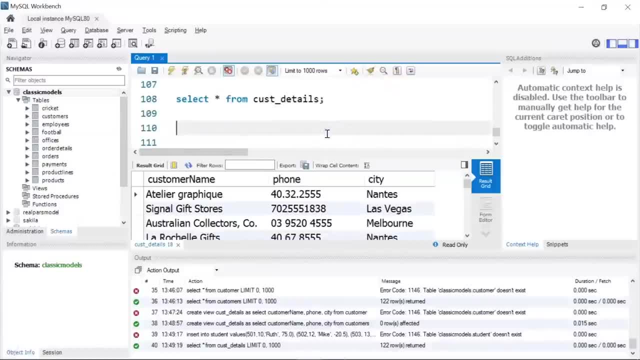 learn how you can create views using joins. so we'll join two different tables and create a view. so for that I am going to use my products table and the products lines table. I'm talking about the products table and the product lines table present inside classic models database. so before I start, let me display the records that 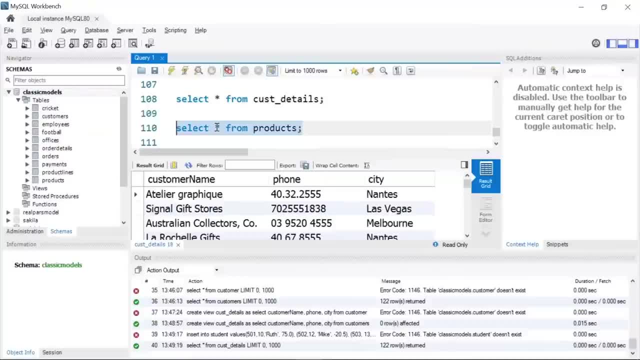 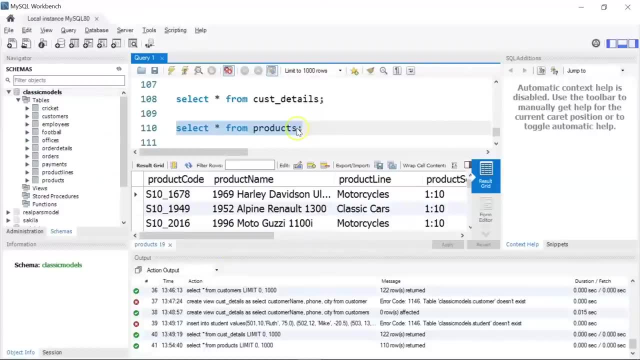 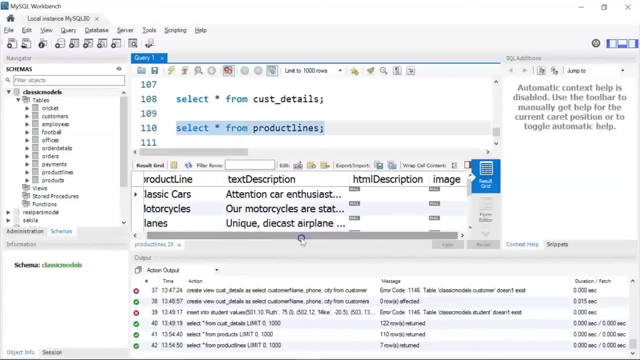 are present inside the products table. let's run it. so these are the different products you can see here. now let's see what we have in product lines table. so we have the product line, the text text description and a some HTML description and image. so I'll create a view by 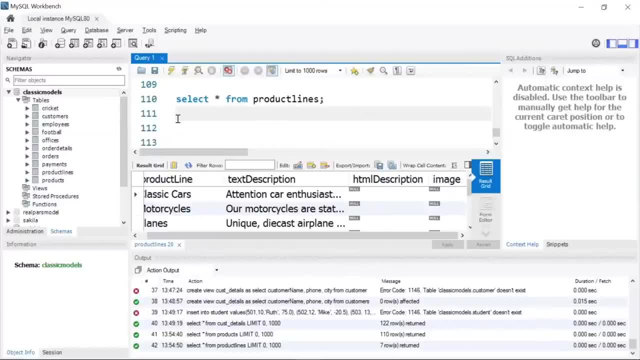 joining these two tables and will fetch specific records that are present in both the tables. so let me first start by writing create view, followed by the view name, that is. product underscore description: as I'll write select product underscore description. product underscore description: as I'll write select product underscore description: as I'll write select. 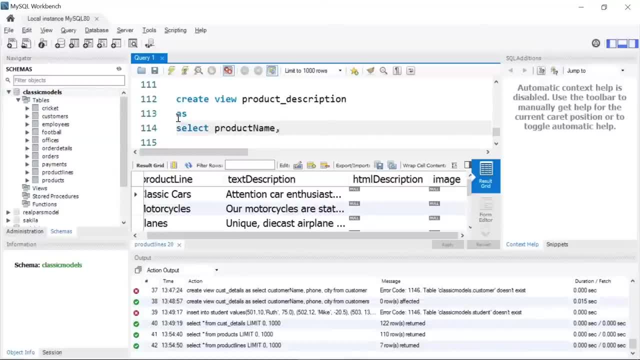 product name comma. then I will write quantity in stock. I also want the MSRP. now these three columns are present inside the products table and next from the product lines table. I want the text description of the products. so I'll write from products table. I'll give an alias. 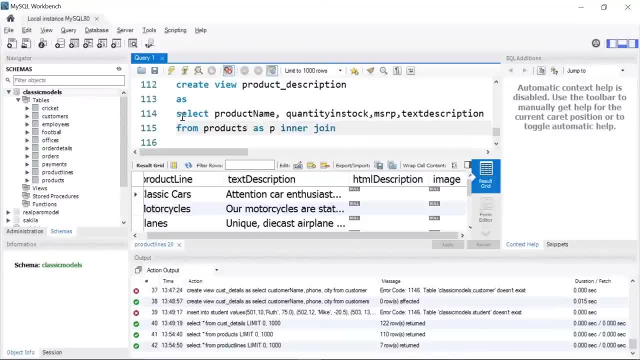 as P followed by inner join. my other table, that is product lines, as let's say PL on the common column that is product line. so P dot product line is equal to- I'll give a space- PL dot product line. okay, so here we have used an inner join. 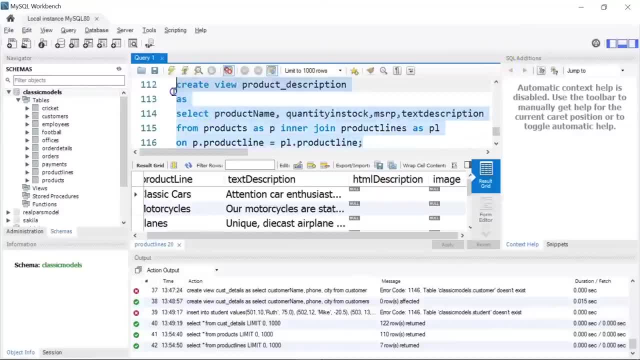 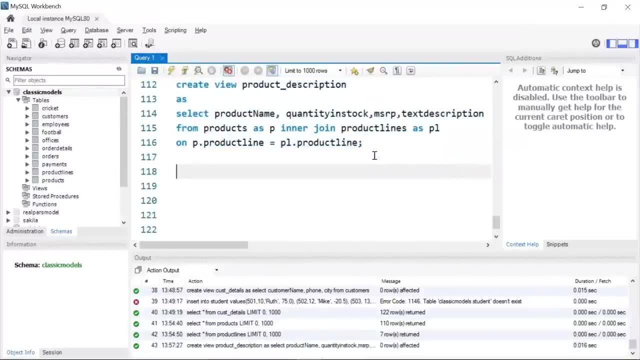 to fetch specific columns from both the tables and our view name is product underscore description. let us run it all right. so we have our view ready. now let me view or display one of the columns from the product table and I will write product underscore description. let us run it all right. so we have our view ready. now let me view or display one of the 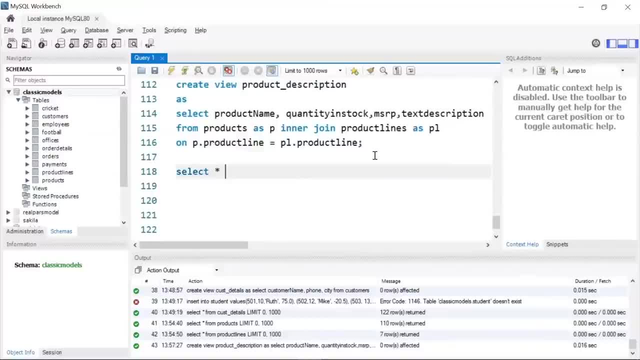 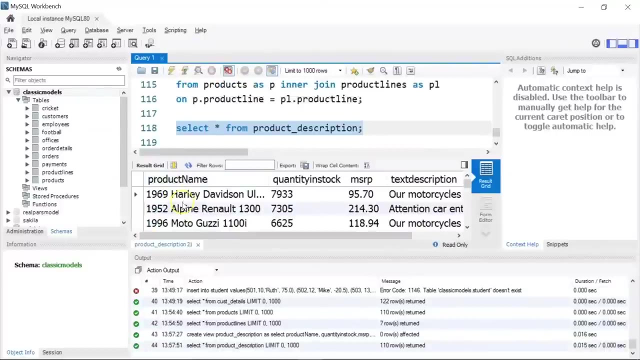 what is present inside our product underscore description view. I'll add select star from product underscore description. let's run it. there you go. so we have the product name, the quantity in stock, MSRP and textual descriptions of the different products in the table. okay, now there are a few other operations that we need to do to get the product name and the quantity in stock. 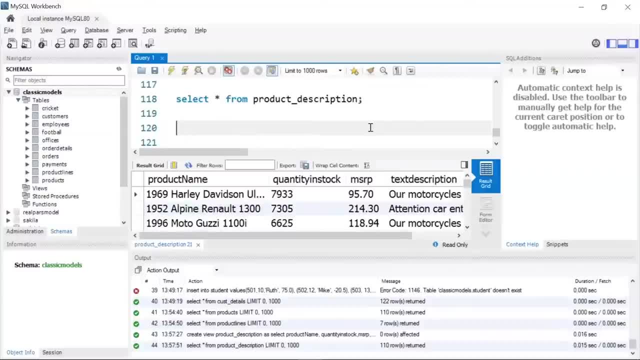 knowledge you can perform. let's say you want to rename a view instead of product underscore description. you want to give some other name, so I'll just give a comment: renamed description. so to rename a description, you can use the rename statement. I'll write: rename table- product underscore description, which is my. 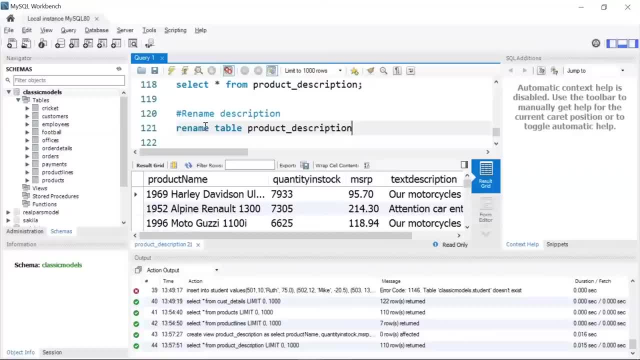 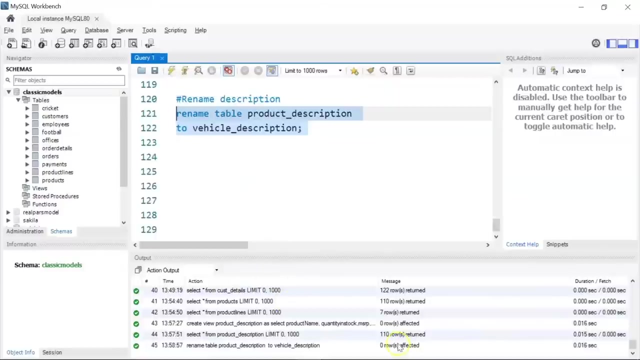 you name. I want to change this name to, let's say, I'll give vehicle description, since all our products are related to some of the other vehicle, so I'll write vehicle description. okay, let us run it all right. so here you can see, have renamed my view, so here, if I, 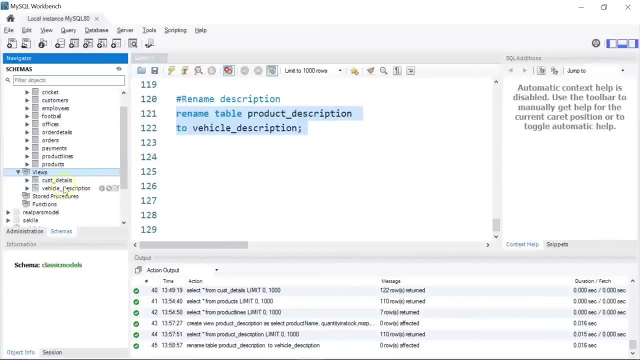 just refresh it and I'll expand this. you can see we have the curse details view and we have the vehicle underscore description view. okay, now either you can view all the views from this panel or you can use a command. let's say I'll write display views. is the comment now to show all the views you can use: show. 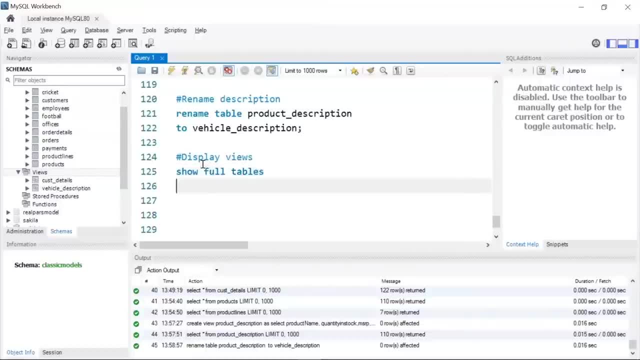 full tables. where table underscore type is equal to within single quote, I'll write view. so this is the command that will display all the views that are present inside a database. there is some error here. let's debug the error. this should be okay. so instead of table types, it should be table type equal to view. 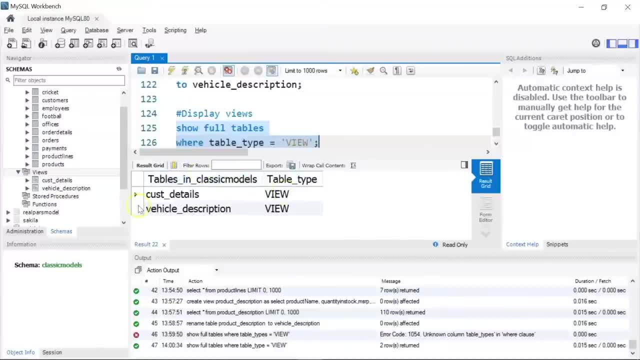 let's run it. you can see the two different views that we have. one is customer details, another is vehicle underscore description. okay, now you can also go ahead and delete a view. for that you can use the drop command. so I'll write drop view followed by the view name. let's say, I want to delete customer. 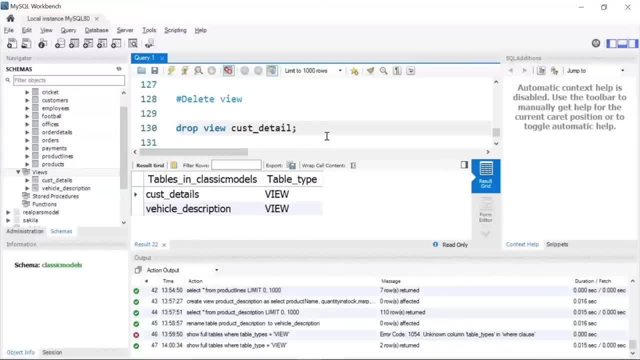 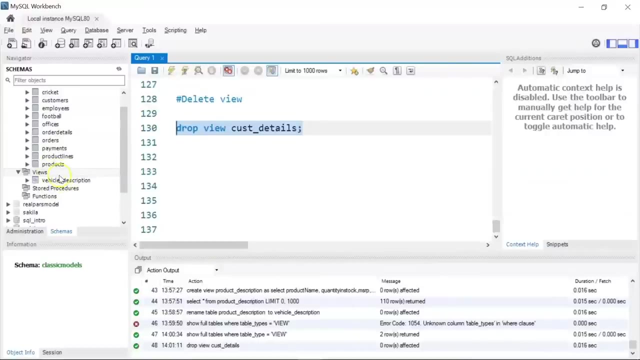 underscore details or customer underscore details view. I'll write: drop view customer underscore details. let's run it. you can see here we don't have the customer underscore details view anymore. all right now, moving to our final section in this demo. here we will learn about Windows functions. 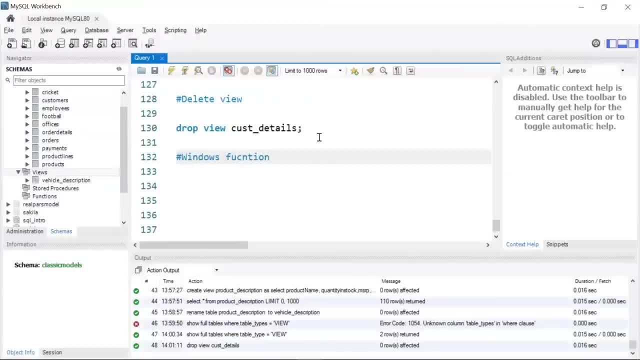 but Windows functions will incorporate it in mySQL in the 8.0 version. so Windows function in mySQL are useful applications in solving analytical problems for using the employees table present inside myACTL underscore intro database. so we will find the total combined salary of the employees for each. 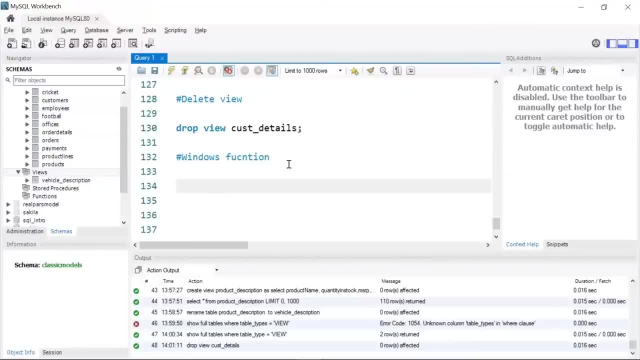 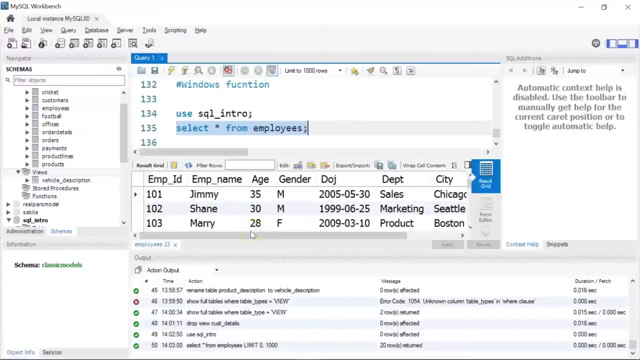 department. so first let me switch my database to sql underscore intro data. I'll run it. okay, I'll display my table. that is employee. so here we have 20 employees in our table. using this table, we are going to find the combined salary of the employees for each department. so we'll partition our table by department. 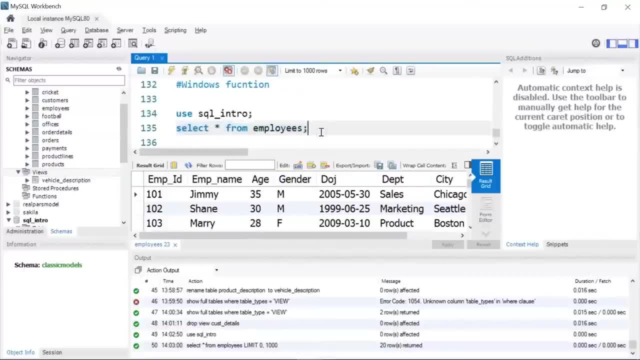 and print the total salary. and this we are going to do using some Windows functions in my sequel. so I'll write select- I want the employee name, the age of the employee and the department of the employee, comma. next I'll write the sum of salary over: I want to partition it by 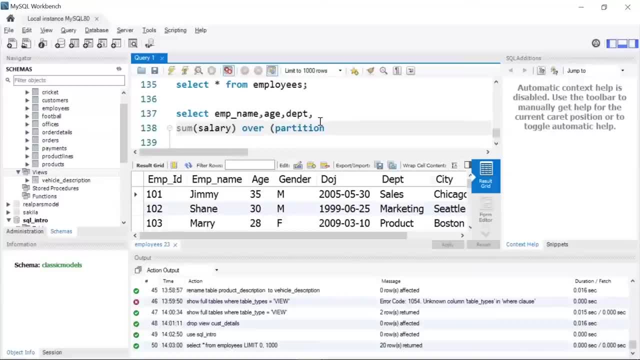 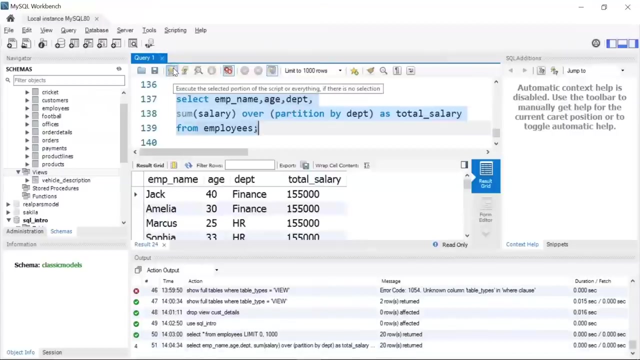 department. so I'll write partition by department, which is DPT, and I'll give an alias as total salary, so that it will create a new column with the name total salary from my table, that is, employees. the output will be a little different this time. let's execute it and see the result. there you go. so here we have. 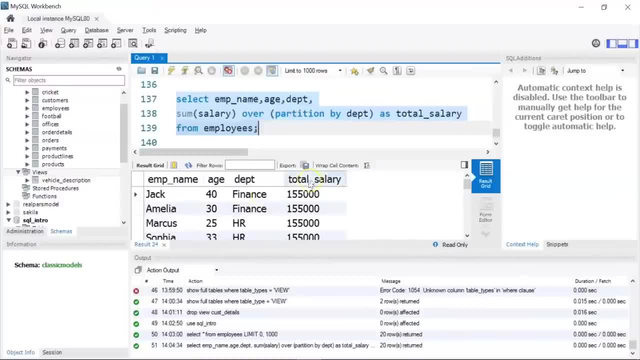 created another column in our result that is total and for each of the employees and the respective departments you have the highest salary. so in finance, the highest salary of one of the employees was $155,000. similarly, if I come down, we have the highest salary from HR, if I 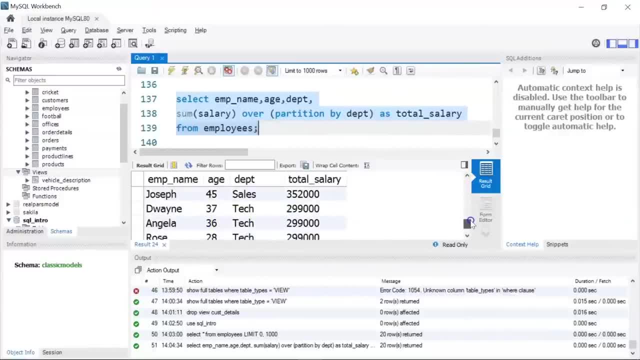 scroll further. we have the highest salary from IT, marketing, product sales and the tech team. all right, now we'll explore a function which is called row number. now, the row number function gives a sequential integer to every row within its partition. so let me show you how to use the row number function. I'll 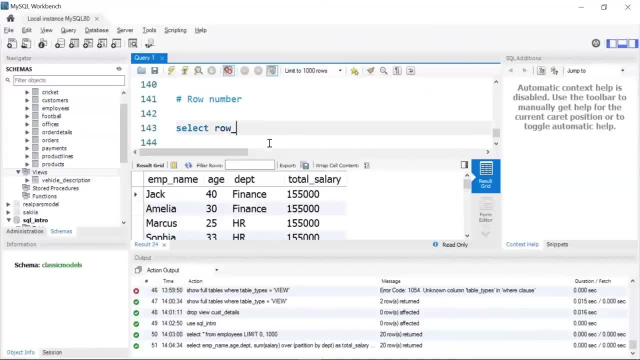 write, select a row underscore number. function over my column would be salary, so I'll write order by salary. I'll give the alias as row number, give a comma and I want to display the employee name and the salary of the employee from my table, that is employees, and I'll order. 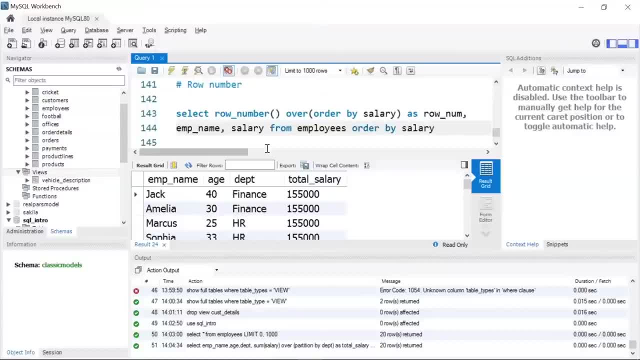 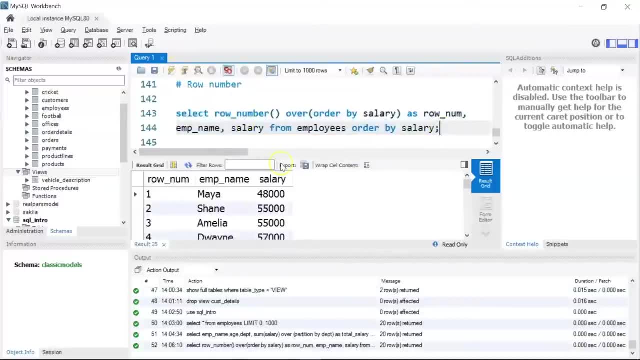 by salary. so let's see how our row number function will create sequential integers. okay, you can see, here we have a row num column and we have successfully given row numbers to each of the records. you can see it starts from 1 and goes up till 20. okay, now this row number function can be used to find duplicate values in a. 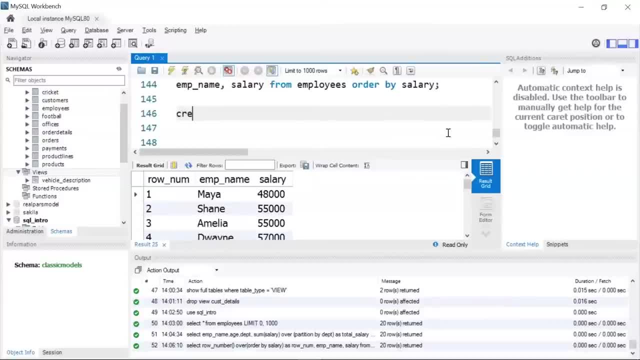 table. to show that first I'll create a table, I'll write: create table. let's say I'll give a random name- that is demo- and let's say we have a row number function. we have in this table the student ID, which is of type integer, and we have the student name. 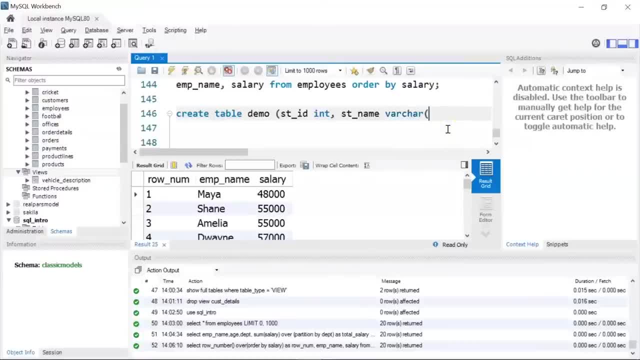 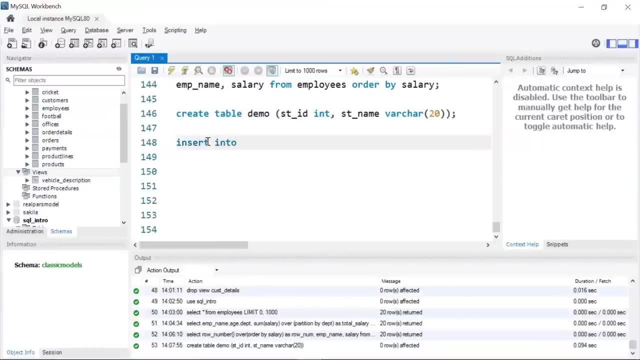 which is of type varchar, the size is 20.. I'll create the small table with a few records. let's create this table first. now we are going to insert a few records to our demo table, so I'll write: insert into demo values. I'll give 101. the name is Shane. give a comma. I'll insert the second student name. 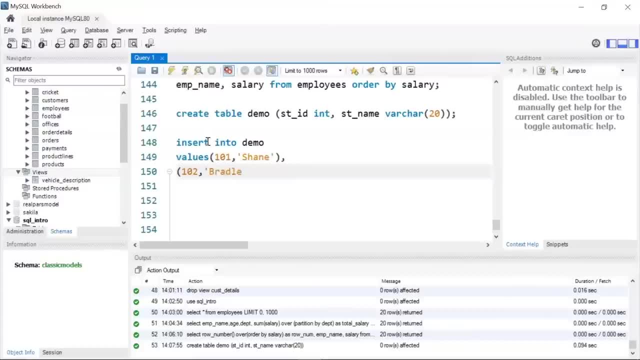 102, the name is Bradley. you give a comma this time for 103. we have two records. let's say the name of the student is Hiruth. give a command, I will copy dámel this time. let's say: give a comma. and now I will copy this current field, part forth. 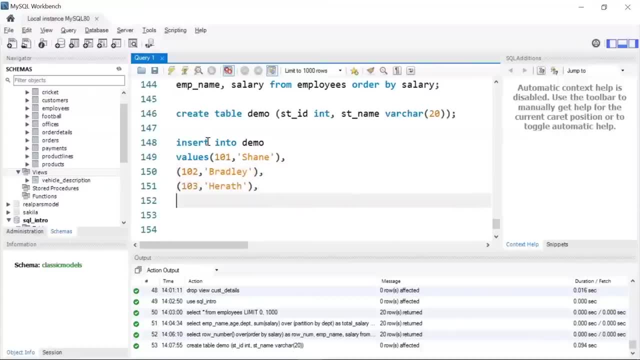 give a comma. I'll copy this and we'll paste it again. so we have duplicated 103. next we have 104. the name of the student, let's say, is Nathan. then again, let's say, for the fifth student, which is Kevin, we have two records. I'll copy this then. 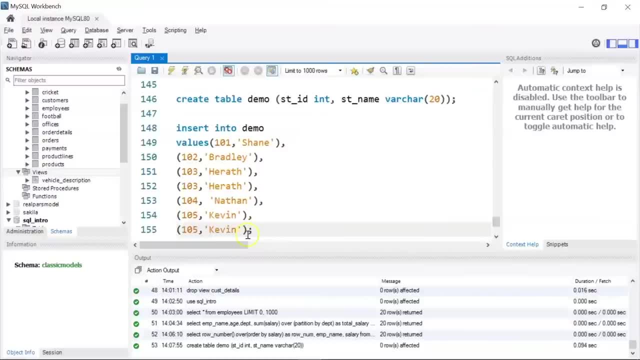 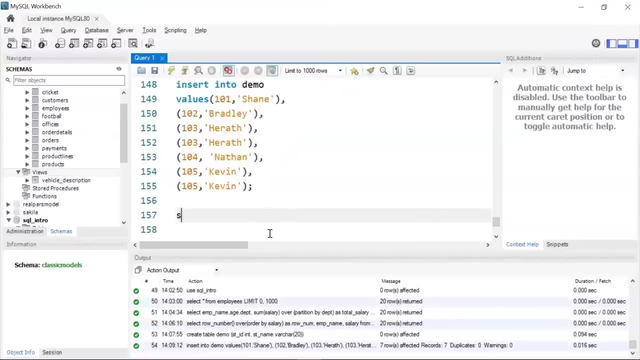 paste it here. let me give a semicolon and we'll insert these records to our table demo. all right, now let me just run this table for you. I'll write select star from demo. if you see this, we have a few information that are duplicated in our table, that is. 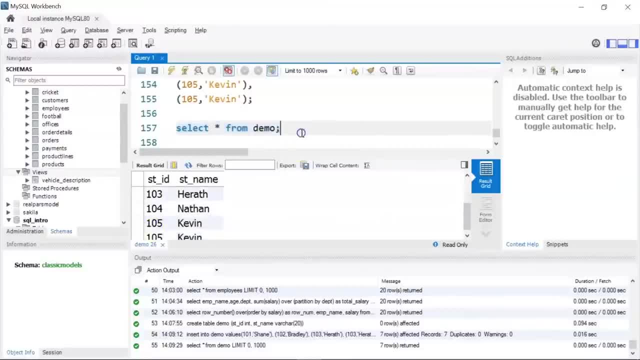 for student ID 103 and student ID 105. now I am going to use my row number function to find the duplicate records present in my table. I'll write select student underscore ID comma. student underscore name. I'll give another comma and write row underscore number over within brackets. 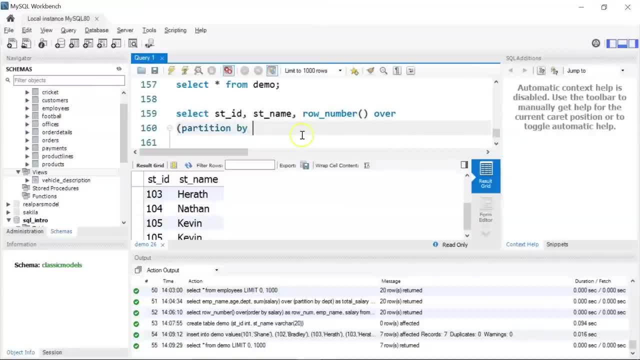 I'll write %1. I'll write partition by st underscore ID: comma, st underscore name. okay, then I will write order by st underscore ID. close the bracket. I'll give an alias as rhona 1 from my table of terms, editor 1 for my table of terms, class including two items. 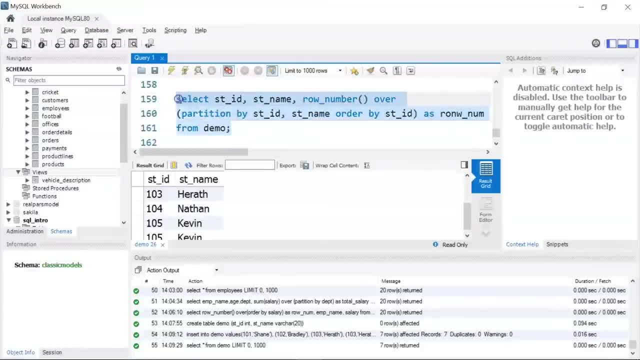 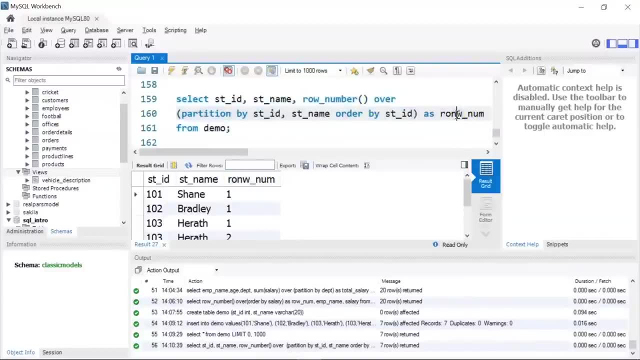 forbrank fields. two for us to search, I'll select theweight colon and we'll put in a. that is demo. let's just run it. you can see here. okay, let me just delete n from here and do it again. all right, if you see here there is just one student in. 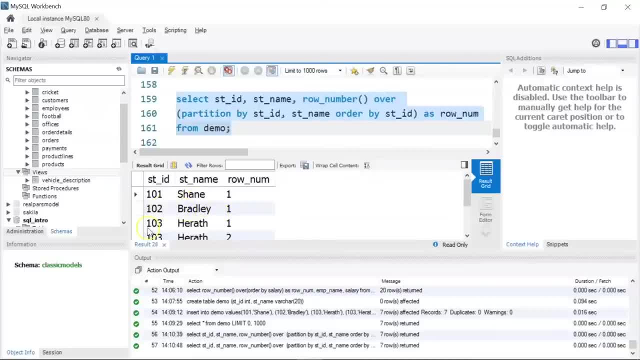 the name Shane. we have one student in the name Bradley, but here, if you see, for here earth, the second record, it says to, which means there are two records for here earth and if I scroll down, there is one record for Nathan and there are two records for Kevin, which means Kevin is also repeated. okay, now we are going to 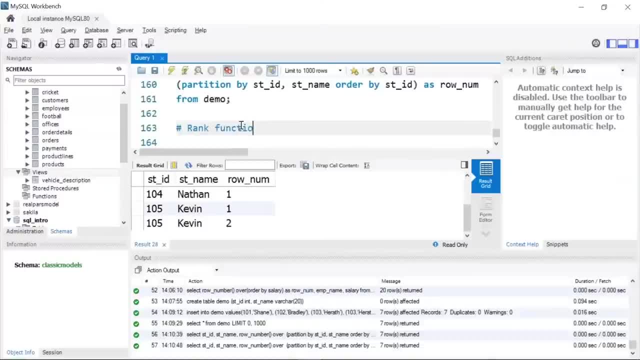 see another Windows function that is called rank function in my sequel. so the rank function assigns a rank to a particular column, but there are gaps in the sequence of rank values when two or more rows have the same rank. so first of all let me create a table and the name of the table. 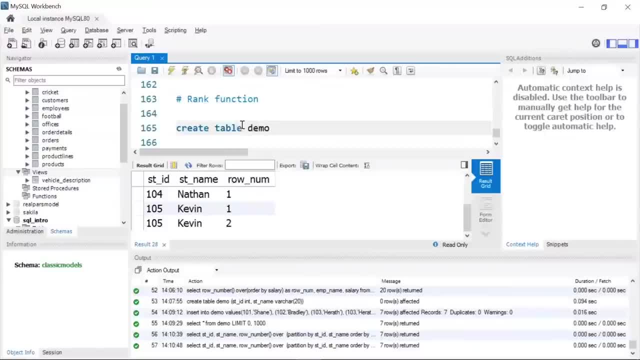 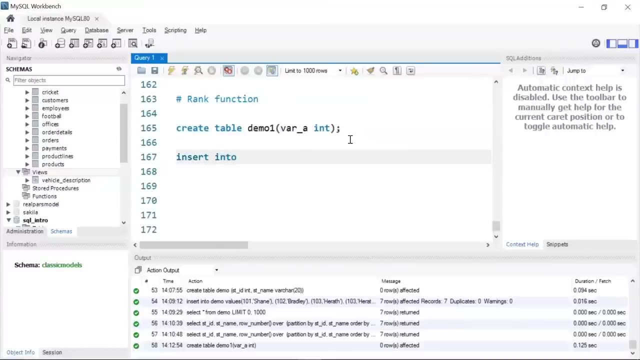 would be a random name, will give it as, let's say, demo 1, and it will have only one column, let's say variable a, of type integer. we'll create this table first. okay, now let's go ahead and insert a few records to our table, which is demo 1. so I'll 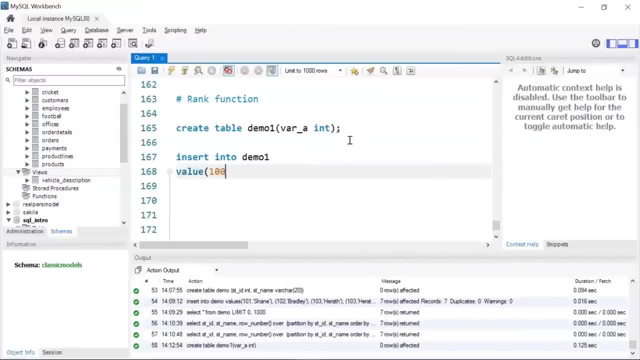 write value 101, 102, let's say 103, is repeated. I'm doing this purposely so that in the output you can clearly distinguish what the rank function does. next, we have 104, 105, we have 106 and let's say, 106 is also repeated. finally, 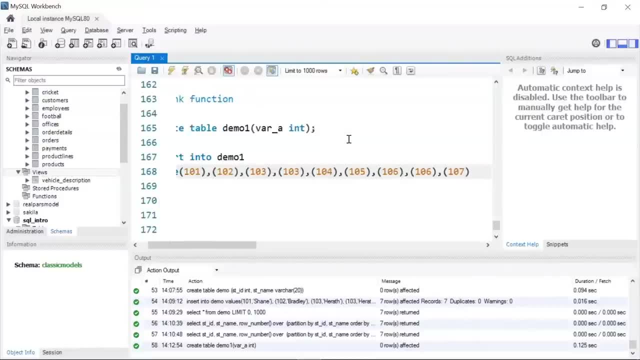 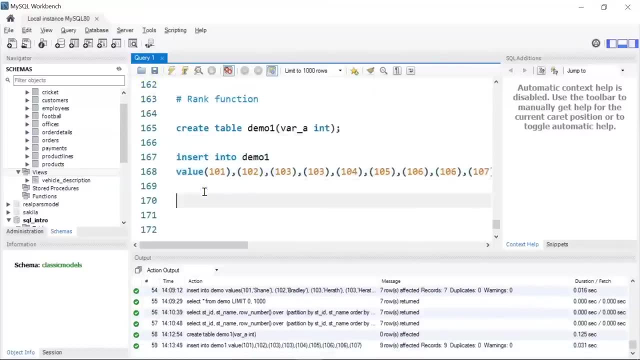 we have 107. okay, let me insert these values to my table. that is demo 1. okay, this is done. now, if I write select var underscore a and use my rank function, I'll write rank over. then I'll order by my variable, that is, var underscore a as an alias name. let's say test. 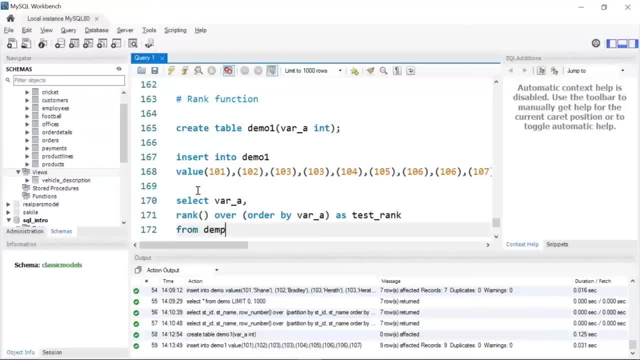 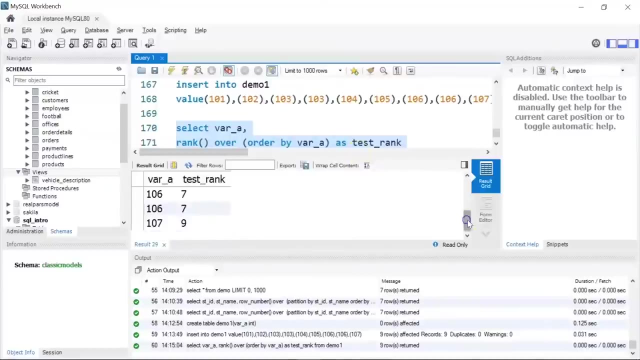 rank from my table, that is demo 1. let me execute this and show you how the rank function works. now, if I run this there, you go, so here. if you mark so, for variable a 101, the test rank is 1. for 102 the test rank is 2, but for this value. 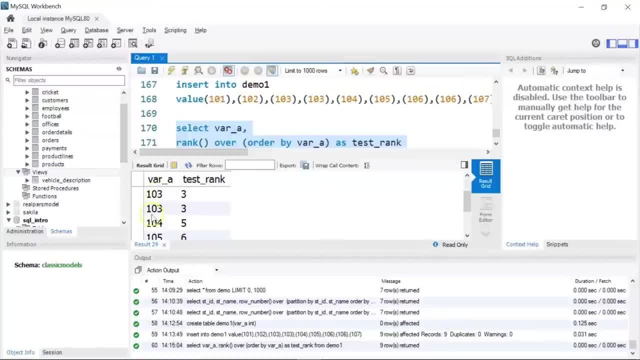 which is 103. the test rank is repeated because there was a repetition for 103, so we have skipped the rank 4 here for 104. the rank is 5, now for 105, the rank is 6, now for 106. again, since the record was repeated twice, we have skipped the 8th rank and 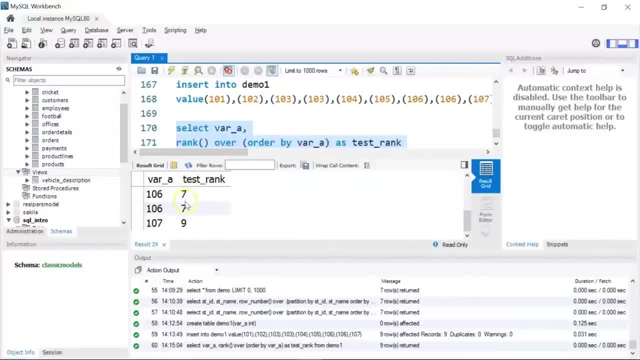 you. we can just see that our rank function assigned the same value, which is 7, for 106 and for the last value, 107, the rank is 9.. all right, now, moving ahead, we'll see our final Windows function, which is called first value. so first value is another important function in my sql. so this function returns the value. 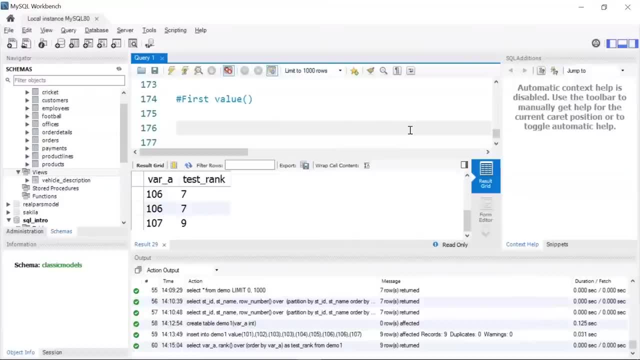 with respect to the first row in the window frame. all right, so what I am going to do is I am going to select the employee name, the age and salary and I will write first underscore value, which is my function, and pass in my employee name, and then I will write over order by. 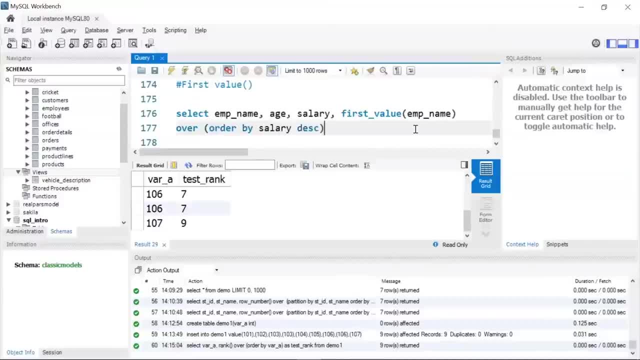 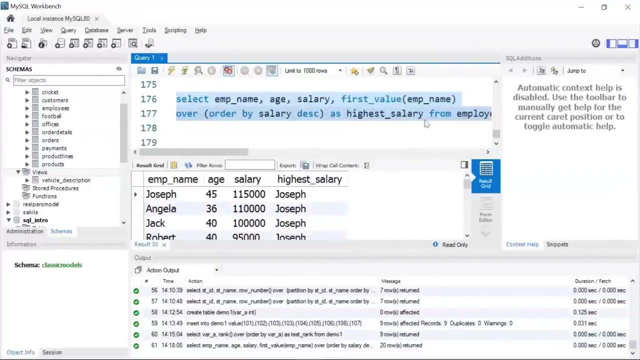 my column, that is salary descending. I'll give an alias as highest underscore salary from my table, that is employees. so let's begin. let me run this and see how the first underscore value function works alright. so in our table, Joseph was the employee who had the highest salary, which was $115,000. so the first value. 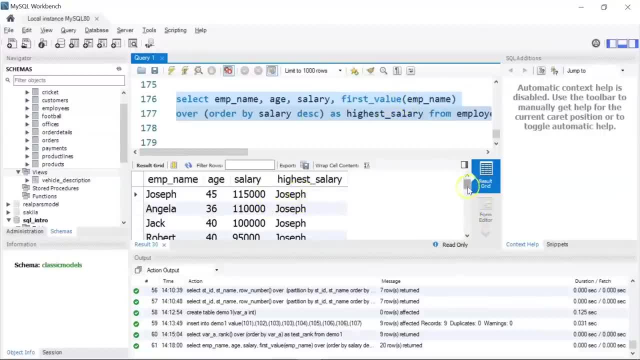 function populated the same employee name throughout the table. you can see it here. now you can also use the first underscore value function over the partition. so let's say you want to display the employee name who has the highest salary in each department, so for that you can use the partition. I'll write select EMP underscore name comma. I want the. 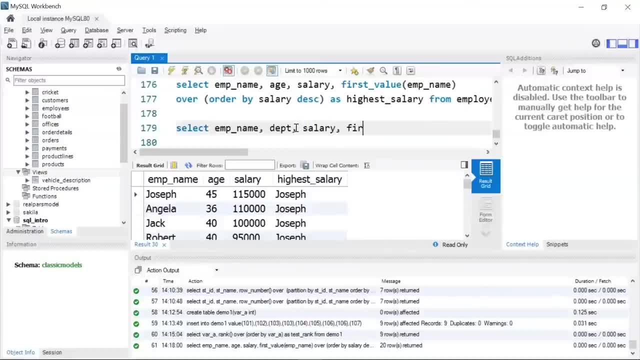 department and the salary comma. I'll use my function, that is, first underscore value followed by the name of the employee. inside my first value parameter I'll write number over here. I am going to use partition. I'm going to partition it by the department, since I want to know the employee name who has the highest salary in each department. 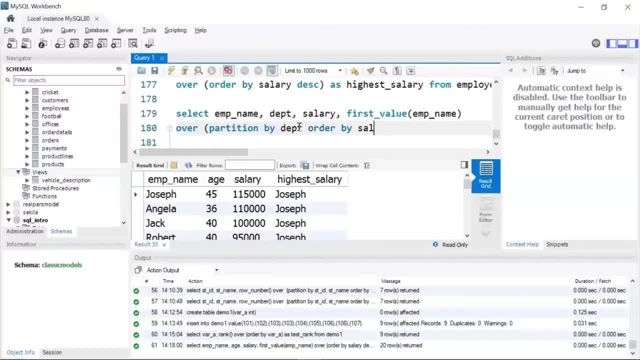 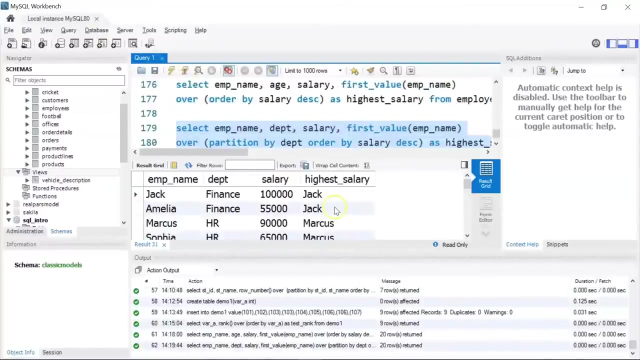 and I'm going to order by salary descending and I will give my alias again as highest salary from department number. my table that is employees. so let's run this and see the difference in the output. okay, so, as you can see, here we have the employee who had the highest salary from each department. 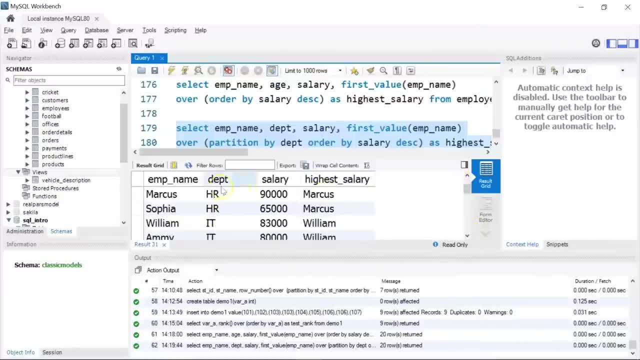 so for finance, jack had the highest salary. from hr, it was marcus. similarly in it it was william. if i scroll down, for marketing, it was john. for product, it was alice who had the highest salary. similarly, in sales, we had joseph, and in tech, we had angela. so this is how you can use the 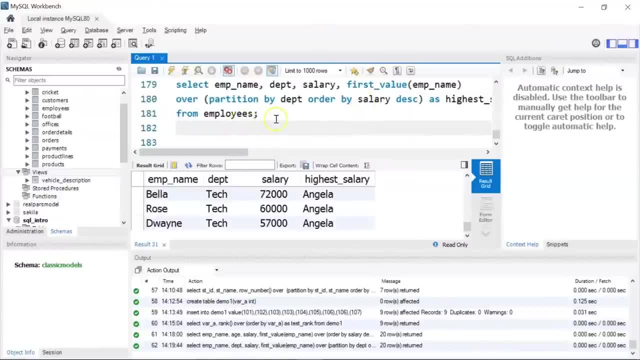 first underscore value function using partition. all right, so that brings us to the end of this demo session on our tutorial, so let me just scroll through and show you what we did from the beginning. first we learned about sub queries in sql, so we initially wrote a simple sub query and then we used our classic models database. 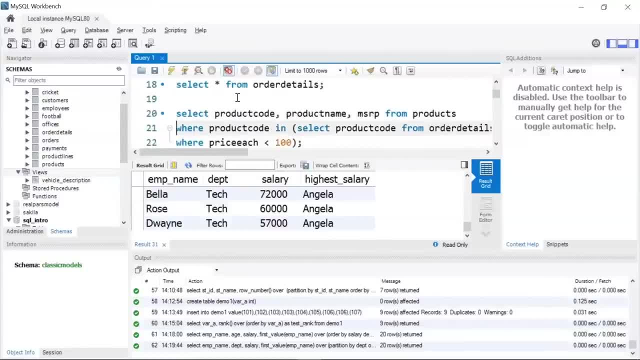 which was downloaded from the internet. i had also shown you the link from where you can download this database here. we used two different tables and we performed a sub query operation. we learned how to create stored procedures, so we learned how you can use the in operator or the in parameter as well as the out parameter in stored procedure. after stored procedure. 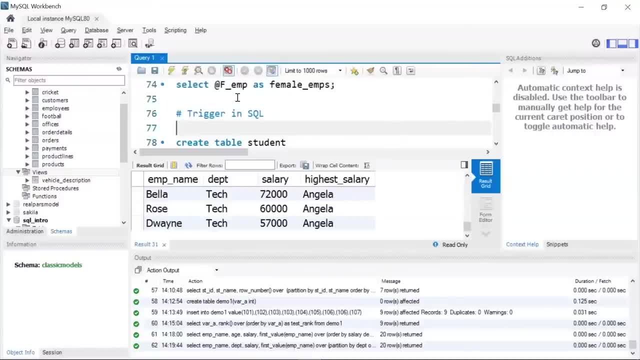 we learned how to create stored procedures, so we learned how you can use the in operator. we learned another crucial concept in sql, which is called triggers. now triggers are also special kind of stored procedures, so we saw how to write a before insert trigger. you can see it here. 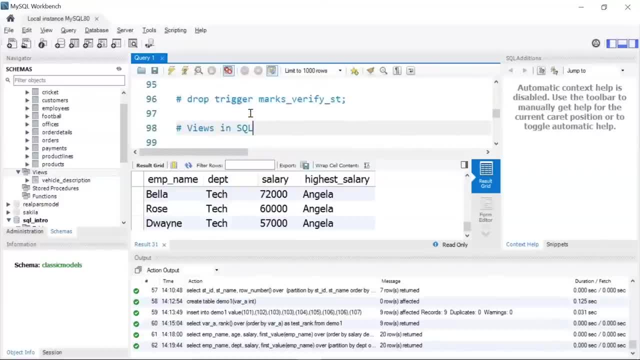 next, we learned how to delete a trigger. we also saw how to work with views in sql, so views are basically virtual tables that you can create from existing tables. we also saw how you can use views using two different tables and an inner join, and we learned how to display views, how to rename. 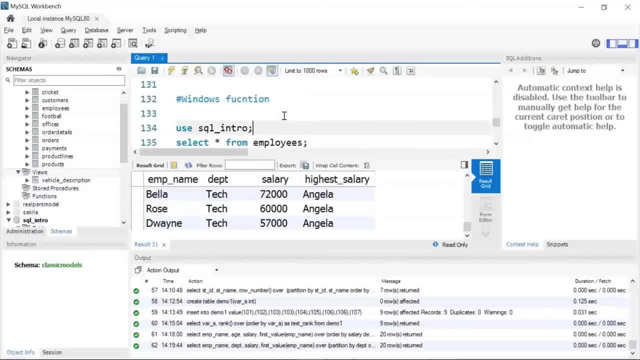 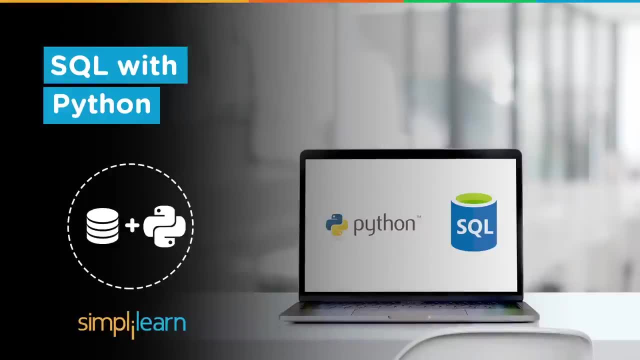 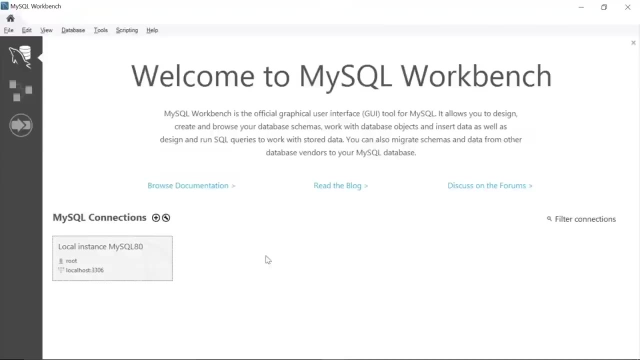 view names, how to delete a view and, finally, we explored a few windows function. in this tutorial we will learn how to work with databases and tables using sql, with python. to do this demo, we will be using our jupyter notebook and the mysql workbench. you can see it here. so we will write our sql queries in the jupyter notebook with python, like syntax. if you don't have mysql or jupyter notebook installed, so please go ahead and install them first. while installing the mysql workbench, you will be asked to give the username and password. 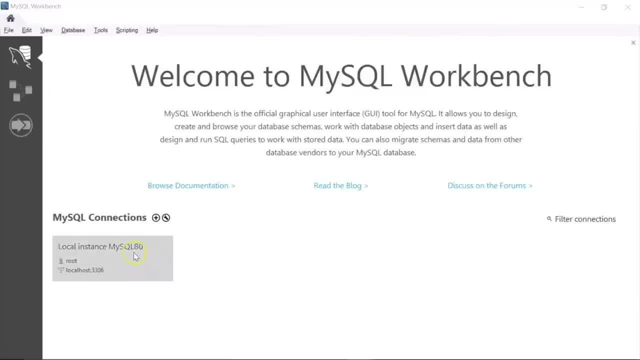 let me show you so. i am on my mysql workbench, so once you connect it will ask for the username and the password. so i have given my username as root and password you can give while installing it. we will be using the same user id and password as root and password you can give while installing it. 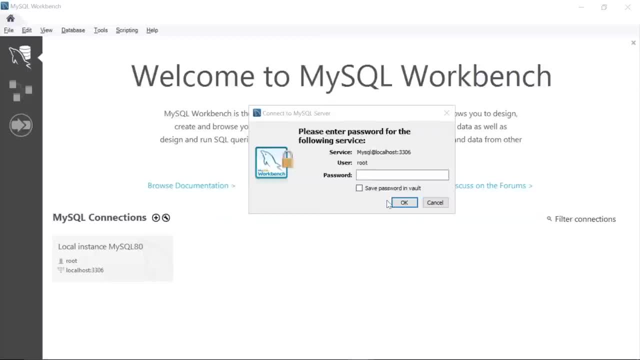 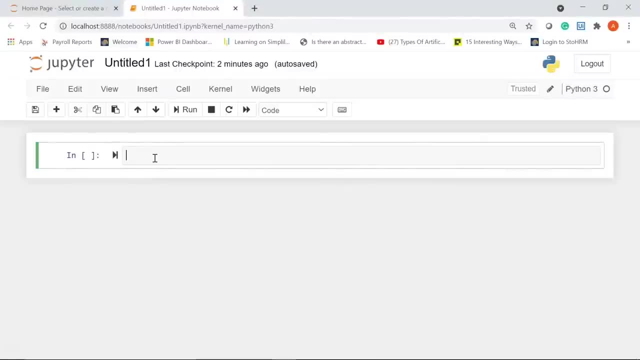 or the username and the password to make our connection. so let's get started with our hands-on demonstration part. first and foremost, let me go ahead and import the necessary libraries. i'll give a comment as import libraries. all right, so first i'll import mysqlconnector, next, 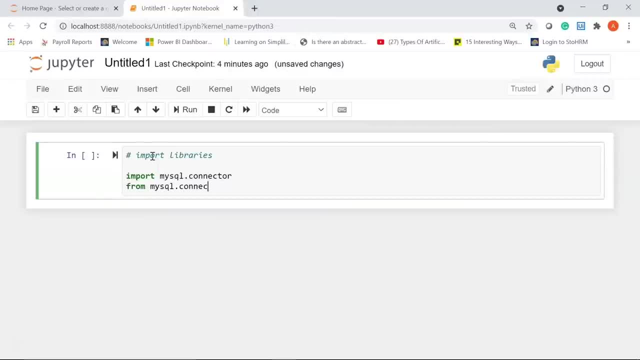 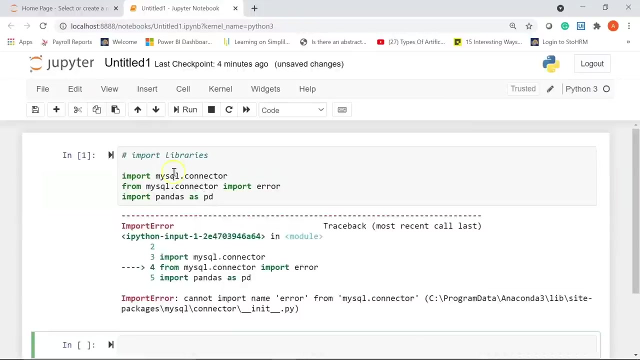 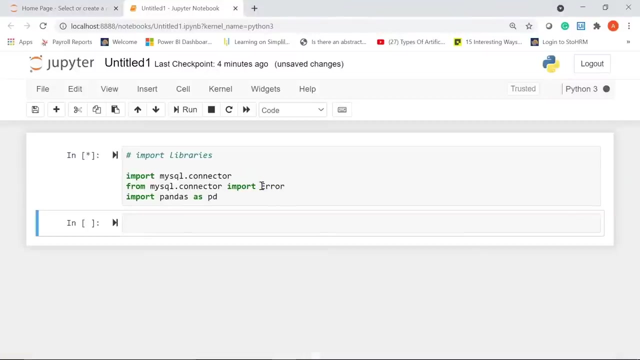 from mysqlconnector. i am going to import my error method or the error module. next i want to import pandas as pd, so let's run this. okay, there is some error here. this should be capital e and not small e. all right, you can see, i have imported my important libraries. 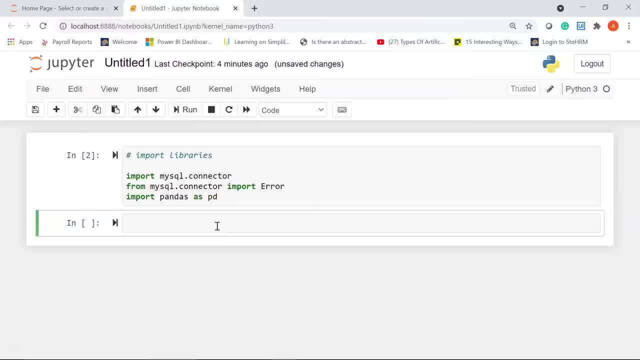 now i'm going to create a function that will help us create a server connection. so i'll write my user defined function by using the def keyword. i'll write: create underscore server, underscore connection. this is going to be my function name and it will take in three parameters. first is the host name. 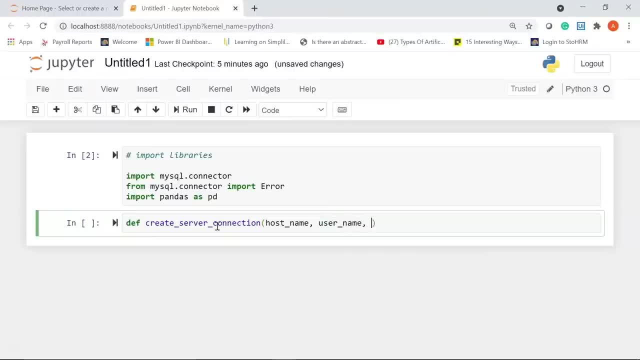 next is the user name and then we have the user password. all right, i'll give a colon and then in the next line, i'm going to define a variable, which is going to be connection, and i'll assign it to a value called none. now we'll be using exception handling techniques to connect to our myself. 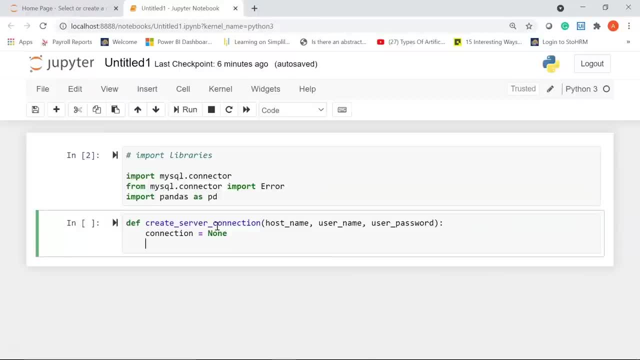 sql server. the try block lets you test a block of code for errors and the accept block will handle the errors. so i'll write try and give a colon, and then i'm going to reassign the connection variable to a method which is mysql: dot connector- dot connect. 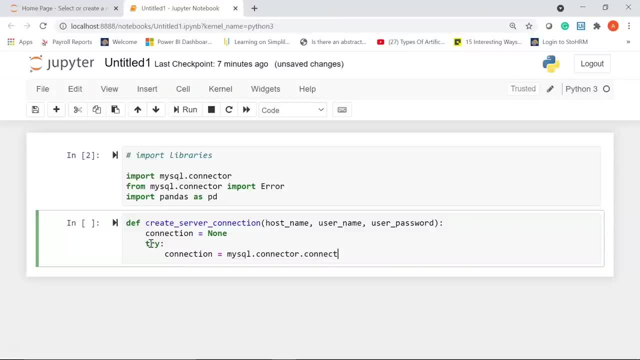 now this mysql connector dot connect method sets up a connection so it establishes a session with the mysql server. if no arguments are passed, it uses the already configured or default values. so here we are going to pass in three parameters. the first is the host name. i'll write host equal to host name, which is host underscore name. 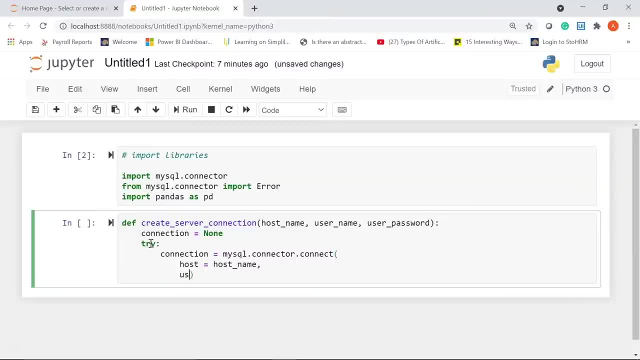 i'll give a comma. then i'll write user equal to user underscore name. next will be my password and i'll assign the value user underscore password. all right, now i'm going to use a print statement and write mysql database connection successful. after this i'll give my accept block, so i'll use the keyword accept here. i'll write error as. 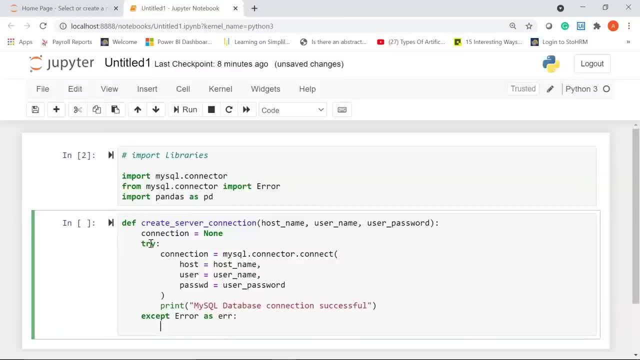 err, give a colon, and then i'm going to use the print statement here. i'm going to use some print formatting techniques. using the f letter, i'll write error, colon and i'll use curly braces: give err and then i'll close the double quotes. after this, i'm going to 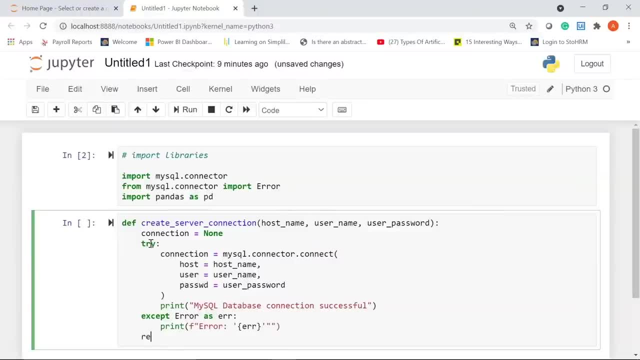 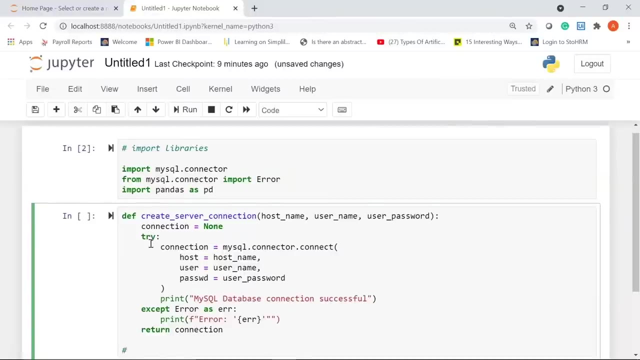 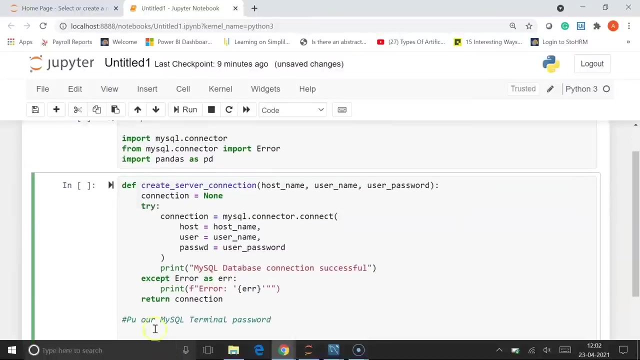 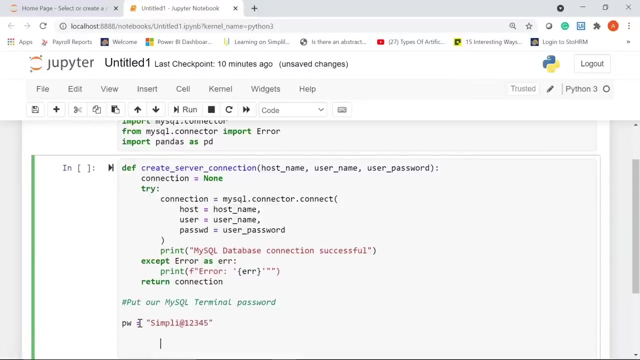 return my connection. all right, let me give a comment. here we are going to assign our password, so we need to put our mysql terminal password and include the password in our plugin. so this is 1, so this password you assign it while installing mysql workbench. i'll write. 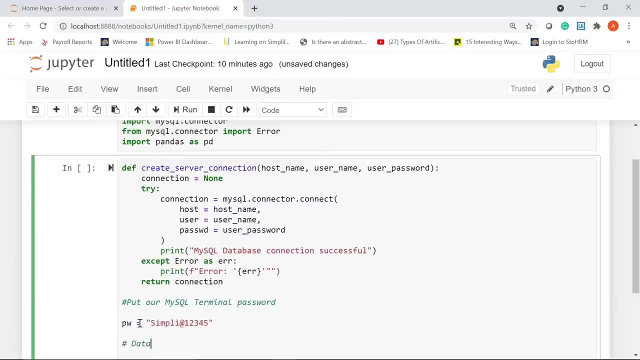 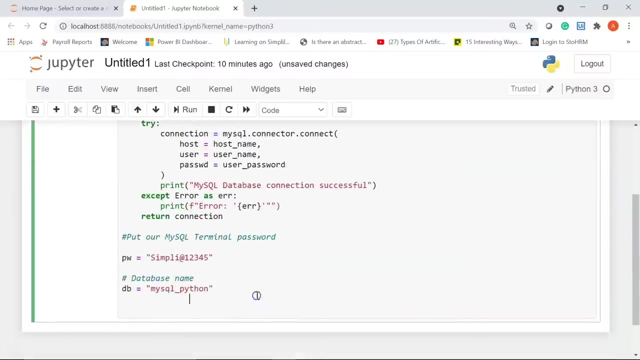 give my database name. so i'll give database name. here i am going to write db equal to. this is the database i want to create, which is going to be mysql underscore python. let me just scroll this down. okay, now i'll say connection equal to. i'll pass in my user defined function name, which is: create server connection. 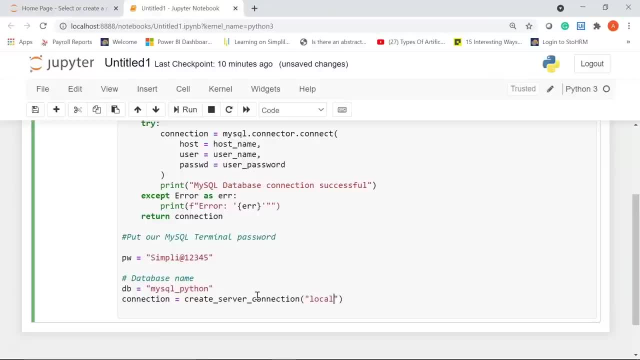 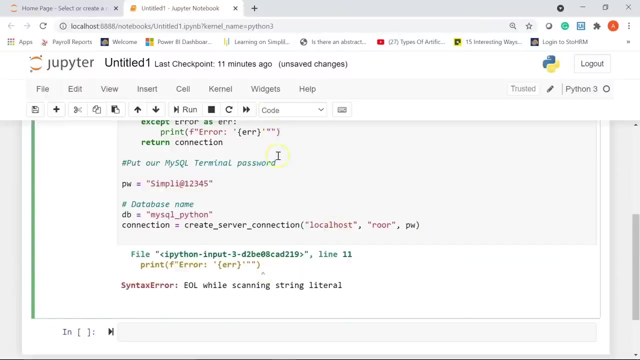 and the parameters, which are going to be localhost. that is my host name, my username, which is root, and then i'll give pw, which is my password. that is exactly, simply, at the rate, one, two, three, four, five. let's just run it now. okay, there is an error here. we need to remove this double quotation. 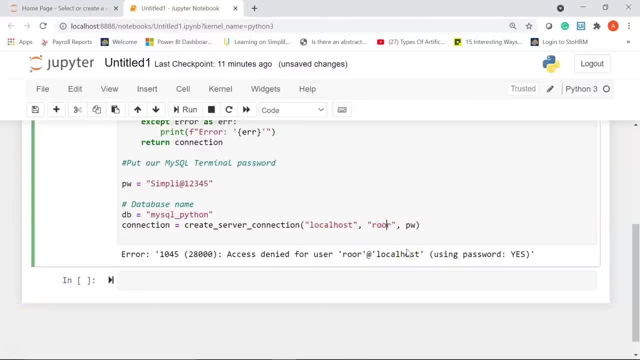 all right, made another mistake here. this: this should be root. okay, you can see here mysqld connection successful, all right. next we are now going to create a database that is mysql underscore python. so i'll give a comment: create mysql underscore python database. again to create: 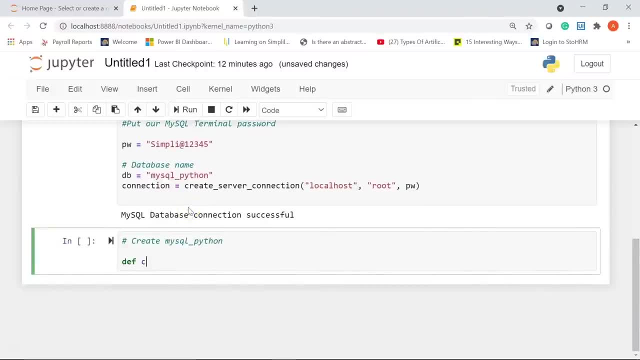 this database. i am going to create another user defined function using the def keyword. i'll write the function name as create database database, passing the parameters as: connection comma query give a semicolon and in the next line i'll write cursor equal to. i'm going to make the connection, so i'll write connection dot cursor. 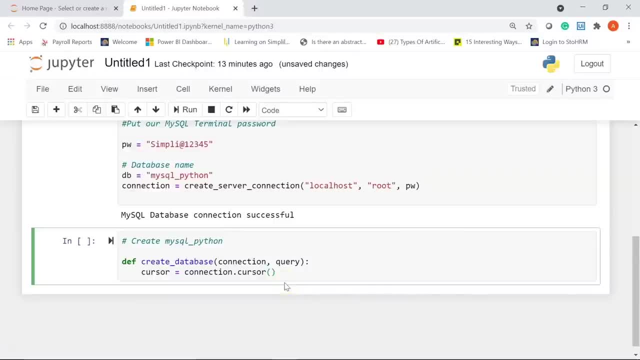 and i'll give the parenthesis. so this mysql's cursor of mysql connector python is used to execute statements to communicate with the mysql database. the mysql cursor class initiates objects that can execute operations such as the mysql statements. okay, next i'm going to again use my try and accept block, so i'll write: try, give a colon. 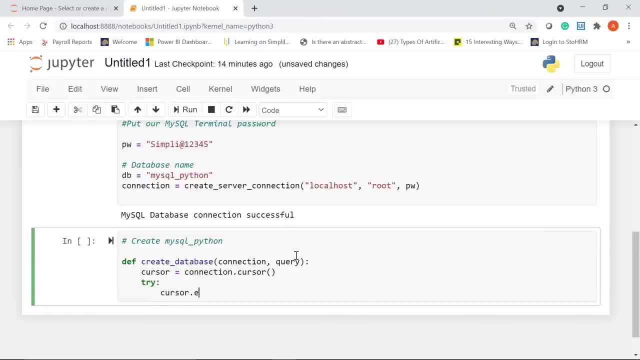 and here i'm going to use cursor dot execute. within that, i'm going to pass in my query. next i'll use a print statement and the message i'm going to display is: database created successfully. after this, i'm going to write my accept block. i'll write accept error as err, give a colon. and then i'll use a print statement. i'll write print. 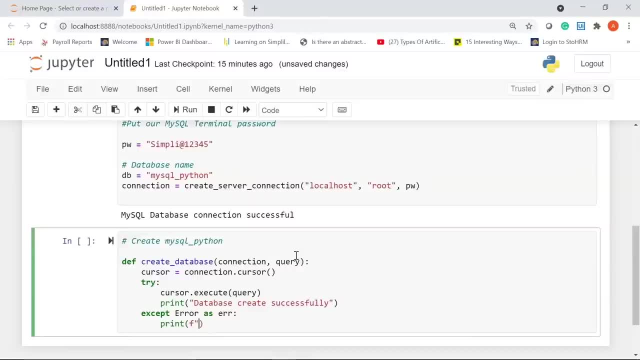 i'll use the formatting again, error, colon, and i'll write within single quotes: i'll give curly braces, err, and then i'll close the double quotes. next let's use the variable create underscore database, underscore query. and here i'm going to write my sql query to create the database. so i'll write create. 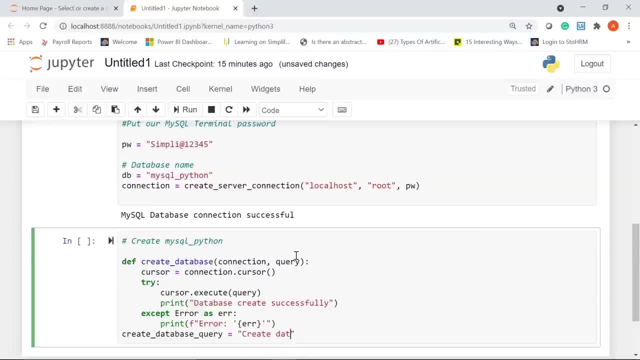 database and, followed by that, i'll give my database name, which is going to be mysql, underscore python. okay, after this I'll call my function, which is create database, and i'll pass in the parameters. the first one is connection and next the query is create underscore database, underscore query. let me just copy it. 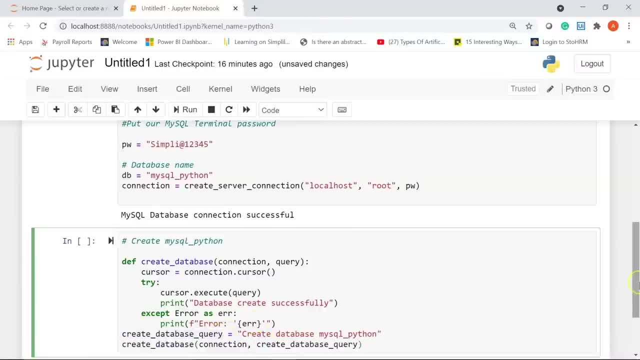 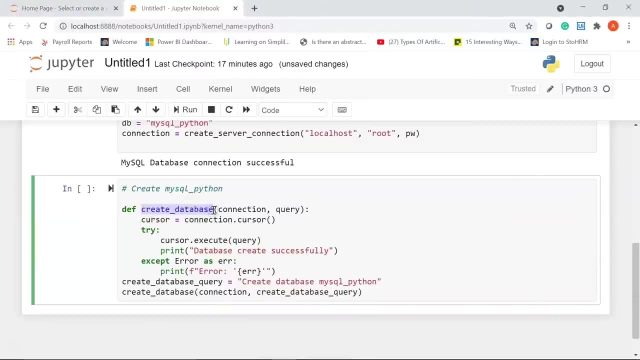 and i'm going to paste it here. all right, so what i am doing here is i am creating a new function, that is, to create a new database with the name mysql underscore python, which you can see it here now. this function takes in two parameters: connection and query. i am using the connection. 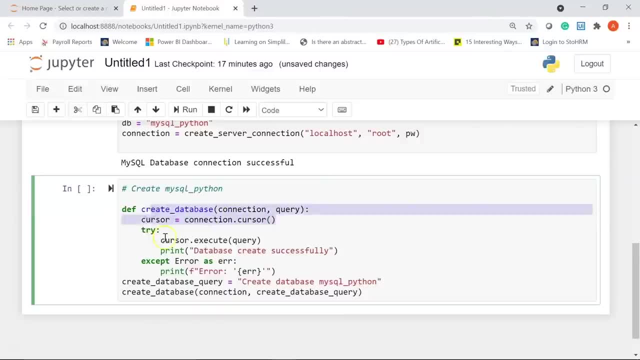 dot cursor function which is often used to execute sql statements using python language. and then i have created my try and exit blocks. so this try block statements will try to create my new database, which is mysql underscore python. in case it fails to create the new database, the accept block will. 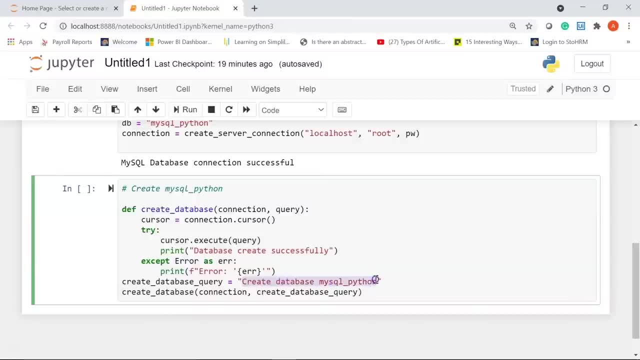 work. so here i am writing my sql query to create a new database, which is create database, followed by the database name, and i am assigning it to a variable which is create database query, and then i am calling my function create database and passing in the two parameters connection and 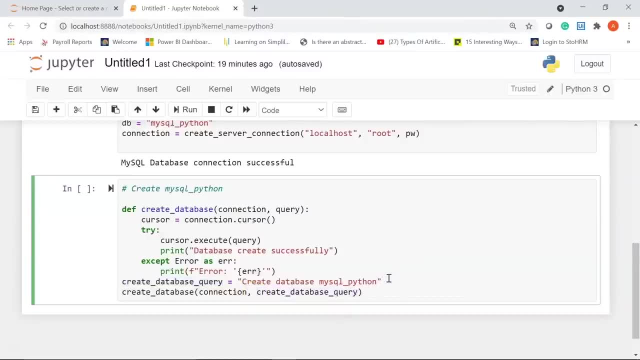 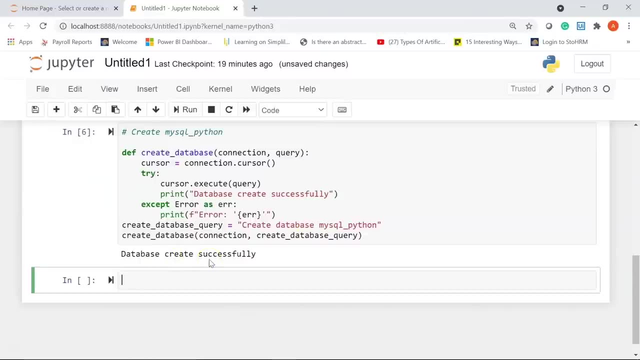 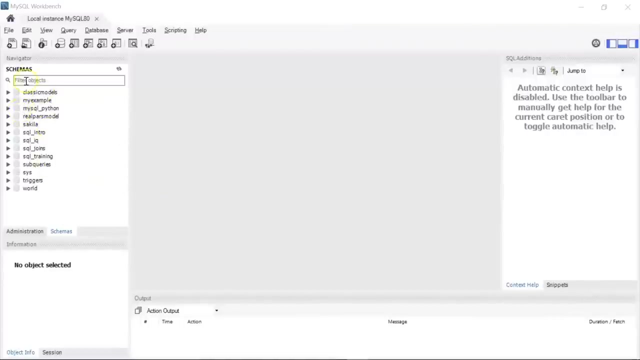 the query. alright, so let's just run it. alright, you can see here it has created my database successfully. now you can verify this by checking the mysql workbench or the mysql shell. you can see on the mysql workbench, here on the left panel under schemas, there is a database called mysql. 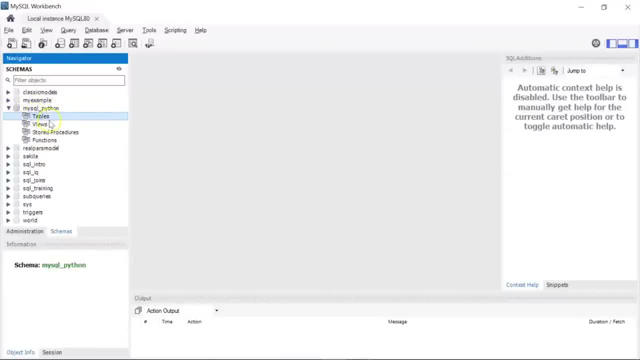 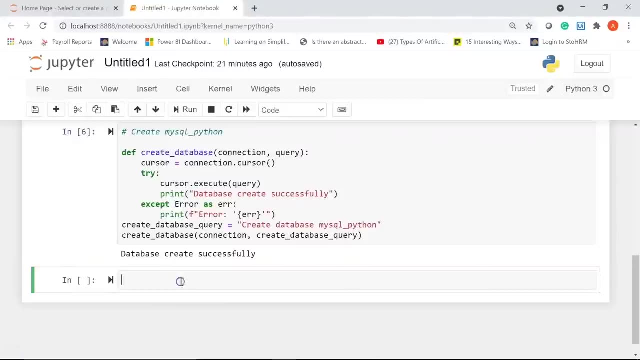 underscore: python. let me just expand it now. we haven't created the database yet, so let's any table. so it's not showing it now. the next step: we are going to connect to this database now, so let's go ahead and connect to our database that we have. 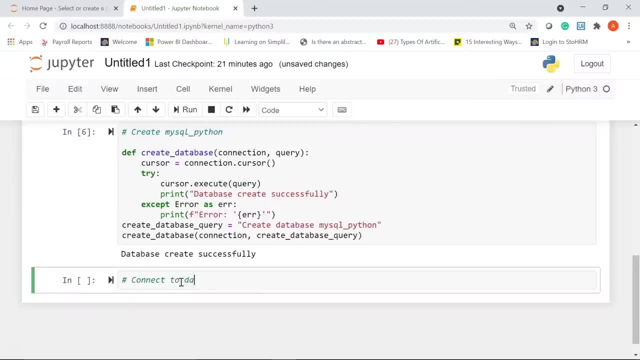 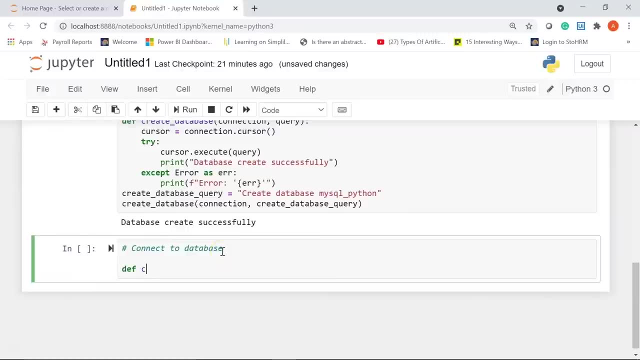 just created. I will write the comment as: connect to database. now, to connect to a database, I am again going to create a user-defined function using the def keyword. I will write create underscore DB, which is for database underscore connection, and the parameters it will take is the host name, followed by the 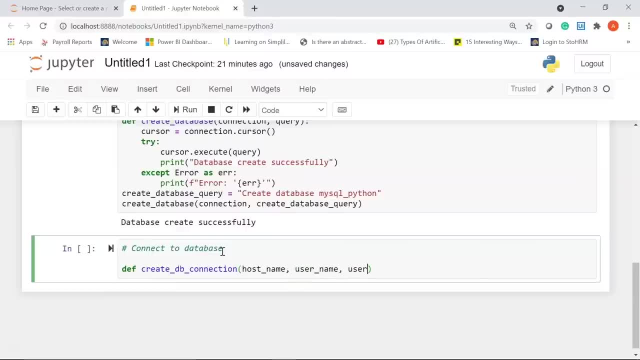 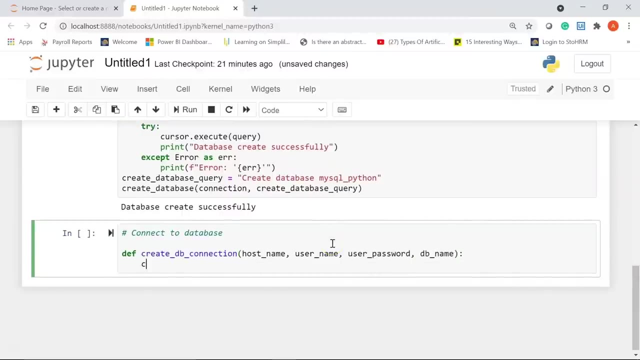 username, then we have the user password and finally we have the database name. I'll give a colon in the next line. I am going to create my variable, which is connection, and then I'll assign it to a value. none after this. I am going to use my exception handling techniques, so I'll 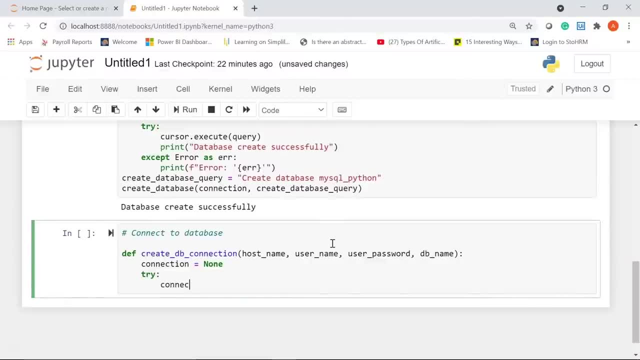 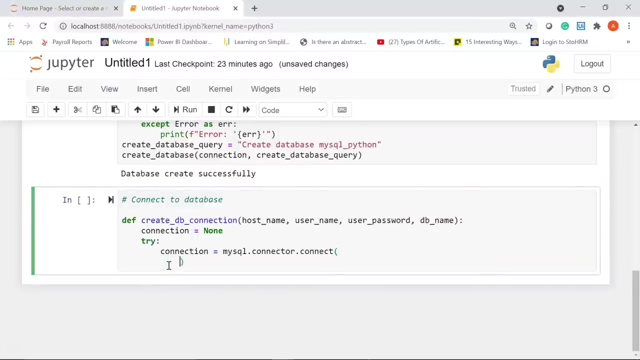 write my try block first. I am going to reassign my connection variable using the mysql connector method. so I'll write mysql dot connector, dot connect. so this method will take in the parameters. so first it will take the host name. I'll write host equal to host. 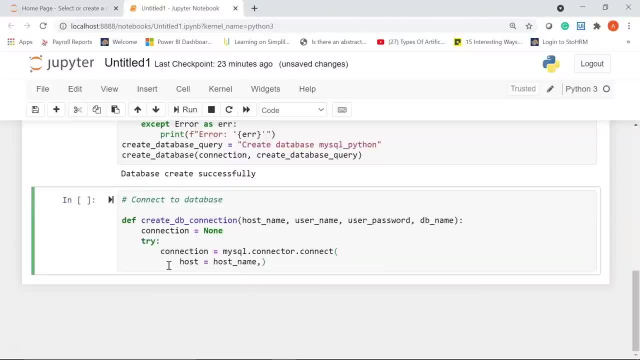 underscore name. I'll give a comma. next it will take the user name, so user equal to user. underscore name. give another comma. next it will take the user password. i'll use passwd equal to user underscore password. we'll give another comma and this time it is going to be the database name, so i'll write database. 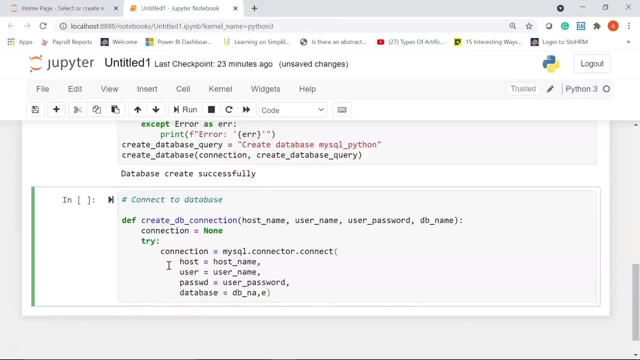 equal to db underscore name. now let's use the print statement and the message we are going to print: is mysql database connection successful? all right, finally, we'll write my accept block. i'll write accept error as err. give a colon and then i'll use the print statement f. 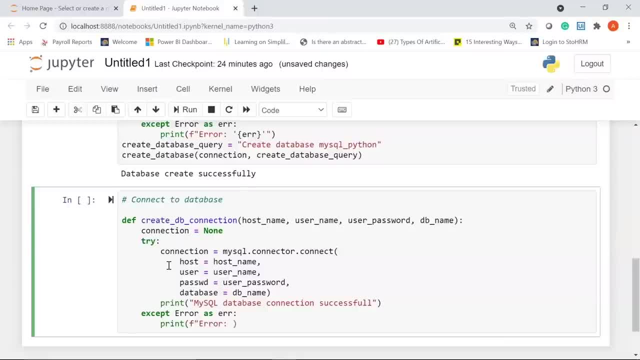 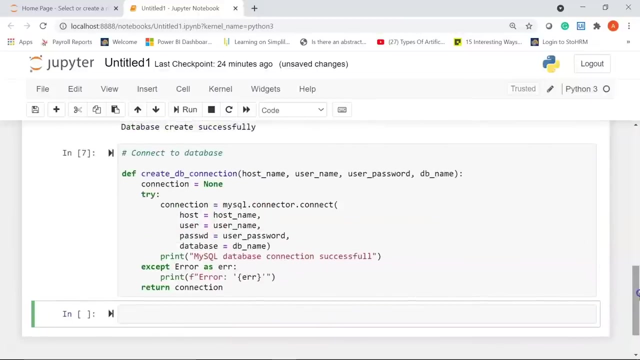 within double quotes, i'll write error colon. within single quotes: curly braces: i'll write err and we'll close the double quotes. finally, this function will return the connection value. all right, let's run it. and there you go. it has run successfully, so we have connected to our database. 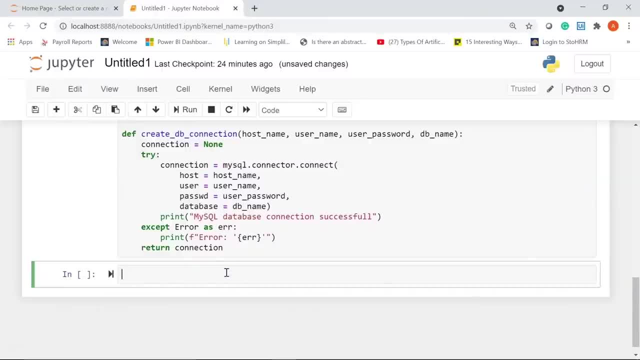 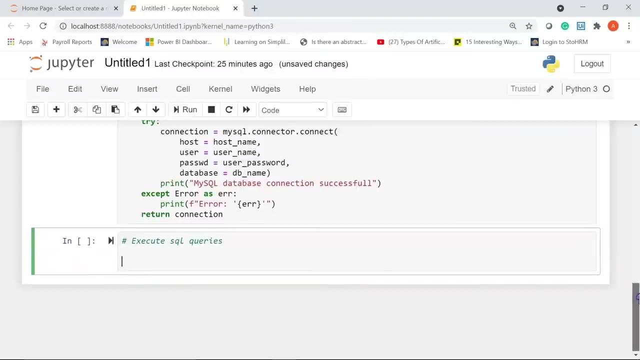 it's time for us to execute sql queries. i'll give another comment saying execute sql queries. all right, now to execute our sql queries, i'll use another user defined function which is execute underscore query and i'll pass in the parameters as connection and query. i'll give a colon. i'm going to write cursor equal to connection dot cursor. 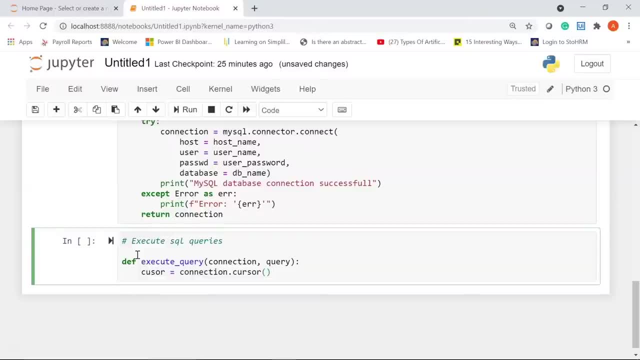 now this is used to establish a connection and run sql statements. next we'll use the try and accept block, so i'll write try cursor dot execute. this will take in one parameter, which is going to be my query, and then i'll write connection dot commit, which is another method. 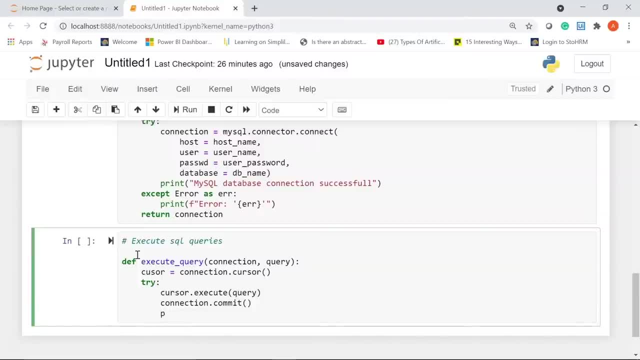 now let's use the print statement, so i'll write print. let's say the message would be: query was successful and then we'll write our accept block, which is accept if the try block doesn't work. throw an error using the print statement within double quotes. inside the inside the curly braces. 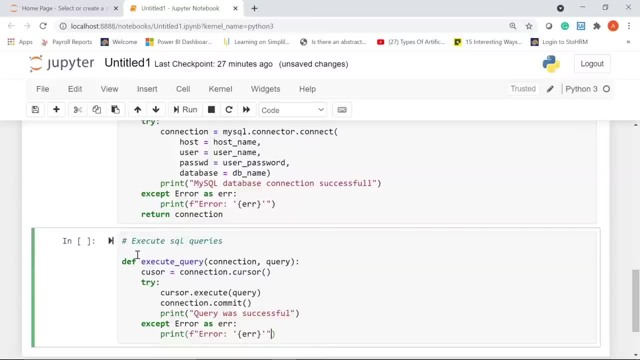 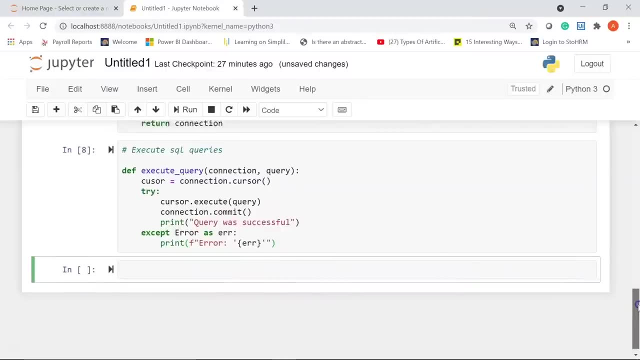 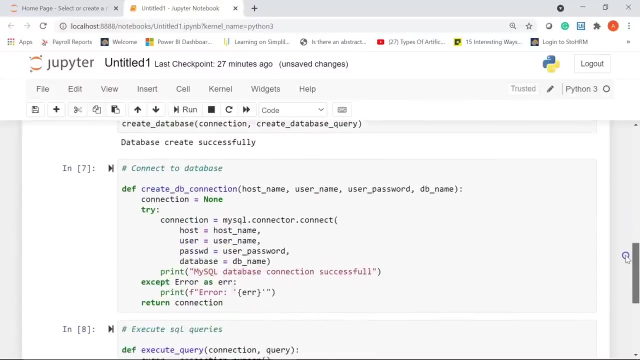 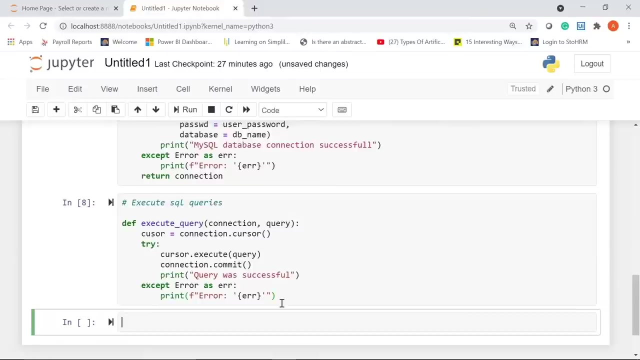 I'll write ERR and close the double quotes. all right, so let's run it. okay, so we have successfully created our various functions that were needed to create a database, establish a connection and to execute our queries. all right, now it's time for us to create our first table. 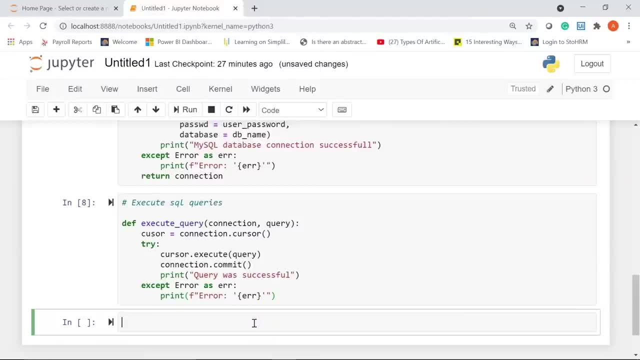 inside the mysql underscore Python database. so to do that, I am going to write my create command in SQL. so first we are going to assign an SQL command to a Python variable using triple quotes to create a multi-line string. so let me show you how to do that. I'll write my. 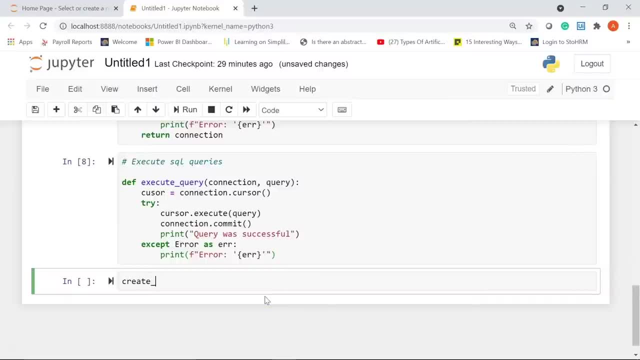 SQL command to a Python variable using triple quotes to create a multi-line string. so let me show you how to do that. I'll write my variable name, which is going to be create orders table. it is always recommended to use relevant variable names to make it more readable. and now, 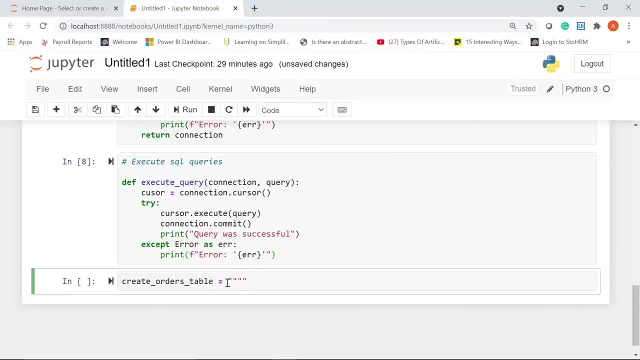 I'm going to use triple quotes, so the triple quote will ensure I can create my multi-line string. inside the triple quote I am going to write my create command, which is create table. here I'm going to create an order stable first, and inside the orders table I am. 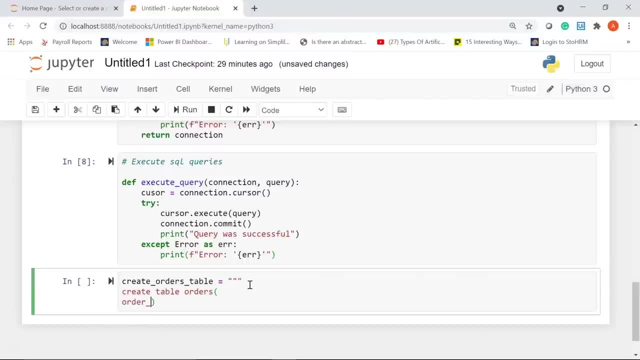 going to create my column names. the first column would be the order ID. it is going to be of type integer and I'll assign this order ID as my primary key column. we'll give a comma next. the second column would be Customer underscore. next style colour which is also open to use, or, if I am not, eventual gate schema or vraag a table. they're pretty much any query. so we have an order state and when I have the item to symbolender girl type table types in procedure: get 말이 service. 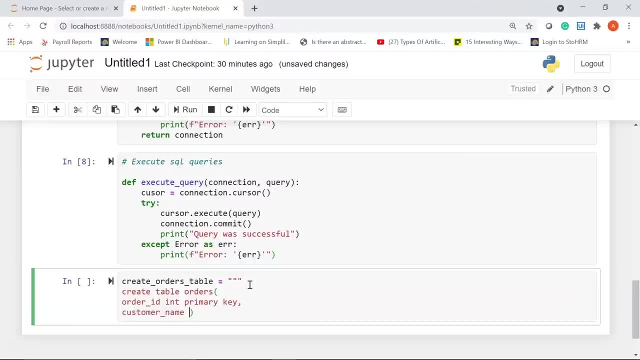 name. the customer name column would be of type varying character, so i'll write varkar and i'll give a size of 30, and this is also going to be not null. moving ahead, my fourth column would be the product name column, so i'll write product underscore name. 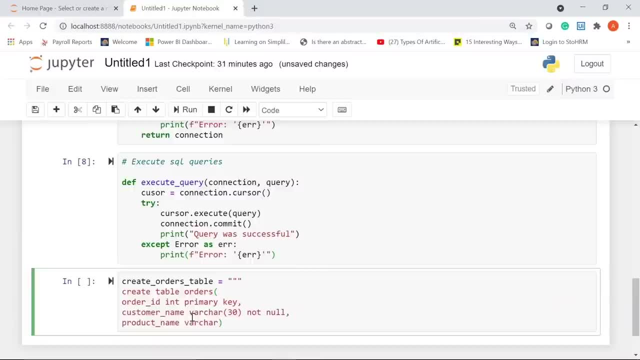 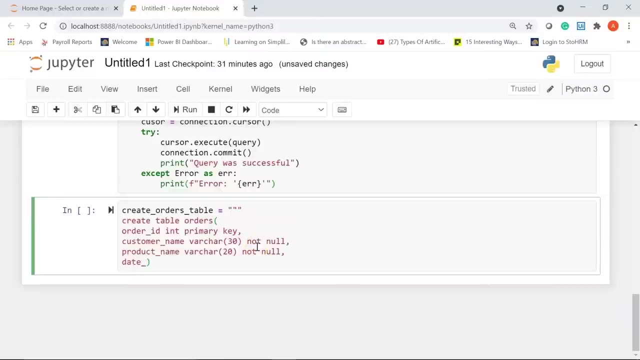 product name will be of type varying character. the size is, let's say, 20, and it is also not null. next, i am going to create my fourth column, which is the date on which the item was ordered or the product was ordered. so i'll write date ordered. the data type will be date. next, i'll create: 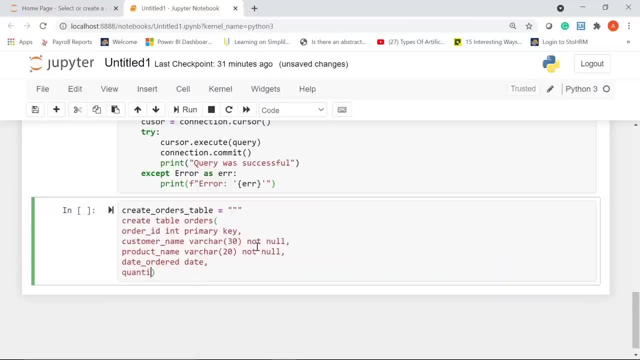 a quantity column to keep track of the number of quantities that were ordered. this is of type integer. my next column would be unit price, which will basically have information about the price of each unit of product. unit price can be of type float. and finally i'll have the 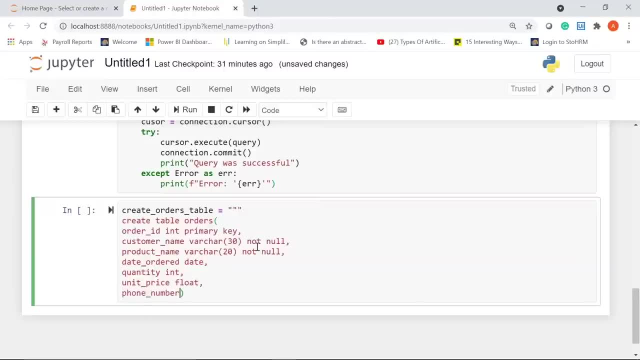 phone number of the customer. i'll write phone number. phone number can be kept as of type varying character. i have assigned a size of 20.. now let's give a semicolon and we'll close the triple quotes. all right, so this is how the syntax would look like next. 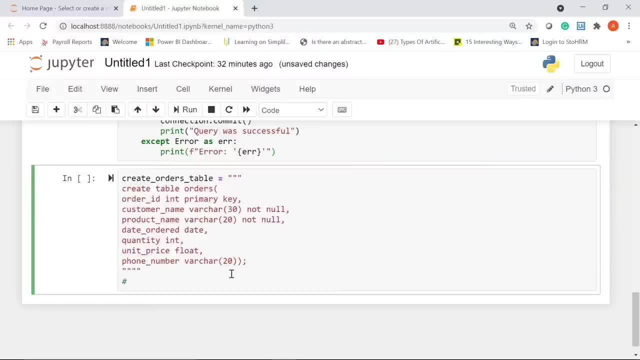 to run this. we are first going to call our create db function. so let me give a comment. as connect to the database, i'll write connection equal to create underscore db, underscore connection. my parameters would be my host name, which is localhost, my username, which is root comma, my password, and then my database name, which is mysql, underscore python. so i'll write just db. 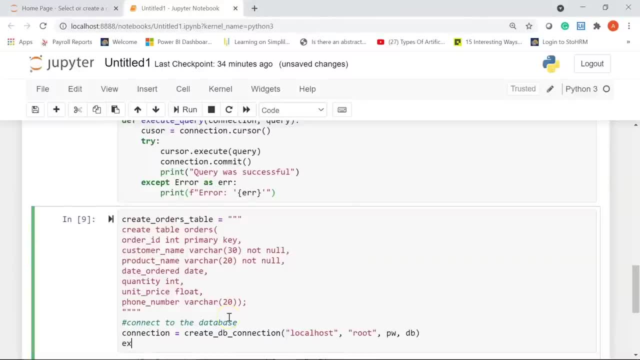 all right. finally, let's execute this query using the execute underscore query function that we created earlier. this takes in two parameter. the first one is connection, followed by the variable name, which is create orders- underscore table. let us run it. okay, there is some error here. let's see what's the error. 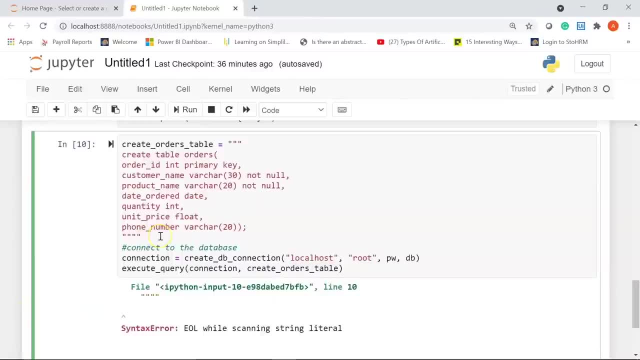 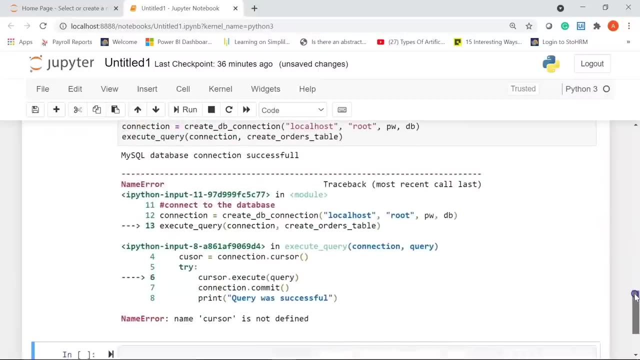 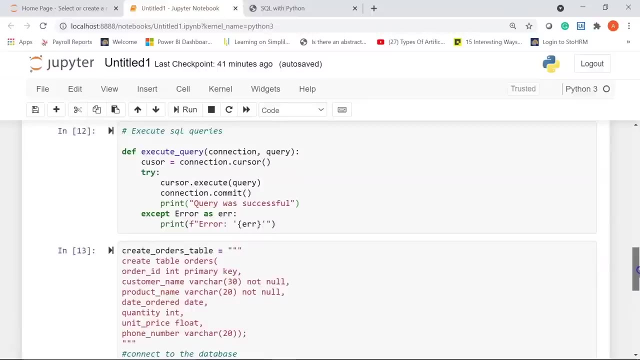 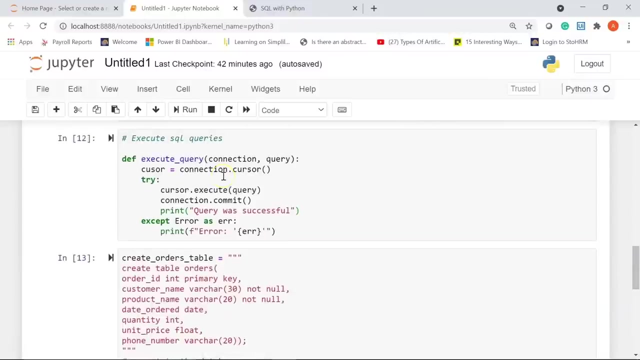 okay, so here we have put four double quotes. this should be triple quotes. now let's run it. okay, there is another here, let's debug it. it says name cursor not defined. let me just roll it to the above cell. if you see here in our execute underscore query, 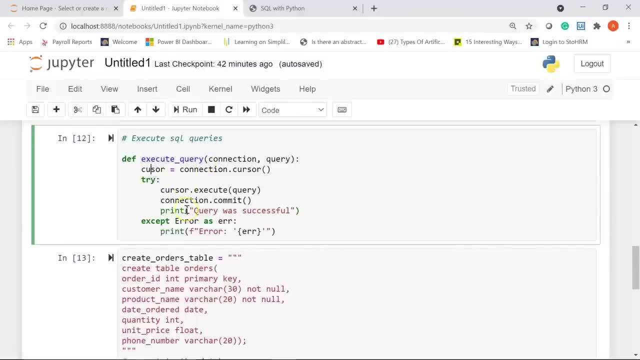 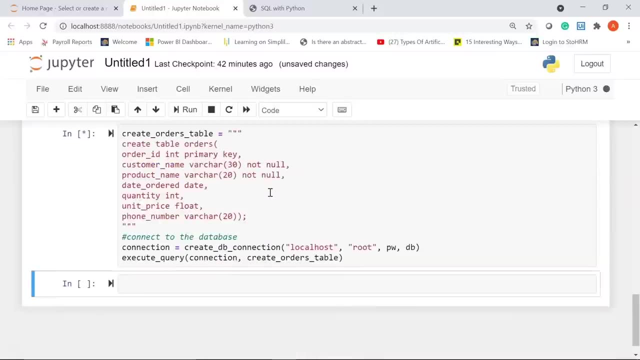 function instead of cursor. i have written cursor, so r is missing. let's redone this. and now let's run this again. there you go. you can see here mysql database connection successful. even our query was also successful. now, if you want to recheck if the table, that is orders, was created or not, you can. 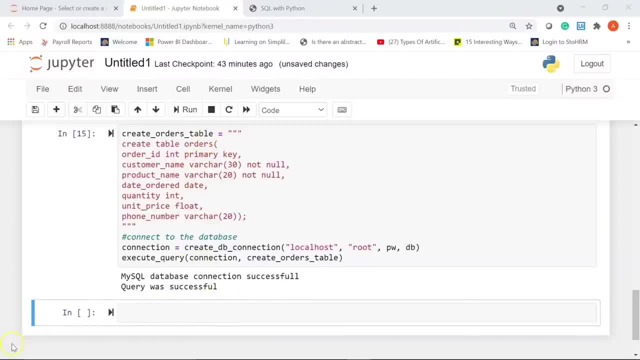 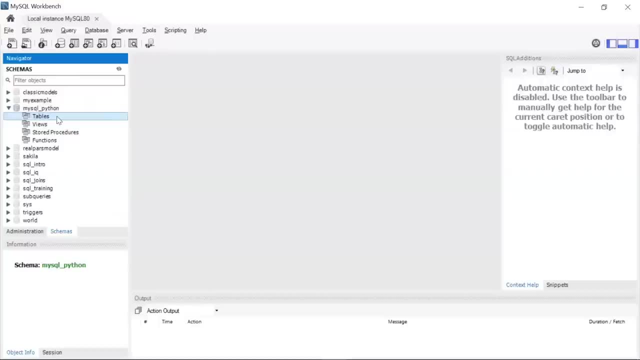 check it on the mysql workbench. so let me show you how to do it. so i am on my mysql workbench and under mysql underscore python database, you have something called as tables. let me just right click and i'll select refresh. all there you go. you can see this arrow. just click on this arrow. 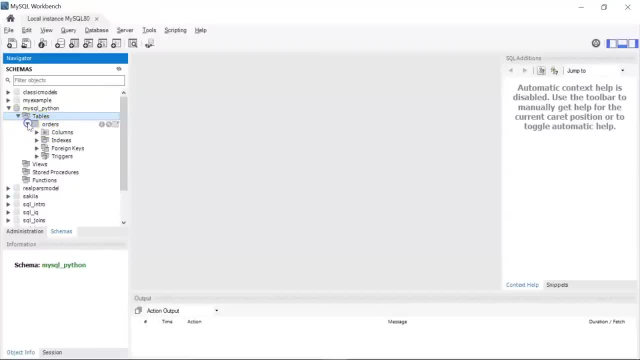 and here you can see we have a table called orders. so we have created our table called orders. now you can check the columns as well. you have the order id. you have the order id, the customer name, product name, ordered date, quantity, unit, price and phone number. now it's time for us to insert. 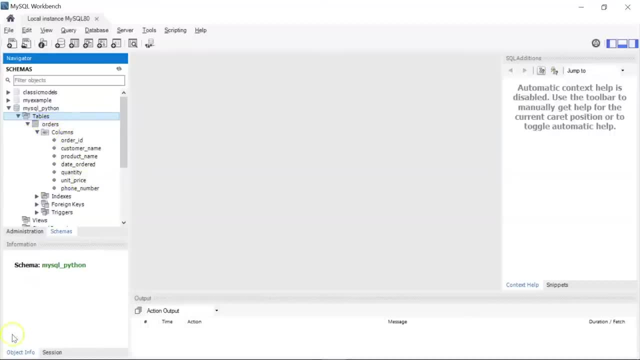 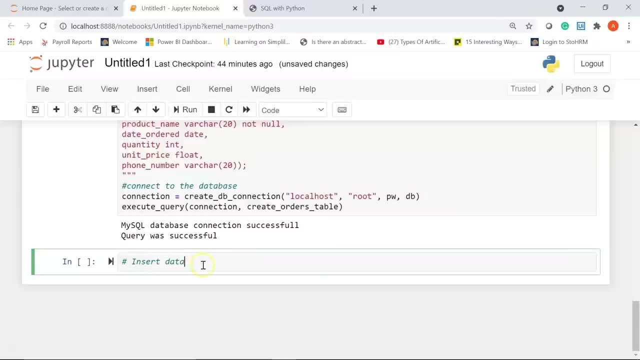 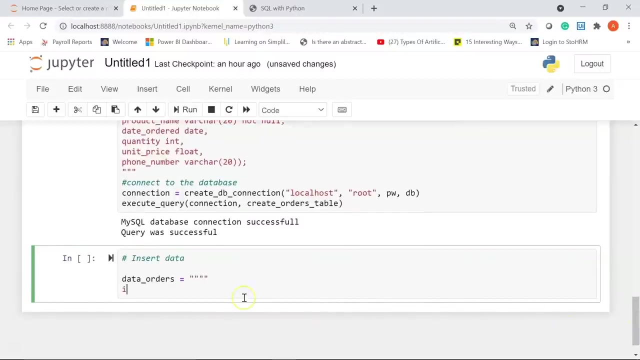 a few records to this table, which is orders. now to insert records, i'll give a comment as insert data. i'll start with the variable name. let's say the variable name is data, underscore orders. i'll give triple quotes. next i'll write my insert into command. so i'll write insert into my table name. that is orders. 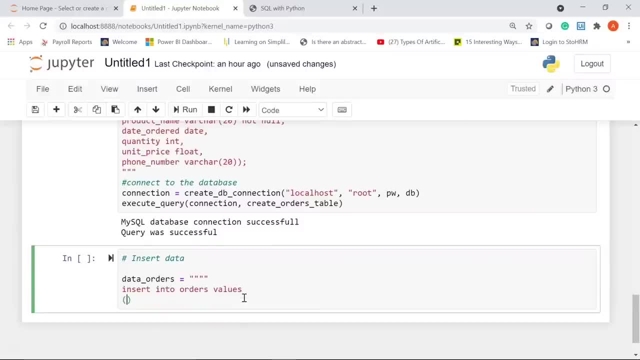 followed by values, and now i'll start entering my records for each of the rows. so first i'll give 101, which is the order, and then i'll add the record number and then, when i'm done, i'll select the record number and then i'll select. 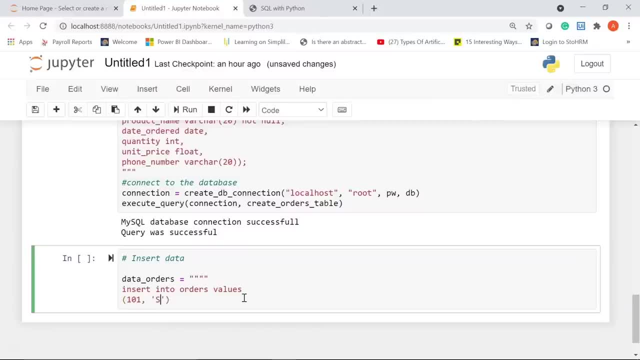 the number and then i'll insert the record number and i'll get the record in my very first cell and than i'll enter the command like i used, so you order ID. then I will give the customer's name, let's say Steve, and the product: he. 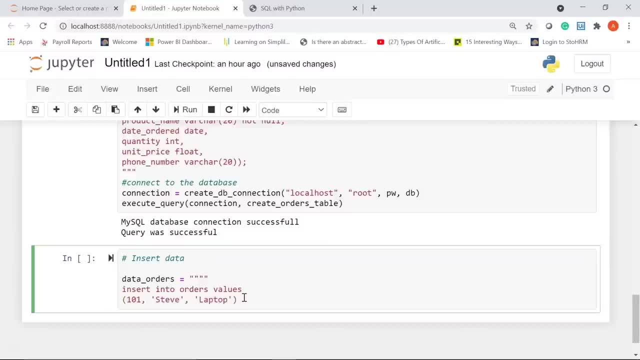 had ordered is, let's say, laptop, then I will give my date in which the item was ordered. let's say it is 2018. I'll choose 06 as the month and the date is, let's say, 12. you give another comma. this time we'll pass in the quantity, which is 2. 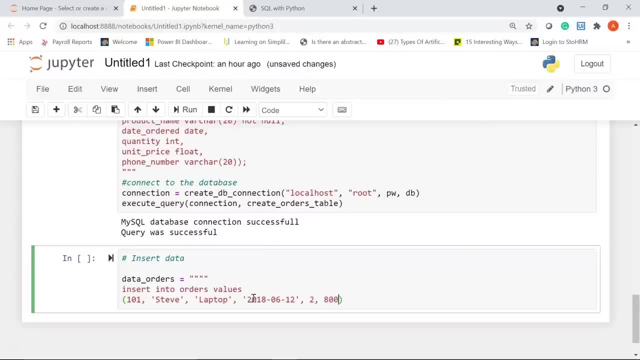 let's say, the price of each laptop was $800 and we'll give a phone number. this is random, let's say 6, 2, 9, 3, 7, 3, 0, let's say 802, all right. similarly, I am going to insert: 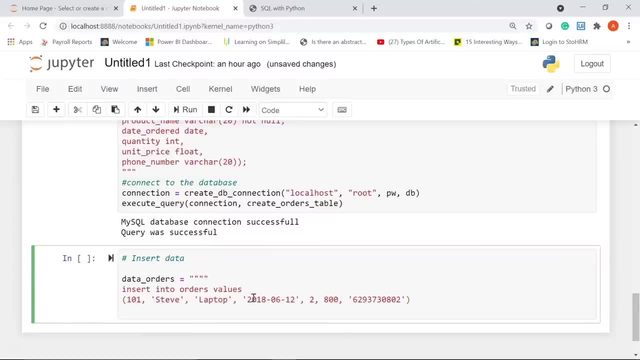 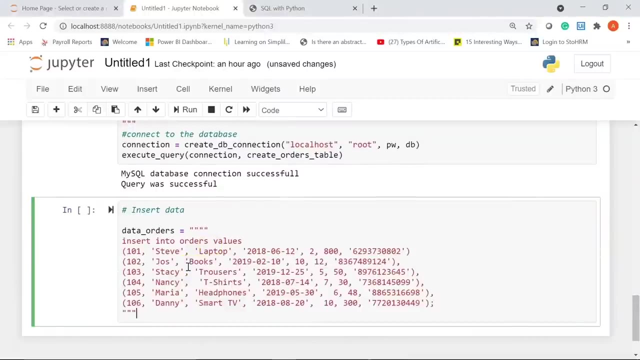 five more records of different customers and their items that they have purchased to this table orders. so here on my notepad I have my rest of the five records. let me just copy it and we'll paste it in the cell here. this will save us some time. okay, let me recheck. if everything is fine, I'll give. 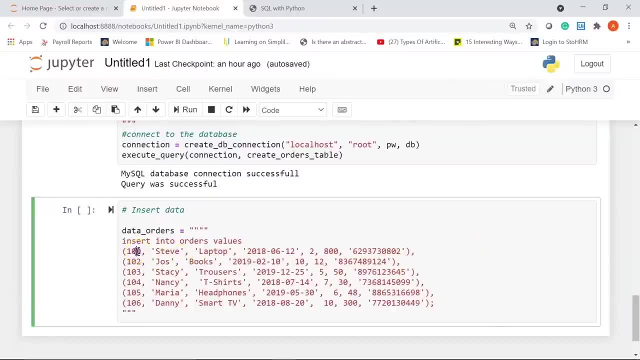 a comma here. all right, so we have six customers in our table which have their customer IDs, from 101 to 106. you have Steve Jaws, Stacy, Nancy, Maria and Danny. you have the different items they have purchased: laptop, books, trousers, t-shirts, headphones and smart TV. is the date on? 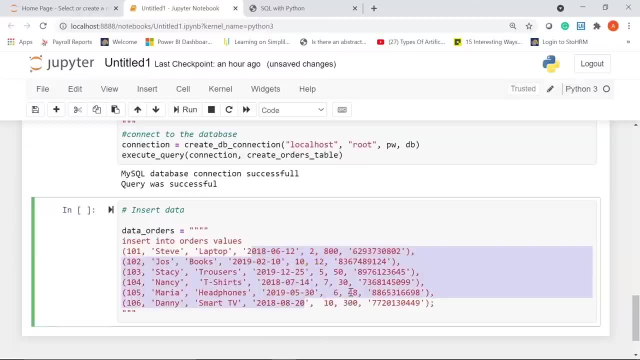 which they had ordered this item, the number of quantities they had ordered, and then we have the unit price and some random phone numbers. so let's create the connection now. I'll write connection equal to. I'll write: create underscore DB, underscore connection. then I'm going to give my same parameters. let me just copy. 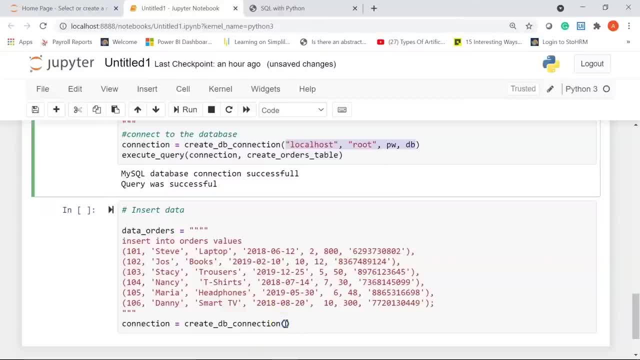 it from the top, which is localhost. the host name root is my username, then we have password and the database name and then I'll use the same query as above, which is execute query. I'll copy this, paste it here and, instead of create orders table variable, I'll put as data. 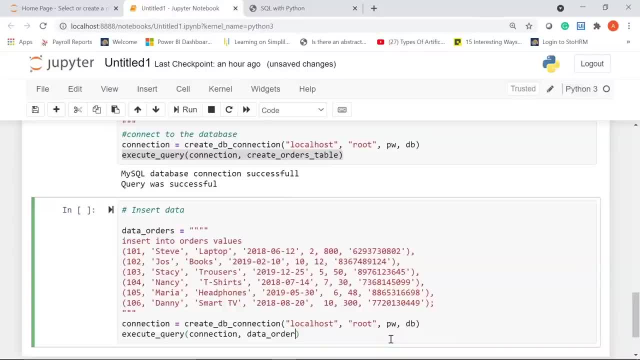 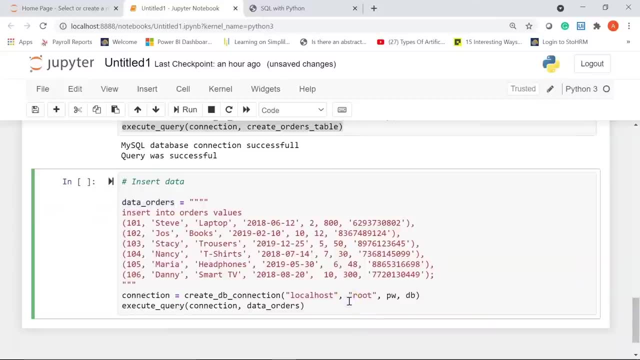 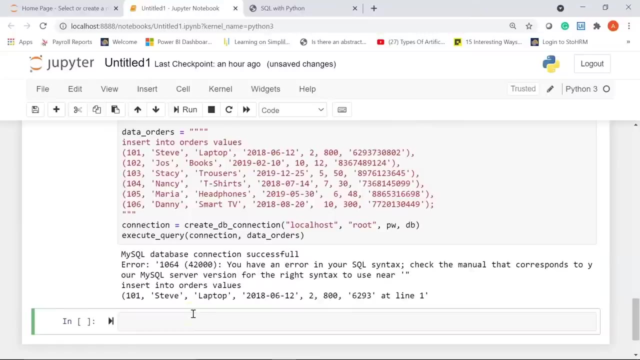 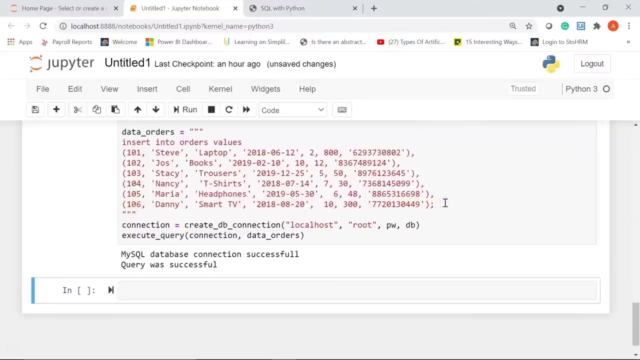 underscore orders. so this will store my insert into command. you can see the variable I've used here is data underscore orders. now it's time. let's just run it all. right, there was some mistake here. let's debug it again. this would be triple quotes and not four. now let me rerun it again. 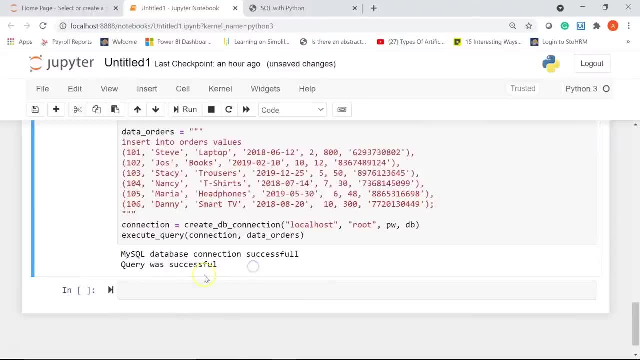 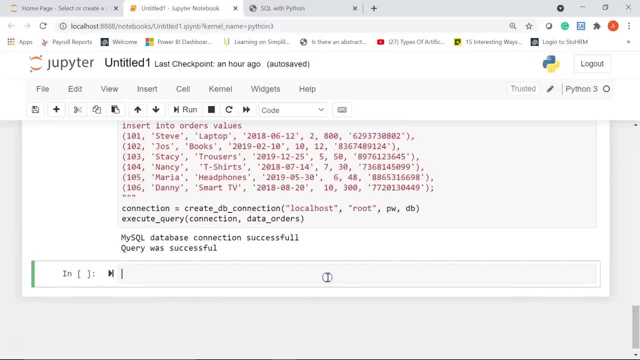 there you go. you can see here my SQL database connection successful and my query was also successful. we'll create another user defined function which will help us read query and display the results. so I'll write my function name as DF: read underscore query. this will take in two parameters: connection and query. then I'll write cursor equal to connection dot. 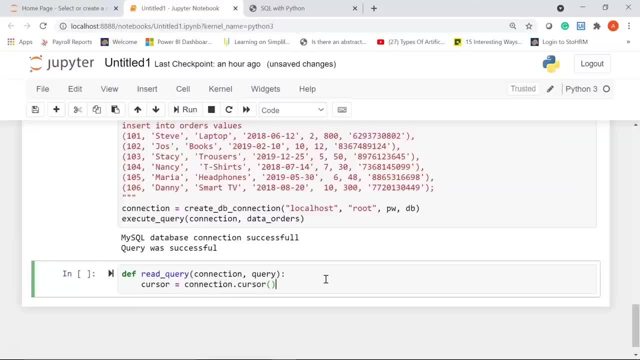 cursor, I'll put my result as none and then I'll use my try and accept block. I'll write try- cursor dot- execute. this will take in one parameters, which is query, and then I'll give another variable, which is result, equal to cursor dot. fetch to the NK file order. I'll just connect. 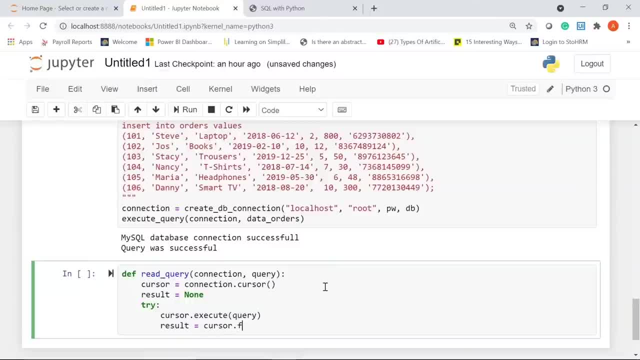 multipletag here, which we've been doing before, and you can have those tamaF query as equals to the NK file. again, we'll see this one as an example URL and this will give me a fiquei ing in all, and then you can also run this in the command. run this return 14 as well, which 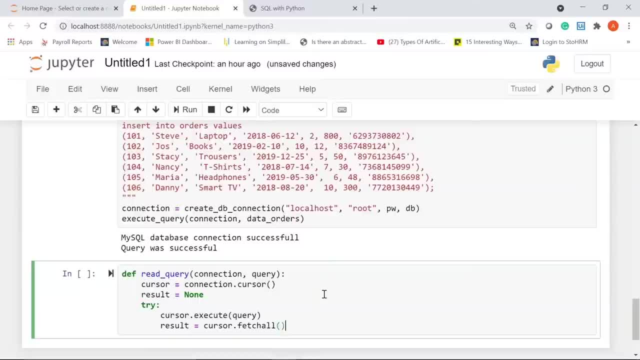 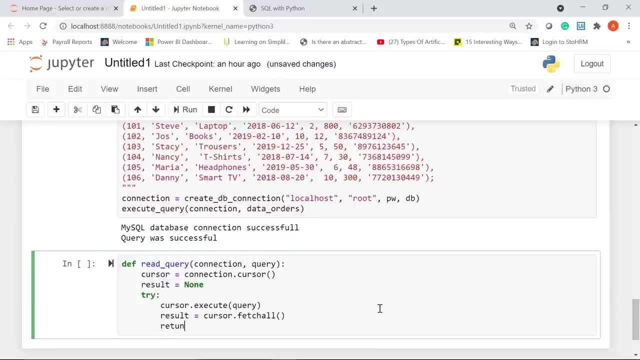 also requires two things. we will run in and then I'll say create and then you can enter those all. now this fetch all method will return all the results in the table. I will write return result. next, we will use the accept block so I will write accept error as err. 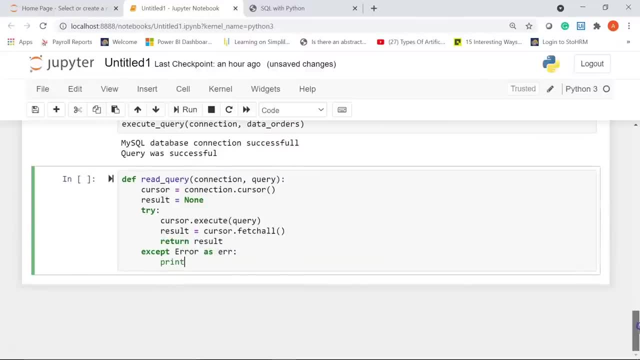 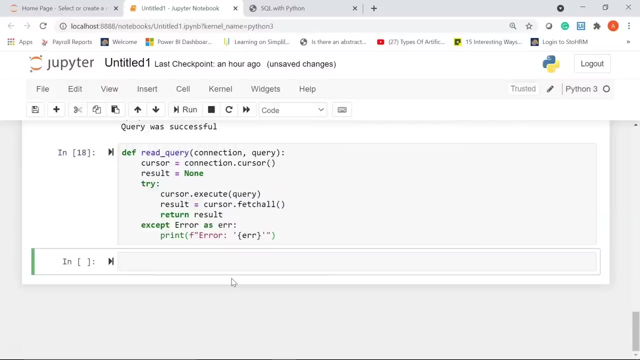 give a colon and I will use my print statement: scroll this down. I will use my formatting f error: give a colon followed by a space within single quotes, inside curly braces. I will give err and close my double quotes. let's run it alright. so now we are all set. now we are going. 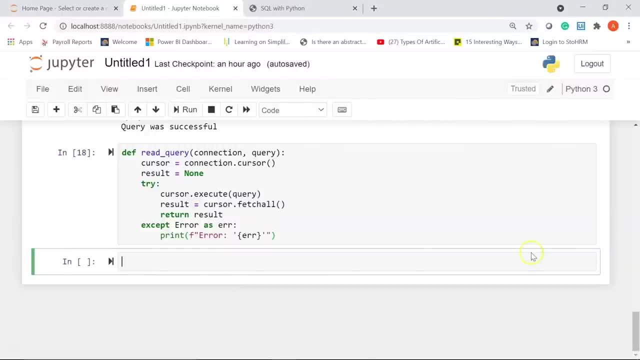 to use our select clause having, whereby then we'll see how to use, order by clause, some inbuilt functions, we'll update some records, delete some records and do a lot of other stuff. so let's start with our first query. so our first query is going to be using the select statement, alright, so suppose 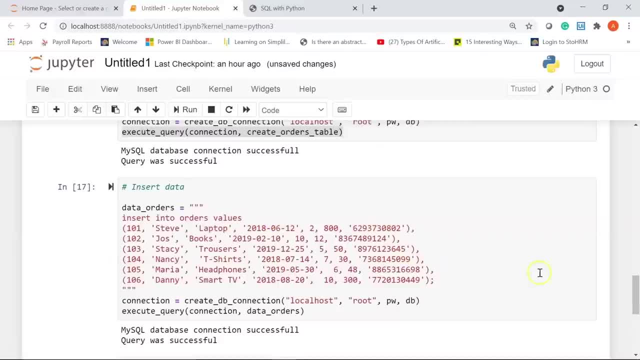 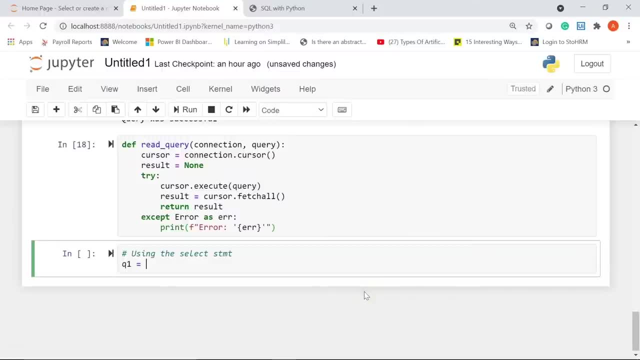 I want to display all the records that we have inserted into orders table. so the way to do is: i'll assign my query to a variable, let's say q1. i'll give triple quotes. within triple quotes i'll write select star from orders. we'll give a semicolon followed by the triple quotes. now we'll establish the connection. so 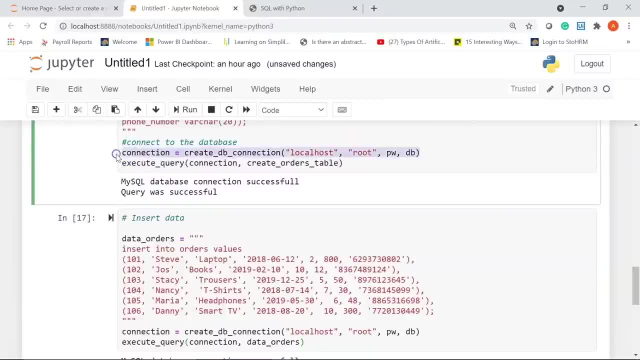 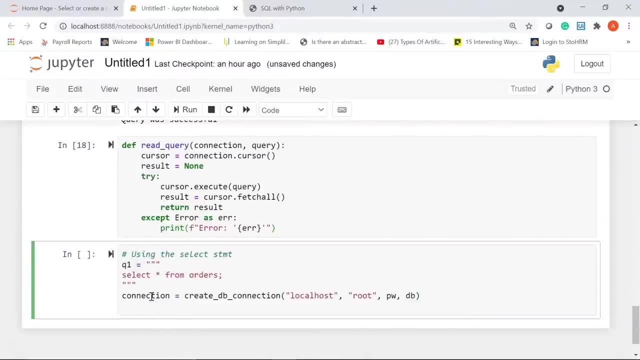 let me just go to the top and i'll copy this line, which is to connect to our database. i'll paste it here now. we'll create a variable called results that will store the result of this query and we are going to assign this variable to our function, that is, read query. 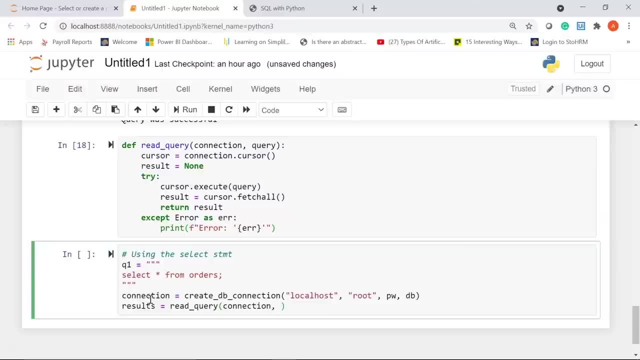 and this read query will have two parameters: the connection and the variable name, which is q1, for the query next to display. i'm going to use a for loop. i'll write for results for result in results print i'll say result. now we are done, let's just run this query. there you go. you can see, here you have. 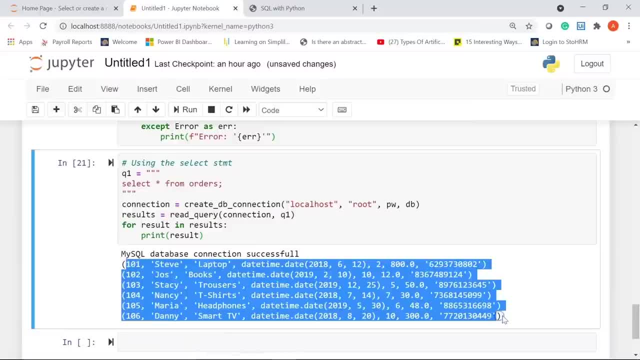 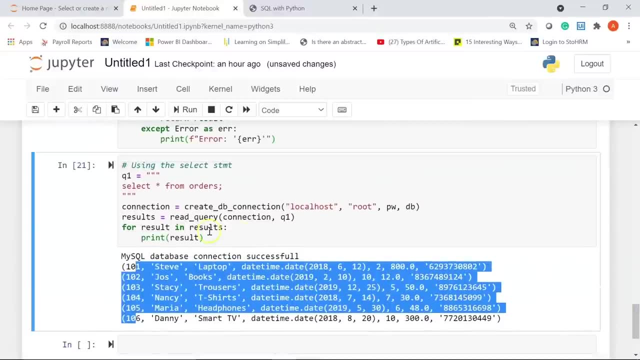 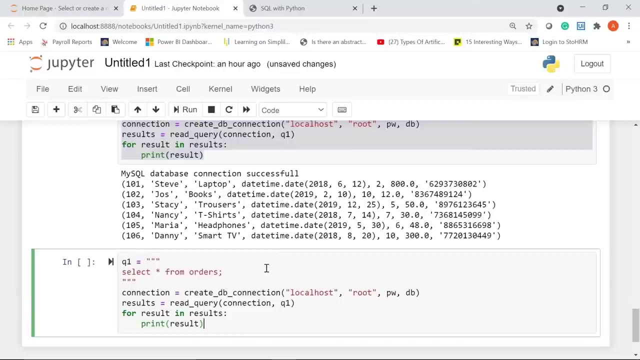 successfully printed all the rows in our table, which is orders. you can see we have six records in total. now we are going to explore a few more queries, so let me just copy this and we are going to edit in the same query. i'll paste it here. next, let's say you want to display: 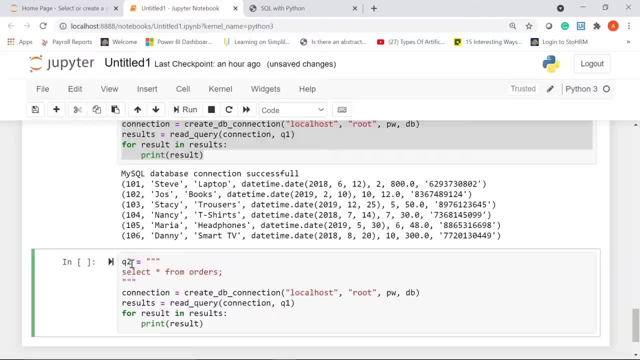 individual columns from the table and not all the columns. so let me, let me create the variable q2. now, instead of star, i am going to display only the customer name and let's say the phone numbers of the customer. so i'll write phone underscore number. all right, the rest all remains the same. let me just recheck it and here, instead of: 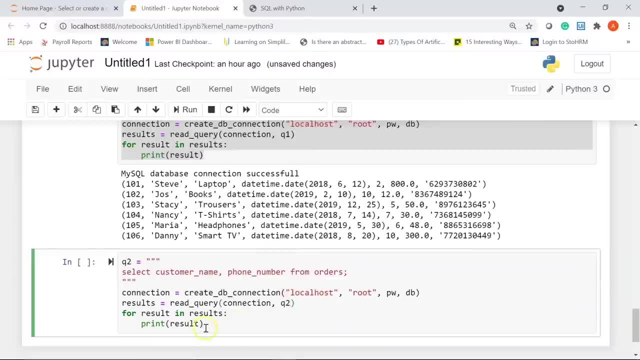 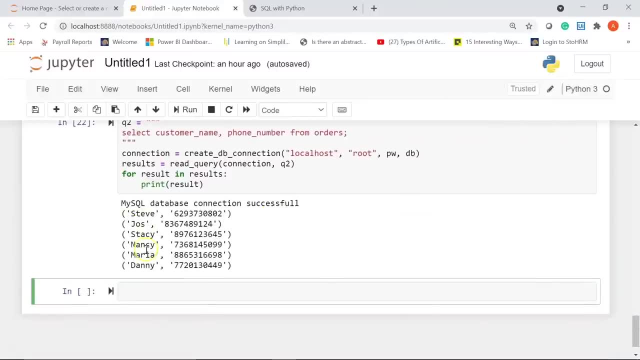 q1 will put q2 and let's run this cell. all right, you can see, here now we have displayed only two columns. the first column is the customer name and then we have our their respective phone numbers. okay, now let me just paste that query again now. 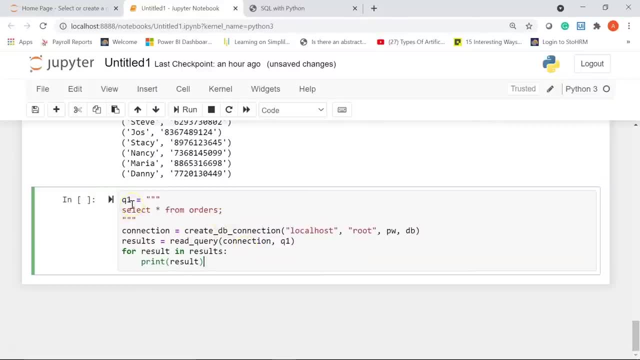 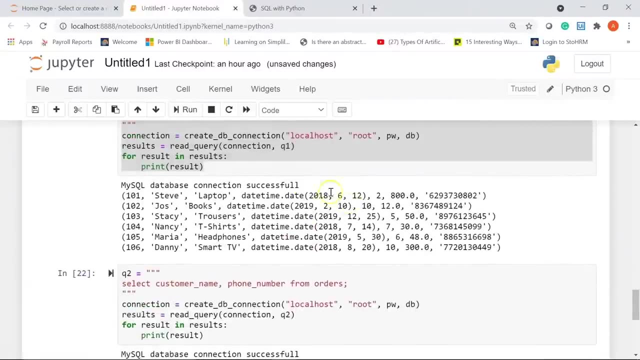 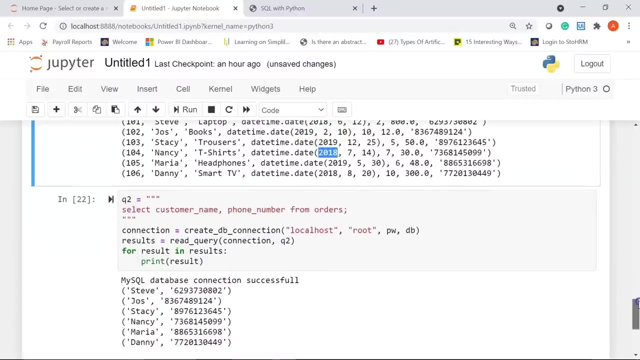 we are going to see how you can use an ill-built function that is in our table. we have the order date and from the order date we are only going to display the different years that are present in the order date. so to do that, I am going. 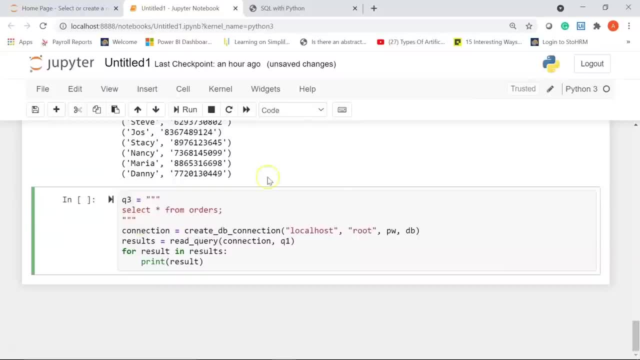 to use the year function, I let this query. instead of q1, I'll make it q3, and here I am going to write select year, which is my function name, from my column, which is date ordered from orders, and here I'll change this to q3. q1, q2, q3 are. 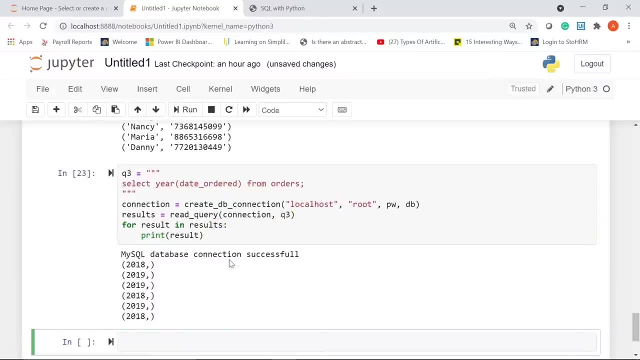 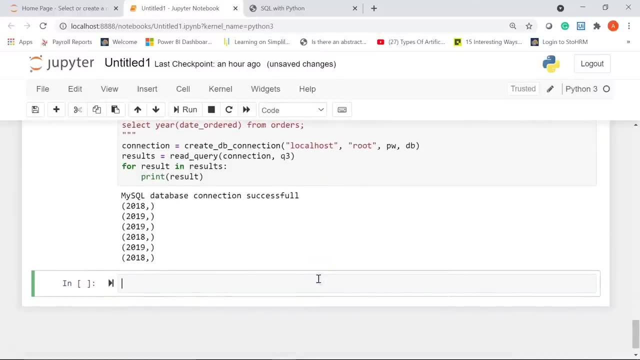 basically query 1, query 2 and query 3. let's run it. there you go. so we have successfully done that and now we are going to see how we can use this function. extracted the different years present in the order date column. now, if you want. 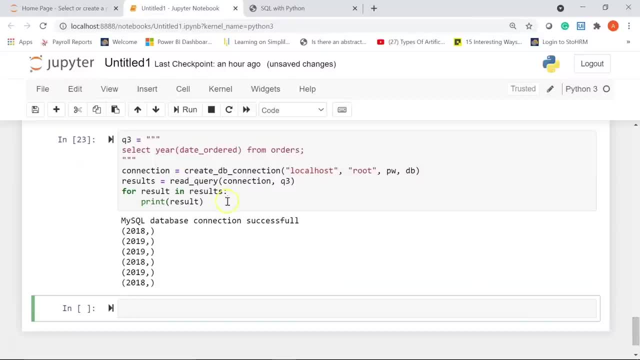 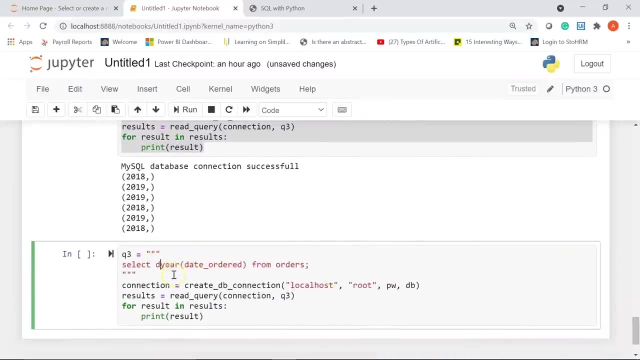 to display the distinct or the unique dates present in the column. you can use the distinct keyword in the select statement. so the way to do it is: I'll write select distinct. give a space. the rest of the query remains the same and here in q3 I'll write q4. I'll make this as q4. 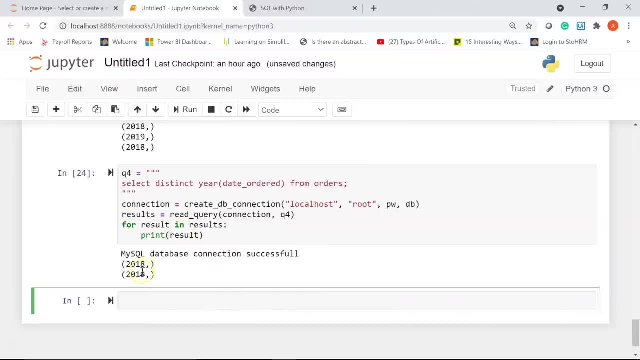 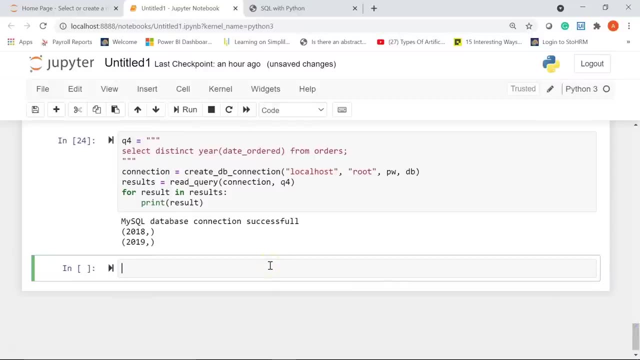 let's run it. you can see, 2018 and 2019 are the unique Зна grinding values that are present in the order date column. ok, now moving ahead, let's write a fifth query, and this time we are going to explore how you can use the. 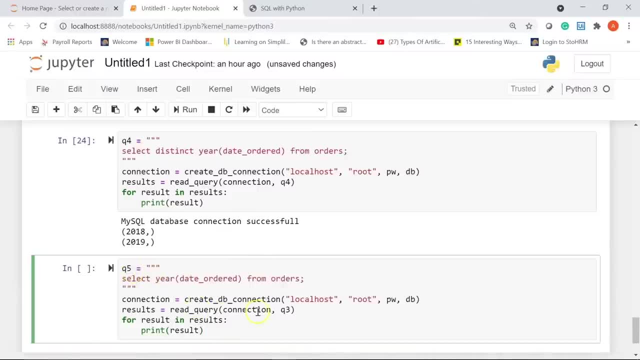 varc проj idea: draw where clause. so I'll change this to q5 before I write my. this will be q4 in order date column. so let's say you want to display all the orders that were in this particular可愛 in order date, for I will type in add, before voting, the order date into the order date column. solutions should need to be amazingly clear. O chef, choose adults three. order straight away". 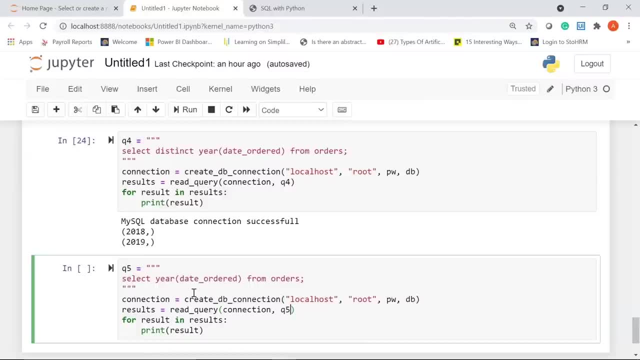 ordered before 31st of December 2018. so to filter this, we are going to use the where clause, so I'll write select star from orders. next, I'll write: where my date underscore ordered is less than within quotes, I'll give my date value, which is 2018, December 31st. so all the items or the products that were ordered. 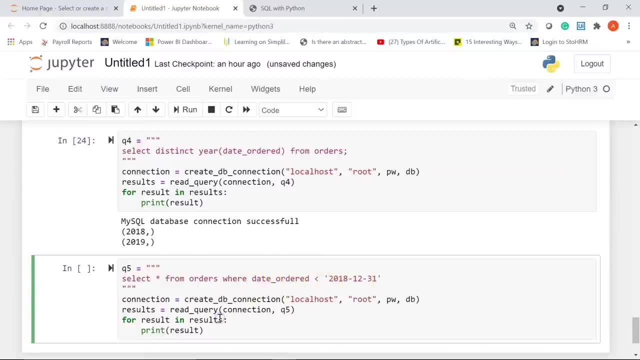 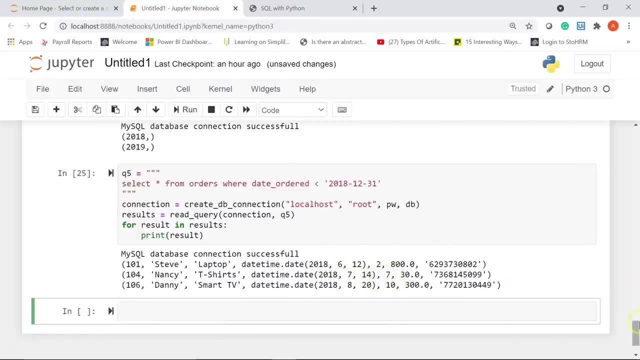 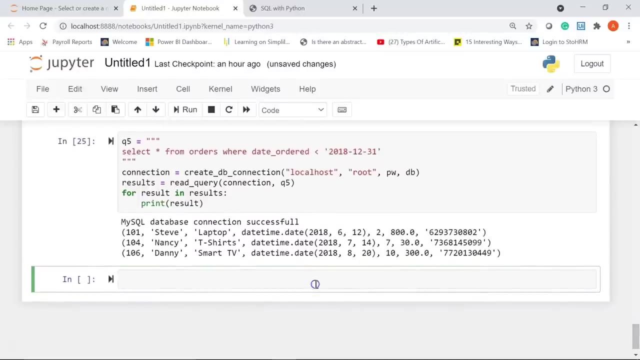 before 31st of December 2018 will be displayed. so let's run it all right. you can see here there are three orders in our table which have been ordered before 31st of December. now, moving ahead, we want to display all the orders that were made after 31st of. 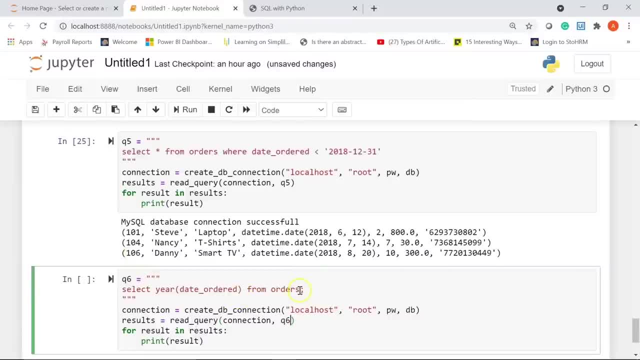 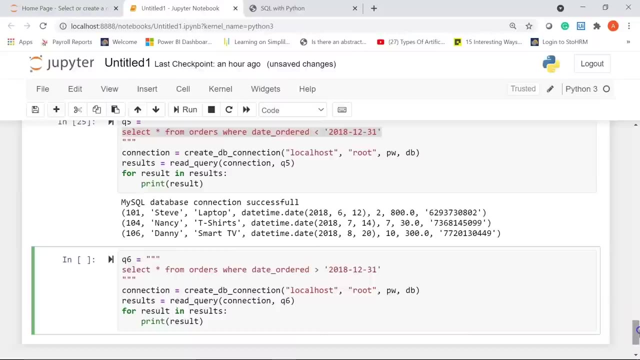 December. so here what you can do is I'll just copy the above query again. I'll copy this line. so, instead of less than 31st of December 2018, I'll make it as greater than so every order that was placed after 31st of December 2018. 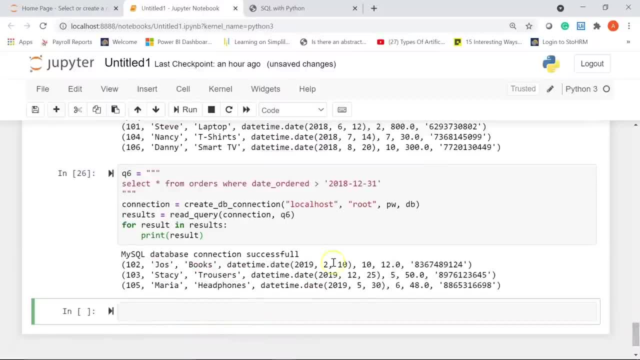 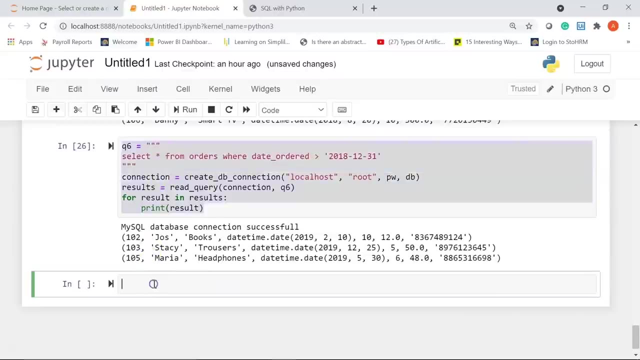 Macron is given one. by the number of items you want to display savory, you run it. so you can see here there are three orders in our table which were ordered after 31st of December 2018. now, moving ahead, let's write a seventh query. 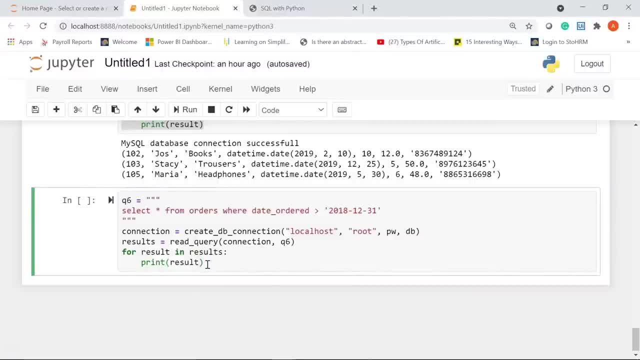 now let's see how the order by clause works in SQL, so you can filter your results based on a particular column or sort it based on a particular column, and So this is going to be my query 7, I'll write it from scratch again. let's say you want. 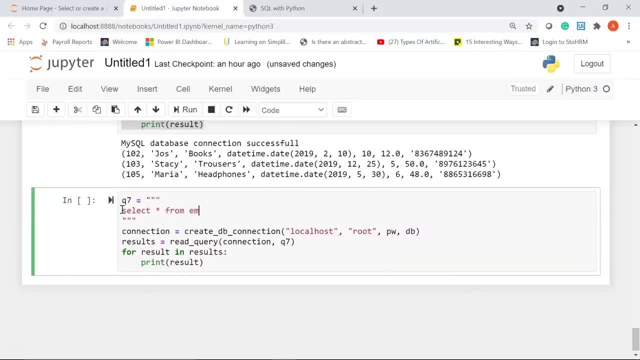 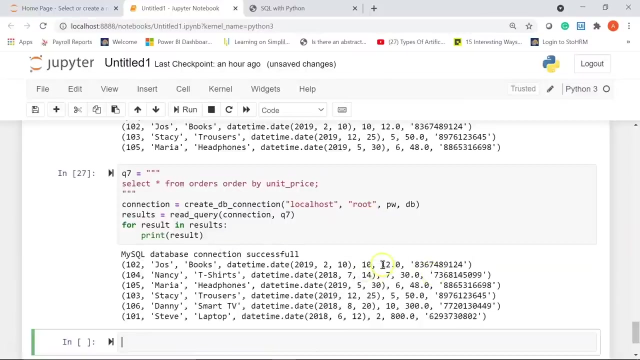 to display all the columns from the table. so I'll write select star from orders. then I'm going to use order by unit price. I'll give a semicolon. let's run this query and see the output. if you see the result here and you mark the unit price column, the result. 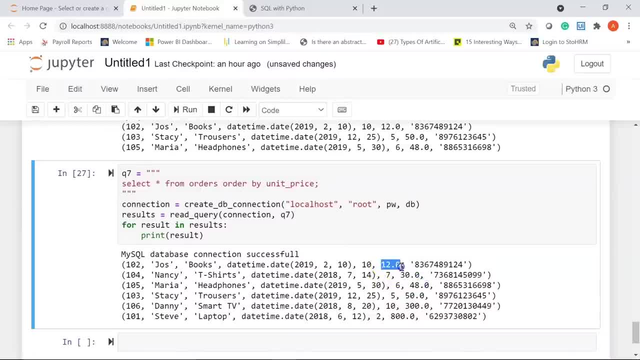 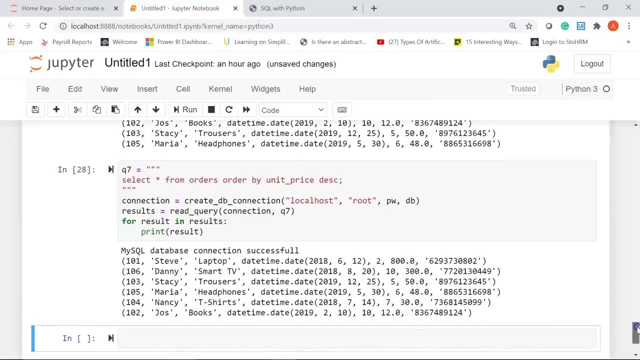 has been ordered in ascending order of unit price. you see here it starts with the lowest price and then goes on with the highest price towards the end. now, if you want to order it in descending order, you can use the keyword DESC, so this will ensure your top or the. 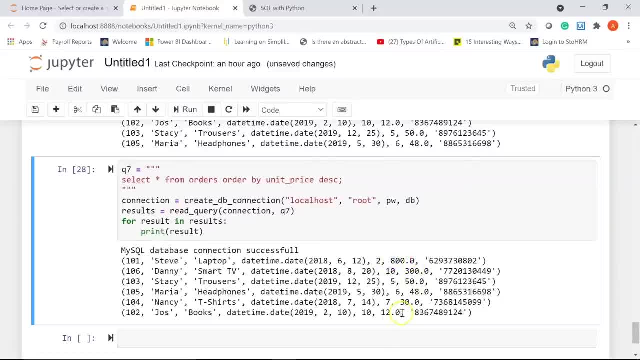 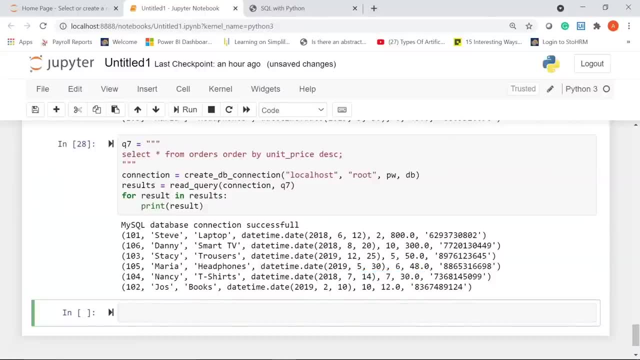 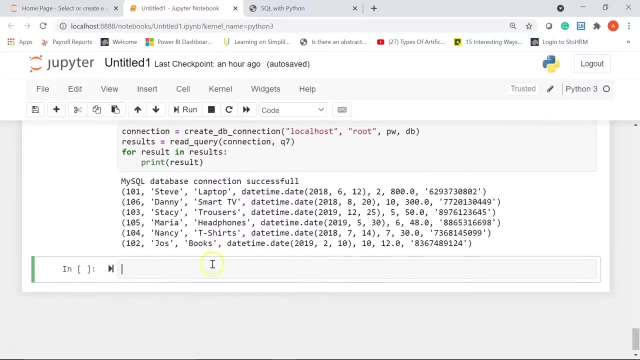 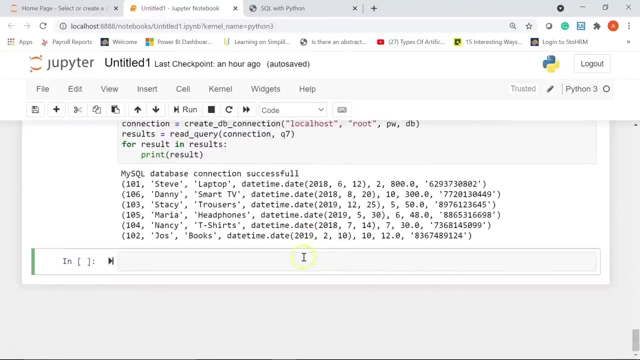 most expensive products appear at the top. Next, let's see how you can create a data frame from the given table. so, as you know, using Jupyter notebook and pandas, you can create data frames and work on it very easily. so with this table also, we can create our own data frame. so for that, let me create. 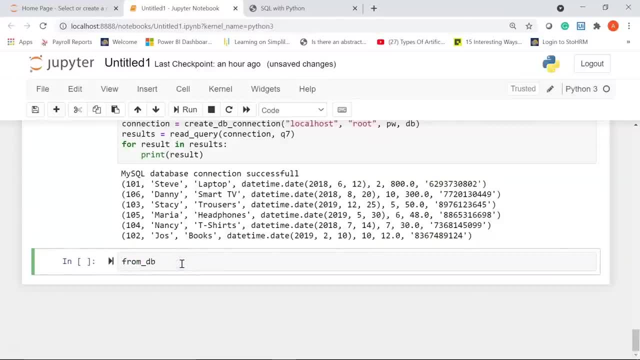 an empty list. first I'll write from DB equal to. I'll assign this as an empty list. so we are going to return a list of lists and then create a pandas data frame. next I'll write my for loop. I'll write for result in results. I'll assign result to list of results. so I'm converting the. 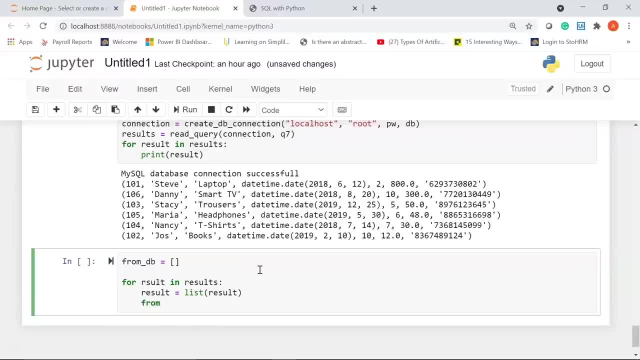 result into a list And then I'm going to append it to the empty variable or the empty list, which is from underscore DB dot append. I'll append the result to my empty list. next we need to pass in the columns. now that will be part of our data frame, so I'll write columns equal to: 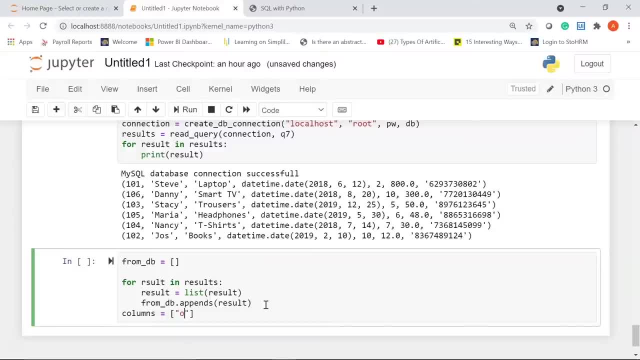 this column. I'll pass it within a list. so I'll give my first column as order ID, then we have the customer name, next I have my product name, then I have the date on which it was ordered. give a comma. 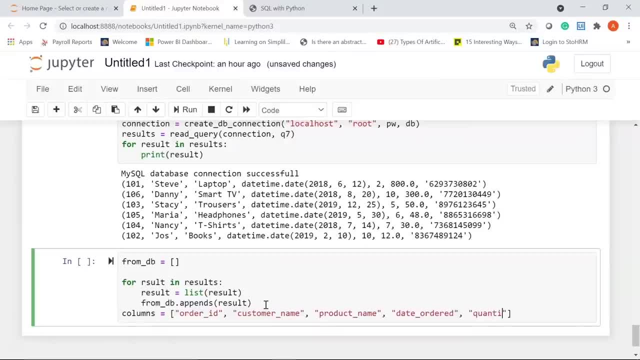 Okay, Give a comma, then we'll have the quantity column. let me write it in the next line. Next we have the unit price column and finally we have the phone number column. so I'll write within double quotes phone number and this. we are going to assign it to a data frame. 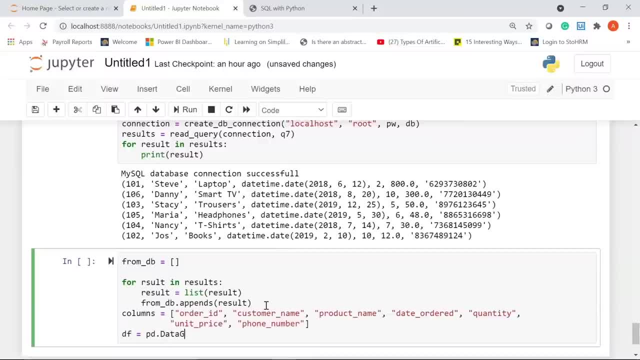 so I'll be using PDF, PDF dot data frame, which is my function, to convert a list into a data frame. My variable I'm going to pass is from underscore DB and I'll write. my next argument is columns equal to my variable name, that is columns. 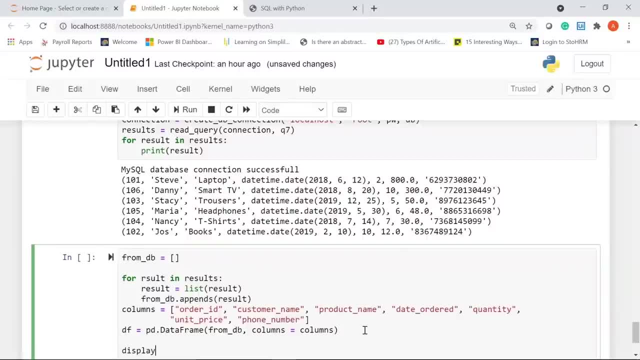 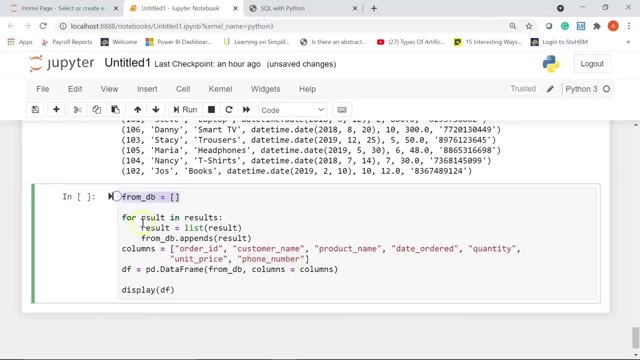 Finally, let's display the data frame, which is DF. Alright, So here I'm creating a empty list first, and then I'm creating a for loop and I'm appending the results to my empty list. Here you can see I have created my column list and, using PDF dot data frame, I'm converting. 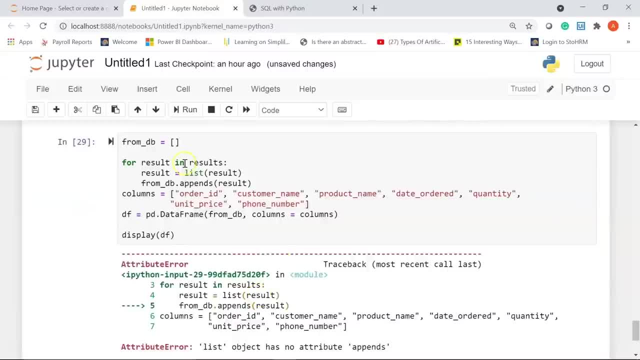 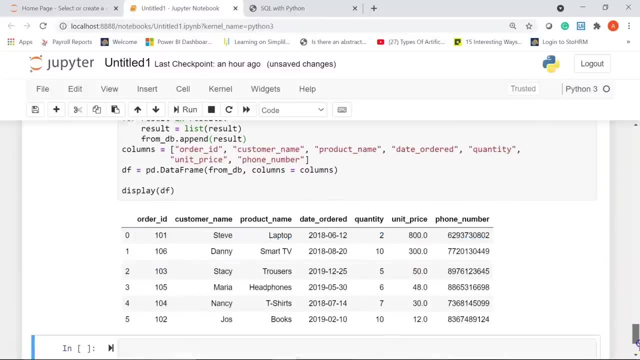 the list into a data frame. If I run this, this is append and not appends. alright, you can see. we have our data frame ready. This is the index column. it starts from zero onwards and then we have the different column. 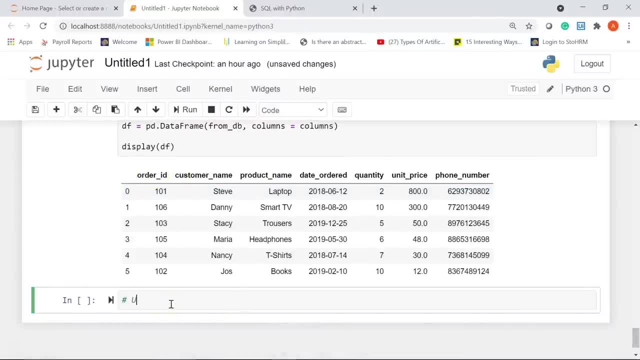 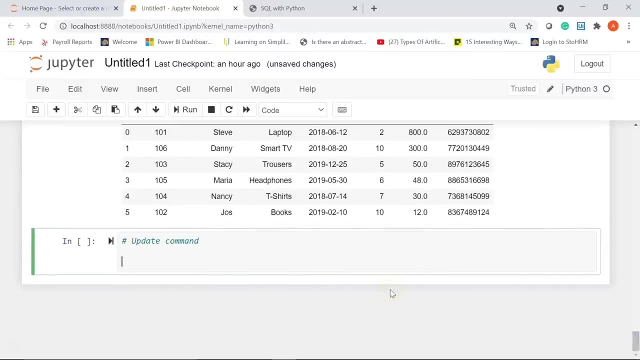 names. Okay, Now let's see how to use the update command. Now suppose you want to change the unit price of one of the orders. you can use the update command. So the way to do it, I'll first create my variable, let's say update. 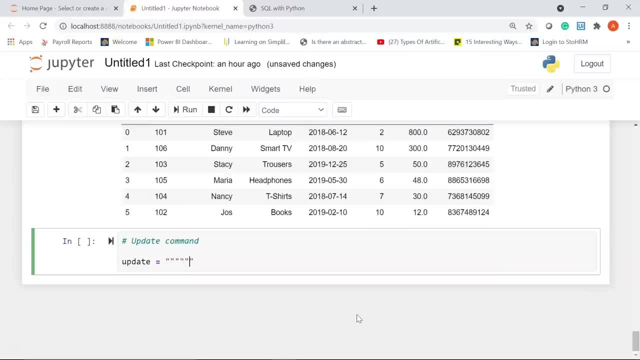 And I'll create my variable. Okay, So I'll give three quotes, or triple quotes, Then I'll use my update command, which is update, followed by the table name, that is, orders. Next I'll write set, let's say unit underscore price. 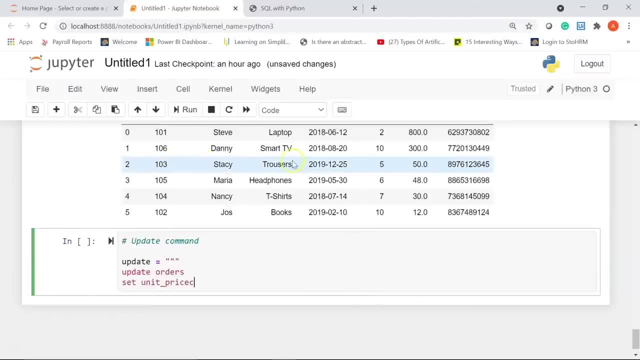 If you see this. let's say I want to set the unit price of trousers from $50 to, let's say, $45.. I want to update this particular record, So I'm going to write: set unit price column equal to $45.. Where the order ID equal to 103.. 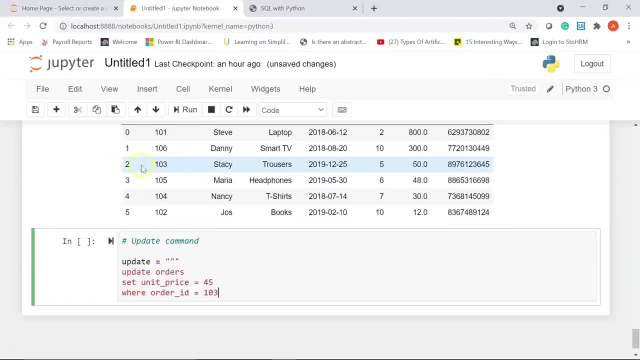 So this query will update the third row in our table, which is order ID 103.. So it will update from $50 to $45.. I'll close the triple quotes And now I'll use the table name. Okay, Okay. 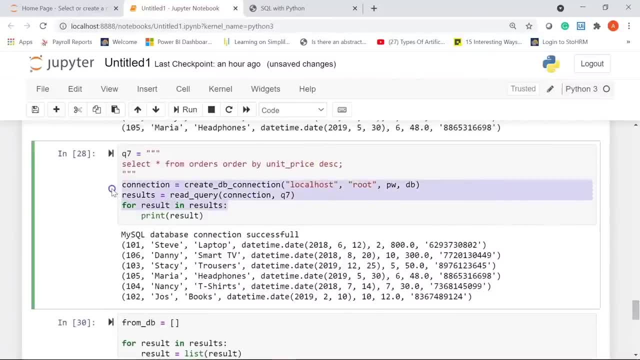 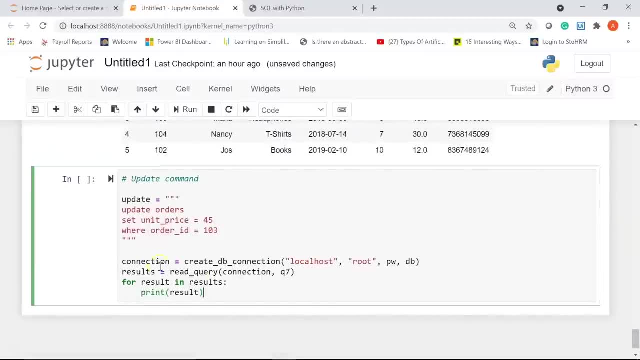 Let's create my connection Connection queries again. Let me just paste it here. All right, I'll delete these three lines of code and instead of that I'll put execute underscore query And this will take into parameters, as always, which is going to be connection, followed by: 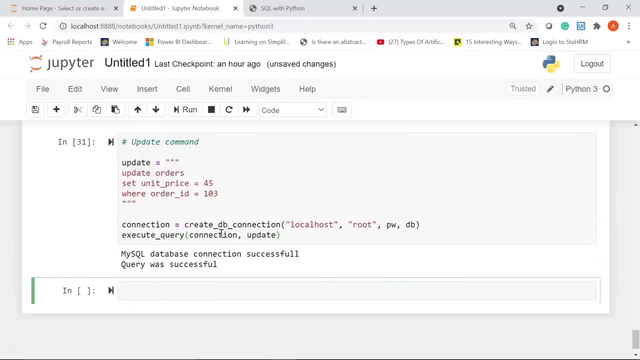 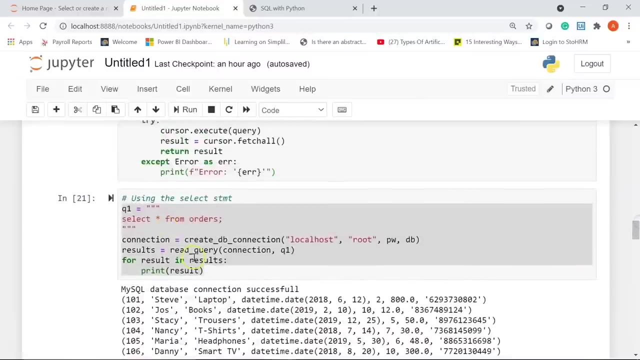 the variable name, that is update. let's run it. you see, here it says mysql database connection successful. query was successful. now you can recheck that. to do it, let me just go to the top and we'll just copy our first query, which is q1. i'll copy this and i'll paste it here. 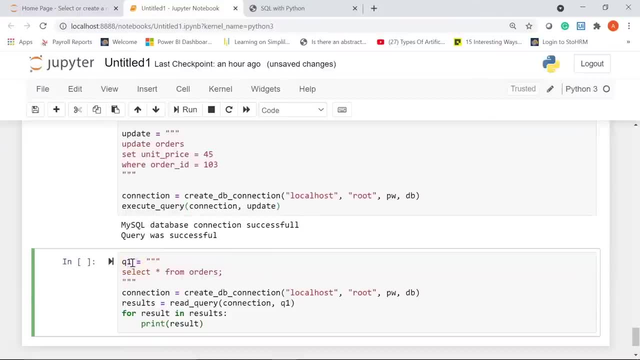 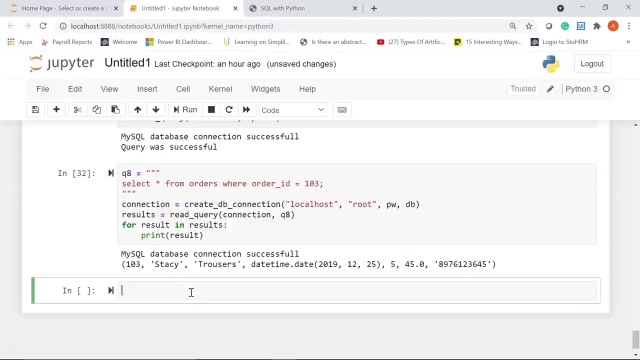 let me just rename this now. this will be q8 and i'll change this as well. i'll write select star from orders where my order id equal to 103. let's see the unit price of 103. now you can see here: instead of 50, now we have updated it to 45 dollars. all right, now the last command we are going to say. 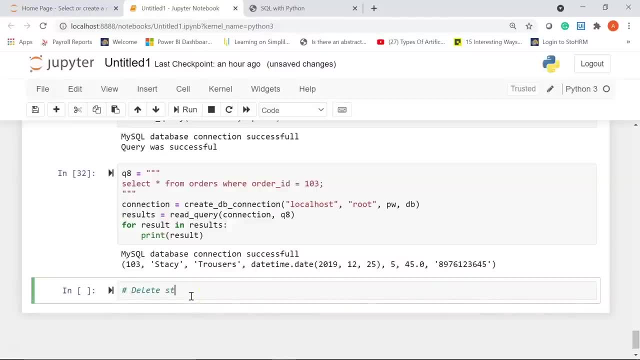 is how you can delete a record from the table. i'll write delete command as my comment. now, to delete a query, i'll first give my variable name, which is delete, underscore order, and i'll pass in within triple quotes. next i'll write my delete query, which is delete from my 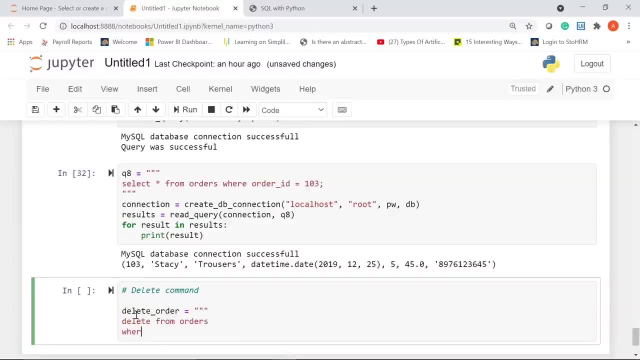 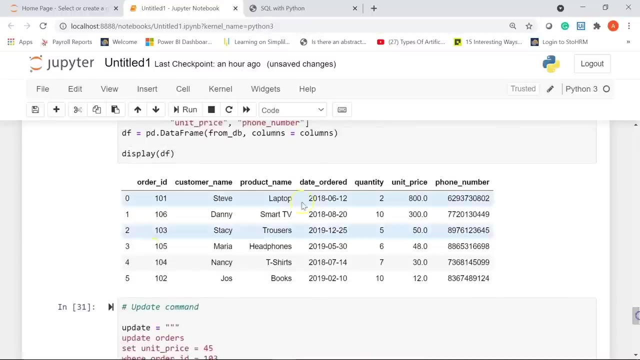 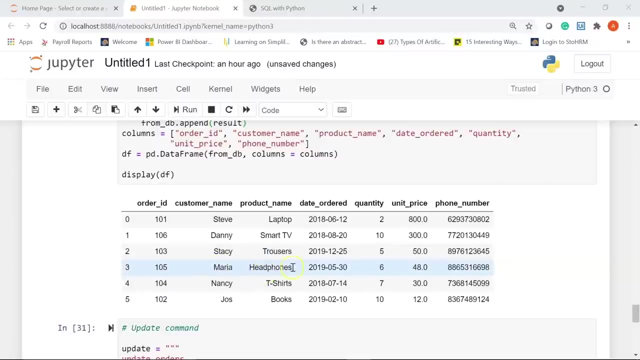 table name, that is orders. then i'll give my where clause where, let's say, i want to delete my order id 105. let me just go to the top and explain you again. so if you say this, we want to delete the order id 105, which was for customer named maria and she had ordered headphones. you want? 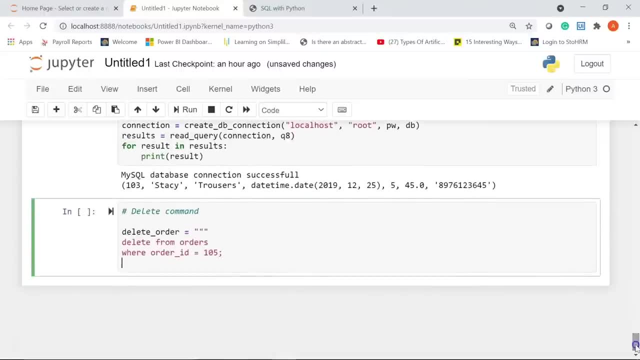 to completely remove this particular record. so i have my delete query ready. now let me just create my connection and display the results. so i'll go to the top and i'll copy this connection command which will actually give auite the question that we just completed and let's see the results now. so i'll go to the top and i'll copy this connection command which also will give me the result. so let me just go to the top and i'll copy this connection command. 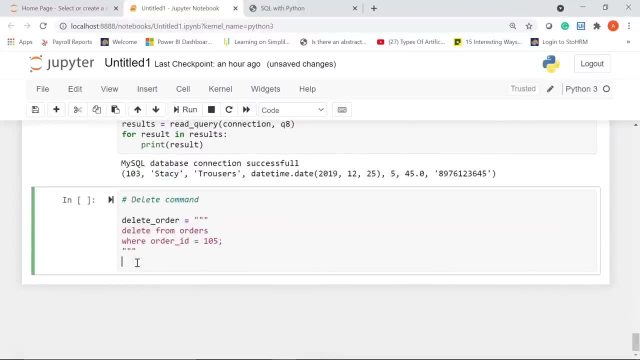 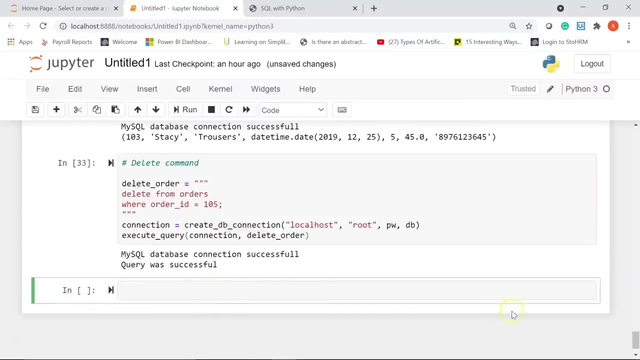 also has the execute query command and I'll paste it here and I'm going to make a change here. instead of update, we'll write delete. underscore order: everything looks good, let's just run it. you can see our query was successful, and now, if you want to print it, let me just 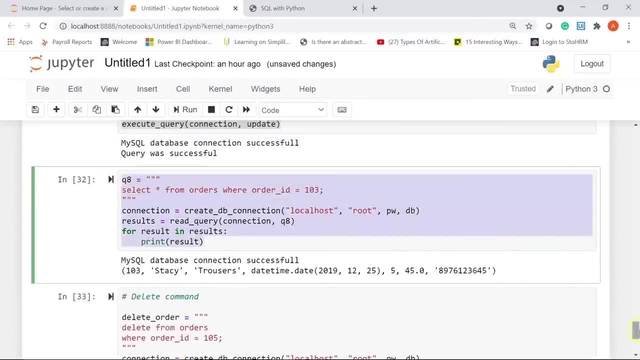 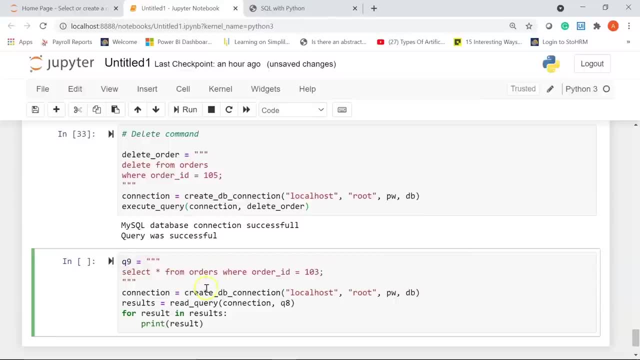 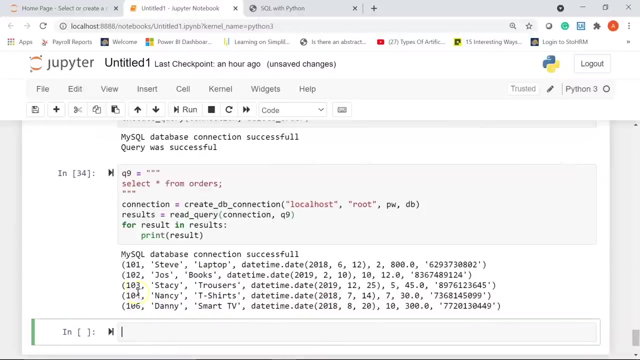 show you. I'll just copy this. we'll paste it here. I'll make this as q9. I want to verify if my order id 105 was deleted or not. instead of this statement I'll write select star from orders and here I'll change this to q9. if I run this, you can see it here. you can mark. 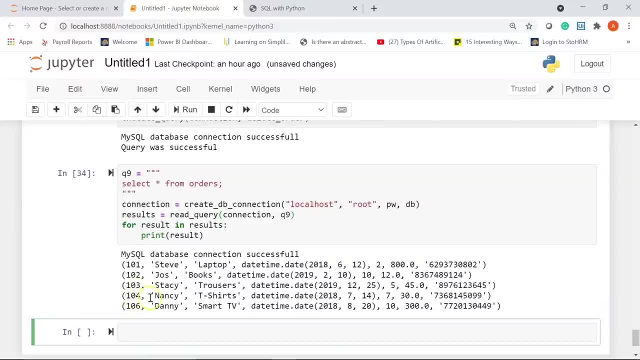 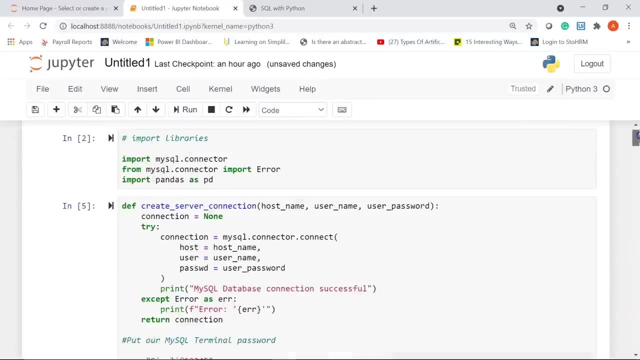 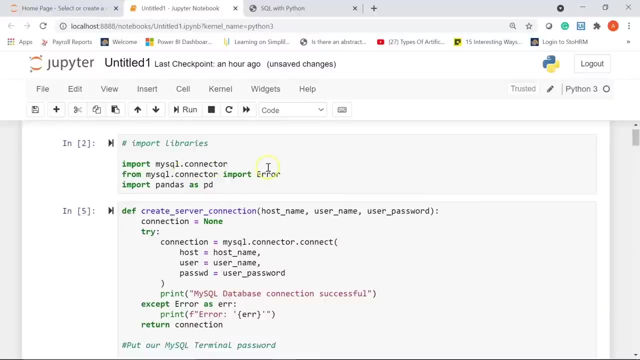 order id 105 was deleted and it no more appears in this table. all right, so this brings us to the end of the demo session on sql with python. let me just scroll you through what we did. so first we imported the important libraries, mysql connector, then we imported the error function. then we imported pandas using pd. 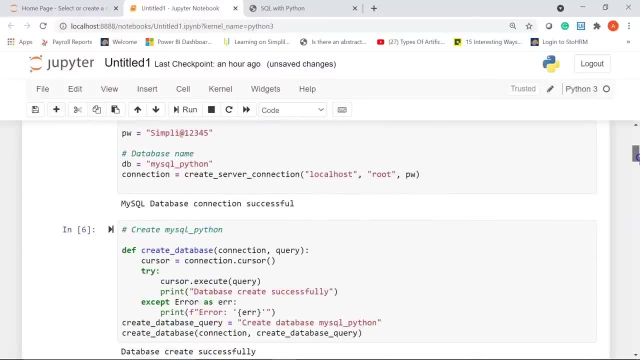 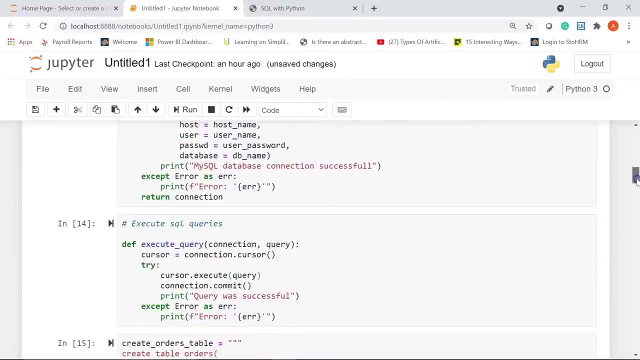 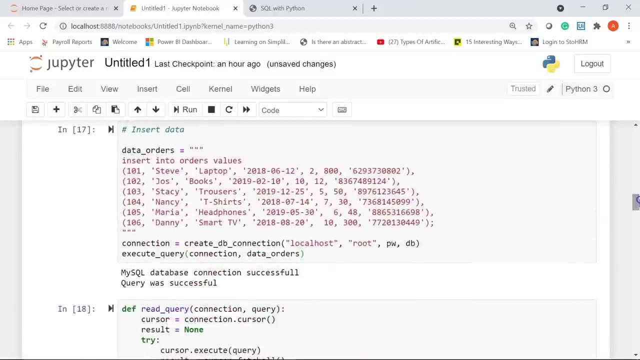 we learned how to create a server connection to mysql database. we created a new database that is mysql underscore python and now we connected to that database. we created a function to execute our queries. we saw how you can write a create table command. then we inserted a few records to our orders table. we created a read underscore query command. 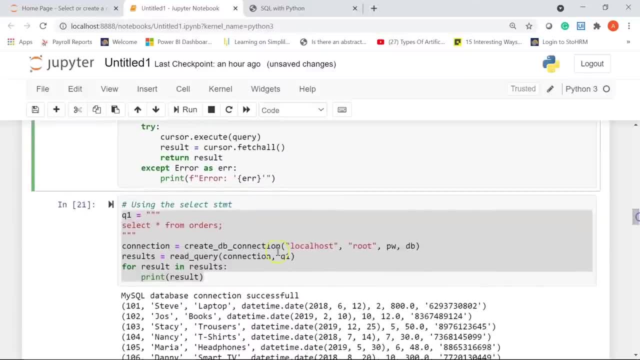 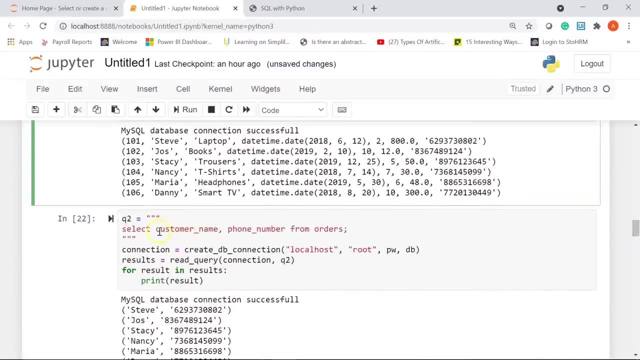 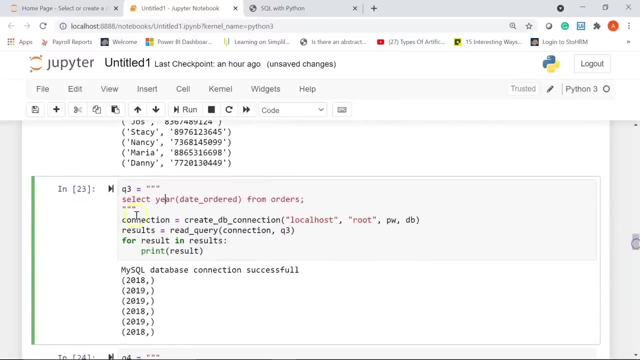 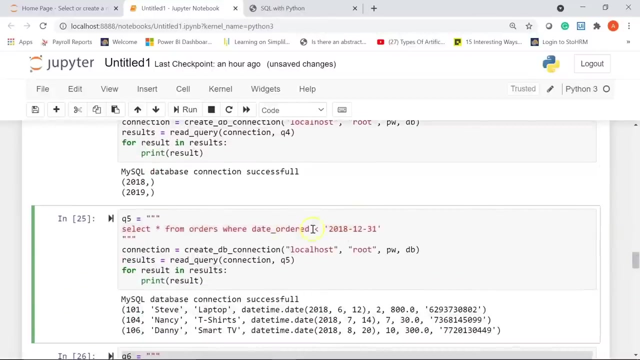 to read the queries and display the results. then we started exploring our different sql commands, one by one. we saw how to use select query. then we selected a few individual columns from our table, followed by using a inbuilt function which was here. then we saw how to use the distinct keyword. after that we used our where clause. 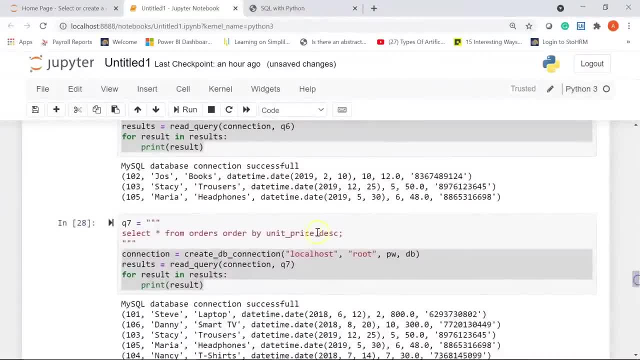 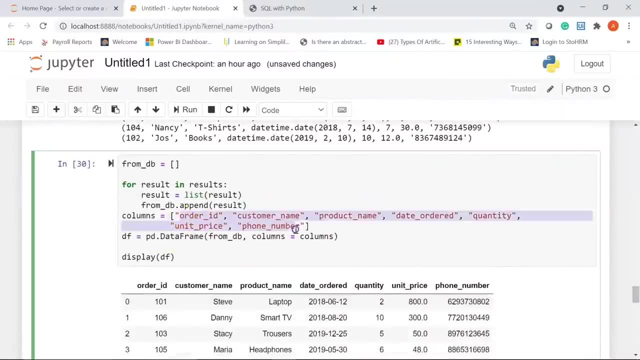 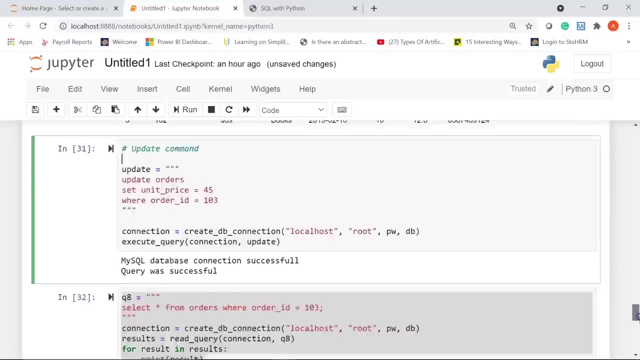 to filter our table based on specific conditions. we saw how to order your results based on a particular column. then we saw how you could convert the table into a data frame using pddataframe function. finally, we learned how to use the update command and the delete command. postgres sql is a very popular and widely used database in the industry. 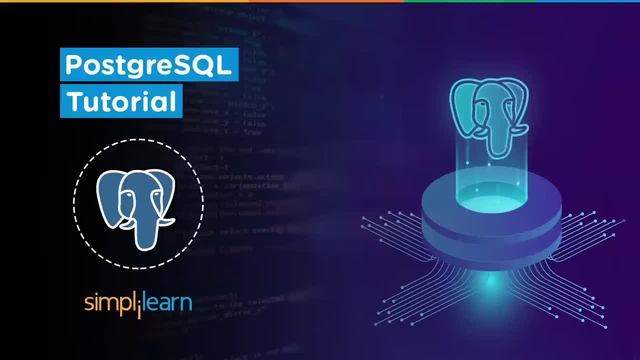 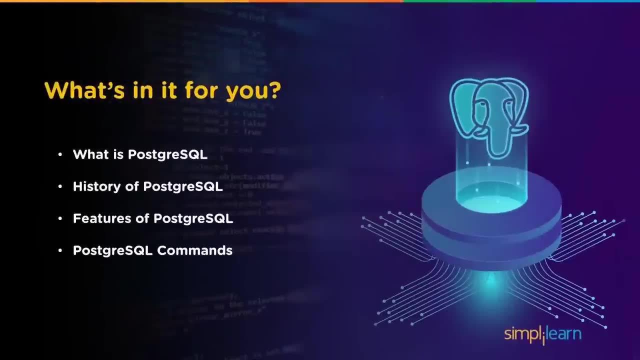 in this tutorial we will learn postgres sql or postgres sql, in detail with an extensive demo session. so in today's video we will learn what postgres sql is and look at the history of postgres sql. we will learn the features of postgres sql and jump into performing postgres sql commands. 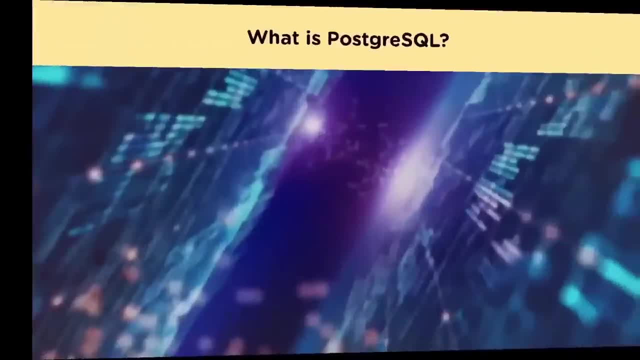 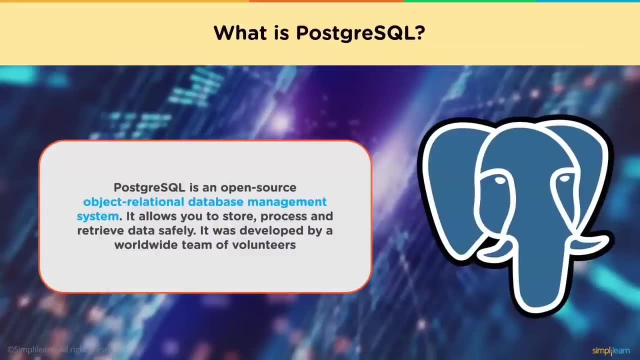 on the sql cell and pgadmin. so let's begin by understanding what is postgres sql. postgres sql is an open source object relational database management tool that uses postgres sql as its own management system. it stores data in rows with columns as different data attributes. according to the db engines ranking, postgres sql is currently ranked fourth in popularity. 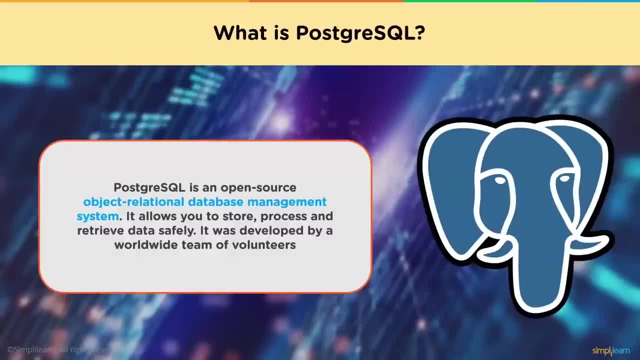 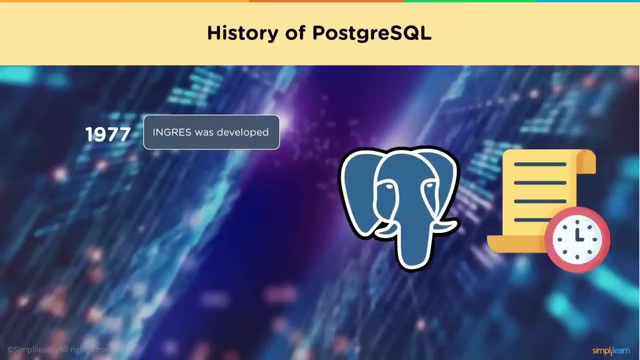 amongst hundreds of databases worldwide. it allows you to store, process and retrieve data safely. it was developed by a worldwide team of volunteers. now let's look at the history of postgres sql. so in 1977 onwards, the ingress project was developed at the university of california, berkeley. in 1986, the postgres project was led by professor michael. 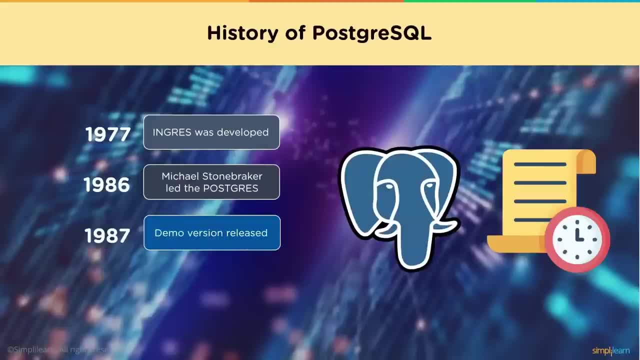 stonebreaker. in 1987 the first demo version was released and in 1994 a sql interpreter was added to postgres. the first postgres sql release was known as version 6.0 or 6.0, on january 29 1997, and since then postgres sql has continued to be developed by the postgres sql global development. 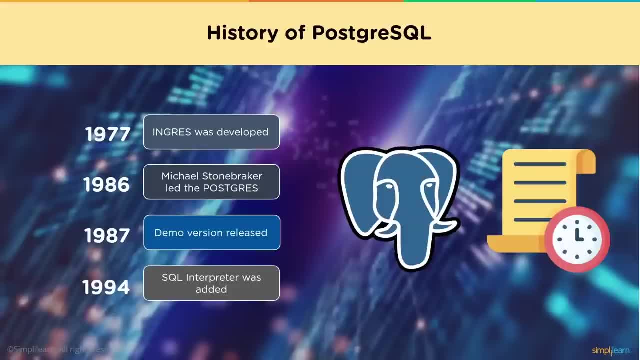 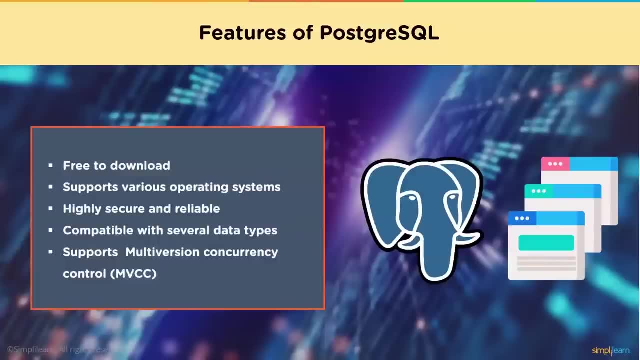 group, a diverse group of companies and many thousands of individual contributors. now let's look at some of the important features of postgres sql. so postgres sql is the world's most advanced open source database and is free to download. it is compatible, as it supports multiple operating systems, such as windows, linux and mac os. it is highly secure, robust and reliable. 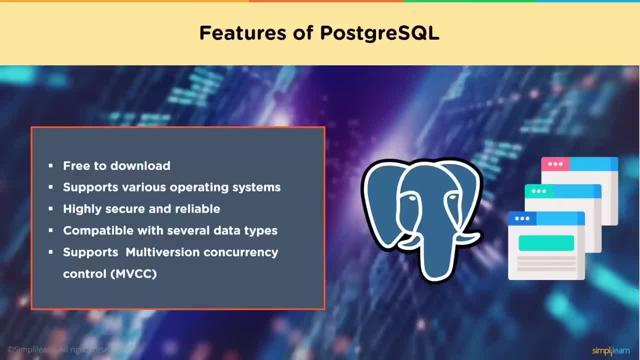 postgres sql supports multiple programming interfaces such as c, c plus plus, java and python. sql is compatible with various data types. it can work with primitives like integers, numeric string and boolean. it supports structured data types such as date and time, array and range. it can also work with documents such as json and xml. and finally, postgres sql supports multi-version. 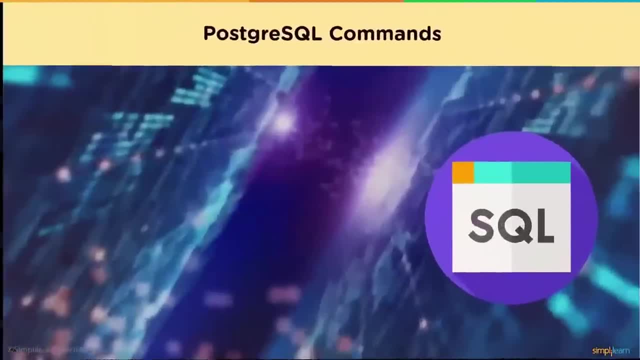 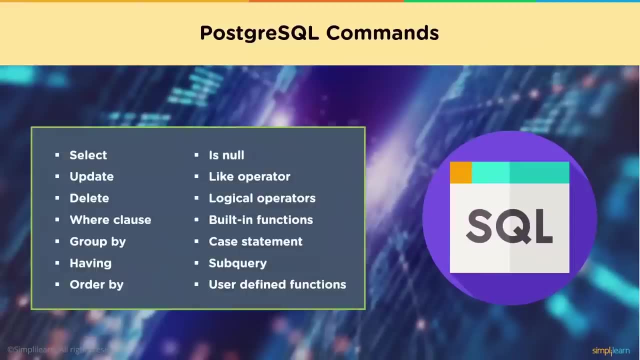 concurrency control, or mvcc. now, with this theory knowledge, let's look at the postgres sql commands that we will be covering in the demo. so we will start with the basic commands, such as select, update, delete. we will learn how to filter data using where clause and having clause in sql. 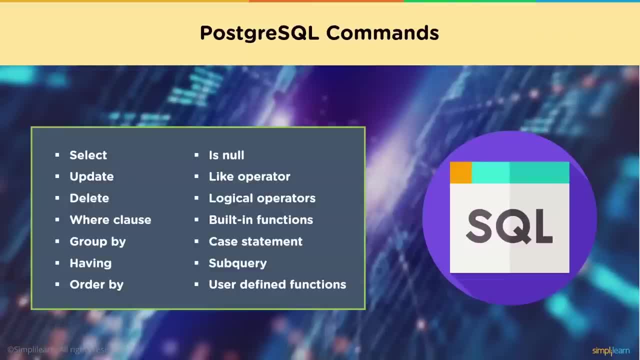 we will also look at how to group data using the group by clause and order the result using the order by clause. you will learn how to deal with null values, get an idea about the like operator, logical operators such as and, and or. we will also explore some of the popular inbuilt mathematical 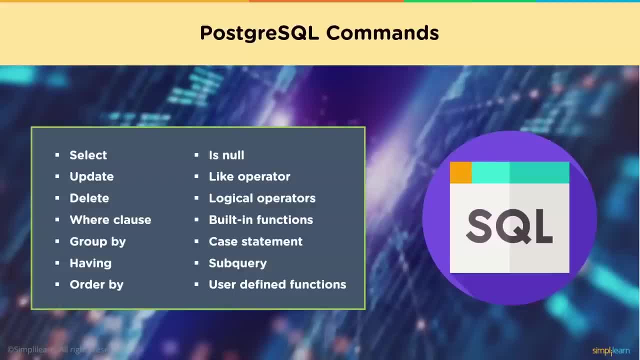 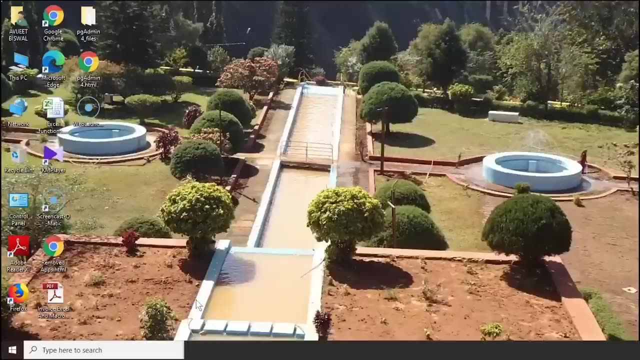 and string functions. finally, we'll see some of the advanced concepts in postgres sql. that is, to write key statements, sub queries and user defined functions. so let's head over to the demo now. okay, so let's now start with our demo. so first we'll connect to postgres sql using p sql cell. 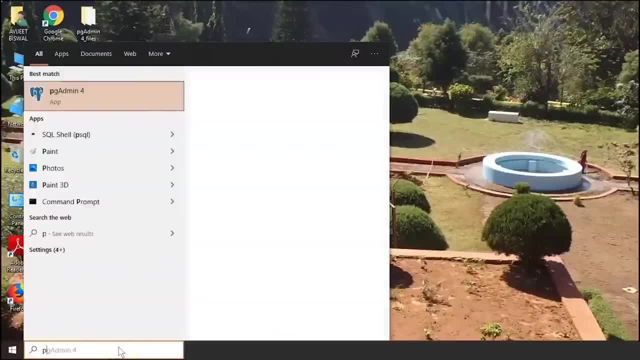 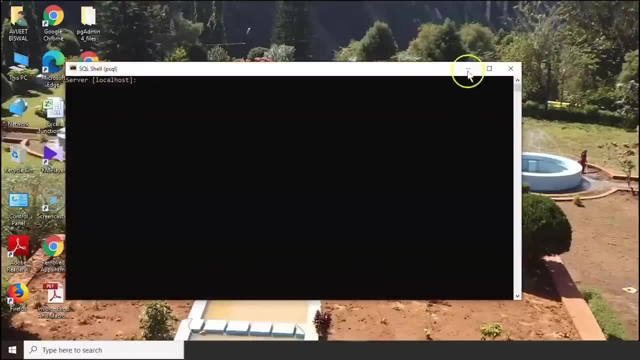 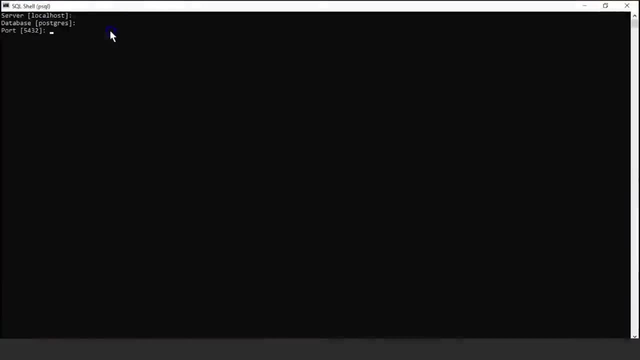 so here under type, here to search, i'll search for p sql. you can see this is the sql cell. i'll click on open. let me maximize this. okay, so for server i'll just click enter database. i'll just click enter. i'll click enter. port number is already taken, which is 5, 4, 3, 2. i'll hit enter. username is: 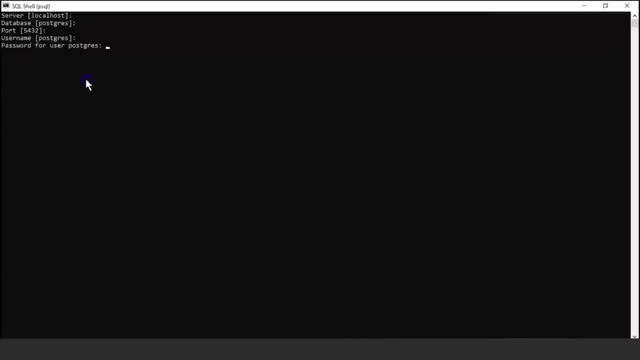 already given and now it is going to ask for password. so here i'll give my password so that i can connect to my postgres sql database. so it has given us a warning, but we have successfully connected to postgres sql. all right, so now to check if everything is fine. 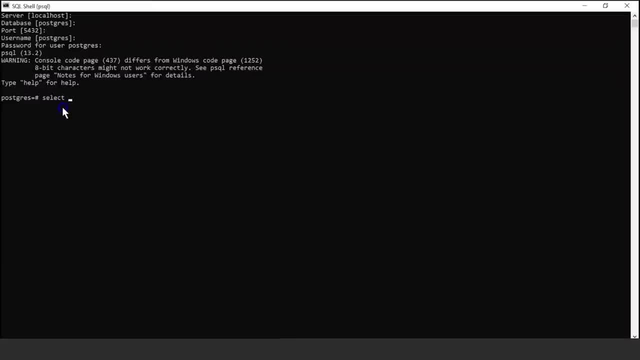 you can just run a simple command to check the version of postgres sql that we have loaded. so the command is select version, with two brackets and a semicolon. i'll hit enter. okay, you can see the version. postgres sql 13.2. okay, now let me show you the command. 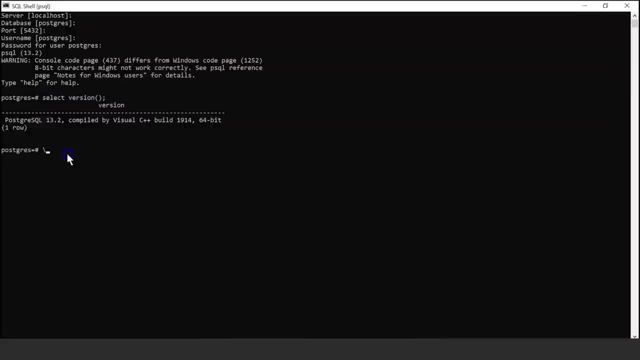 that will help you display all the databases that are already there. so if i hit slash l and hit enter, it will give me the list of databases that are there. so we have postgresql, there's something called template 0, template 1 and we have a test. 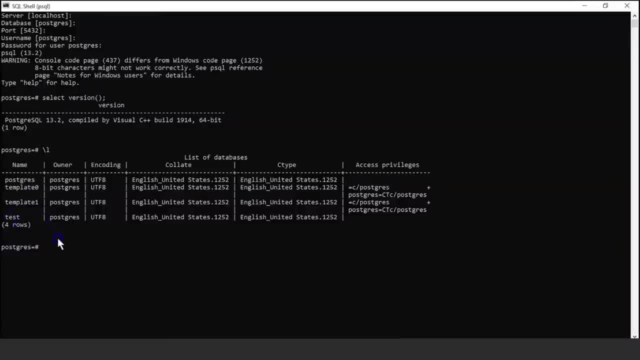 database as well. okay, now for our demo. i'll create a new database. so first i'll write create space database and i'll give my database name as sql underscore demo. i'll give a semicolon and hit enter. you see we have a message here that says create database. so we have successfully created. 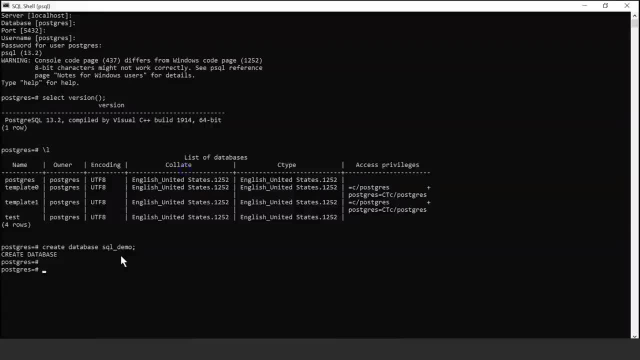 our sql demo database. now if you want to connect to that database you can use backslash c space sql underscore demo. there you go. it says you are now connected to database sql underscore demo. so here we can now create tables. we can perform insert operation, select operation. 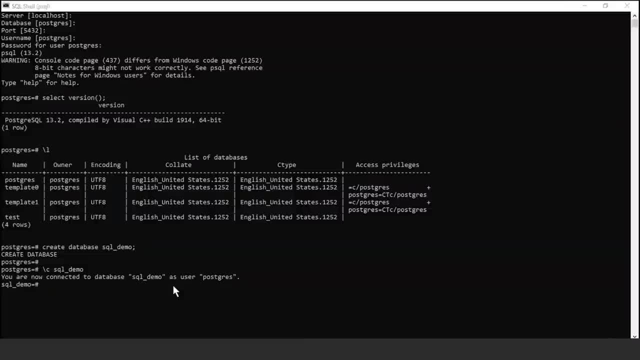 or bench你在 the database. we can now create tables. we can perform insert operation, select operation or benchFCM. do you know is it does it's not going to do or not? it's not going to do update, delete, alter and much more. now i'll show you how to connect to. 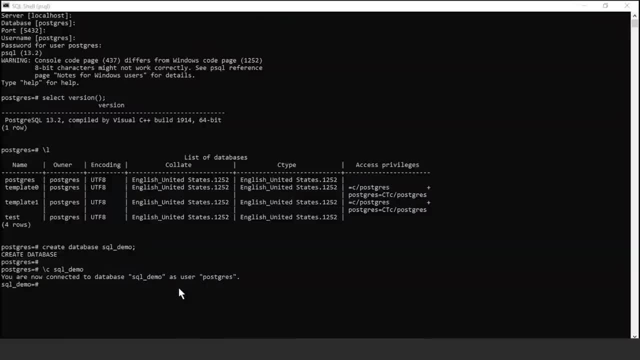 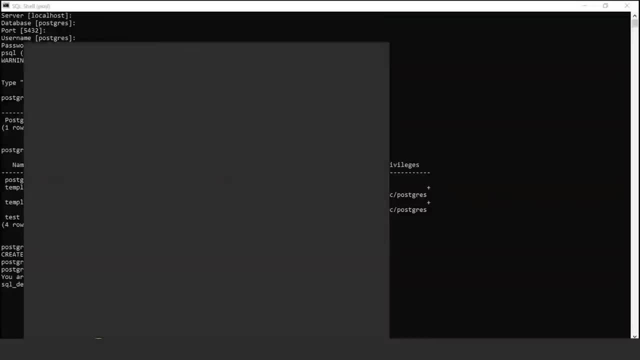 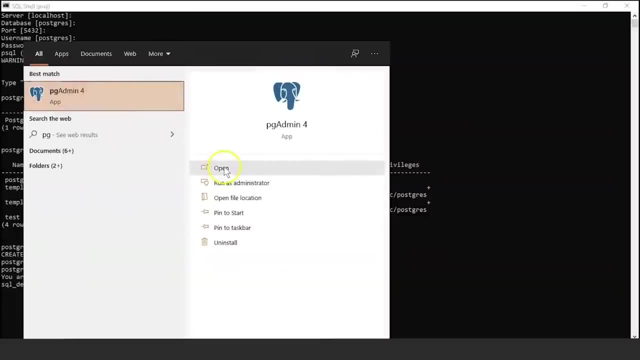 postgres sql using pg admin. so when you install the postgres sql database you will get the sql cell and along with that you also have the pg admin. so i'll just search for pg. you can see here it has prompted pg admin. i'll click on open. this will open on a web browser. 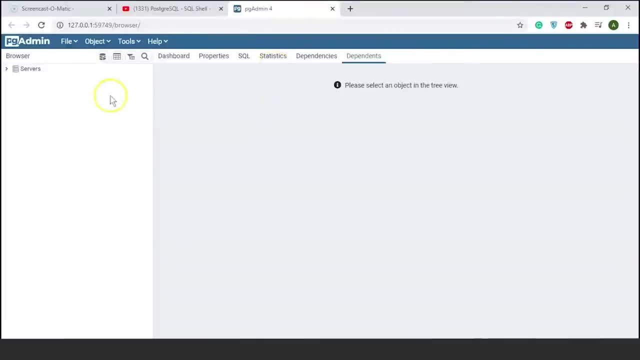 you can see it has opened on chrome and this is how the interface of pg admin looks like. it is a very basic interface. so on the top you can see the files. we have object, there's tools and we have the help section as well, and here you have dashboard properties. 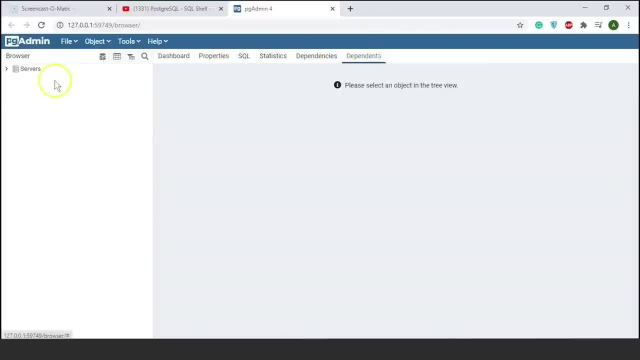 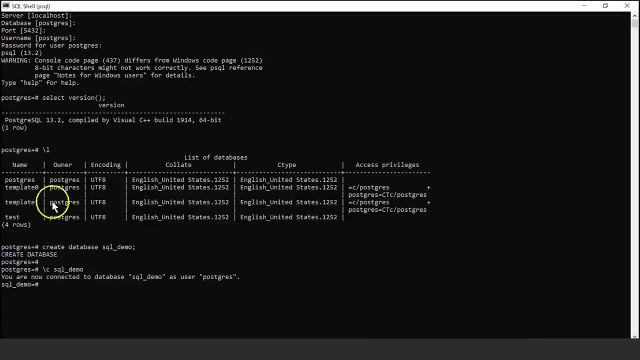 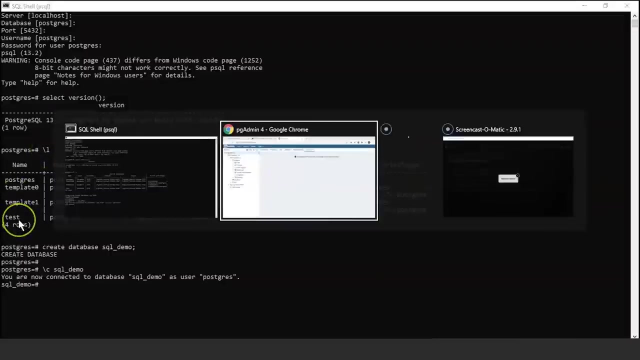 sql statistics, dependencies, dependence, and here on the left panel you have servers. let me just expand this so it will connect to one of the databases. all right, so if i go back, you see, when i had run backslash l to display the databases, it had shown me postgres sql and test. now you can see, here we have the postgres sql database and the. 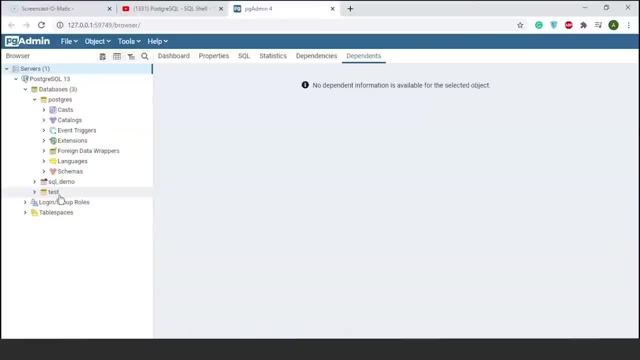 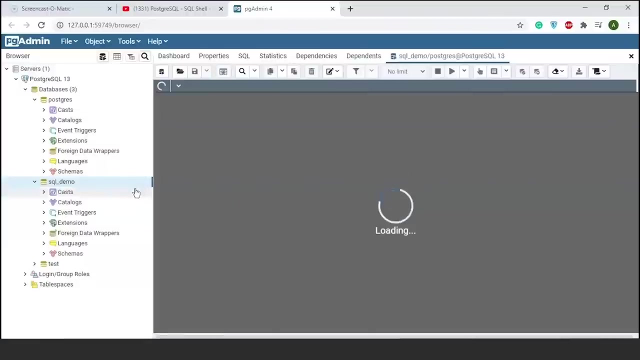 test database. all right. now we also created one more database, which was sql demo. so let me show you how to work on this: pg admin and the query tool. all right? so i'll right click on sql demo and i'll select query tool. i'll just show you how to run a few commands on the query tool. 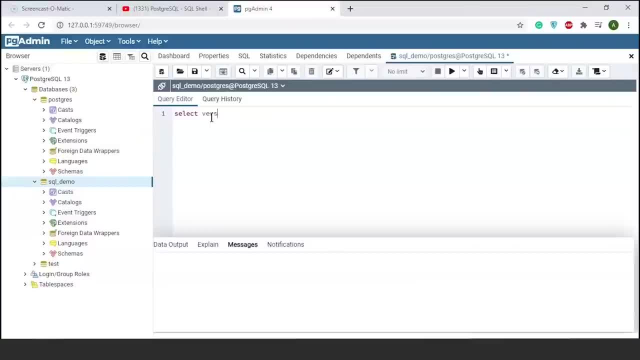 so let's say you want to see the version of postgres sql that you are using. so you can use the same command that we did on psql cell, which is select version, closed with brackets and a semicolon. i'll select this and here you can see we have the execute button. so if i 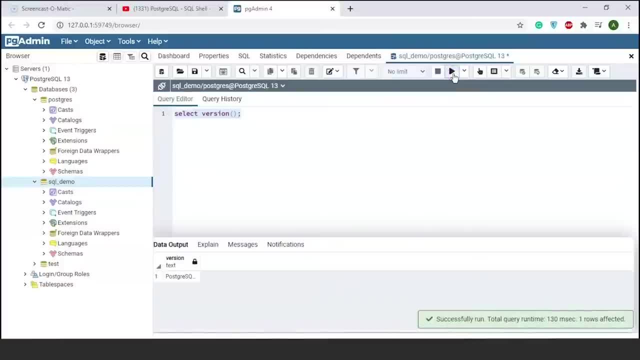 hit execute or press f5. it will run that query. you can see we have the output at the bottom and it says postgres sql 13.2, compiled by visual c plus. plus, it has a 64-bit system. okay, now let me tell you how to run postgres sql and test. now let me tell you how to run postgres sql and test. 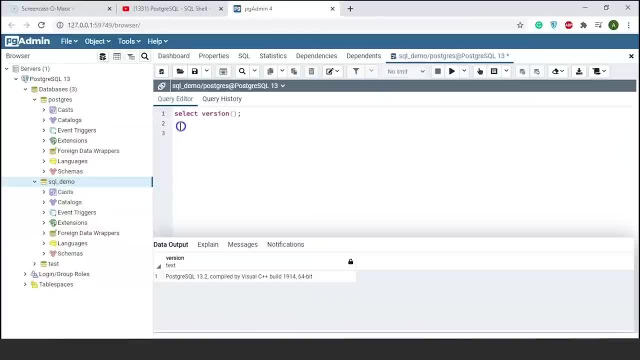 you how to perform a few basic operations using postgres sql commands. so here let's say i'll write: select five into three, i'll give a semicolon, select this and hit f5. so this will run the query and it returns me the result that is the product of 5 and 3, which is 15.. similarly, let's edit this: 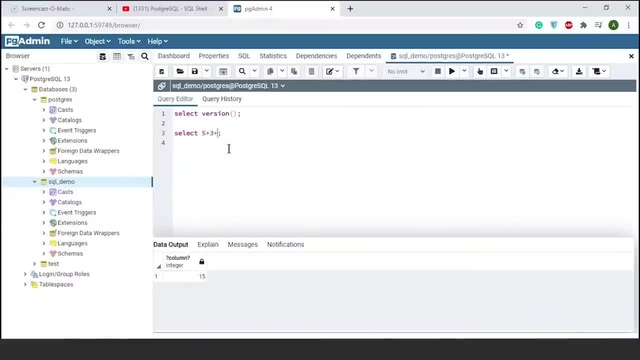 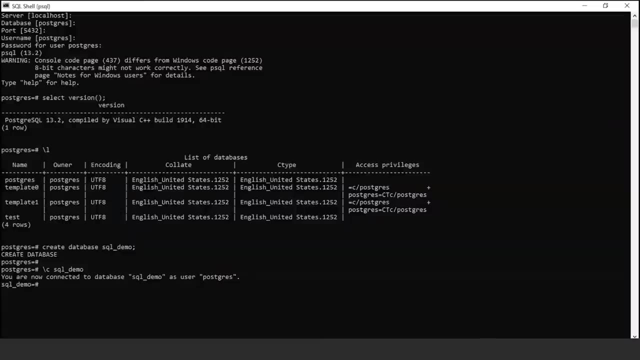 let's say i'll write 5 plus 3 plus, let's say, 6.. I'll select this and hit F5 to run it. It gives me the sum of 5 plus 3 plus 6, which is 14.. Now the same task. you can do it on this cell as well. Let me show you how to do it. 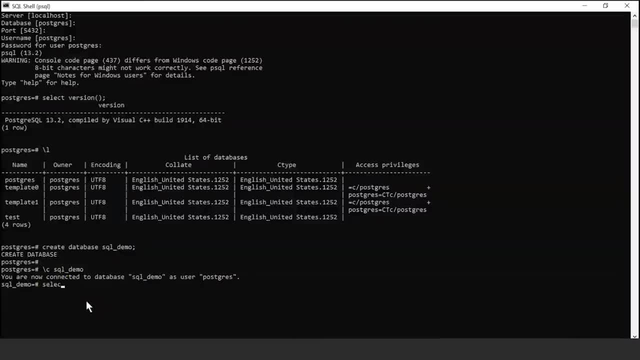 here. So let's say I'll write select. Let's say I want to multiply 7 into, let's say, 10.. You know the result: it should be 70.. If I hit enter, it gives me 70.. Now this question mark, column. 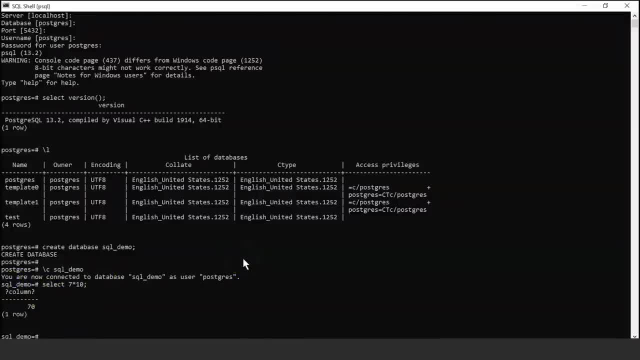 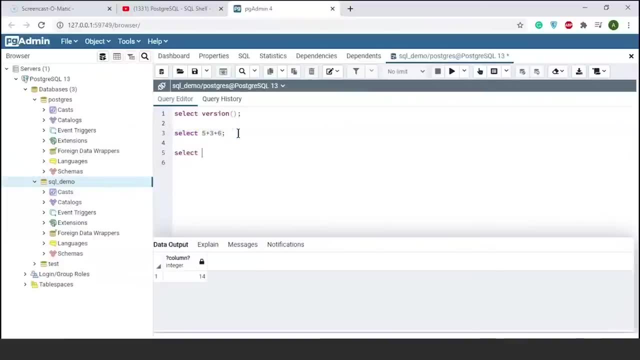 question wall will deal with this later. All right, let me go back to my pgadmin again. Let me do one more operation. Let's say, this time I'll write select 5 multiplied by, and within brackets I'll write 3 plus 4.. I'll give a semicolon. So what SQL will do is: first it will. 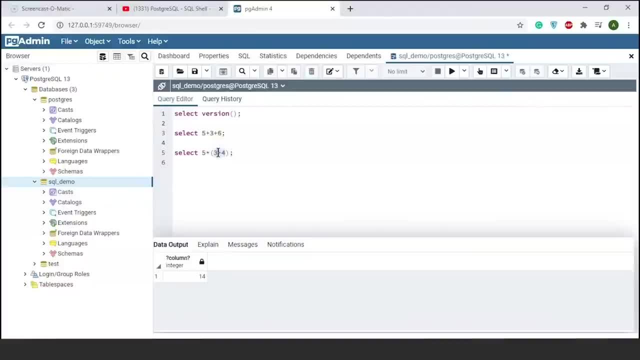 evaluate the expression that is there inside the bracket, that is 3 plus 4, which is 7, and then it will multiply 7 with 5.. Now let me select this and I'll hit execute So you can see: 7 multiplied by 5 is: 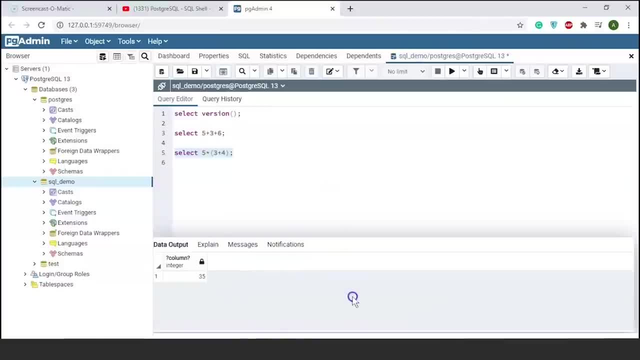 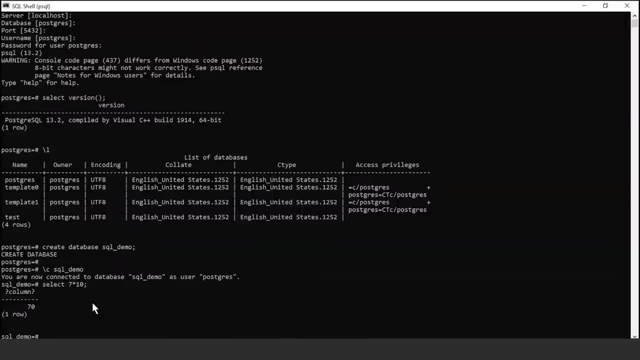 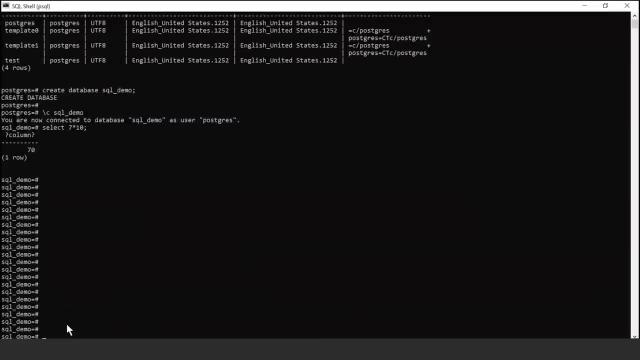 35.. All right, now we'll go back to our cell and here I'll show you how to create a table. So we are going to create a table called movies on the cell that is psql cell. So here we will learn how you can create a table and then you can enter a few data into. 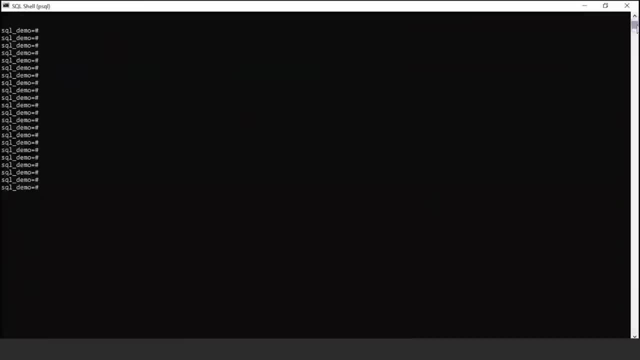 that table. All right, let me just scroll down a bit. Okay, so my create command goes something like this, So I'll write create table followed by the table name, that is, movies. Next, my movies table will have a few columns. Let's say: I want 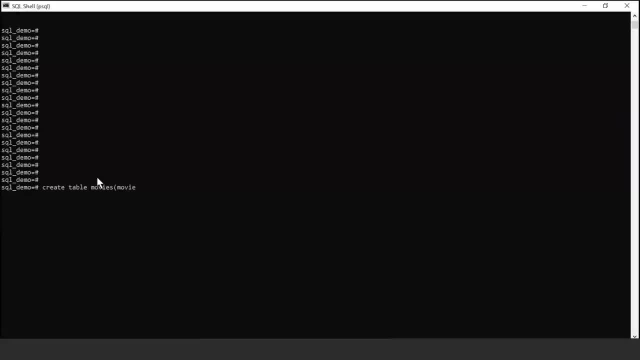 movie ID. after the column name we need to give the data type, so movie ID. I'll keep it as integer, so integer is one of the data types that is provided by postgres sequel. next my second column: the table would be the name of the movie, so I'll. 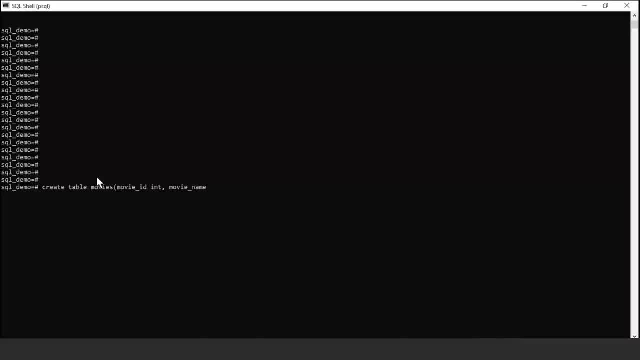 write movie underscore name. so all the variables of the column name should be as per SQL standards. so there shouldn't be any space between the column names. so I have used underscore to make it more readable. so my movie name will be of type: var, char or variable character or varying character, and I'll give the size. 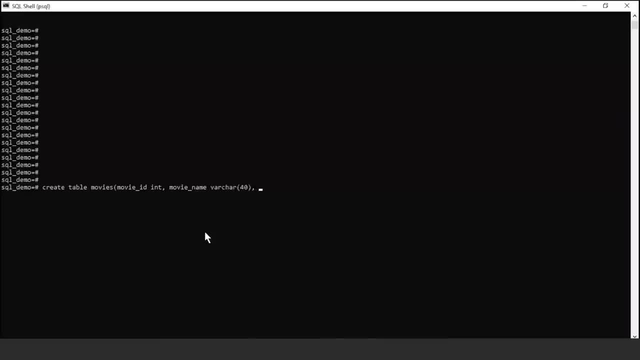 as 40, so that it can hold 40 characters maximum. next, my third column will have the genre of the movie, so I'll write movie underscore, genre. again, genre is of type var char. I'll give the size as, let's say, 30. and my final and the last column will have the IMDB rating, so I'll write IMDB. 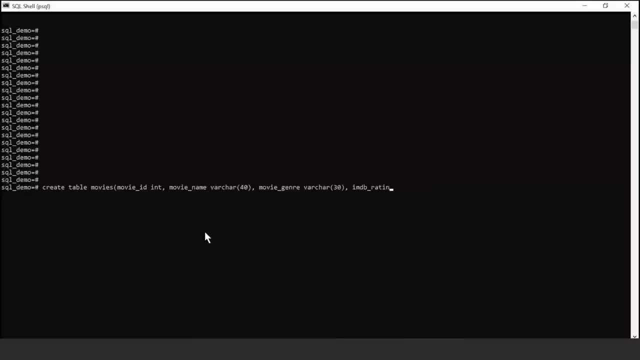 underscore ratings. now the ratings will be of type real, since it can have floating or decimal point values, and let me just forget about this table. so there will really be a table like that. contents here in the protocol description of the area. after closing the bracket, without skeptical and all, I'll hit enter. there you go. so we have successfully. 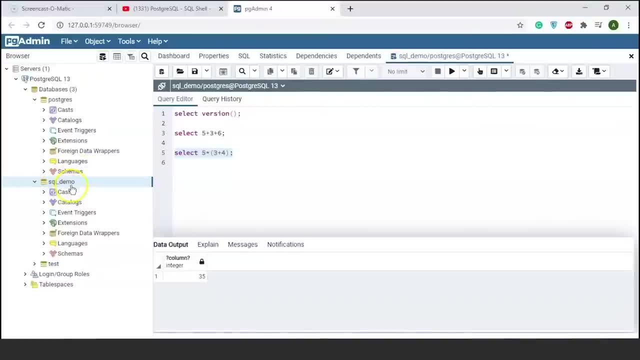 created a table called movies. now let me go back to my PG admin. all right, so here I have my database. that is a sql demo. I just right click on this and click on refresh. now let me go to ski Mars. I'll just roll down a bit here under skimmers. 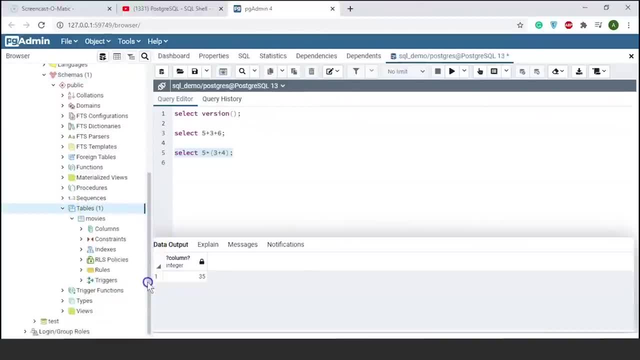 let me expand this. okay, so you can see, we have a table called movies in the SQL demo database now, and here you can check the columns that we have just added. so our movies table has movie ID, movie name, genre and ratings. all right, now there is another way to create a table. the previous time we created using the 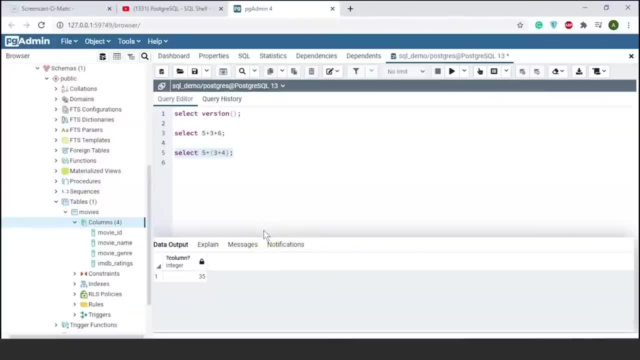 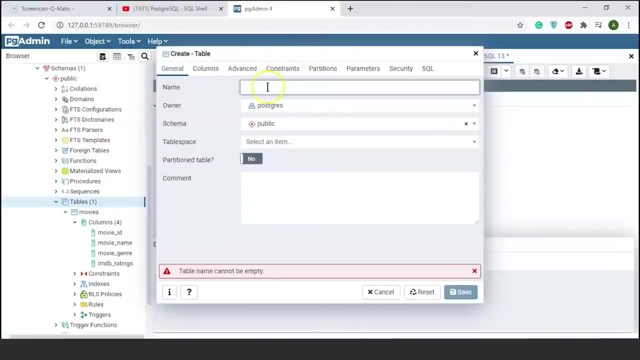 SQL cell. now I will tell you how to create a table using the PGA admin. so here under tables, I'll right click and I have the option to create a table. so I will select table. okay, so it's asking me to give the name of the table, so this: 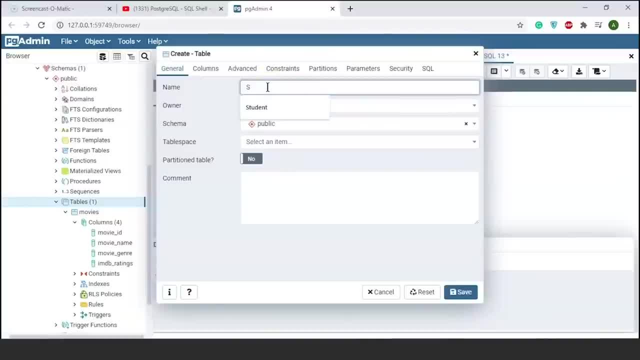 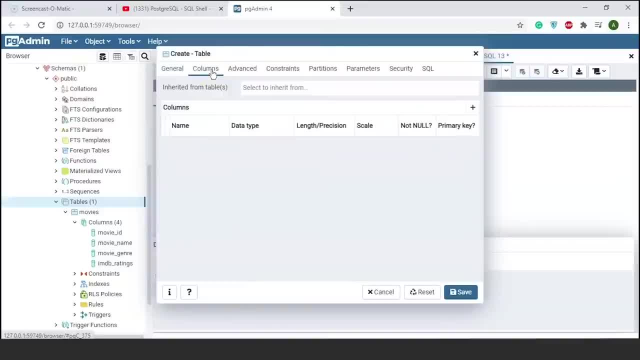 default as it is now. I'll go to the default as it is now. I'll go to the columns tab. so here you can create the columns tab. so here you can create the columns tab. so here you can create the number of columns that you want. so you. 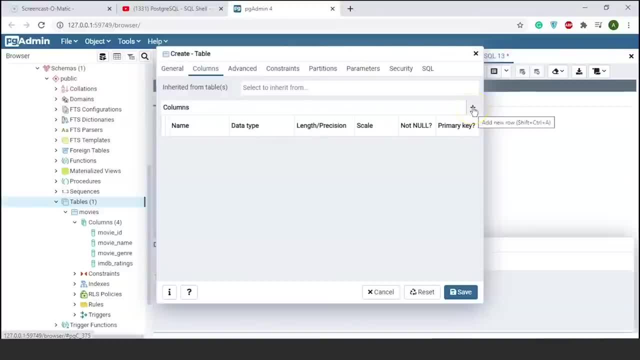 number of columns that you want. so you number of columns that you want. so you can see on the right: I have a plus sign. can see on the right. I have a plus sign. can see on the right. I have a plus sign. I'll just select this so that I can add. 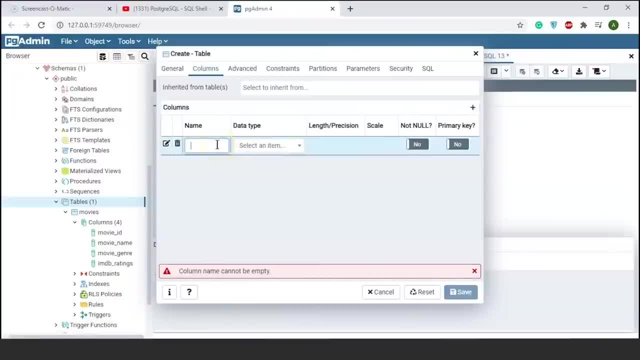 I'll just select this so that I can add. I'll just select this so that I can add a new row, so my first column would be a new row. so my first column would be a new row. so my first column would be, let's say, the student roll number. I'll. 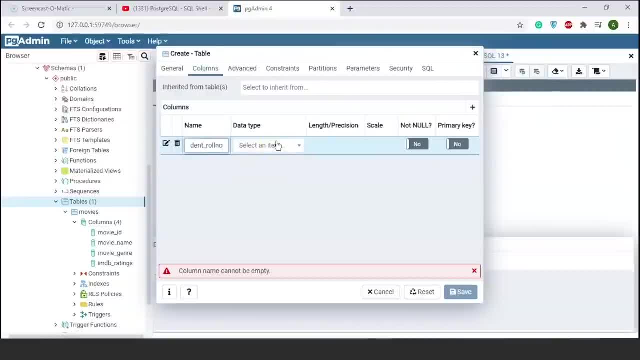 let's say the student roll number. I'll. let's say the student roll number. I'll write student underscore roll number. write student underscore roll number. write student underscore roll number. again. the column name should be as per. again. the column name should be as per. again. the column name should be as per SQL standards, the data type I am going. 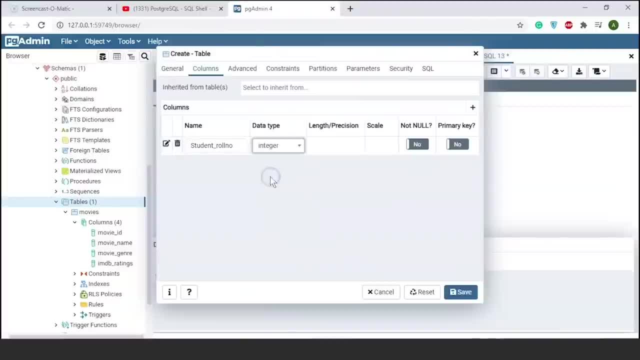 SQL standards. the data type I am going SQL standards. the data type I am going to select is integer- all right now. if to select is integer, all right now. if to select is integer, all right now. if you want, you can give these constraints. you want, you can give these constraints. 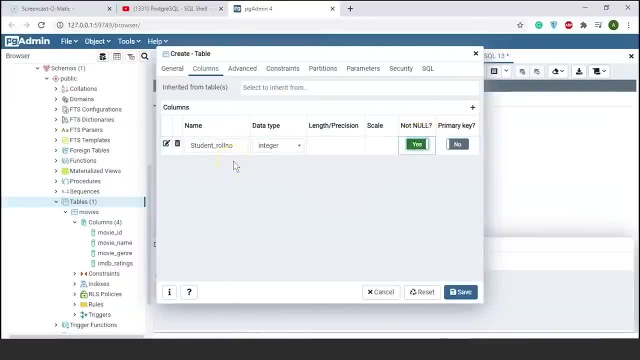 you want, you can give these constraints: such as not null, so that student roll such as not null, so that student roll such as not null, so that student roll number column will not have any null number column will not have any null number column will not have any null values. and I'll also check primary key. 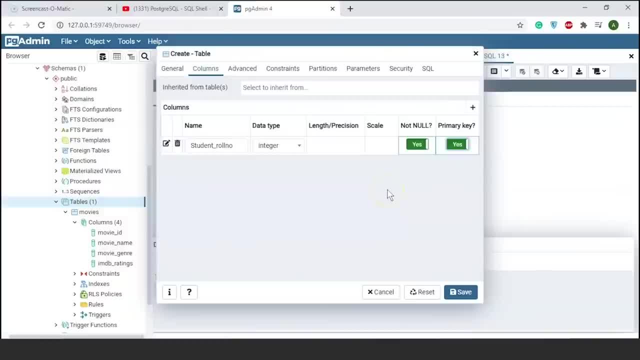 values and I'll also check primary key values and I'll also check primary key, which means all the values will be. which means all the values will be, which means all the values will be unique for roll numbers. all right if you. unique for roll numbers. all right if you. 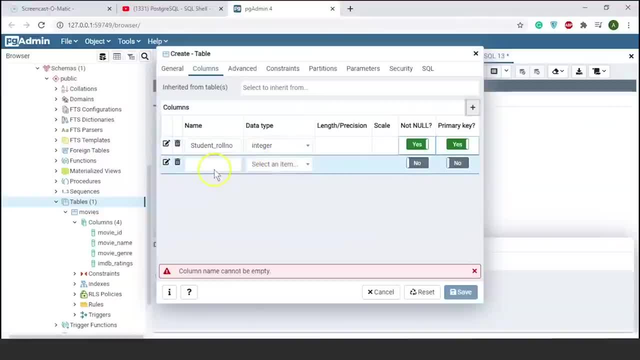 unique for roll numbers. all right, if you want to add another column, you can just want to add another column, you can just want to add another column. you can just click on that plus sign and let's say: click on that plus sign. and let's say, click on that plus sign and let's say: this time I want to give the student. 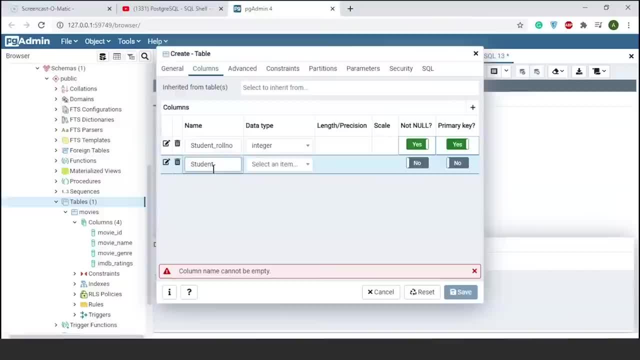 this time I want to give the student, this time I want to give the student name as my second column, so I'll write name as my second column. so I'll write name as my second column. so I'll write student underscore name- student name. student underscore name- student name. 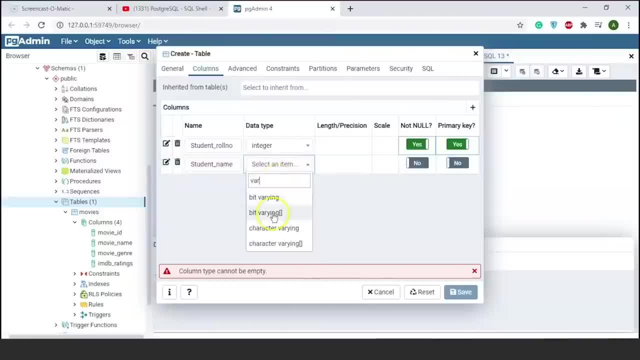 student underscore name: student name will be of type. let's say character will be of type. let's say character will be of type. let's say character varying if you want to give the length varying, if you want to give the length varying. if you want to give the length, you can specify the length as well. let's: 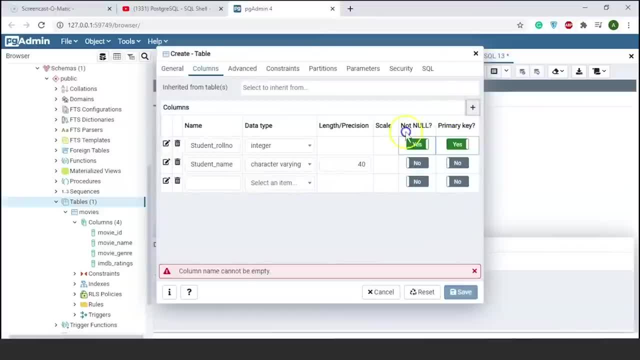 you can specify the length as well. let's: you can specify the length as well. let's say 40. I'll click on the plus sign. say 40. I'll click on the plus sign. say 40. I'll click on the plus sign again to add my final column, the final. 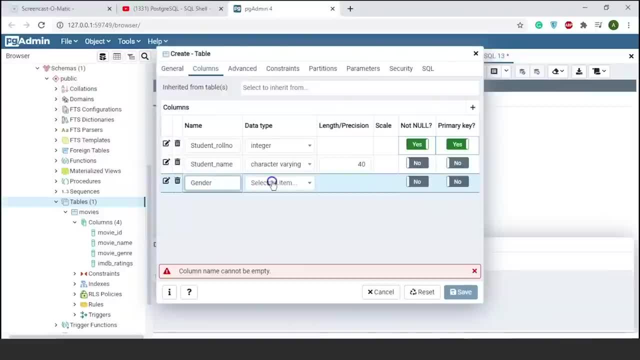 again to add my final column, the final. again to add my final column. the final column would be gender, so gender I'll column would be gender, so gender I'll column would be gender, so gender. I'll keep this time as type character. okay, keep this time as type character okay. 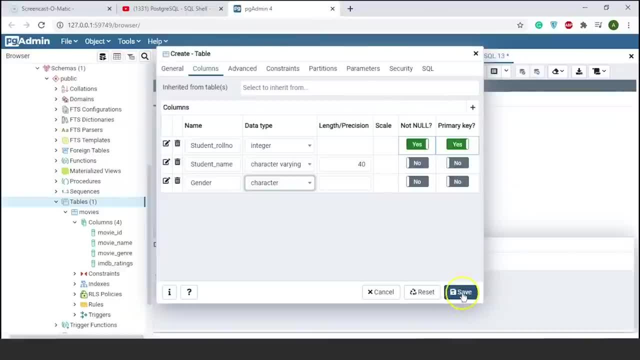 keep this time as type character. okay, now you can click on save, so that will. now you can click on save, so that will. now you can click on save, so that will successfully create your students table successfully create your students table. successfully create your students table. there you go. so here on the left panel. 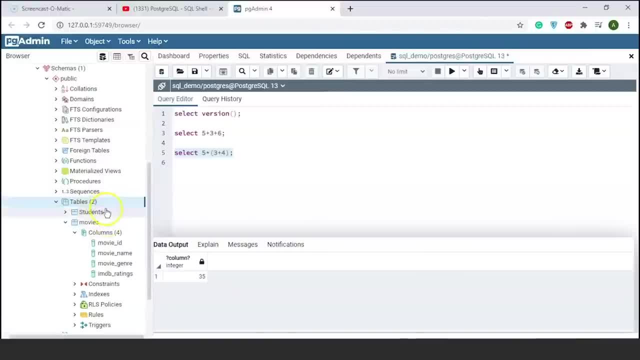 there you go. so here on the left panel. there you go. so here on the left panel, you can see. earlier we had only one, you can see. earlier, we had only one, you can see. earlier we had only one table, that was movies, and now we have two. 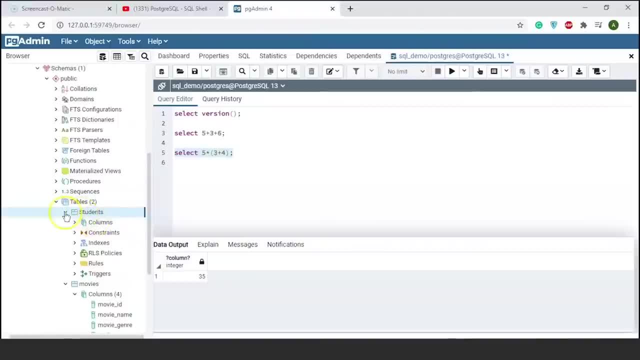 table that was movies, and now we have two table that was movies and now we have two tables. so one would be added that was tables. so one would be added that was tables. so one would be added that was students. if I expand this under columns: students. if I expand this under columns: 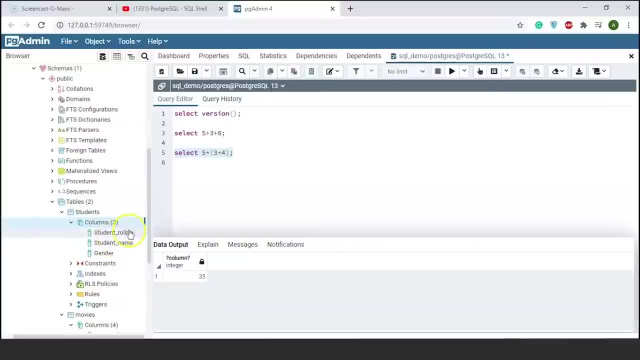 students. if I expand this under columns, you can see we have the three columns. you can see we have the three columns. you can see we have the three columns here. student rule number. student name here. student rule number. student name here. student rule number. student name and gender. you can also check the. 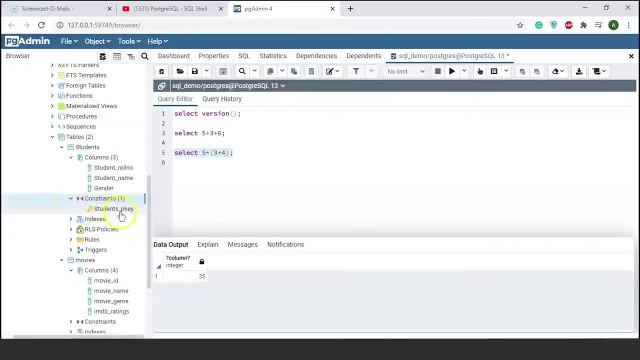 and gender. you can also check the and gender. you can also check the constraints. it will tell you if you have constraints. it will tell you if you have constraints. it will tell you if you have any constants. so you can see it says any constants. so you can see it says 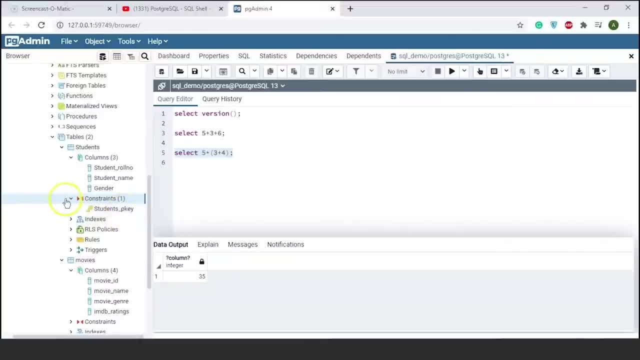 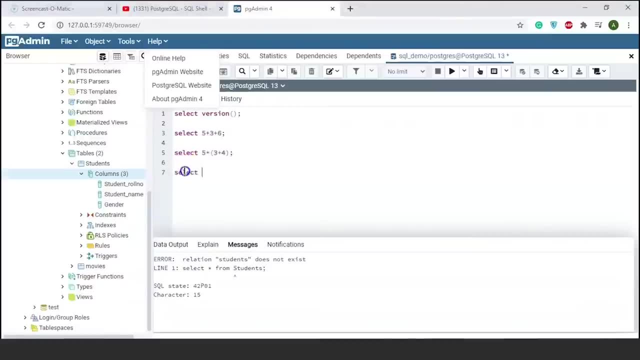 any constants so you can see. it says students rule number. there's one primary students rule number. there's one primary students rule number. there's one primary key. all right, all right now, let me run a key. all right, all right now, let me run a key. all right, all right now let me run a select statement to show the columns. 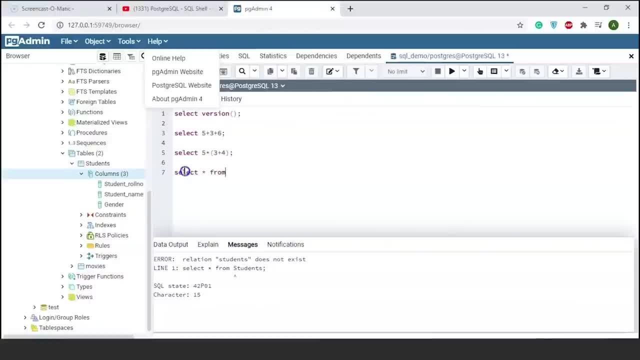 select statement to show the columns. select statement to show the columns that we have in the movies table. so I'll that we have in the movies table. so I'll that we have in the movies table. so I'll write: select star from movies- give a. write. select star from movies, give a. 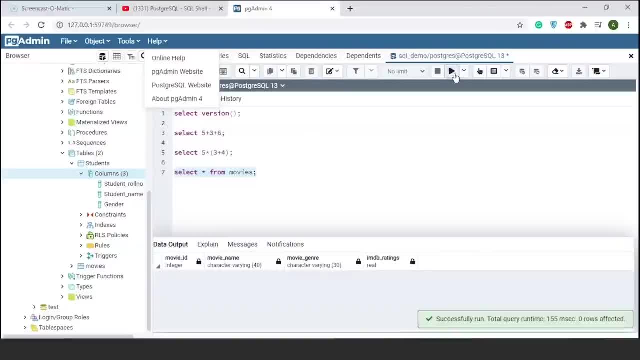 write: select star from movies. give a semicolon and let me execute this. okay, semicolon, and let me execute this. okay, semicolon, and let me execute this okay. name movie genre and IMDB ratings. now. name movie genre and IMDB ratings. now. name movie genre and IMDB ratings. now the next command we are going to learn. 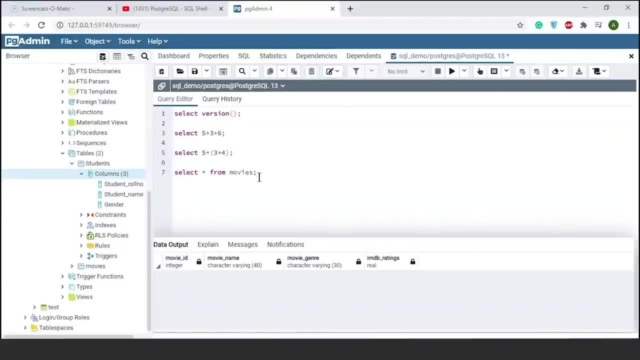 the next command we are going to learn. the next command we are going to learn is how to delete a table. so there is one is how to delete a table. so there is one is how to delete a table. so there is one way: by using the SQL command, that is: 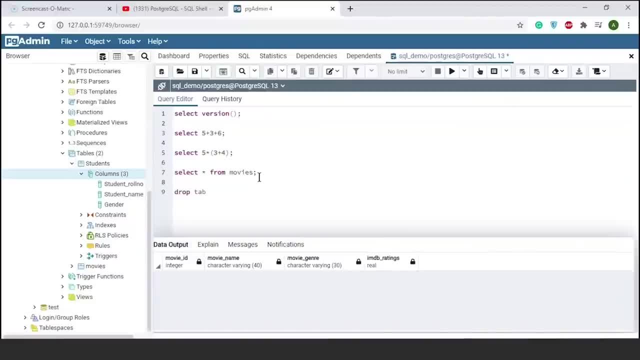 way by using the SQL command. that is way by using the SQL command. that is: drop table followed by the table name. drop table followed by the table name. drop table followed by the table name. let's say you want to delete students. let's say you want to delete students. 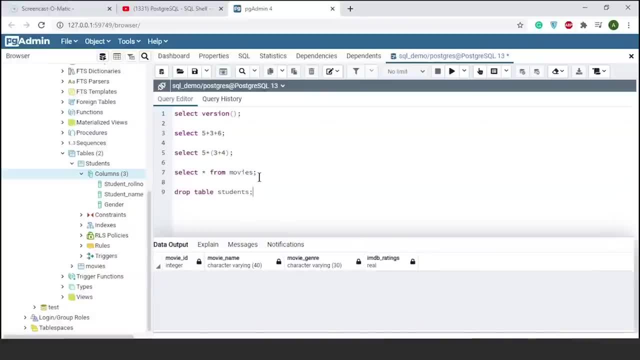 let's say you want to delete students, you can write drop table students and you can write drop table students and you can write drop table students and that will delete the table from the. that will delete the table from the. that will delete the table from the database. this is one of the methods. so 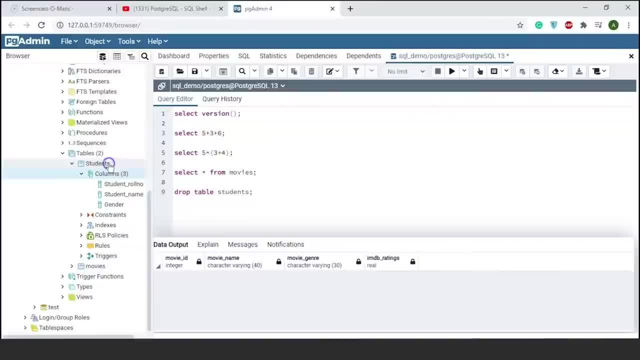 database: this is one of the methods. so database: this is one of the methods. so you just select and run it now. the other: you just select and run it now. the other: you just select and run it now. the other way is to you just right click on the. 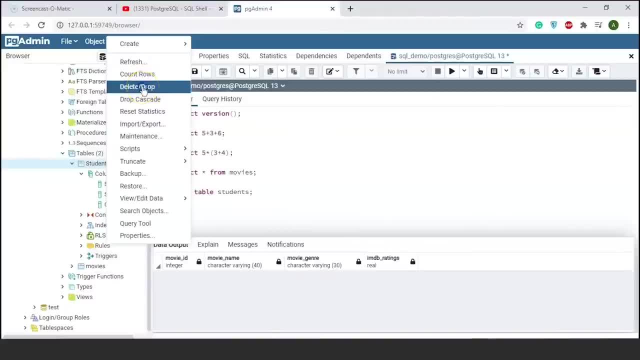 way is to you: just right click on. the way is to you: just right click on the table name, and here you have delete table name. and here you have delete table name. and here you have delete slash drop. if I select this, you get a slash drop. if I select this, you get a. 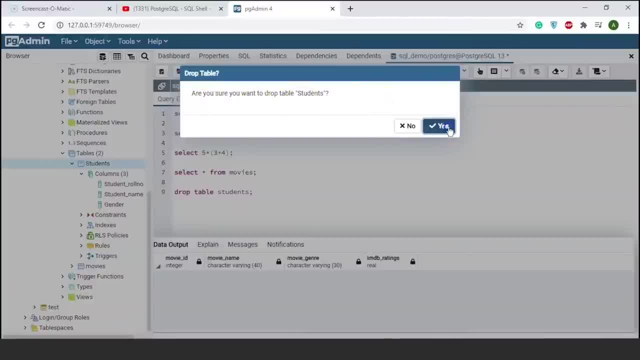 slash drop. if I select this, you get a prompt. are you sure you want to drop prompt? are you sure you want to drop prompt? are you sure you want to drop table students? I'll select yes, so you table students. I'll select yes, so you table students. I'll select yes, so you can see we have successfully deleted our. 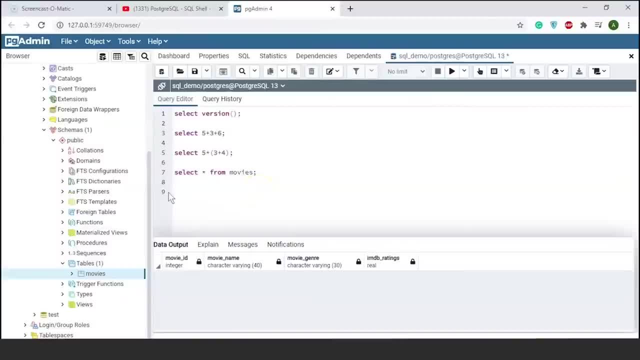 can see we have successfully deleted our. can see we have successfully deleted our. students table all right now. let's students table all right now. let's students table all right now. let's perform a few operations and learn a few. perform a few operations and learn a few. 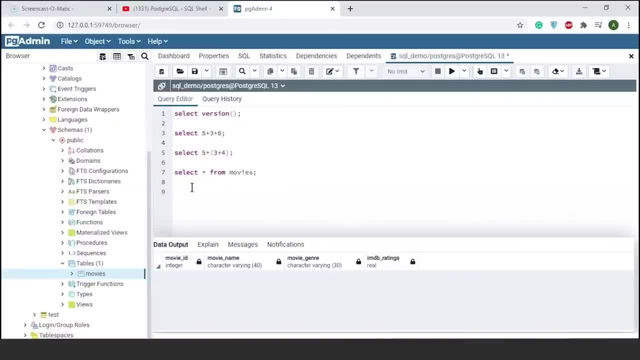 perform a few operations and learn a few more commands in PostgreSQL. so to do more commands in PostgreSQL, so to do more commands in PostgreSQL. so to do that, I am going to insert a few records, that I am going to insert a few records, that I am going to insert a few records to my movies table. so for that I'll use. 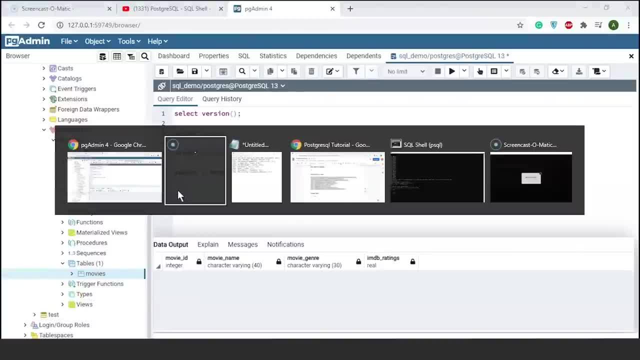 to my movies table. so for that I'll use to my movies table. so for that I'll use my insert command. so I have my insert, my insert command. so I have my insert, my insert command. so I have my insert query written on a notepad. I'll just. 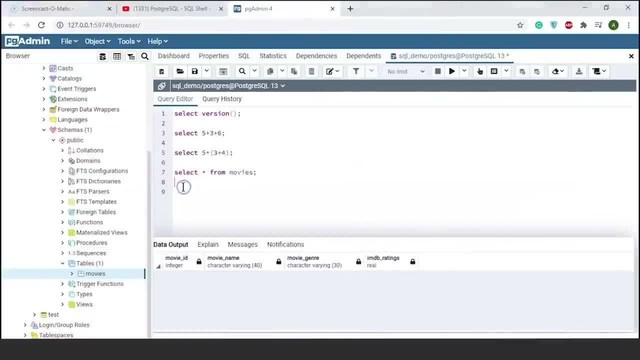 query written on a notepad. I'll just query written on a notepad. I'll just copy this and I'll paste it on my query. copy this and I'll paste it on my query. copy this and I'll paste it on my query. editor. okay, so let me just scroll down. 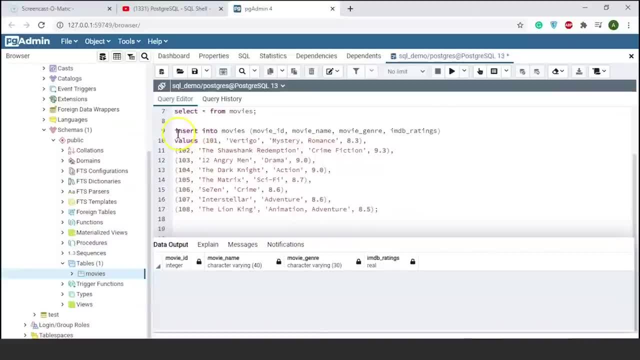 editor. okay, so let me just scroll down editor. okay, so let me just scroll down. alright. so here you can see I have used alright. so here you can see I have used alright. so here you can see I have used my insert command. so I have written my insert command. so I have written. 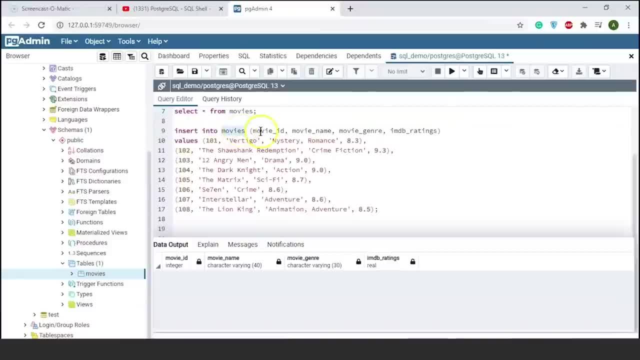 my insert command. so I have written: insert into the name of the table. that. insert into the name of the table. that. insert into the name of the table. that is movies and we have the movie ID: the is movies and we have the movie ID: the is movies and we have the movie ID, the movie name, movie genre and IMDB ratings. 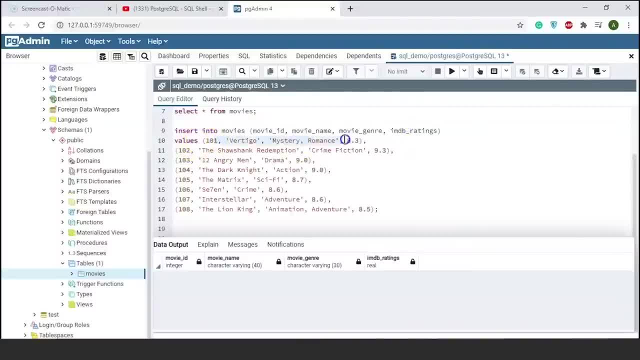 movie name, movie genre and IMDB ratings: movie name, movie genre and IMDB ratings. and these are the records or the rows. so, and these are the records or the rows. so, and these are the records or the rows. so we have the first record as movie ID 101. 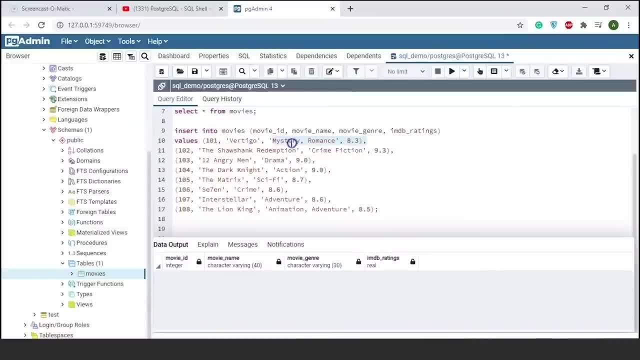 we have the first record as movie ID 101. we have the first record as movie ID 101. the name of the movie is a very popular. the name of the movie is a very popular. the name of the movie is a very popular movie, which is vertigo. then we have the. 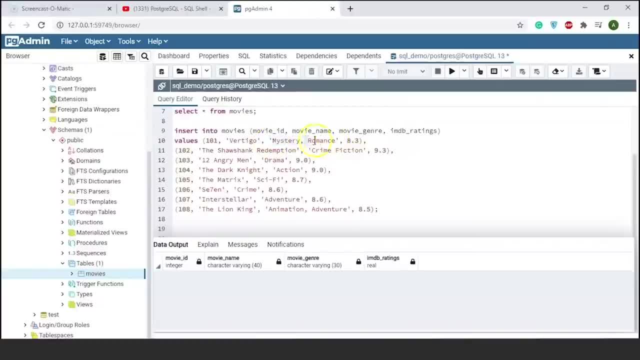 movie which is vertigo. then we have the movie which is vertigo, then we have the movie genre that is mystery. it is also a movie genre that is mystery. it is also a movie genre that is mystery. it is also a romance movie. and then we have the IMDB. 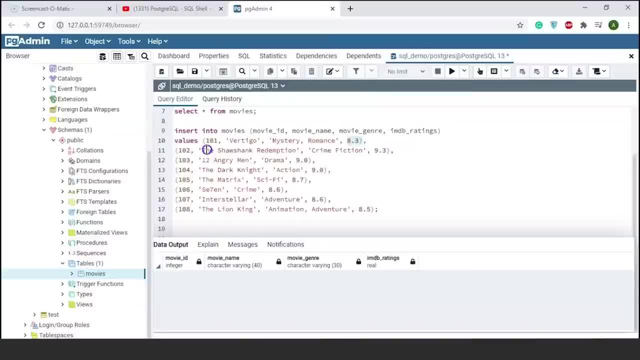 romance movie, and then we have the IMDB romance movie and then we have the IMDB ratings. the current IMDB reading: that is ratings. the current IMDB reading: that is ratings. the current IMDB reading: that is 8.3. similarly, we have saw shank. 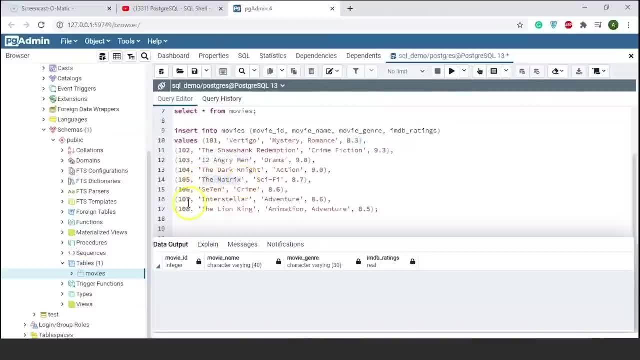 8.3. similarly, we have saw shank 8.3. similarly, we have saw shank Redemption. we have 12 angry men there's Redemption. we have 12 angry men there's Redemption. we have 12 angry men. there's the matrix 7 interstellar and the Lion. 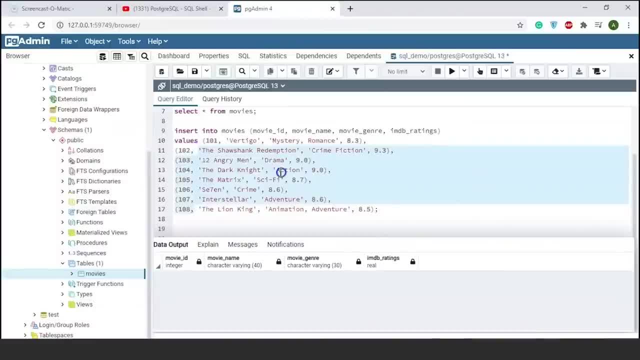 the matrix 7 interstellar and the Lion, the matrix 7 interstellar and the Lion King. so there are total 8 records that King. so there are total 8 records that King. so there are total 8 records that we are going to insert into our movies. 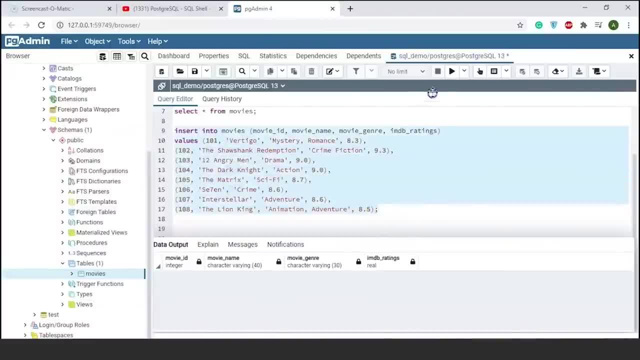 we are going to insert into our movies. we are going to insert into our movies table. so let me just select this and hit table. so let me just select this and hit table. so let me just select this and hit execute- okay, you can see it has. execute- okay, you can see it has. 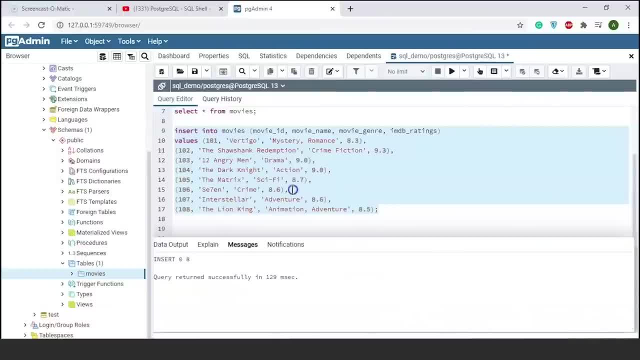 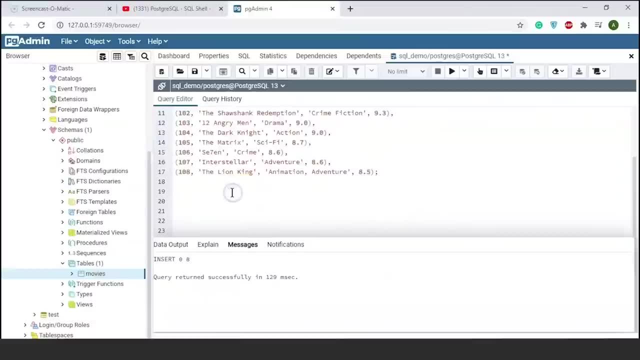 execute. okay, you can see it has returned successfully. eight records now returned successfully. eight records now returned successfully. eight records now. if I run select star from movies, you can. if I run select star from movies, you can. if I run select star from movies, you can see the records that are present in the 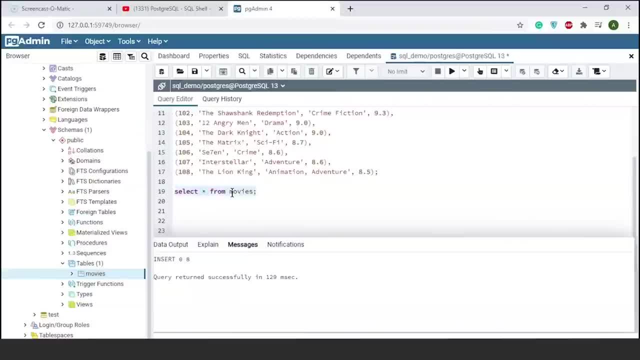 see the records that are present in the see the records that are present in the table. so I'll write select star from table. so I'll write select star from table. so I'll write select star from movies and select this and I'll execute movies and select this and I'll execute. 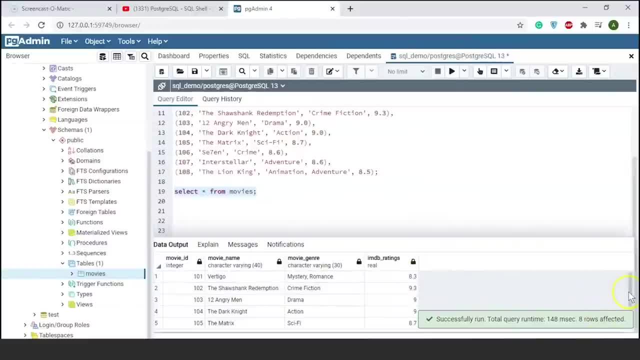 movies and select this and I'll execute it there you go at the bottom. you can it there. you go at the bottom, you can it there. you go at the bottom. you can see eight rows affected if I scroll this. see eight rows affected if I scroll this. 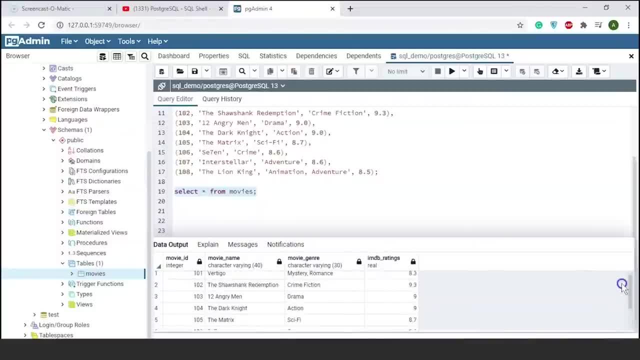 see eight rows affected if I scroll this down. you have the eight records of down. you have the eight records of down. you have the eight records of information in the movies table- alright. information in the movies table: alright. information in the movies table: alright. now if you want to describe the table, 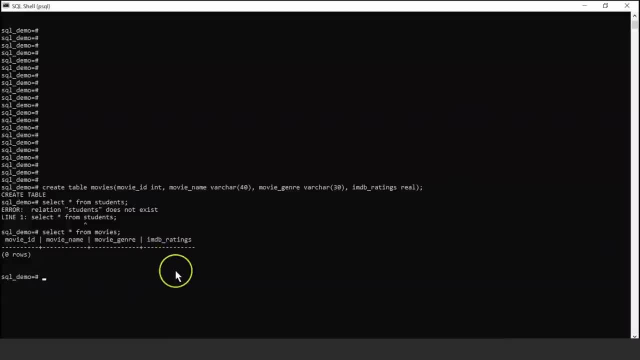 now if you want to describe the table. now, if you want to describe the table, you can go to the SQL cell. and here, if you can go to the SQL cell, and here, if you can go to the SQL cell, and here, if you write backslash D and the name of 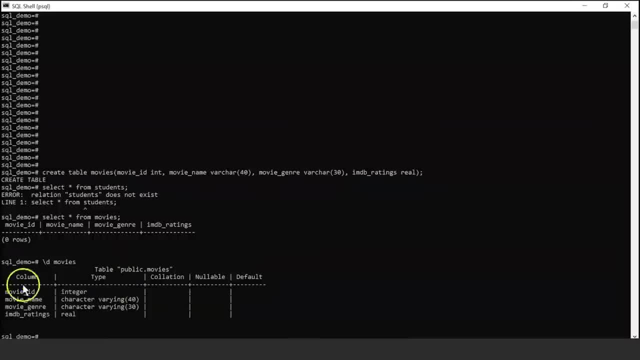 you write backslash D and the name of. you write backslash D and the name of the table that is movies. this will the table that is movies. this will the table that is movies. this will describe the table. so here you have the. describe the table. so here you have the. 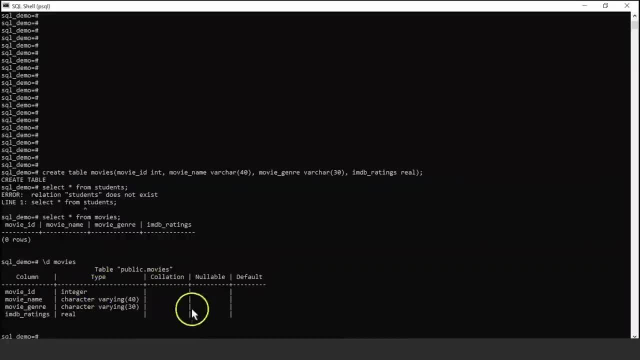 describe the table. so here you have the column names. this has the data type and column names. this has the data type and column names. this has the data type and here you can specify if there are any. here you can specify if there are any. here you can specify if there are any null values or any constraints, like 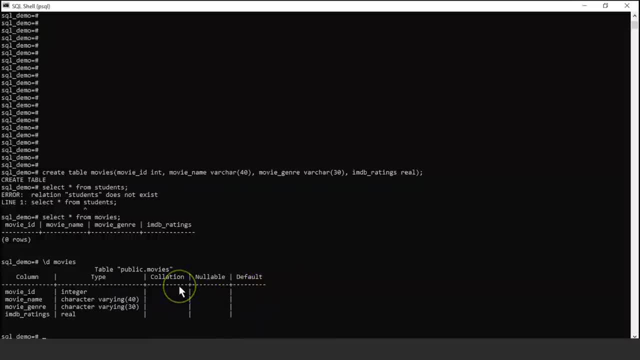 null values or any constraints like null values or any constraints like default constraint or primary key or default constraint or primary key or default constraint or primary key or foreign key and others. let me go back to foreign key and others. let me go back to foreign key and others. let me go back to my PG admin. okay, now, first and foremost, 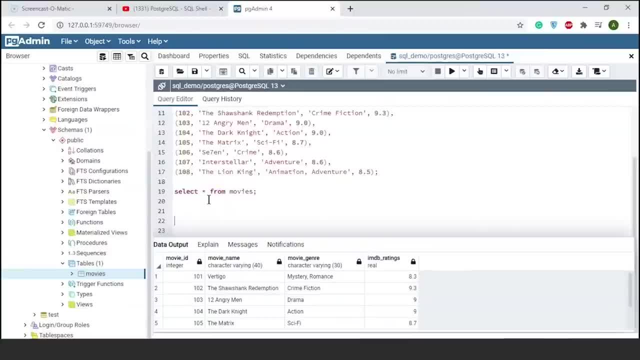 my PG admin. okay, now, first and foremost, my PG admin. okay, now, first and foremost, let me tell you how to update records in. let me tell you how to update records in. let me tell you how to update records in a table, so suppose you have an existing. 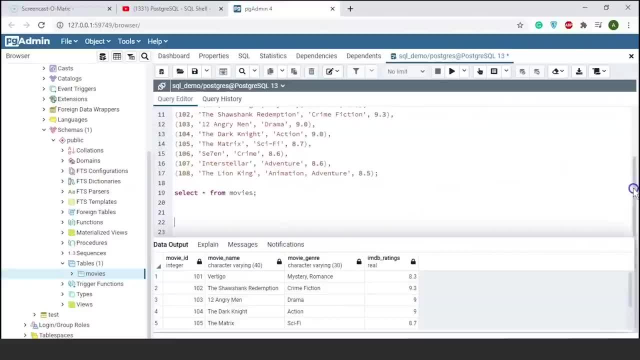 a table. so suppose you have an existing a table. so suppose you have an existing table and by mistake you have entered table and by mistake you have entered table and by mistake you have entered some wrong values and you want to update some wrong values and you want to update. 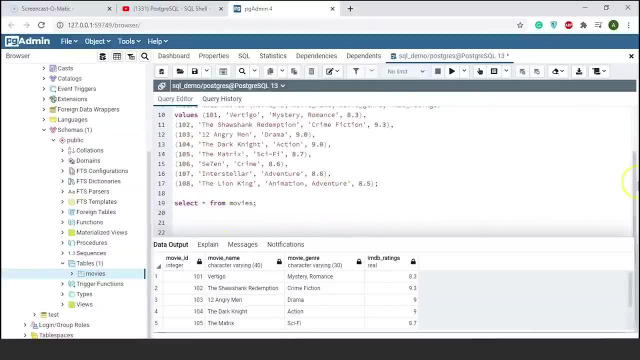 some wrong values and you want to update those records later. you can use the those records later. you can use the those records later. you can use the update query for that. so I am going to update query for that. so I am going to update query for that. so I am going to update my movies table and I'll set the. 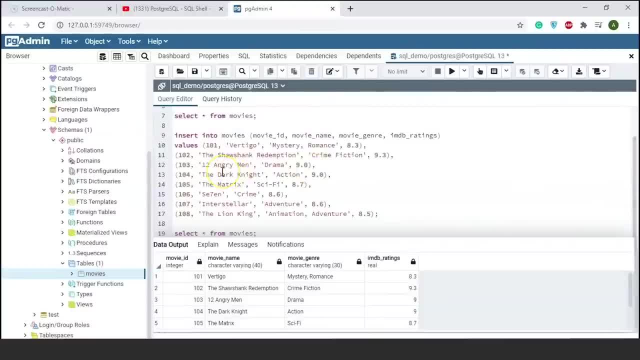 update my movies table and I'll set the update my movies table and I'll set the genre of movie: ID 1 0 3, which is 12, genre of movie. ID 1 0 3, which is 12 genre of movie. ID 1 0 3, which is 12: angry men from drama to drama and crime. 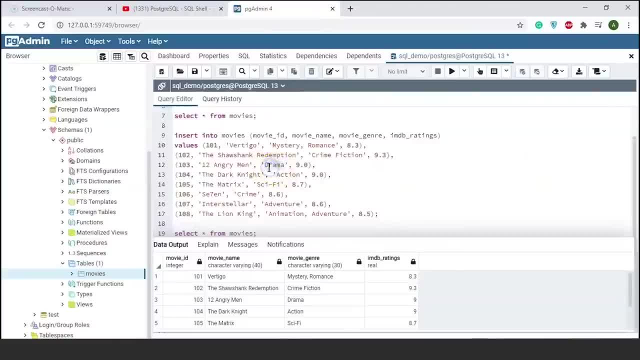 angry men from drama to drama and crime. angry men from drama to drama and crime. so in our current table we only have so. in our current table we only have so. in our current table we only have genre as drama for 12 angry men. I am. genre as drama for 12 angry men. I am. 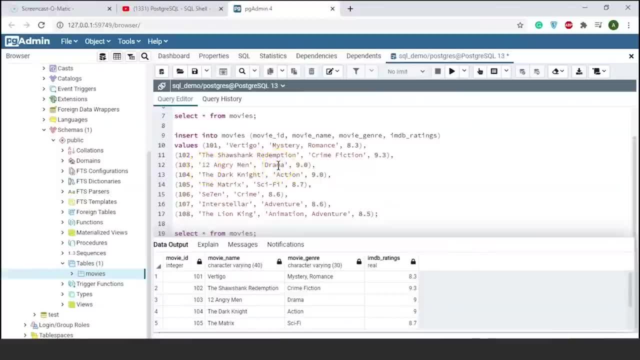 genre as drama for 12 angry men. I am going to update this column, which is the going to update this column, which is the going to update this column, which is the movie genre to drama and crime. okay, so, movie genre to drama and crime. okay, so, movie genre to drama and crime. okay, so let me show you how to do it. I'll write. 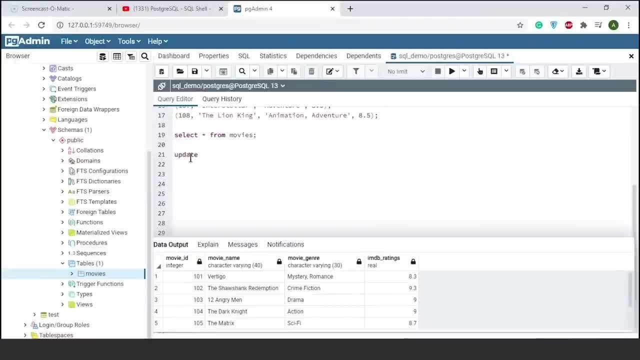 let me show you how to do it. I'll write. let me show you how to do it. I'll write: update, followed by the name of the table. update, followed by the name of the table. update, followed by the name of the table, that is, movies. go to the next line. I'll. 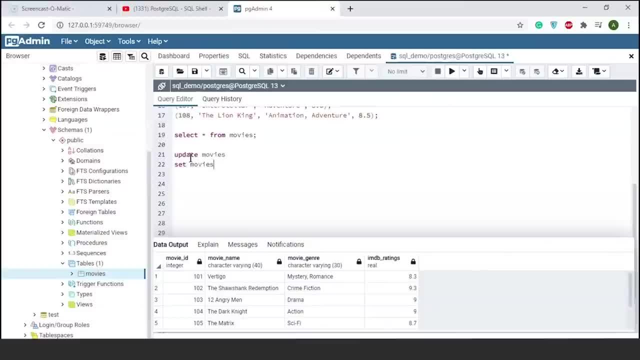 that is movies go to the next line. I'll. that is movies go to the next line. I'll write set. then I'll give the column name write set. then I'll give the column name write set. then I'll give the column name, which is movie underscore genre equal to. 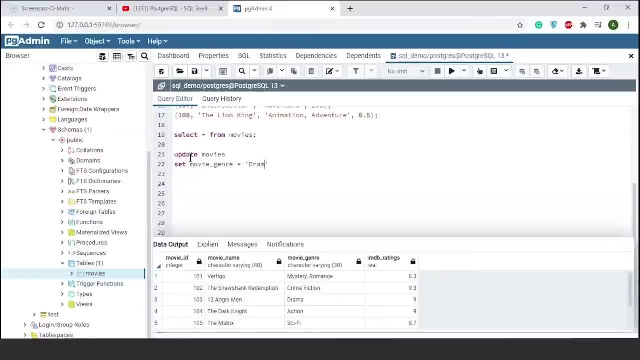 which is movie underscore genre equal to. which is movie underscore genre equal to. I'm going to set it as drama comma. I'm going to set it as drama comma. I'm going to set it as drama comma. crime: earlier, it was only drama and I'll. crime. earlier, it was only drama and I'll. 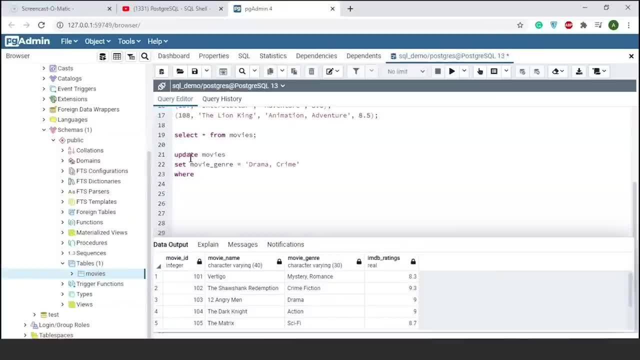 crime earlier it was only drama and I'll give my condition using the where. give my condition using the where. give my condition using the where clause. we'll learn where clause in a bit clause. we'll learn where clause in a bit clause. we'll learn where clause in a bit. so I'll write where: movie underscore ID. 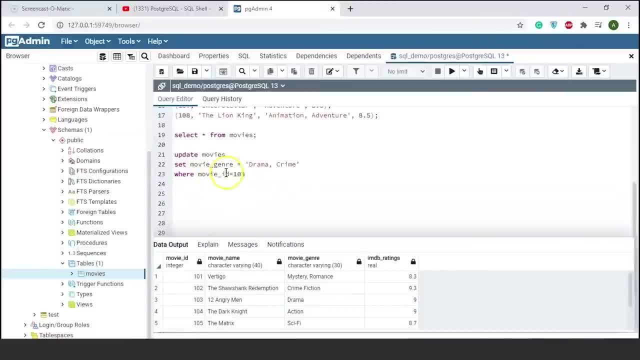 so I'll write where movie underscore ID. so I'll write where movie underscore ID is equal to one zero three. so here is equal to one zero three. so here is equal to one zero three. so here our movie ID is the unique identifier. so our movie ID is the unique identifier. so 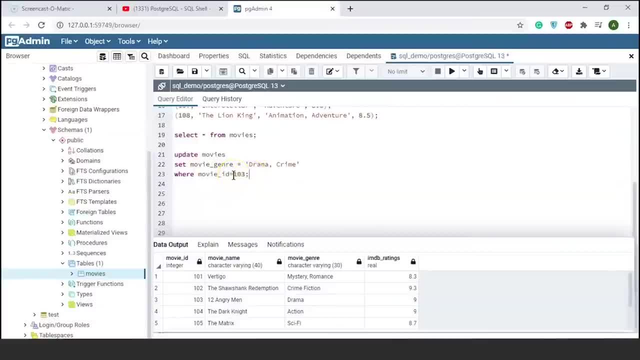 our movie ID is the unique identifier, so it will first look for movie ID 1 0 3 it. it will first look for movie ID 1 0 3 it. it will first look for movie ID 1 0 3. it will locate that movie and will change. 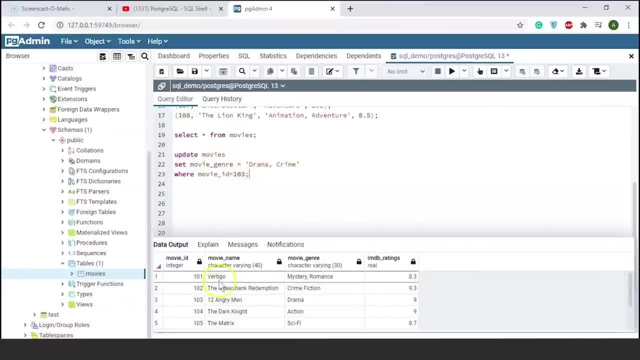 will locate that movie and will change. will locate that movie and will change the genre to drama and crime. so now you the genre to drama and crime, so now you the genre to drama and crime. so now you can see the difference earlier we had, can see the difference earlier we had. 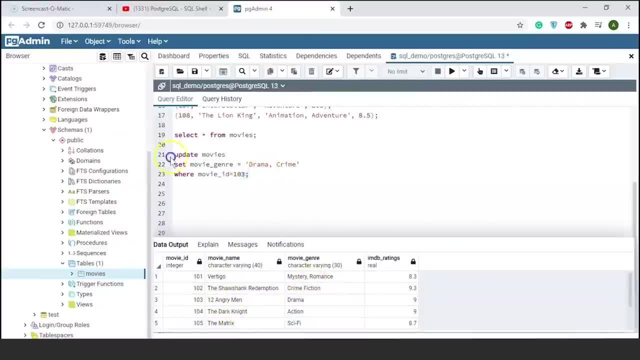 can see the difference. earlier we had 12 angry men as drama as the movie. 12 angry men as drama as the movie. 12 angry men as drama as the movie genre. now, if I run this update statement genre, now if I run this update statement genre, now if I run this update statement, okay, you can see we have successfully. 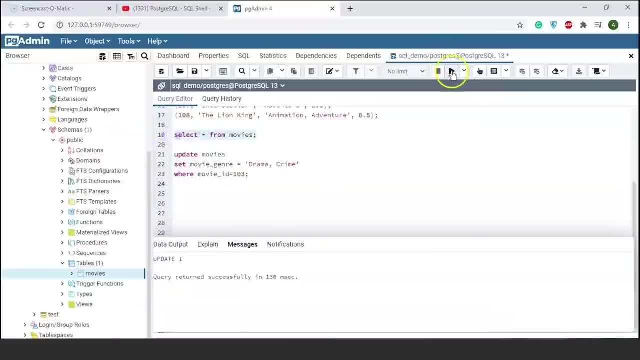 okay, you can see we have successfully. okay, you can see we have successfully updated one record. now, let me run the updated one record now. let me run the updated one record now. let me run the select statement again. okay, so here you. select statement again. okay, so here you. 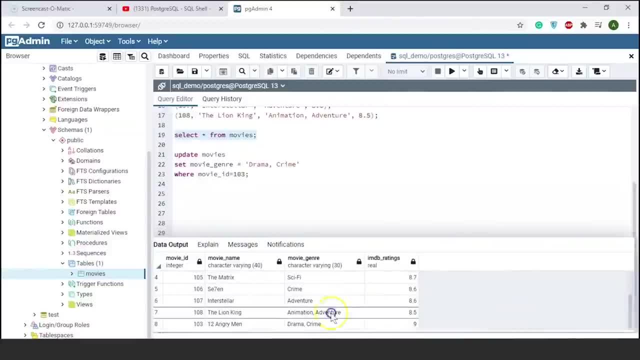 select statement again. okay, so here you can see if I scroll down there you go, so can see, if I scroll down there you go, so can see, if I scroll down there you go. so movie ID: 1: 0, 3. movie name: 12: angry men. 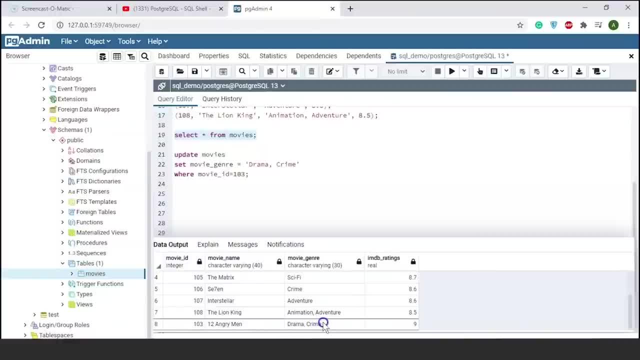 movie ID 1 0- 3. movie name: 12: angry men. movie ID 1 0- 3. movie name: 12: angry men. we have successfully updated the genre. we have successfully updated the genre. we have successfully updated the genre as drama comma crime. okay, now let me tell. 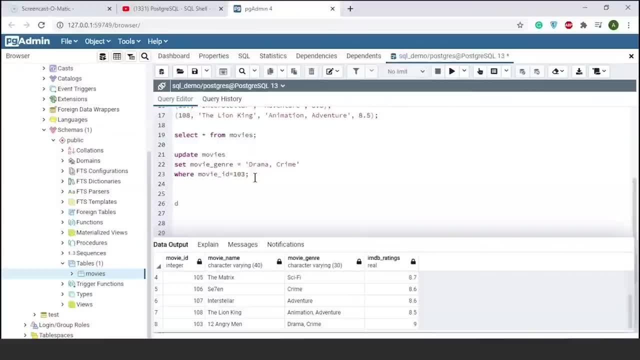 as drama comma crime. okay, now, let me tell as drama comma crime. okay, now let me tell you how you can delete records from a you, how you can delete records from a you, how you can delete records from a table, so for that you can use the delete. 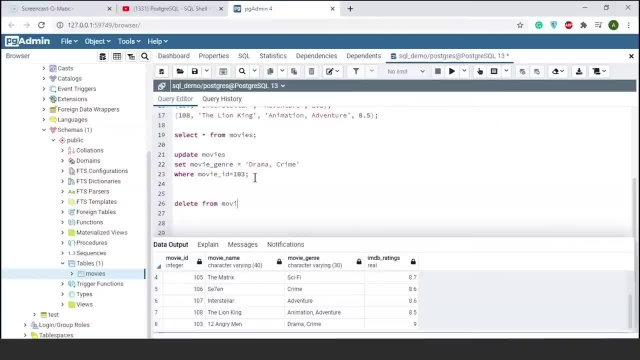 table. so for that you can use the delete table. so for that you can use the delete command. so you'll write delete from the command. so you'll write delete from the command. so you'll write delete from the table name. that is movies where let's table name. that is movies where let's. 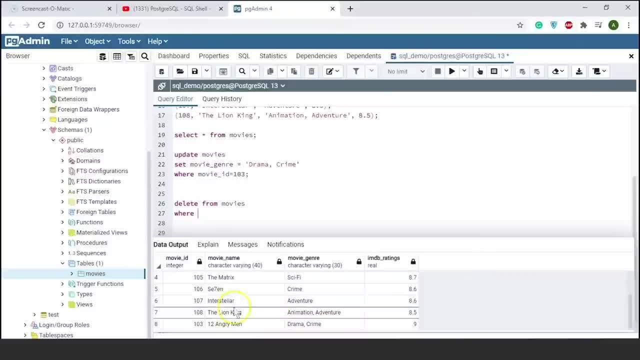 table name, that is, movies where let's say I want to delete the movie ID 1 0 8. say I want to delete the movie ID 1 0 8. say I want to delete the movie ID 1 0 8, which is the Lion King. so I'll write: 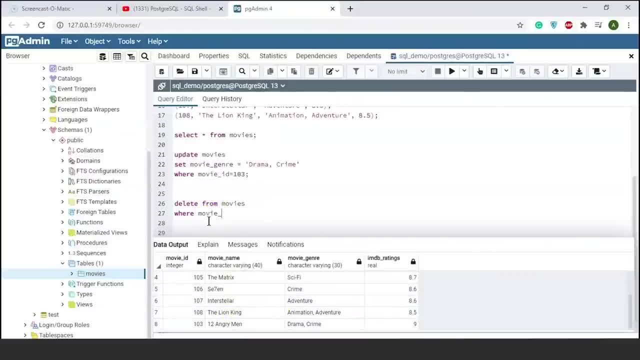 which is the Lion King, so I'll write which is the Lion King. so I'll write. where movie underscore ID is equal to 1: 0. where movie underscore ID is equal to 1: 0. where movie underscore ID is equal to 1 0- 8. this is one of the ways to delete this. 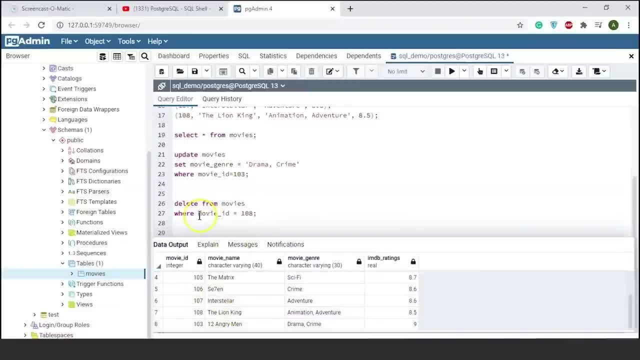 8. this is one of the ways to delete this. 8. this is one of the ways to delete this particular movie. or you can give let's particular movie, or you can give let's particular movie, or you can give, let's say, where movie name is equal to the. 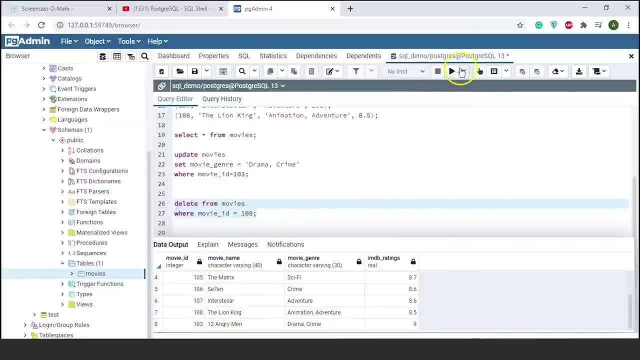 say where movie name is equal to the. say where movie name is equal to the Lion King. let me select this and I'll Lion King. let me select this and I'll Lion King. let me select this and I'll hit execute now if I run my select query. 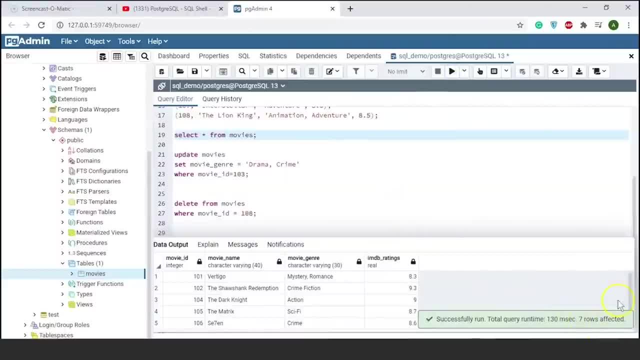 hit execute now if I run my select query. hit execute now if I run my select query again. you see, this time it has returned again. you see, this time it has returned again. you see, this time it has returned seven rows and you cannot find movie. seven rows and you cannot find movie. 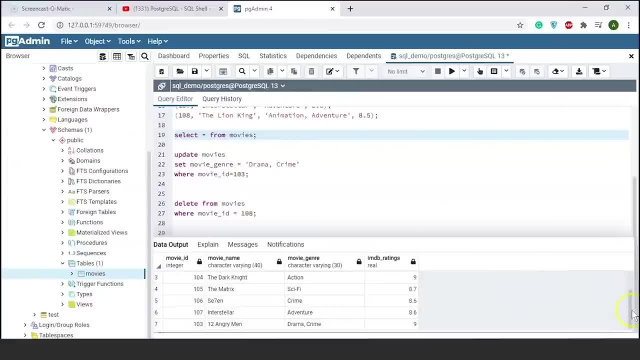 seven rows and you cannot find movie with movie ID 108- that was the Lion King. with movie ID 108, that was the Lion King. with movie ID 108, that was the Lion King. so we have deleted it all right next. so we have deleted it all right next. 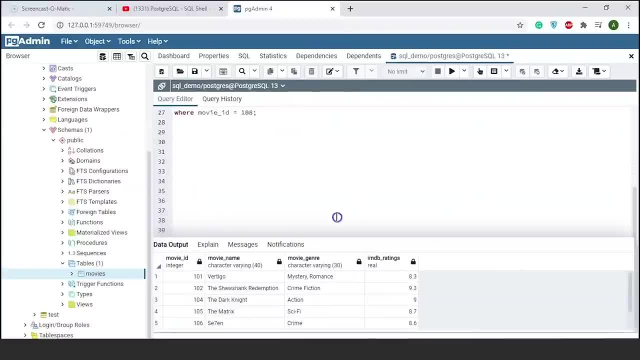 so we have deleted it all right. next, we are going to learn about where clause. we are going to learn about where clause. we are going to learn about where clause in postgresql. so to learn where clause in postgresql. so to learn where clause in postgresql. so to learn where clause. I'll be using the same movie table again. 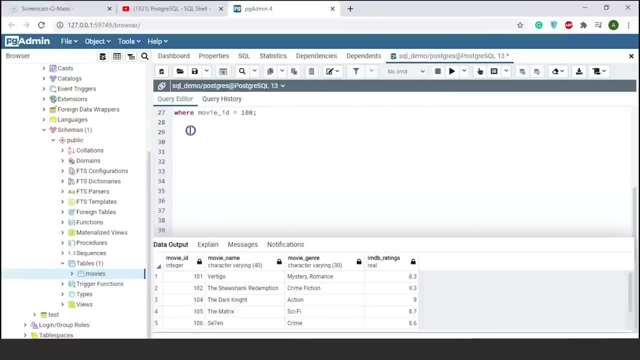 I'll be using the same movie table again. I'll be using the same movie table again. let's say we want to filter only those. let's say we want to filter only those. let's say we want to filter only those records for which the IMDB ratings of 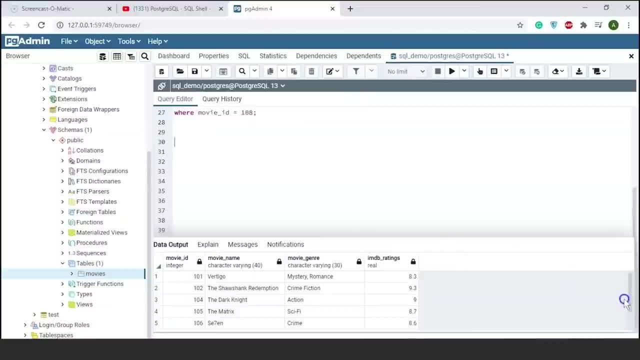 records for which the IMDB ratings of records for which the IMDB ratings of the movies is greater than 8.7. so this the movies is greater than 8.7. so this the movies is greater than 8.7. so this is my updated table. now I want to. 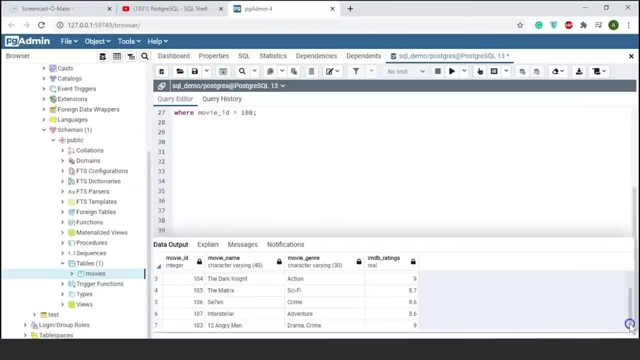 is my updated table now. I want to. is my updated table now. I want to display only those records or those movies. display only those records or those movies. display only those records or those movies whose IMDB ratings is greater than. whose IMDB ratings is greater than. 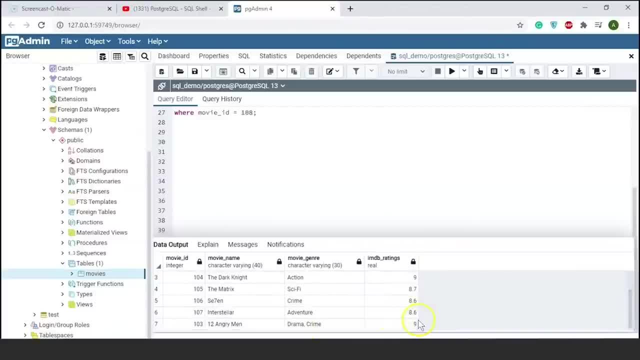 whose IMDB ratings is greater than 8.7. so we'll display 12 angry men, which is 8.7. so we'll display 12 angry men, which is 8.7. so we'll display 12 angry men, which is 9. then we are going to display the dark. 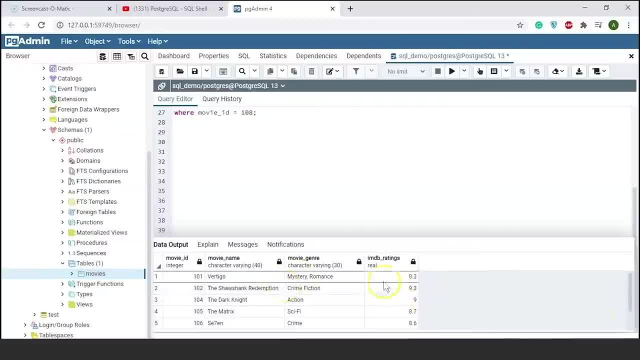 9, then we are going to display the dark 9, then we are going to display the dark night, which is again 9, and we are also night, which is again 9, and we are also night, which is again 9, and we are also going to display the Shawshank. 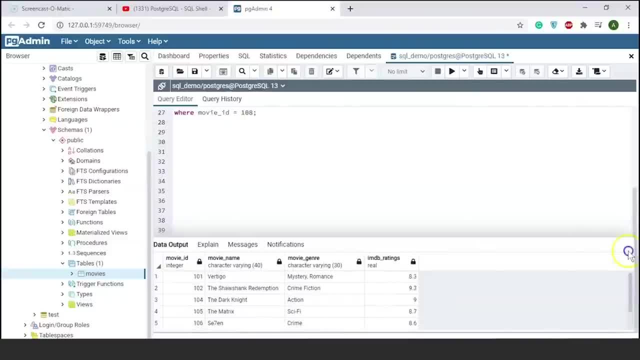 going to display the Shawshank. going to display the Shawshank Redemption, which has 9.3. the rest of the Redemption, which has 9.3. the rest of the Redemption, which has 9.3. the rest of the movies have an IMDB rating less than. 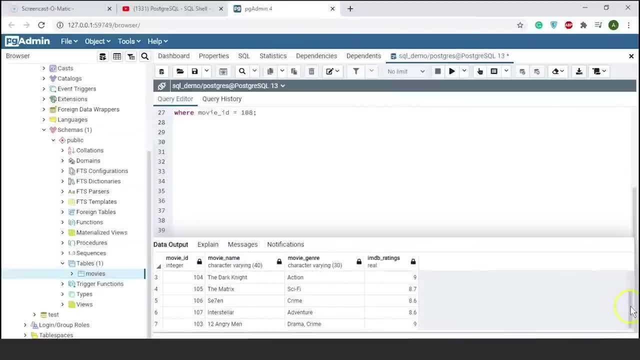 movies have an IMDB rating less than movies have an IMDB rating less than 8.7. so we are not going to display those 8.7. so we are not going to display those 8.7. so we are not going to display those. alright, so let me show you how to write. 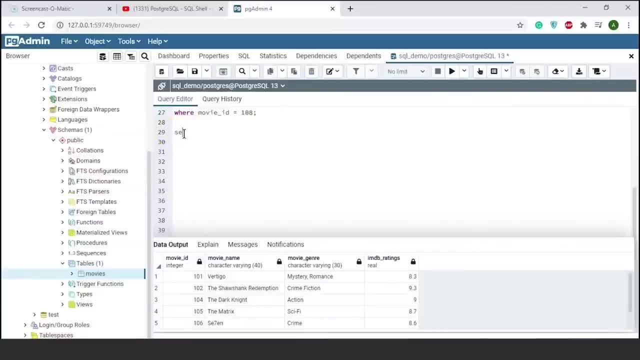 alright, so let me show you how to write. alright, so let me show you how to write a where clause. so I'll write select a where clause. so I'll write select a where clause. so I'll write select star from movies where I'll give my star, from movies where I'll give my 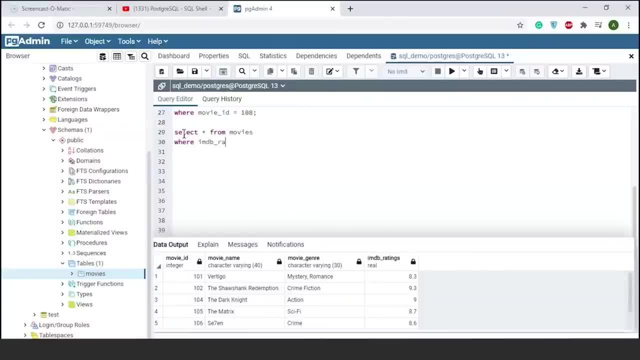 star from movies where I'll give my column name that is IMDB underscore column name that is IMDB underscore column name that is IMDB underscore. ratings is greater than I'll use the ratings is greater than I'll use the ratings is greater than I'll use the greater than symbol, then I'll pass my. 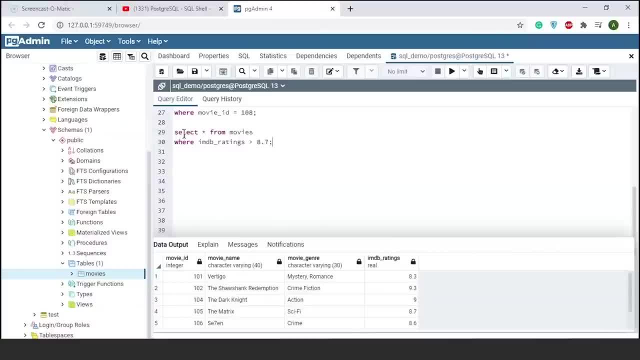 greater than symbol, then I'll pass my greater than symbol. then I'll pass my value that is 8.7. I'll give a semicolon value that is 8.7. I'll give a semicolon value that is 8.7. I'll give a semicolon and let's run it. I'll hit f5. there you. 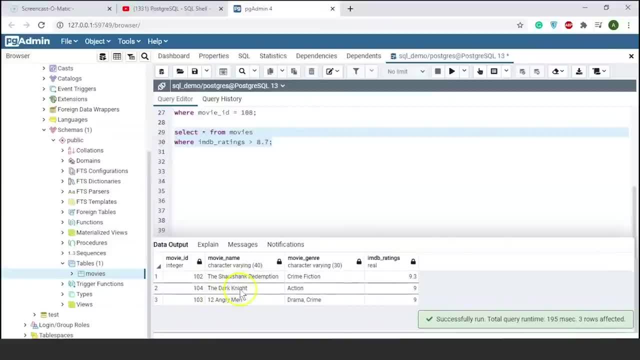 and let's run it, I'll hit f5. there you. and let's run it, I'll hit f5. there you go. so we have returned the source and go. so we have returned the source and go. so we have returned the source. and redemption, the Dark Knight and 12. 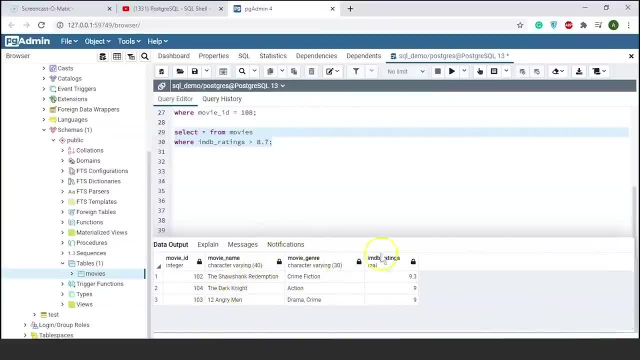 redemption, the Dark Knight and 12. redemption, the Dark Knight and 12 angry men. because only these movies had angry men, because only these movies had angry men. because only these movies had IMDB ratings greater than 8.7- okay now. IMDB ratings greater than 8.7- okay now. 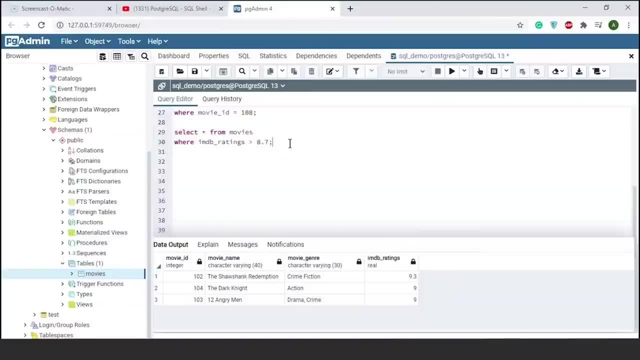 IMDB ratings greater than 8.7. okay, now, let's say you want to return only those. let's say you want to return only those. let's say you want to return only those movies which have IMDB ratings between movies which have IMDB ratings. between. 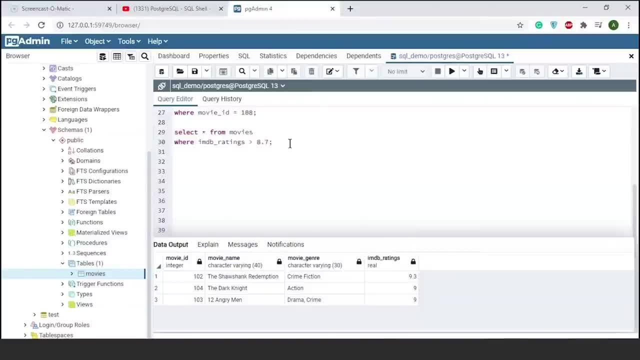 movies which have IMDB ratings between 8.5 and 9. so for that I am going to use 8.5 and 9. so for that I am going to use 8.5 and 9. so for that I am going to use another operator called between along. 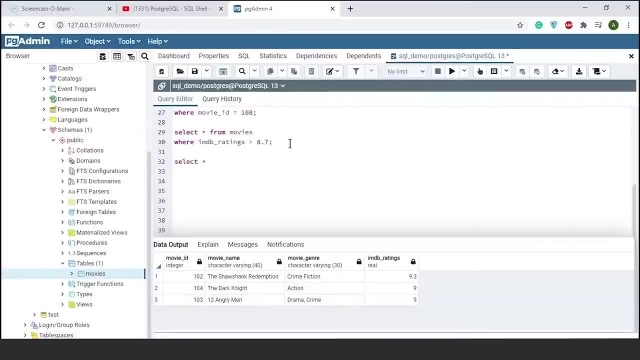 another operator called between, along. another operator called between along with the where clause. let me show you with the where clause. let me show you with the where clause. let me show you how to use between with where clause. how to use between with where clause. how to use between with where clause. I'll write. select star from movies where. 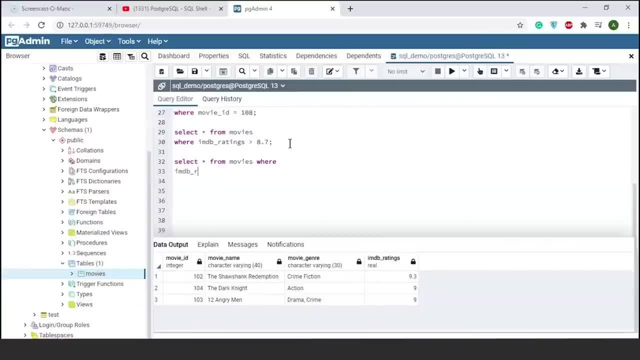 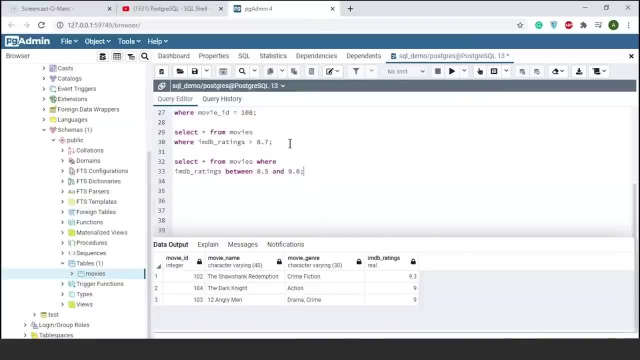 I'll write 8.5, I'll give an and operator. I'll write 8.5. I'll give an and operator. and 9.0. so all the movies that are and 9.0. so all the movies that are and 9.0, so all the movies that are between 8.5 and 9.0 ratings will be. 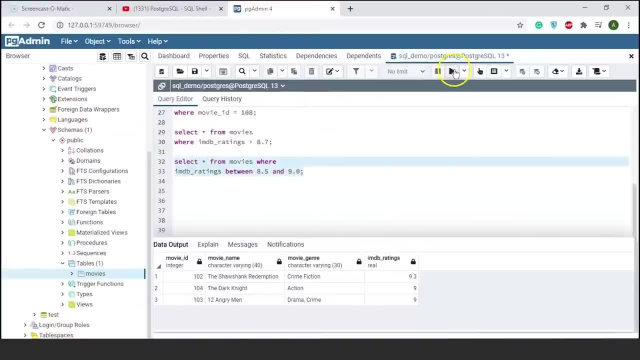 between 8.5 and 9.0 ratings will be: between 8.5 and 9.0 ratings will be displayed. so let's select this and I'll displayed. so let's select this and I'll displayed. so let's select this and I'll run it. there you go. so we have returned. 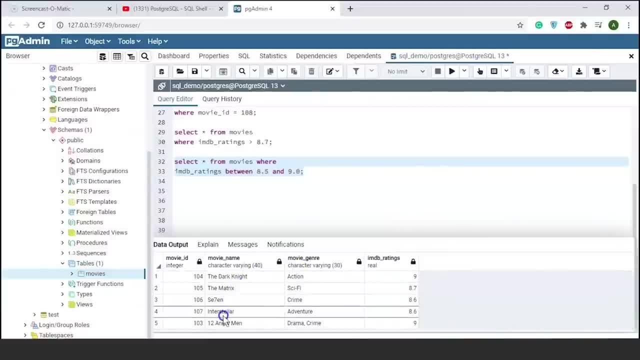 run it, there you go. so we have returned. run it, there you go. so we have returned the Dark Knight, the matrix, the seven, the Dark Knight, the matrix, the seven, the Dark Knight, the matrix, the seven, interstellar, and we have the 12 interstellar and we have the 12. 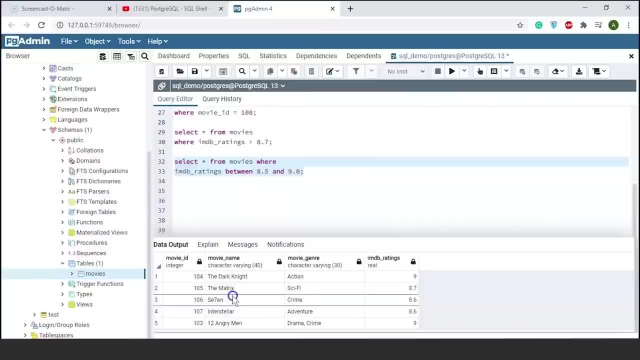 interstellar and we have the 12 angry men. so a few of the records that we angry men. so a few of the records that we angry men. so a few of the records that we missed out where I think vertigo which missed out where I think vertigo which. 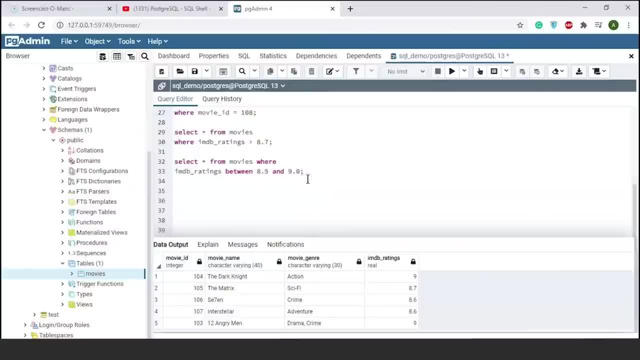 missed out where I think vertigo, which has 8.3, and there's one more. all right, has 8.3 and there's one more. all right, has 8.3 and there's one more. all right. now, moving ahead, let's say you want to. 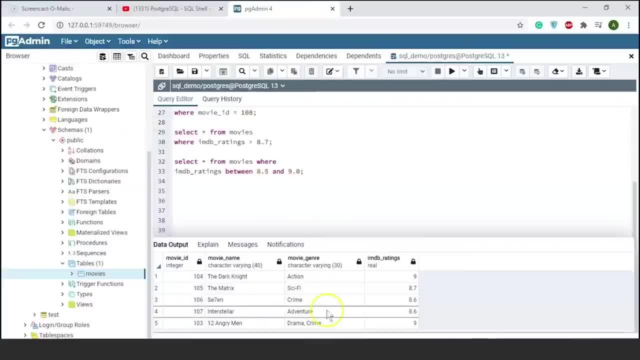 now moving ahead. let's say: you want to now moving ahead. let's say you want to display the movies whose movie genre is display, the movies whose movie genre is display, the movies whose movie genre is action. you can see in a table: we have a action. you can see in a table: we have a. 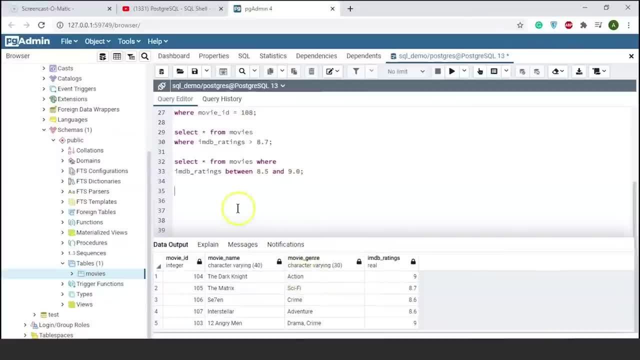 action. you can see in a table we have a few movies whose genre is action movie, few movies whose genre is action movie, few movies whose genre is action movie. so you can do that as well, I'll write. so you can do that as well, I'll write. 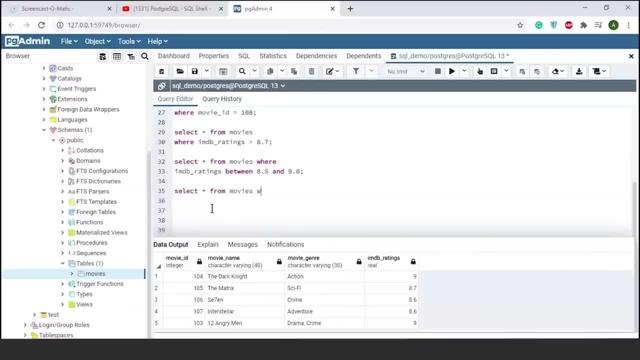 so you can do that as well. I'll write: select star from movies where the movie select star. from movies where the movie select star. from movies where the movie genre. I am writing this time in one line. genre. I am writing this time in one line. genre. I am writing this time in one line. you can break it into two lines as well. 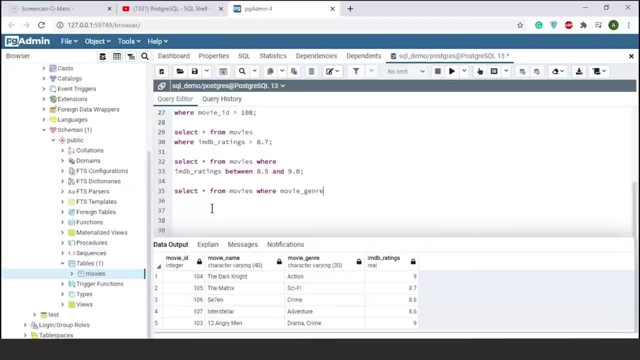 you can break it into two lines as well. you can break it into two lines as well. I'll write movie underscore genre. which I'll write movie underscore genre. which I'll write movie underscore genre, which is my column name equal to. I'll give. is my column name equal to? I'll give. 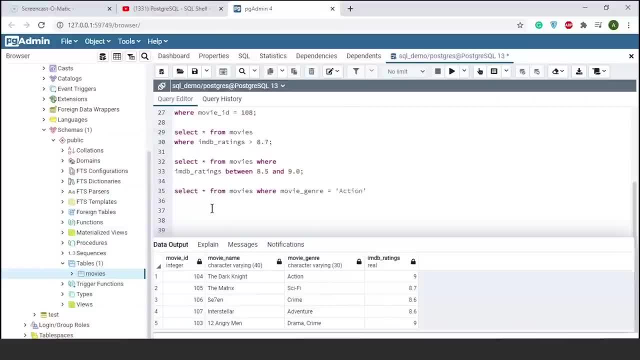 is my column name equal to. I'll give within single quotes action now. why? within single quotes action now. why within single quotes action now. why single code? because action is a string. single code because action is a string. single code because action is a string. hence we need to put it in single quotes. 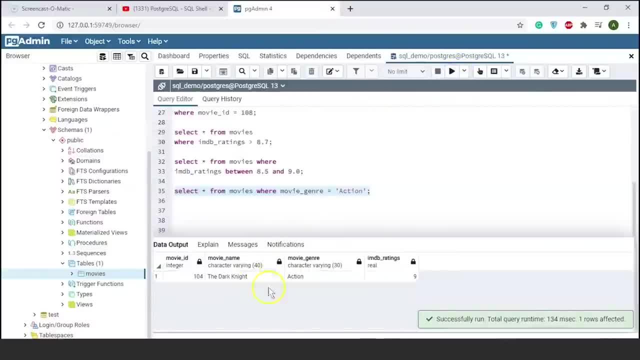 hence we need to put it in single quotes. hence we need to put it in single quotes: if I run this, there you go, so we had one. if I run this, there you go, so we had one. if I run this, there you go. so we had one movie in our table whose movie genre was: 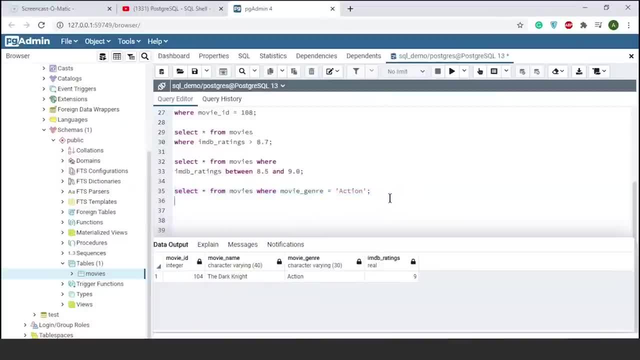 movie in our table. whose movie genre was movie in our table. whose movie genre was action: that is the Dark Knight. okay now, action that is the Dark Knight. okay now, action, that is the Dark Knight. okay, now you can also select particular columns. you can also select particular columns. 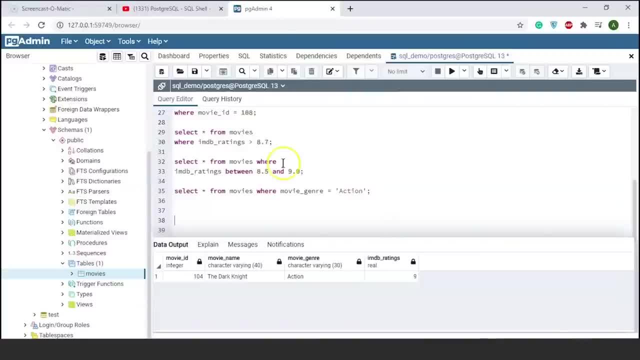 you can also select particular columns from the table by specifying the column from the table. by specifying the column from the table by specifying the column. names now here. names now here. names now here. in all the examples that we saw just now, in all the examples that we saw just now. 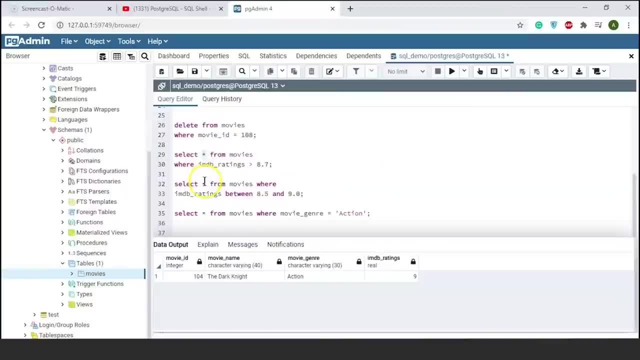 in all the examples that we saw just now. we are using star now star represents it. we are using star now star represents it. we are using star now star represents it. will select all the columns in the table. will select all the columns in the table. will select all the columns in the table. if you want to select specific columns. 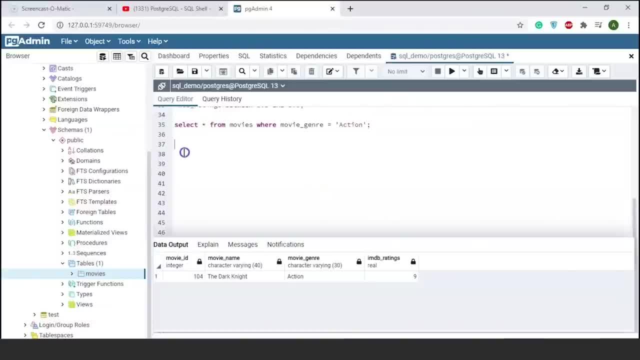 if you want to select specific columns. if you want to select specific columns in the table, you can use the column in the table. you can use the column in the table. you can use the column names so you can specify the column names. so you can specify the column. 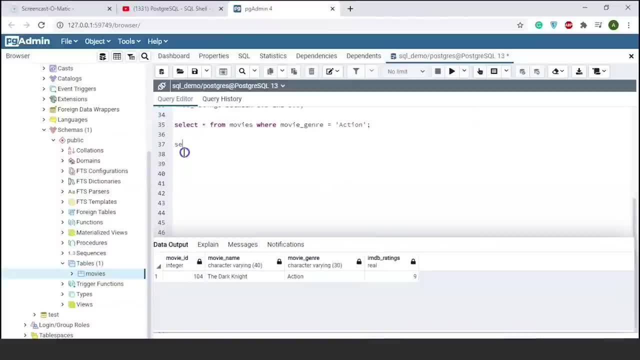 names so you can specify the column names in the select statement. let me show names in the select statement. let me show names in the select statement. let me show you. let's say, you want to display the names in the select statement. let me show you. let's say you want to display the. 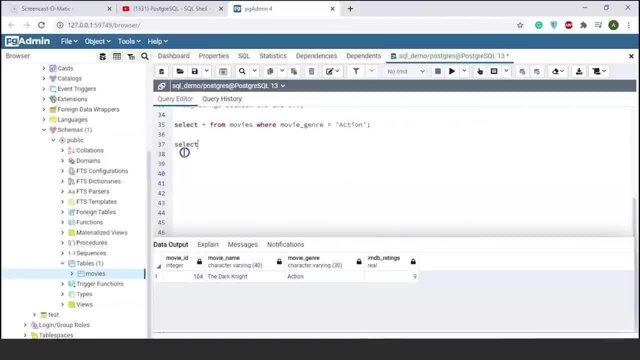 names in the select statement. let me show you. let's say you want to display the movie name and the movie genre from the movie name and the movie genre. from the movie name and the movie genre. from the table so you can write select movie table. so you can write select movie. 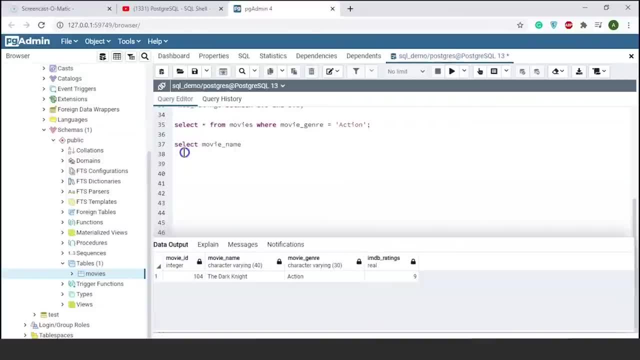 table so you can write select movie underscore name comma. I'll give the next underscore name comma. I'll give the next underscore name comma. I'll give the next column as movie underscore genre from my column as movie underscore genre from my column as movie underscore genre from my table name, that is, movies, where let's. table name. that is movies where let's table name. that is movies where let's say the imdb, say the imdb, say the imdb underscore, underscore, underscore, underscore from my table name. that is movies where let's say the imdb from my table name. that is movies where let's say the imdb. 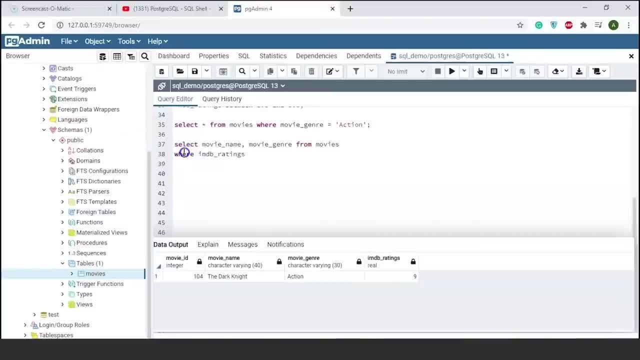 from my table name, that is, movies where, let's say, the imdb ratings is less than 9.0. so this time in our ratings is less than 9.0. so this time in our ratings is less than 9.0. so this time in our result it will only show two columns. 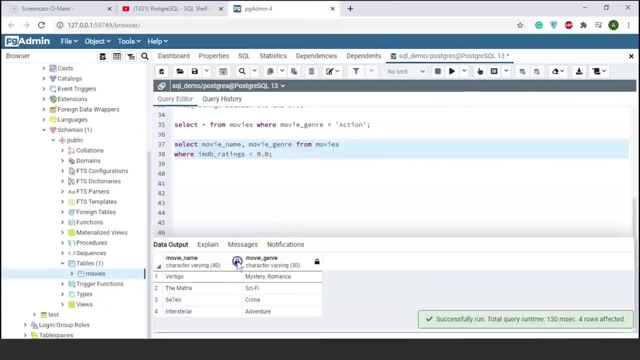 result: it will only show two columns. result: it will only show two columns. that is movie name and movie genre. let, that is movie name and movie genre. let, that is movie name and movie genre. let me run it, there you go. so these are the me run it, there you go. so these are the. 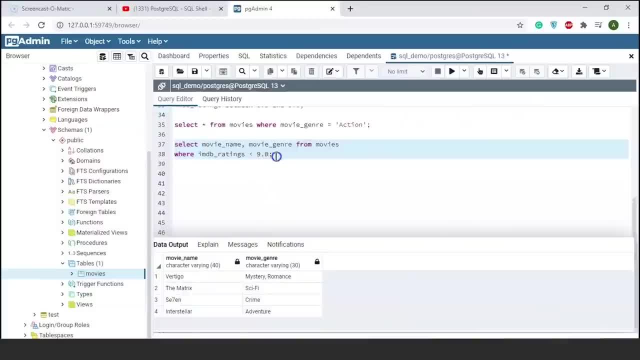 me run it. there you go. so these are the movie names and the movie genres. you can movie names and the movie genres. you can movie names and the movie genres. you can see that have an IMDB ratings less than see that have an IMDB ratings less than. 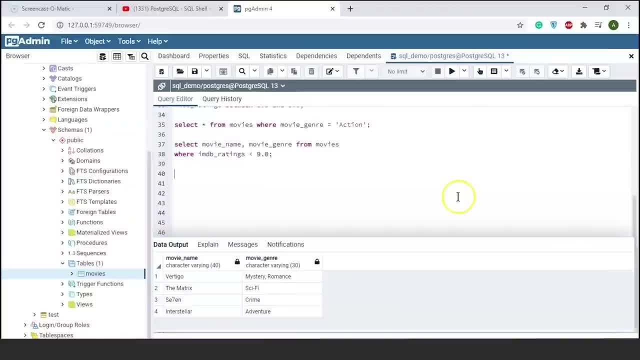 see that have an IMDB ratings less than 9.0. all right, like how you saw the 9.0. all right. like how you saw the 9.0. all right. like how you saw the. between operator. there is one more. between operator. there is one more. 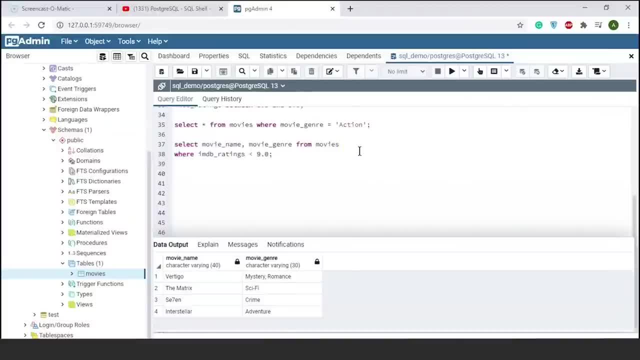 between operator. there is one more operator that you can use with the where operator that you can use with the where operator, that you can use with the where clause, that is the in operator. so the in clause, that is the in operator. so the in clause, that is the in operator. so the in operator works like a or clause or in. 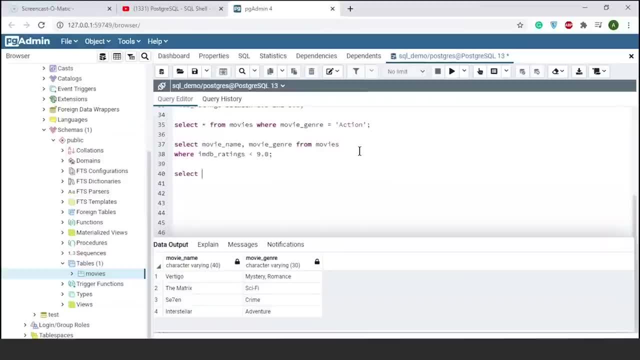 operator works like a or clause or in operator works like a or clause or in our operator. so let's say I want to our operator. so let's say I want to our operator. so let's say I want to select all the columns from my movies. select all the columns from my movies. 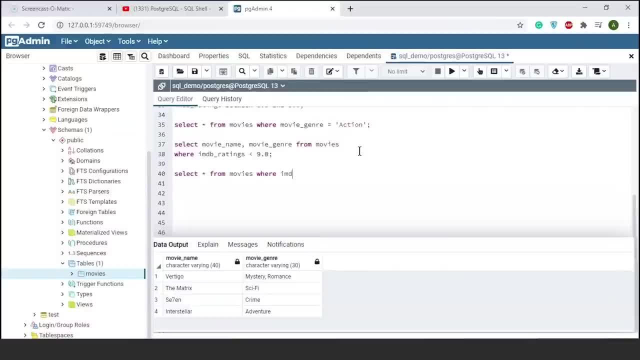 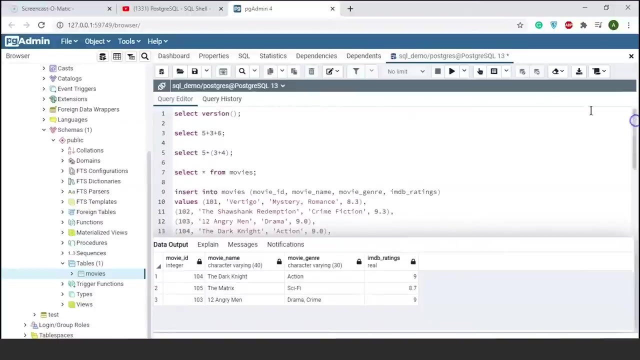 select all the columns from my movies table where the IMDB ratings is in 8.7 or 9.0. if I run this, it will display only those records whose IMDB ratings is 8.7 or 9.0. all right, so up to now we have looked at how you can work on basic. 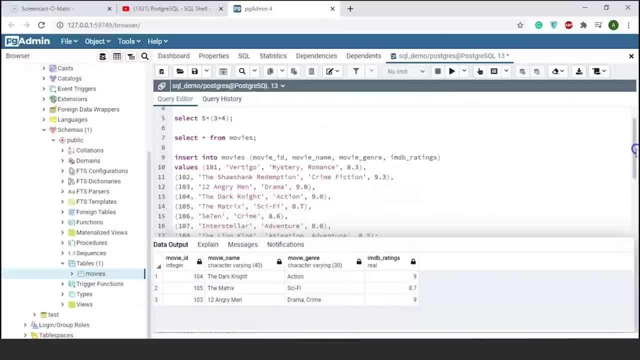 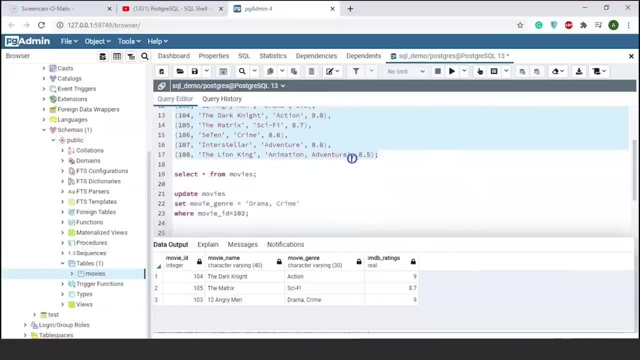 operations in SQL, like your mathematical operations. you saw how a select statement works. we created a few tables. then we inserted a few records to our tables. we saw how you can delete a table from your database and we have performed a few operations like update, delete and we saw how a where clause 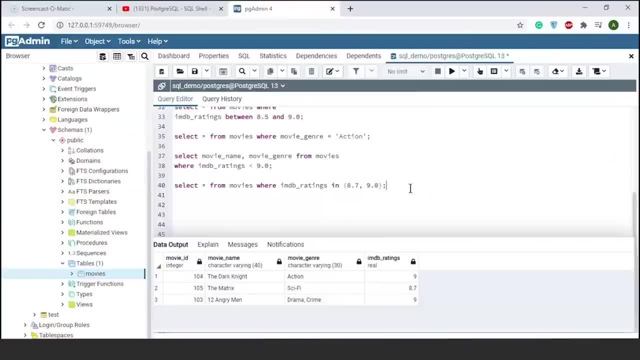 works. now it's time to load a employee CSV file or a CSV data set to Postgres SQL, so I will tell you how you can do that. you can do that in Postgres SQL, so I will tell you how you can do that. but first of all, before loading or inserting the records we need to create. 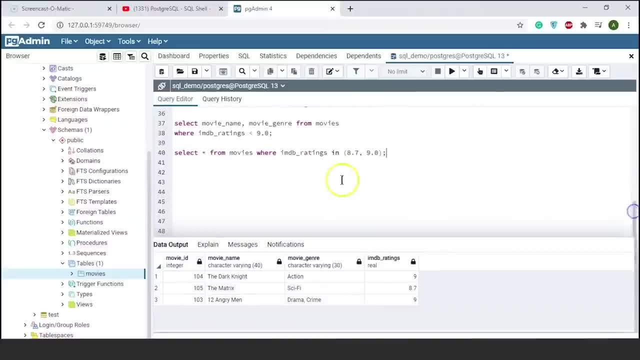 an employee table. so let me first go ahead and create a new table called employees in our SQL underscore demo database. so I'll write create table. my name of the table would be employees. next I'm going to give my column names. so my first column would be employees, and then I'm going to give my column names. 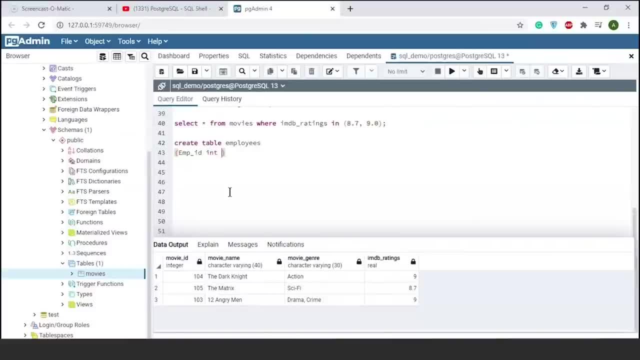 so the first column will be employee ID, so the table would be employee ID and then I will hit add and the type will be employee ID. so the employee ID will be of type integer. it is not going to contain any null values, so I'll write not null and I will give my constraint as primary key. so the 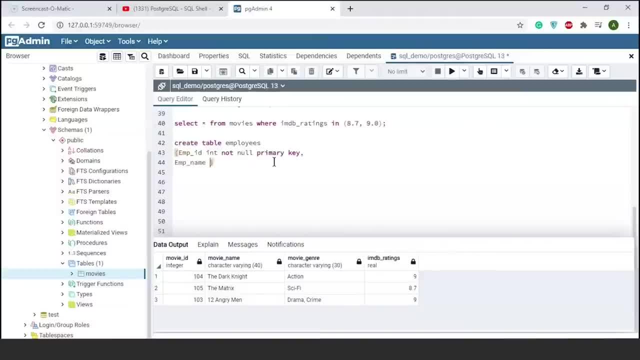 I'll have my employee name. so my employee name is going to be of type Varkar and I'll give my size as 40. okay, next we'll have the email address of the employee. again, email address would be of type Varkar and the size is 40 again. 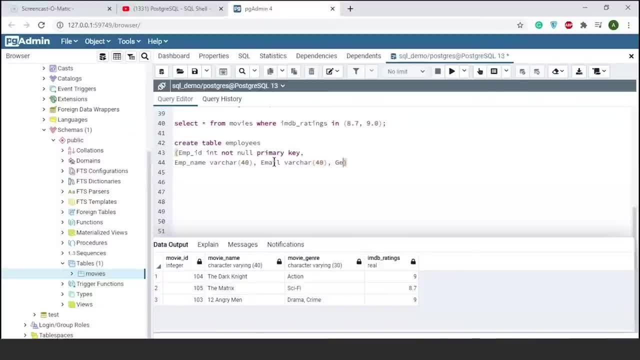 I'll give another comma. this time we'll have the gender of the employee. gender is again Varkar. of size, let's say 10. okay, now let's include a few more columns. we'll have the department column, so I'll write Department Varkar, let's. 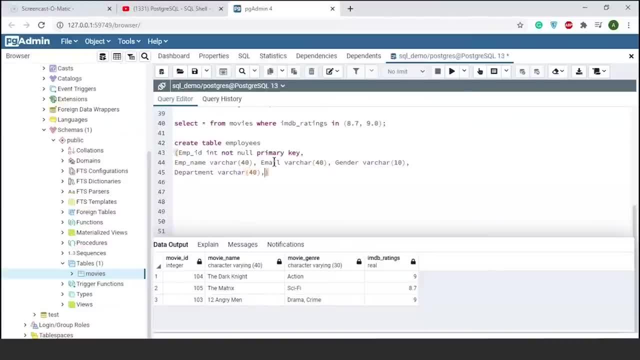 say the size is 40, then let's say we'll have one of the column that is called address. so the address column will have the name of the employee and the size of the employee, the country names of the employees address is also worker and finally we 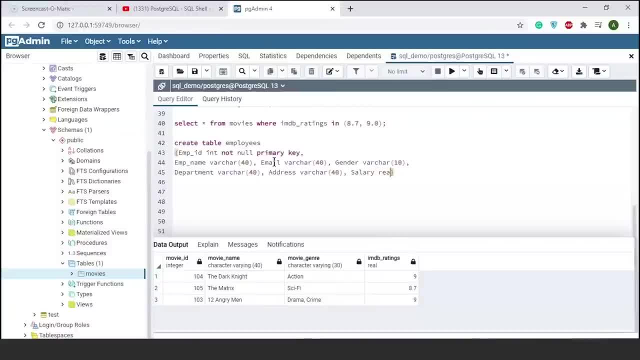 have the salary of the employee salary. I am going to keep it as type real, so real will ensure it will have decimal or floating-point values. okay, so now let me select this create table statement and execute it. alright, so we have successfully created our table. if you want, you can check by using select star. 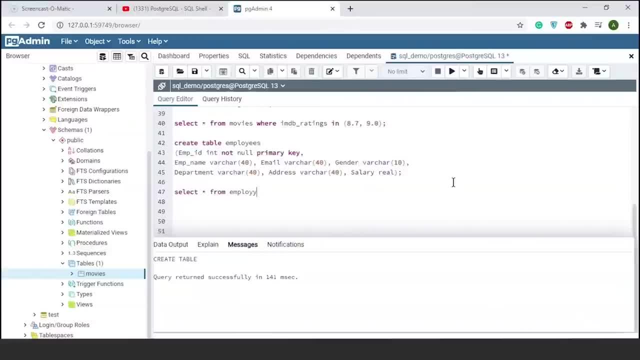 from employees. let me select this and I'll hit execute. all right, you can see. we have our employee ID as primary key. there's employee name, email, gender, this department address and salary, but we don't have any records for each of these columns. now it's time for us to insert a few records to our 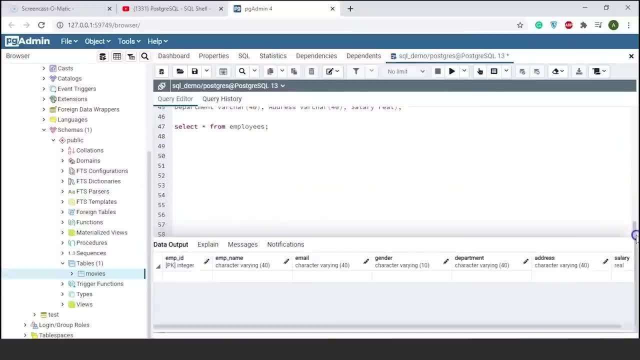 employee name and gender, but we don't have any records for each of these columns. now it's time for us to insert a few records to our employee table now. to do that, I am going to use a CSV file, so let me show you how the CSV 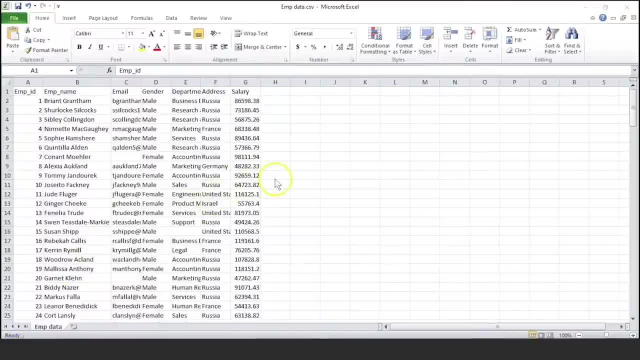 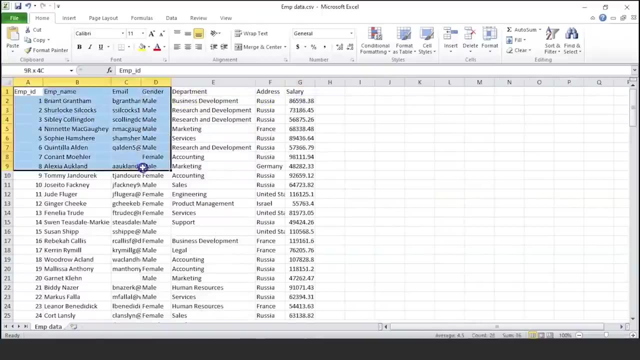 file looks like. okay. so now I am on my Microsoft Excel sheet and on the top you can see this is my employee data dot CSV file. here we have the employee ID, the employee name, email, gender, this department address and salary. now this data was generated using a simulator, so this is not validated and you can see it. 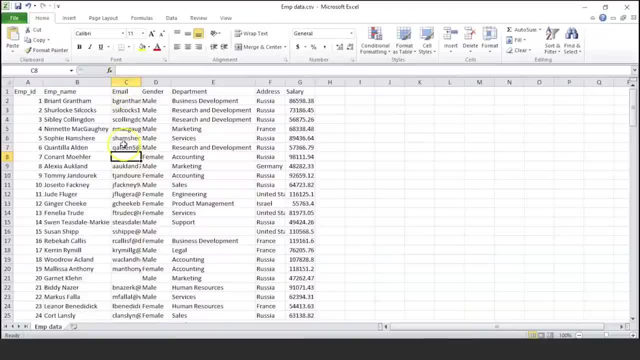 has a few missing records. so I am going to insert a few records to our employee data and you can see it has a few missing values. so under email column we have a few employees don't have an email ID. then you can see under department. also there are some missing values here, as 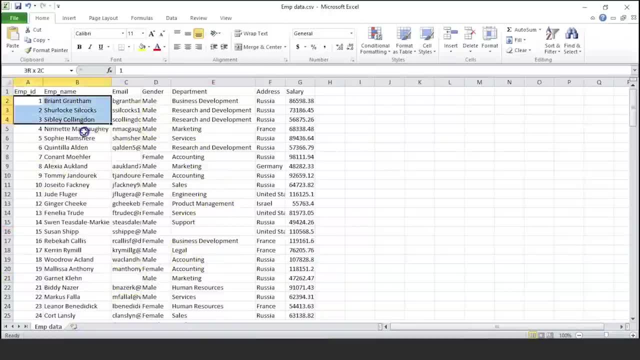 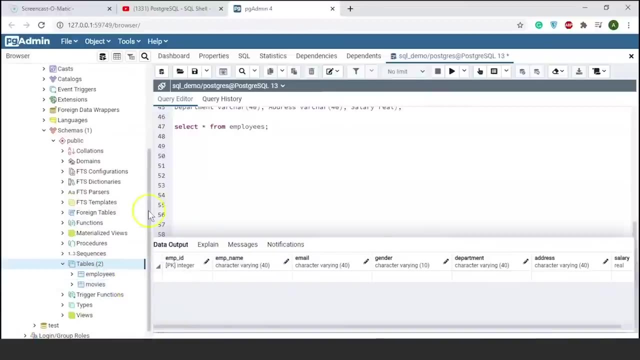 well, all right, so we'll be importing this table, or the records present in this CSV file, on to postgresql, all right, so here in the left panel under tables, let me right click and first refresh this. there you go. so initially we had only movies table, and now we also have the employees table. now what we need to do: 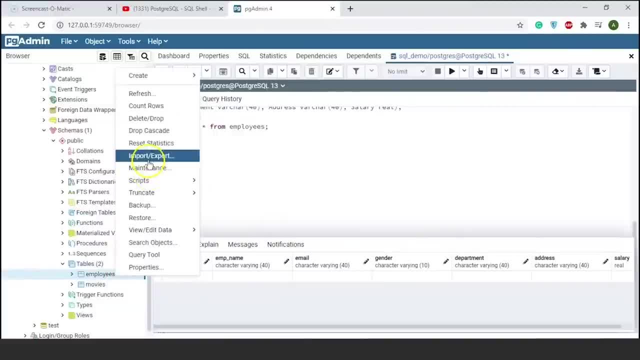 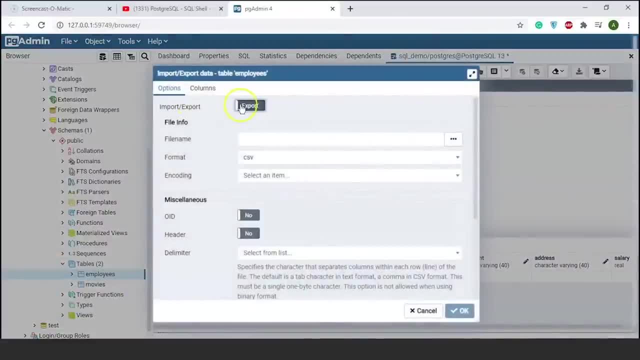 is, I will right click again and here you see, we have the option to import or export. let me click on this, and I don't want to export. I need to import, so I'll switch on import. all right now it is asking me to give the file location, so 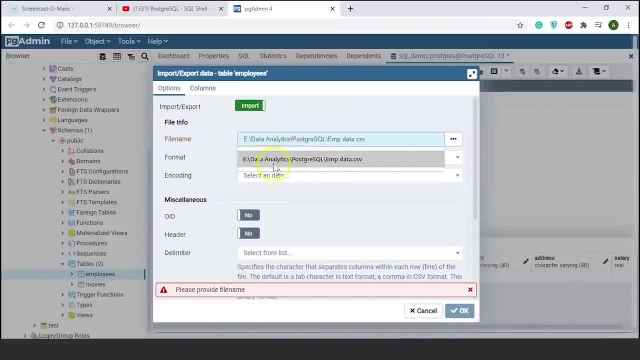 let me show you how to get the file location. so this is my file location actually. so my excel file, which was this, is present in my eDrive. under the data analytics folder I have another folder called postgresql, and within the postgresql folder I have my CSV file, that is, employee data, DOS, CSV. so I'll 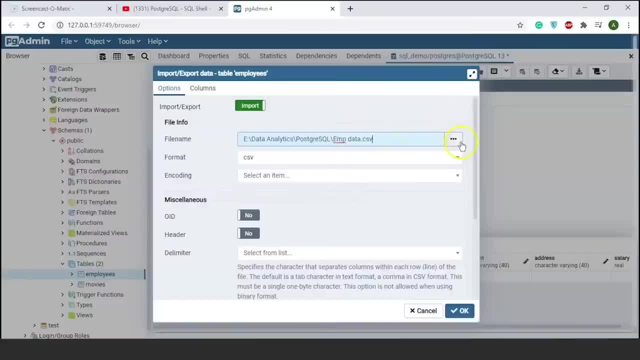 just select this. you can either do it like this or you can browse and do: okay, now my format is CSV. next I am going to select my headers as yes, and then let me go to columns and check if everything is fine. alright, so I have all my columns here, let's click on. 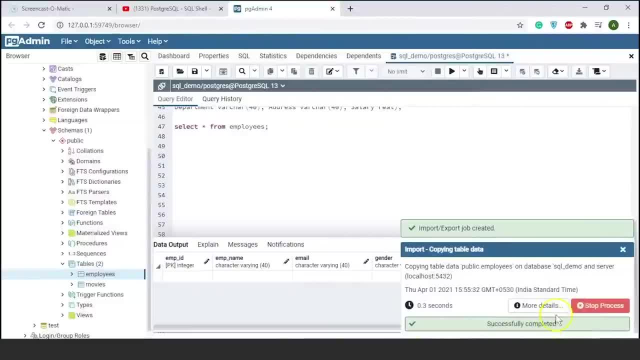 ok, you can see. I have a message here which says import underscore export: alright. so here you can see: successfully completed. we can verify this by using select star from employees. again, if I run this, all right, let me close this. there you go. it says 150 rows affected, which means 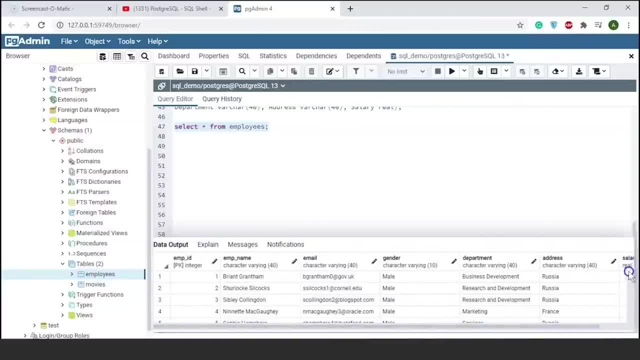 we have inserted 150 rows of information to our employees table. you can see we have the employee ID. these are all unique. we have the employee name, the email, we have the address and the salary. let me scroll down so that, okay, you can see we have 150 rows of information. that means we have 150 employees in our table. 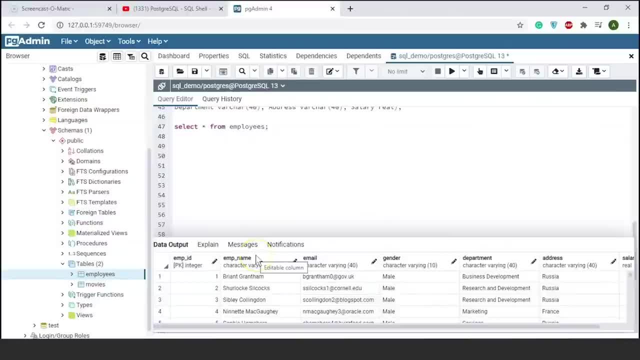 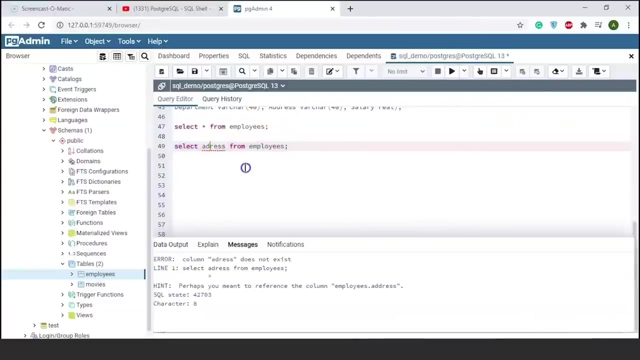 okay, now we are going to use this employees table and explore some advanced SQL commands. now there is an operator called extinct, so see, if I write select address from employees, this is going to give me 150 address of all the employees. there's some problem here. I did a spelling mistake. there should be another D. if I run this again, I'll query. 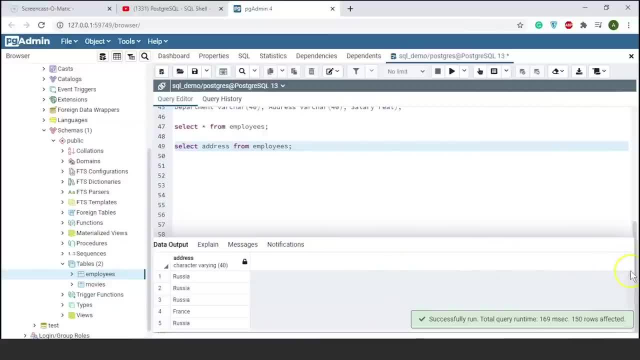 will return 150 rows. you can see we have the different country names under address. that is Russia, we have France, there's United States, we have Germany, okay, and I think we have Israel as well. yeah, now suppose you want to display only the unique address or the country names? you can use the extinct keyword. 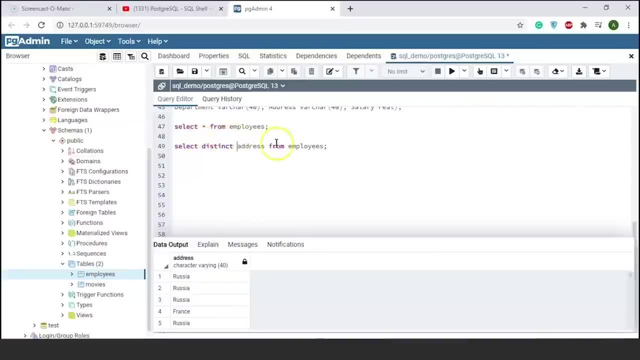 before the column name. so if I write select distinct address from employee, it will only display the unique country names present in the address column. if I run this see it has written us six rows of information. so we have Israel, Russia, Australia, United States, France and Germany. all right now, as I said there. 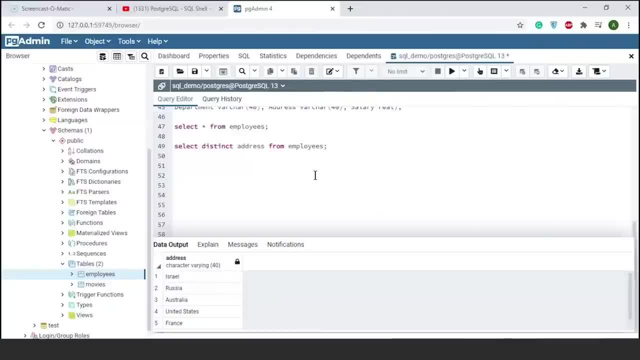 are a few null values which don't have any information, so you can use the is null operator in SQL to display all the null values that are there. suppose I want to display all the employee names where the email ID has a null value, so I like select star. 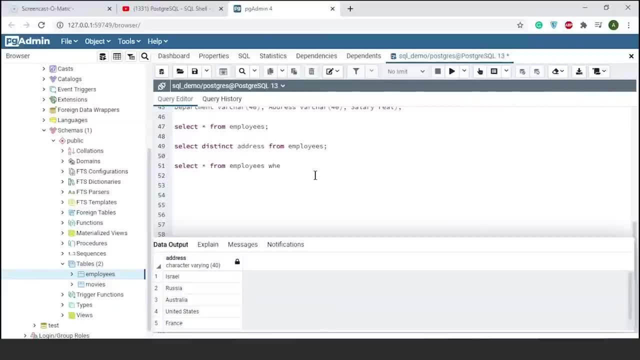 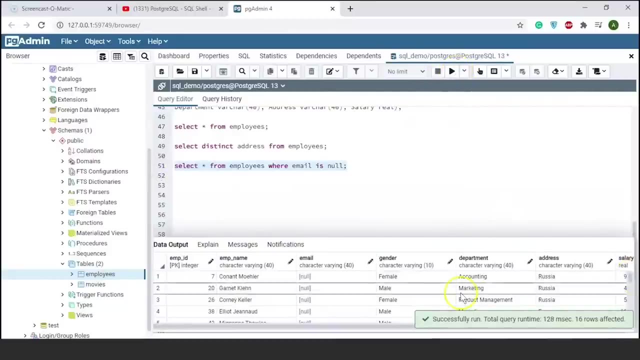 from employees where email is null. so this is another way to use your where clause. if I select and run this, there you go. so you see, here you can see all the here for all these employee names. there was no email ID present in the table, so it has returned us 16 rows of information, so around 10% of employees. 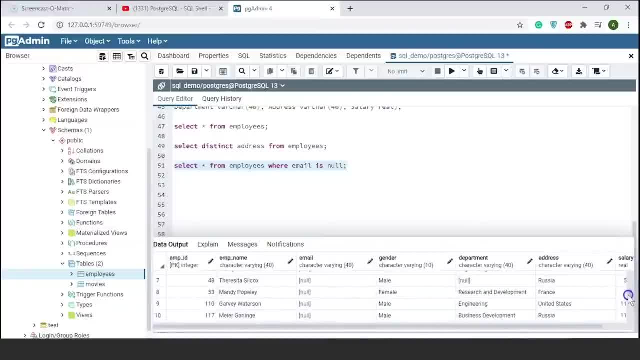 do not have an email ID and if you see a few of them do not have an email ID and also they don't have a department. so if you want to know for those employees which do not have a department, you can just replace where department is null. 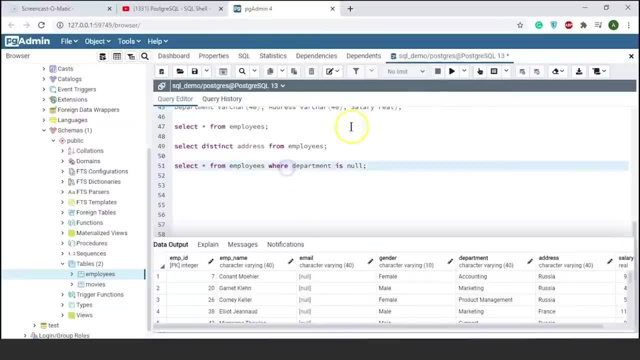 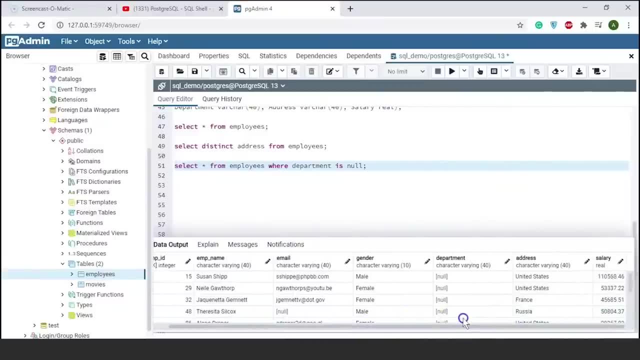 instead of where email is known. now, if I select this, okay, it has written dose: 9 rows of information, which means around 5% of employees do not have a department. moving ahead now let me show you how the order by clause works in SQL. now the order buy is used to order your result in a particular format. let's say: 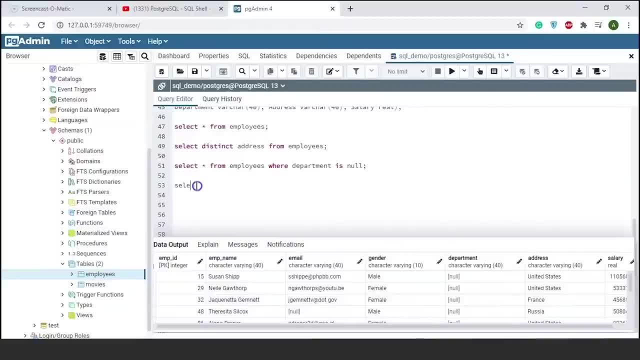 ascending or descending order. so the way to use is: let's say i want to select all the employees from my table, so i'll write select star from employees order by. i want to order the employees based on their salary, so i'll write order by salary. let me select and run it. 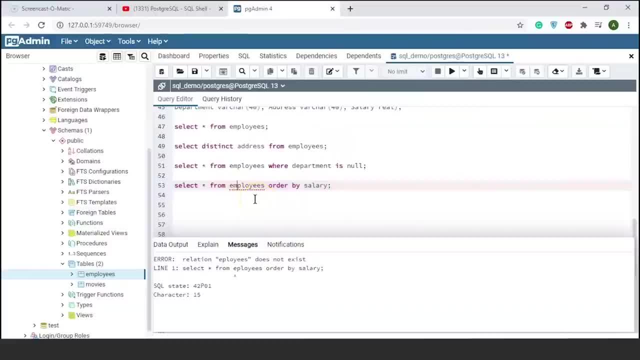 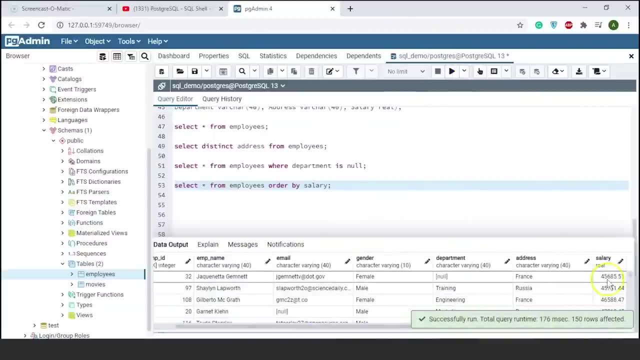 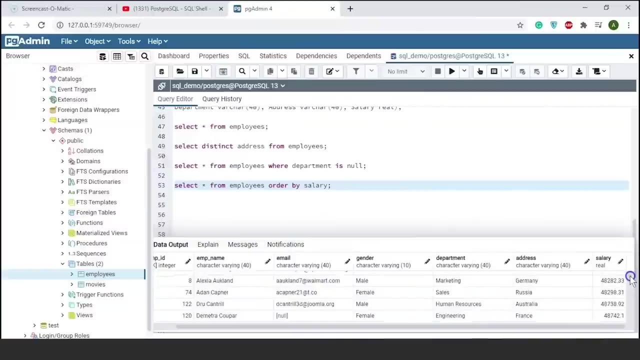 okay, there is some problem. i made a spelling mistake. this should be employees. let me run it again. okay, now, if you mark the output, a result has been ordered in ascending order. so all the employees which have salary greater than 45 000 appear at the top, and the 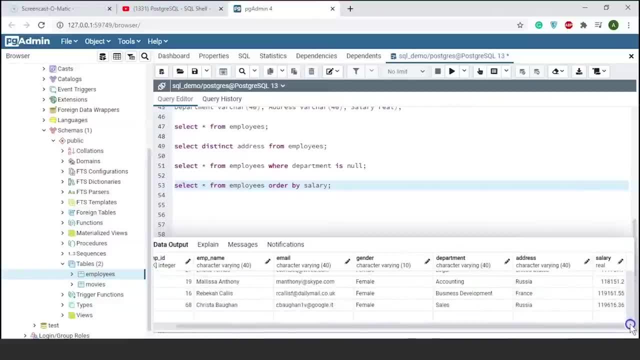 employees with the highest salary appear at the bottom. so this has been ordered in ascending order, which means your sql, or postgres sql, orders it in ascending order by default. now let's say you want to display the salaries in descending order so that all the top ranking employees in terms of salary appear at the top. 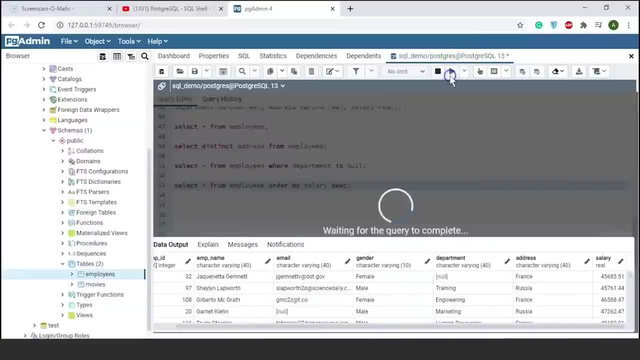 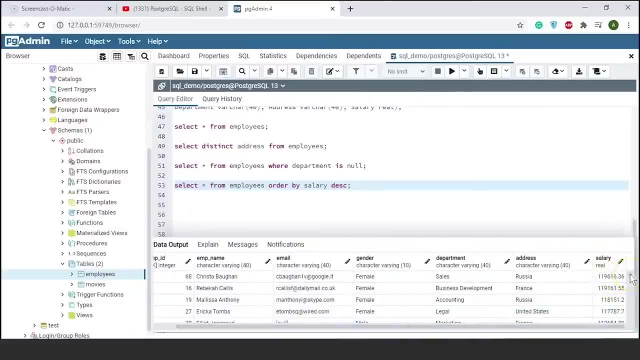 so you can use the desc keyword, which means descending. if i run this, you can see the difference now. so all the employees with the highest salary appear at the top, while those with the lowest salaries appear at the bottom. so this is how you can use an order by clause. okay, so now i want to make a 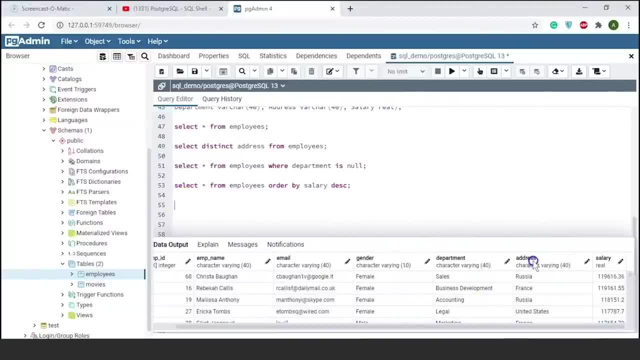 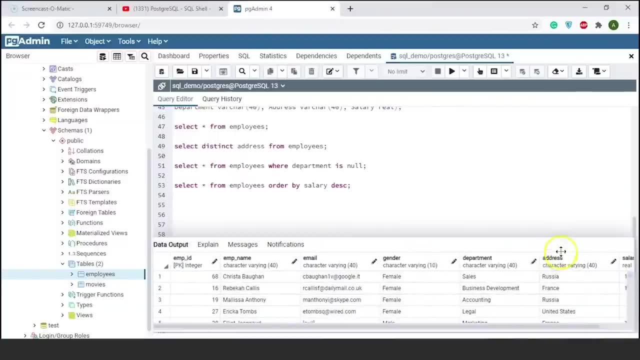 change in my existing table. so here, if you see, under the address column we only have the country names. so it would be better if we change the name of the address column to country. so i want to rename a column to country. you can do this using the alter command in PostgreSQL. so let me show you how to. 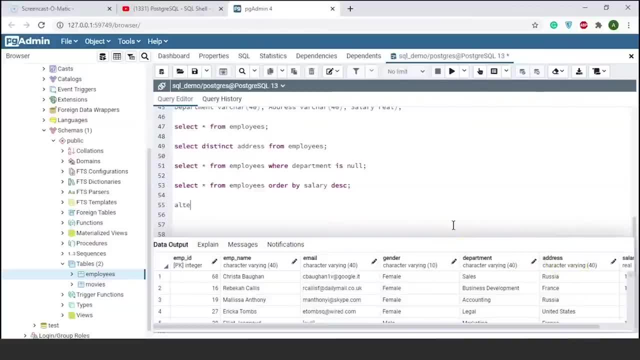 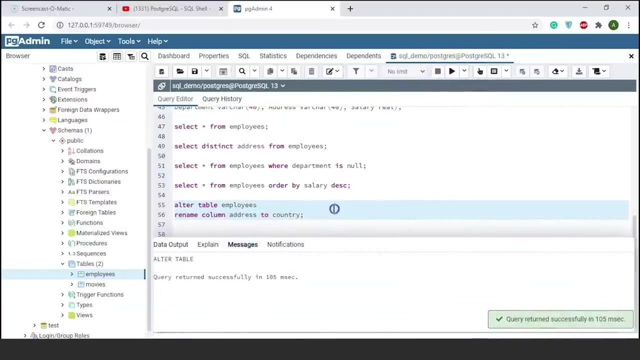 rename this column. that is address. so I'll write alter table followed by the table name, which is employees. then I'm going to use a rename column address. I'll write to: I want to change it to country. if I give a semicolon and hit execute, it will change my column name to country. now you can verify this if I run. 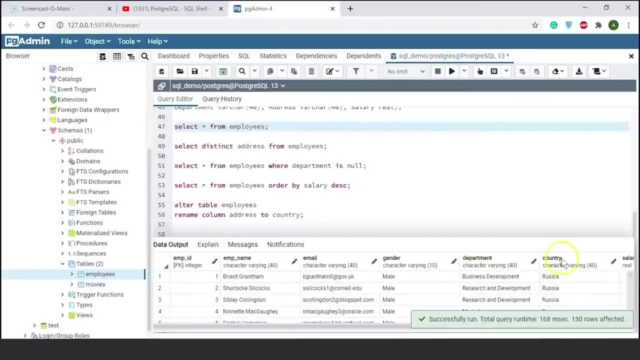 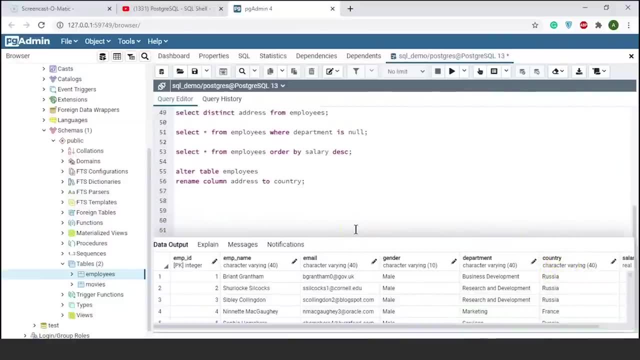 the select statement. again. there you go. earlier it was address column and now we have successfully changed it to country column. okay, let me come down now. it's time for us to explore a few more things in PostgreSQL. so let's go ahead and start a few more commands. so this time I'm going to tell you how an AND and an OR 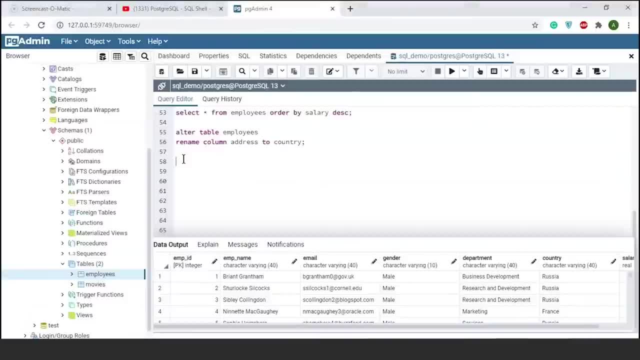 operator works in SQL, so you can use the AND and OR operator along with the WHERE clause. so let's say, I want to select the employees who are from France and their salary is less than $80,000. so let me show you how to do it. I'll write. 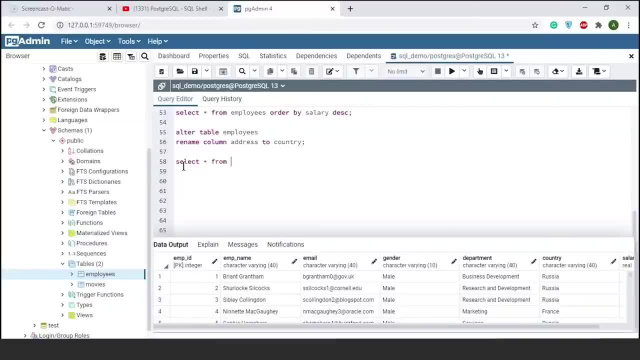 select star from employees where I'm going to give two conditions. so I'll use the AND clause or the AND operator. here I'll write where country is equal to France. now mark. here I'm not using address because we just updated our table and changed the column. 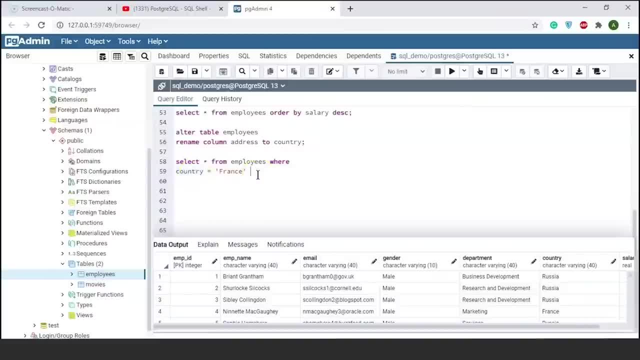 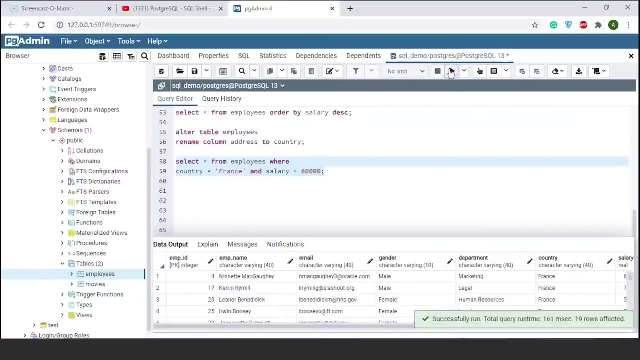 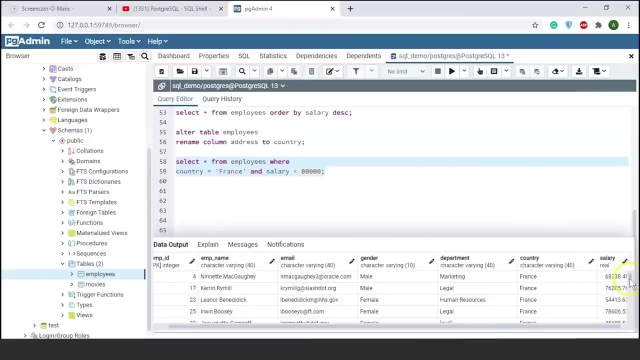 name from address to country. so I'll write country equal to France and my next condition would be: my salary needs to be less than $80,000. I'll give a semicolon. let me run this all right. so it has returned 19 rows of information. you can see all my country names of France and the salary is less. 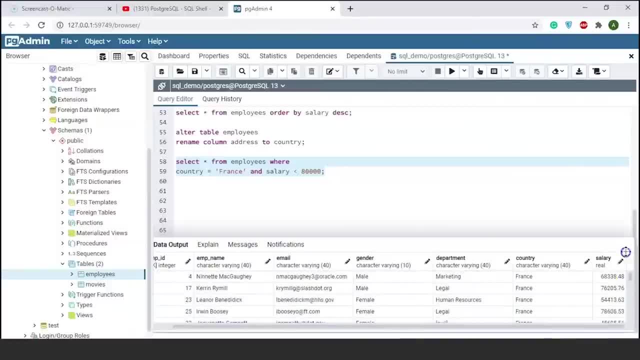 than $80,000. so this is how you can use or give multiple conditions in a WHERE clause using the AND operator. now let's say: let's use the AND operator to indicate that you want to use the or operator and less you want to know the employees who are from country Germany or the. 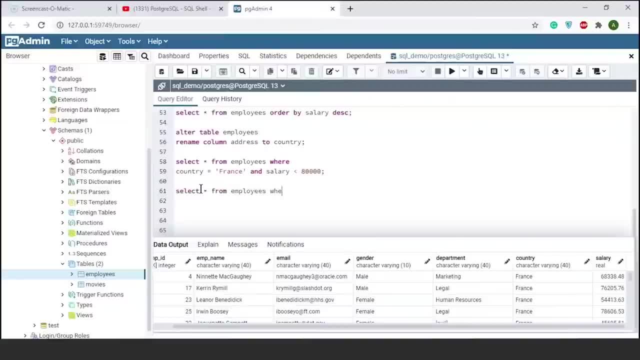 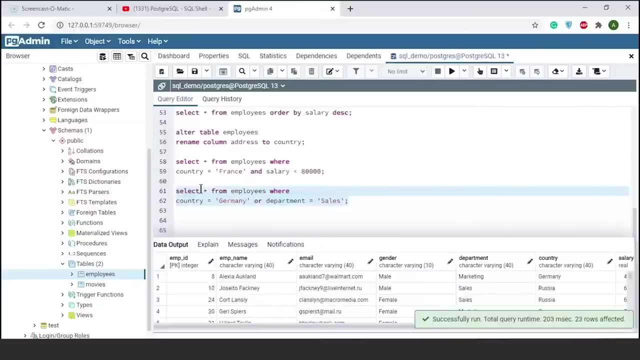 department should be sales. so I'll write select star from employees where country is equal to Germany and instead of- and I'm going to- or their department should be sales. okay, now let's see the output. i'll hit f5 this time to run it all right. so we have 23 rows of information now. 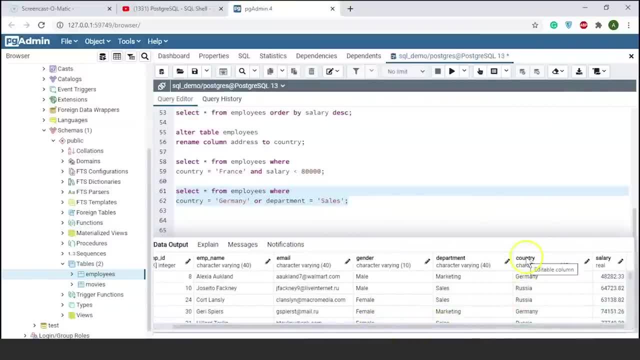 let me scroll to the right. you can see either the country is germany or the department is sales. you see one of them in the table. so here, for the first record, the country was germany. the second record: the department was sales. again, sales, again. for the fourth record, the country is: 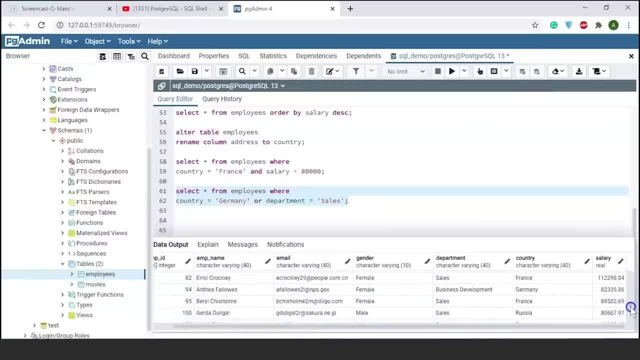 germany. so this is how the or condition works. so if one of the conditions are true, it will return the result. it need not be that both the conditions should satisfy. now in postgresql there is another feature that is called limit. so postgresql limit is an optional clause on the select statement. now this is used as a constraint. 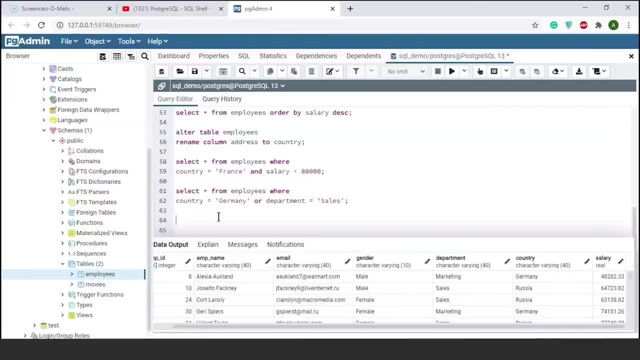 which will restrict the number of rows written by the query. suppose you want to display the top five rows in a table. you can use the limit operator. suppose you want to skip the first five rows of information and then you want to display the next five. you can do that using. 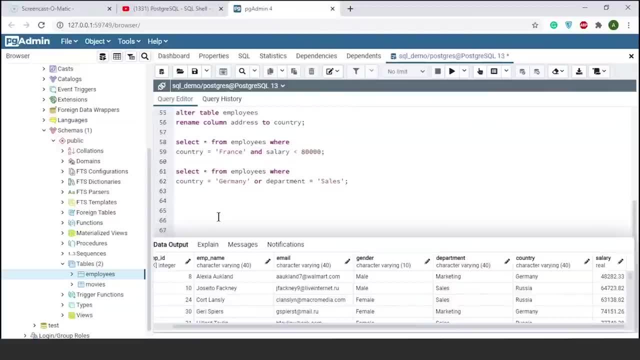 limit and offset. so let's explore how limit and offset works. i'll write select star from employees. let's say i'll use my order by clause. i'll write order by salary. let's say, in descending, and limit it to five. this is going to display the top five employees which have the highest salary. if i run this, the 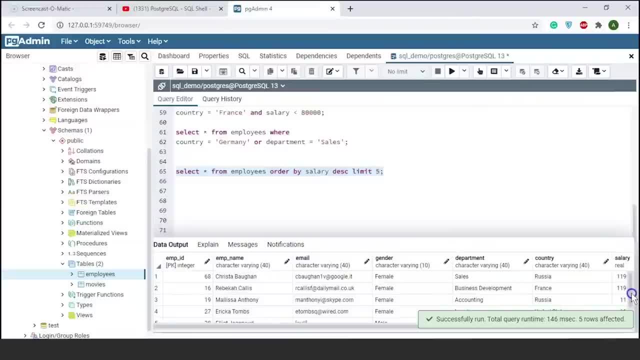 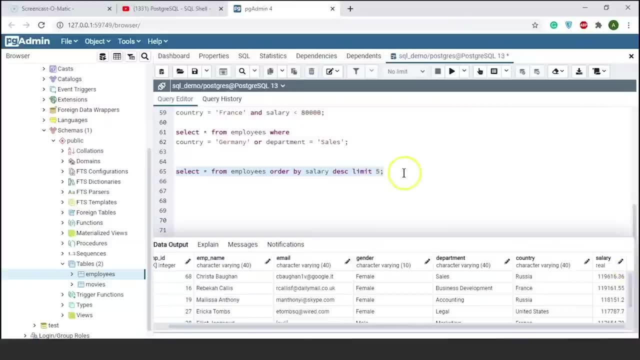 way you go. you see, it has given us five rows of information and these are the top five employees that have the highest salary. okay, so this is one method of or one way of using the limit clause. now, in case you want to skip a number of rows before returning the result, you can use offset. 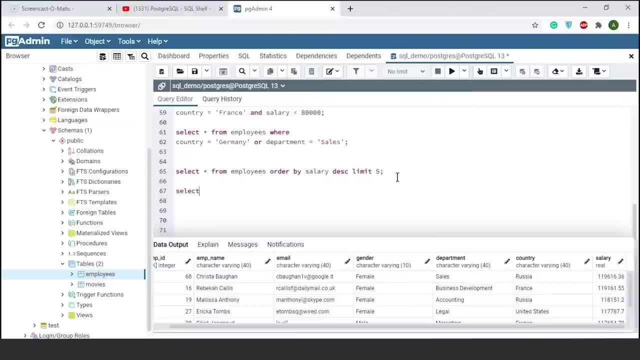 clause placed before the limit clause. so i'll write select star from employees, let's say order by salary descending. this time i'm going to use limit five and offset three. so what this query will do is it will skip the first three rows and then it will print the next five rows. if I run this, there you go. so this is how the result. 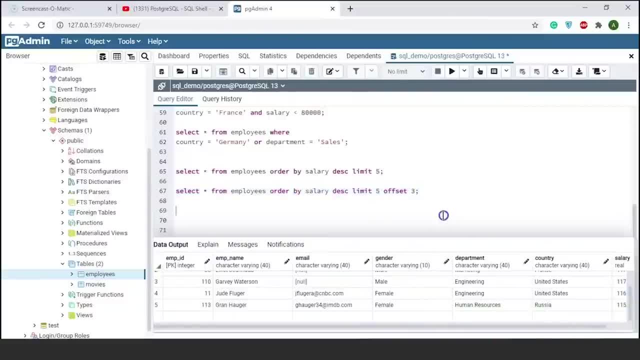 looks like okay. now there is another clause, which is called fetch. let me show you how that works. I'll copy my previous SQL query. I'll paste it here and here, after descending, I'm going to write fetch first, three row only. so my fetch is going to give me the first. 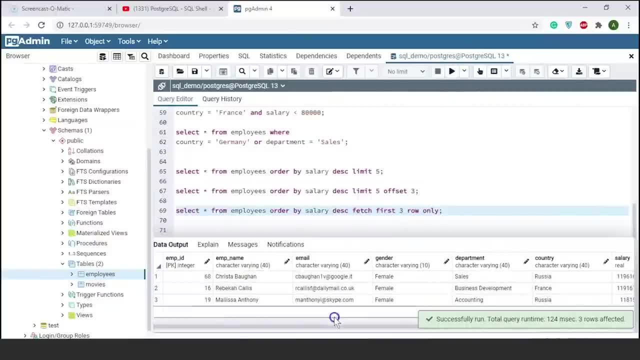 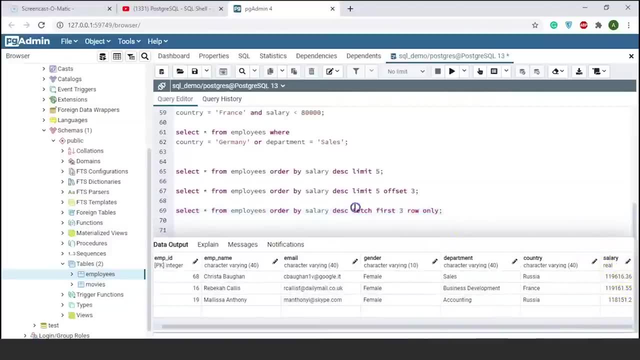 three rows from the top. there you go. it has given us the first three rows and you can see the top three employees that have the highest salary, since we ordered it in descending order of salary. all right, you can also use the offset along with the fetch clause. I'll copy this again and let 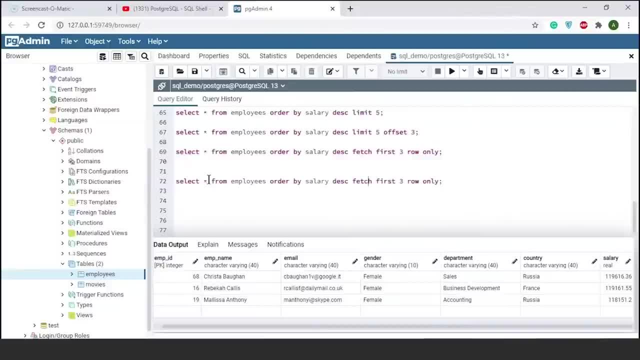 me paste it here now, after descending. I am going to write offset, let's say three rows, and fetch first five rows only. so what this SQL query is going to do is it will skip the first three rows and then it will give me the first three rows and then it will give 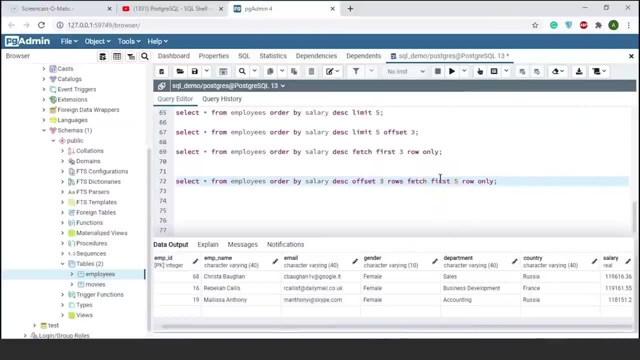 me the first three rows and then it is going to display the next five rows. it is going to work exactly the same as we saw for this query. let me run it. there you go. so these are the first five rows of information, after excluding the top three rows. all right, we 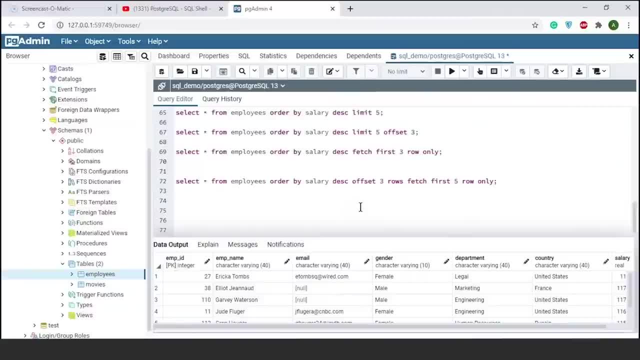 have another operator that is called as like in PostgreSQL. so like is used to do pattern matching. so suppose you have a table that has the employee names. you forgot the full name of an employee but you remember the few initials, so you can use the like operator to get an. 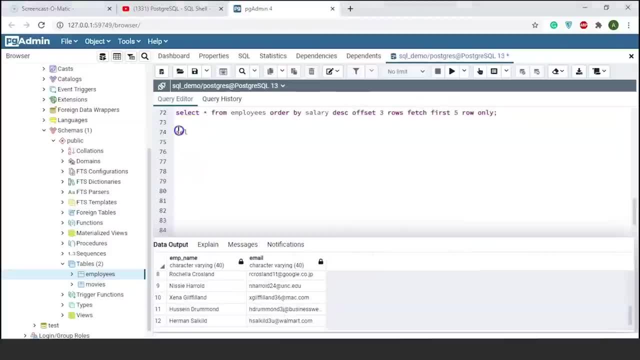 idea as to which employee name it is. now let's explore some examples to learn how the like operator works in PostgreSQL. so suppose you want to know the employees whose name starts with a, so for that you can use the like operator. let me show you how to do it. so I want to. 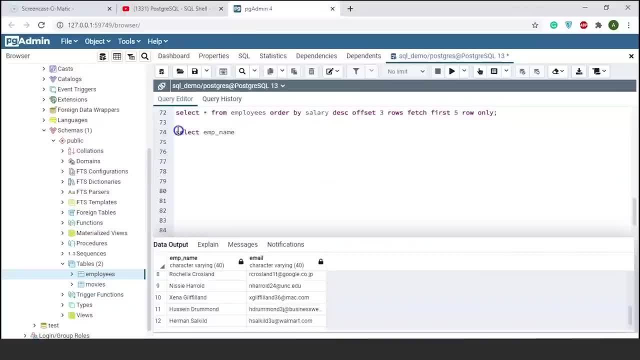 display the employee name and let's say, I want to know that email IDs from the table name that is employee where. since I want to know the employee whose name starts with a, so I will write employee name like now to use the pattern as within single course I. 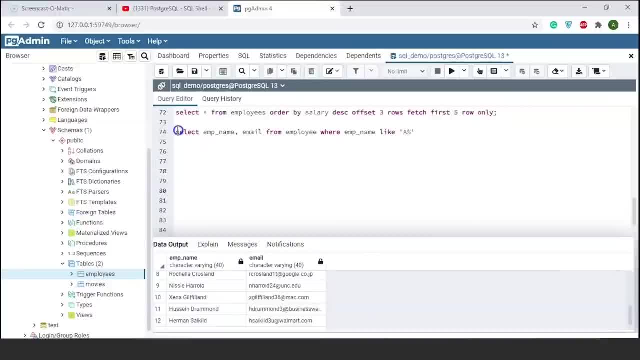 will write a and then followed by percentage. so this means I am going to know the employee name. that is employee name. I will write employee name and at the end I will write employee name means the employee name should have an a in the beginning and percentage suggests it can have any. 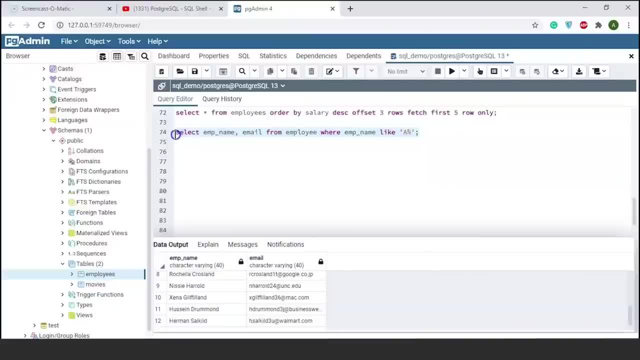 other letter following a, but in the beginning or the starting should be a. if i run this, so there is an error here. the name of the table is employees and not employee. let's run this again. there you go. you can see there are 16 employees in our table whose name starts with a. you can. 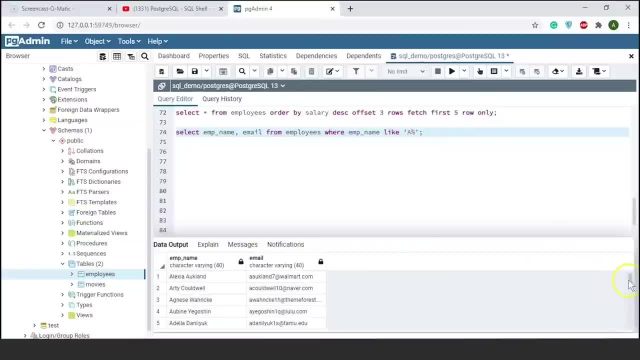 see this column employee name. all of them have a letter a in the big name. okay, now let me just copy this command or the query. i'll paste it here. let's say this time: you want to know the employees whose name starts with s, so instead of a i'll write s. so this means the starting. 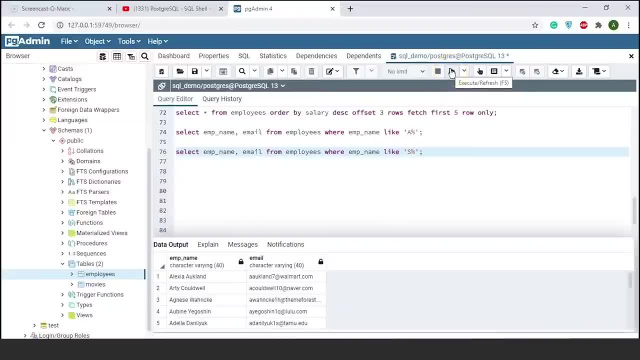 letter should be s and followed by it can have any other letter. if i run this, so there are 10 employees in the table whose name starts with a, so this means the starting letter should be s with S. okay, let's copy the query again, and this time I want to know the. 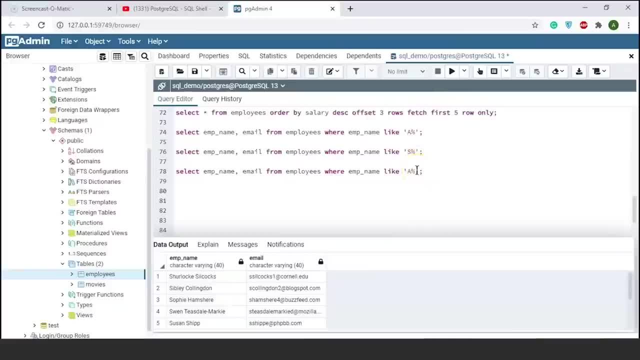 employees whose name ends with D. now the way to do it is, instead of a percentage, I'll write this time percentage D, which means at the beginning it can have any letter, but the last letter in the string or in the name should be ending with D. now let me copy and run this. so there are 13 employees in the table whose name 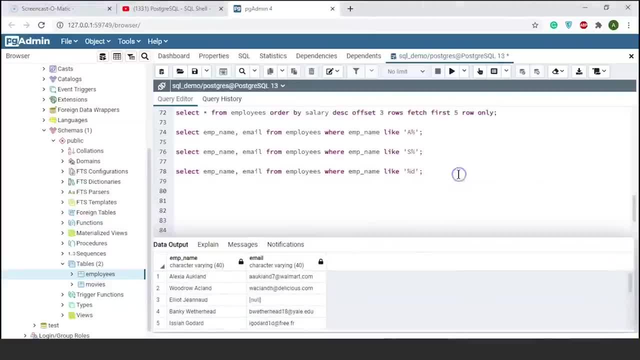 ends with a D. you can see it here. all right now. let's say, you want to find the employees whose name contains ISH, or have ISH in their names, so the way to do is something like this. so I'll copy this now here: instead of a percentage, I'll 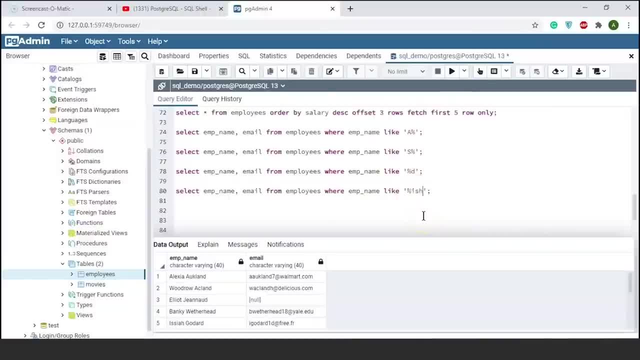 replace this with percentage: ISH percentage. now, this means that in the beginning it can have any letter and towards the end also it can have any letter, but this ISH should appear within the name. let me run and show it to you. okay, so there is one employee whose name contains ISH. you can. 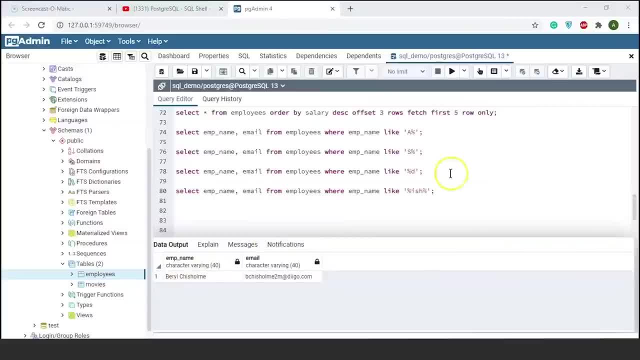 see here there's an ISH in the last name of the employee, on the top and at the bottom where it says ISH, and the other where it says N, and so the final name is limitation. all right now, suppose you want to find the employee name which has u as the second letter. 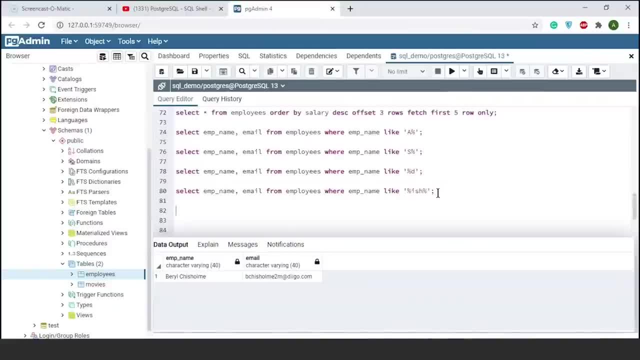 it can have any letter in the beginning, but the second letter of the employee name should have u. now the way to do is i'll copy this and instead of a percent i'll write underscore u followed by percent. now this underscore, you can think of a blank that can take any one letter. 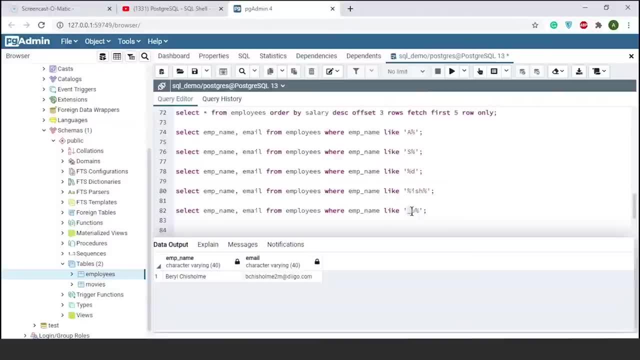 so the beginning can start with a, b, c, d or any of the 26 alphabets we have then then it should contain u as the second letter, followed by any other letter or letters. let me run this okay, so there are 10 employees in the table whose name has a- u. 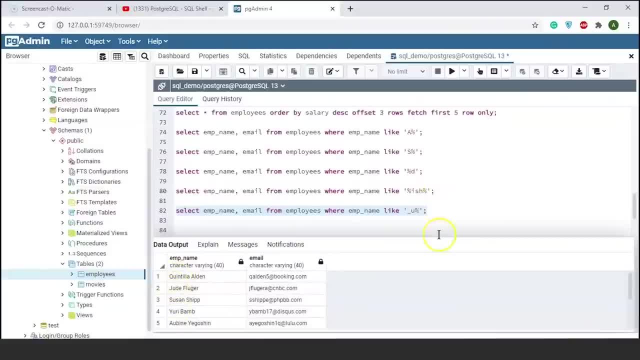 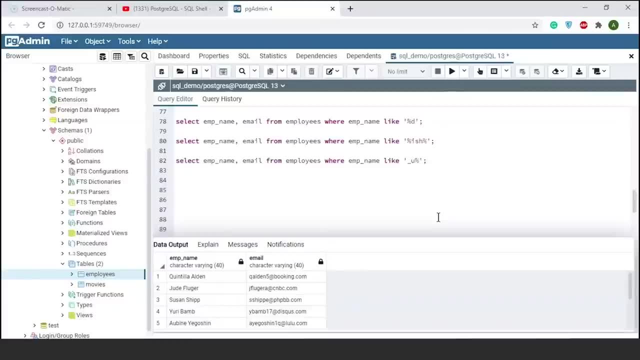 as the second letter, you can see these. okay, now, moving ahead, let me show you how you can use basic sql functions or inbuilt functions. so we'll explore a few mathematical functions now. so let's say you want to find the total sum of salary for all the employees. 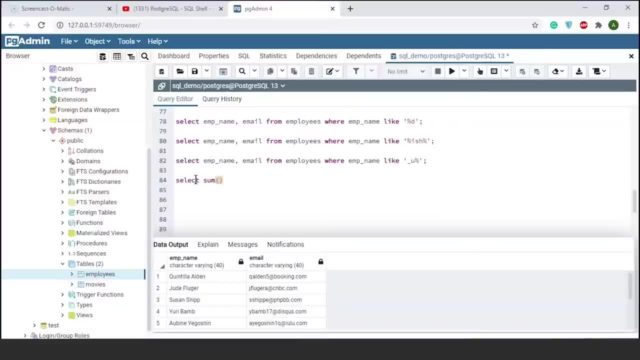 so for that you can use the sum function that is available in sql. so i'll write sum and inside the sum function i'll give my column name- that is salary- from my table name- that is employees. let's see the result. this will return one unique value. 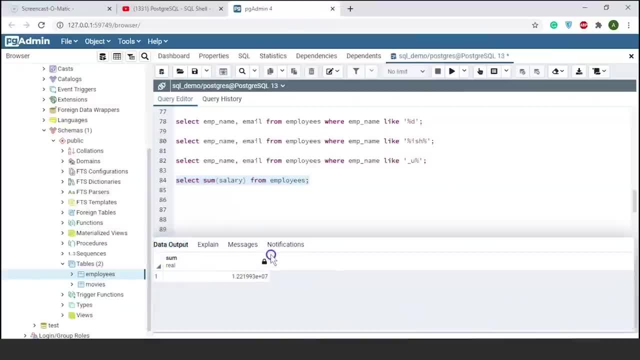 there you go now. this is the total salary. since the value is very large, it has given in terms of e. now one thing to note here is if you see the output, the column says some real. so this output column is not really readable. so sql has a method which can fix this that is called 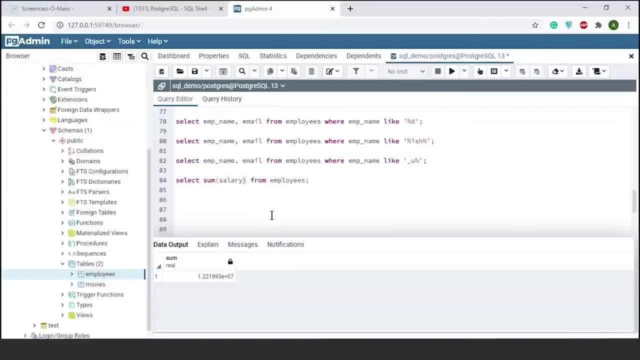 an alias. so since we are doing an operation of summing the salary column, we can give an alias to this operation by using the as keyword. so if i write sum of salary as, let's say, total salary, Then this becomes my output column. you can see the difference if I run this. okay, you can see now. 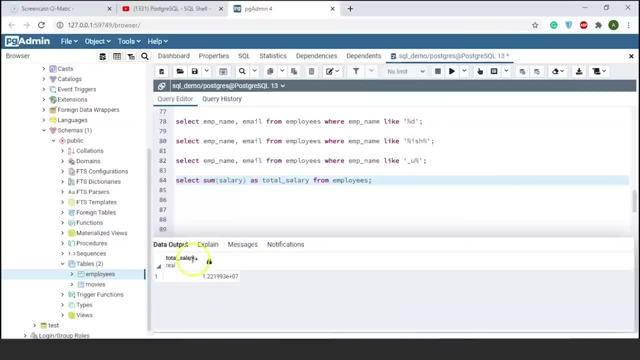 in the output we have the total salary. now this is much more readable than the previous one. so this is a feature in Excel where you can use or give alias names to your columns or your results. now, similarly, let's say you want to find the average of salary for all the employees. now SQL has a function called 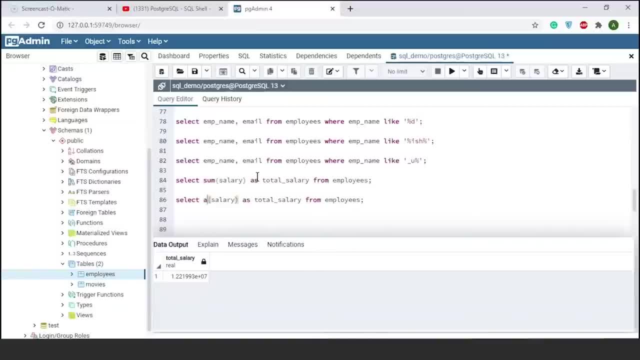 AVG, which calculates the mean or the average salary. if I write AVG- and I can edit my alias name as well, let's see I'll write mean salary. let's run it. you can see the average salary for all the employees. it's around $81,000. okay now. 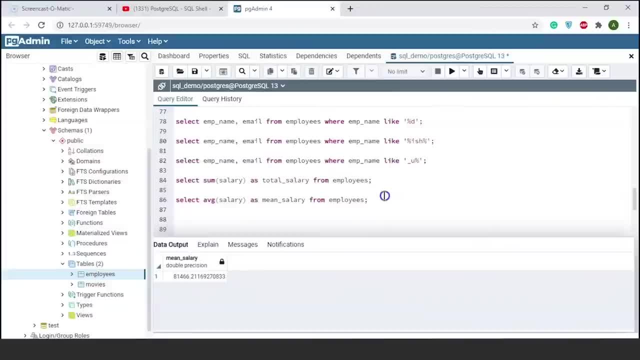 there are two more important functions that SQL provides us, which is max and minimum. so if I write select maximum or max, which is the function name of salary, as, let's say, instead of total I will write maximum. so this will return me the maximum salary of the employee. let's run it and see what is the maximum salary. 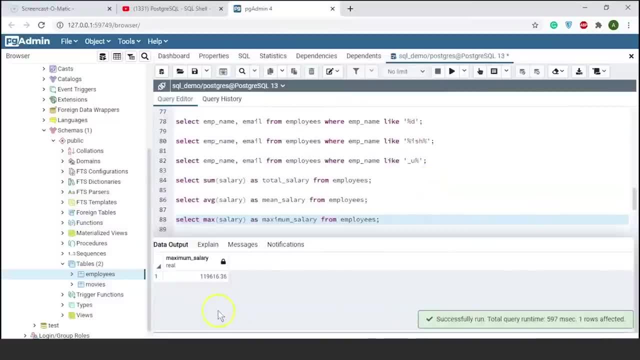 that is present in the salary column. all right, so we have $119,760. so this is the maximum salary of the employee. and now in the next column, let's: this is the maximum salary of the employee. and now in the next column, let's: six hundred and sixteen dollars as highest salary of one of the employees. 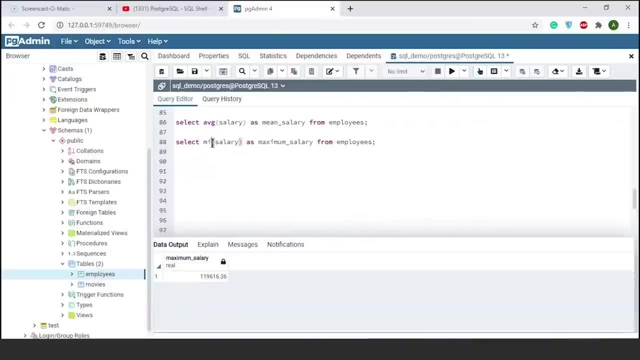 similarly, you can use the min function as well. I'll just write minimum and this will return me the minimum salary of one of the employees in the table. I'll replace the is alias name as minimum. okay, now run it. this will give me the minimum salary that is present in our table. so it is forty five thousand six. 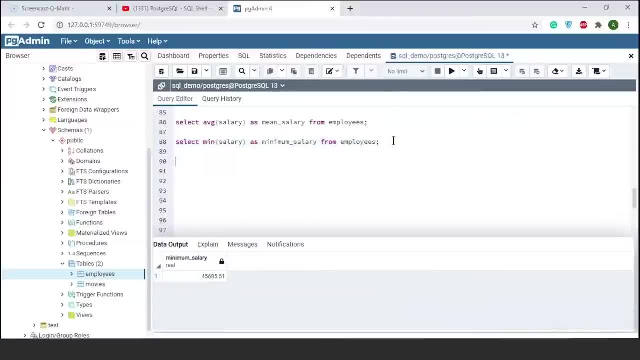 hundred and eighty five dollars. okay, now let's say you want to find the count of department in the employees table, you can use the count function. so if I write select count- let's say I want to know the distinct department names- I can write inside the count function. 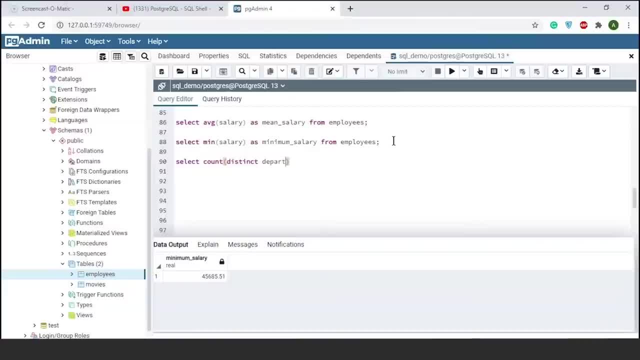 function: distinct department as total departments from employees. let's run this. this will return me the total number of departments that are there. so it gives me there are twelve departments. okay, you can write like that. okay, now, if you run the count function: active statement: ACど 1, dis church project, these two functions as the line of action. 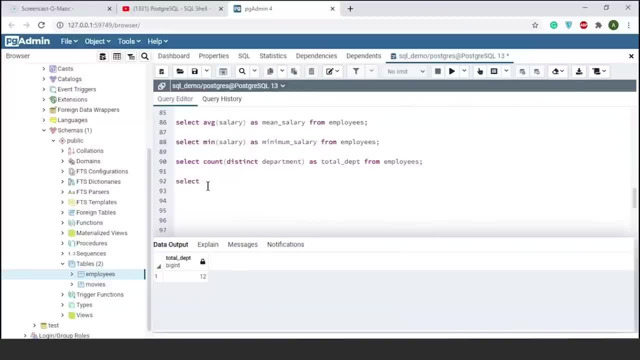 now let me show you one more thing here. if i write select department from employees, let's run this okay. so it has returned me 150 rows of information, but what i'm going to do is i'll place my distinct keyword here just before the column name, so that i can verify how many departments 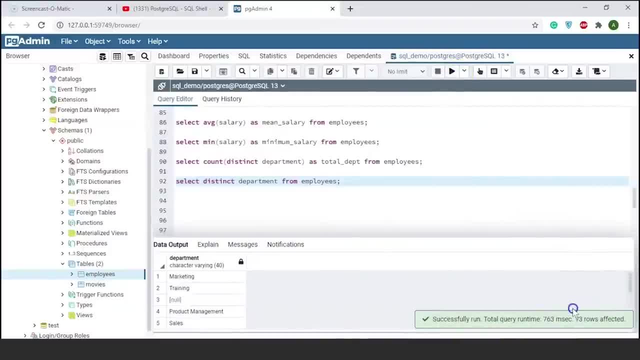 are there in total. there you go. so there are 13 departments and one of them is null. so, moving ahead, we'll replace this null with a department name by updating our table. okay, so now let's update our department column. so what we are going to do is: wherever. 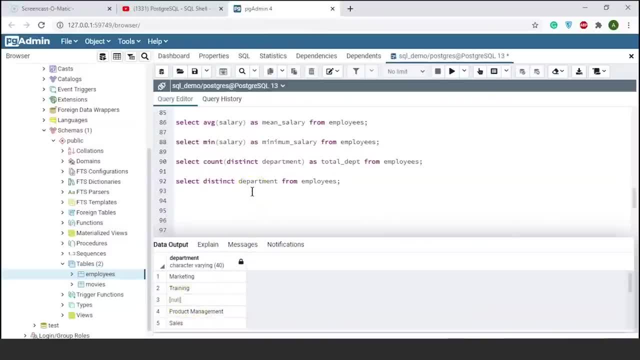 department has a null value. we are going to assign a new department called analytics. so earlier we have also learned how to use the update command, so i'm going to show it again. so we'll write update, followed by the table name, that is, employees. i'm going to set my column, that is. 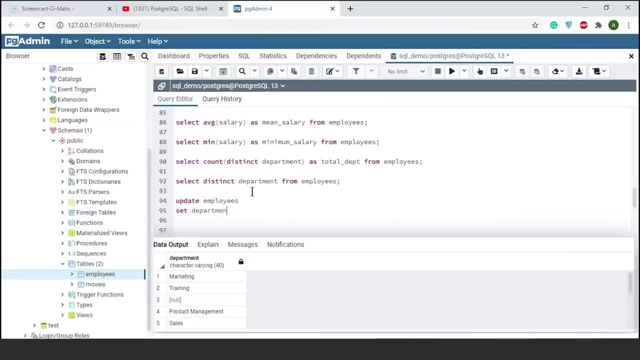 department equal to within single quotes, my name of the department would be analytics. where department is, i'll say null. so wherever the department has a null value, we'll replace those information with department. that is, analytics. let's run this. you can see query returned successfully. now let's say: 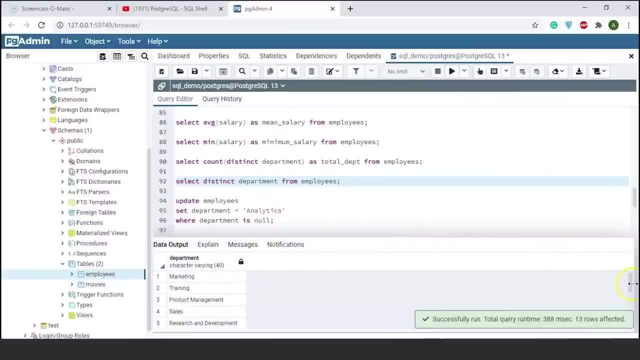 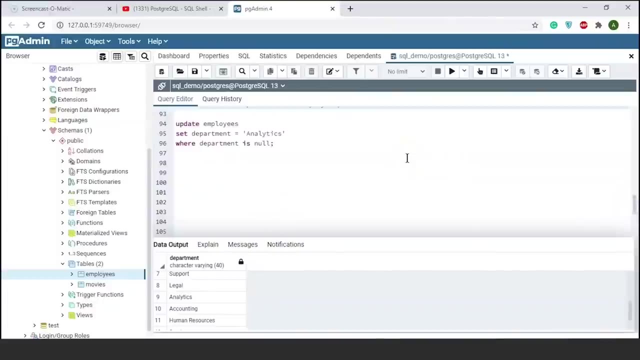 i'll run this command again and this time you can see the difference. there you go. so we have 13 rows of information and there is no null department. now we have added a new department, that is analytics. okay, now we are going to explore two more crucial commands or clauses in sql, that is: 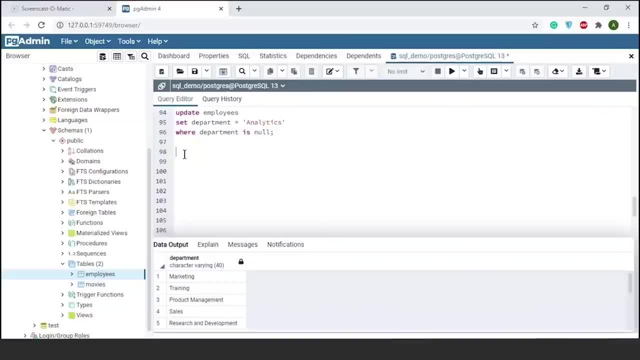 group by and having. so let's learn how group by clause works in postgresql. so the group by clause is used in collaboration with the sql statement, groups rows that have the same values into summary rows. for example, you can find the average salary of employees in each country, or 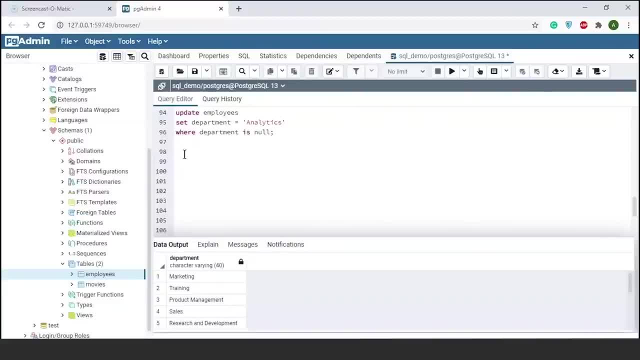 city or department. so the group by clause is used in collaboration with the select statement to arrange identical data into groups. so suppose you want to find the average salary of the employees based on countries. you can use the group by clause. so let me show you how to do it. 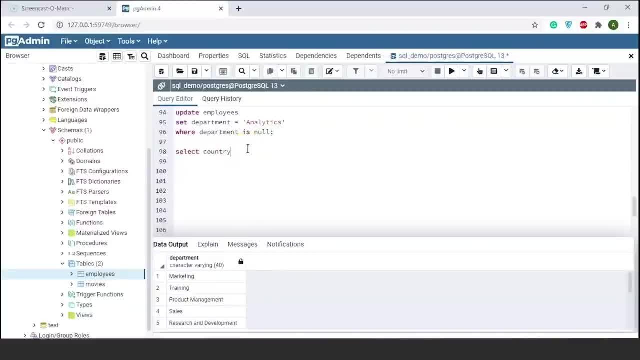 i'll write select. i want the countries and the average salary for each country, so i'll use the average function, that is evg, and inside the function i'll pass my column, that is salary. i'll give an alias name as, let's say, average underscore salary, from my table name, that is employees. 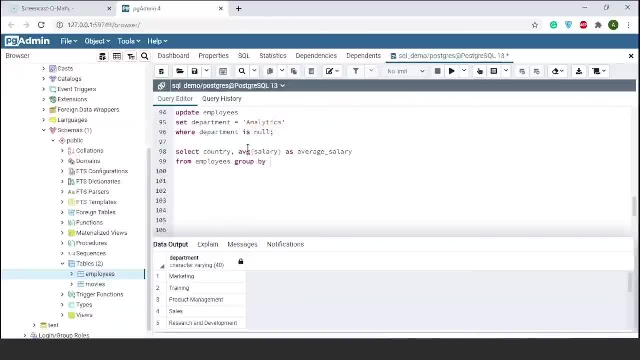 next, i'm going to use my group by clause, so i'll write group by, since i want to find the average salary for each country, so i'll write group by country name. let's give a semicolon and let me run it. i'll use f5. there you go. so here on the left you can see the country names we have: israel, russia. 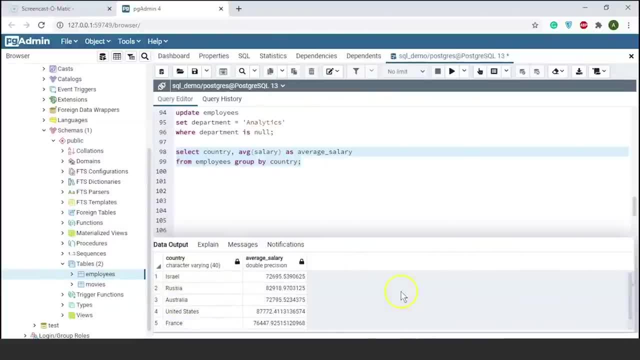 australia, united states, france and germany, and on the right, the second column, you can see the average salary for each of these countries. now you can also order the result in whichever way you want. suppose you want to arrange the results based on the average salary, so you can use the order. 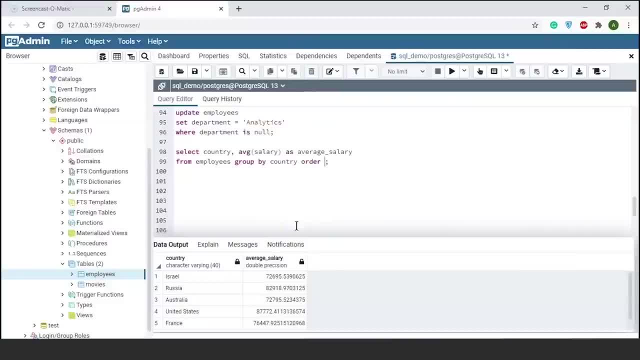 by clause, after the group by clause, so i'll write order by here. you can use the alias name. that is average salary. this is actually average underscore salary and let's say i want to arrange it in descending order, so i'll write desc. now let's run this. you can mark the difference in the average. 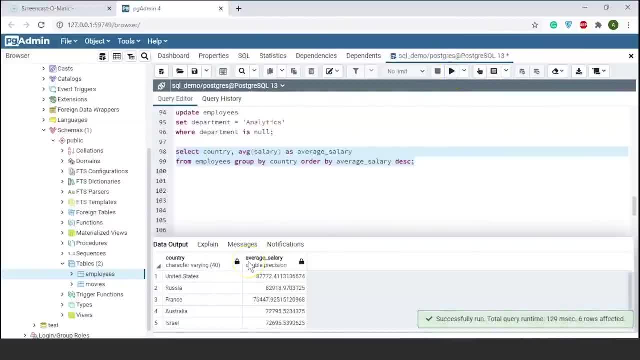 salary column. there you go. so, as per our result, in united states the average salary is the highest and if i scroll down, the average salary is the lowest in germany. now let's see one more example, using group by suppose this time you want to find the maximum salary of male and female employees. 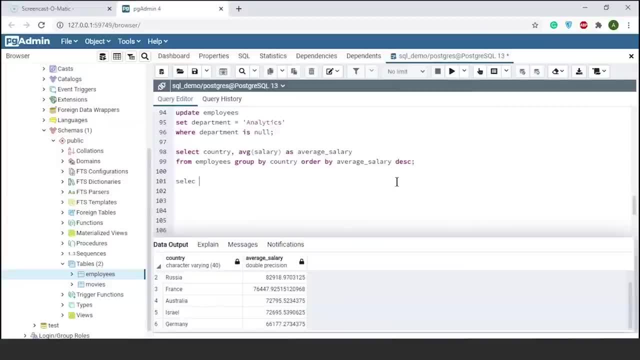 you can do that too, so let me show you how to do it. so i'll write select. this time we want to find the maximum salary based on gender, so i'll select my gender column comma, and this time i'll use my max function, since i want to find the maximum salary for male and. 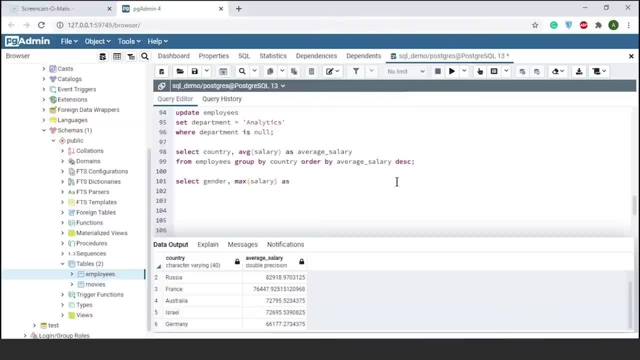 female employees. i'll give an alias name as maximum underscore salary from my table, that is employees group, by i'll write gender. okay, so let's run this. there you go, you can see. so one of the female employees had a highest salary of one lakh nineteen thousand six hundred and sixteen dollars. 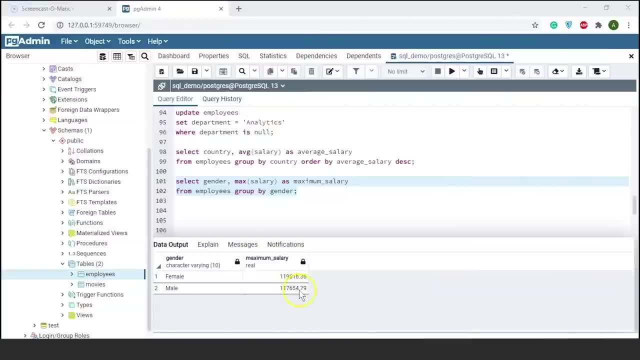 while of that of a male was one lakh seventeen thousand six hundred and fifty four dollars. all right, now suppose you want to find the number of employees based on each country. you can use the count function along with the group by clause, so i'll write the select statement- select, since i want to count the employees based on each. 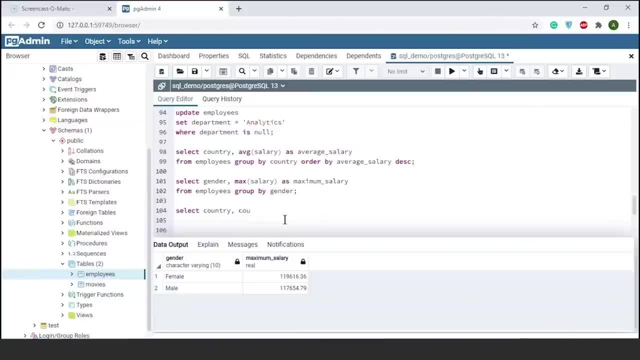 country. so i'll first select my country column and then i'm going to use the count function. i'll write count emp underscore id from my table name, that is, employees. i'm going to group by it, by country, so this query will give me the total number of employees from each. 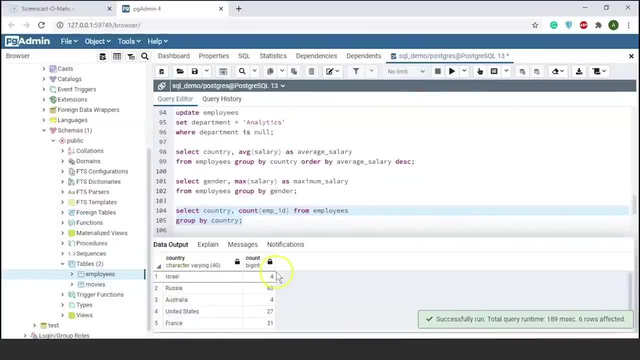 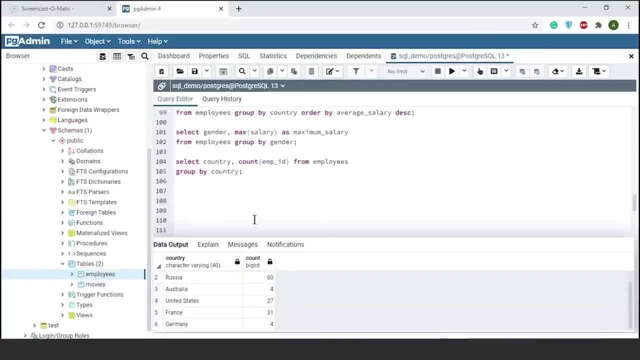 country you can see here, Israel. there are four employees. in Australia, there are four employees. in Russia, we have 80 employees. in France, there were 31. in United States, we have 27, so on and so forth. let me scroll down. okay, now it's time to explore one more clause, a very important. 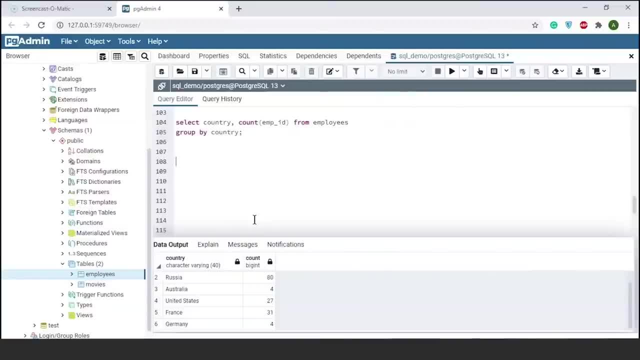 clause that is used in PostgreSQL, that is having. so the having clause works like the where clause. the difference is that where clause cannot be used with aggregate functions, the having clause is used with the group by clause to return those rows that meet a condition. so suppose you want to find the countries. 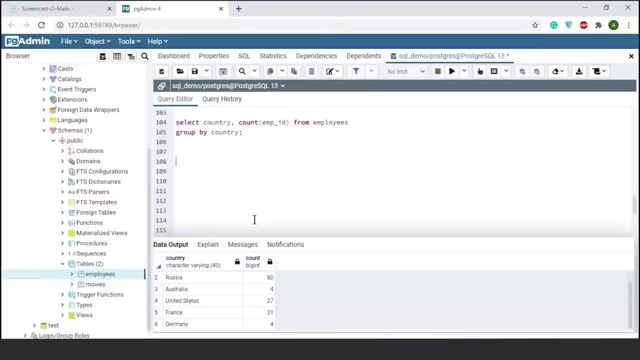 in which the average salary is greater than $80,000. so you can use the groupby clause and the having clause to get the result. so I'll write my select statement as select country comma. I want the average salary, so I'll write AVG of salary. I can give an alias name as average salary. 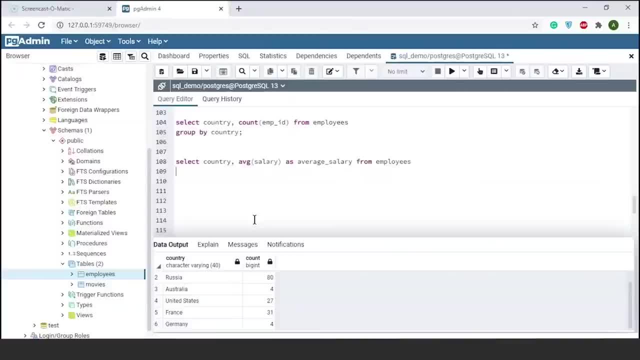 from employees. now I am going to group it by each country, so group by country column, since I want to find the countries in which the average salary is greater than 80,000, so I'll use having clause. after the group by clause I'll write having average of salary is greater than 80,000. 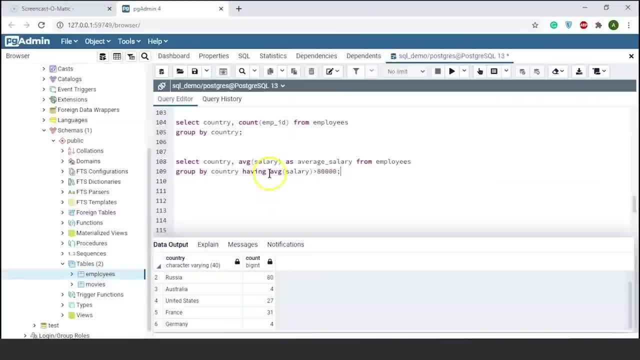 now, this condition cannot be specified in the where clause, so we need a having clause. you cannot use aggregate functions along with where clause. let me just run it now. there you go. so we have Russia and United States, where the average salary is greater than $80,000. all right, 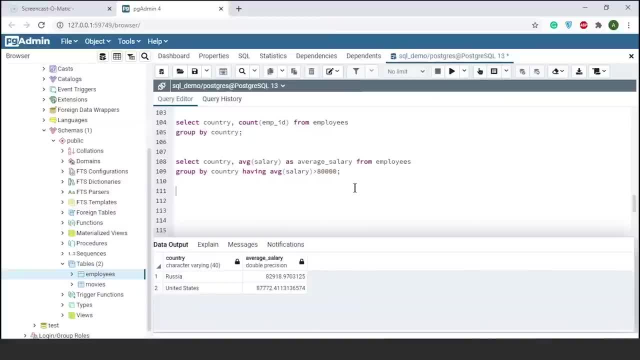 now let's say you want to find the count of employees in each country where there are less than 30 employees. so for this I am going to use the count function. first let me select the country column, then I'm going to use the count function and in the 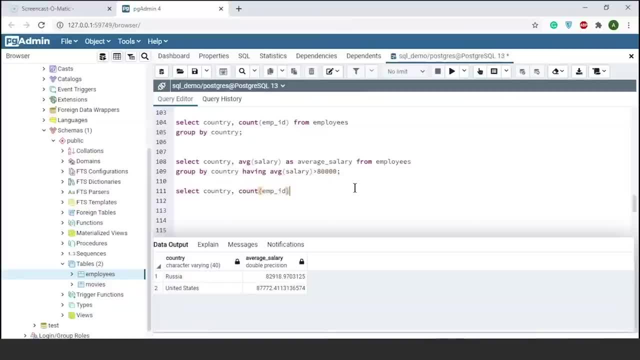 count function. I am going to pass my employee ID so that we can count the number of employees from my table, that is employees. now, if you want, you can use an alias name for this as well, but I am just skipping it for the time being and I'll write group by country. next I'll write having count of employee ID less. 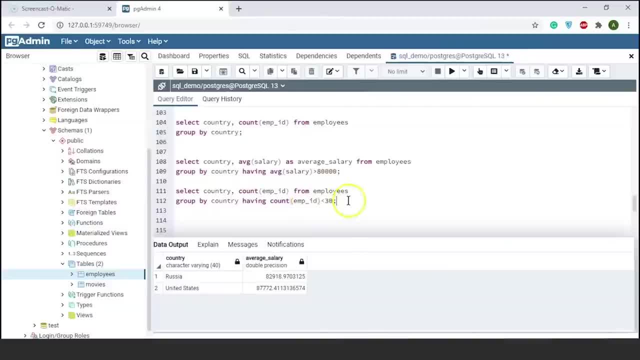 than 30. so this will return me the countries in which there are less than 30 employees. let's run it. you can see here: Israel, Australia, United States and Germany are the countries in which there are less than 30 employees. okay, and if I want to find the total number of employers in each country, then I will just 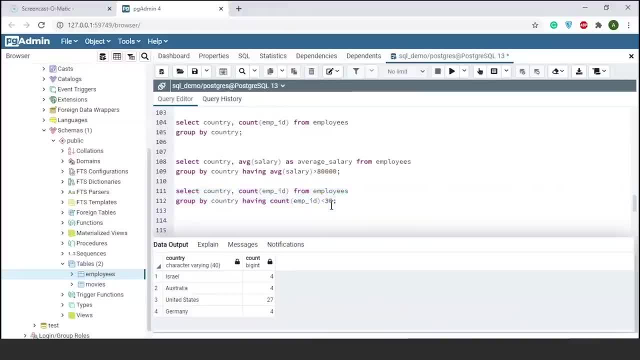 name it as come to the never, I will write by the number of employees in each country, so this will return me the countries in which there are less than 30 employees. Now, if you want, you can use the order by clause as well, So suppose I will write here. order by count of employee ID. So what this will do is it will arrange my result in ascending order of employee ID count. 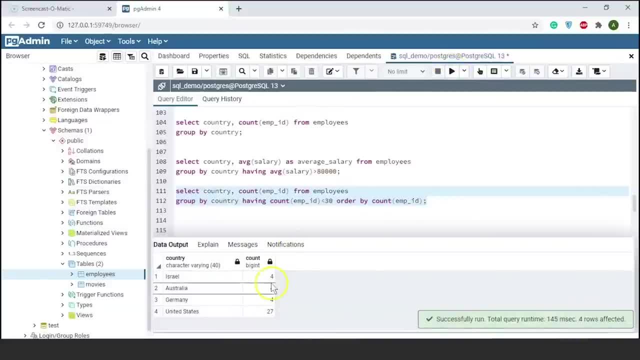 There you can see, we have successfully arranged our result in ascending order of employee IDs. Okay, Next we are going to explore one more feature of Postgres SQL, that is, of using a case statement. Now, in Postgres SQL, the case expression is same as if else statement in any other programming language. 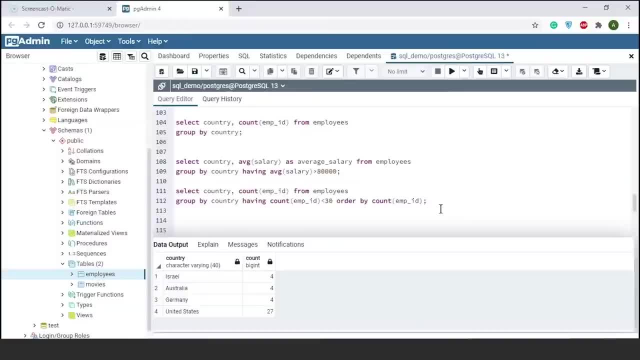 It allows you to add if else logic to the query to form a postgres SQL. Now let me just scroll down and I will show you how to use a case statement. This is very similar to your if else statement that you use on Excel, in C++, in Python and or any other programming language. 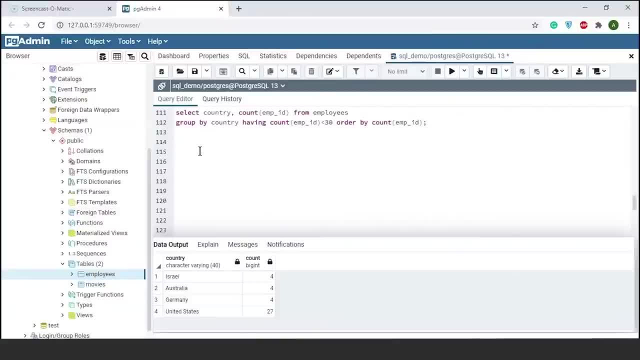 So what I am going to do is I am going to write a SQL query that will create a new column and the name of the column would be, let's say, salary range. So I am going to divide my salary, Suppose, if the salary is greater than 45,000. 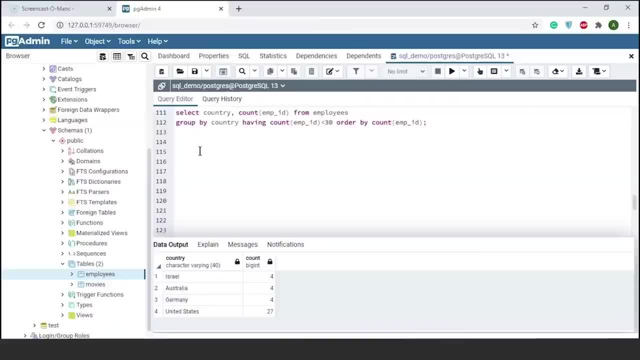 And if it's less than 55,000 dollars. in the new column- that is, salary range, we are going to assign a value: low salary. Now, if the salary is greater than 55,000 dollars and if it is less than 80,000 dollars, we are going to assign a value that is medium salary. 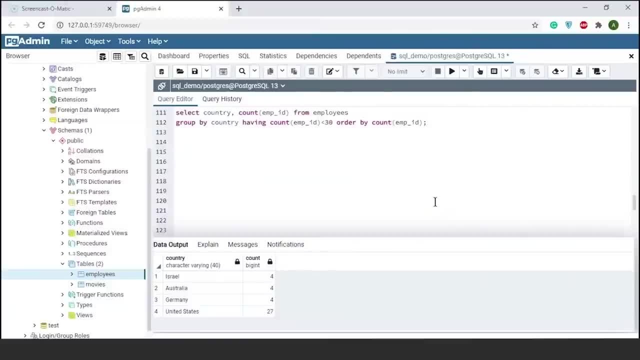 If the salary is greater than 80,000 dollars, we'll assign a value: high salary. So all this we are going to do using our case expression in Postgres SQL. So I'll start with my select statement, But before that let me show you how to write a comment in Postgres SQL. 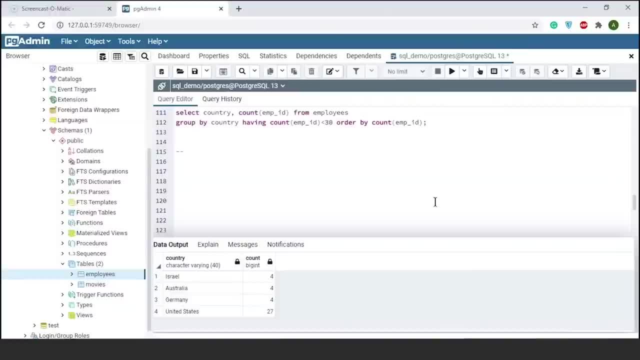 So you can write a comment by giving a double dash. Comments are very helpful because they make your codes or the scripts readable. I'll write case expression in Postgres SQL. Similarly, if you want, you can go to the top and. 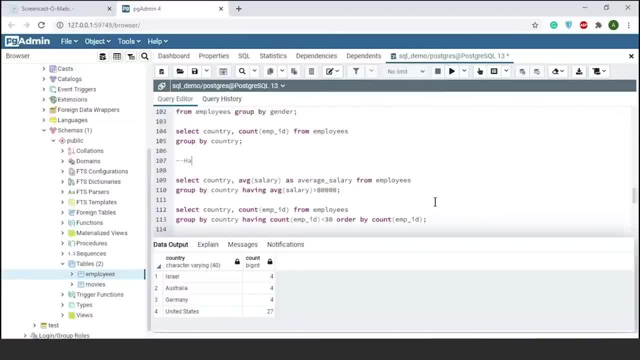 Let's say: here you can write with double dash having clause: Okay, Let's come down. So I'll write my select statement. as select I want, the department, the country and the salary column. I'll give a comma. 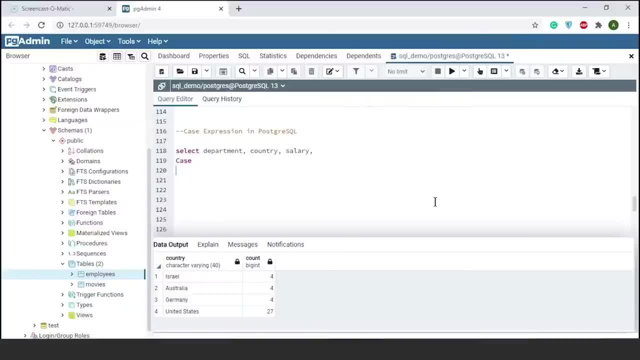 And I'll start with my Case statement. I'll write case when my salary is greater than 45,000. And my salary is less than 55,000. Then the result would be within single quotes. I'll write low salary. 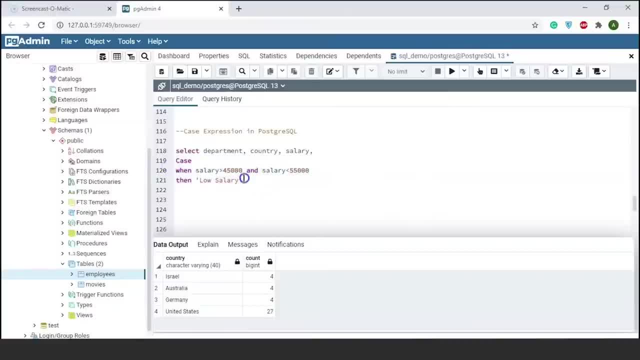 So this is exactly like an if-else condition. Next, I'll write another case when salary is greater than 55,000. And salary is less than, let's say, 80,000. Then the result would be medium salary. 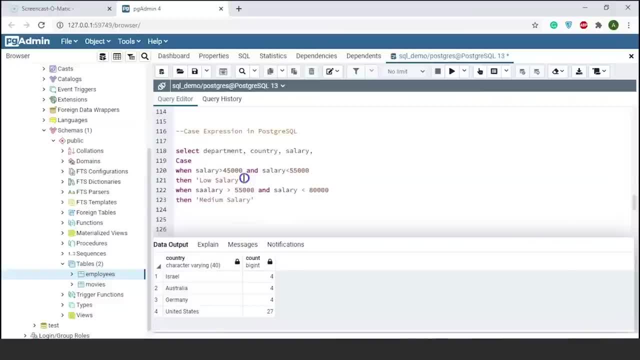 And finally, I'll give my last condition, That is, when salary is greater than 80,000,, then the result will be high salary. Let me write this in a single line: Then high salary. Now one thing to remember: in Postgres SQL, the quotes are insensitive. 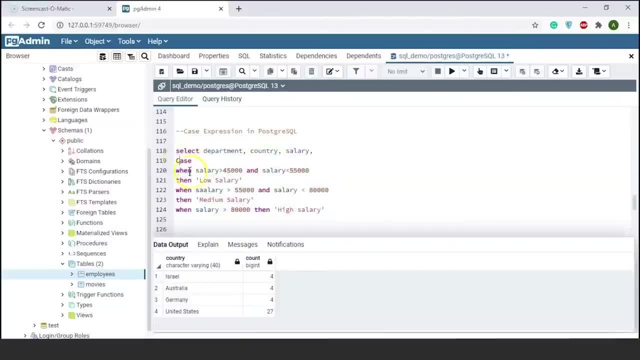 So you can write your select statement in capital, in lowercase or in sentence case. Similarly, I can. You can write case as small c, or you can write as capital C. All right Now, moving ahead. After this, I'm going to write end. 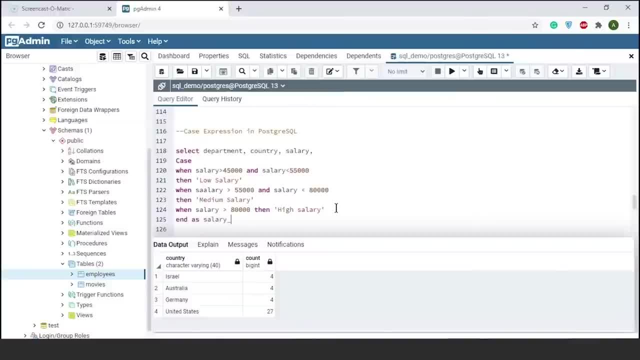 I'll give an alias name as salary range. Now this is going to be my new column in the output. Let me just come down And After this we need to To give our table name from employees. I'll order it by salary descending okay. 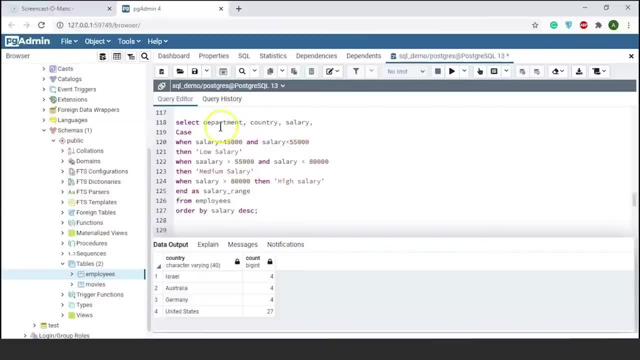 So what I'm going to do here is I'll first select department, country and salary column from my employees table And then I'm creating a new column, that is salary range, And I'm specifying the range. So I have three conditions here. 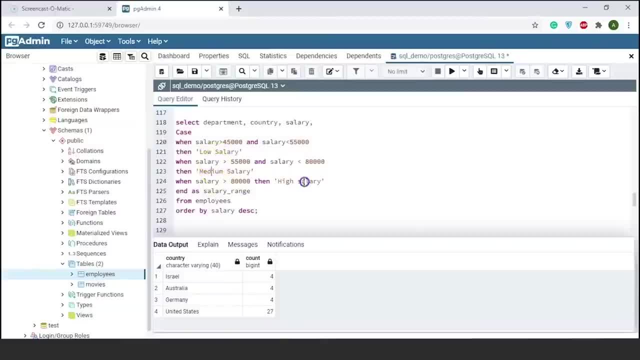 First, low salary for medium salary and high salary. So let's run this and see the output. There you go. Here you can see we have added a new column known as salary range And we have order our salary in descending order. 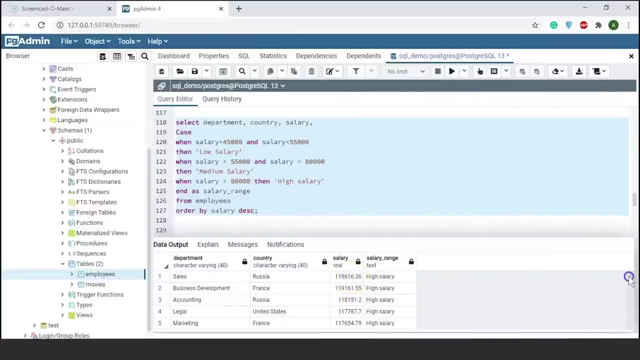 So all the highest salaries appear at the top. If I just scroll down you can see we have medium salaries here, And if I scroll down further you can see these low salaries. So I'm going to add a new column here. 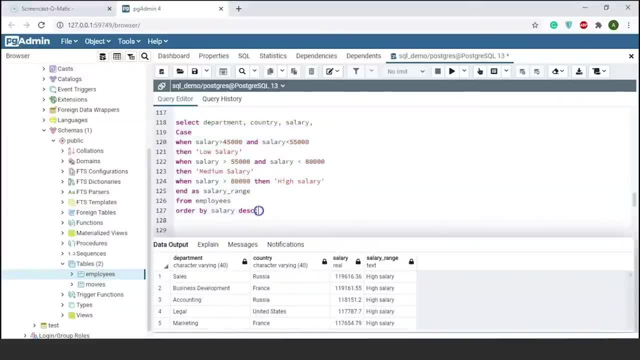 And then under specialist, I'm going to apply subscribers. If I click on no season, our salary will be counted to that number only So I can select how much salary I want. After that I can run the baselines. 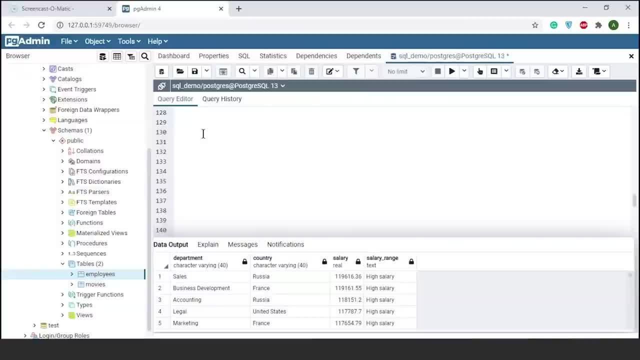 I'll enter my salary hashtags. Take care of yourself and try to explain some basic, fundamentally useful requirements. Let's go back, Sir. do you have any good tomorrow? No salary is greater than the average salary, so in such cases you can use sub queries. now let me. 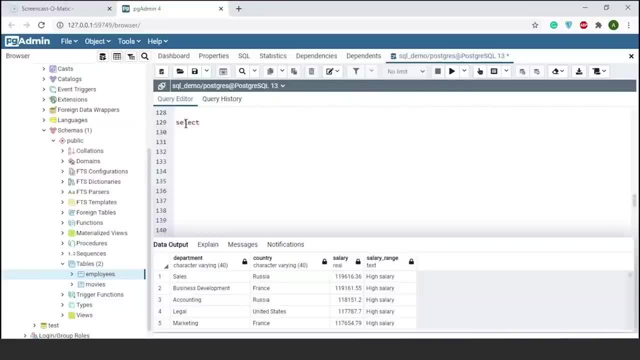 show you how to write a query inside another query. first i'll write the select statement. i am going to select the employee name comma. i want the department comma also want to display the country name and the salary from the employees table where my salary should be greater than the average salary. so after this, where salary greater than i, 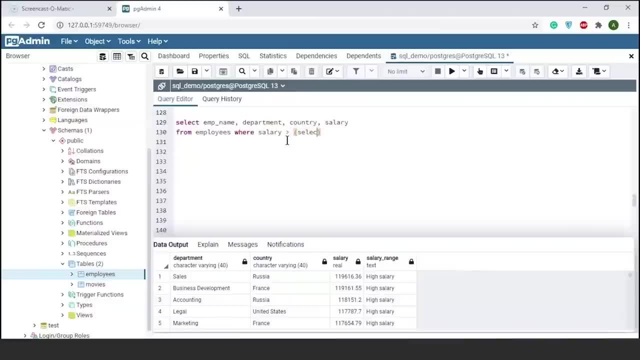 am going to use brackets and write my sub query, that is, select average salary from employees. now let me break it down for you. so first we are going to select the average salary from the employees, so this particular sql statement will find the average salary from the table. 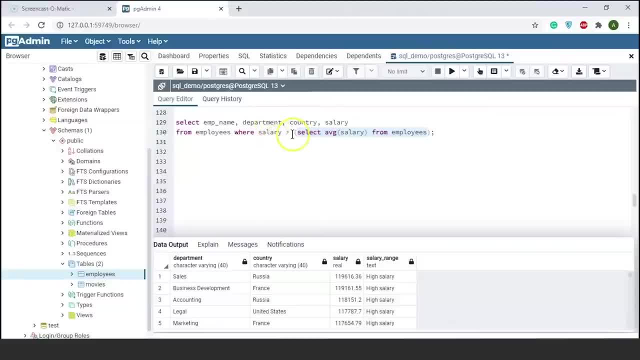 we will compare this average salary with salaries of all the employees. so whichever employee has the salary greater than the average salary will display their names, the department, country and their original salary. so if you want, you can run this statement as well, this statement, and run it for you. you can see we have written the average salary of all the 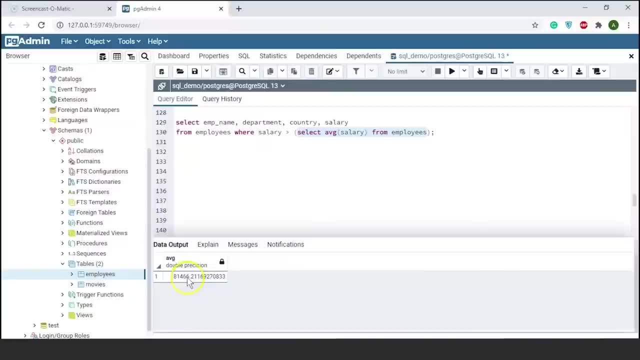 employees, which is nearly eighty one thousand four hundred and sixty six dollars. so we want the salaries of the employees to be greater than this average value. so let me run this and see how many employees have a salary greater than the average salary. there you go. so we have. 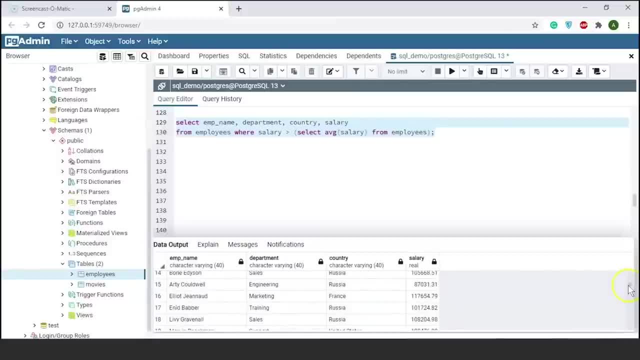 around seventy five employees whose average salary, or whose salary is greater than the average salary. all right, now, moving ahead, this time I'm going to tell you how to use some inbuilt functions. we learn some inbuilt mathematical functions and string functions that are available in postgresql, so I'll just give a comment. there's another way to write a comment. 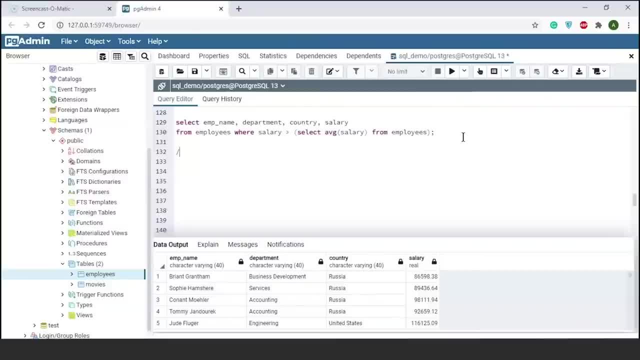 instead of a double dash you can use the forward slash and an asterix, and inside the asterix you can write, let's say, sql functions and you need to close this. so I'll give another asterix and a forward slash. so this is also a comment in postgresql. all right, so first of all we'll explore a few math functions. 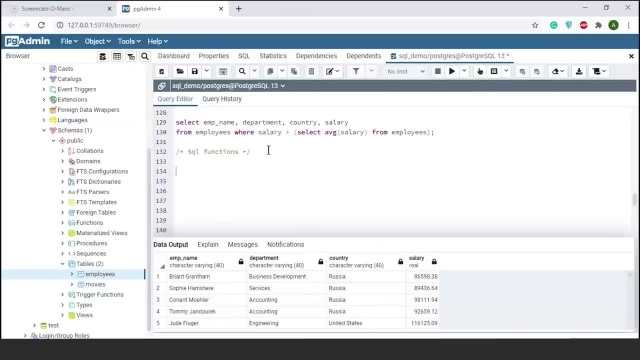 so there is a function called abs which is used to find the absolute of a value. so if I write select abs of, let's say, minus hundred, it is going to return me positive hundred or just hundred because, as you know, the absolute of any value will remove the negative sign involved in. 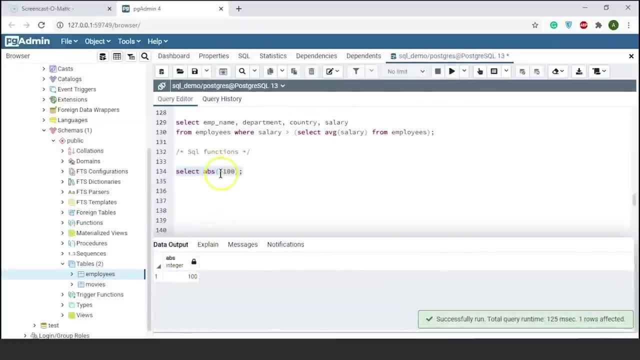 that value. there you go. so our original input was minus hundred. the absolute of minus hundred is plus hundred. next let's see another function that is called greatest. so the greatest function in postgresql will return the greatest number in a range of numbers. so suppose I write select greatest inside the greatest function. I'll pass in a few numbers. 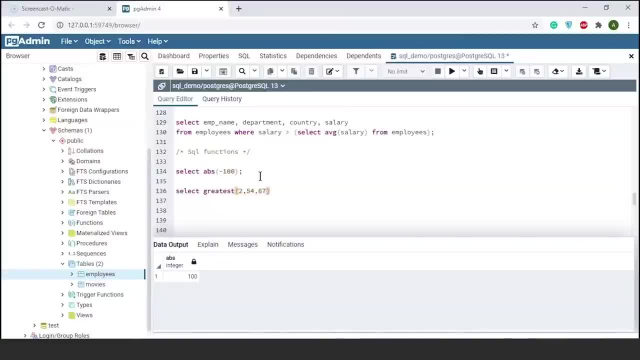 let's say two. I'm just randomly passing a few numbers. let's say 490, that's a 56.5, and let's say 70. I'll give a semicolon. let me run this. you will see. the greatest function will return the greatest integer value or greatest number that is present in the range of numbers. 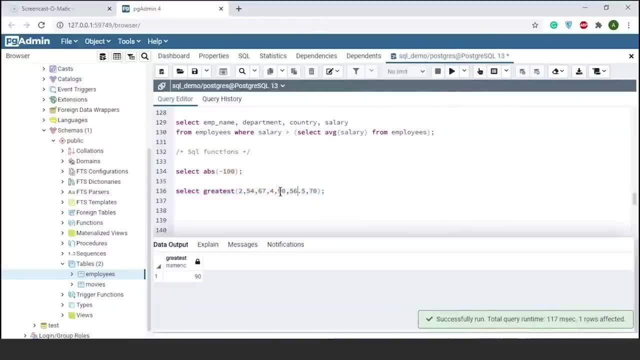 that we have provided so. in this case, 90 was the largest number or the greatest number, so we got the result as 90 again. you can use an alias for each of these statements. now, like greatest, we also have a function called least, which is going to return the greatest number in a range of numbers. 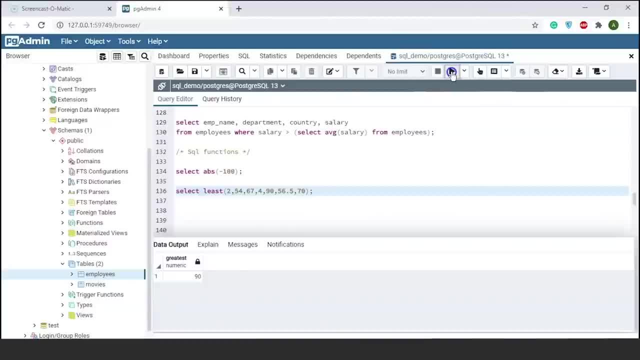 return the least number present in a range of numbers. we run this, so the result is 2, because 2 is the least number that is present in this selection. all right, now there's a function called mod which is going to return the remainder of a division. so suppose I write select mod and this takes two. 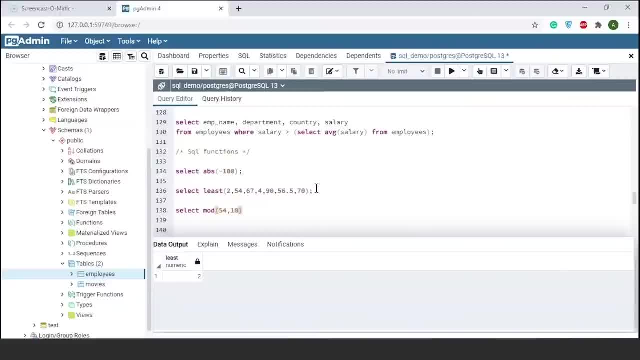 parameters. let's say 54 divided by 10, and this is going to return the remainder of a division. so, as you can guess, the remainder is 4 and so is our result. you can see it has written the remainder 54 divided by 10. the remainder is 4. all right, I scroll down. now let's see how to use the power. 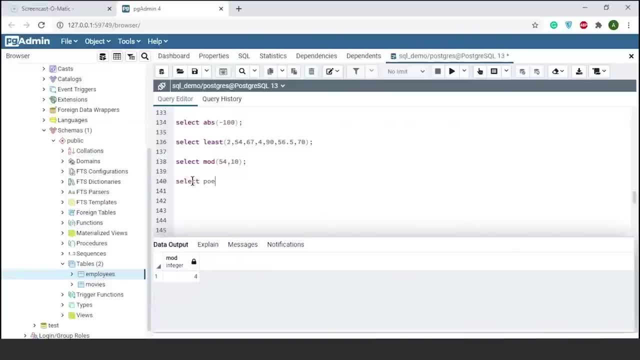 function. so I'll write select power. let's say: I want to know power 2 comma 3, which is 2 cube, that is 8. let me just run this. there you go. so the result is 8. you can also check, let's say, power of. 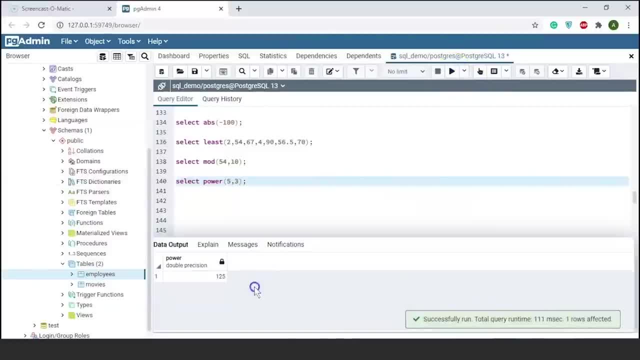 5, comma 3, it should be 125. all right. next you can use the sqrt function that is available in postgresql to find the square root of a number. I'll write sqrt and let's say I want to find the square root of 100. you can guess the result. the output should be 10. if I run this, you can see the output here: 10. 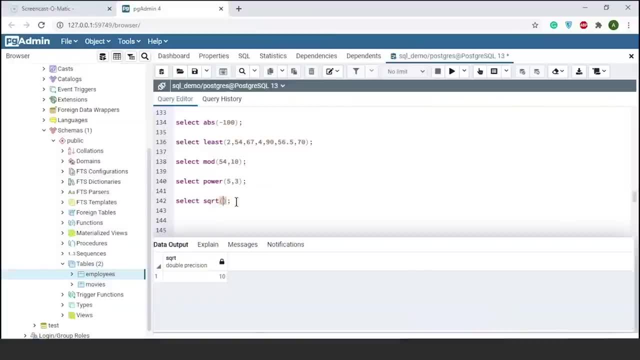 let's say I want to find the square root of, let's say, 144. you can again guess the result. it should be 12. let's verify it. okay, there is some error. let me verify it again. there you go, it is 12 now. there are a few trigonometric functions as well. you can use the sine function, the cos function and 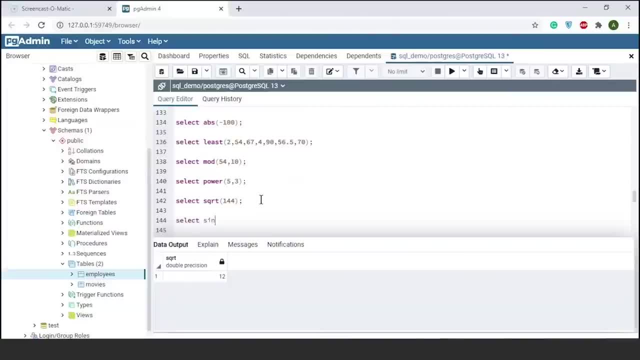 the tan function. let's say I want to know the sine of zero. if you have studied high school mathematics you would know the sine of zero is zero. you can see the result: it is zero. let's say you want to know sine 90. if I run it, you can see the output here: 0.89. all right, 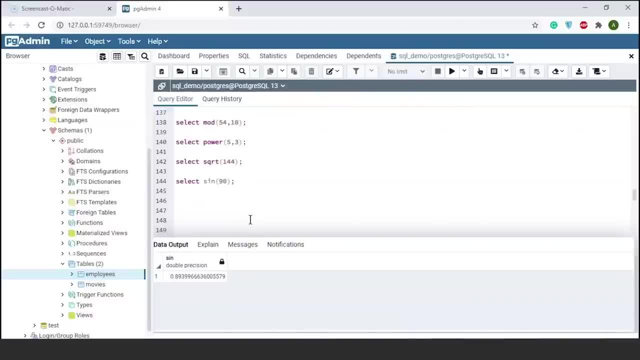 there are other functions like ceiling and floor that you can use. so let me show you what the ceiling and floor function does. I'll write ceiling, let's say I'll pass my floating value as 6.45 and let me run it. you can see the ceiling function returns the next highest integer, that is, seven, in. 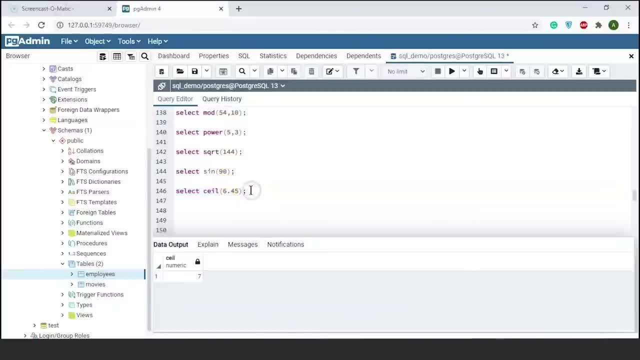 this case, since the next highest integer after 5 is seven. let's see what the floor function does and let me run it. as you can see, the floor function returns the next lowest integer, that is, six in this case, or the nearest lowest integer to any provided decimal value. okay, 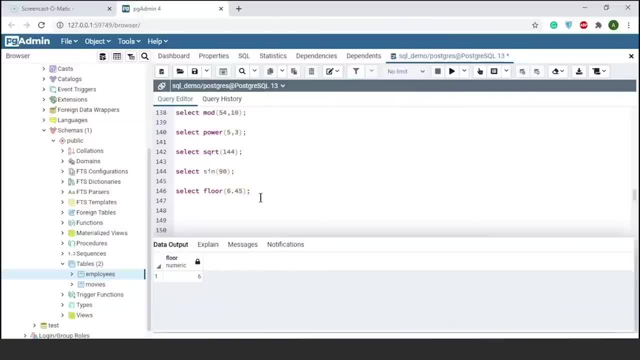 now that we saw how to use mathematical functions, there are a few string functions available in postgresql, so let's explore them as well. i'll write string functions. okay, scroll down. cool. there's a function called character length that gives you the length of a text string. suppose i write select, give the. 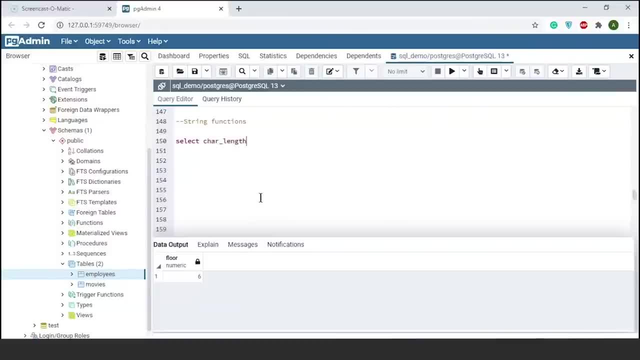 function as character length and inside this function, i am going to pass in a text. let's say: india is a democracy. this is my text. let me run this. okay, you can see the result here, which is 20, since there are 20 characters in my string. that i have provided. all right, now there's another. 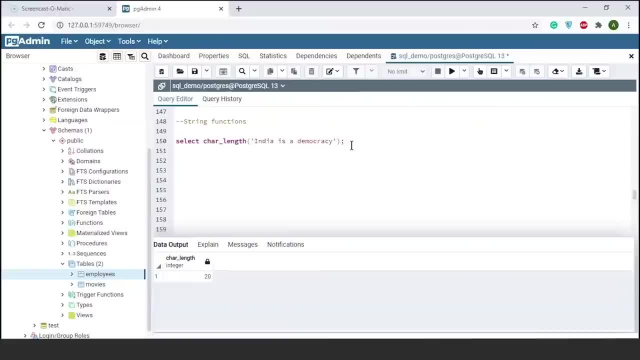 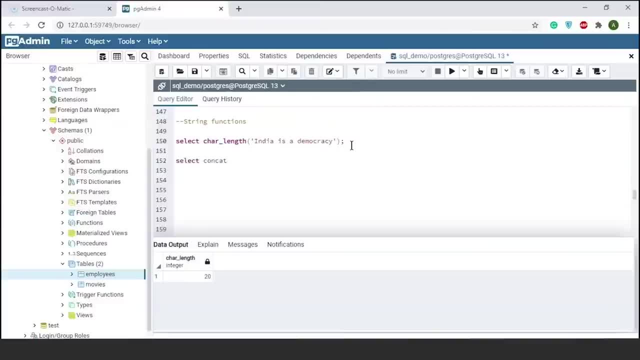 i have given it a name. so i have given it a name. so i have given it a name. so i'll write select concat. within brackets, i'll give the text string. now let's say i want to combine postgres sql. i'll give a space comma. i want to merge postgresql is. 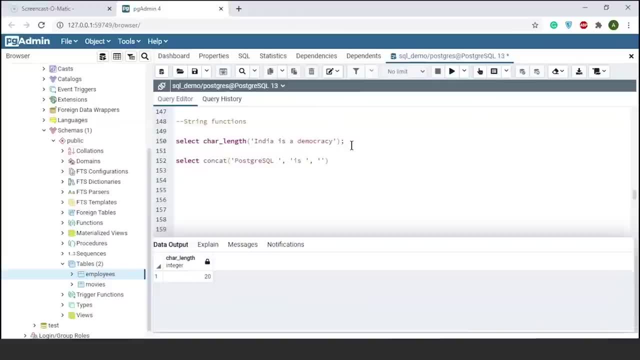 i'll give another comma and write my final word. that is interesting. now, what we have done is, inside the concat function, we have passed in separate strings and now, using the concat function, we want to merge the three strings. let's see what the result is. i'll run it all right. let me just expand this. you can see here that the result is: 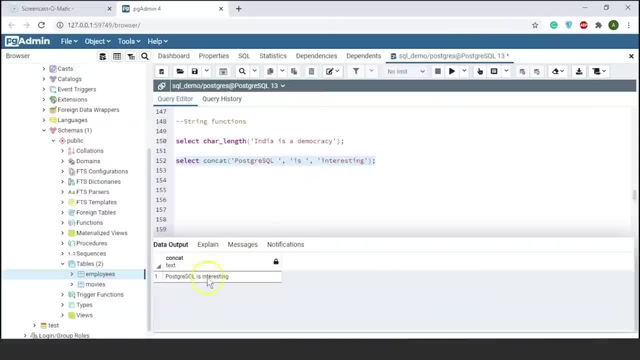 linear. we have concatenated the three strings successfully, so the output is postgresql is interesting. okay, now there are functions like left, right and mid in postgresql. so what the left function does is it will extract the number of characters that you specify from the left of a string. let's say i'll write select left. 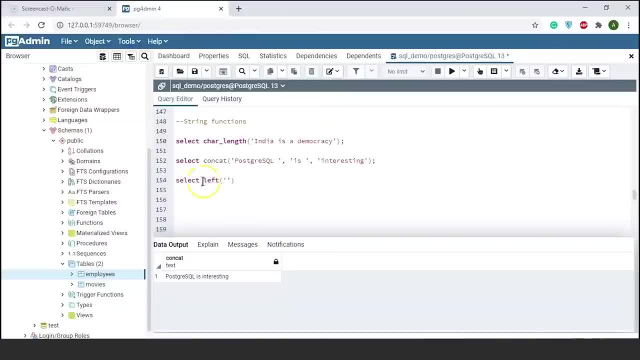 select left and i'll pass in my text string as india is demographic string democracy. I'll copy this and I'll paste it here. let's say I want to extract the first five characters from my string, so I'll give five. so what it will do is it? 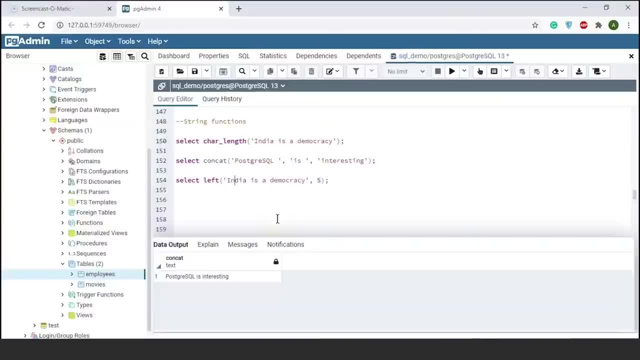 will count five characters from left, so one, two, three, four and five. if I run this, it should ideally print India for me. there you go, it has printed India for us, all right. similarly, you can use the right function to extract few characters from the right of a string. let's say you want to extract. let's say: 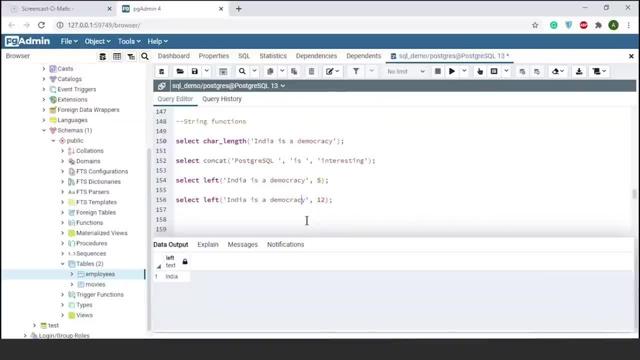 I'll give 12 characters from right, so from here onwards it will count 12 characters. I'll change left to right. now let me select this and run it so you can see here. this is the output from the right. it has counted 12 characters and. 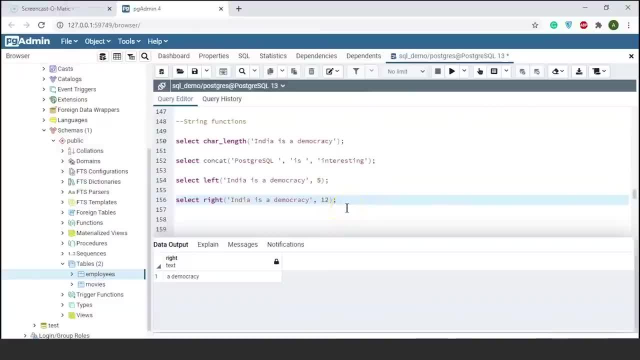 returned a democracy. okay, now there is a function called repeat, so the repeat function is going to repeat a particular string, the number of times you specify. let's say, I want to select and use my repeat function and inside the repeat function I am going to pass in, let's say, India, and I want India to be displayed. 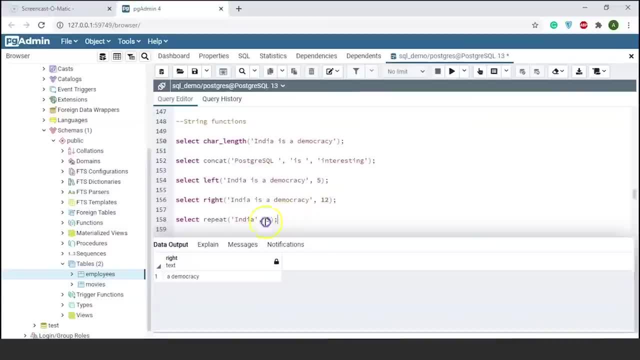 five times. I will give a semicolon and run it. in the output you can see India has been printed five times. okay, let's scroll down. there is another function, a string function in PostgreSQL, called as reverse. so what reverse function is going to do is it is going to print any string passed as an input in reverse order. so if I 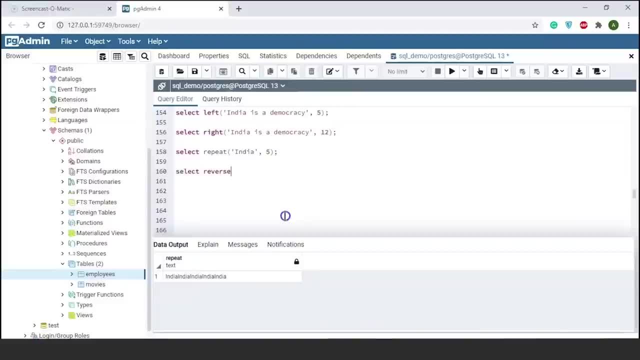 write, select, reverse, and inside the reverse function I'll pass in my string that is: India is a democracy. I'm going to use the same string. I'll copy this and I'll paste it here. close the course and the brackets. let's print this. you can see it here. 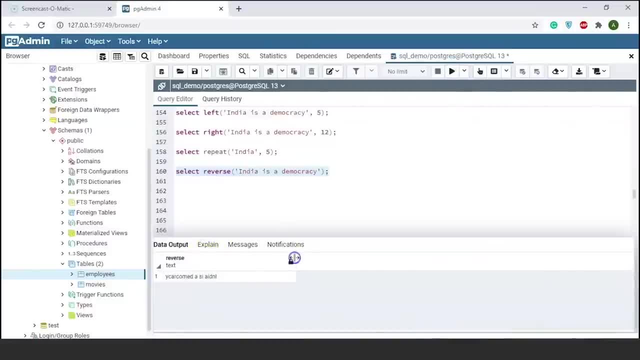 India is a democracy has been printed in reverse order. there you go all right now. this time we explored a few inbuilt functions that are already present in postgres sequel. now postgres sequel also has the feature where you can write your own user-defined functions. so now we will learn how to write a function of. 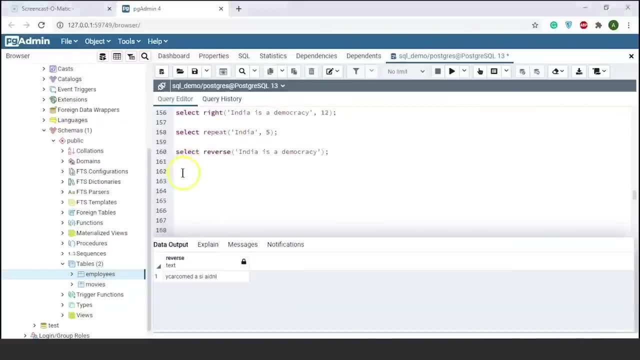 our own in postgres sequel. so let's create a function to count the total number of email IDs that are present in our employees table. so for this we'll write a function, a user-defined function. so let me give my comment as user-defined function. okay, so let me start by first writing: create so. 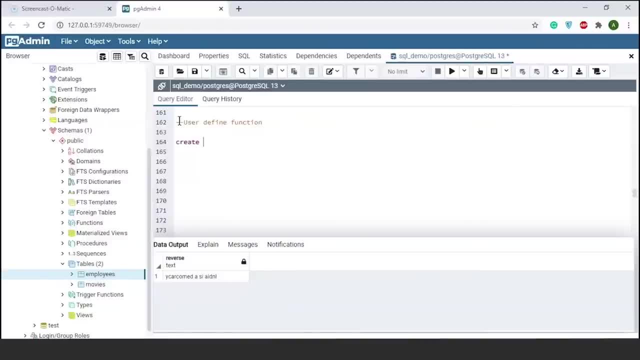 this is the syntax to write a function in postgres sequel. so I'll write create or replace function, then I'll give my function name as count emails and, as you know, functions have brackets. then I'll write returns, the return type as integer, then an alias with dollar symbol. I'll write total emails. since I'm going to 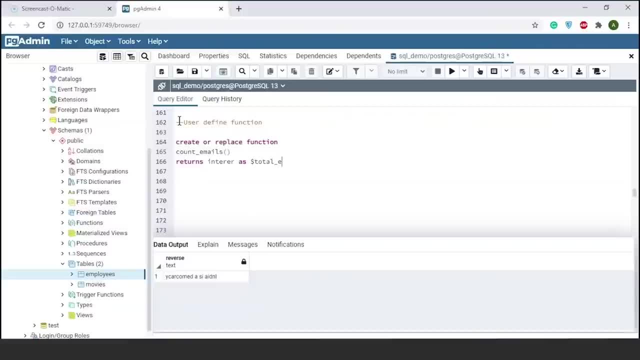 display the total number of email IDs that are present in my table, I'll close the dollar symbol. then I'm going to declare a variable. the variable name is going to be total, underscore emails. this is of type integer. I'll write begin and inside begin I'll write my select statement. so I'll write select. I want to count the email IDs that are present, so I'll pass my column name, that is email, into total emails from my table name that is employees, and inside begin I'll write my select statement, so I'll write select. I want to count the email IDs that are present, so I'll pass my column name, that is email, into total emails from my table name that is employees, and inside begin I'll write my select statement. so I'll write select. I want to count the email IDs that are present, so I'll pass my column name, that is email, into total emails from my table name that is employees, and inside begin I'll write my select statement. so I'll write select. I want to count the email IDs that are present, so I'll pass my column name, that is email, into total emails from my table name that is employees, and inside begin I'll write my select statement. so I'll write select. I want to count the email IDs that are present. so I'll pass my column name- that is email- into total emails from my table name, that is employees and inside. 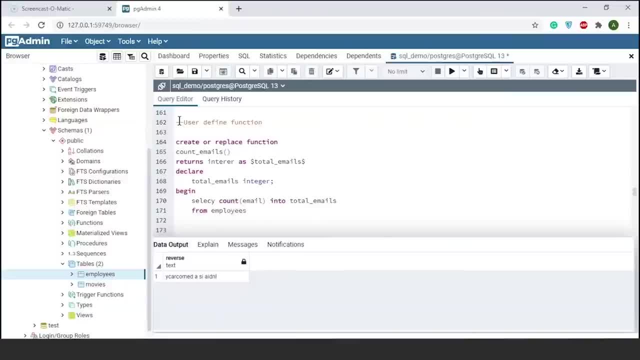 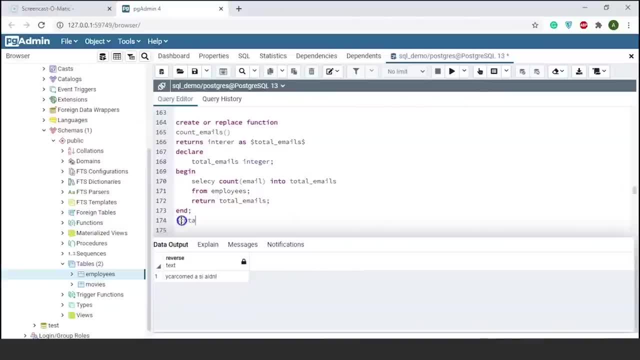 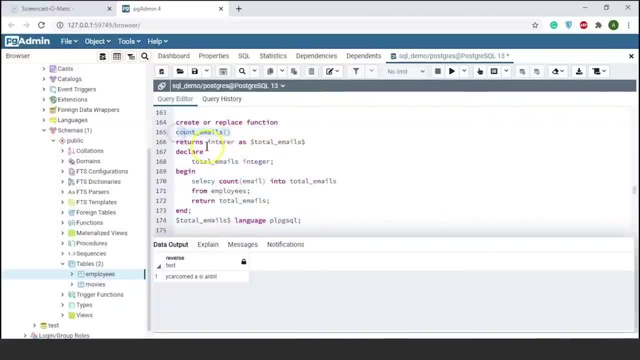 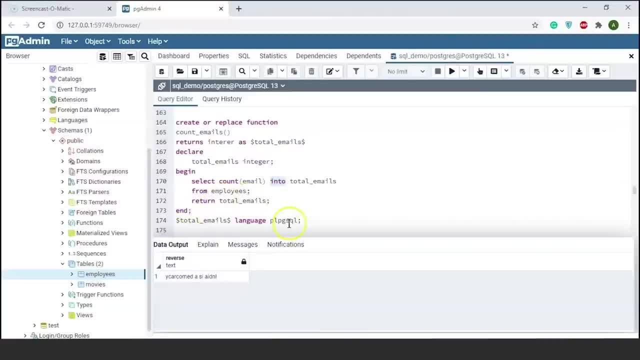 email IDs that are present. so I'll pass my column name that is employees, and inside begin I'll write select. I want to count the email IDs that are present. so I'll pass my column name that is employees, and inside begin I'll write select- I want to count the. 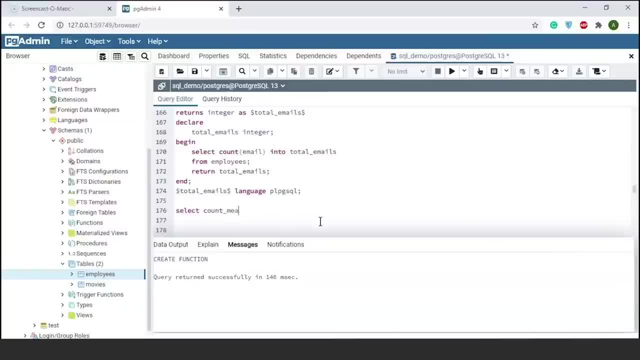 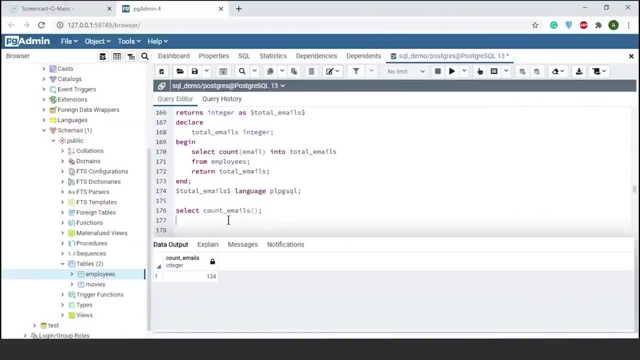 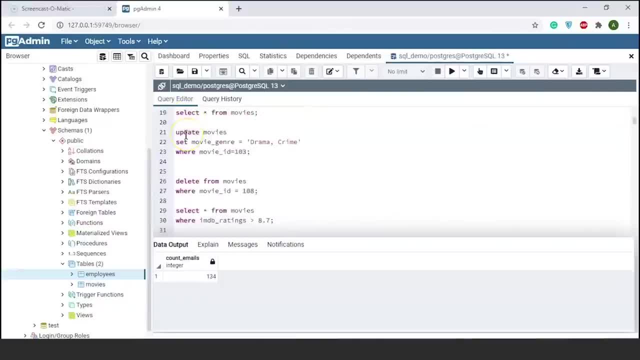 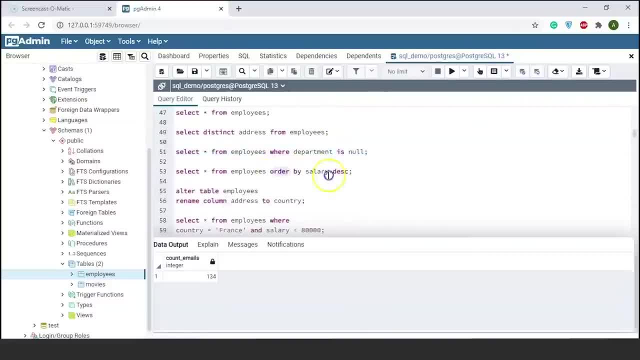 to use is null. with where clause, we learnt about the order by clause, we saw how to alter or rename a column. then we explored a few more examples on where clause, we learnt about and and or operator. then we learnt how to use limit and offset, as well as the fetch operator or the fetch. 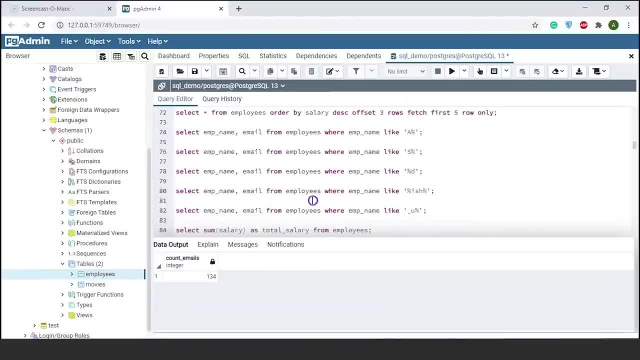 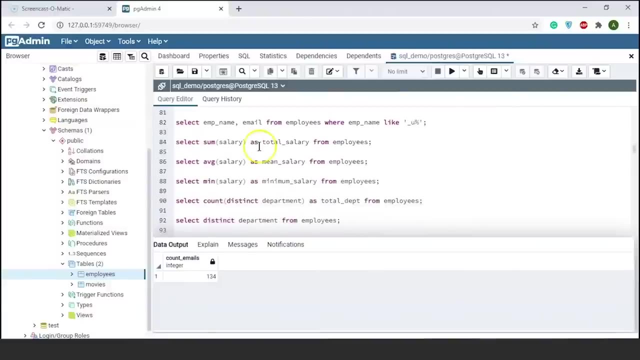 keyword in postgresql. moving further, we learnt about the like operator in sql which was used to perform pattern recognition or pattern matching. you can say: here we saw how to use basic inbuilt postgresql functions like sum, average, minimum, count, maximum. next we saw how to update: 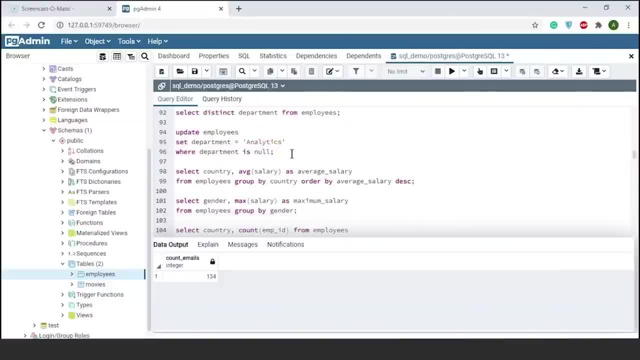 a value in a column. using postgresql update command we learned how to use group. by then we learned how to use having clause. then we learned how to use case expressions in postgresql. so we saw how case expression is similar to our, if else, in any other programming language. 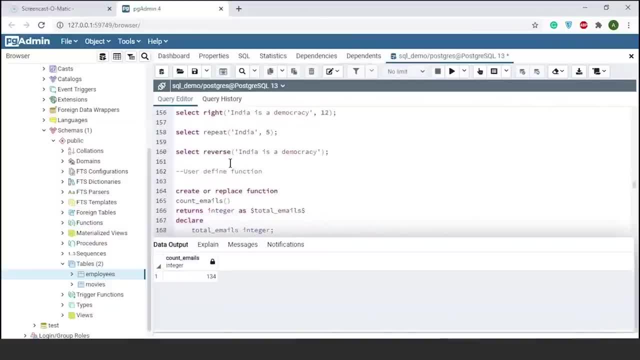 we explored a few mathematical and string functions and finally we wrote our own user defined function. so that brings us to the end of this tutorial on postgresql. now, if you want to get this sql file that we have used in the demo, you can give your email. 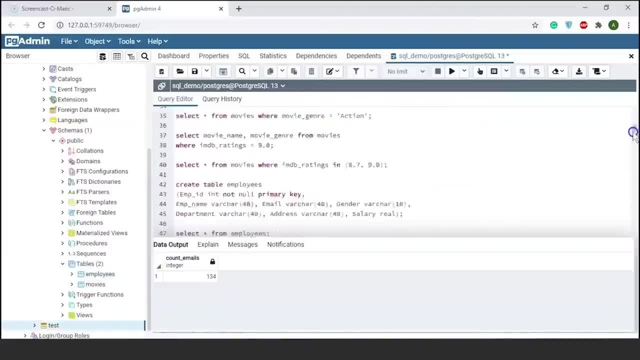 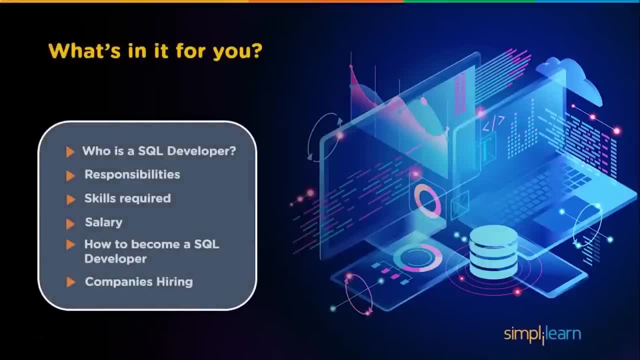 IDs in the comments section and our team will share this SQL file with you over email inferences in sq: los, sql, Igor. we will learn who is the SQL developer and what are the responsibilities in a company. then we will focus on the skills required to become a successful sql developer. we will see the 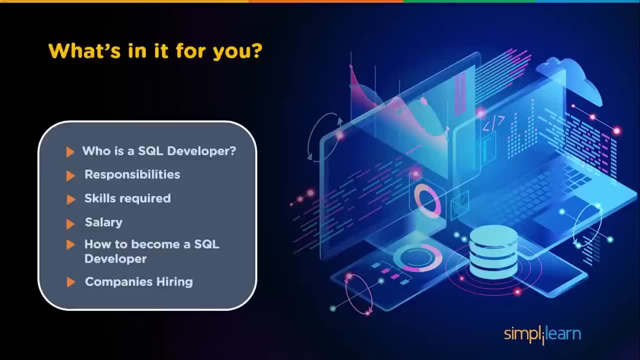 expected average salary in both us and java and开 dinner center office. we have an inventory phone gay- us and india. we will also discuss how to become a sql developer and look at the top companies hiring for sql developers. so hey everyone, i'm abhisar ahuja from simply learn and welcome to 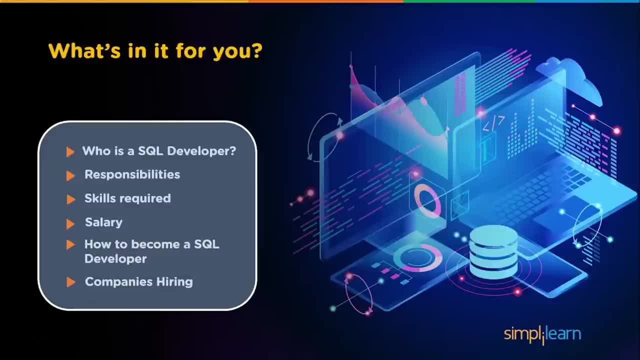 this video on how to become a sql developer. but before we begin, if you love watching tech videos, subscribe to our channel and hit the bell icon to never miss an update. when going through some of the popular job boards online, you would easily see sql developer is one of the most demanding. 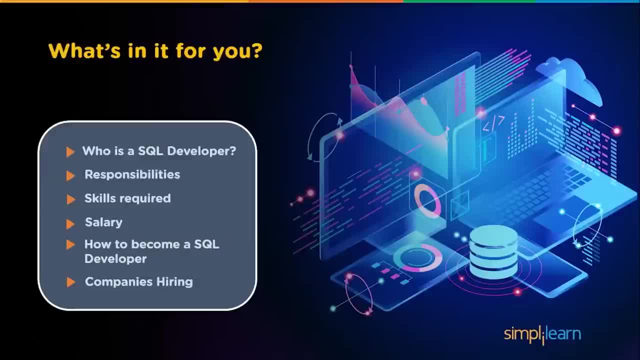 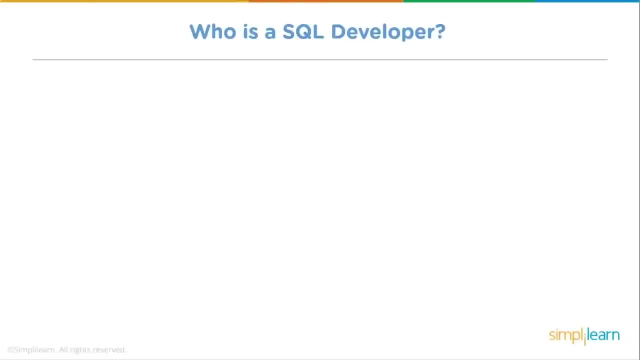 jobs seeked by companies. as we all know, today companies collect vast volumes of data and store it in their own databases. they want professionals with a good understanding of data who can keep it safe and secure. so first we will understand who is a sql developer. sql developer is a person who 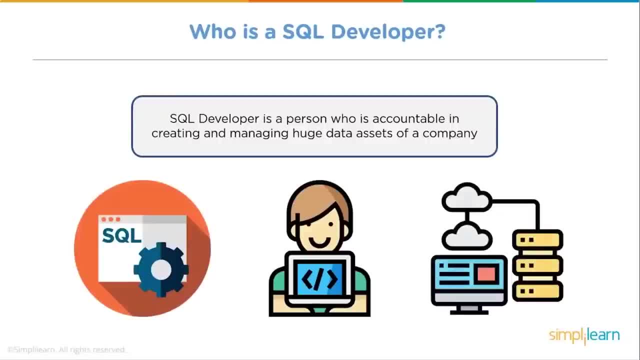 is accountable in creating and managing huge data assets of a company. in other terms, sql developer is a person who can develop sql databases as well as write and test code. let's understand this with the help of an example. let's say we want to search a particular product on amazon website and amazon has stored all its 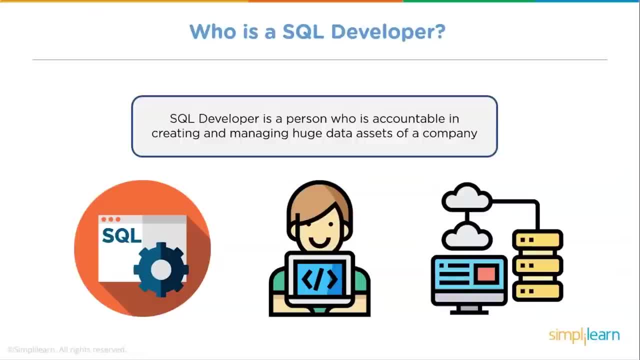 data about products in a database. now we will write the product name in the search bar and when we click on the search button it will run a sql query that fetches all the information about the product and displays us on the website. so this is the basic task done by 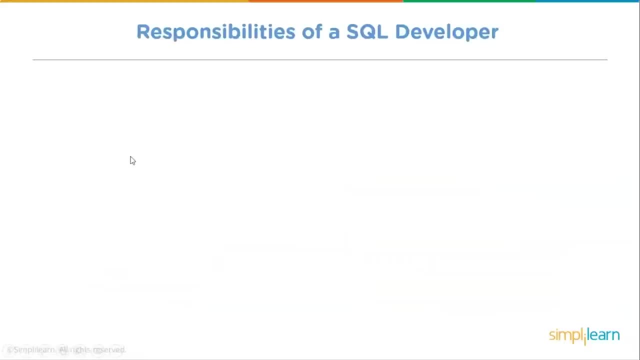 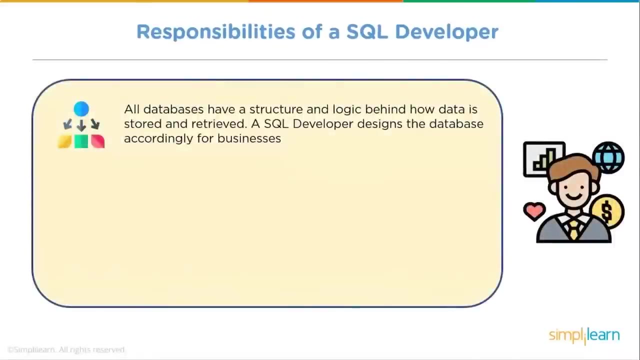 sql developer. now we will understand the responsibilities of our sql developer. all databases have a structure and logic behind how data is stored and retrieved. a sql developer designs the database accordingly. for businesses that is called database modeling. after the database is created and deployed, it's the sql developer who is responsible for fixing the 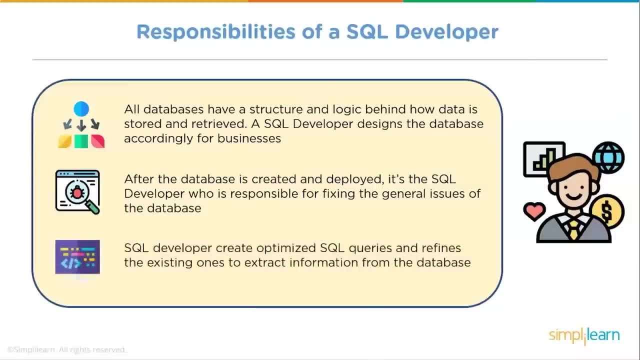 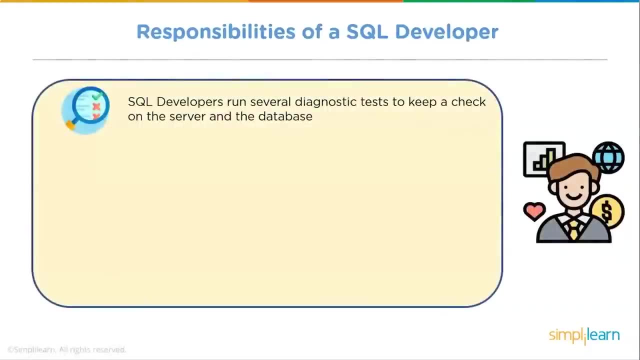 general issues of the database. sql developer should be well versed with structured query language to create optimized sql queries and refines the existing ones to extract information from the database, sql developers run several diagnostic tests to keep a check on the server and the database. in order to understand how to organize company's data, sql developers must communicate. 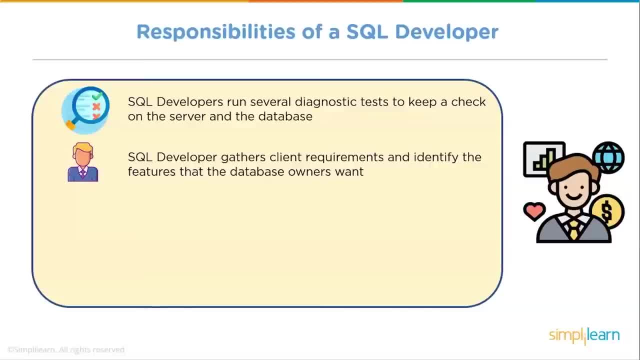 with tactical and non-technical persons from the business, and sql developer also gathers client requirements and identifies the features that the database owners require to organize the respond. As data is an asset to a company, SQL developers backup and restore data for their clients. They also perform tasks like data management and data migration. 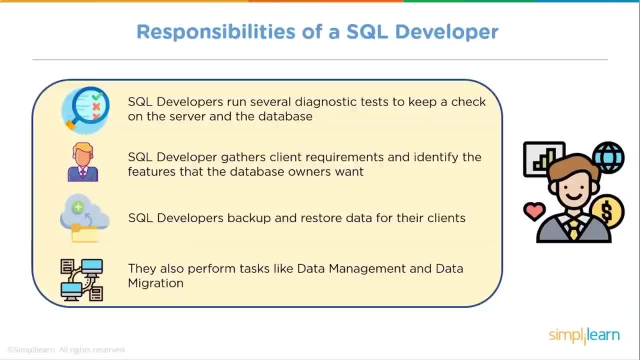 That is, if a company has stored all its data on a local storage and now it wants its data to be stored in a cloud storage. so the safe transmission of the data from local storage to cloud storage is known as data migration, And that is done by the SQL developers. 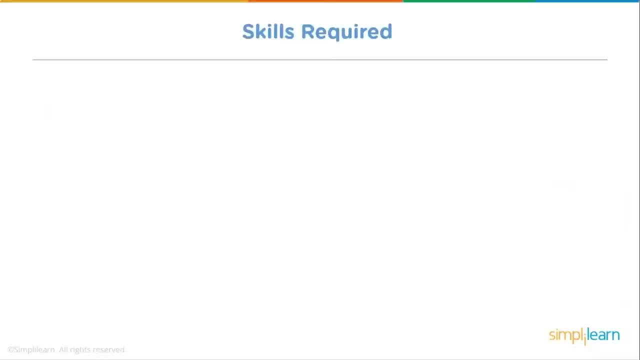 After knowing the responsibilities now we should look for skill set required to be a good SQL developer. One should have a good knowledge of SQL commands, functions, joints and procedures. Let's have a look at few commands, such as create, drop, alter and truncate. 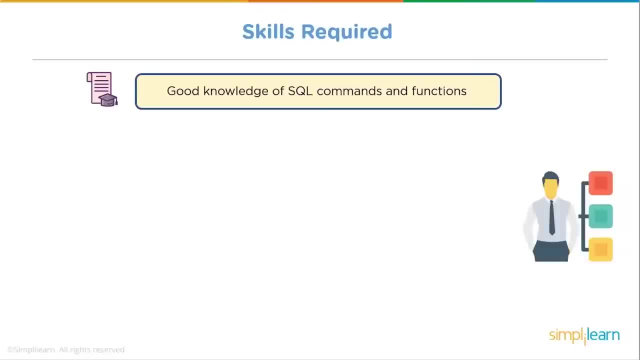 These commands come under data definition language. We also have insert, update and delete commands. These commands come under data manipulation language. We have grant and revoke commands. These commands come under data control language. We also have commit, rollback and save point commands. 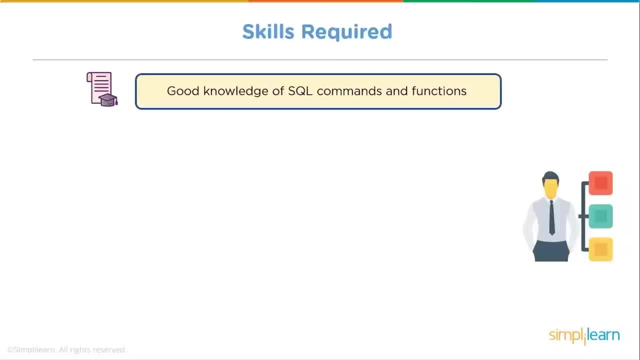 These come under transaction control language. These are the basic commands a SQL developer should be familiar with, And a SQL developer may have a little command on any one programming language. You don't have to be expert in programming. All you need is how to interface between application and your database. 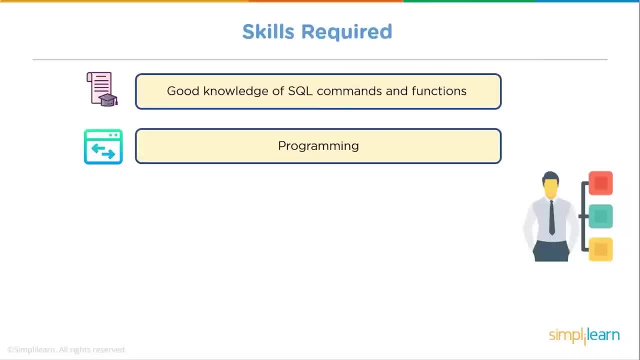 For example, you are using MySQL and your web application is based on PHP, Then you should know how to connect your application to your database And how to issue queries, how to fetch results and then how to display it to the users. One should have a good understanding of various database management systems, such as MySQL. 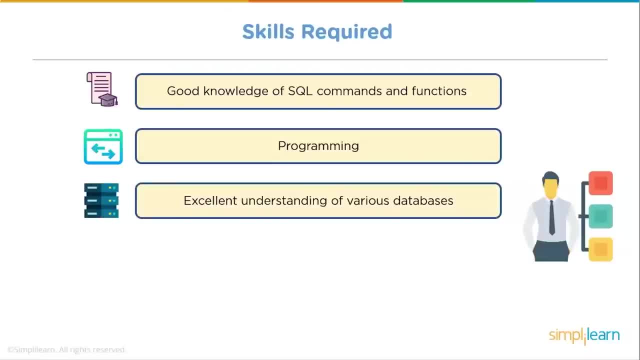 Microsoft Access, Oracle, PostgreSQL DBase, FoxPro, SQLite, IBM DB2, LibreOffice Base, MariaDB and Microsoft SQL Server. You can also have a great understanding of data visualization software such as Power BI and Tableau, which helps businesses to make better decisions and give you an add-on as. a SQL developer, One should develop critical thinking and problem solving skills to create optimized queries. Now we will see how a SQL developer is compensated in both United States and India. In the United States, SQL developers draw an average salary of $72,254.. 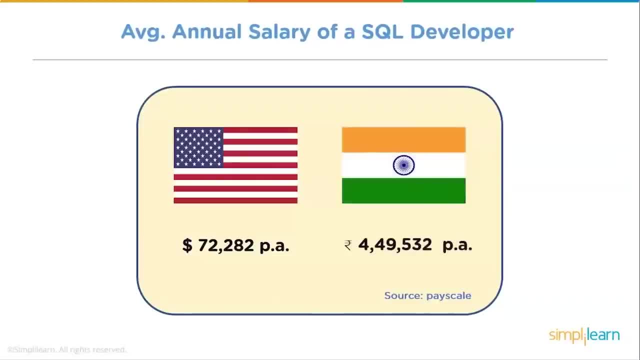 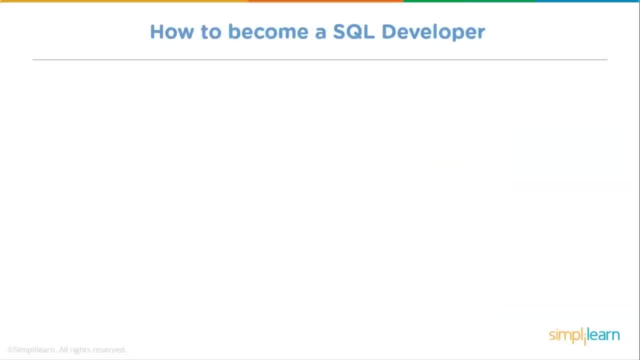 282 per annum. in india, the average salary of a sql developer is rupees 4 lakh 49 532. now we'll see how person can become a good sql developer. for that one should have a good command on structured query language and know how to interact with database management system. 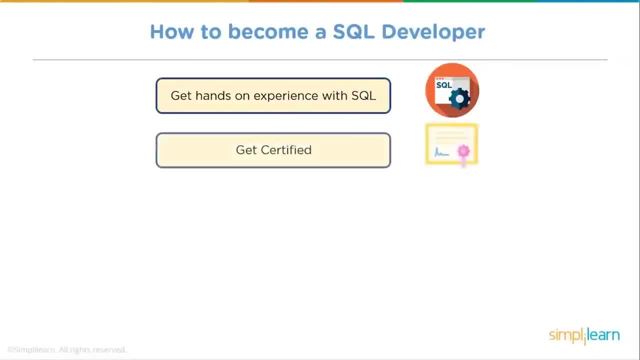 and can issue queries to get the desired result, earning industry recognized sql developer certifications, such as microsoft certified professional developer, mcpd or oracle pl sql developer certified associate, which usually require a passing score on an exam, and it's important to accumulate as much practical experience as possible. start by designing. 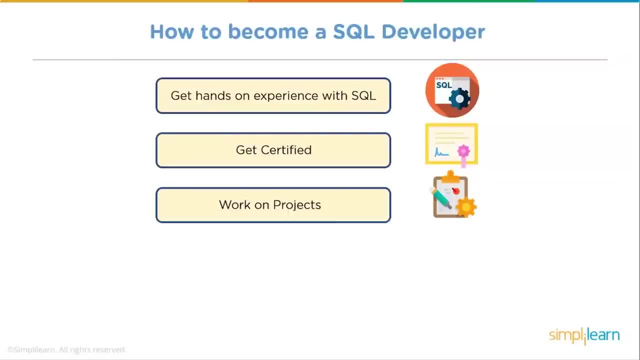 creating and querying small databases connected with your hobbies and interests, for example, your favorite music videos or your personal finances. this will enable you to gain experience, test your knowledge and build your project portfolio, which will be highly beneficial when you start applying for your first full-time position. 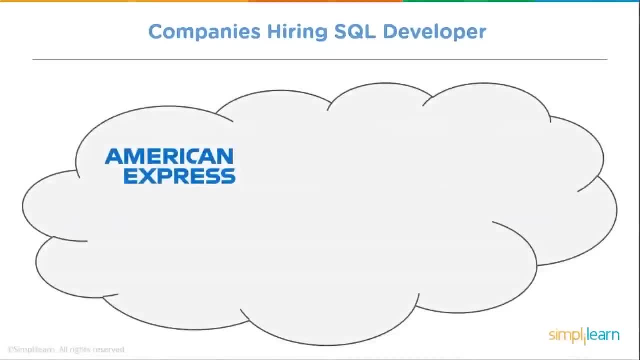 now we will see some major companies recruiting sql developers. first we have the multinational financial services corporation, american express, followed by the multinational professional services network, ernst and young. we also have the messaging company whatsapp. then we have the e-commerce giant amazon, as well as the technology and computer solutions company dell. finally, in our list of companies, we 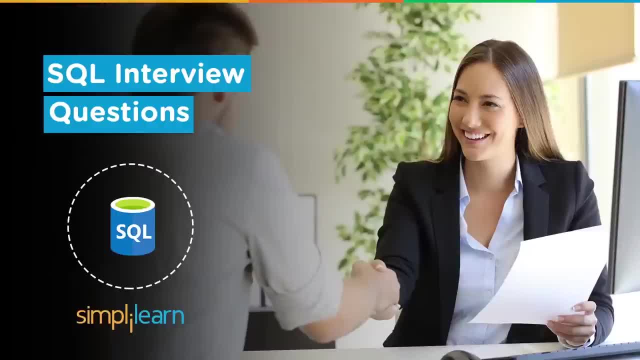 have the multinational technology company google. sql is a very important technology that is used in the id industry. professionals working as application developers, web developers, data analysts, data scientists, software testers and cyber security experts need to know sql. in this video, we will cover 30 important sql questions that are most frequently asked in the interviews. 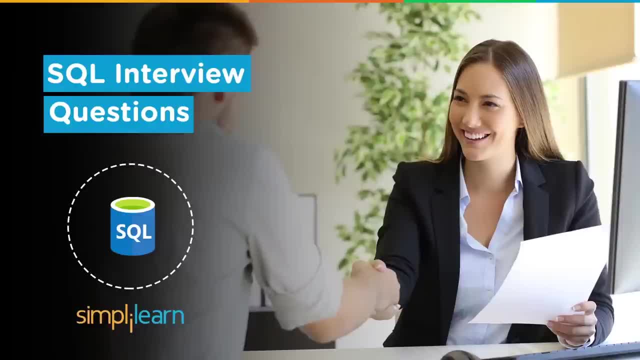 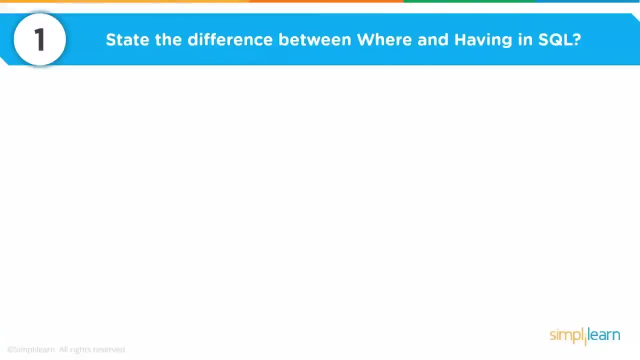 now, these questions consist of a set of theoretical and practical questions, so we will use different commands, functions, joints and other functionalities in excel to solve the problems. so let's get started with the first question. so the first question is to state the difference between where and having clause in sql. 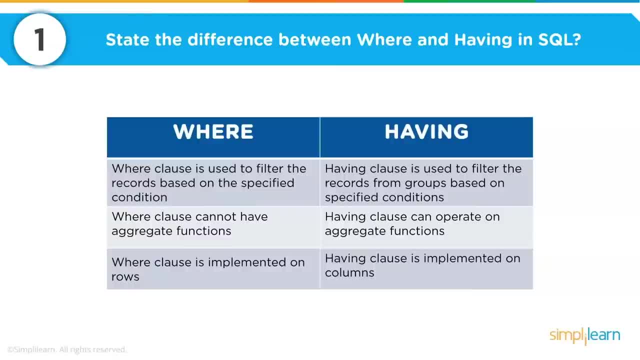 now where and having are very widely used in sql to solve specific problems. now let's look at the difference one by one. so where clause is used to filter the records from the table based on the specified condition and can be used without the group by clause, on the other hand, having clause is used to filter. 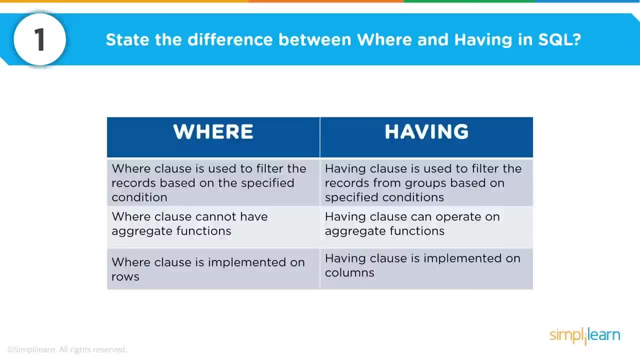 the records from groups based on specified conditions. now, where clauses cannot have aggregate functions, so you cannot use sum, count, average, min and maximum functions in the where clause, while in the having clause you can operate on aggregate functions and those aggregate functions are used to filter values from a group. 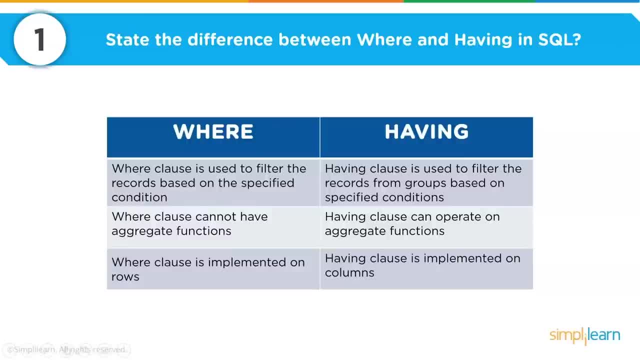 now where clause is implemented on rows or at row level. so for each row of data, you have the where condition applied. now. having clauses are implemented on columns, so for each column of data, you have the having condition applied now. another important difference between where and having is that the where clause is executed before the execution of the group by clause. 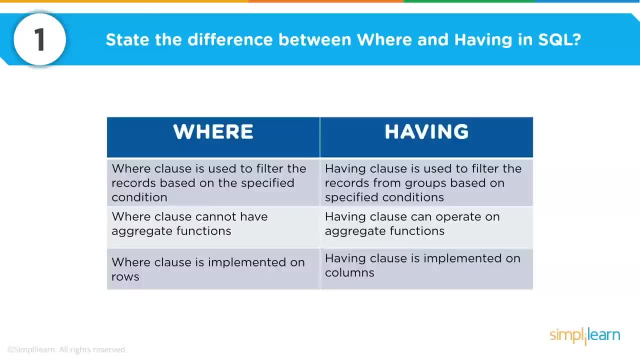 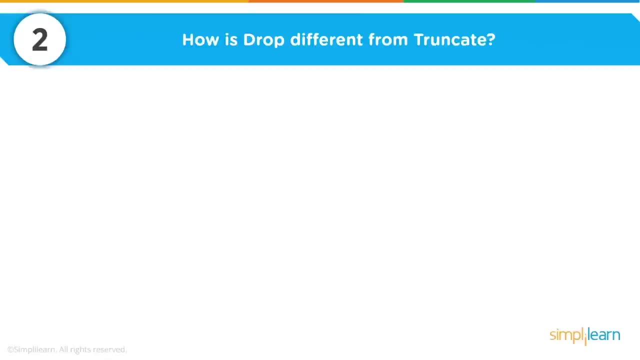 and after the execution of the from clause. on the other hand, the having clause is executed after groups are created. now we will learn more about where and having and understand the usage better when we tackle practical problems in this video. now moving to our next question, which is: 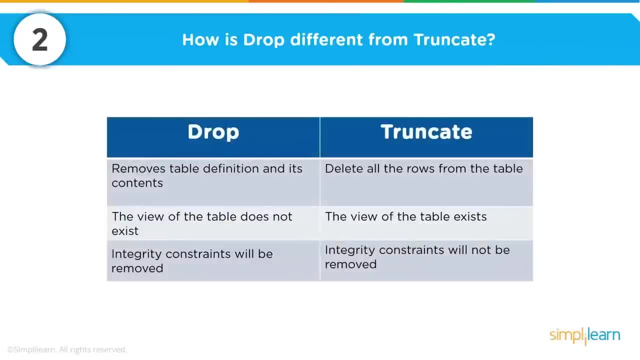 how is drop different from truncate? so drop and truncate are two different commands. so drop command drop the whole table, removing the table definition and its contents. while truncate deletes all the rows from the table, we can drop the whole table structure in one go. so the view of the table does. 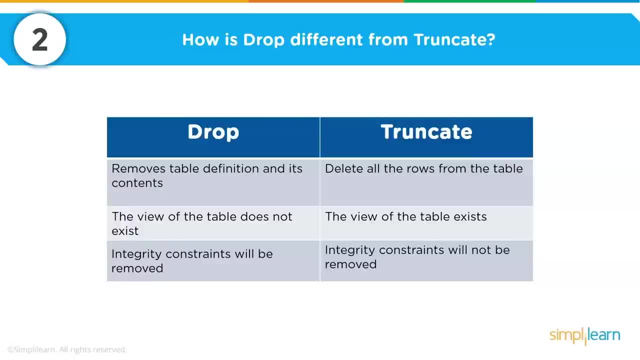 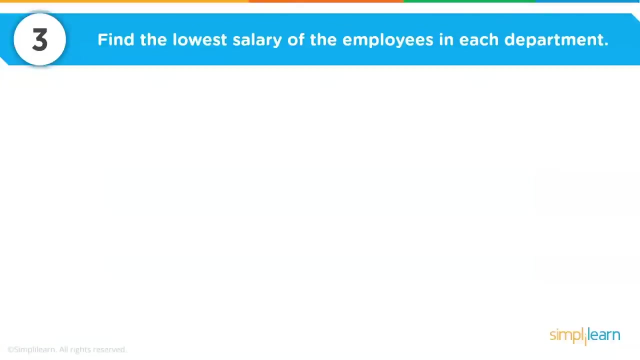 not exist. by using the truncate command, the existence of all the rows in the table is lost, but the view in the table exists. now integrity constraints will be removed in drop command, while the integrity constraints will not be removed when you use the truncate command. now moving to our third question. now, this is a practical question, so we will be using a table. 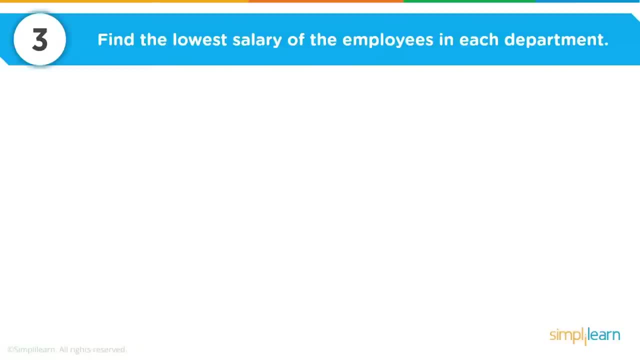 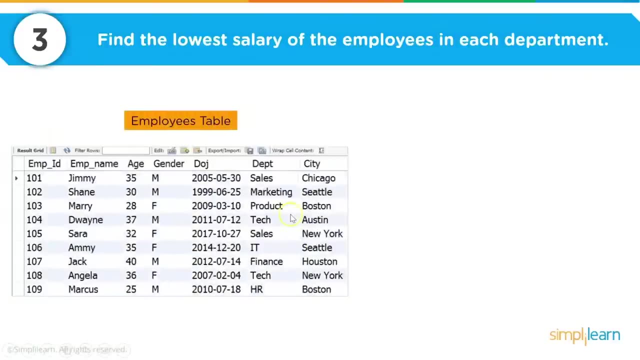 which is present in my mysql database. so the table name is called employees and i want to find the lowest salary of the employees in each department. you can see here. this is how my employees table looks and the output query would be something like this. so here, since i want to, 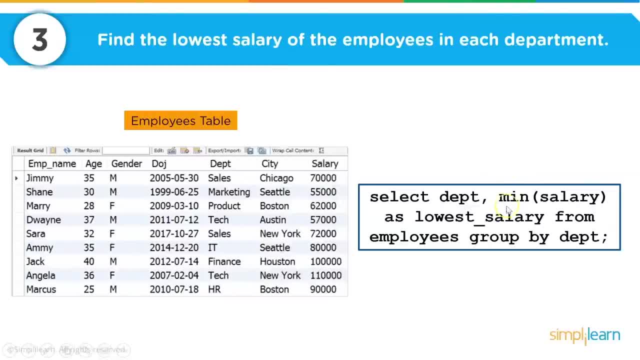 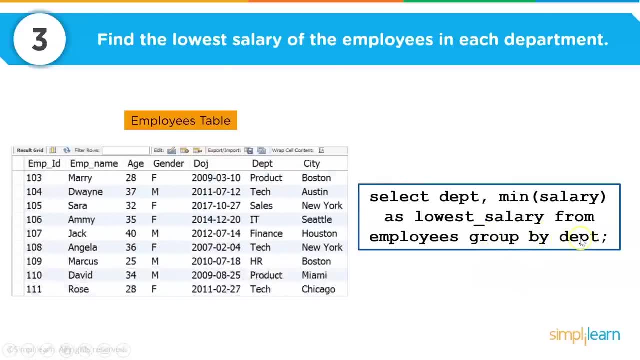 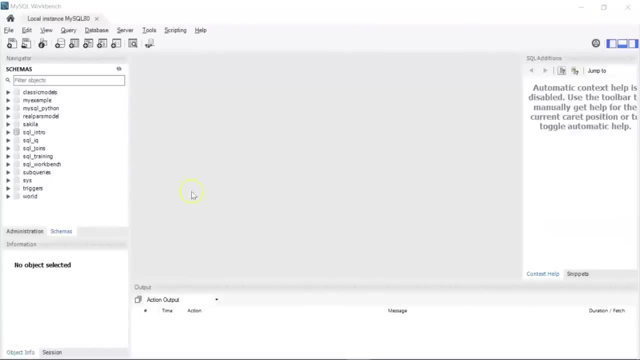 find the lowest salary of the employees. so i'm using a min function to find the lowest salary in the table and then i'm grouping all the employees and the results by department. so let's do this on mysql workbench, okay, so here i am on my mysql workbench. first, let me go ahead and create a new sql script, so i'll 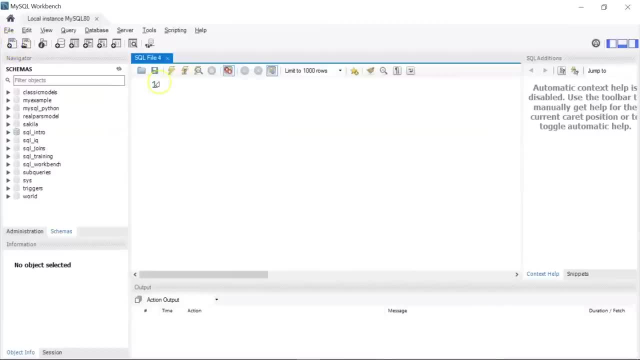 click on this and that will create a new script. okay, so here we'll write our commands, right? so our question was to find the lowest salary for each department. okay, so i've given my comment to make my commands and whatever i'm doing more readable. so first, before i proceed, 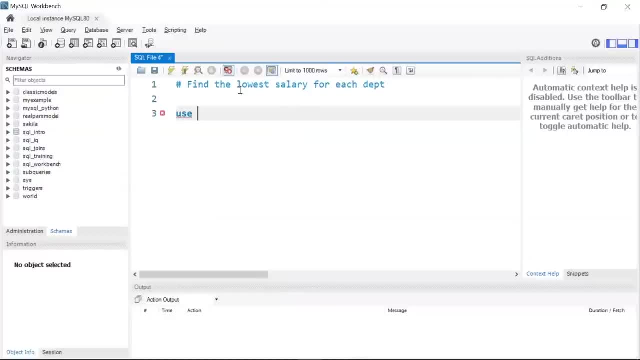 i need to select my database, so i'm going to use my sql underscore intro database. so i'll write: use sql underscore intro. now this database has a lot of tables that we'll be using in this interview questions video. i'll run it. okay, we are in our sql intro database now there's a. 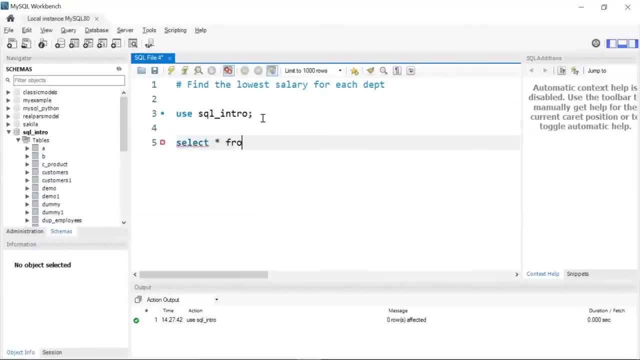 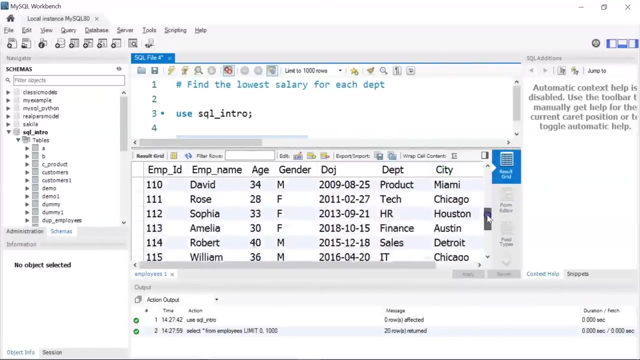 table called employees. let me show you the table first. if i write select star from employees, okay, here, sql intro database, okay. so here it is. you can see. this is the table I am talking about now. these are the rows that are present in the table. we have 20 rows and here you can see the different. 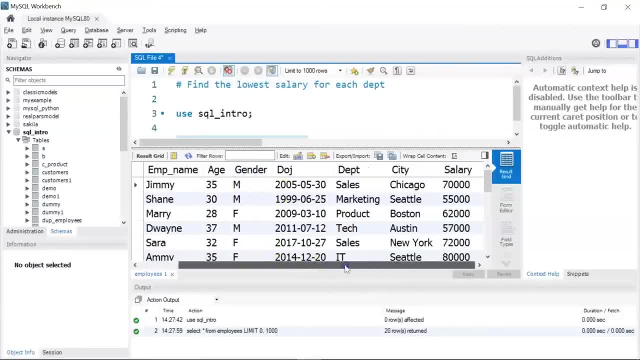 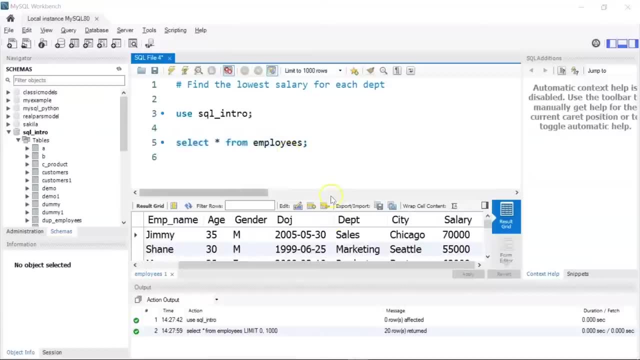 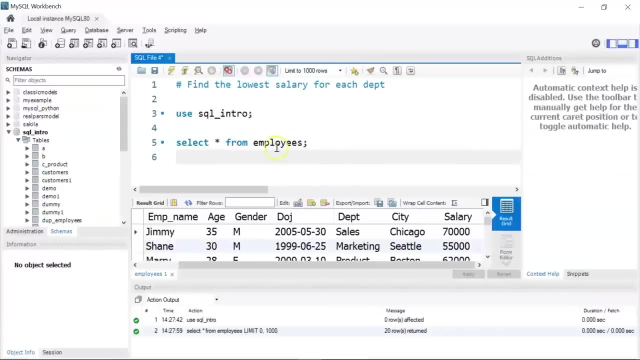 columns. we have the employee ID: employee name, age, gender. we have the department, city and salary. now this is the same table that we have also used in our other videos that are already live on YouTube. okay, so let's solve our question: to find the lowest salary for each department. now for that I'll write. 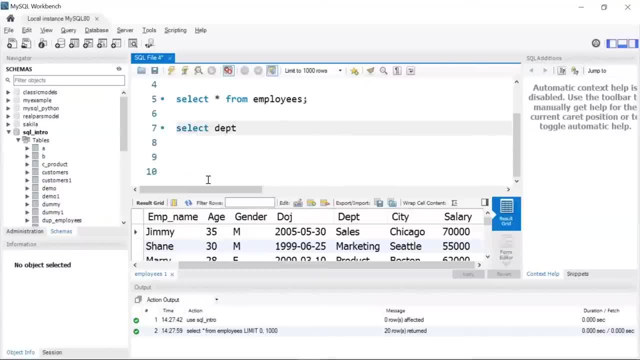 select. I'll select my department column, which is DEPT comma, and then to calculate the lowest salary or to find the lowest salary, I am going to use the min function, so that will return the minimum salary present in the salary column. so I'll write min salary as I am giving an alias name, as let's say: 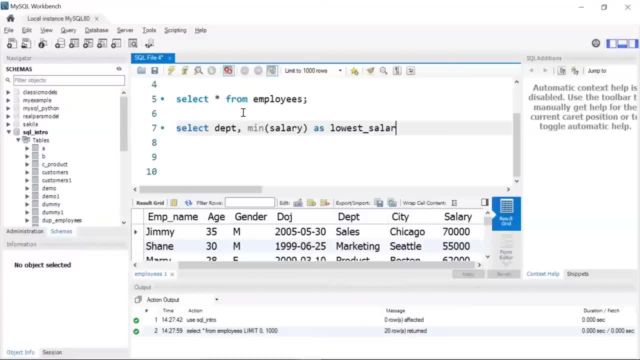 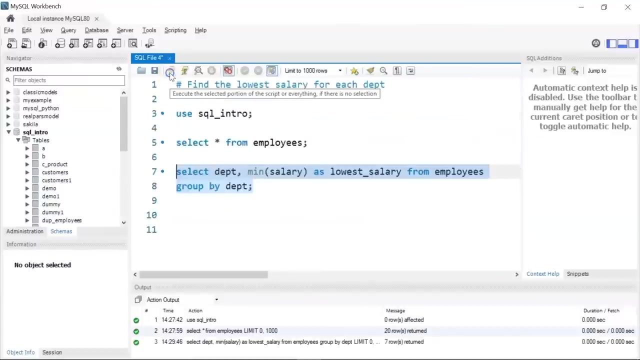 lowest underscore salary from my table name, that is employees, then I'll write group by department. I am grouping it by department because we want to find the lowest salary of the employees in each department. now let's run and see the result. there you go, I'll just move it. 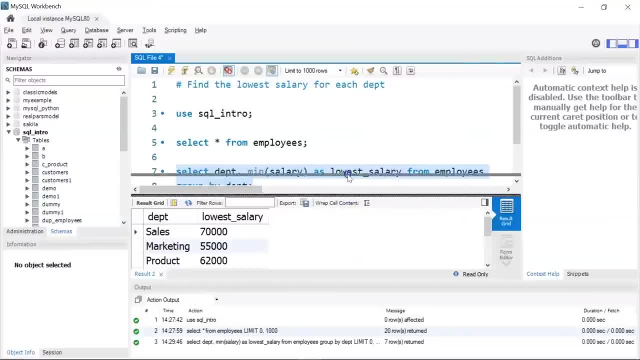 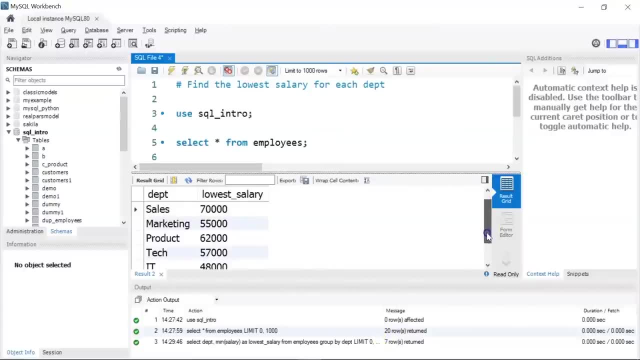 to the top so that you can see the results clearly. okay, so here we have total seven departments you can see at the bottom. and in these seven departments you can see in sales, 70,000- let's say dollars- was the lowest salary. in marketing we had fifty five thousand dollars as the lowest salary. similarly, 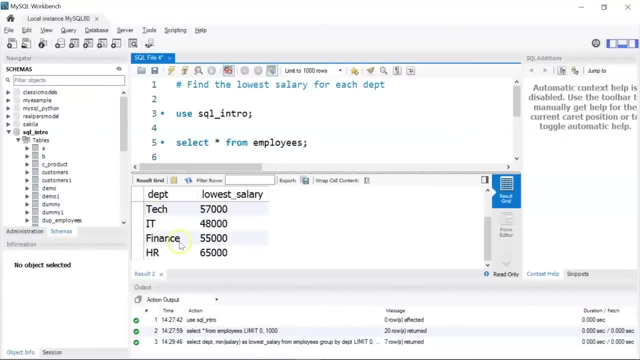 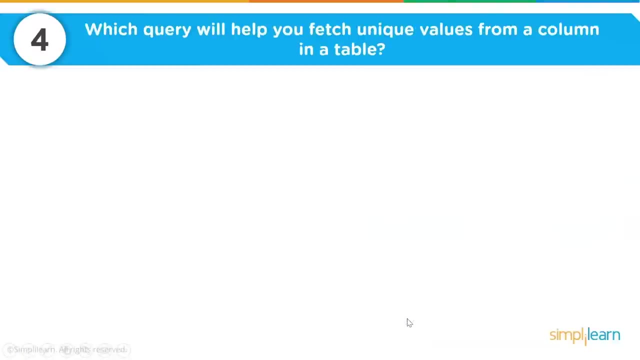 if I scroll down, we have other departments like tech, IT, finance and HR, so these are the lowest salary in each department. all right now moving to our next question. so our fourth question is: which query will help you fetch unique values from a column in a table? so this is a multiple choice question, which is: 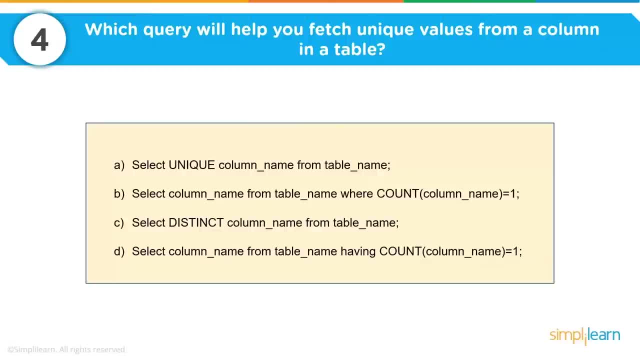 another type of question that is often asked in the SQL interviews. now we have multiple queries here and you need to choose the right query. that will solve our problem. so since I want to get the unique values from a column in a table, so the right option would be to use the district keyword in the query. so if I 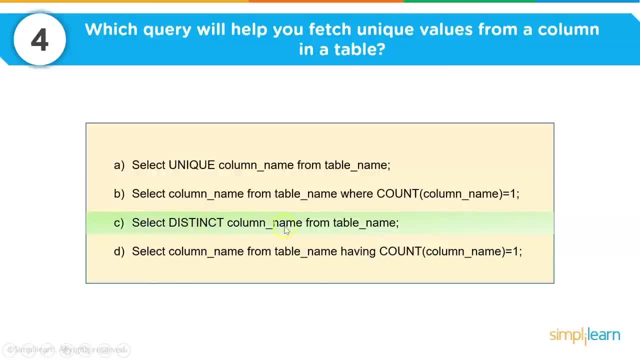 write select distinct followed by the column name. let's say you want to find the district, cities or the distinct departments in the employees table. so the query would be: select distinct City or let's a department from the table name, that is, employees. What we are doing is we are atenciónBut is peopleIn this query not specific to the? 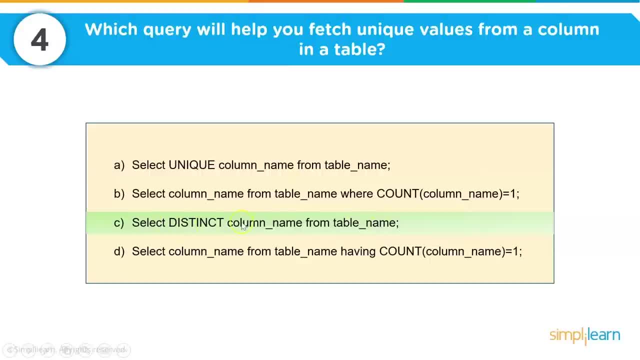 this query is specific to the other. thankfully, if this query is specific to extra to the other threatened, which I would. Frankly, everyone is notucated of my hence this is the right option if you want to find any unique values from a column. now, moving to the 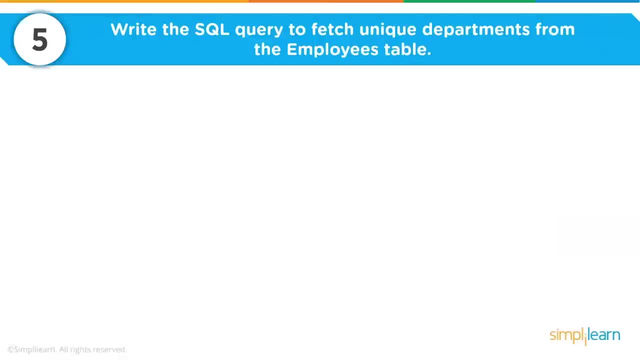 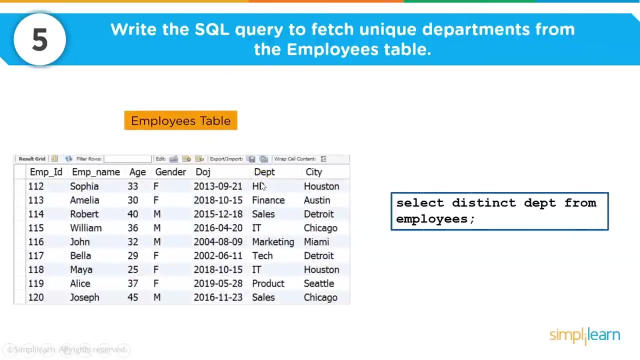 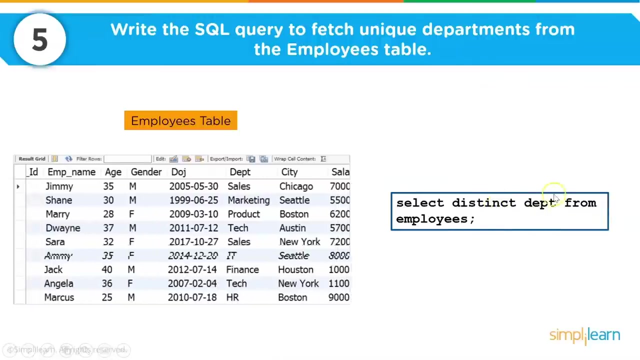 fifth question. now the fifth question says it is actually a similar question. here we want to write the sql query to fetch unique departments from the employees table. so, as we saw, this is our employees table and if you want to find the unique departments from the employees table you can just write select distinct, then followed by the column name. 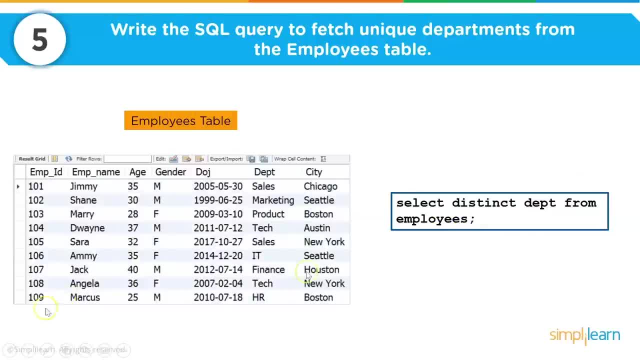 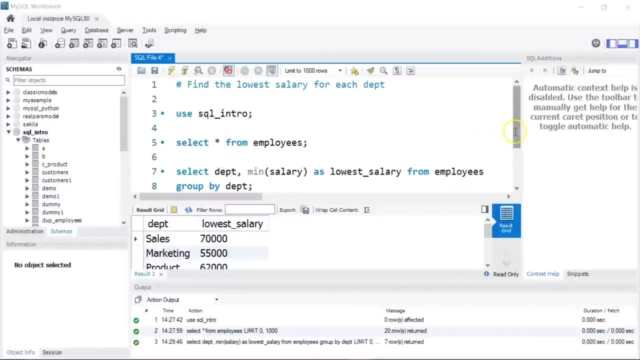 which is departments here, so dept from employees. let's do this on our mysql workbench, okay? so let me just scroll down and i'll give a comment here. that is, we want to find the unique departments, so the query would be select. then i'll use the distinct keyword. if i hit tab, it will auto complete. 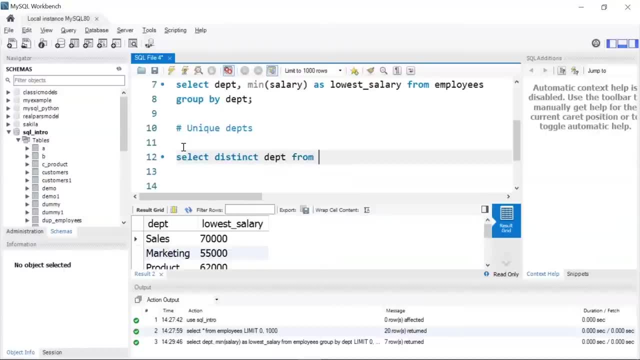 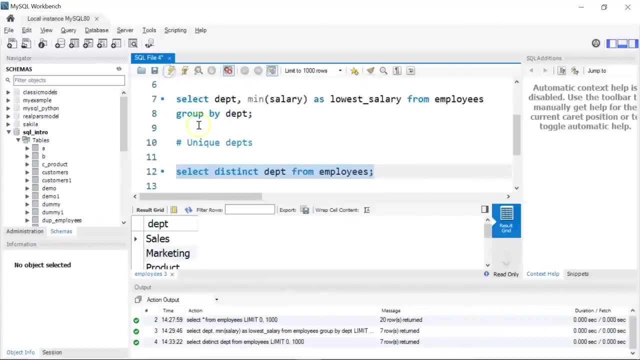 then i have my column, that is department from my table name, that is employees. if i run this, the query will give us the unique departments that are present in the table. so here we have total seven unique departments in the table. you can see here we have sales marketing. 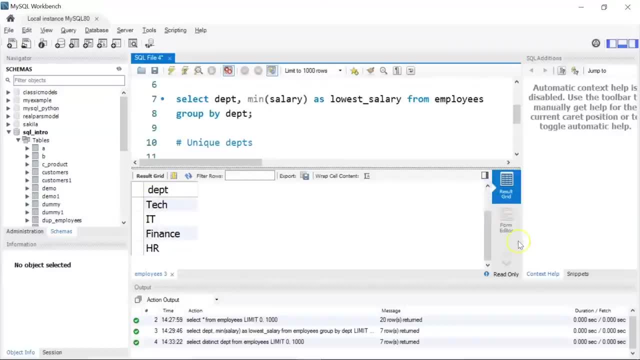 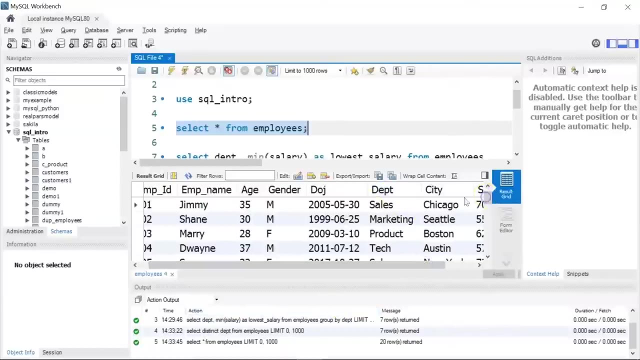 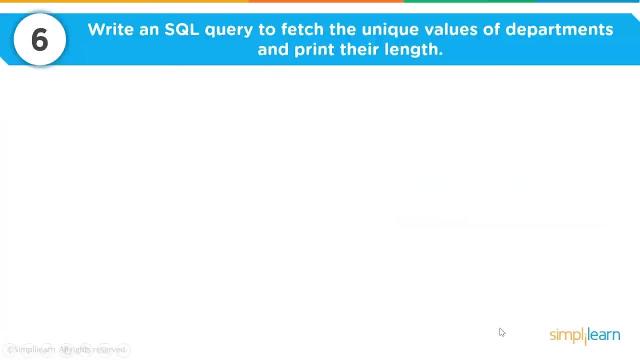 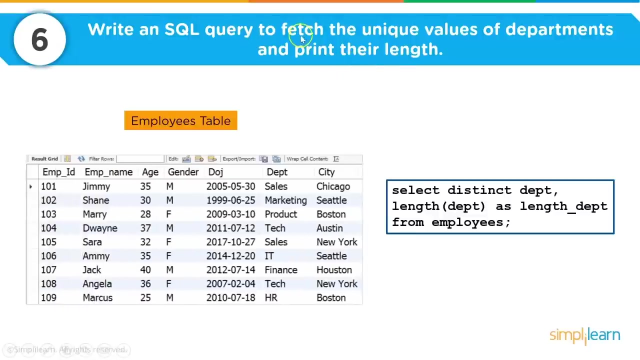 product, tech, it, finance and hr. but if you see our original table, which is the employees table, so there are total 20 records and if you see the department column, there are multiple departments to which each of these employees belong to. okay, now moving ahead with the jargon, so here i have given you a số one, and it says these are: 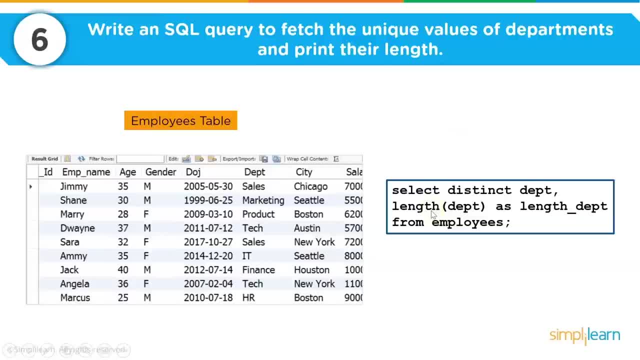 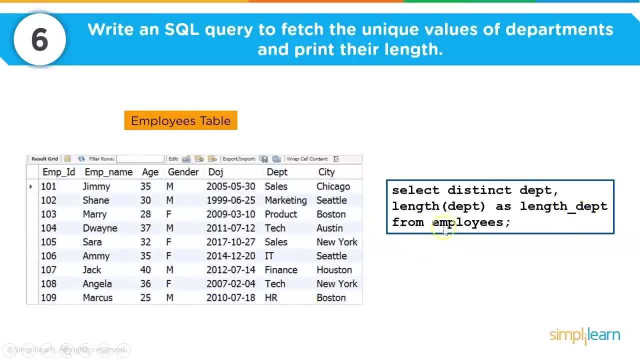 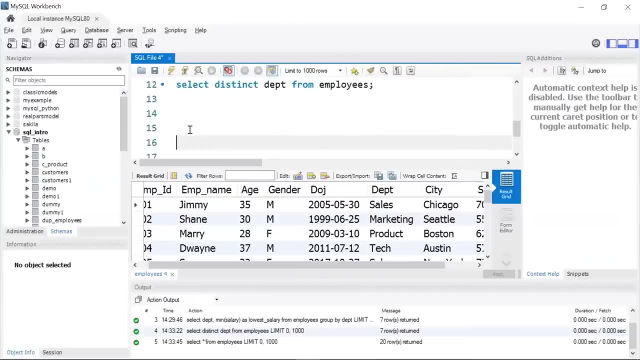 the inbuilt length function that is present in mysql to find the length of the department, and then i am using an alias that is length underscore: department from employees. so let's say this on our workbench, okay? so let me give a comment. i'll say unique departments and 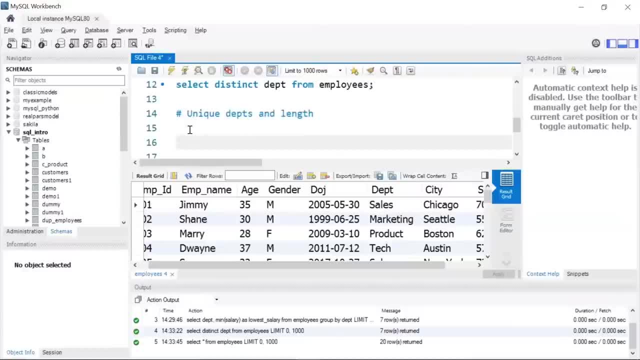 length. okay, so the query would be: i'll write select distinct department and then let me just scroll down. i'll give a comma and use my inbuilt length function. see, i'm hitting tab to auto complete and inside the length function i'll give my column name, that is department. 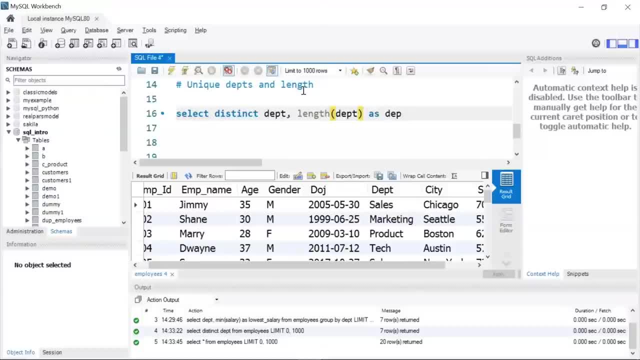 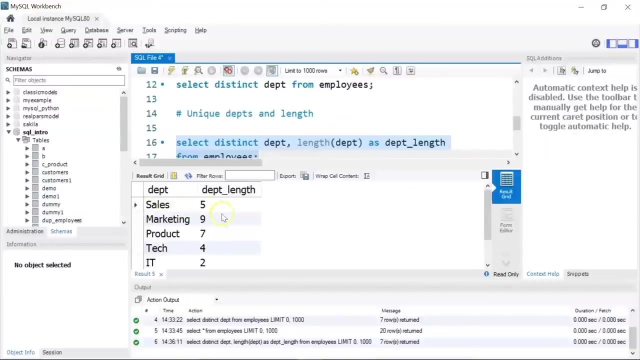 i'll give an alias as department underscore length from my table, that is, employees. this is pretty simple. so first i am finding the unique departments and then using the length function, i am finding the length of each department. let's run and see. okay, you can see the result here. so, sales: the length is 5. marketing: the length of marketing is 9. 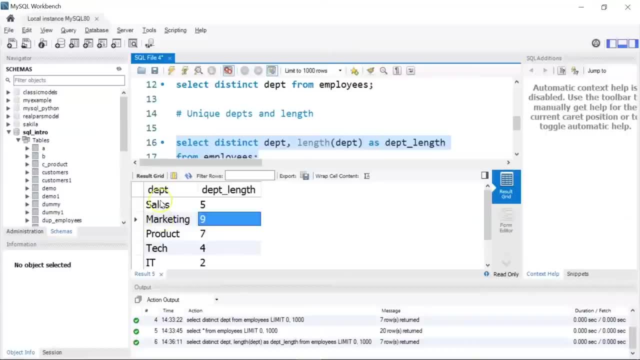 basically you are counting the number of characters that are present in each of the departments. so in sales, there are total 5 characters. in marketing, there are total 9 characters. in product, there are total 7 characters. in it we have just two letters, i and t, so hence the 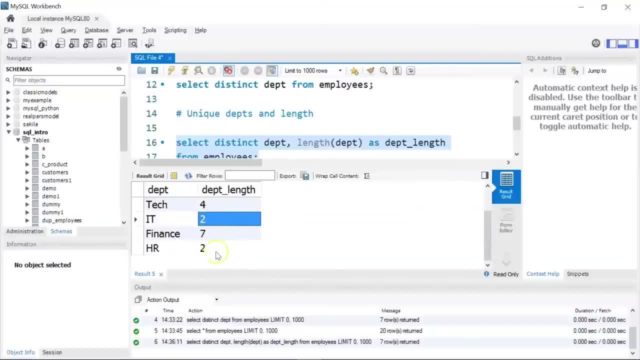 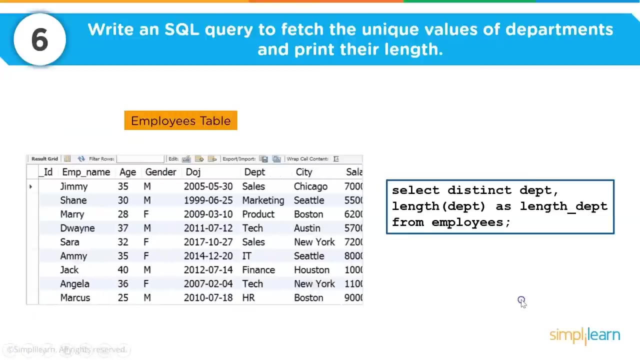 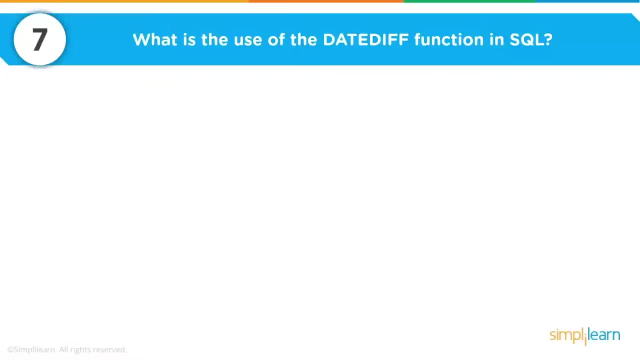 length is 2. similarly, finance is 7 and hr is 2, because we have just two letters, h and r. okay, so this is another variation of using distinct along with any inbuilt function. all right now, moving to the seventh question. the question is: what is the use of dative function? 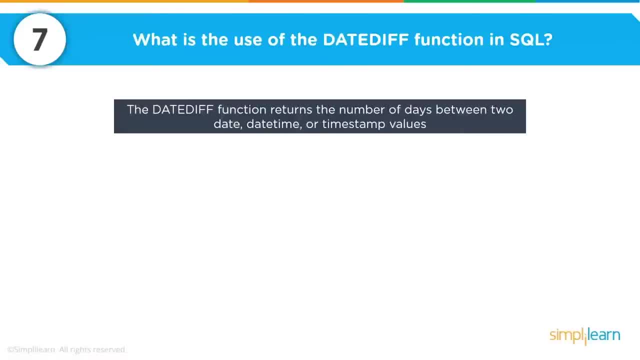 in sql. now dative returns the number of days between two date or date, time or time stamp values. so datediff is another crucial inbuilt function that is present in mysql. so here is how you can use the datediff function. so it will the number of days between two dates or date, time or timestamp values. so here i have two date values. 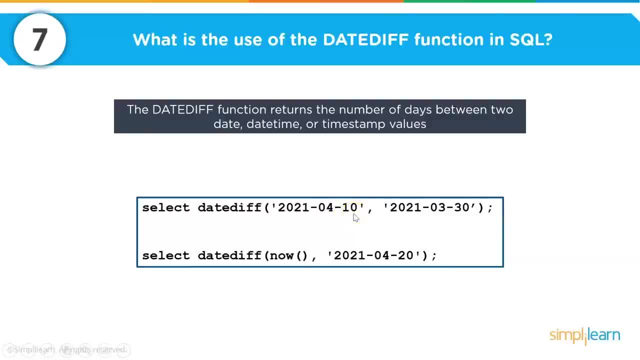 that is 10th of april 2021 and i have 30th of march 2021. so this query will give us the total number of days that lie between these two dates and, similarly, here is another example of using the date dip function. so i want to calculate the total number of days that are present between 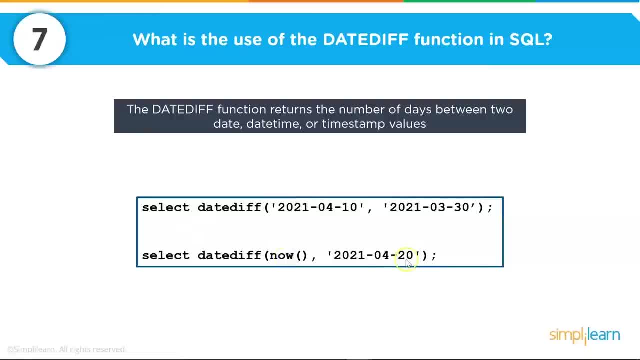 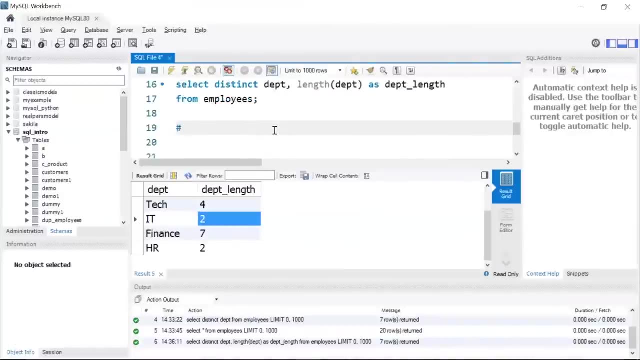 today's date- so i'm using the now function- and between 20th of april 2021. so let's do this demo on the workbench, all right? first i'll give a comment saying date dip function. okay, now the way to use is i'll write select and then you can see here once i type date. 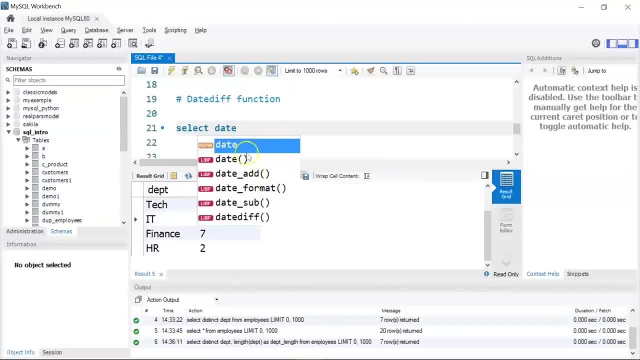 mysql workbench is automatically suggesting some of the inbuilt functions. i'm going to use date diff and within date diff, i'm going to pass in two values. so i'm passing in two date values. let's say 2021 april, so i'll write 04. 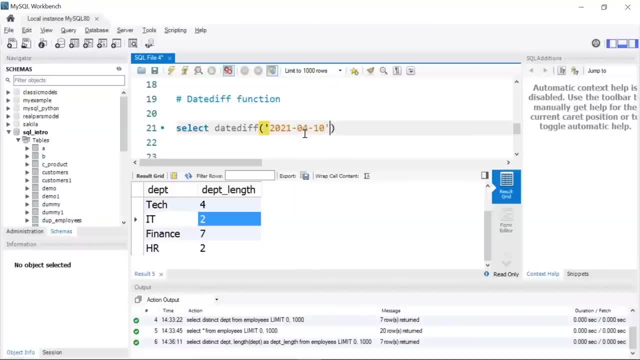 and let's say 10th of april. i'll give another comma and i'll pass in my second date value. that is going to be 30th of march 2021. all right now. another thing to note here is the date value should be present inside quotations. if you want, you can give an alias as well. i'll write. 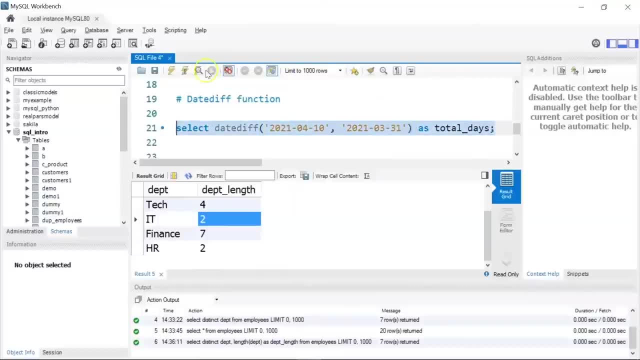 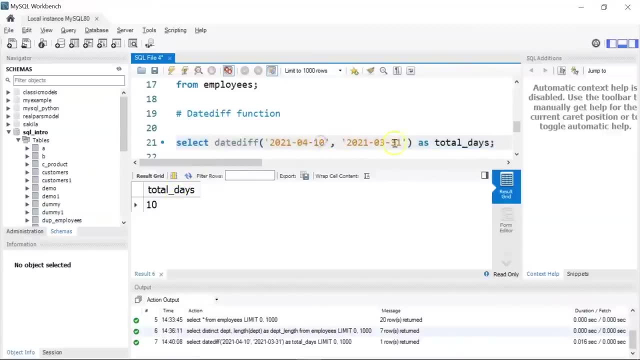 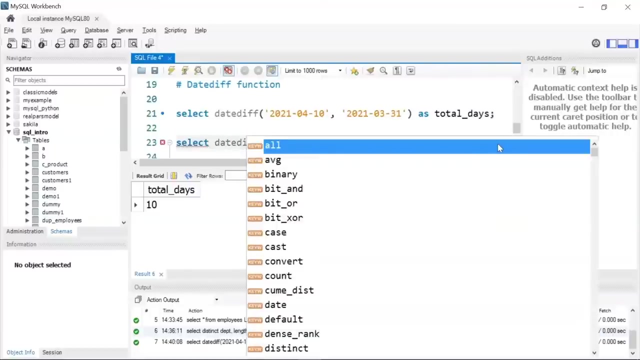 total days. let's run it. there you go. it has given us the output as 10, so there are total 10 days between 31st of march to 10th of april. now let's see another example. i'll write select date diff and we'll pass in my now function. so the now function returns the 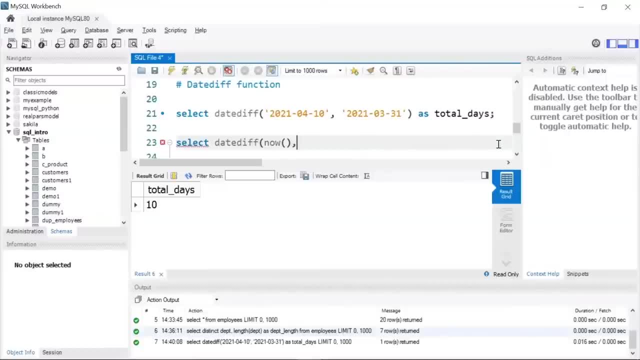 current date, that is today's date, and i'll give another date value, let's say 2021, april 20th. now we'll see the results. if you want, you can give an alias name so that the output is more readable here. i'll run it. okay, so between today's date and my previous date, that was 20th of. 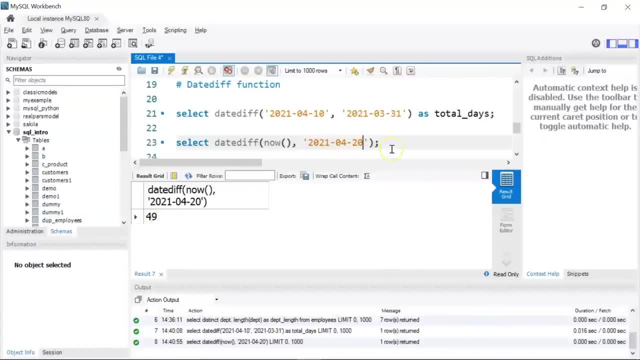 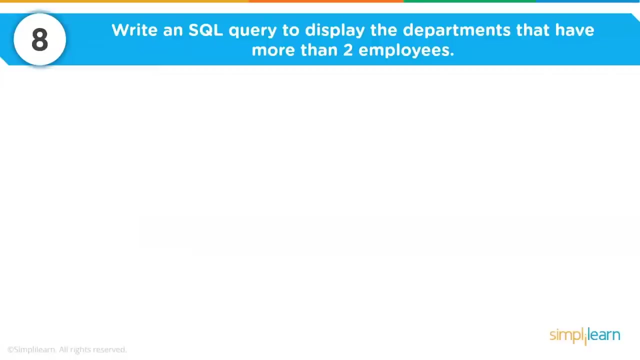 april, there are total 49 days. so today's date is actually 8th of june. so between 20th of april and 8th of june there are total 49 days. all right now. moving ahead. now in the eighth question, we want to write an sql query to display the departments that have. 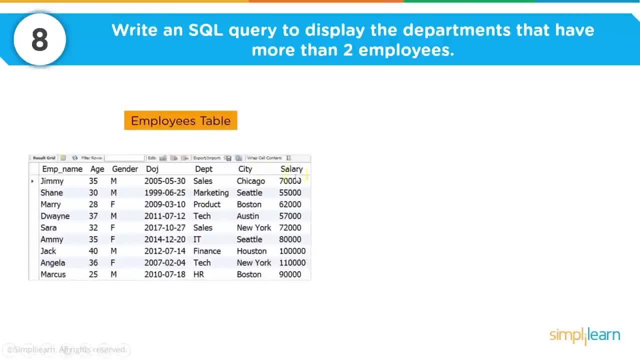 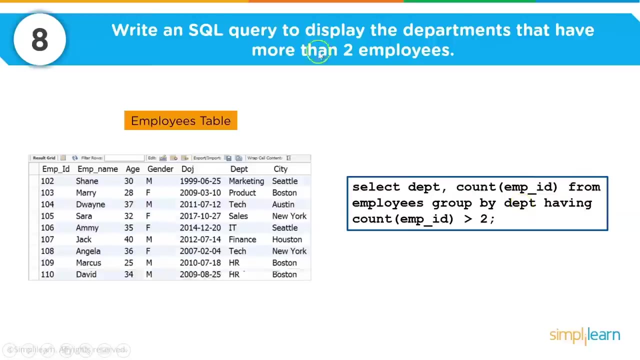 more than two employees. so this is our employees table that we have been using and here is how the command looks like. so here we are, using both group by and having. now i am grouping by department because i want to display the departments that have more than two employees. now for the second filter, i am using the 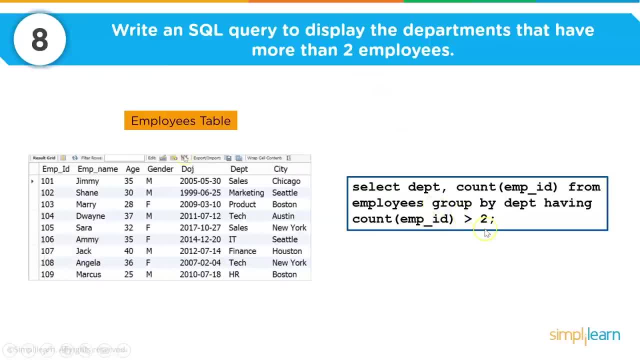 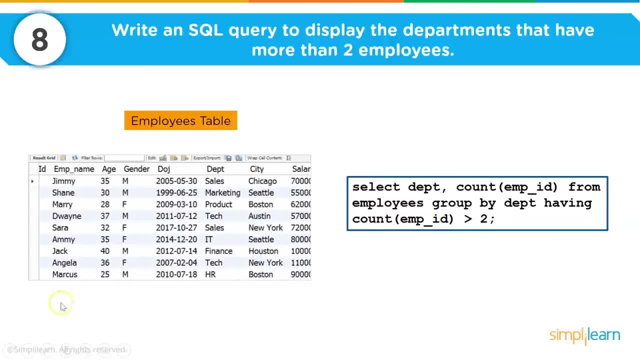 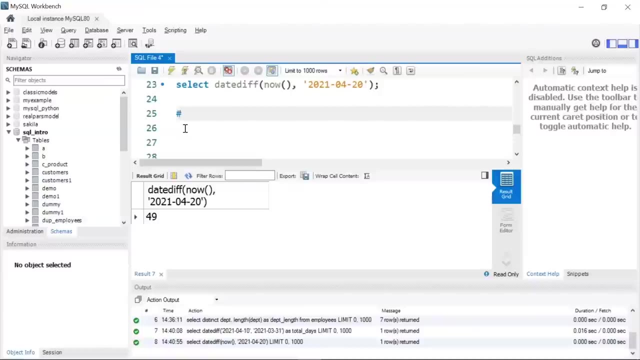 count, function of the employee ids and checking if the employees in each department are more than two or not. let's do this. let me move down a bit and i'll give a comment. departments with more than two employees. okay, now let's write our query. so i want to select. 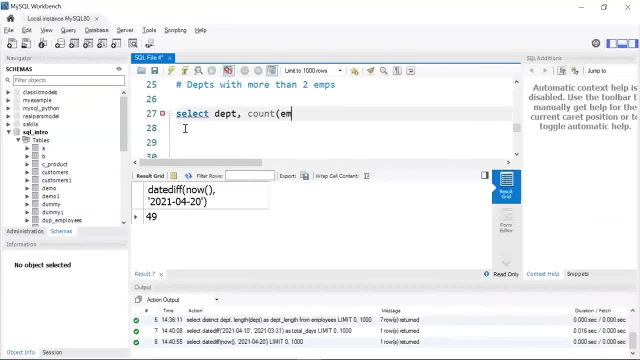 the department and then i'm using the count function to count the employee ids in each department or the employees present in each department from my table, that is, employees i'm going to group by department and then i'll use having my count of employee id. this should be greater than two, so our query will return only those departments which have more than. 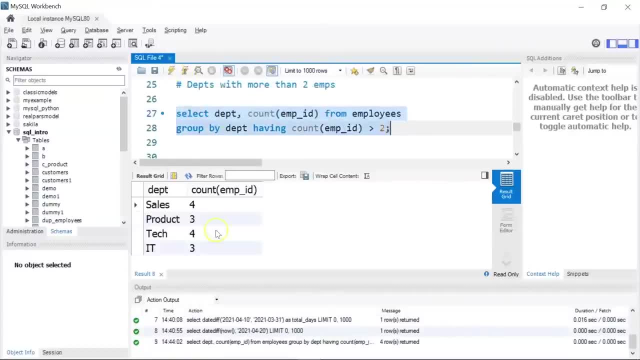 two employees. let's run and see there you go. so we have total four departments, that is, sales, product, tech and it, where we have more than two employees. you can see here, sales has four employees, product has three, tech has four and it has three. the rest of the departments, like finance. 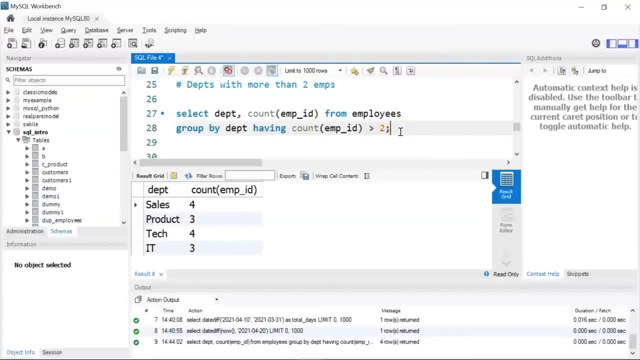 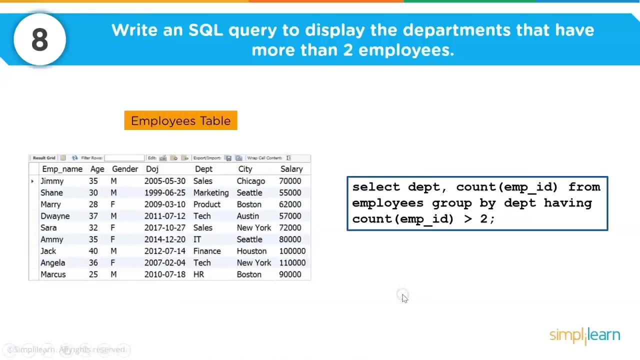 hr and others have less than two employees. now, if you want, you can give an alias as well, let's say as total employees. okay, let me run it again and here you can see i have the column name as total employees. okay, so moving ahead. the ninth question: we want to display the details of the employees for 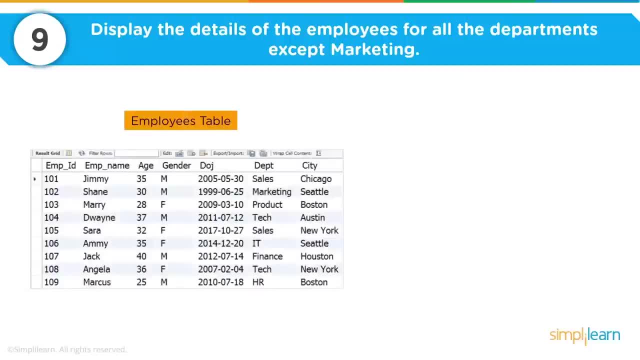 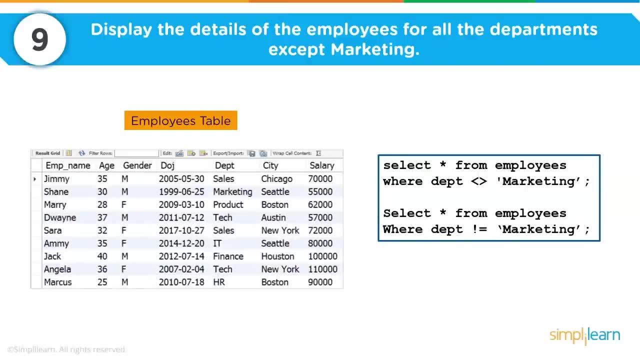 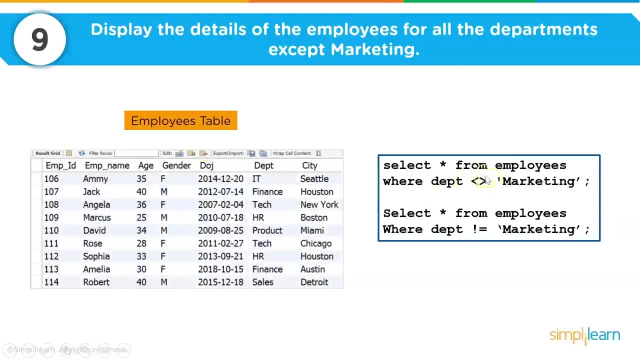 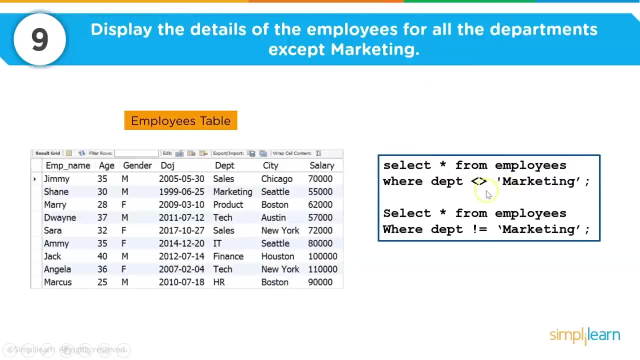 all the departments except marketing. now here i have my employees table. if i were to display all the details of the employees apart from marketing department, i can give a condition like: where department not equal to marketing? so this is the way how you write: not equal to. so you use the less than and greater than symbol. another way to do is: 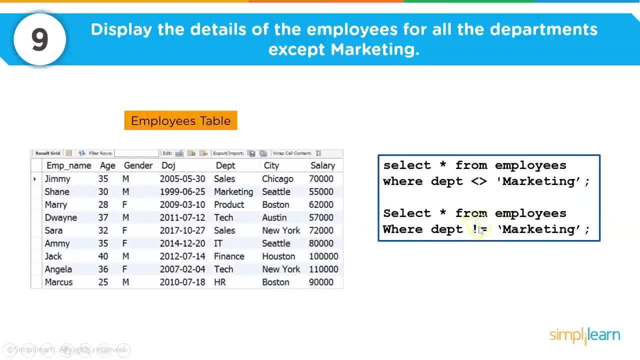 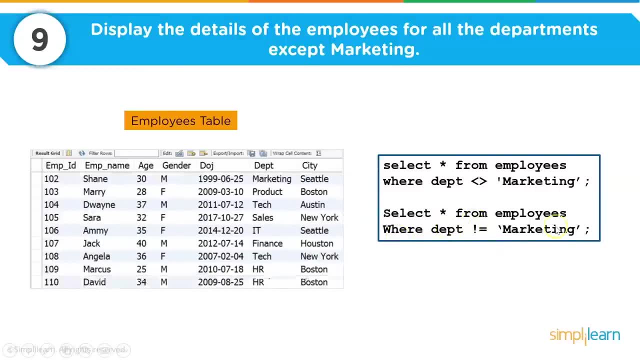 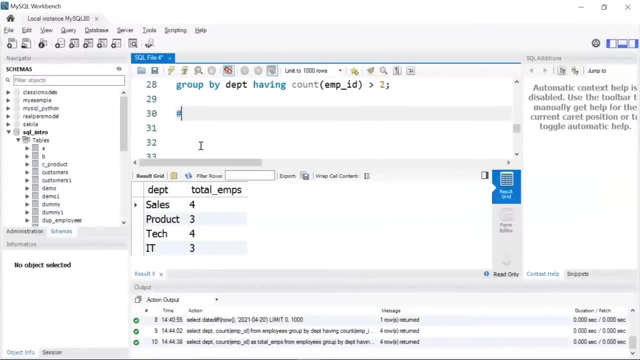 use the exclamation mark and give equal to. so this means select all the employees where department is not equal to marketing. now let's do this. i'll move down a bit and we'll give a comment as details of employees apart from marketing. so the query would be: select star from employees? i'm using star because i want to display 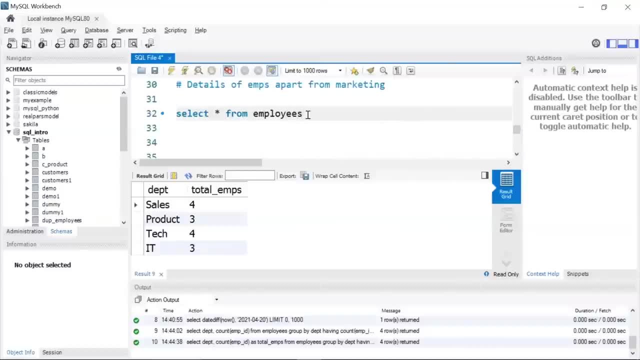 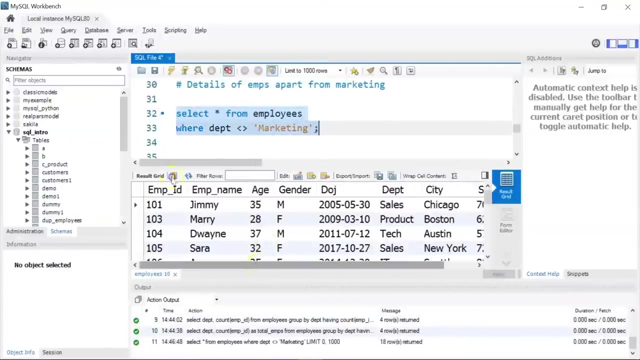 all the details. that means i want to display all the columns. then i'm going to use my where condition. where department not equal to marketing, i'll put marketing under quotes. let's run it and see the results. there you go. so we have total 18 rows of information and if you see, the department column. 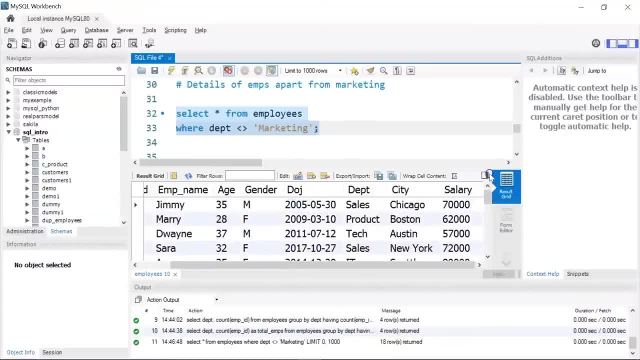 we have all the departments apart from marketing. now, if you remember, our employees table had total 20 rows of information, out of which two are missing, which means there were two employees who were from marketing department and those departments were not displaying. now, another way to do is to use 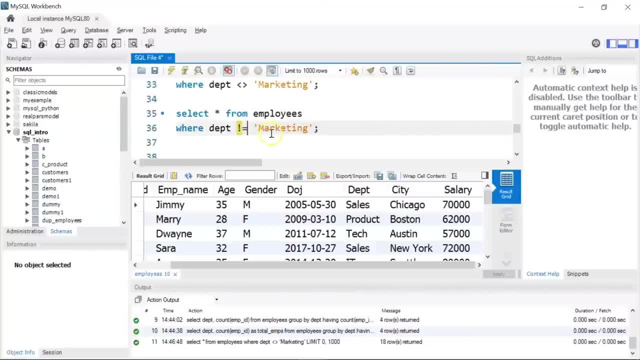 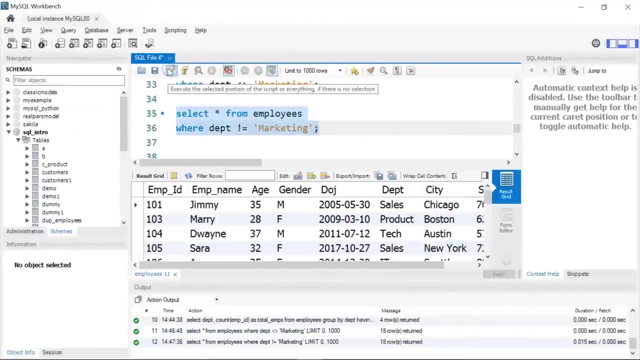 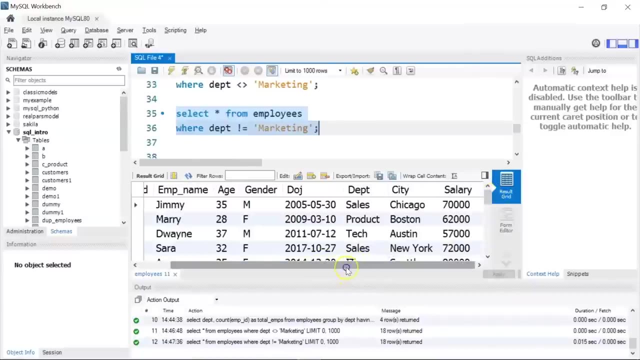 exclamation mark and equal to. so this also means select all the employees where department is not equal to marketing. let's run this. you see here it gives us the same result and has returned us 18 rows of information, leaving apart the employees from the marketing department. all right, now moving ahead. 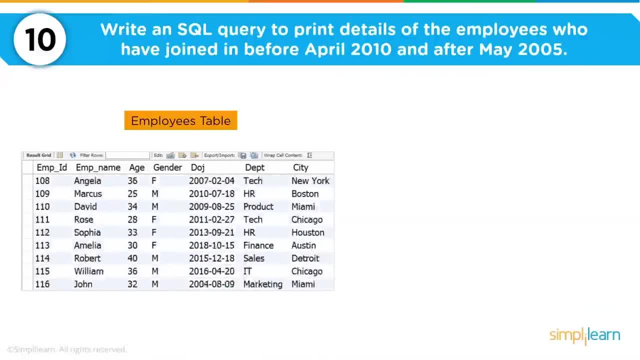 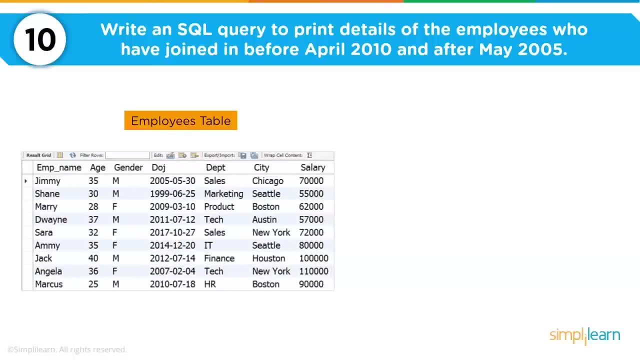 so our 10th question is to write an sql query to the marketing department. so i'm going to use my sql query to print the details of the employees who have joined before april 2010 and after may 2005. so here is my employees table and this is my sql query. so here, 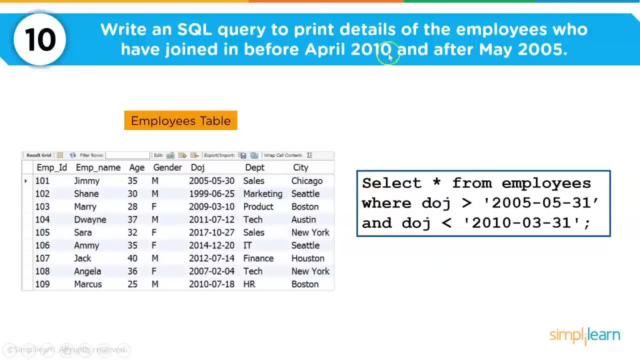 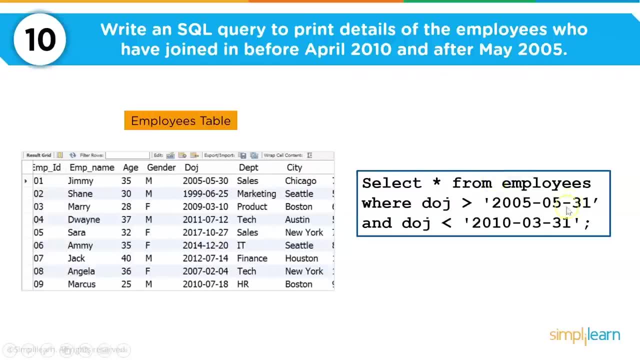 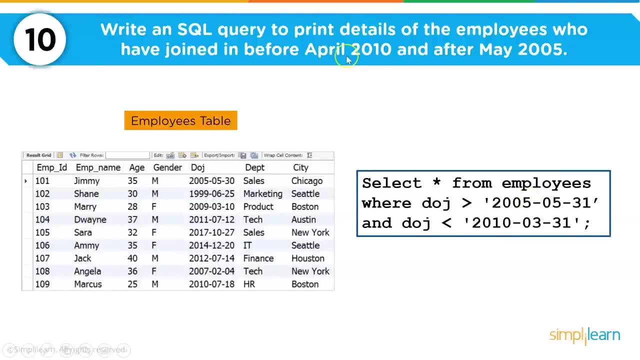 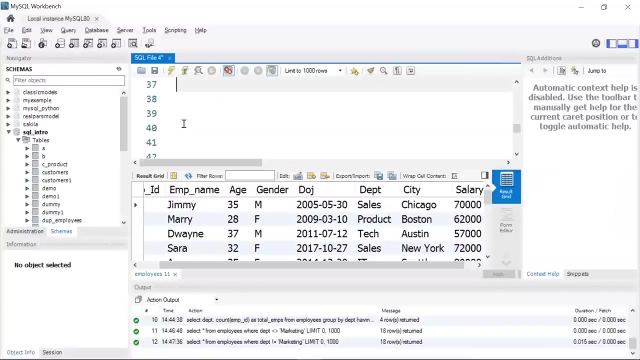 we are using just a where condition to filter our results and my condition is: the employee should have joined after May 2005. so I have written after 31st of May 2005 and before April 2010, which is before 31st of March 2010. let's do this. I'll give a comment here. will write: employees joined. 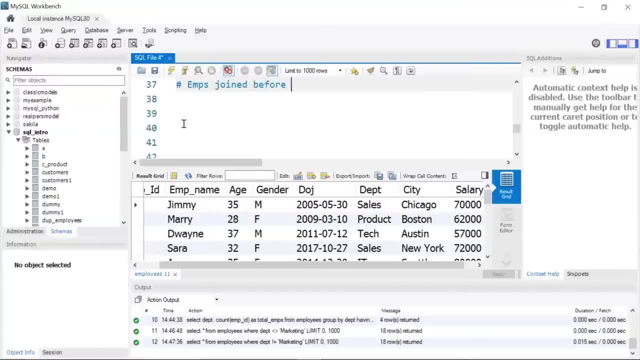 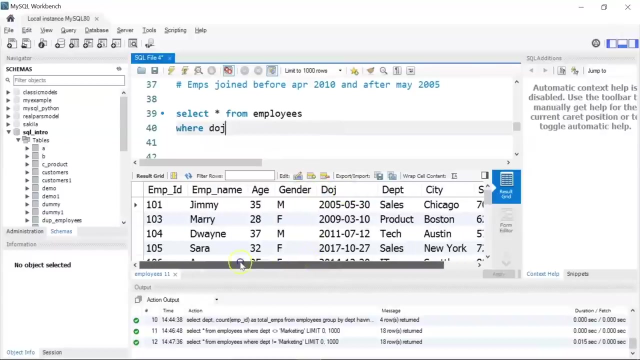 before April 2010 and after May 2005. now let's write our SQL query. so I'll write select star from employees where my date of join. if you see, here I have a column called date of join which has the details about the day on which the employee had joined the company. so I'm 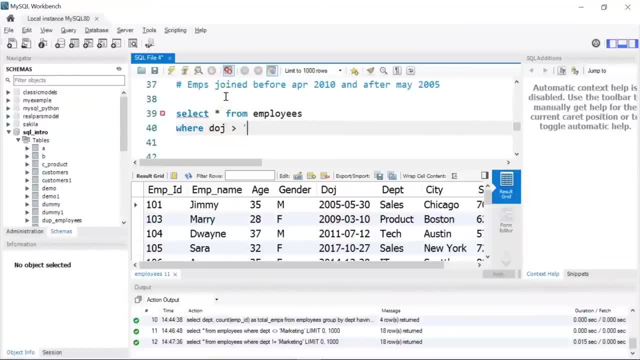 going to write where date of join is greater than 31st of May 2005, so I'll write 2005. this is one of the formats to use date values. so this is the year value, this is the month value and this is the day value and my date. 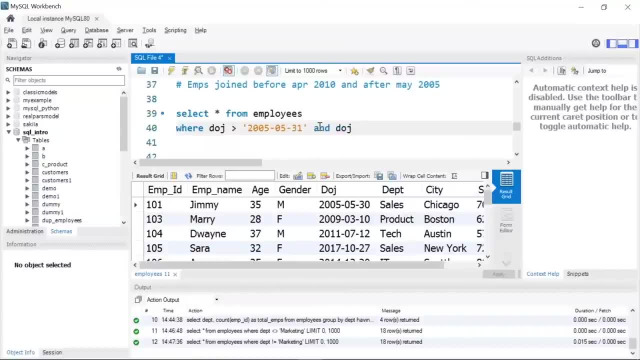 of join should be less than 31st of March 2010, so I'll write 2010, March 31st. I hope you were able to understand this. understand this date of join. greater than 31st of may 2005 means after may 2005 and date of join. 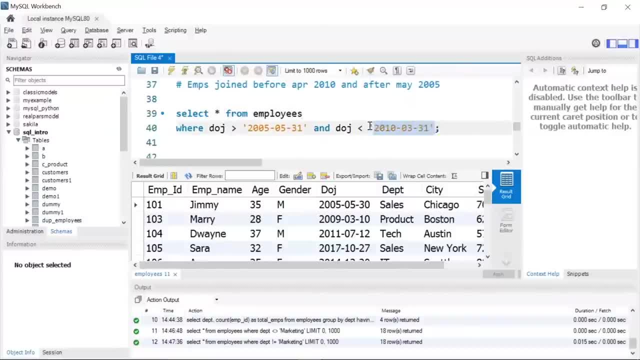 less than 31st of march 2010. this means employees joined before 2010- april. let's run it okay. so we have total three employees in our table. you can see the date of join and all of them have joined after may 2005 and before april 2010. okay, now moving ahead to the 11th question. 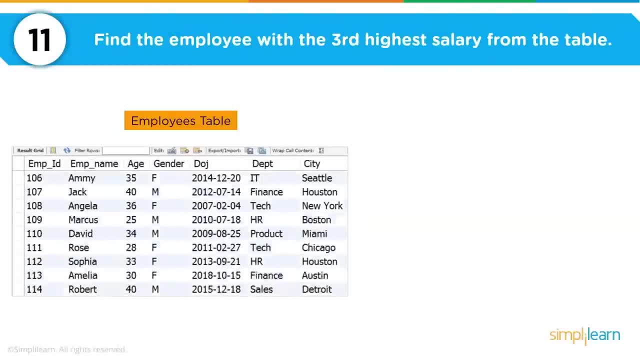 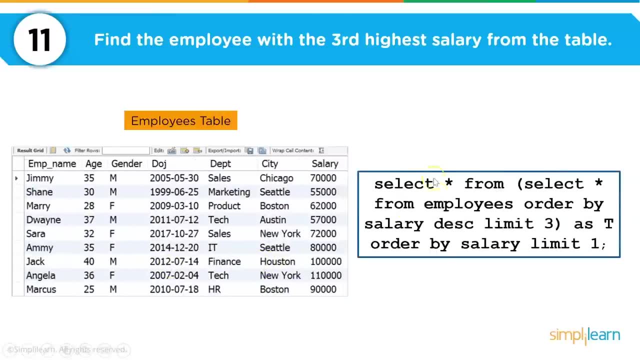 so here we want to find the employee with the third highest salary from the table. so i have my employees table here and my command would look something like this: so here we want to find the employee with the third highest salary from the table. we are going to explore how to write sub queries in SQL, so I'm using a sub query. 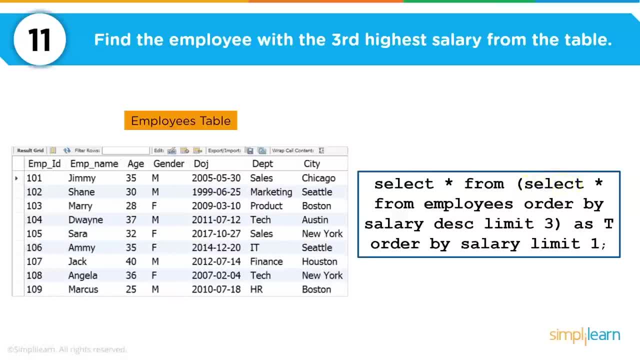 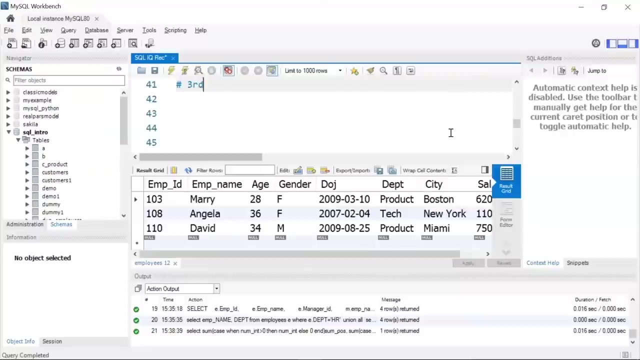 here where I am trying to find the employees who have the top three salaries, or the top three employees who have the highest salaries, and from that I am going to filter out my third highest salary employee. so let's do it on our workbench, okay, so I'll come down and let me give a comment as third. 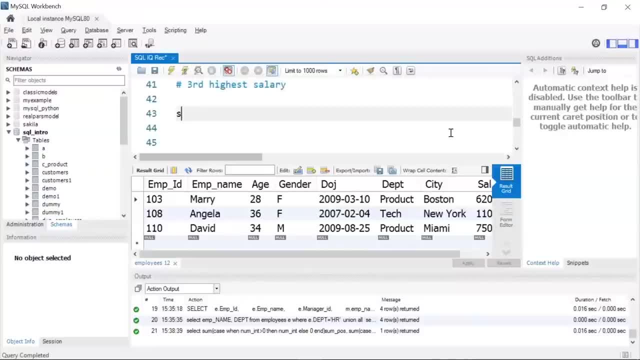 highest salary. okay, so let me first write down my SQL query and then I'll explain. so I'll write select star from. after that I'll start a bracket and write my inner query. so I'll write select star from employees order by salary descending. then I'll use my limit keyword and I'll write. 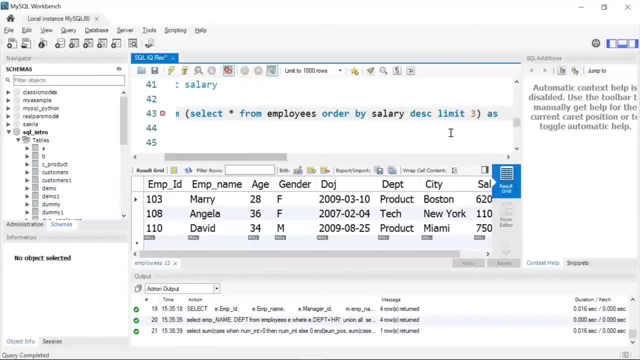 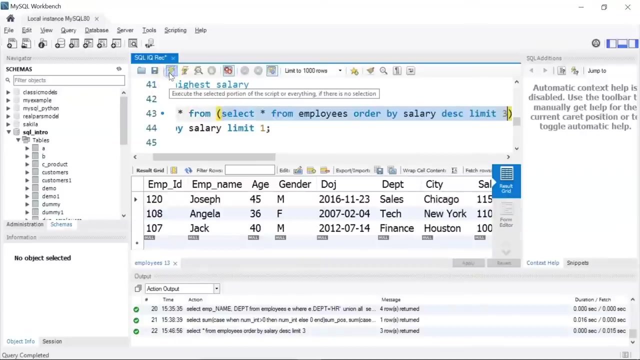 limit three, as I'll give an alias name, let's say T, and then I am again going to use my order by salary. limit one. okay, now let me explain you the flow. so first let me run the inner query. I'll select my inner query and I'll run it, so the inner query returns my top three. 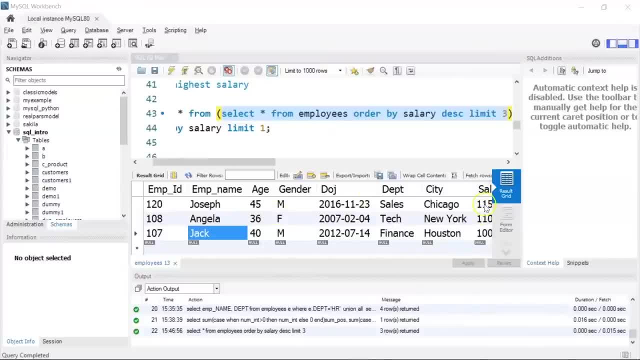 employees who have the highest salary, and this is ordered in descending order. since I used salary descending, now let me just use this. okay, now you can see it clearly. so these are my top three employees who have the highest salary. so Joseph has the maximum salary, followed by Angela, and then we have Jack. now from 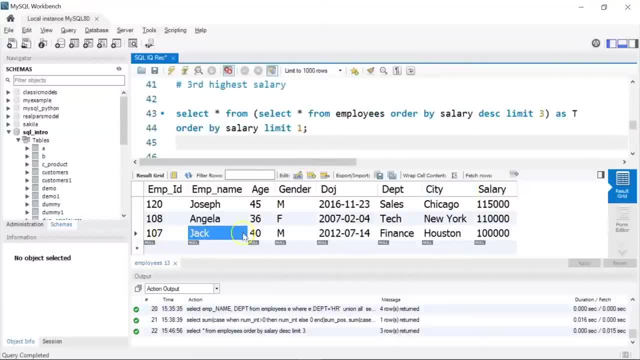 this. I want to return only the record for Jack, because Jack is the employee who earns the third highest salary. so for that I am going to use the result returned by my sub query or the inner query, and on top of this I'm going to order the salary and say limit equal to 1. so I'm again ordering this salary in. 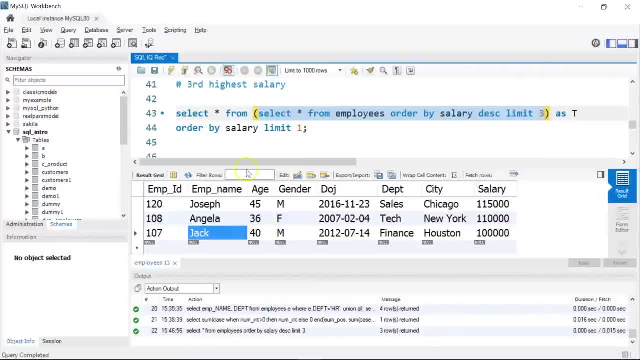 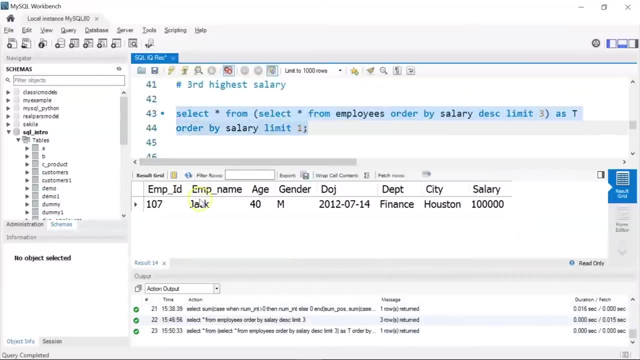 ascending order. so what will happen? Jack will appear at the top, Angela will be at the second place and Joseph will come to the third place and from there I'm using limit 1 so that I can only get the record for Jack. now, if I run the entire query, you see the result. I have my employee name. 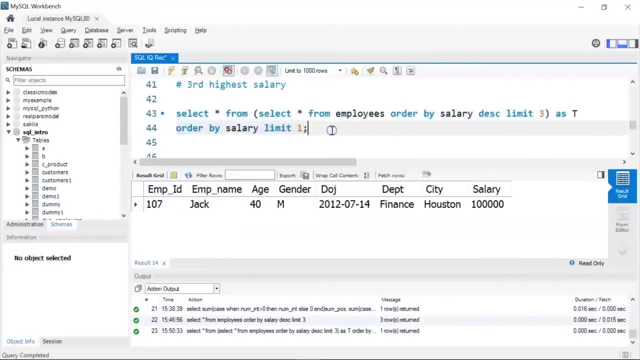 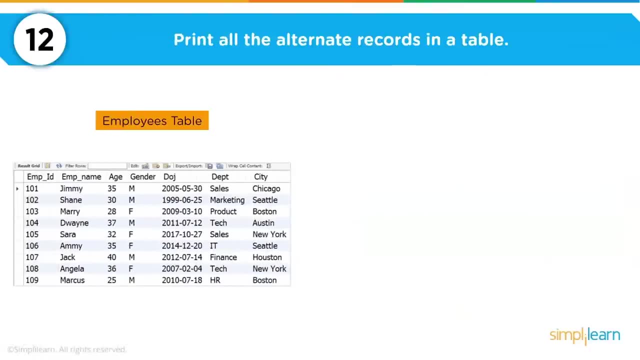 as Jack, who owns the third highest salary. okay, now, moving ahead to the 12th question. the question is to print all the alternate records in a table. so here is my employees table and from this table I am going to print all the alternate records. for example, I am going to: 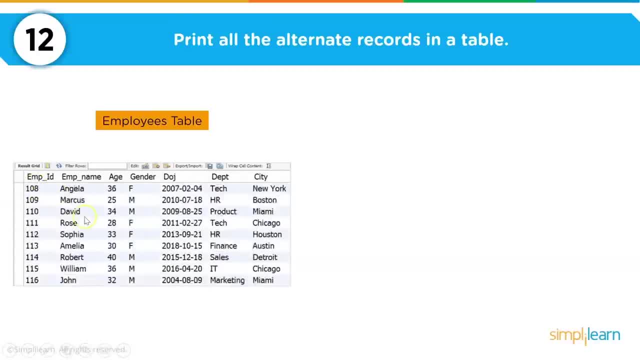 print the my employee ID, 1 0 1. then I am going to skip 1 0 2 and print 1 0 3, followed by 1 0 5, 1 0 7, 1 0 9. so learn the�. 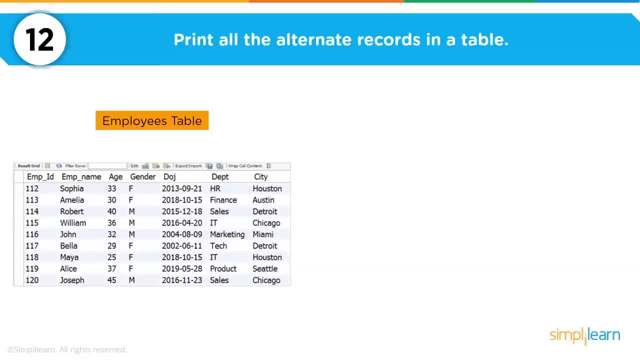 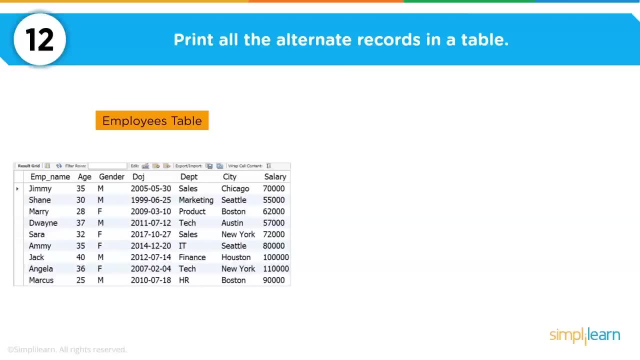 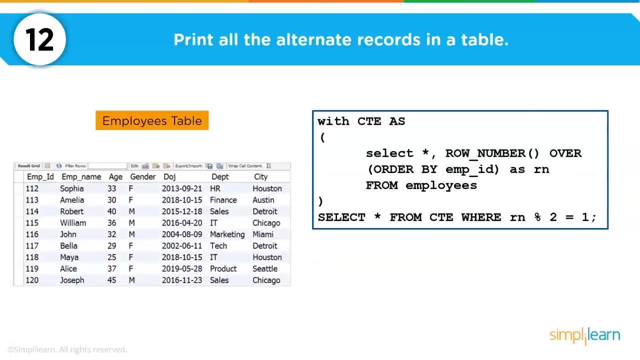 all the employee ids that have an odd value. and you can look at this example in another way of displaying the employees which have an employee id of even numbers, so 102, 104, 106 and so on. now the way to do is either you can use a simple select clause and say employee id percentage, or 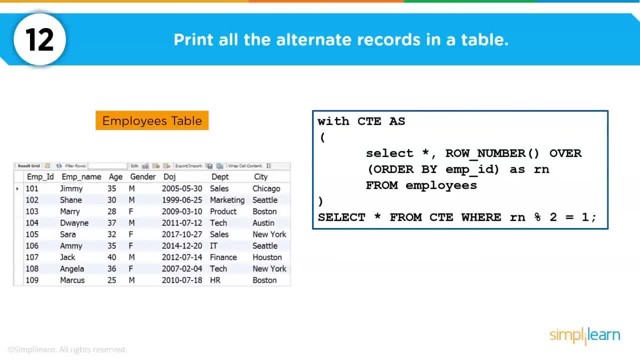 modulus 2 equal to 0, which means i want to filter only those employees which have an even employee id. else, what you can do is you can use a cte, as you can see here. so cte, or the common table expression, is a temporary named result set that you can reference within a select insert. update. 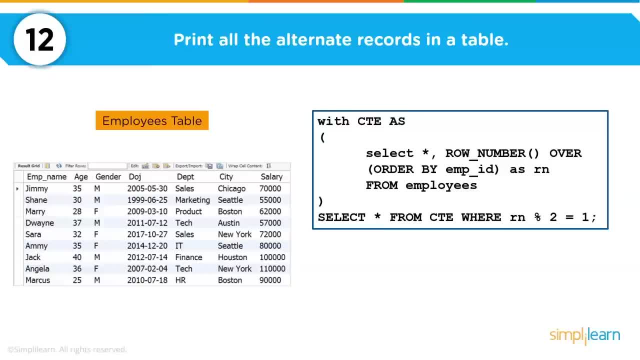 or delete statement. now it is used to simplify complex joints and sub queries and to provide a means to query hierarchical data. now let's write this query on our workbench and see how it works. so before that, let me explain you. i am using a few new functions, such as row number. this will 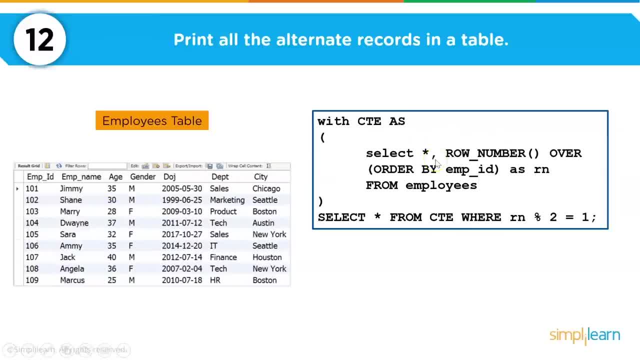 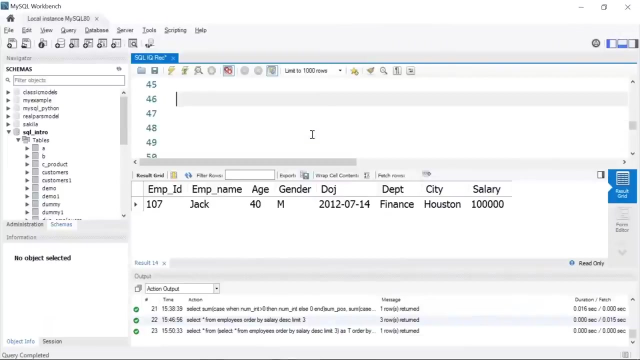 create a row number for each of the rows or the records present in my table, and then from this cte i am going to use my filter clause, or the where clause, where rn, which is row number, percentage, 2 equal to equal to 1, so this will return only the odd records from the table. let's see how to do it okay, so i'll give a. 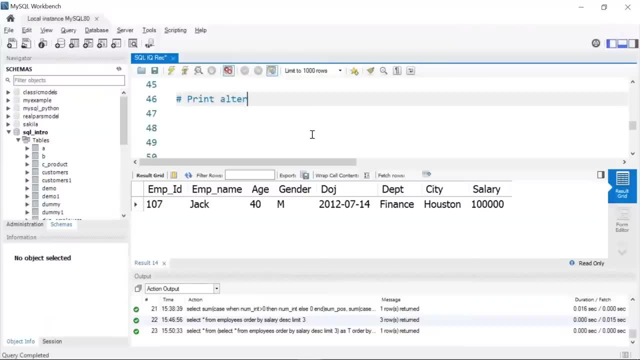 comment print alternate records. okay, now i'll start with my simple query, which is select star from employees where, let's say, i want to find only the even employee ids or the employees who have an even employee id, so i can use employee id percentage 2 equal to 0, so it has to be a perfect division. 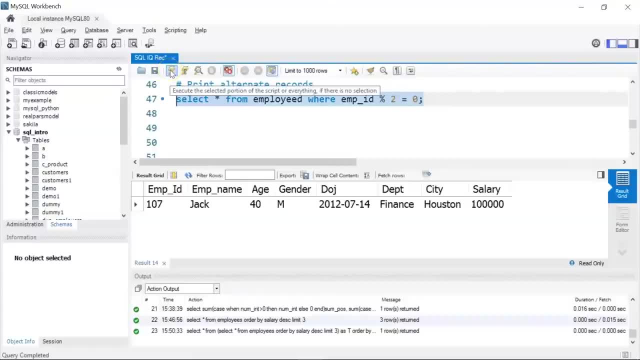 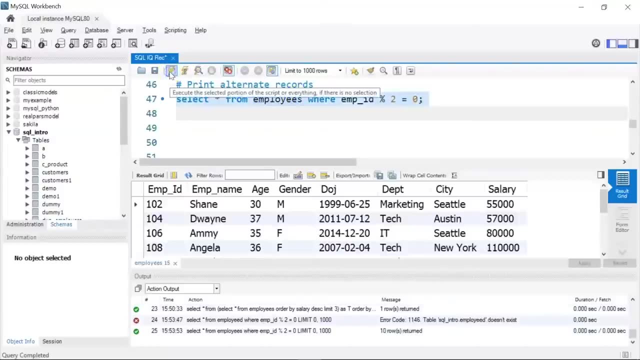 and the result should be 0. only then i can get only the even employees if i run this. okay, there was an error here. it should be employees. i'll run it again. you can see here. i have printed the alternate records in the table and i have printed in print records in the table. give me an. 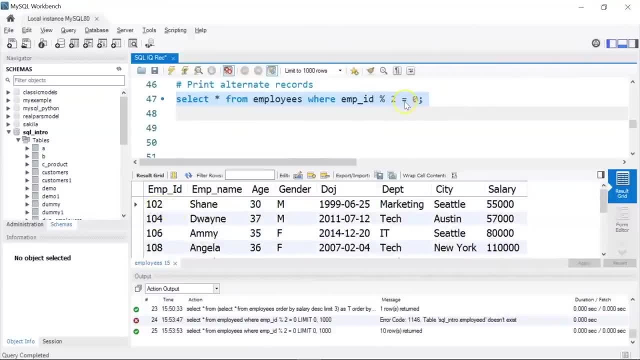 a table. so we have skipped 101 because it is not divisible by 2. i've started with 102, followed by 104, 106, 108 and then finally we have 120 or 120.. now if you want to print only the odd records in the table, you can use employee id percentage 2 equal to 1. so you can see here: 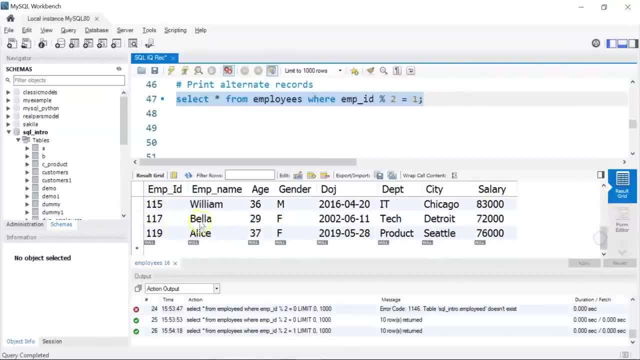 i have 101, 103, 105, 107, up to 119. now the best way to do this is to use a common table expression of cte. so i'll start with my command, that is, with cte. as i'll start with my bracket, i'll write select. 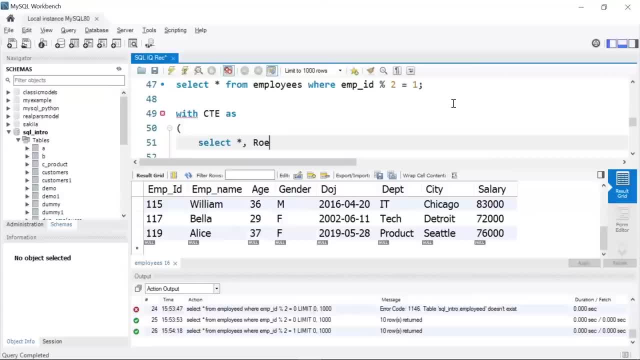 star comma, then i'm going to use my row number function. i'll write row number, then i'll write over, then i'll use order by employee id. so this row number for each of the rows is going to be created over my employee id column and that is sorted in ascending order. i'll give an alias as rn, which stands for row number from. 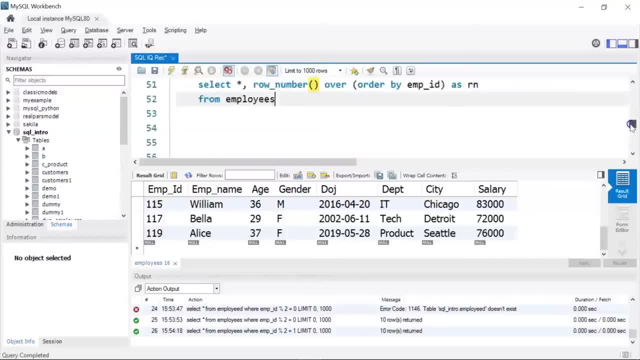 my table, that is employees. i'll scroll down and then i'm going to close my bracket. i'll write select- let me remove the space here. okay, i'll add select star from cte, where my row number percentage 2 equal to 1.. now let's see this from the top. so i have my 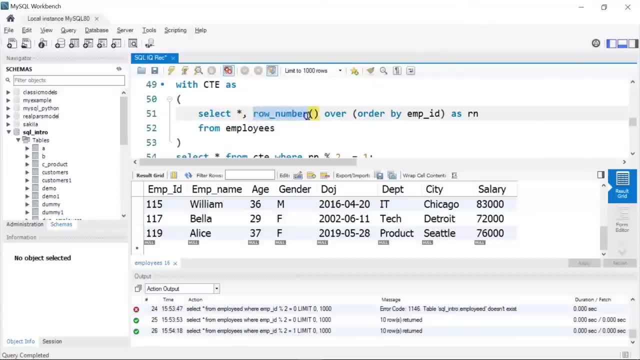 common table expression where i am going to create a row number column named as rn and this row number column is based on my employee id column, which is sorted in ascending order, and from that i'm going to filter only those row number values that are not divisible by 2, or i'm going to print only the 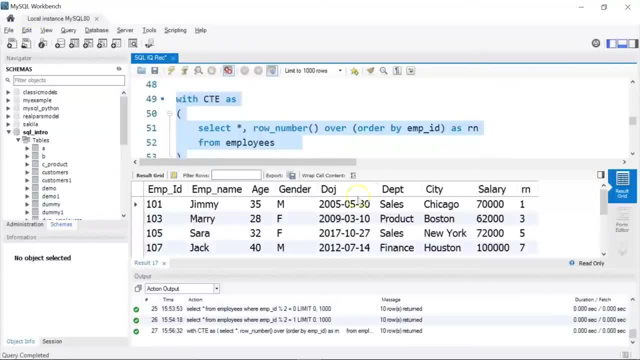 odd records from the table. so let's run it and see the results. there you go. so here, if you mark, i have my row number column created and i am filtering only the odd records in the table. so it starts with 1, 3, 5, 7 and goes up to 19.. and similarly, here you can see the employee ids: the name, the age, gender. 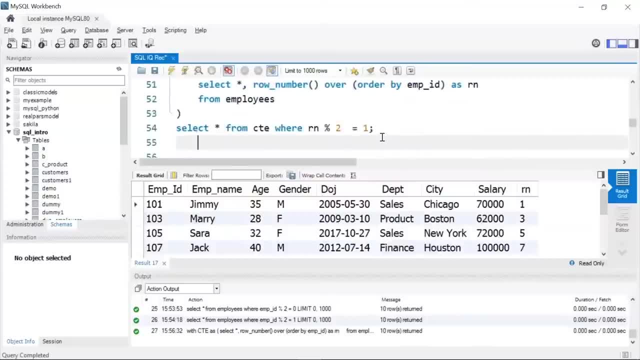 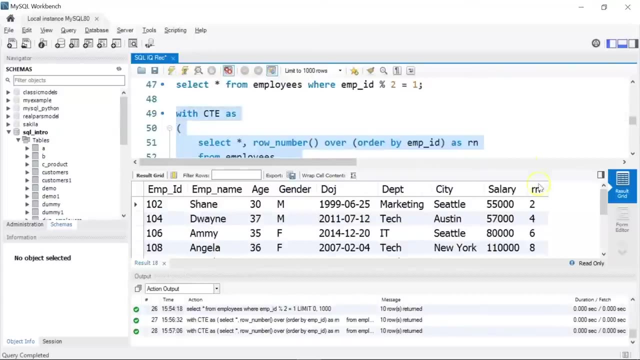 and other information. now, if you were to print the even records in the table, the alternate even records, you can use rn percentage 2 equal to 0.. let's see the difference. i'll run this. there you go. so i have my even row number, starting from 2, which goes up to 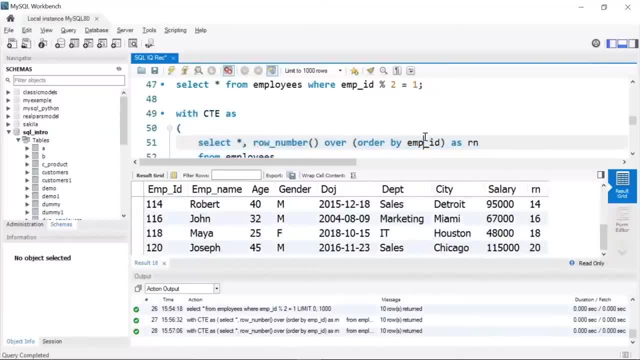 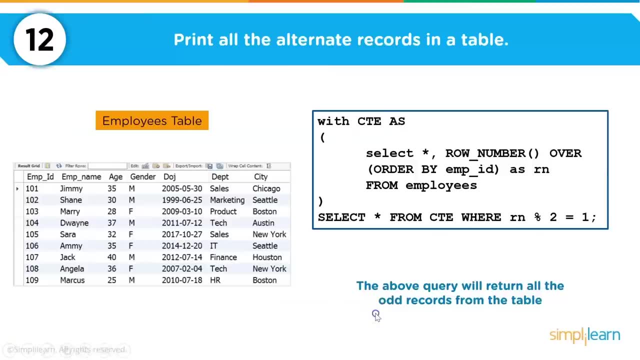 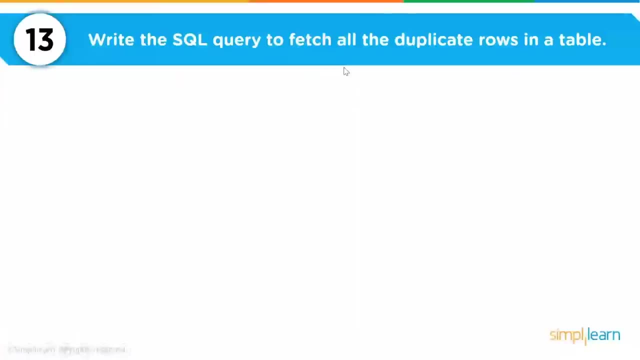 20.. okay, so this is how you can print alternate records in a table. now moving the next question. now, in the 13th question, we want to write an SQL query to fetch all the duplicate rows in a table. now this is another crucial interview question that is often asked in most. 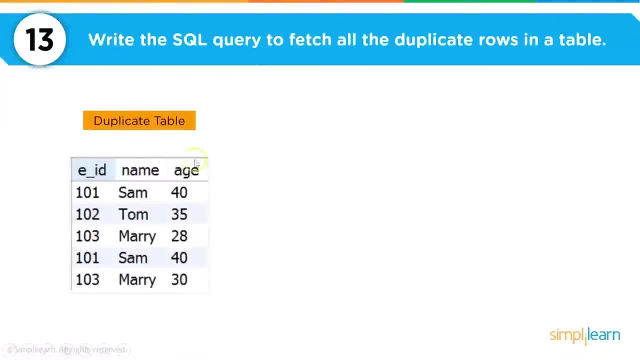 of the interviews. now I have a table which is named as duplicate table and here you can see I have some employee id name and age and a few records are duplicated. for example 101, sam 40. the first record is duplicated and you can see here it has the same values. now if you mark 103. 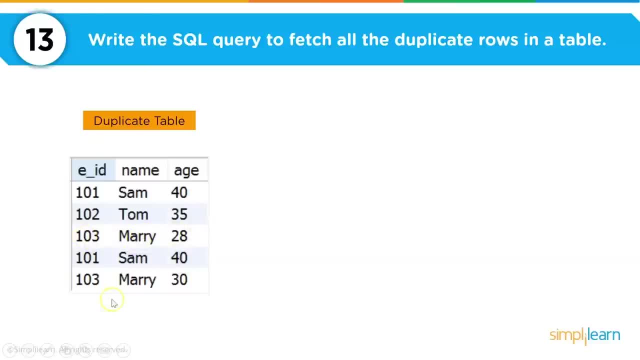 Mary and 28 is not duplicated because here the age is different, so this is a different person than compared to the third name that you have. so this is how you can find the duplicate rows in a table. so I am going to select my employee id name and age and a few records are duplicated and you can see here it has the same values. 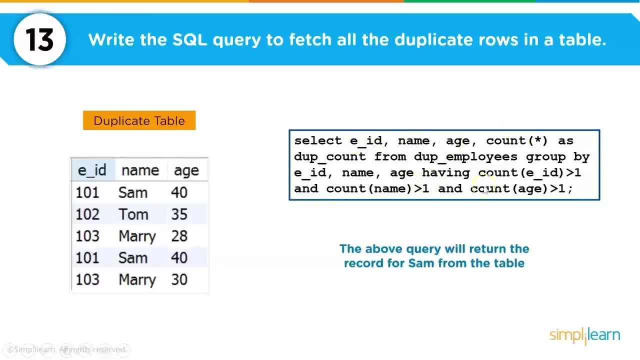 name and age and then count all the employee ids- the names and each, and compare them with whether they are greater than 1 or not. so if they are greater than 1, then I will see that particular record is duplicated or is present more than one time in the table. let's do this. 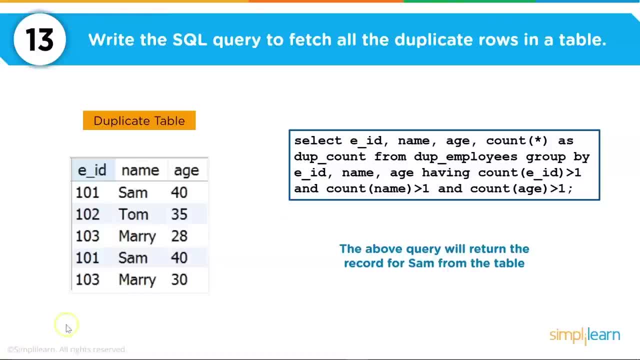 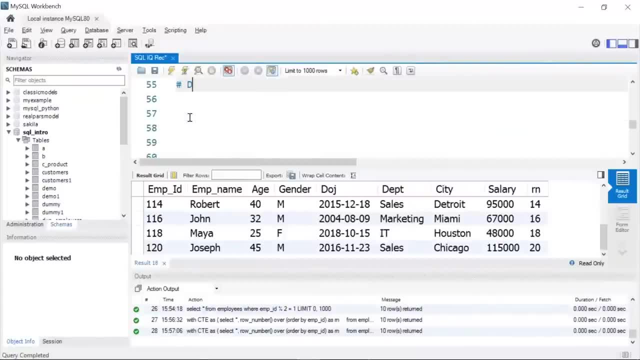 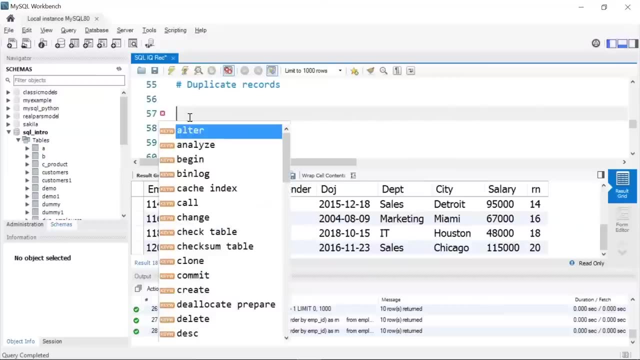 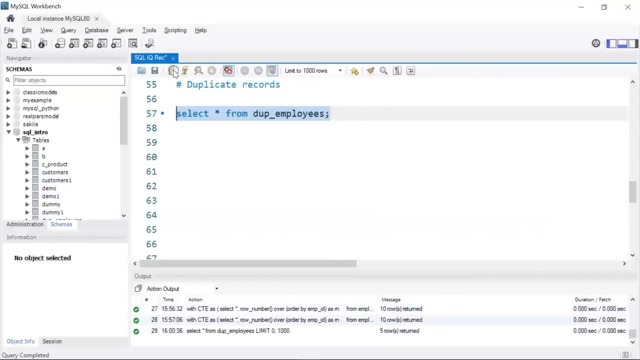 implementation on our workbench. okay, so I'll come down and let me give my comment as duplicate records. okay, so let me first show you the records that are present in my table. so I'll write select star from dup underscore employees. I'll run it. okay, you can see here I have my table that we saw in the slides. so employee id 101 with name sam and. 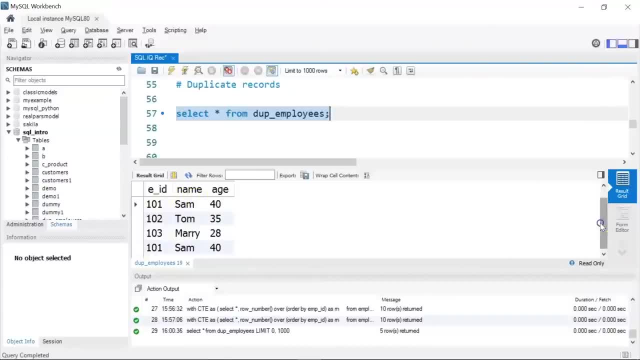 age 40 is duplicated, so we want to find this duplicate record. the way to do is I'll write select e underscore id, which is employee id comma, name comma, age comma. I'm going to count all of the records and I'm going to count all of the records and I'm going to count all of the records. 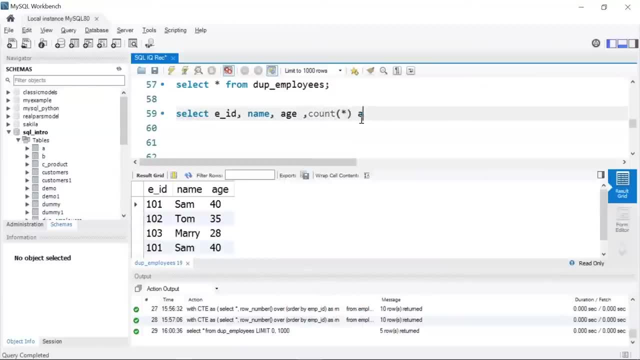 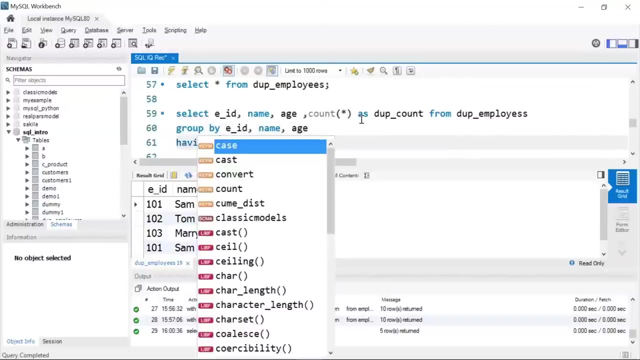 them. so I'll write count star as duplicate count. this is my alias name from my table. that is dup underscore employees. I'll say group by employee id, name and age, and then I'm going to use my having clause saying having count off employee id is greater than 1 and count off name should also be greater. 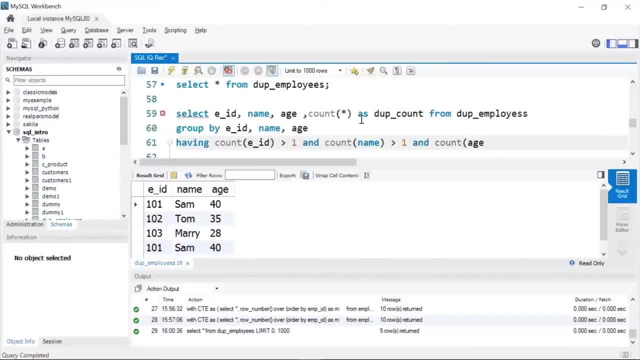 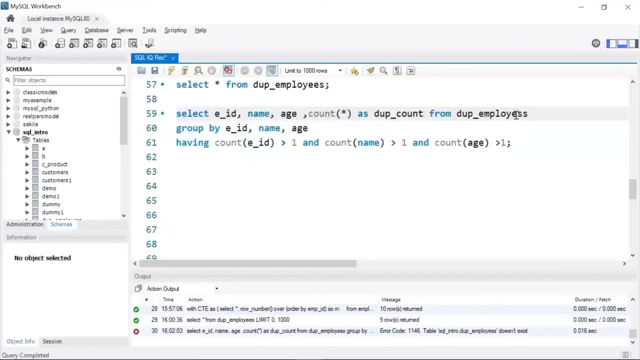 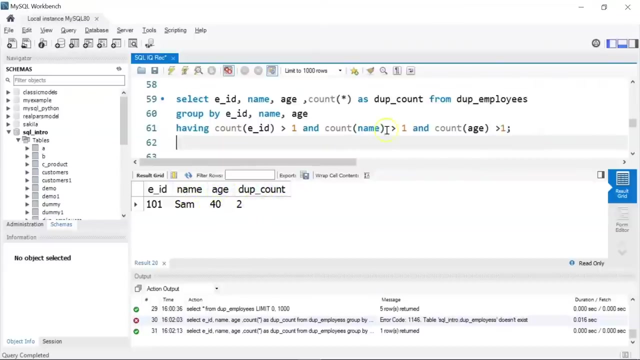 than 1 and my count off each should also be greater than 1. let's run it and see the results. okay, there is some error here. the name of the table should be employees. okay, let's run again. we have our correct result. that is employee ID 101 with name Sam and age 40 is duplicated, so the value is 2. great, now moving. 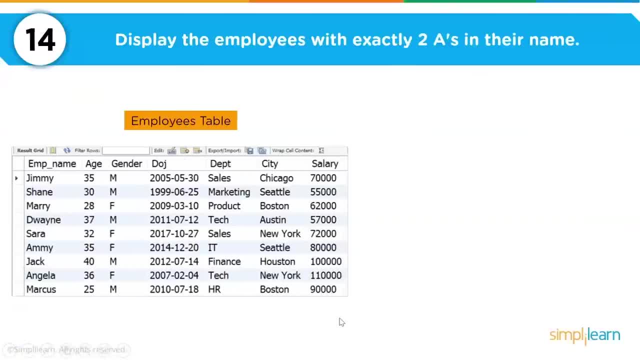 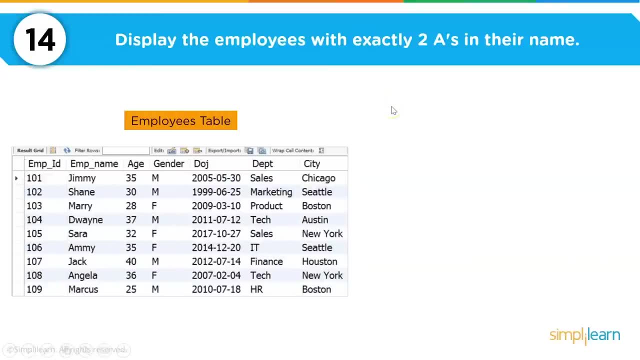 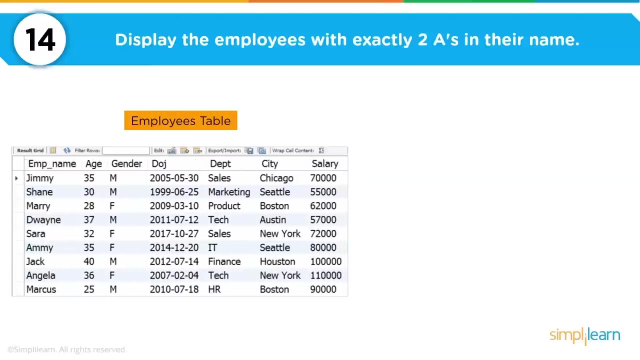 ahead. now. the 14th question is a bit tricky, wherein we want to display the employees with exactly two A's in their name. so you see, here I have my employee names and there are certain employees who have just two A's in their names. so I want to find those employees. only now the 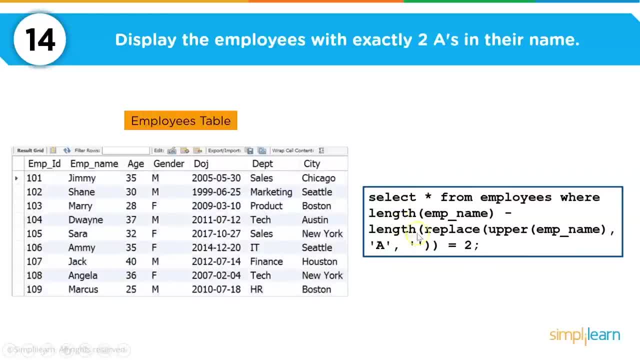 way to do is. it is a bit tricky to understand. I am going to break it down and make you understand. on my mysql workbench, so here you can just have a glance. I write select star from a employees, where I am finding the length of my employee name and then subtracting my length. 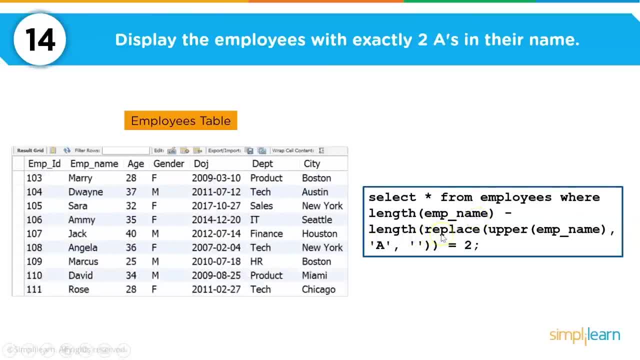 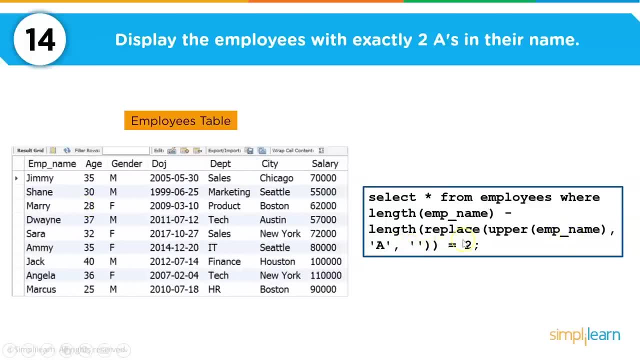 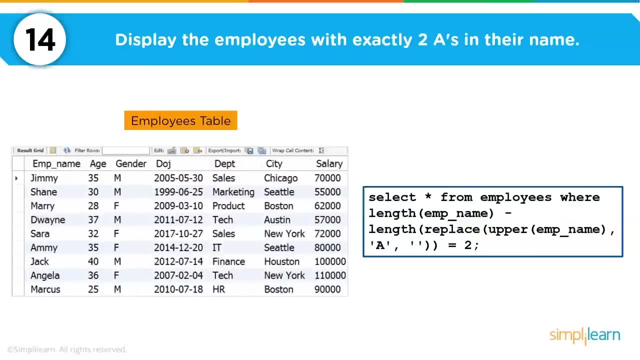 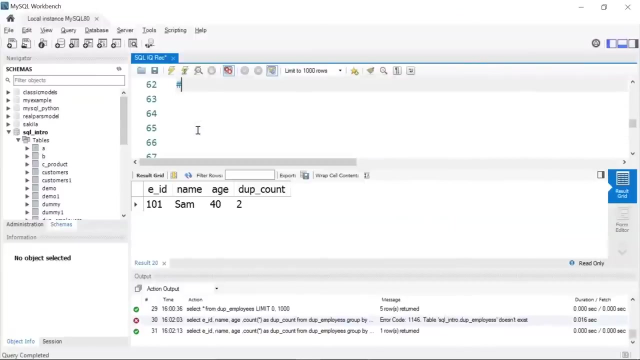 wherein I have replaced my employee name that has a with a blank and this subtraction is equal to 2, then that particular employee has two A's in their names. so let me show this first. let me first give my comment as employees with two E's, okay. so first I'm going to write a select. 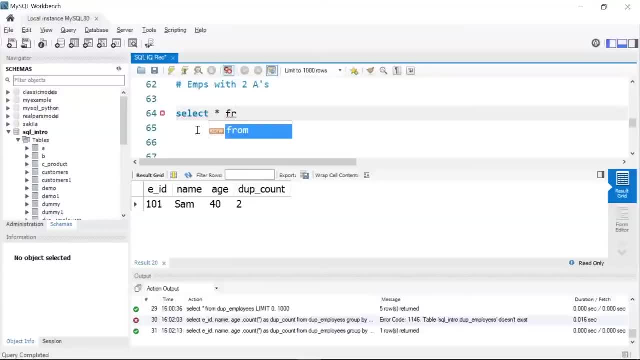 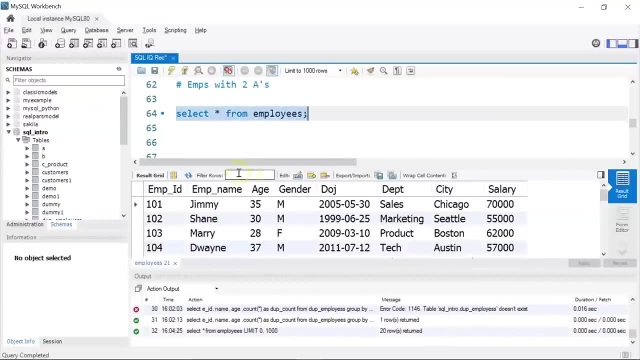 statement. okay, before that, I'll show you the records present in my table. okay, if you see here that we already have ndane and jagg, so I think I have it. this is the only one successfully created. I want to kill you right now, as we gonna use this notion to worry about um. no, 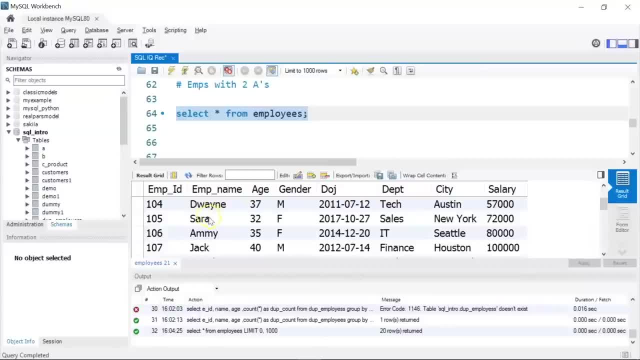 change as a human. so at this particular point, the way we want to categorize the number one is adaptable. so I'm just gonna use add a and add third hair, which essentially is just the least right. as you know, not too big of a big living thing, a little bit bigger so that it. 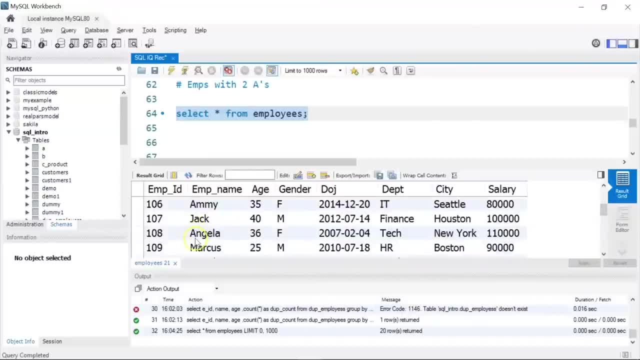 keeps it in a place which may or may not be recommendable. it's cute like this. I'm just going to refit, don't you know what I was implying? okay, so, for instance, we want to abstract if the employees have two a's in their name and similarly, if i scroll down, let me check if we have. 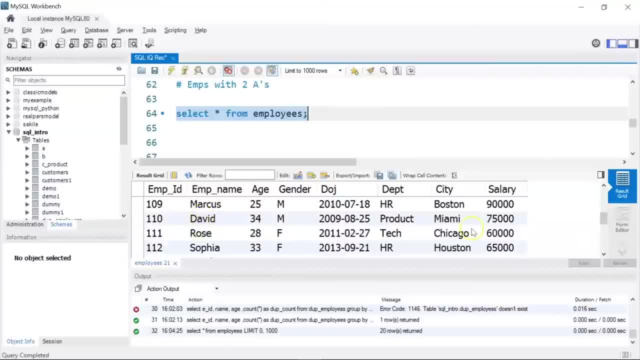 any other employee with two a's in their name. marcus has one, david has one, sophia has one, we also have amelia that has two a's in its name or in her name, and we also have maya. okay, now let me go ahead and write a sql query, and then i'll explain you what i'm trying to do. 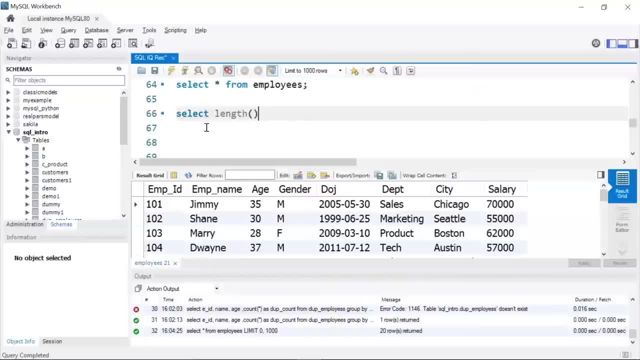 i'll write select, i'm using the length function and in the length function i'm going to replace. then i'll use another function called upper. on top of employee name i'll write a and then replace it with a blank. so i'm using quotations to represent blank from employees. 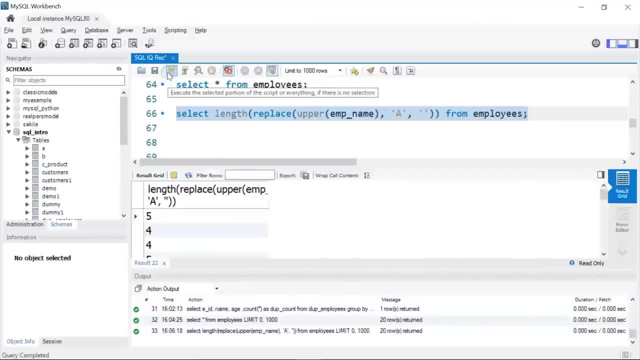 okay, let's run this and see the results. you see, here it has given us the length of the employee strings after replacing all the a's with a blank. so here i'm essentially converting my employee names to uppercase and i'm changing. wherever there is an a, i'm replacing that a with a blank and then i'm 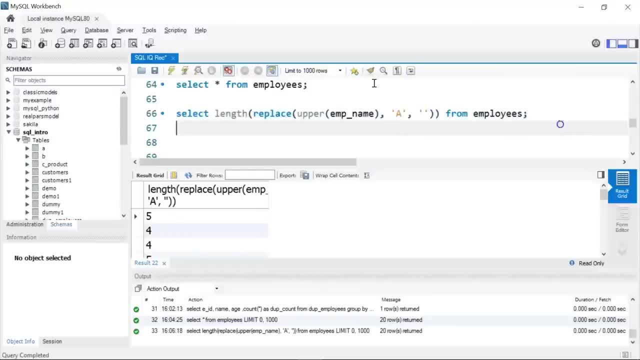 finding the length. so this trick i'm going to use in my final query. so i'll write select star from employees where what i'm going to do is i'll bring this to the next line. i'll write length of employee name minus. then i'm going to use my above condition. 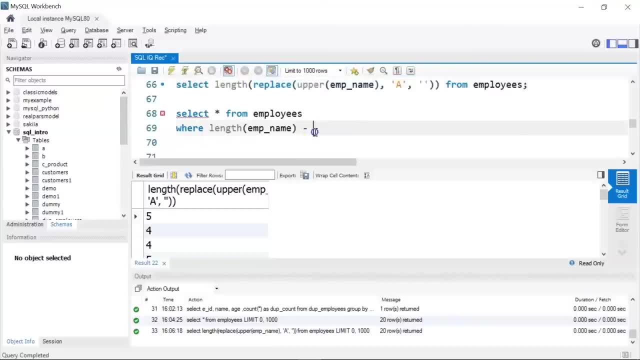 i'll copy this, i'll paste it here, and this value should be two. so what i'm doing is i am first finding out the length of my employee name, from that i'm subtracting the length after replacing the a's present in the employee name with a blank, and this value should be equal. 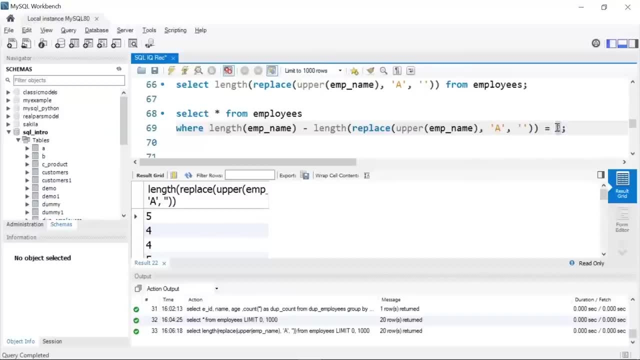 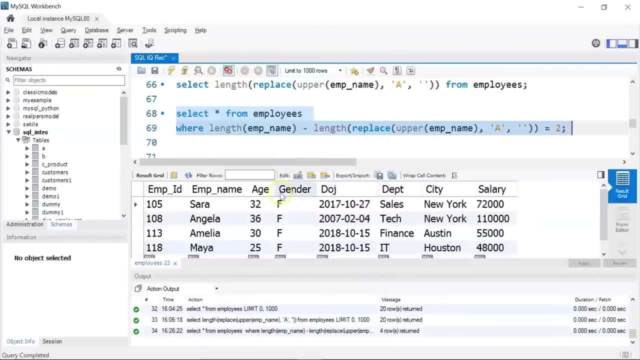 to two, the reason being we are only trying to find the employees who have two a's in their name. let's run and see the results. okay, if you see, here we have sarah, angela, emilia and maya, who have two ways in their name. so we have sarah that has two a. 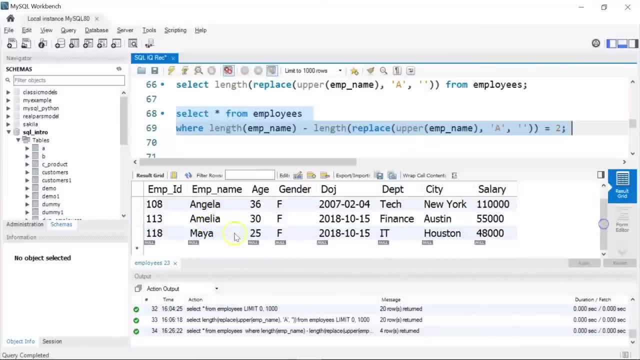 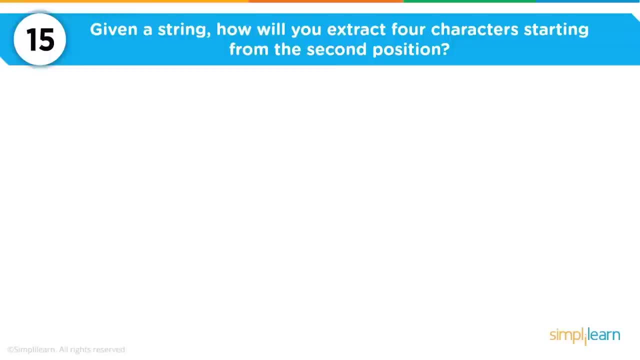 angela has two way, amelia has two ways and then maya also has two. a. okay, now moving ahead. now the 15th question is: given a string. will you extract four characters, starting from the second position. so i have my string here which says michael balak of michael balak, you must be aware, is a popular footballer. he is from. 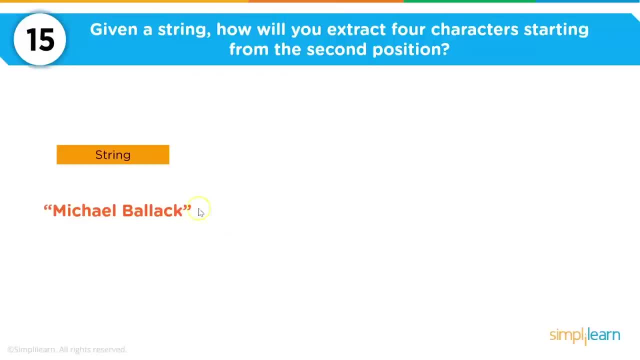 germany and also was the captain of germany. so from the string michael balak, i am going to extract four characters, starting from the second position. you can use two inbuilt mysql functions to do this. the first is called substr, wherein we pass in the string, then we give the position. 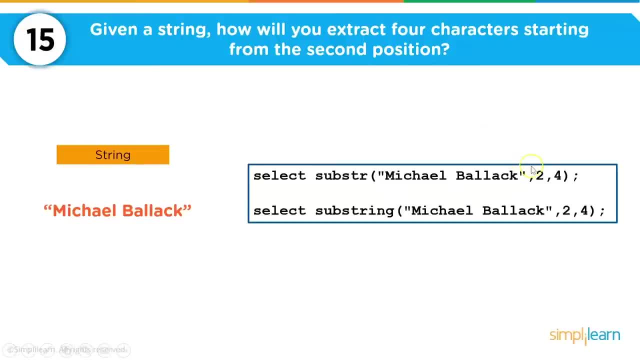 from where we want to extract the characters. so here i am going to extract from the second position. so hence two, and then the number of characters that you want to extract, which is four. the other way is to use the substring function, which is again similar to the substr function. 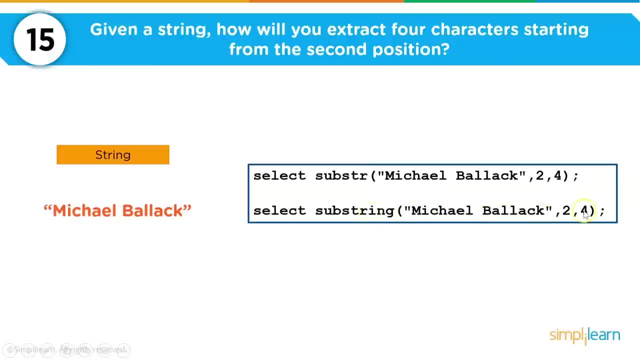 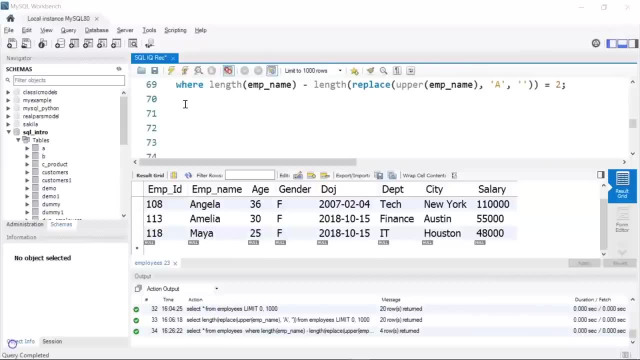 in the substring function also, i am first passing in my string and then giving my starting position, which is two, and then i want to extract four characters from it. let's do it, i'll give a comment: extract strings. so here i'm going to write select. first i'm going to use substr, which is my inbuilt function. 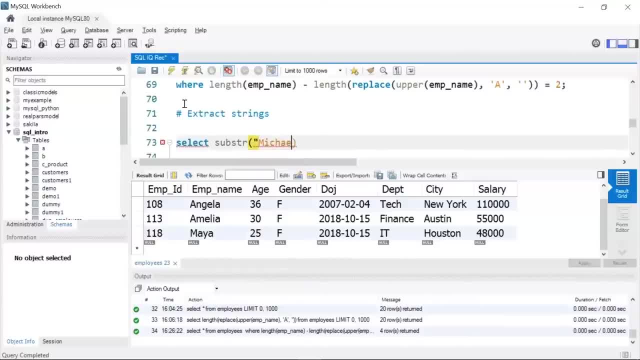 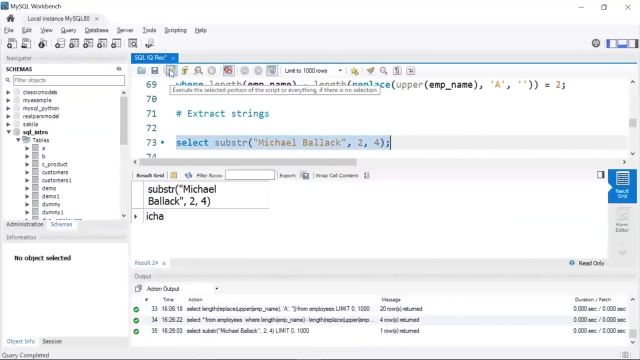 i'm going to pass in my input string which says michael balak, and then i'll give my starting position, which is two, and then the number of characters, that is four. let's run it and see the results. you can see here. it has given us icha. so if you see, 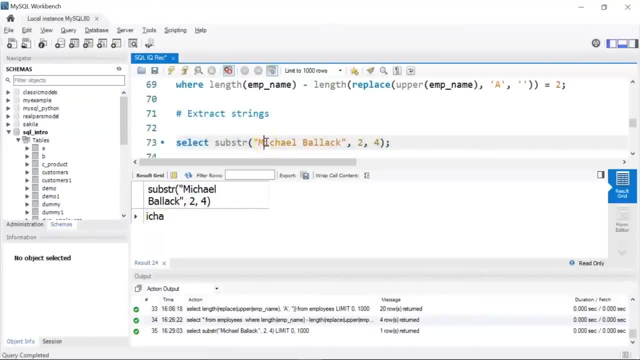 m is at the first position. from the second position onwards, i needed four characters, so m, c, h and e. these are the four characters starting from the second position. similarly, let me just copy this and instead of sub str i'm going to use the substring function. i'll write just: 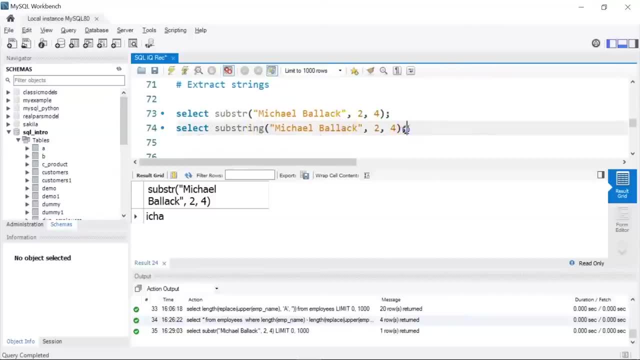 ing that becomes substring. let's select and run it and this also returns the same result. suppose you wanted to extract from the fourth position. you wanted to extract, let's say, three characters. let's see the results. it gives us h, a and e, if you see here. 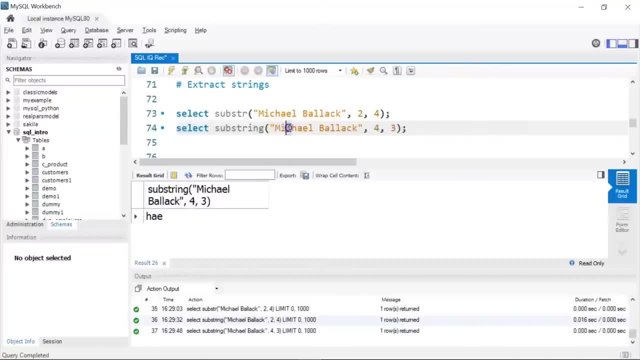 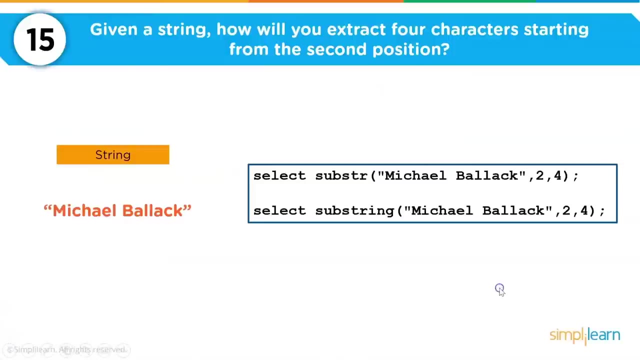 m is the first position, i is at the second position, c is at the third position. h starts from the fourth position. so h, a and e are the next three characters starting from the fourth position. so hence, this is the result. all right now, moving ahead now. my 16th question is on: 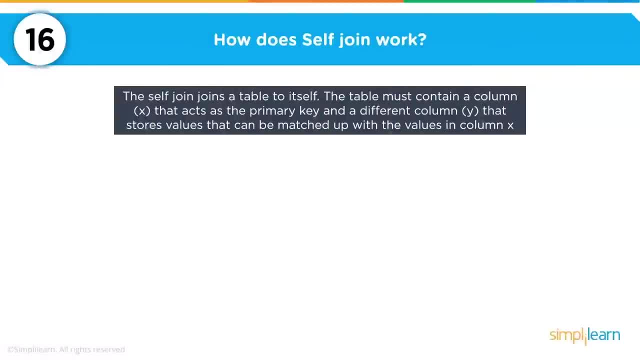 how does self join work? so self join joins the table to itself. so the table must contain a column x that acts as the primary key and a different column, let's say y, that stores values that can be matched up with the values in column x. now this might not be. 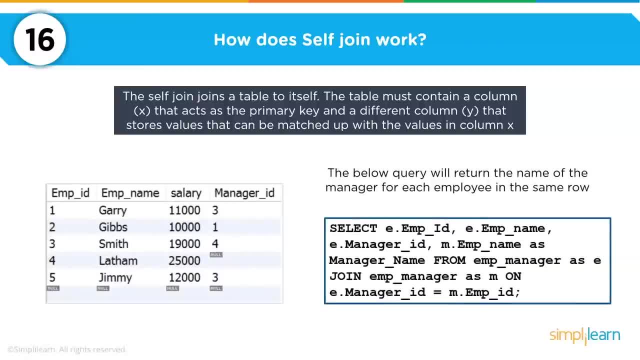 really easy to understand. you'll get to know once we do this demo. so i have a table which is called employee manager. so this is my table. let me tell you how to interpret this table. we have five different employees, starting from employee ID 1 to employee ID 5: Gary Gibbs, Smith, Latham and Jimmy. 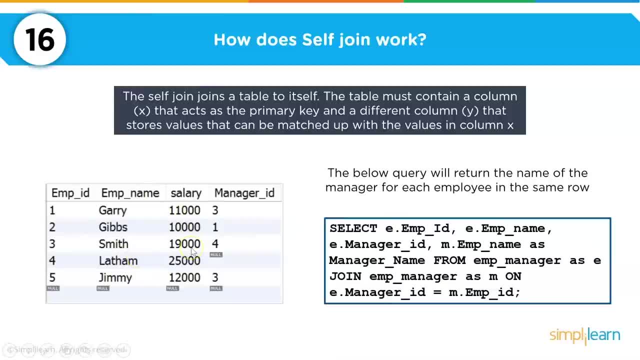 are the different employees we have. you have their salaries and now you have the employees reporting to which manager. if you see here, Gary's manager ID is 3, so if you see a table at 3, we have Smith. so Gary is reporting to 3, or in other words, 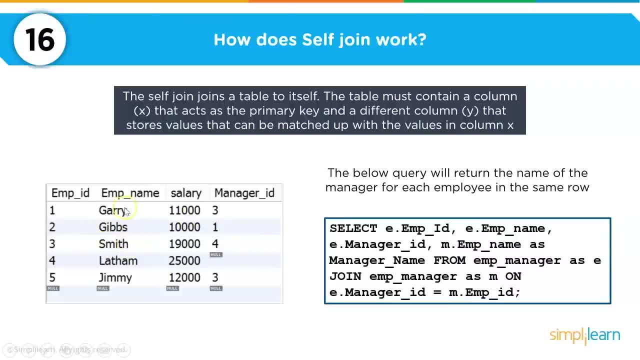 Smith has a employee under him who is Gary. similarly, Gibbs is reporting to manager ID 1 or employee ID 1, which is Gary, so Gibbs manager is Gary. similarly, if you see for Smith, Smith is reporting to the person with manager ID 4 or employee ID 4. we have Latham, so Latham has one employee under him who is Smith. 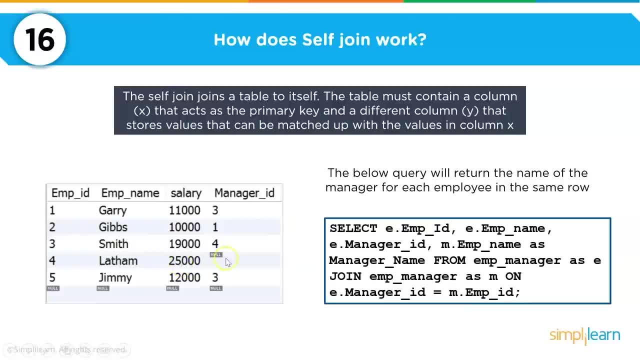 okay, Now Latham, in our table, has no managers. Then we have Jimmy, who is reporting to the employee ID 3, who is Smith. Okay, Now I want to use this table and return the name of the manager for each employee. To do that, I am going to use my self join. 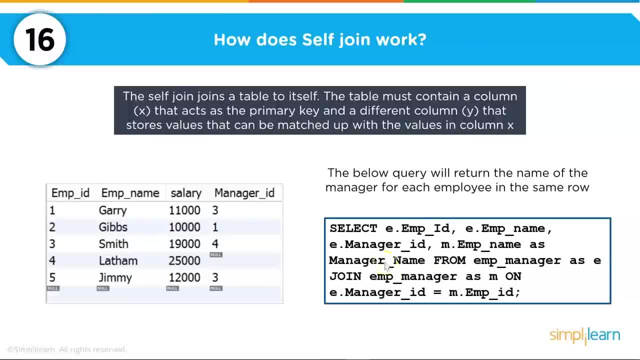 So here I am using a self join to join both the tables Here. both the tables mean I am using the same table twice. So I have written select eemployee ID, eemployee name, Then we have emanager ID, Then I am using another alias for managers, So memployee name as manager. underscore name from employee underscore: manager as e. 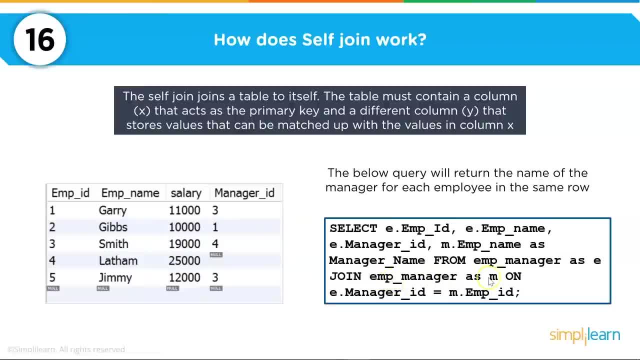 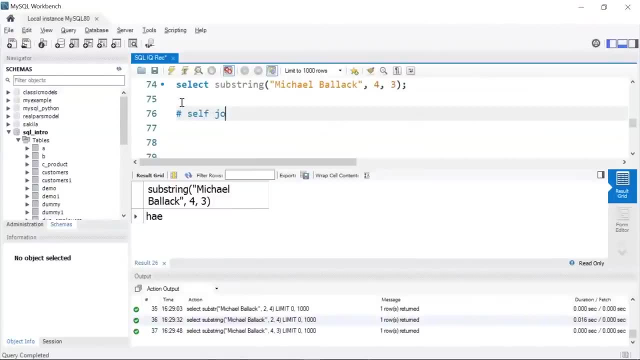 This join means self join. employee underscore: manager as m on emanager ID equal to eemployee ID. So this is my common column. that is employee ID or manager ID. Let's do it All right. I'll give a comment here saying self join and I'll start with my self join. I'll write select. Let me first display my table. I'll write select, star from, and my table name is emp. underscore. 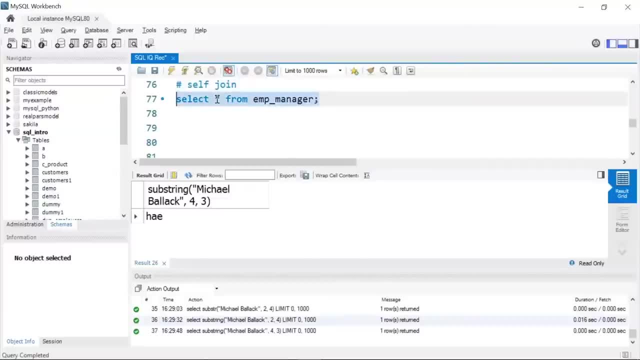 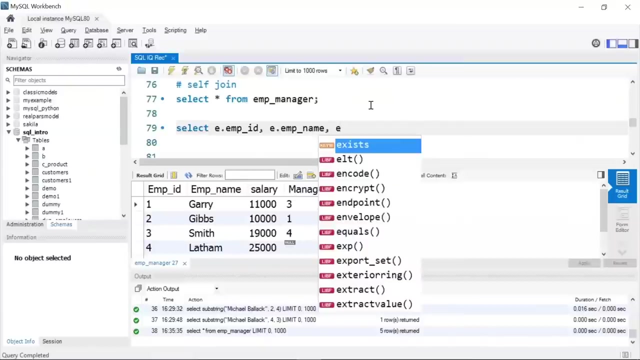 manager. I'll run it. You can see the table here. This is the same table that we saw in the slides. Now I'll write my join query. I'll write select eemployee ID. eemployee name, emanager ID- comma. Then I'm using another alias as m for finding the manager name. So memployee name as manager name. There shouldn't be any space in the alias name. Then I'll write from. 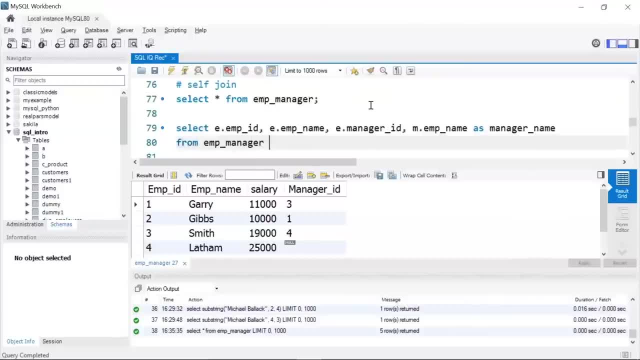 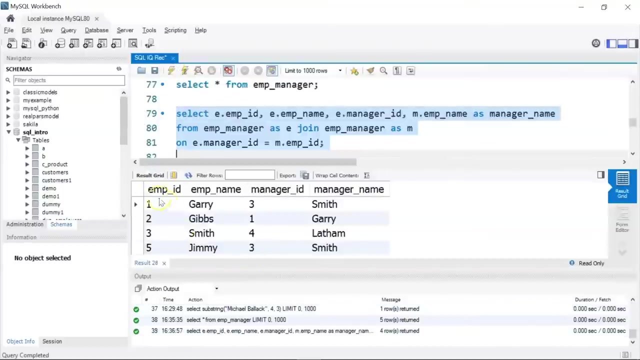 emp underscore: Teacher as E. join EMP underscore manager as M. on E dot manager underscore ID equal to M dot EMP underscore ID. let me run this and we'll see the results. there you go. so Gary reports to the manager ID 3. so from the table 3 is for Smith. so Gary's manager is Smith. Gibbs manager is Gary. 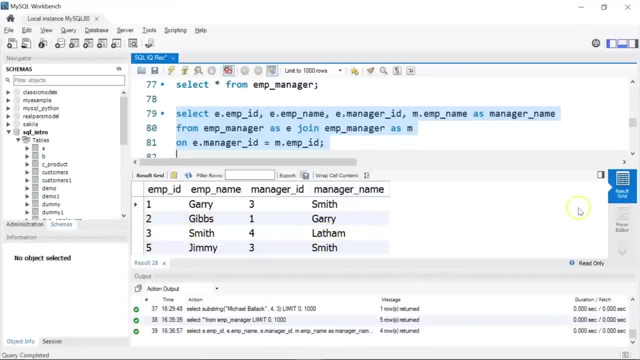 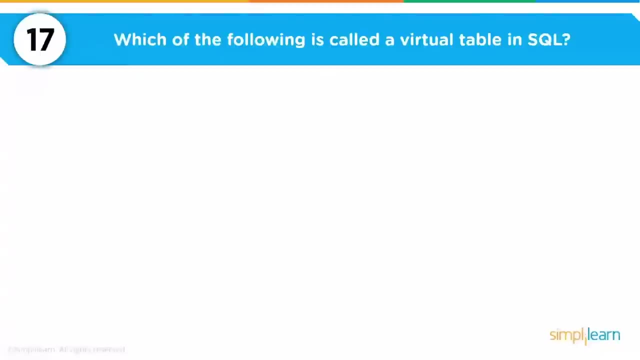 Smith's manager is Latham and Jimmy's manager is Smith. okay, so this is how you can use self join now, moving ahead with our next question. so the 17th question is on which of the following is called a virtual table in SQL? so again we have a multiple choice question, so the answer is view. you can see here. so view is. 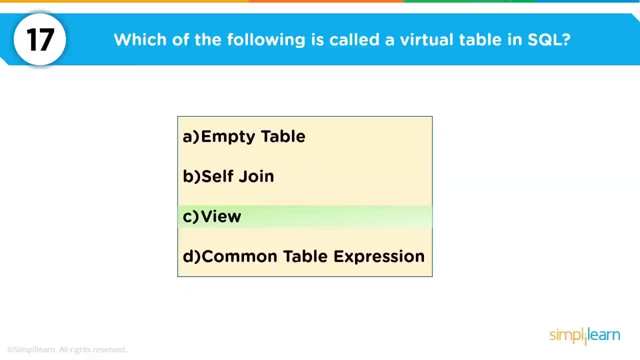 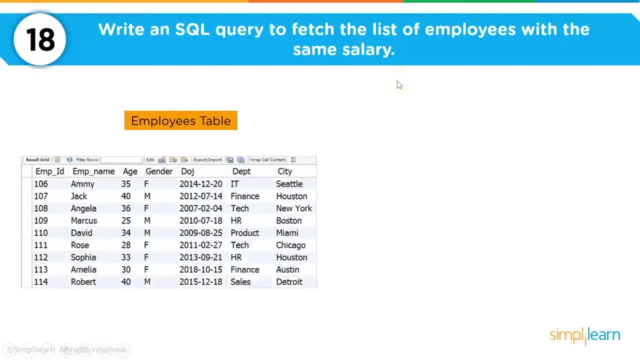 a virtual table that has rows and columns as they are in a real table in the database. now we can create a view by selecting fields from one or more tables present in the database. you next moving to the 18th question. so here we want to write an SQL query to fetch the list of 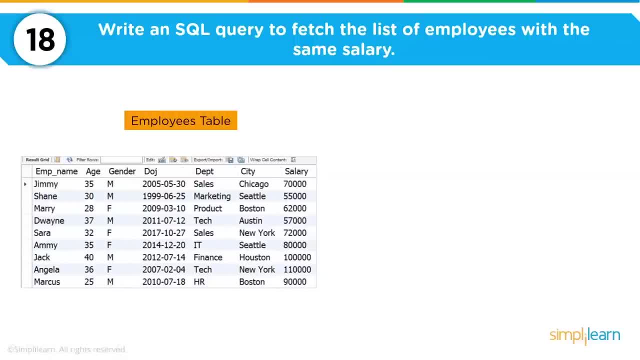 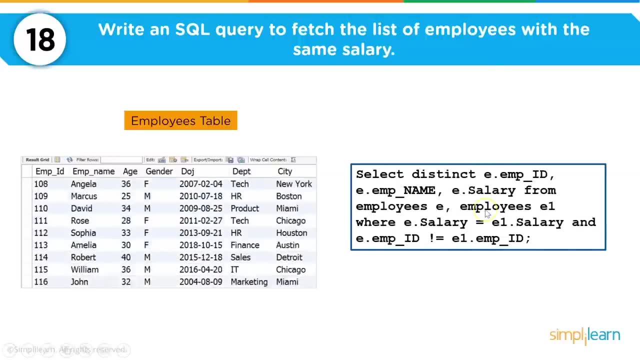 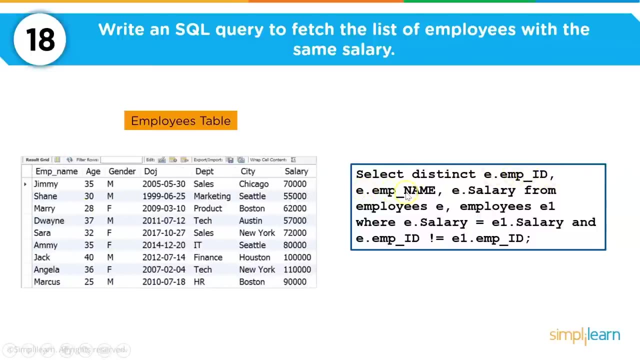 employees with the same salary. again, I am going to use a self join here wherein I'll join the same employees table, and this is how my query would look like. so I am selecting distinct employee ID, so E dot employee ID, E dot employee name, E dot salary from employees, then I'm joining. 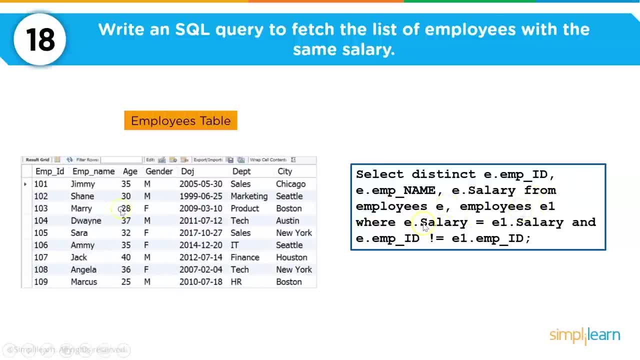 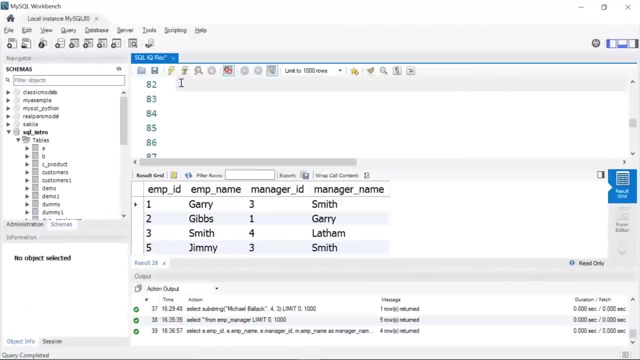 E on E one where e dot salary equal to E one dot salary. because I want to fetch the list of employees the same salary and I'm ensuring that the employee IDs from both the tables are different. Let's do it. I'll give a comment here and write employees with same salary and I'll start with my query. 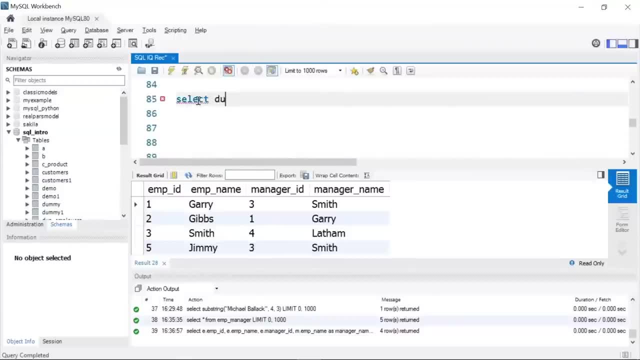 I'll write select distinct E dot employee ID comma. I'll write E dot employee name comma. E dot salary from employees as E, Then employees as E1, where E dot salary equal to E1 dot salary and E dot employee ID is not equal to E1 dot employee ID. 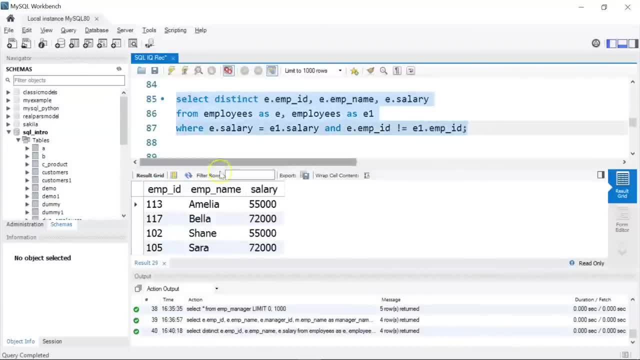 I'll give a simulation. Let's print the results. You see, here we have Amelia, Bela, Shane and Sara, who have the same salary. So Amelia and Shane have the same salary of $55,000.. Bela and Sara have the same salary of $72,000. 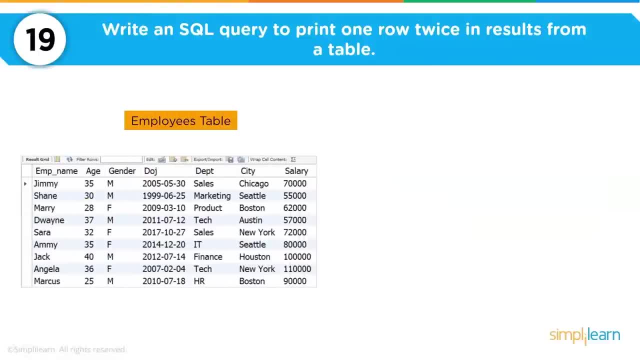 Okay, Now moving to the 19th question. So the question is to write an SQL query to print one row twice in results from a table. So I have a table, I have a table here called employees and I want to print one row twice in the results. 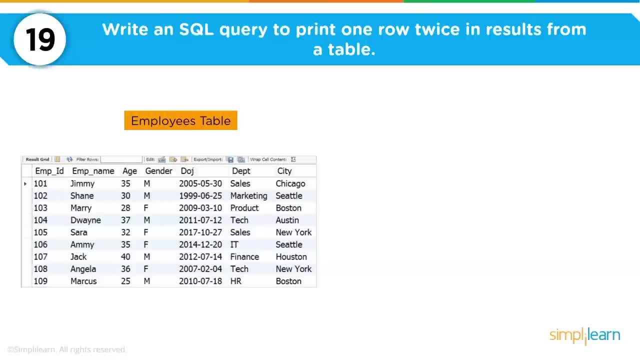 So to solve such kind of problems you need to use the union all operator in SQL. So union all combines the result sets of two or more select statements. It does not remove duplicate rows between the various select statements. All the rows are returned. 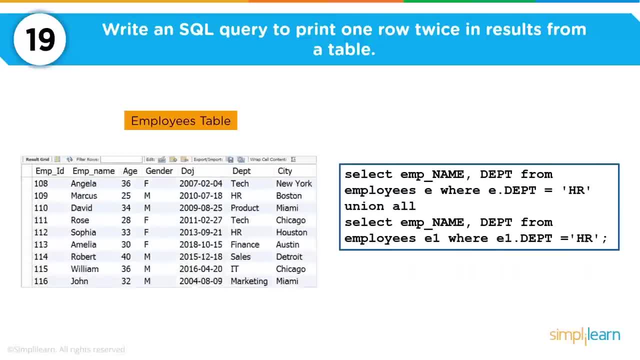 So let's say, I want to print the employee name and department for those employees who are from the HR department. So let's say, I want to print the employee name and department for those employees who are from the HR department. Now, to do this we can use the union all operator. 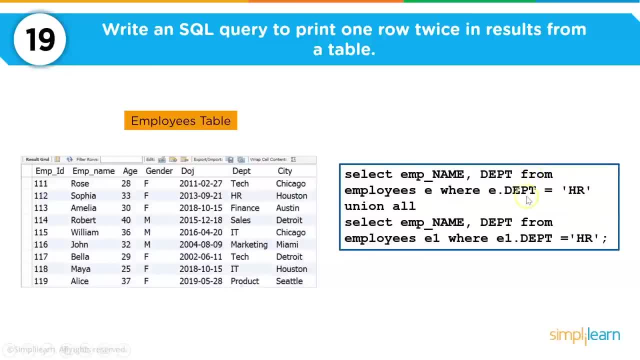 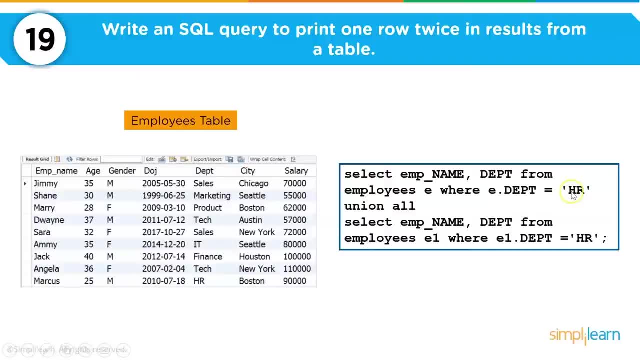 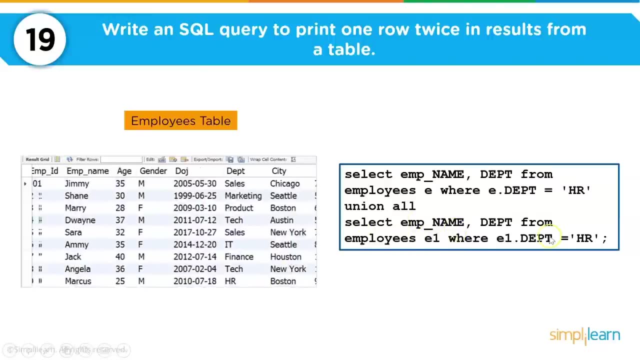 You can see it here. So I am selecting my employee name, the department, from my table employees as E, Then I am giving my where clause where Edepartment equal to HR And then I am using the union all operator. Then I am again selecting my employee name, department, from employees with another alias as E1, where E1.department equal to HR. 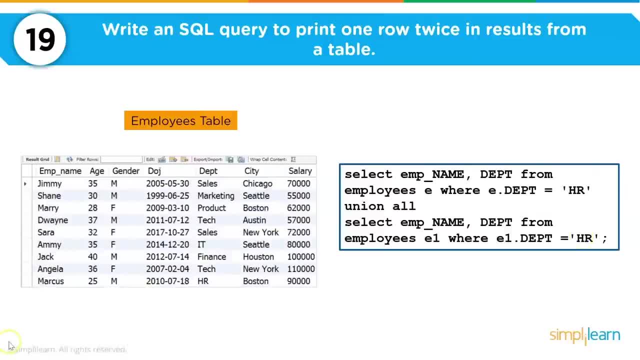 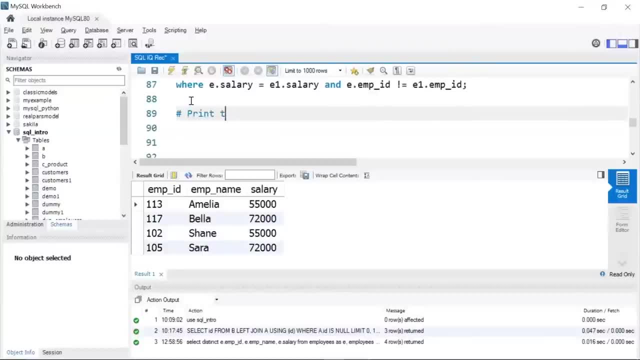 So let's do this. Okay, So I will give my comment as print row twice. Okay, Now I will start with my query. I will write: select my employee name, the department from my table, that is employees, as E. 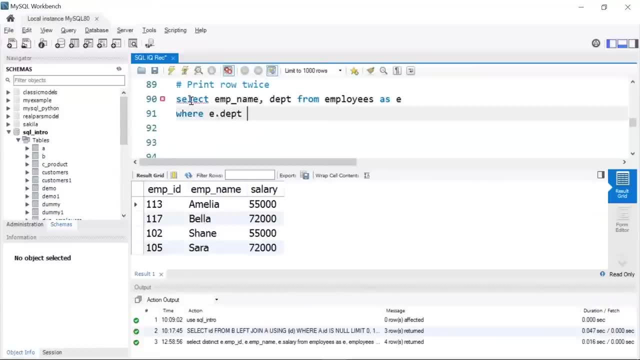 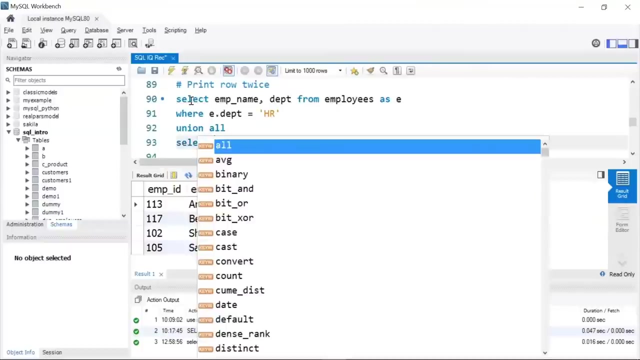 Then I will use where Edepartment equal to HR, Then I am going to use the union all operator, So the union all will combine the result set of two or more select statements. Then I am going to write select emp underscore name comma. 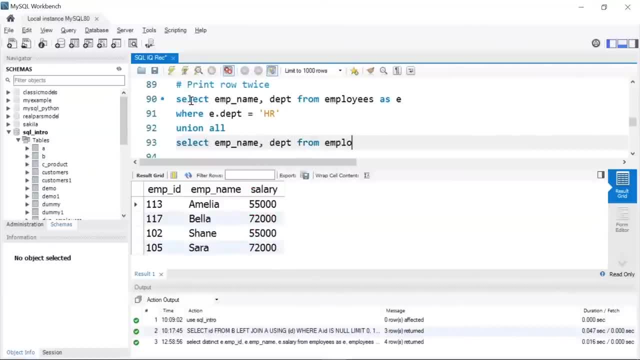 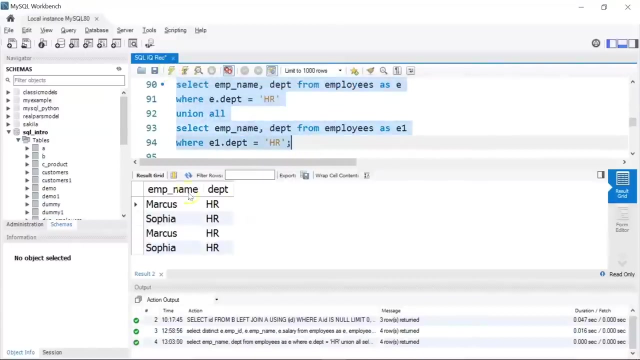 My department from employees as E1, where E1.department equal to HR. I will give a semicolon Now. let's run it. There you go. You can see here Marcus and Sophia are from the HR department And we have printed them twice in our results. 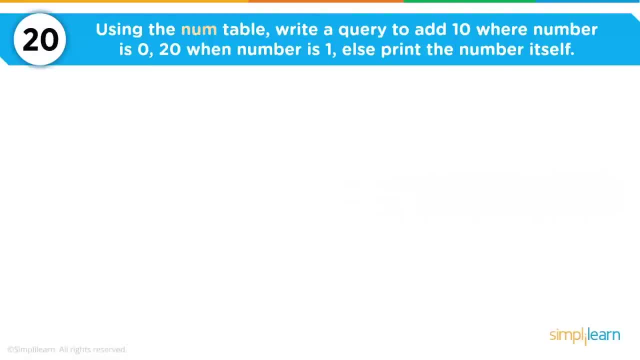 Coming to the next question. The question is, using the num table, write a query to add 10 when number is 0,, 20 when number is 1.. Else print the number itself. So you can see here. I have my table called num. 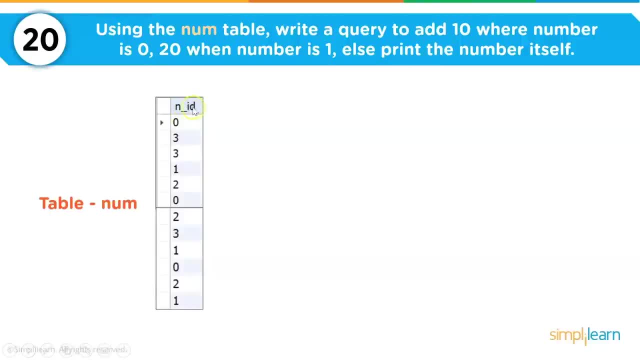 And it has just one column which is num ID or number ID. We have some numbers here, And from these numbers I want to add 10 if the number is 0,, 20 if the number is 1.. Else I would print the number itself. 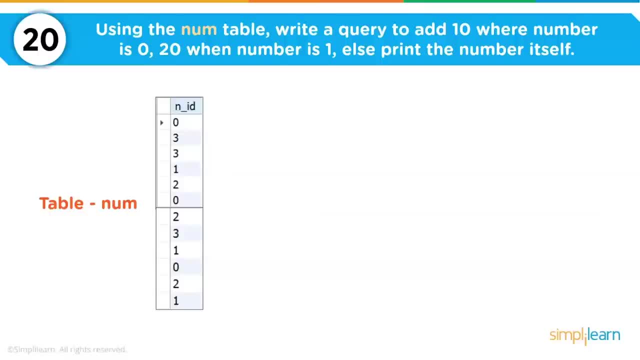 So to answer this question, we will use the case statement in SQL. So the case statement is SQL's way of handling if-then logic. The case statement is followed by at least one pair of when and then statements. So here you can see I have my case statement. 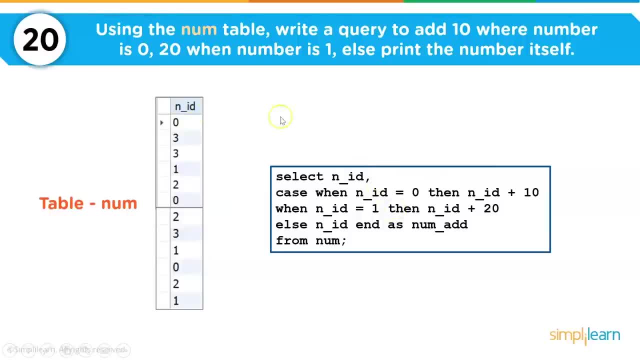 I am writing one case. My column name n underscore ID equal to 0., Then add plus 10.. If it is 1,, then add plus 20.. Else, we will just return the number ID. Now, let's do this. 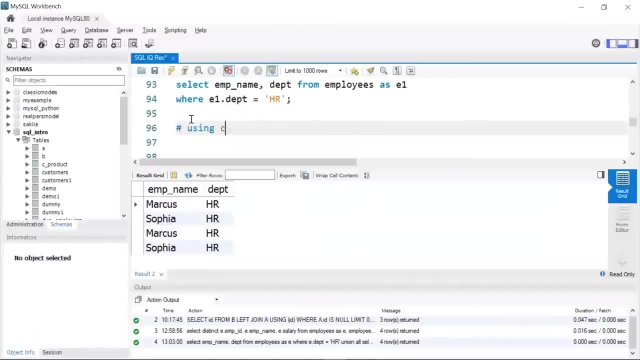 Okay, I will give a comment saying using case statements. Okay, First of all, Let me display the values present in my num table. You can see here this is my table and there are total 12 rows of numbers. Now let's start with our query. 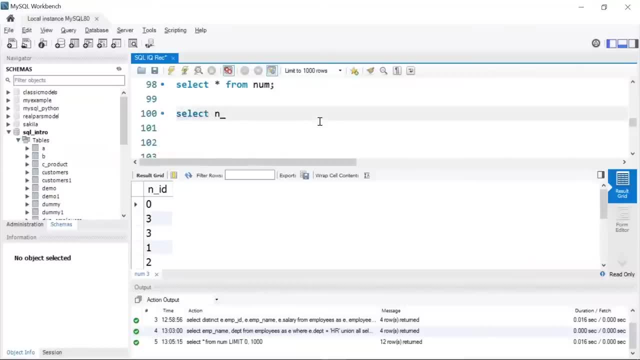 I will write: select n underscore ID comma. Then I am going to write my case statement. So I will use the keyword as case When n underscore ID equal to 0. I will use then n underscore ID plus 10.. I will write when n underscore ID equal to 1.. 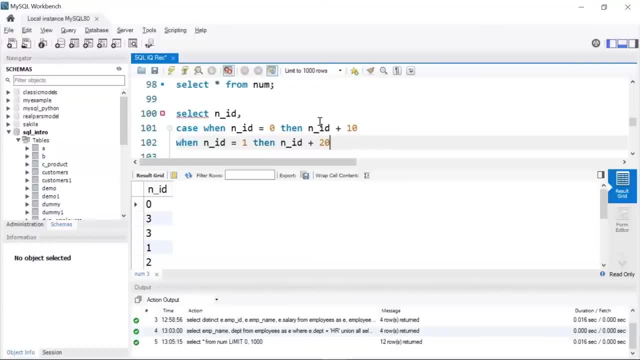 Then n underscore ID plus 20.. Else I will just print an ID. Now I will end my case statement. I will write end as an alias name, Let's say num, underscore add from my table that is num. Let's run and see the results. 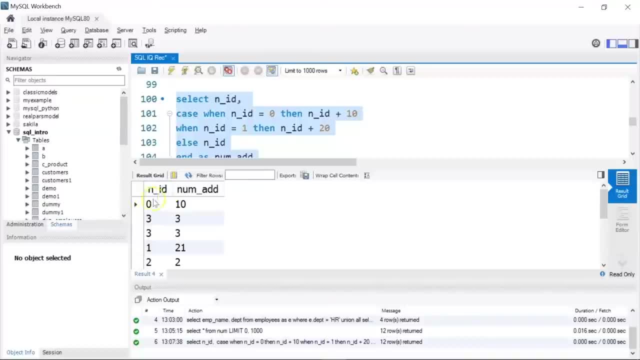 Okay, You can see here. my first number was 0. So since it was 0,, we have added num ID or n ID plus 10. So the result is 10.. Now, wherever the num ID is 1.. 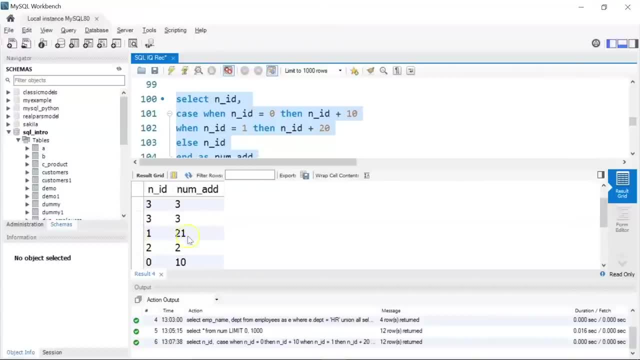 For example, here we have added 20. So the result or the output becomes 21.. Similarly, here the value was 0. So we have added 10. The output is 10. And you see here again, Here we had another 1.. 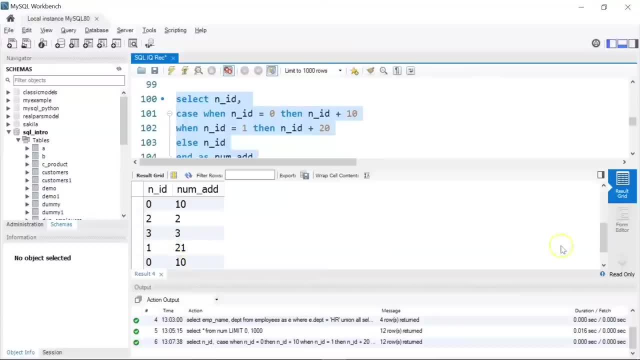 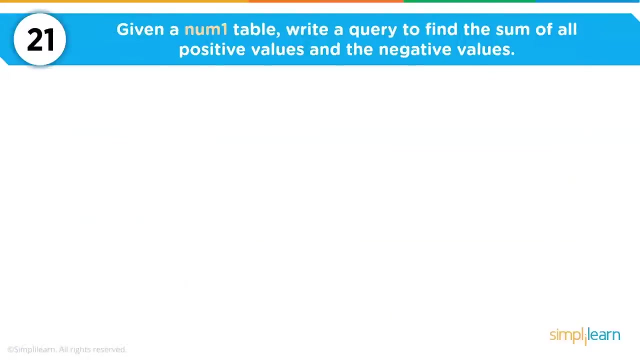 So we added 1 to 20. So the result becomes 21.. And for the rest of the numbers, For example 3. We had 2. The values are the same. Okay, Now moving ahead. So we have a table called num1.. 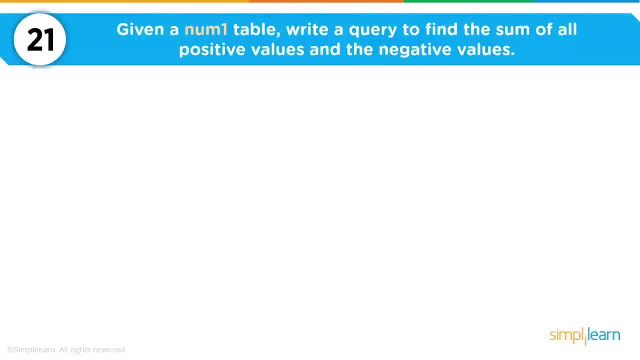 And using this table, We want to write a query to find the sum of all positive values and the negative values. So let's see the table first. So this is my table, which is num1.. You can see, here We have a list of integers. 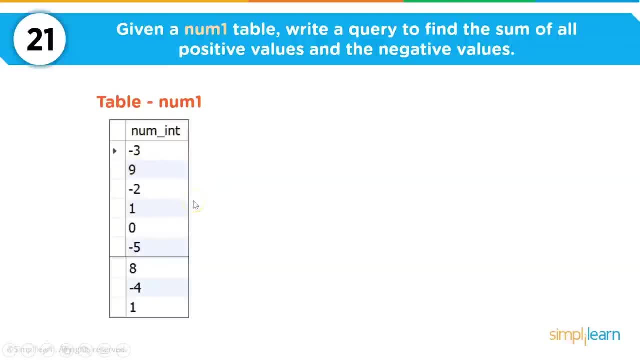 And there are positive as well as negative integers. So for positive values and the negative values We want to find the sum separately. So again for this we are using the case statement. You can see here I have used 2 case statements. 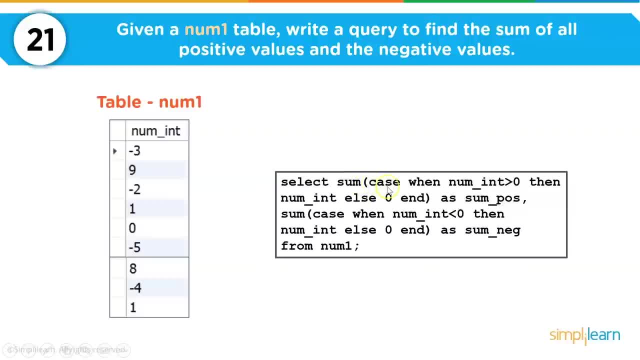 I am writing SELECT And then I am using the case to find if the number is greater than 0. Which means it's a positive number. So I am finding out the sum And then I am checking case when the integer is less than 0.. 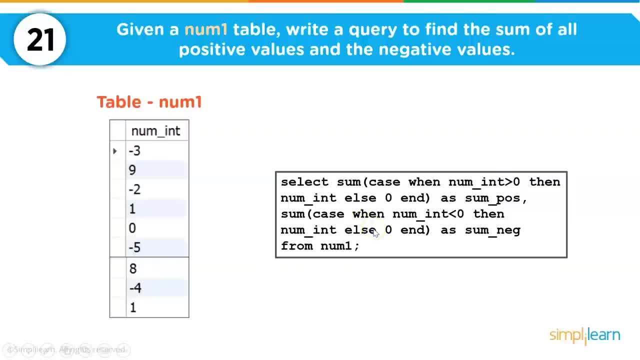 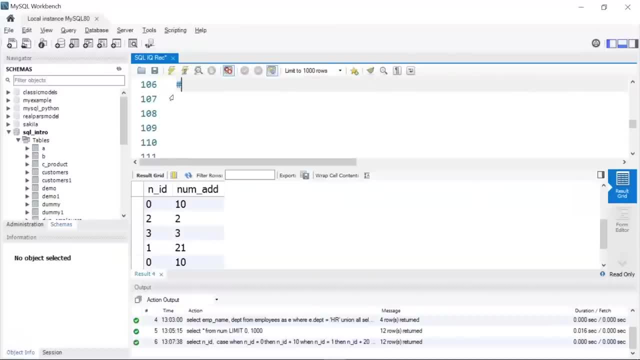 So it's a negative number And I am finding the sum for the negative numbers as well. Let's do this, Okay, So I will give my comment as add positive and negative numbers. Okay, So let's start with our SELECT query. 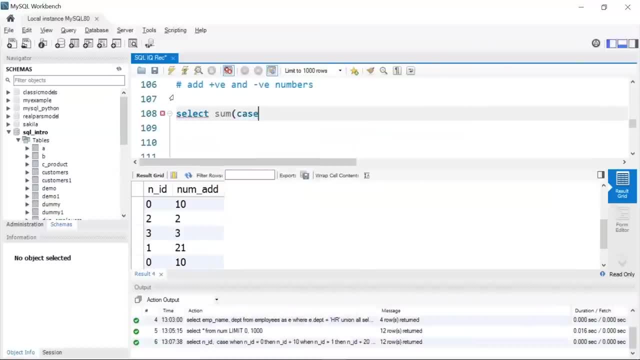 I will write SELECT, I will use the SUM function And inside the SUM function I will use my case statement. So I will write case when num underscore integer. Okay, Before that, let me just print the values present in my table. So I will write SELECT. star from my table name, that is num1.. 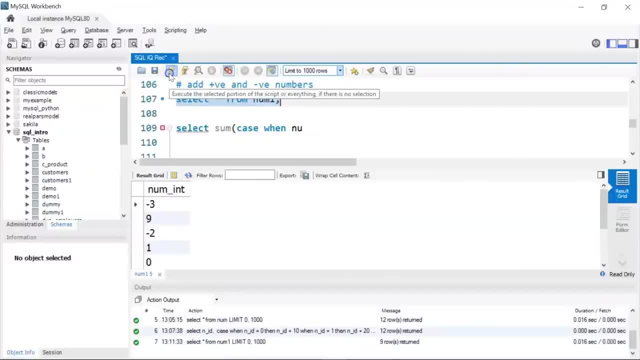 Okay, So you can see here these are the values or the list of integers that we have. There are some positive as well as negative integers. Okay, Let's continue with our query. So here I am going to write case when num underscore integer. 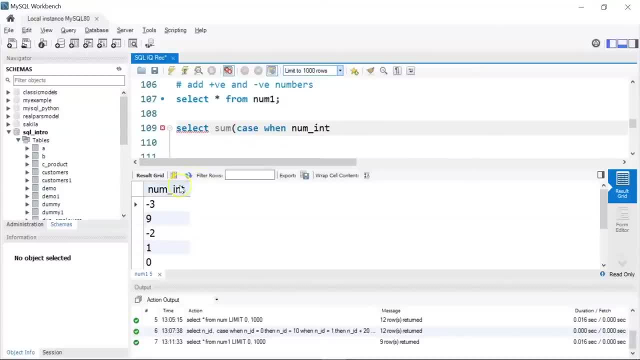 So I will write SELECT num underscore integer or int, which is my column name. If it is greater than 0, then I will return num underscore int, Else I will say 0 and end my case statement. I will give an alias as sum of, let's say, positive numbers. 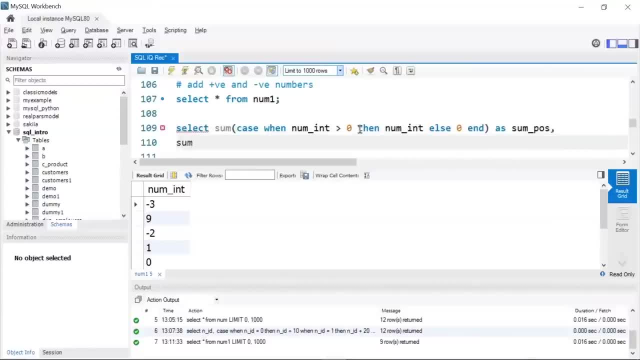 I will give a comma, Then I will use another SUM function And inside the SUM function we will use the case statement to find the sum of negative numbers or integers. So I will write num underscore int. If it is less than 0, then num underscore int. 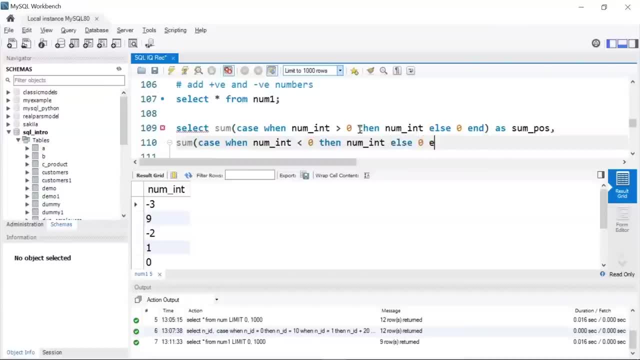 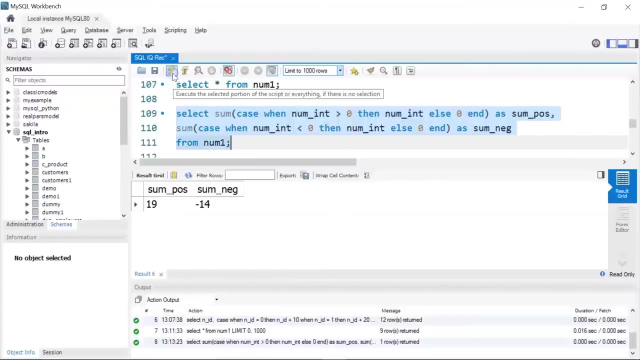 Else 0 and I will end Okay, And I will give another alias name, as, let's say, sum underscore, neg, which stands for negative, POS, is for positive integers, And then I will write from my table: that is num1.. Let's run it. 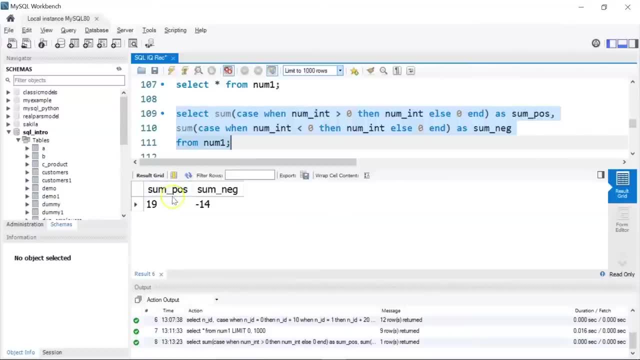 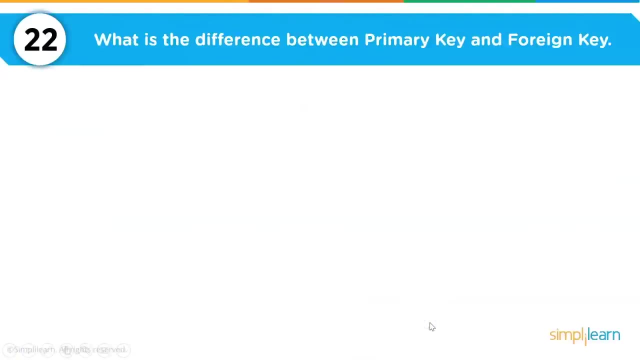 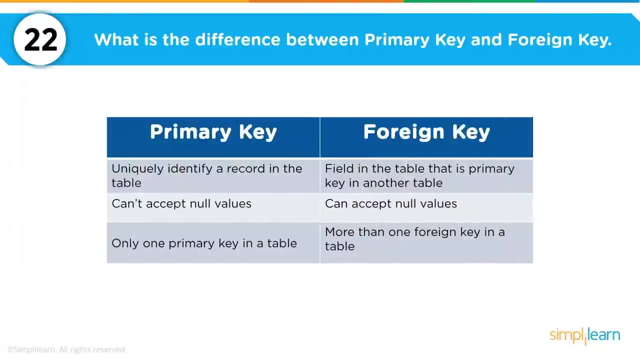 Okay, There you go, We have our results. So we have two columns: Sum of positive integers and sum of negative integers. You can see the results: 19 and minus 14 respectively. Okay, Now moving ahead. Now, in question number 22, we want to list the difference between primary key and foreign key. 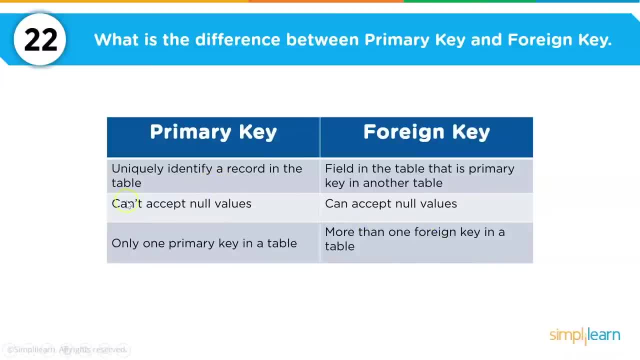 So, as you can see here, primary key is something that can uniquely identify a record in a table. So if you consider a school database, a primary key would ideally be the roll number or the registration number of the student, Because that is unique to all the students in a school. 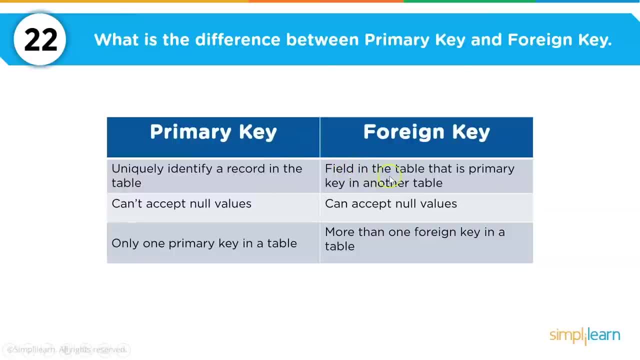 Now, foreign key is the field in the table that is primary key to another table. So suppose you have another table called courses to which the students have enrolled to. Now if you have a roll number or a registration number column in the course table, that becomes the foreign key. Now the other difference is: primary key don't accept or cannot be accepted. So primary key accept or cannot accept null values, while foreign key can accept null values. Now you can have only one primary key in a table, but you can have more than one foreign key in a table. 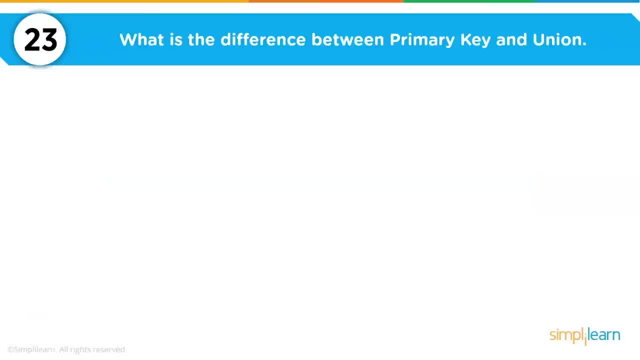 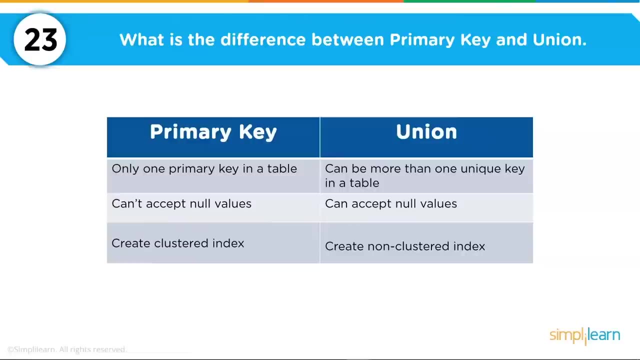 Now coming to the 23rd question: What is the difference between primary key and union? So you can have only one primary key in a table, as we discussed in the previous question, But you can have more than one unique key in a table. 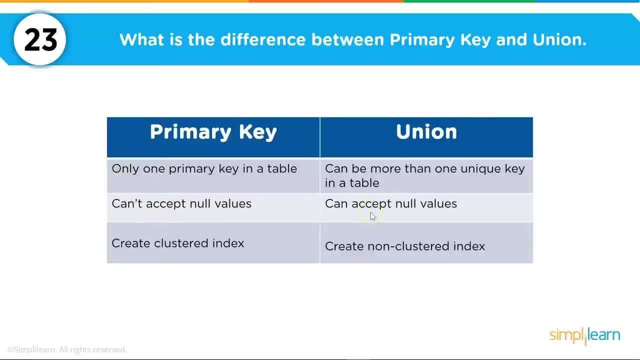 Now, primary key column cannot have null values, but union can accept null values. Now, if you assign a column as a primary key, you create a clustered index, And similarly, if you assign a column with union, you create non-clustered index. Okay, Now, coming to the 24th question. 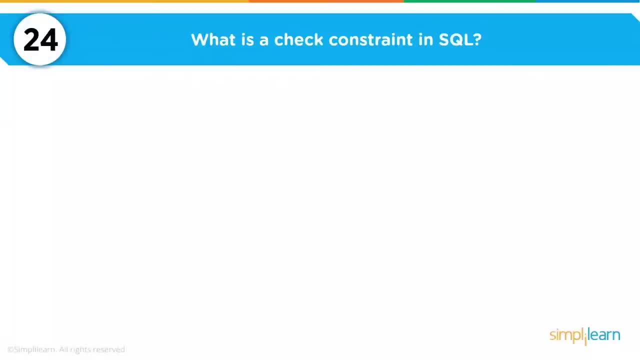 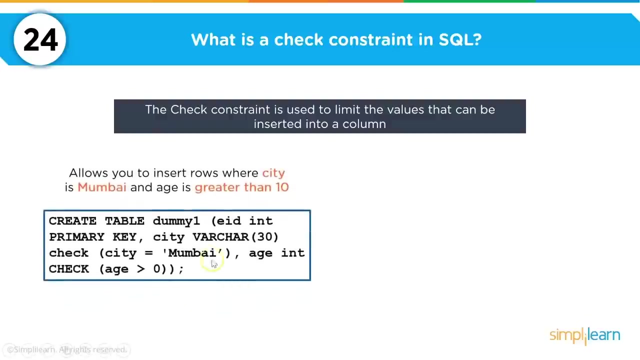 What is a check constant in SQL? So check constraints are used while creating tables. Check constraint helps to limit or restrict the values that can be inserted into a column. For example, we have a table here. Let's say dummy 1.. 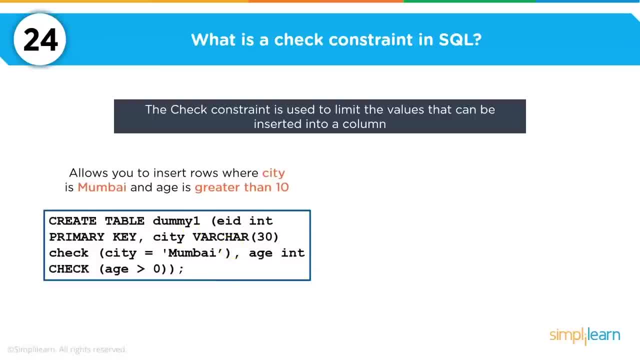 And you want to ensure that every time you insert the age of people or persons in the table, You want to make sure that age should be always greater than 0.. Reason being: a person cannot have, or an animal cannot have, or a tree cannot have a negative age. 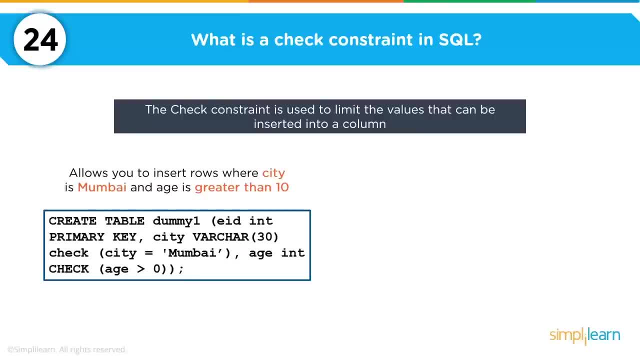 Similarly, you can set a constraint for the salary column in a table to ensure that it is always greater than 0., Because you cannot earn a negative salary, or it cannot be less than 0.. Now we are going to create a dummy table on my MySQL workbench. 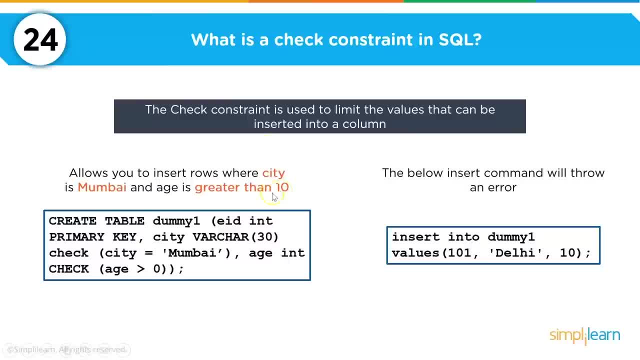 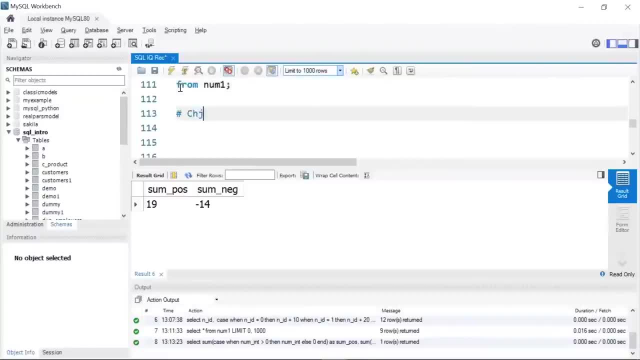 And see how check constraints can be applied. Check constraints can be applied. Okay, So let's give a comment as check constraints. Alright, So I am going to create a table called dummy. Let's say underscore SQL. Let's say underscore SQL. 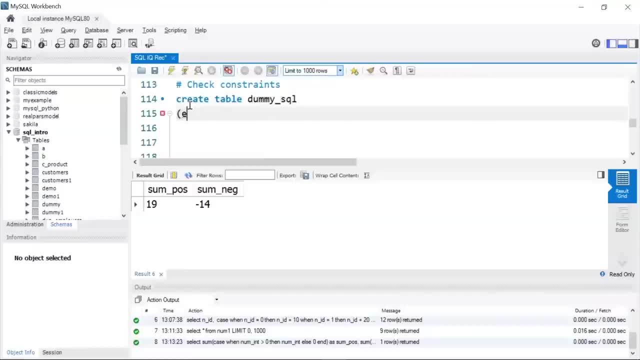 Now this table will have a few columns. First we have, let's say, EID, which stands for employee ID. The data type is integer And I am going to assign employee ID as my primary key. So I will write primary key here. 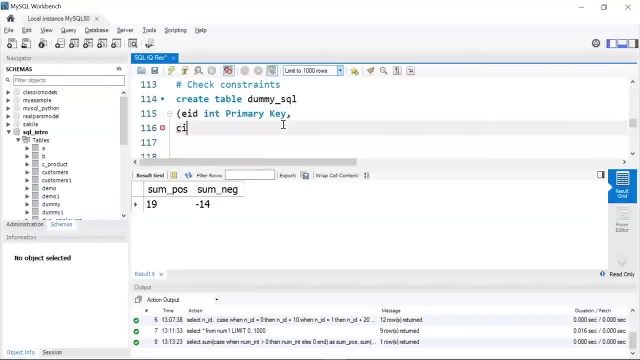 Okay, I will give a comma. Next we will have a city column. City column is of type, var, char or varying character. I will give the size as 30. And here I am going to apply my check constraint to this city column. 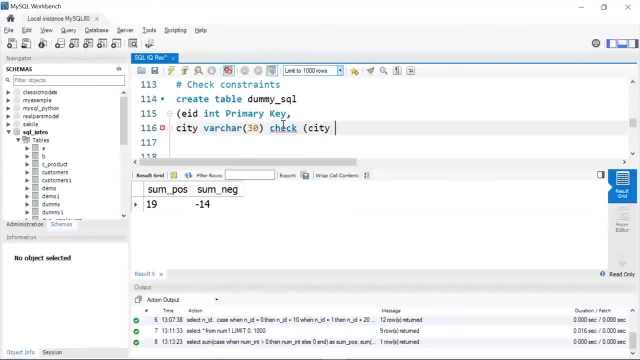 I am going to check. the city should take only values as Mumbai. Let's see. I will have my final column, that is age. Age is of type integer, And here I am going to check. my age should always be greater than 0.. 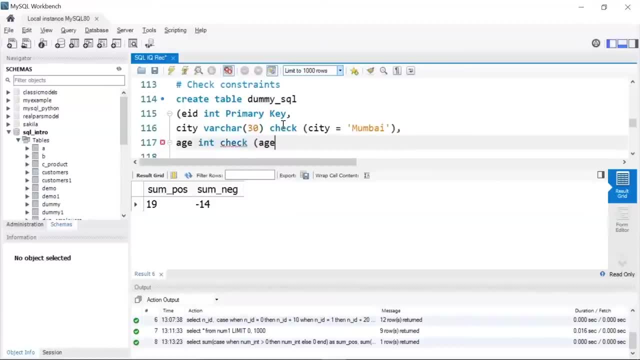 So I will write check age greater than 0.. Okay, So our dummy SQL table has one primary key constraint And we have applied two check constraints on city and age column. Let's run this, Okay. So we have created our table successfully. 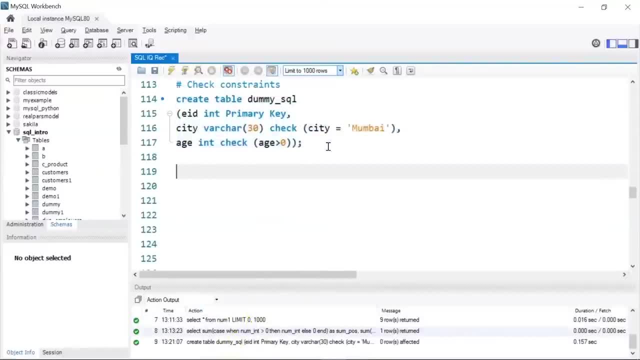 You can see it here. Now let's insert a few records and we can see the difference. I will write insert into dummy underscore SQL. I will write values. I will have my employee ID as 101.. I am giving my city as Mumbai, which is what we want. 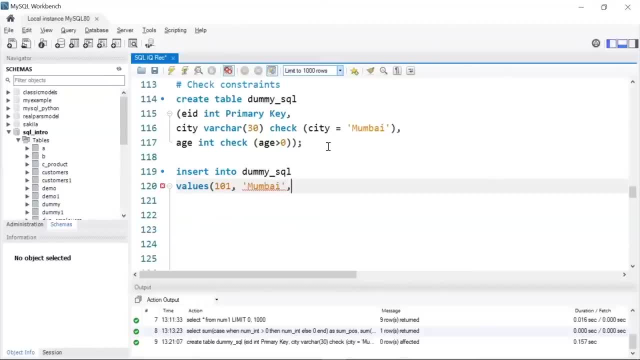 And let's say I will give my age as 10.. Now this should perfectly work, because my city is Mumbai and my age is greater than 0. So I should be able to insert this record successfully. You can see here: I have inserted this record to the table. 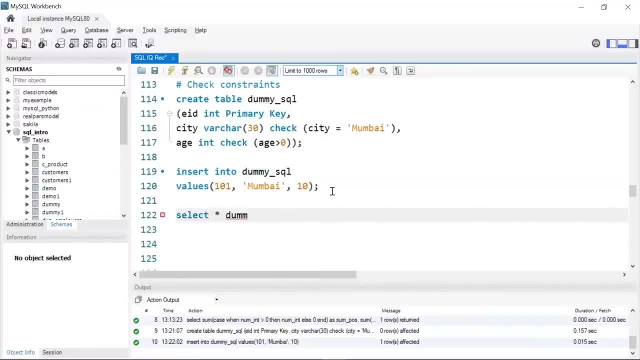 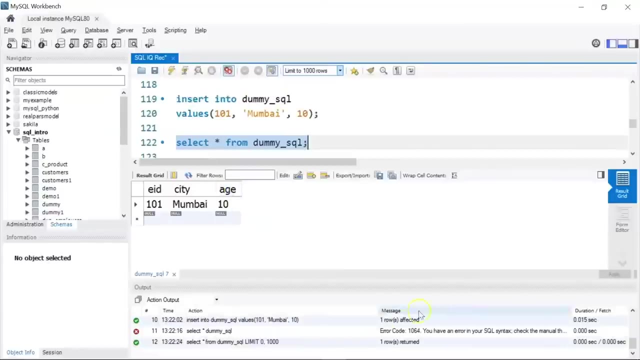 I will write select star from dummy SQL so that you can check. Let's run it. There is some mistake. I should write from: Okay, Let's run it. You can see it here. We have one record or one row returned. 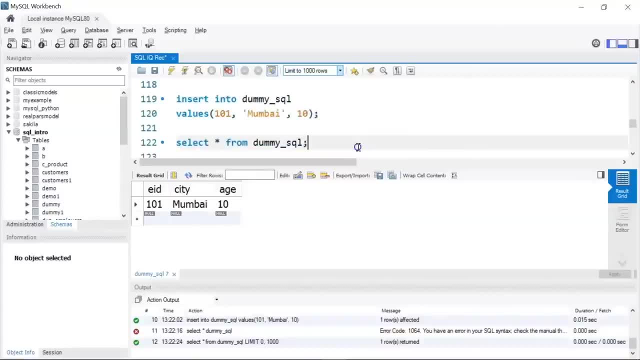 Now let's see. We will insert another record, And this time I am going to give my employee ID as 102, because it has to be unique, And this time, instead of Mumbai, I am going to give my city as, let's say, Delhi. 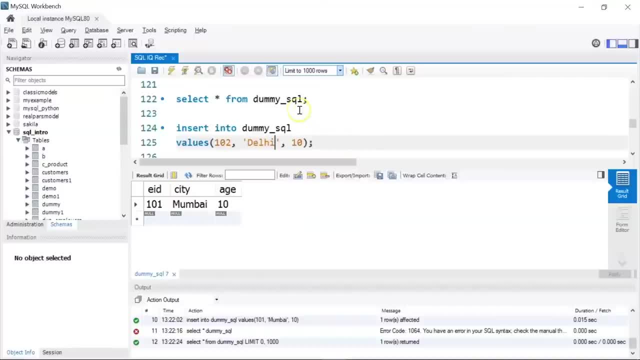 So I am not following my check constraint where I am supposed to give only Mumbai, I am purposely giving Delhi here to see the difference. If I run this, let's say we will have ages 40, which is greater than 0.. Let's run it. 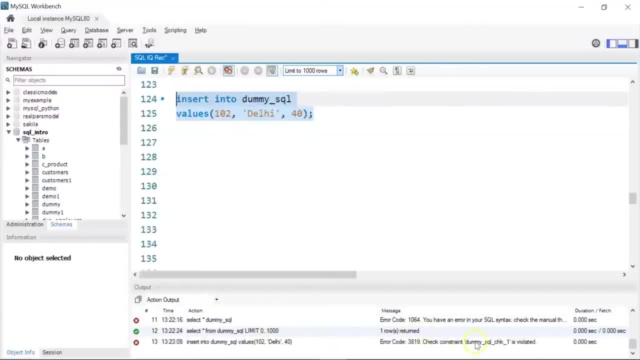 You see, here we get an error saying check constraint dummy underscore SQL, underscore Check is violated. Similarly, let's say I change this to Mumbai again, And instead of 40, let's say I will give us minus 30. So your age can never be in negative numbers. 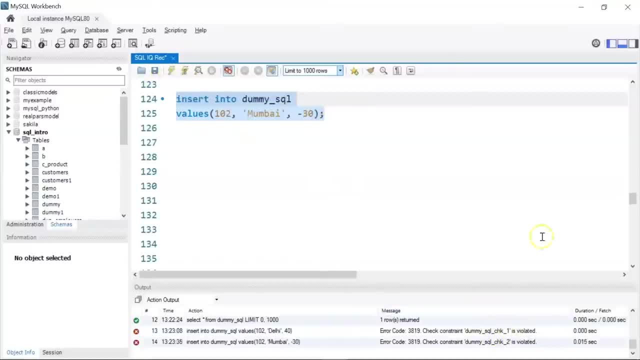 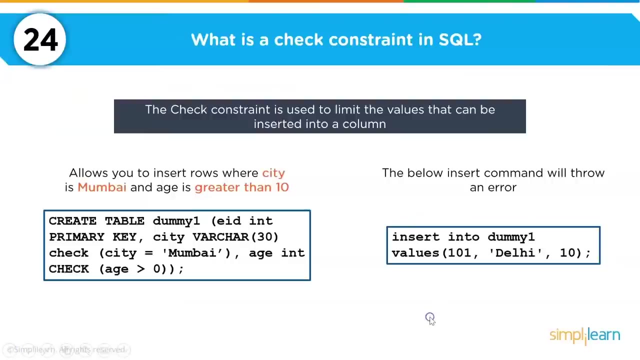 If I run this, I get the same error. My check constraint has been violated because age should be greater than 0.. Okay, So this is how you can use check constraints in SQL. Now, coming to the 25th question. 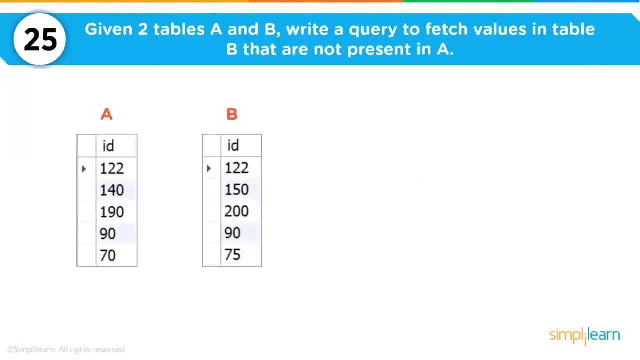 So, given two tables, A and B, you want to write a query to fetch values in table B that are not present in table A. Now, to answer this question, you can use the left join. So what left join does is it returns all the rows from the left table and only matching rows from the right table. 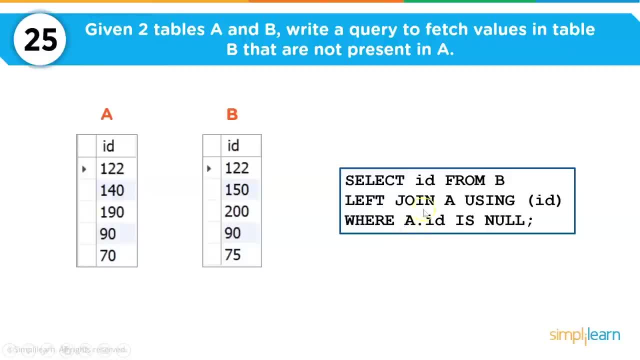 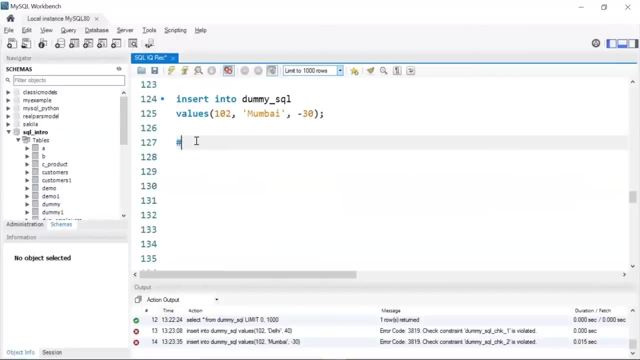 And I have used my condition. as aid which is in the right table should be null, Let's write this query on the workbench. Okay, So I will give my comment Using left join. First of all, let me display my tables. 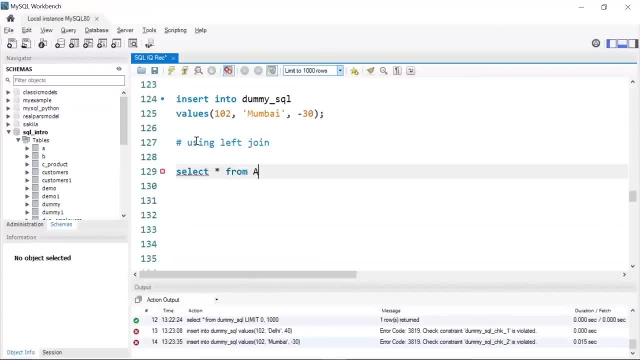 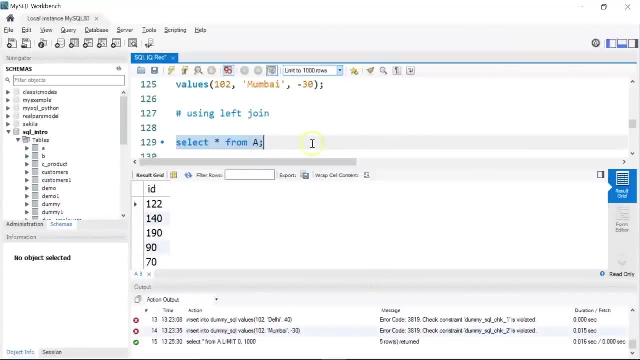 I will write select star from A Where on this I have the ids. There are total five ids in table A. Similarly, I will copy this and will see the values that are present in table B. Again, I have five values. 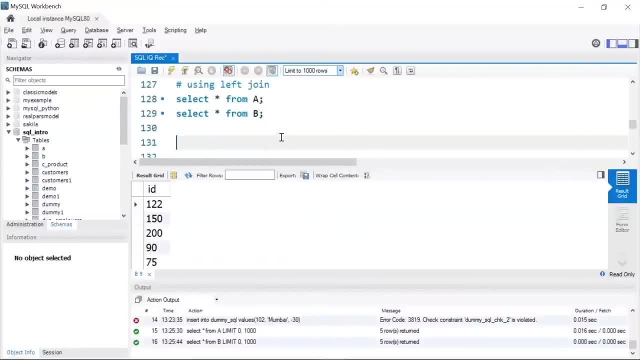 There are a few non-matching values as well, So I want to return those non-matching values that are not present in table A. So for that I will write select id from table B. I will use left join A using my id column. 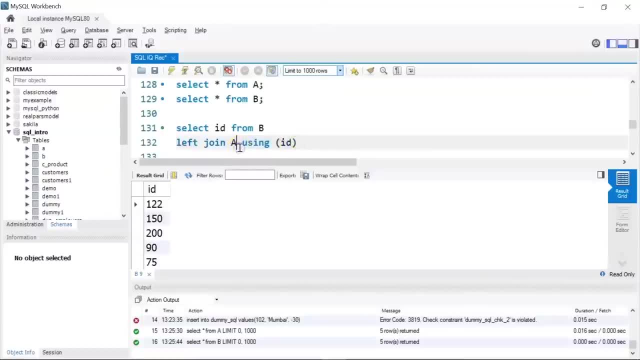 This is another way to give the condition. You can use the on operator, Then I will give. where Aid is null. Let's run and see the results. There you go. So 150, 275 are not present in table A but are present in table B. 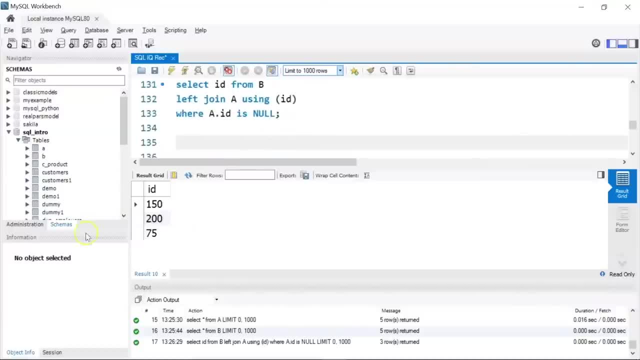 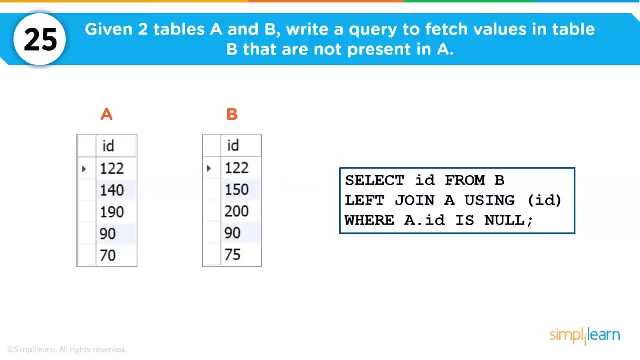 Okay, Now moving ahead. So now we will look at the last set of five questions. So these questions are based on the popular Northwind sample database provided by Microsoft. There are several tables in this database, So we have an order table, customers, employee products, region table and others. 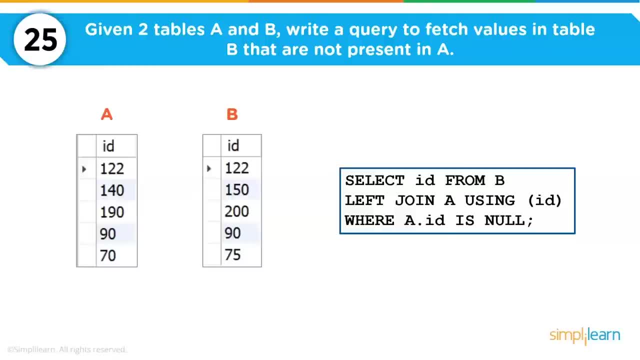 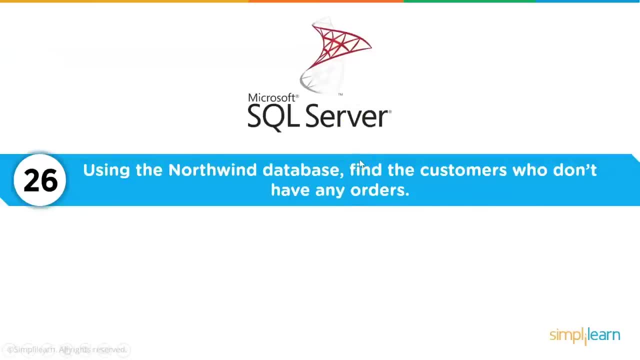 We will use our Microsoft SQL server to solve the five questions. So my next question, which is based on Microsoft SQL server, The question is: using the Northwind database, find the customers who don't have any orders. Okay, So I am on my Microsoft SQL server management studio. 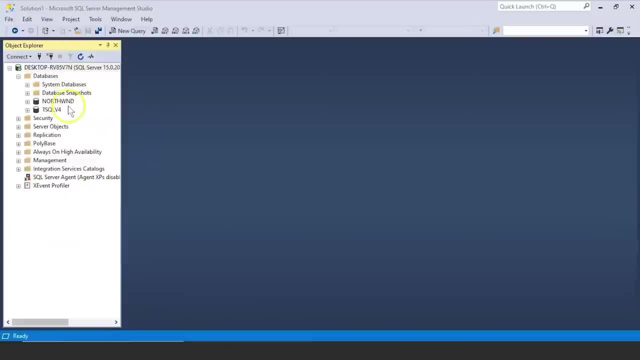 So this is how the interface looks like, And here you can see. I have a list of databases. Now to solve the last five questions, I am going to use the Northwind database. If I expand this, I will click on the plus sign. 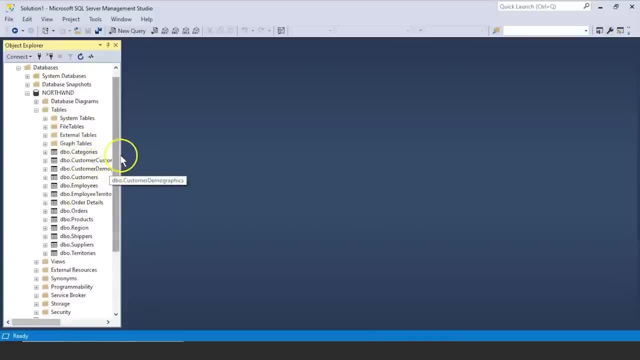 You can see there are a lot of tables that are already present In the database. you can see, here we have customers, employees, employee territories, order details, orders, products, region, shippers, suppliers, territories and more Okay. 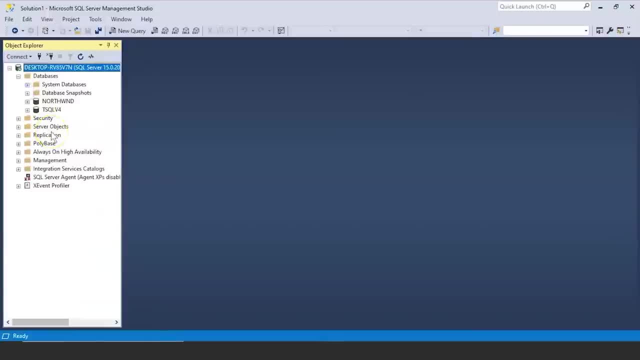 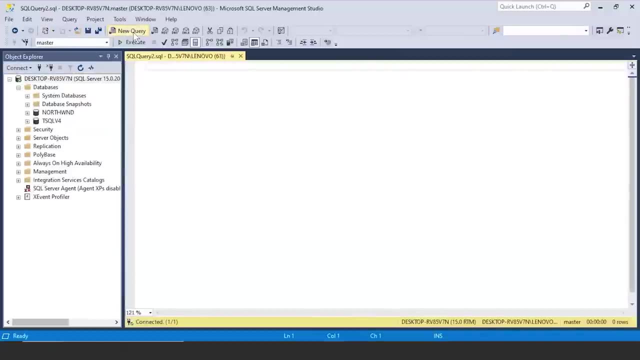 Let me just collapse this, Alright. So to write my queries, I am going to create a new query file And here you see I am currently on my master database. I am going to change this to Northwind database so that we can utilize all the tables that are present. 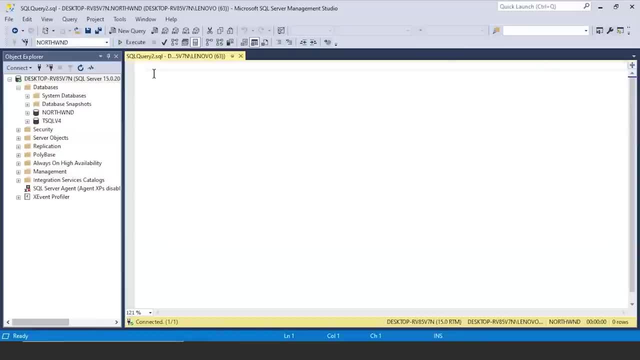 So my 26th question was to find the customers who don't have any orders. So for that I am going to use two tables: customers and orders. So let me first give a comment saying customers with no orders. 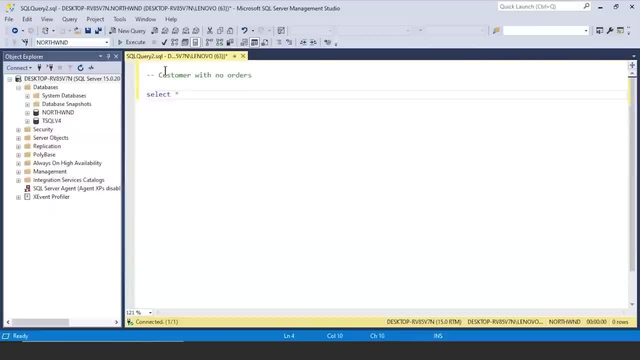 And now let's go ahead and display the columns that we have and see the records present in the tables: customers and orders. So first I am checking all the columns and the rows present in the customers table. I will execute using this button or you can hit F5 as well. 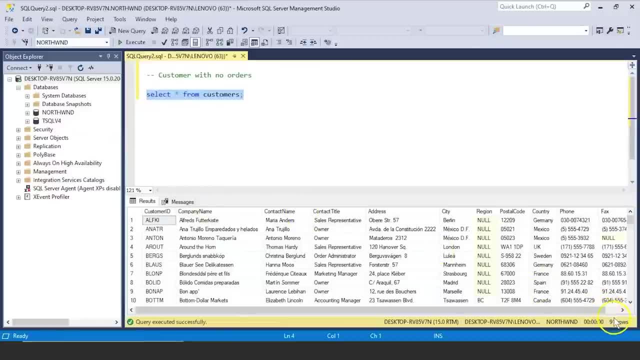 Okay, You can see here there are total 91 customers. These are all unique customers. You have total 91 unique customer IDs. You see here the company name of the customer. You have the contact name, the contact title, address, city to which the customers belong to. 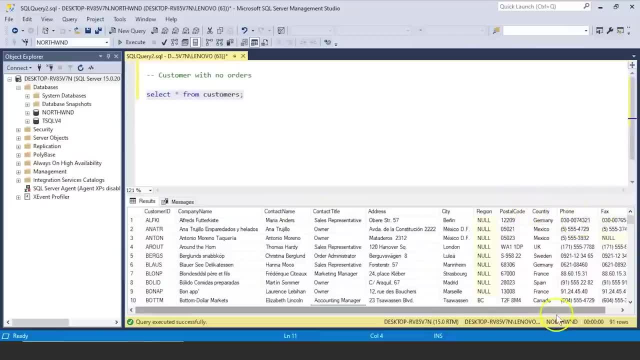 then the region, postal code, country, phone, fax number. Okay, Now let me just copy this query, And now we will check for the orders table. I will write select star from orders And let's execute it or run it. 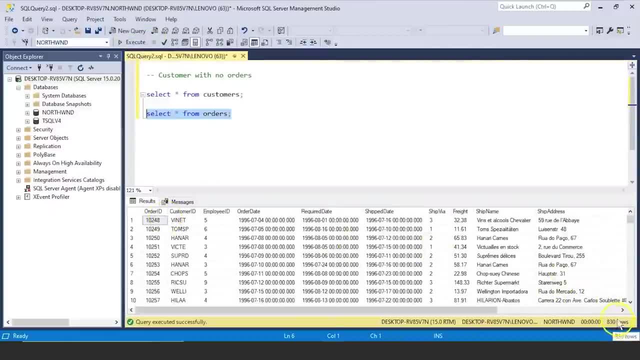 Okay, So there are total 830 rows of information. So there were total 830 orders or order IDs. We have the customer ID Now. this customer ID is actually the foreign key for the orders table, But for the customers table, customer ID is the primary key. 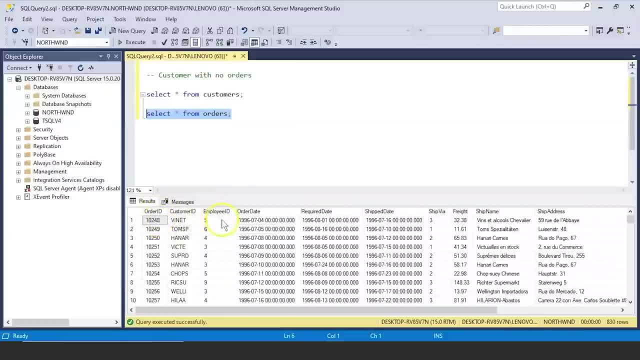 And in the orders table, order ID is the primary key. We also have the employee ID. Again, this employee ID is the foreign key for this orders table. We have the order date. We have the required date. ship date: ship via, which means by which medium the order was shipped. 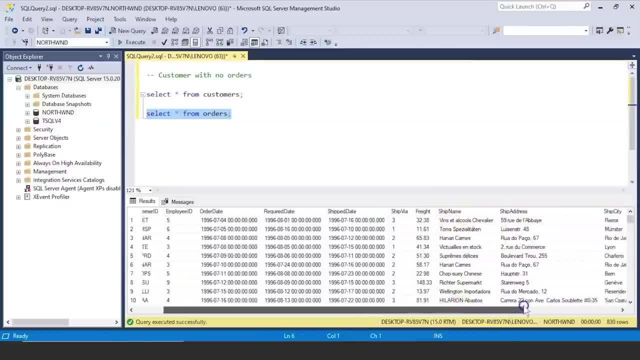 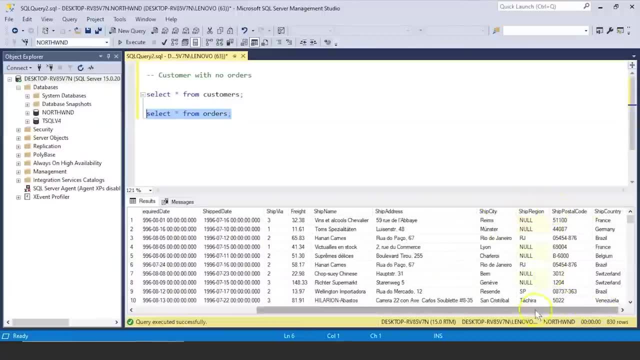 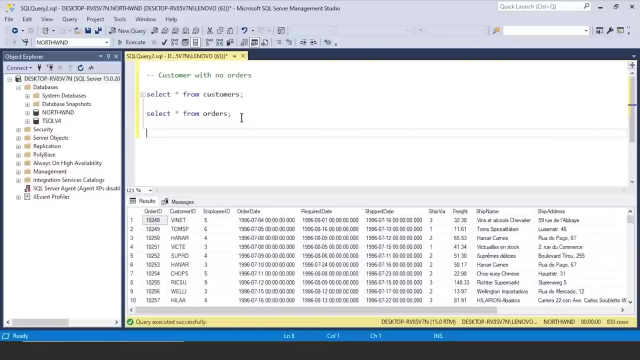 We have the freight charges, ship name and ship address as well. Then you have the city from which the item was shipped, the region, postal code and the country. Okay, Now let me use the distinct keyword. I will write: select. 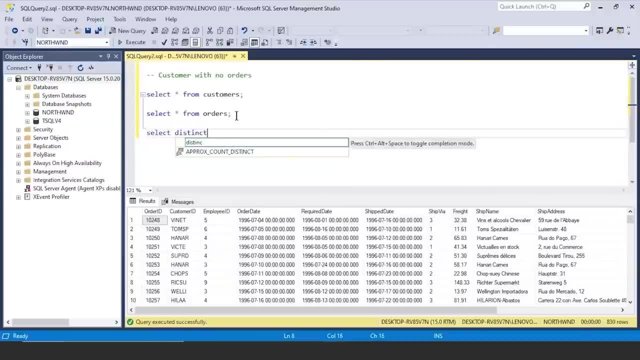 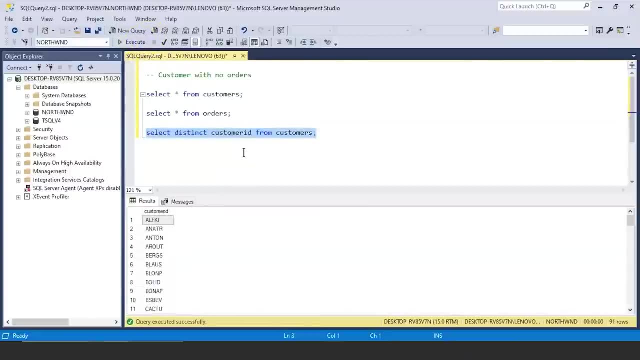 distinct. I want to find the distinct customer IDs from my customers table. Let's run and see how many unique customer IDs we have. So there are total 91 customer IDs or customers. Now let's check for the orders table. Let's run it and see the difference now. 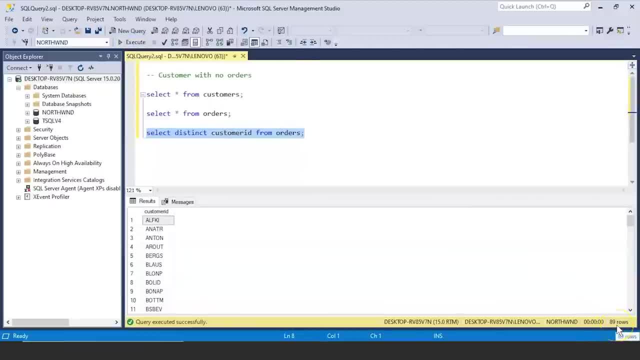 If you see here, there are total 89 customer IDs in the orders table, which means there are two customers missing from the orders table And that implies those two customers don't have any orders. So to get the result, I will use two different queries to derive at the same output. 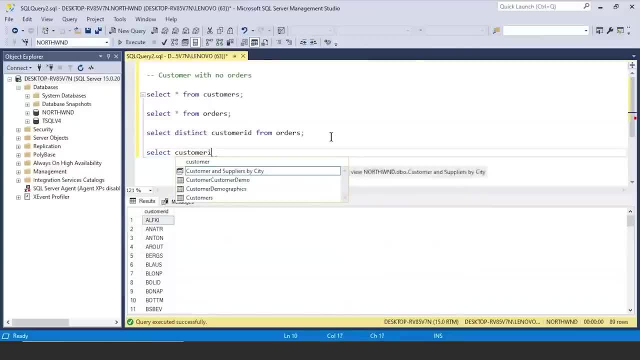 So I'm going to select my customer ID from my table, that is customers. I'm going to use where My customer ID And then I'm going to use the not in operator. I'm going to use a sub query: Select. 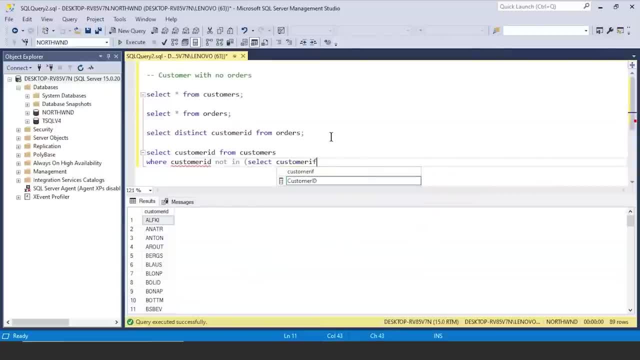 Customer ID From My orders table, Close the bracket and I'll give a semicolon. Now what this query essentially does is: it is first going to find all the customer IDs that are present in my orders table And in the outer query we are only going to return the customers that are present in both the tables. 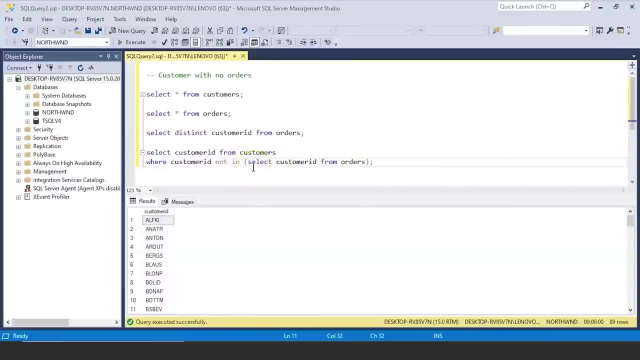 And we are going to exclude those customers which are not present in the orders table. So let's run and see the results. We should get two customer IDs. There you go. So these are the two customer IDs which are present in the customers table and are not present in the orders table. 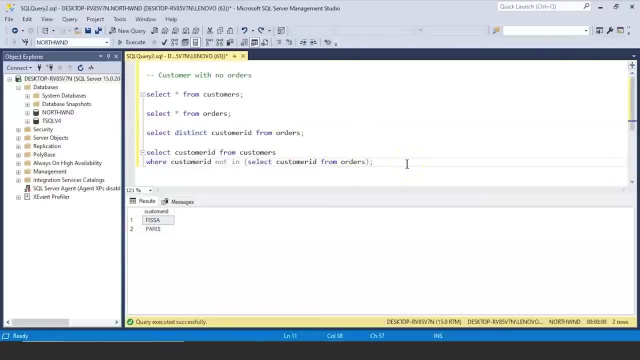 Meaning that they don't have any orders in their name. Now there is another way to do it. That is to use the not exists operator, wherein you can write another sub query to get the same result. We'll leave that to you. You can try this out using the not exists operator as well. 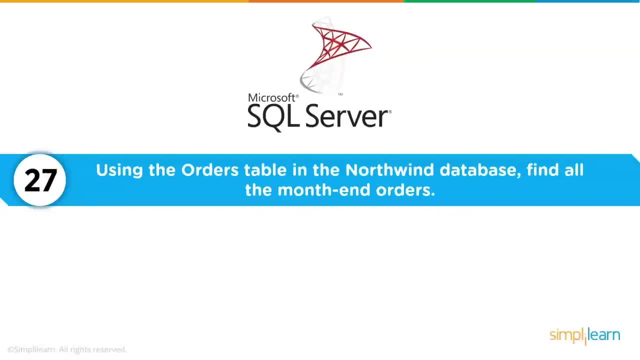 Coming to the 27th question, Using the orders table in the Northwind database we want to find all the month end orders. So such problems you will face while dealing with sales data. So very often sales executives would try hard to meet their month end targets. 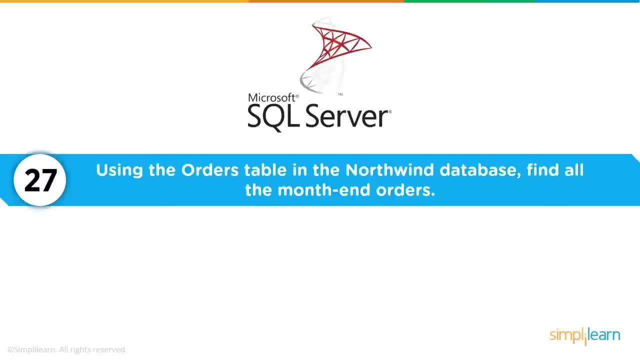 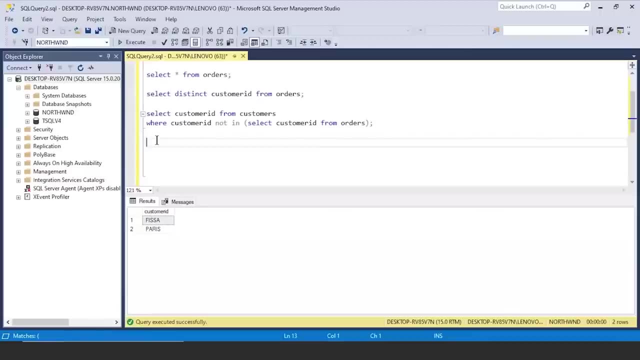 We want to display all the orders made on the last day of the month. So let's solve this question on our Microsoft Word, Microsoft SQL Server. Okay, So let me first give my comment for the 27th question. So the question is to find all the month end orders. 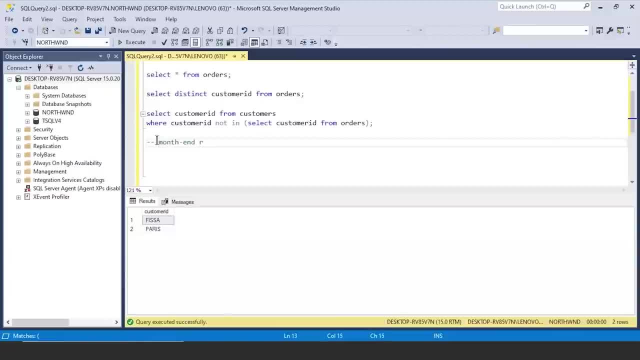 So I'll just write month end orders. Okay, Now to get the month end orders, we are going to use a built-in EO month function which stands for end of month. So let's start with the query. I'll write select. 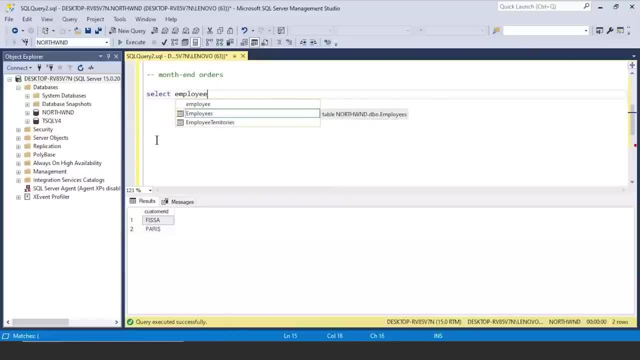 We are going to select the employee ID. I also want the order ID and we want the order date from my table. that is orders. I'll then give my where clause, I'll write where My order date equal to and I'll use my inbuilt function. that is end of month. 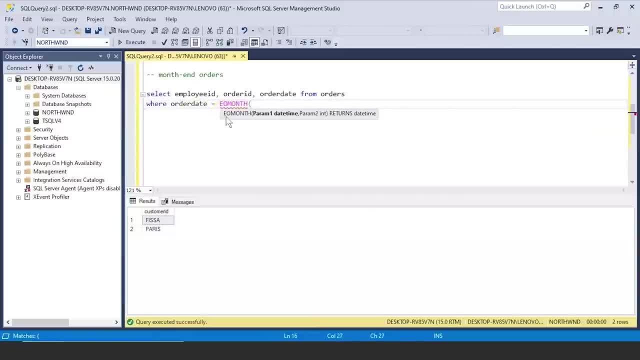 I have hit tab to autocomplete and inside this function I'll pass in my order date column. Then I'm going to use the order by clause. I'm going to order it by employee ID and the order ID. I'll just move down and hit tab. 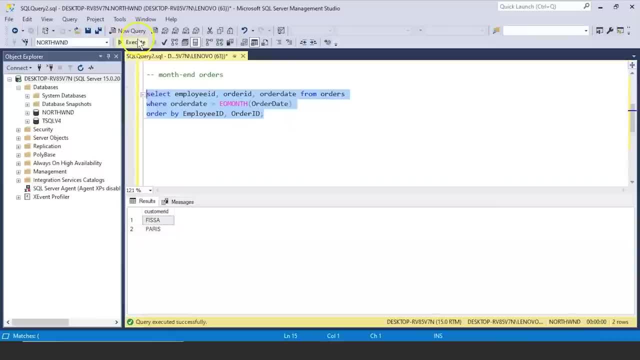 Okay, Let's run the query. There you go. We have got 26 rows of information. You see, on the left side we have the employee IDs, the order IDs and then we have the order date column. Now, if you mark the values present in the order date column, these are all the end of month date values. 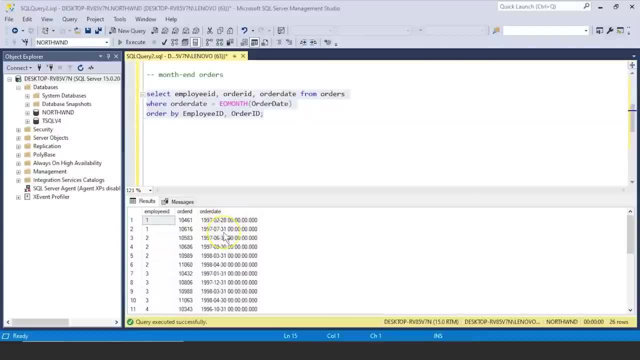 You see, this is 28th of Feb, Then we have 31st of July, We have 30th of June, So on and so forth. So these are the list of all the orders that were placed on the last day of the month. Coming to the 28th question, We want to find the top 5 countries with the highest freight charges in the year 1997.. So freight charges: The freight charge is the amount paid to a carrier company for the transportation of goods from origin to another location. 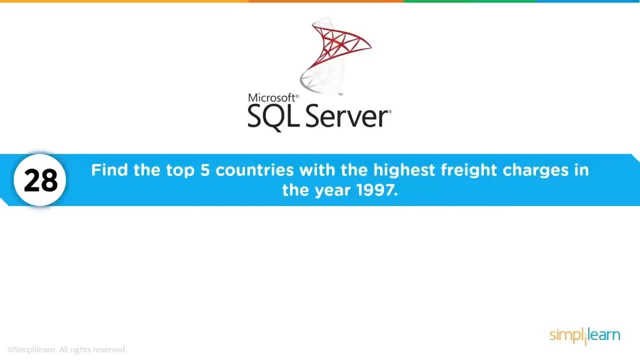 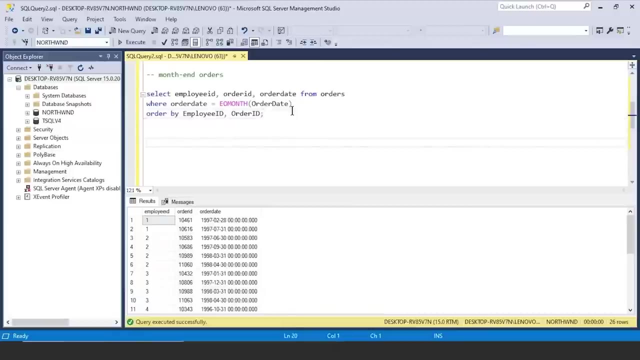 The freight charge is calculated based on the mode of transportation and the distance between the pickup place or the pickup location and the destination. So let's try this out on the Microsoft Server Management Studio. Okay, So let me go ahead and give my comment. 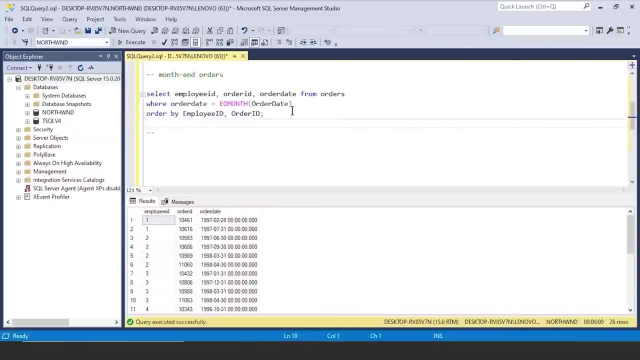 So we want to find the top 5 countries with the highest freight charges. I'll just give my comment as highest freight charges. Okay, Now to solve this question, I'll just change this to ght. Okay, We are going to use our orders table. 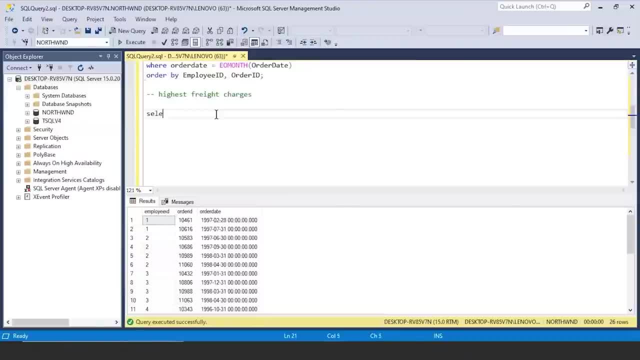 Okay. So the way to do is I'll write select, I'm going to use the top 5. So top is another keyword or an operator. So I'm going to find out the ship country and then I'll calculate the average freight prices. 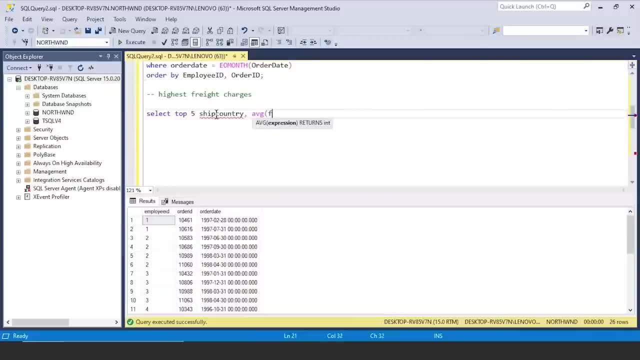 So I'm going to use the average inbuilt function on top of my column Column, that is freight. I'll give an alias as, let's say, average freight. There should be no space. I'll give a underscore. I'll write from my table: that is orders. 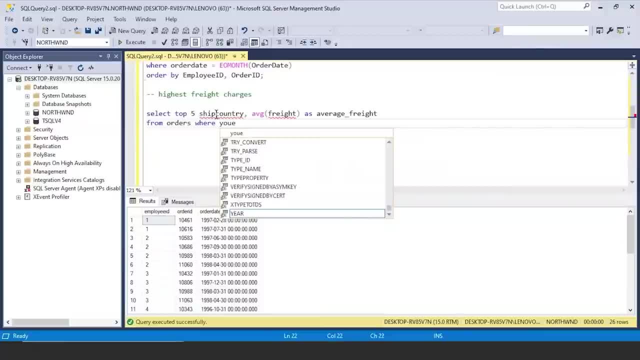 I'll use my where clause, where, and then I'm going to find the year From my order date column, and this year should be 1997.. I'm going to group it by my ship country and I'll use order by my alias name. that was average freight. And in descending order I'm going to sort it. Let's see the top 5 shipping countries who have the highest freight charges. These are the results. You have Austria, Switzerland, Sweden, Canada and Ireland, And here you can see the average freight prices, sorted in descending order. 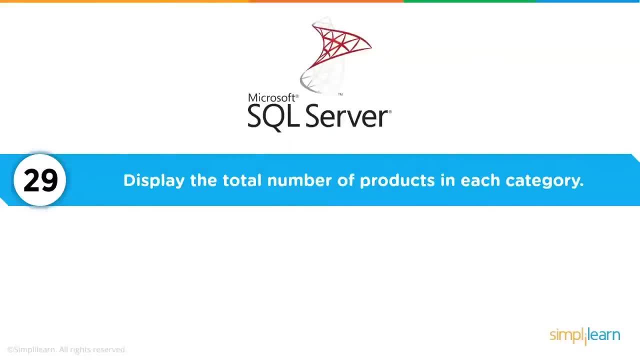 Okay Now moving ahead to the 29th question. So here we want to display the total number of products in each category. So we have two different tables: products and categories. So both these tables we are going to use to find a solution to this problem. 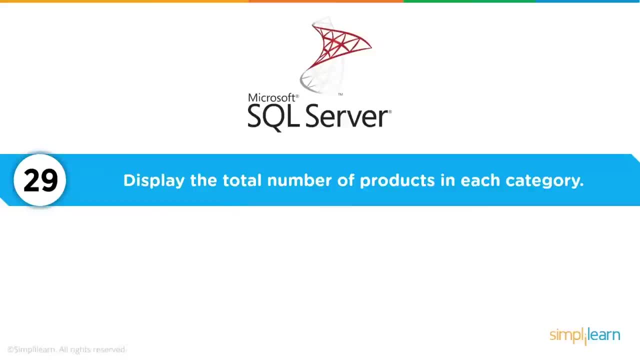 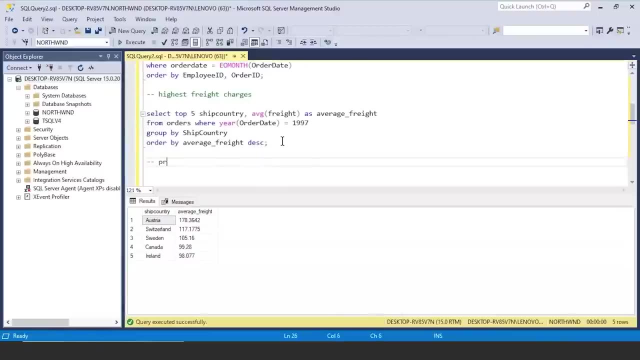 That is, to display the total number of products in each category. First let me give my comment. to display the total number of products in each category, I'll just write: print total products. Okay, So to solve this problem, We are going to use our two tables. 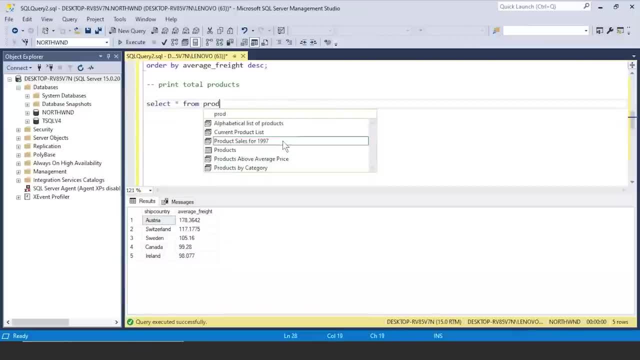 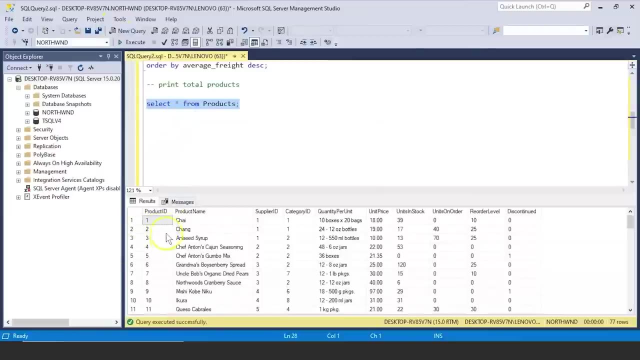 So let me first display the rows and columns from both the tables. The first table is products. Okay, It is products. Let's run this and see the columns that we have in this table. Okay, So you have the product ID, which is the primary key. 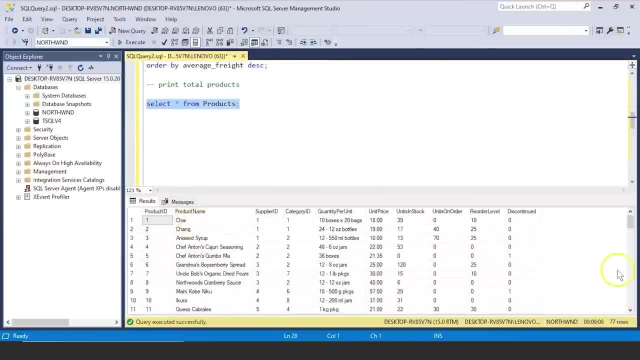 You have the product name, So there are total 77 different products. Okay, Then you have the supplier ID. You have the category ID, So these two columns are the foreign key columns. You have the quantity per unit unit. price units in stock, units in order. 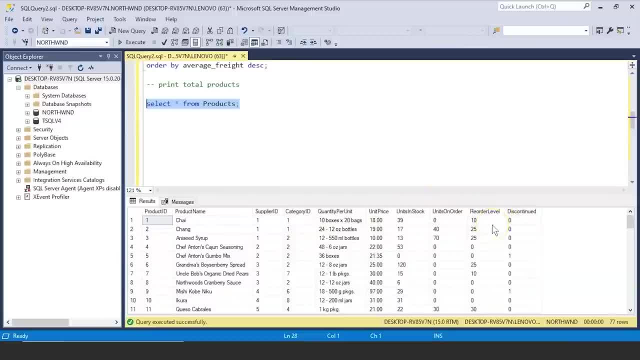 And if you want to reorder some product to fill in the stocks, So you have information for that as well, And if the product has been discontinued or not. I'll copy this and let's see what rows and columns we have in my categories table. 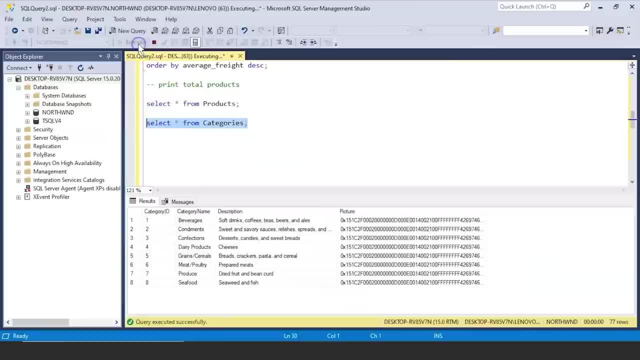 Okay, Let me execute this. Okay, So we have total eight categories of products. You can see beverages. We have dairy products, meat or poultry. You have produce seafood. These are the description. Okay, Now to find the total number of products in each category, I'll write my query as select. 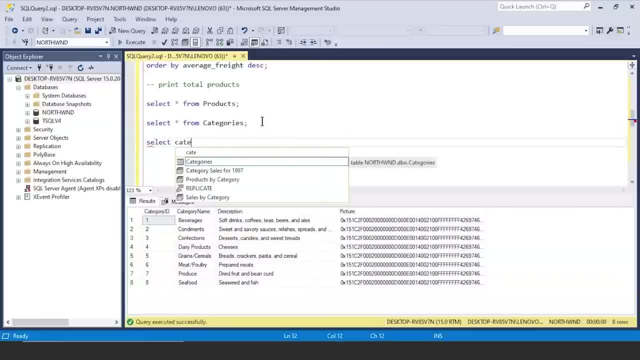 I'll write category name, comma, count star. I'll give this an alias name as total products given underscore and write products from my first table, that is, products given alias as p. I'm going to use an inner join with my categories table and I'll give my alias as c. 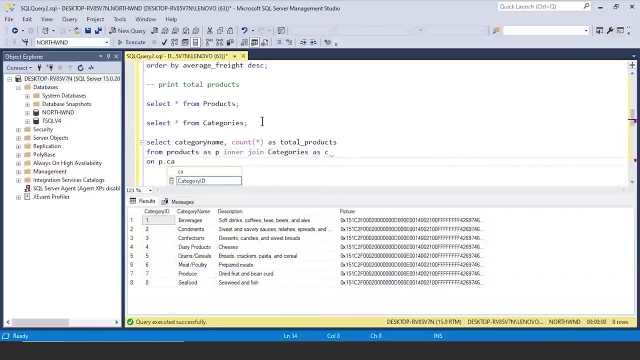 on my common key column, that is p dot category id is equal to c dot category id, then I'm going to group my results based on the category names, so I'll write category name and we'll use the order by clause. I'll write order by count, star as descending. so 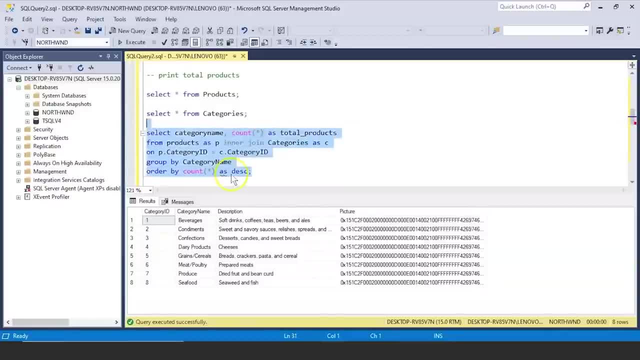 let's see the total number of products that we have in each category. so this shouldn't be as descending, should be just count star descending. okay, I'll select and run it the user name and I'll give this an alias name, as c dot category id is equal to c dot category. 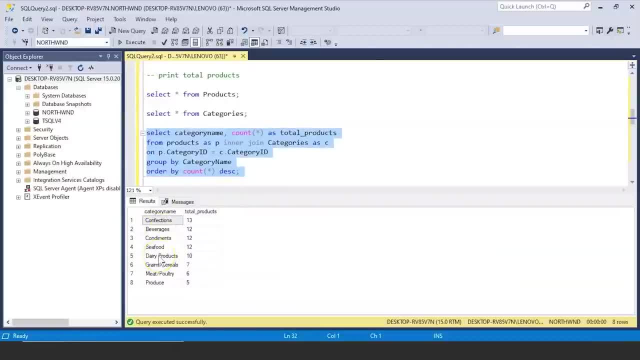 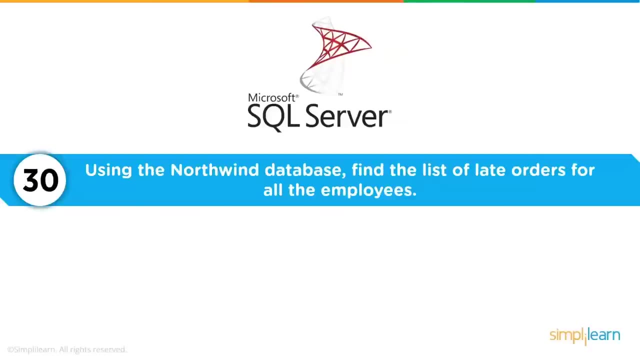 id. so here, on the left hand side, you have the different category names and on the right you have the total number of products that belong to each of the categories. all right now, moving on to the final question. so the last question is to use the Northwind database and using this, 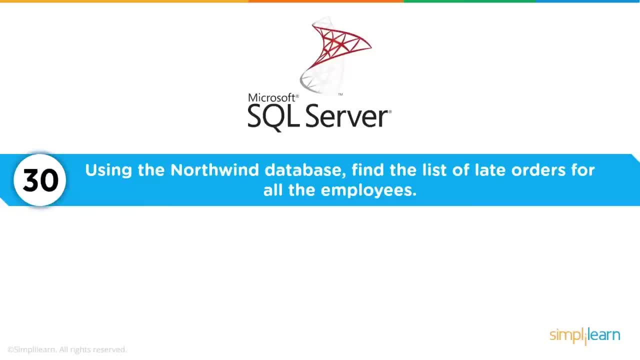 database. we want to find the list of late orders for all the employees. so this is a real-world problem that often occurs, so the shipment of your orders might get delayed due to logistic issues or if the products are not available on time. there can be various other. 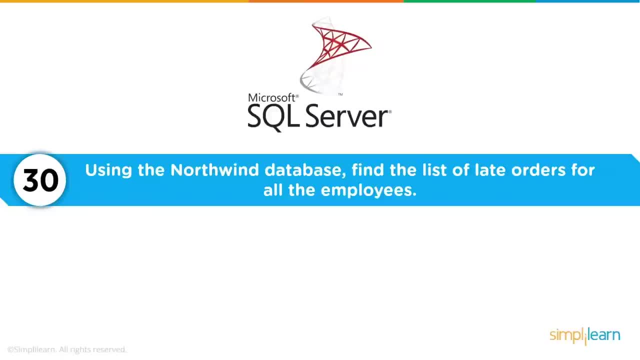 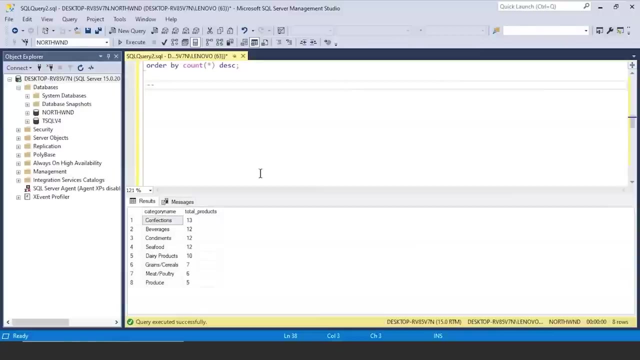 reasons as well. so here we want to find those orders for the employees or where the required date is less than the shipment date. we are going to use two different tables, that is, orders and employees. okay, now let me give my comment for the final query, that we are 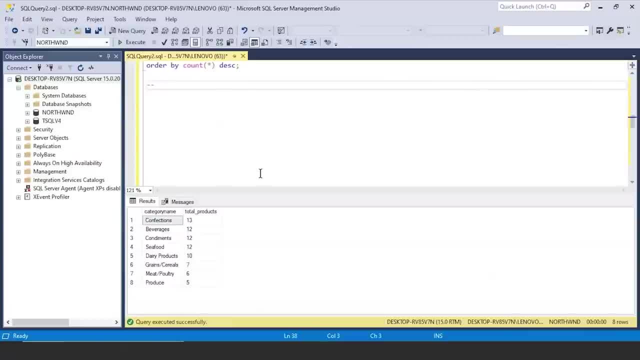 going to write in this interview questions tutorial. so, using the orders table, I want to find the list of orders for all the employees. so I'll just give list of late orders, not just orders for employees. I write emps, which stands for employees. so here I'm going to use two tables: orders and employees. orders table. we. 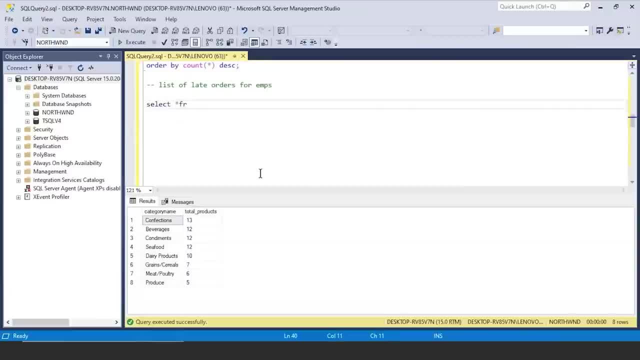 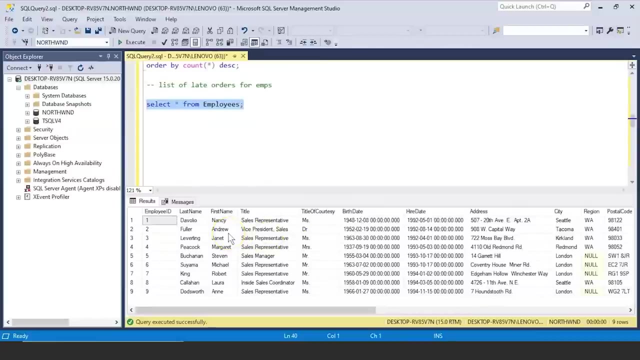 have already seen. let's see the rows and columns that are present in the employees table. I'll write select star from employees and let me run it. okay, so there are total nine employees we have. so we have the employee ID. this is the primary key column, which goes from one to nine. we have 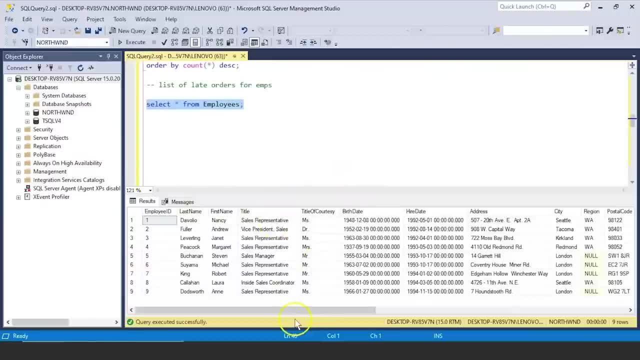 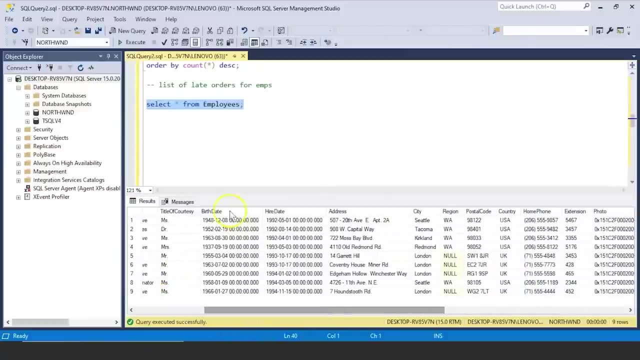 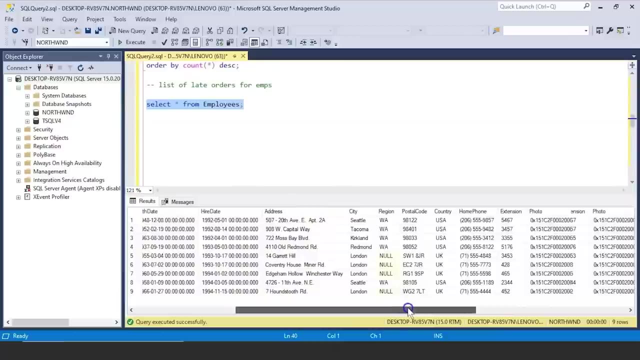 the last name of the employee, the first name of the employee, we have the title, then we have the title of courtesy, whether doctor, Mr, Mrs. we have the birthday of the employee, the higher date or the date of joint. you have the address, city, region, postal code and other information. all right, so let's see how you can. 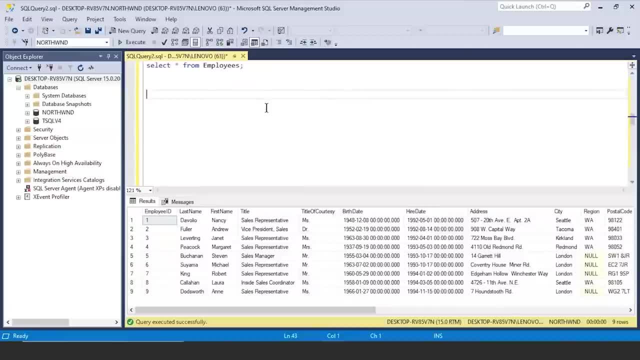 join the orders table and the employees table to get the list of late orders. and we must remember that late orders are those where the required date is less than equal to the shipped date. so I'll start with select E dot. I'll write employee ID comma. I want the first name. 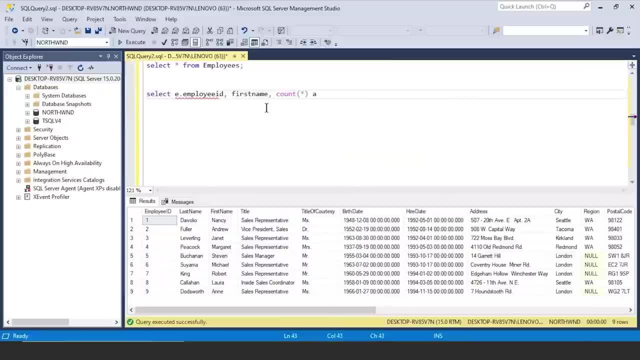 comma. I'm going to count star as late orders from my table. orders as O, then I'll use my inner join. I'll write employees as E. it doesn't matter actually, if you use small E or capital E, then I'm going to use my on condition on E dot. on E dot employee ID equal to O dot employee ID. 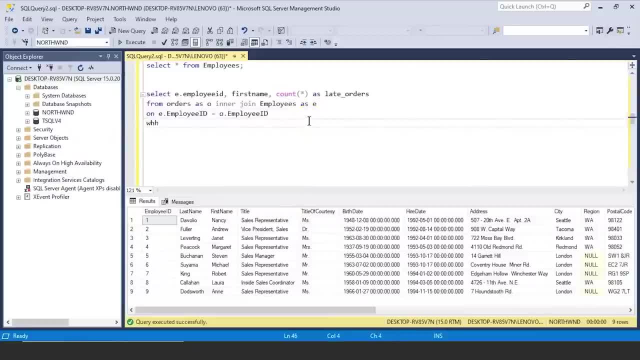 so this is my common key column that is present in both the tables. then I'll use my where clause, where you should be careful and you should give the right clause. so my required date should be less than or equal to my ship date. so this is my condition and then I am going to group by E dot employee ID comma: E dot employee ID.